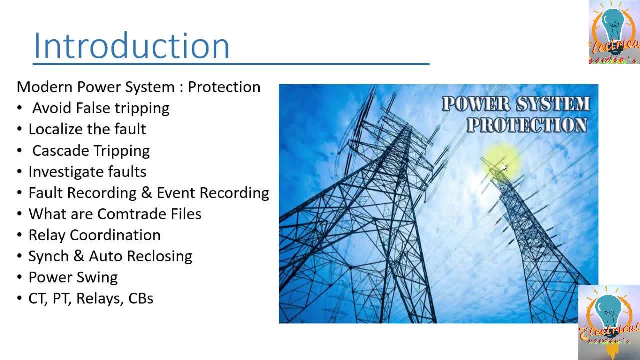 coordination and power system production is really important because if you misunderstood the power system production, then the result will be false tripping because of wrong settings, false tripping because of wrong interlock diagrams or less adequate interlocks available in a system. so you can calculate the cost of single tripping which resulted in. 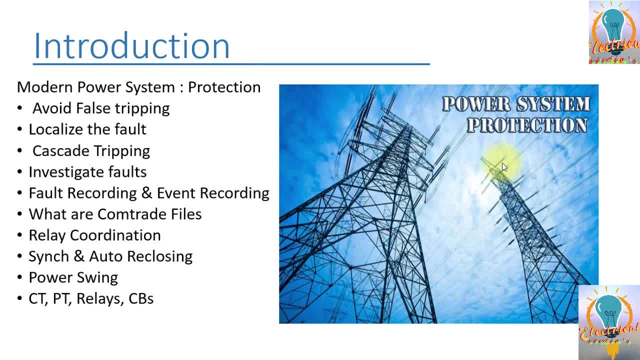 cascade tripping and which resulted in holes, country blackout for 12 to 24 hours, so you can calculate the cost by yourself. whole industry is off, all the hospitals are off and all the power plants are off. so this is a huge loss and also the reliability issue. any investor- if you want to come and invest in a country, he 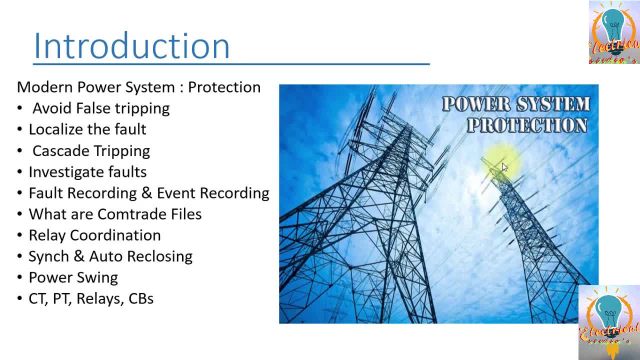 will be susceptible that the power network is not healthy, so how I can invest and how I can meet the deadlines. so we need to avoid the false tripping, false trippings: one is a real tripping, another one is a false tripping. variable tripping is because of fault. 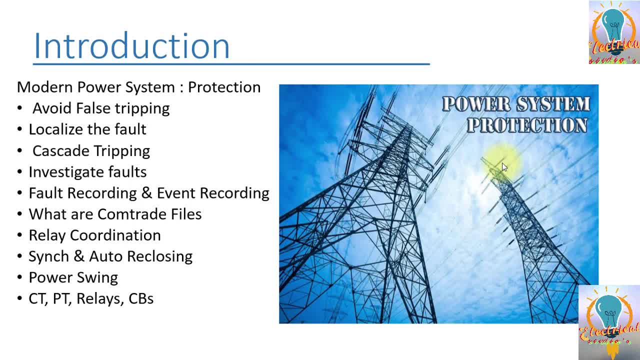 false tripping is because of fault, because of wrong settings or because of malfunction of the relay. so we need to test the relay. that's why there is always annual testing, routine testing. there is a. we need to keep on testing and check the system. second thing is: 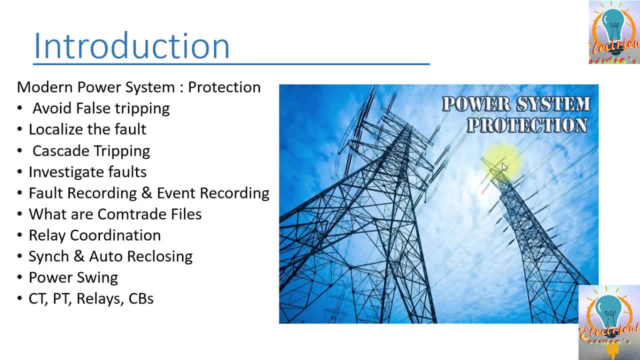 localizing the fault. so if and a part of the network has a fault, even though it's a three-phase short circuit, only that part for them will. if a line is dead short, if somebody has forget to remove the portable temporary grounds from the line there, I will tell you one interesting thing that used to happen in 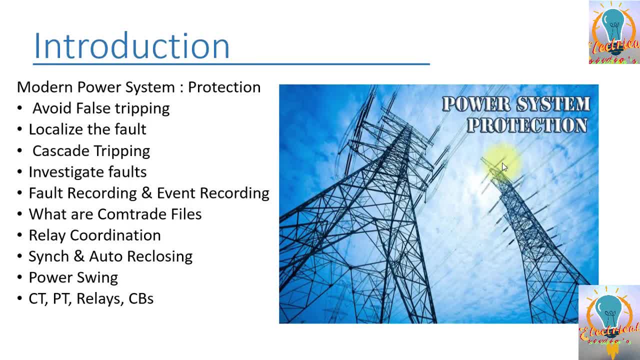 the past if somebody installed a portable ground. because portable ground is just like connecting copper wires to the conductor of transmission line and to the ground, so there is no interlock in it and nobody can monitor it unless that person who has taken the permit. he knows if somebody else came, he cannot check even. 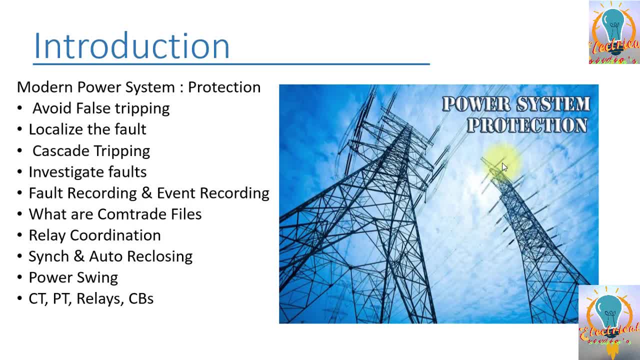 the operator is, there is no interlocking, there is no indication, it cannot monitor it. so it used to happen. nowadays also there is a chance then when a person is trying to close the line, he will check all everything. he will make a visual inspection first of all. normally, 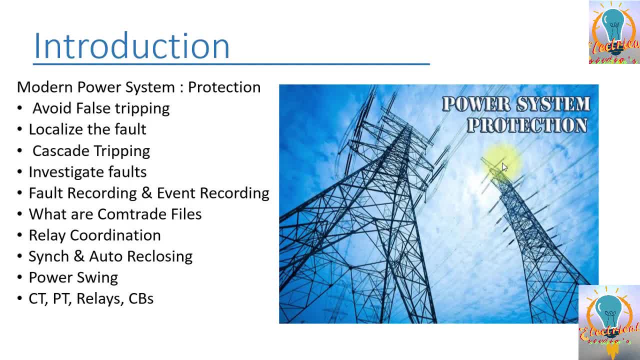 what is required is before, after you finish of all of your permit. if you cancel it, then you have to go to the site- you should make a visual inspection always- and then you can go back and issue your permit. then you can go back and continue the process of another addition. so in case of portable temporary 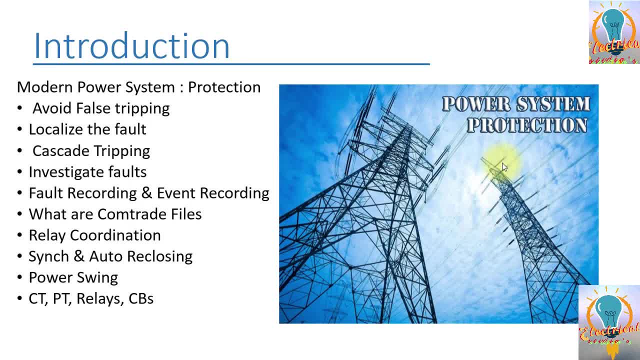 ground. as soon as you can close the breaker, there is a fault, there is an already built-in fault, it's. this fault also has a very special name. it's called a switch on to fault and it's, in other words, we can say: as it is a SOTF, the other name of this fault is a bolted fault. so it's, you can say it's a. 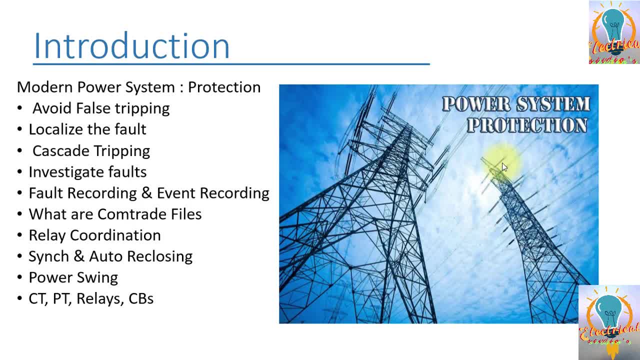 very heavy short circuit because it's a dead short using three wires and if you have, if you know that three-phase short circuit has the highest level of short circuit current, it can feed highest level short circuit current in the network as compare to single-phase ground or two-phase ground faults. so 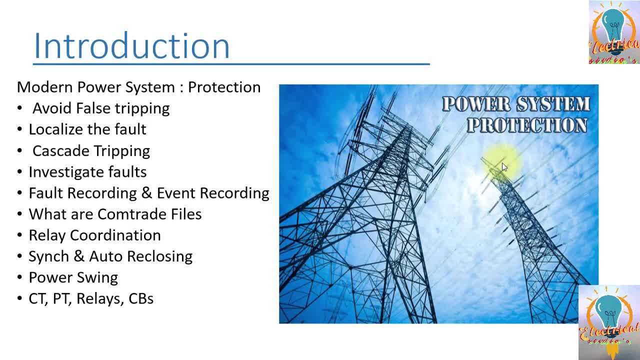 then this is example of switch on to fault- and each protection relay, especially in the distance and also in over current, which is protecting the line they have. that's why they haven't to use a separate function which is called a switch on to fault function. so whenever the breaker is close, at that instant. 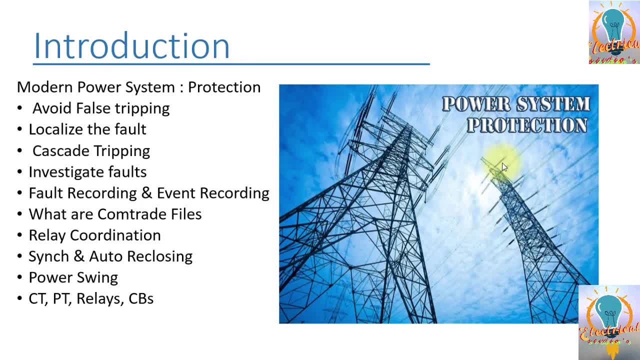 this function is switched on, faulted only 200 milliseconds, or 300 milliseconds enough that it is disabled. so what the relay is doing, it is setting its priority to check. switch on to fault first, because it's these are. these are these days. we have numerical relays and 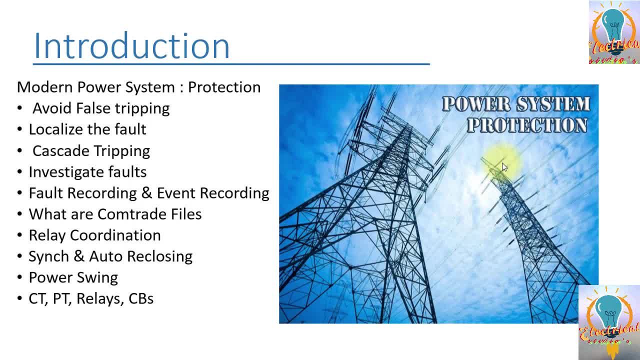 you have. you have done the programming. you know that the program is executed line by line. so the part the relay is doing, it is calculating the voltages and grants and then it's executing the code checking what pages under limit card is an under limit, impedance under limit, one by one is checking all the conditions. 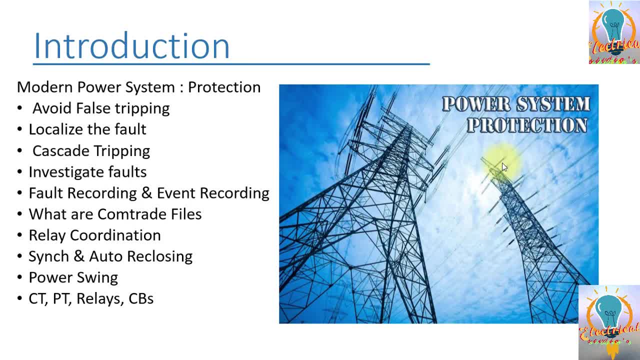 and it is in the loop always. but and it mean that we can give priority here to give certain types of faults. we can give priority that first you need to check, for example, distance protection, zone one, then you need to check zone two, then you can tell you can check. 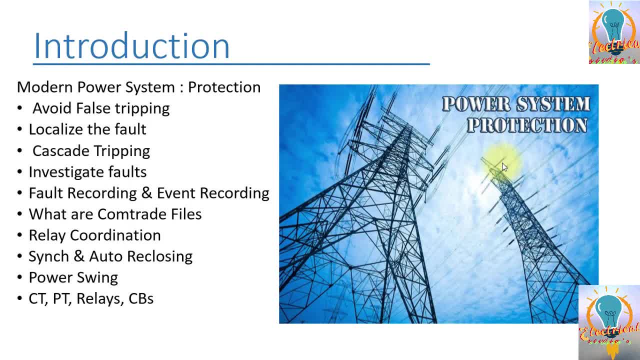 okay, earth fault over current backup. so you can, depending upon your priority, there will be a. you can save few milliseconds, which is really important for big networks. so if a person switching it on the network on a fault, then it's a severe steep, a short circuit fault, so that fault should what should? 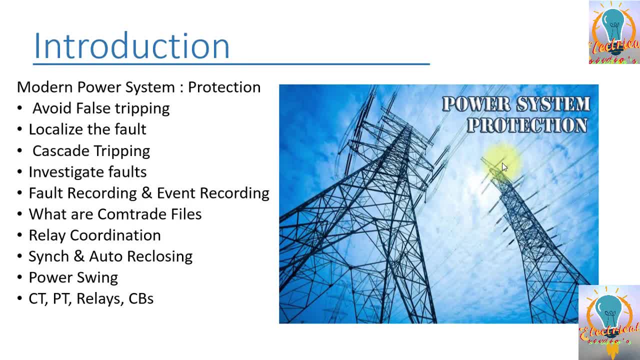 happen technically that that only line can be set to that location and that only line can be set to that location and that only line can be set to that location and that only line can be set to that location should be tripped. but what has? I have told you example already that the 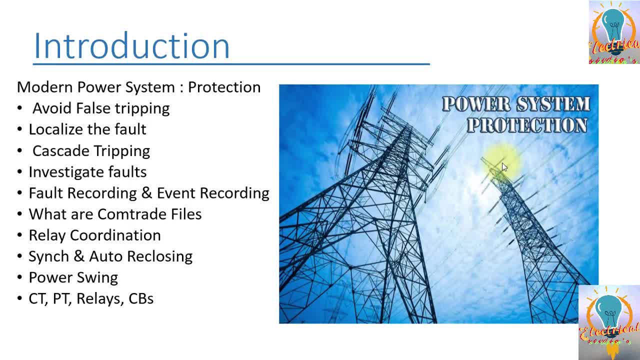 similar fault happened and it resulted in tripping of for the country. also, I have experience in Saudi Arabia, where we have similar type of a fault: earth fault to ground. the line was breaker, was closed to a solidly connected earth and it was a new substation. it was under commissioning and by mistake, this 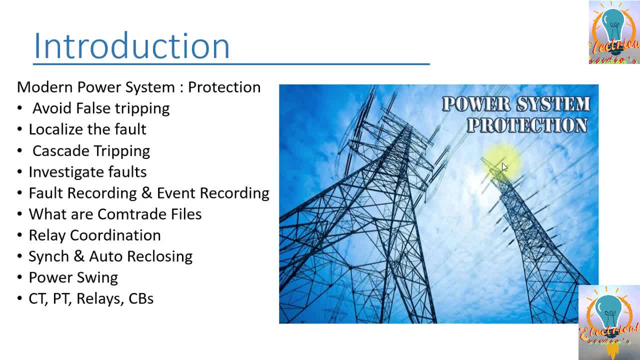 interlocking was not working and they closed the breaker and was closed until there was no interlocking and the result was whole: the region was blackout for few hours. so this is very common. so what happened? if you are switching on to a fault, switch on to fault in this condition, and if the relay did not work? 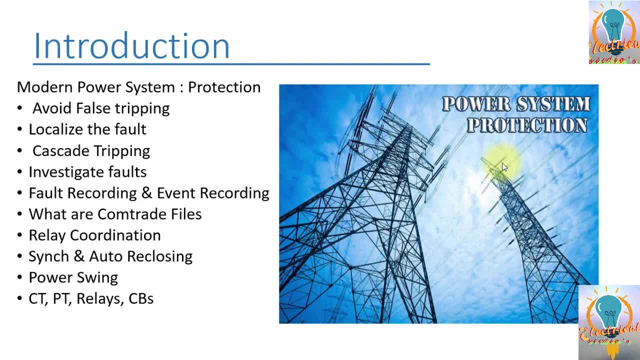 or it it is working delayed. I there, there is in the network a. there are always two things: or there is basically sources which are supplying the power and there is a load also. so we are keeping generations and we are keeping balance between generation and we are also keeping balance between load. 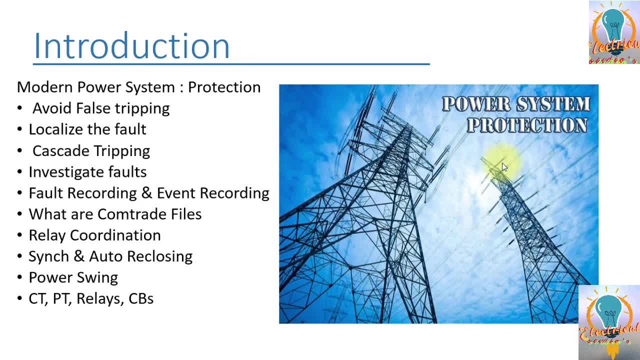 and also there is another thing that I will tell you is basically spinning reserves. so we are keeping some generators and we are keeping them on and they are rotor or turbine is spinning. whenever there is a change in the generation, you can immediately take the power from the spinning turbines. 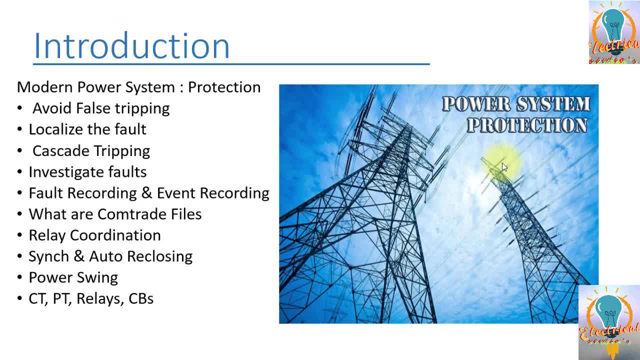 these are called spinning reserves of the network. so what happened that? if the line was, if the line flows on the earth, three-phase earth is already connected to the machine. this is the output of the power that is being treated at the path, at the path in terms of the current. so what will happen? that the line should? 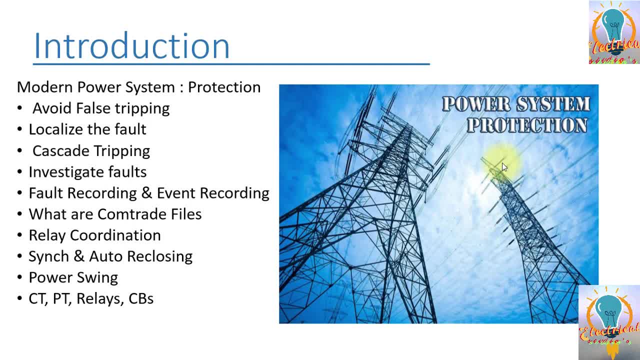 trip. there is a delay, tripping in the line and that resulted in tripping of a power plant nearby power plant because power plant could not sustain that much short-circuit levels. there is under put under over current production, there is out of step production, so these productions operated and it tripped the generation. so 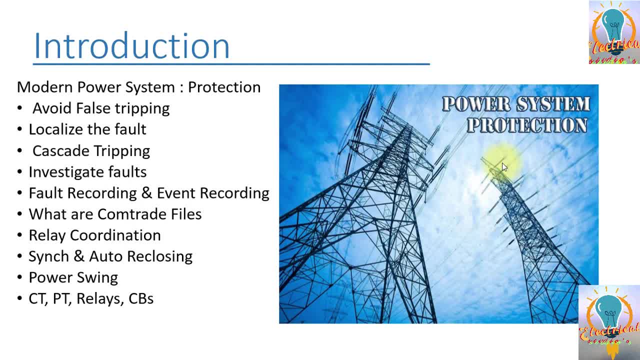 fault is not clear. so now also, the spinning reserve in the network was not not enough. so when one generators goes down, fault is still available. now the load is more and the generation of the network is less, because we are not keeping enough spinning reserves also. so the next generator trips, and after some 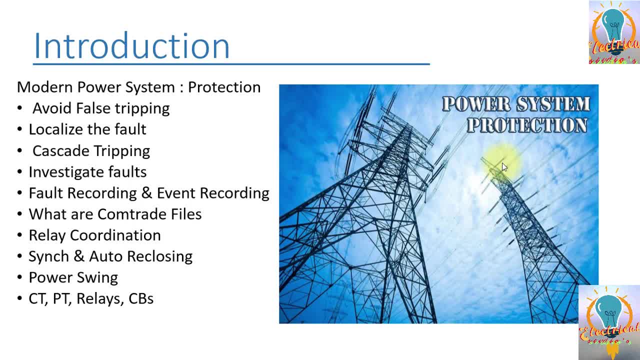 time hold the network trip. so this, this is called also a cascade trapping. so this could happen: that if you have a load, if you have one thousand megawatt of megawatt of load and we have one thousand megawatt of generation and you are not keeping any spinning reserves with you, if one of the line trips which 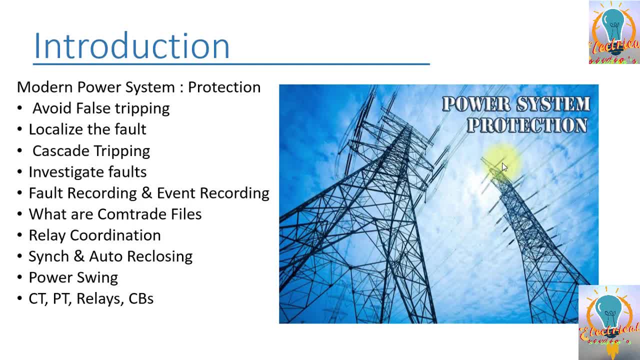 is applying for double 200 megawatts, then there is a sudden decrease in generation of 200 megawatts versus one thousand megawatts of load you. so now you don't have any spinning reserves with you. so what will happen? that further generators will trip and it might result in cascade tripping. so 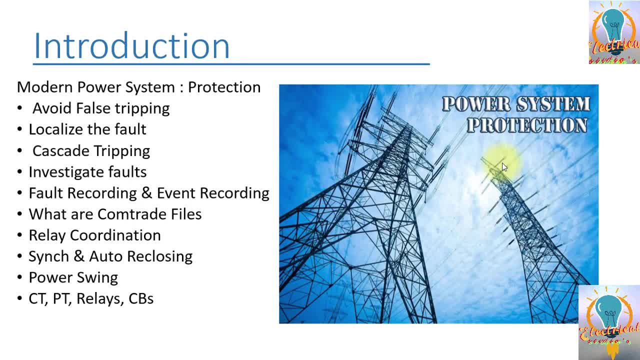 that's why it's very important to have a good protection coordination, good under frequency scheme installed and you should have proper coordinated settings: which area should trip first and which area should trip afterwards. so whenever the fault happened there comes always investigation. so you need to investigate the fault. welcome friends in. 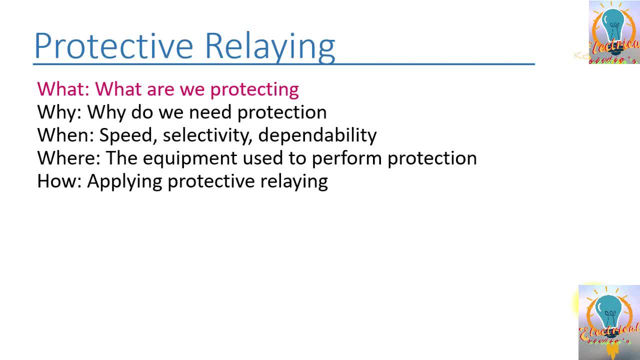 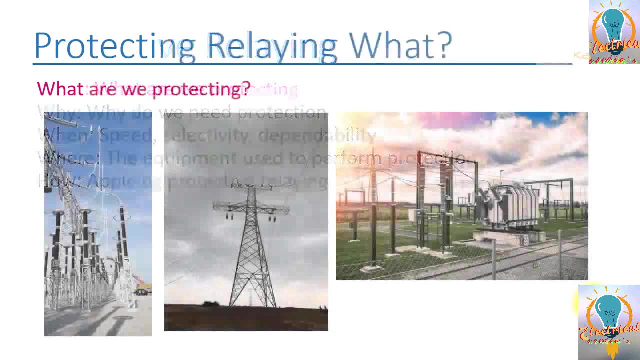 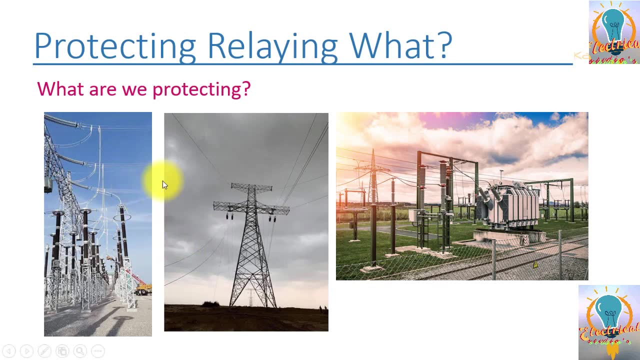 this section we will discuss that, what we we have to protect in a power system. so let's start. so in a power system, we have a different components. we have substations, we have transmission line, we have transformers, we have the knitting stations, we have a cat deixons for each separately to lash each other down the chain. see you in my como mesa. 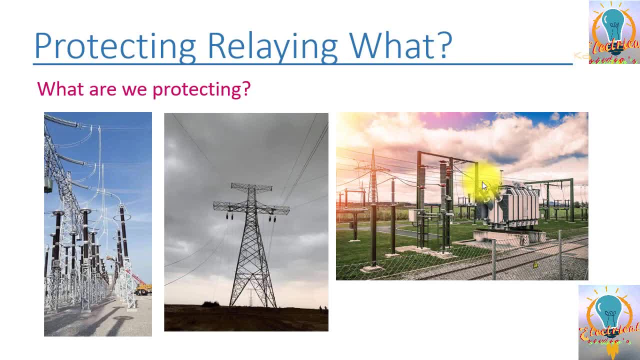 have justice. CT prior than the main body point, as indicated. we are not salt cats like us, as you think. These are the those air currents that you should follow. have solar system. we have a lot of equipments which is installed, so power system protection, it will. what is the purpose is that it has to. it cannot prevent the fault, protection cannot. 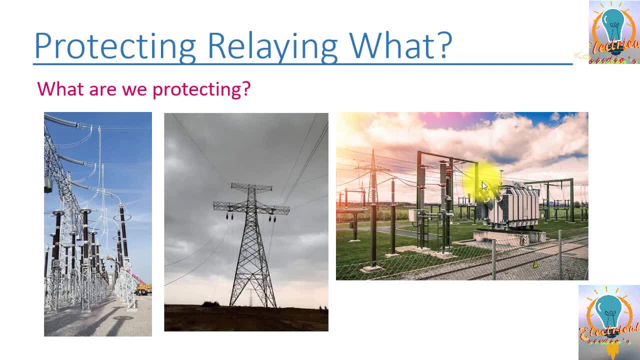 prevent the fault, but it can reduce the severity of the fault. it can reduce the, basically the damage to the equipment or to the network as minimum as possible. it can reduce. it cannot prevent the outages, but it can reduce the duration of outages as minimum as possible. so the basic concept of 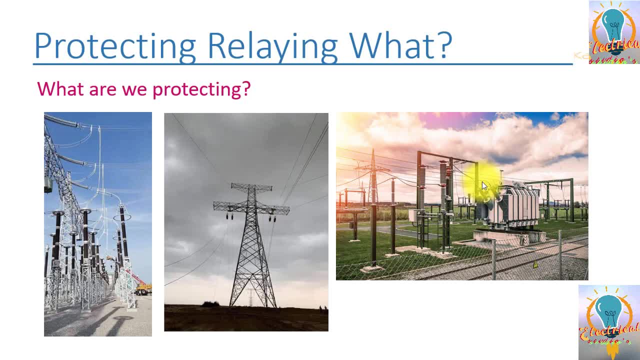 power system. protection is not only to trip and the fault occur, but it has to take care, all of these things that interruption should be. there should be no interruption. if there is an interruption, it should be as minimum as possible. there should be no damage to the equipment. but if there is a fault and the damage should be as 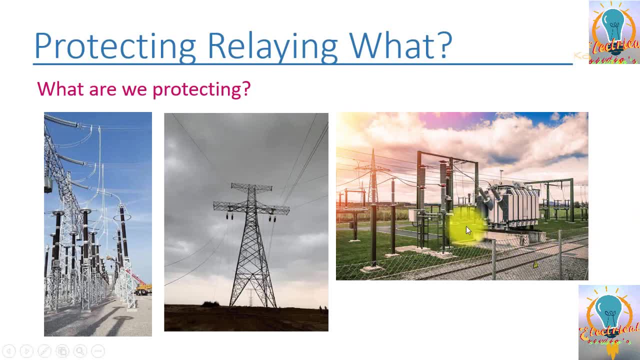 minimum as possible, for example, in the transformer. if you see the example of the production here, the buckles really is installed here in it and this really is basically monitoring. if there is any gas is available in the transformer, these are trapped in this. first of all, it will give alarm. 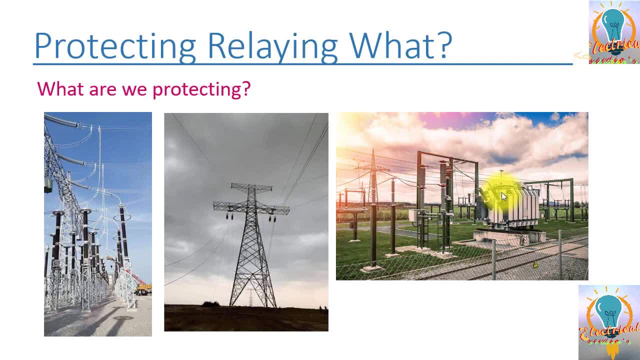 and if the alarm is not basically appearing, if alarm is not clear, the gas is further increase. it will give issue the trip. so in this way we are monitoring the transformer and instead of having a complete fire in the transformer, we are fire. we are. we can in this way monitor a small spark or small fault in which is 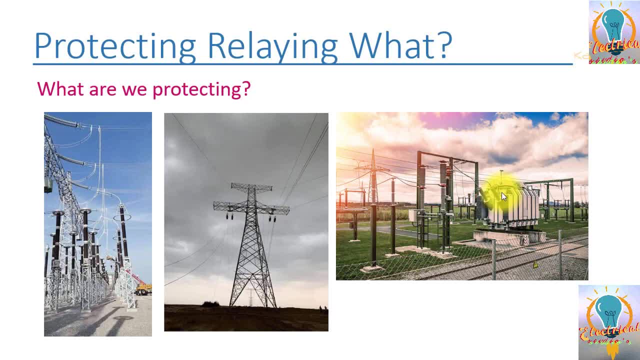 still developing into a big fault. we can monitor it and if the alarms is coming, then we have to take the shutdown on the complete transformer and we have to do the testing and try to find out what is a for real the fault. in this way, for example, in this way, we are minimizing the fault on the transformer. another: 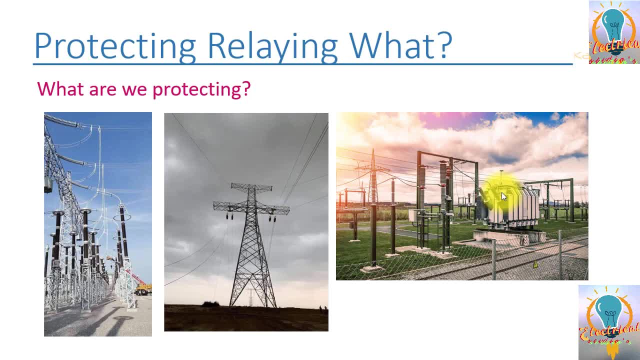 example of monitoring the fault and when is I minimize, minimizing the damages? we have installed here temperature, winding temperature and oil temperature indicators. so we are continuously monitoring the temperature of winding and the oil and if beyond certain limit alarm and in also possible, the tripping is initiated. so instead that the 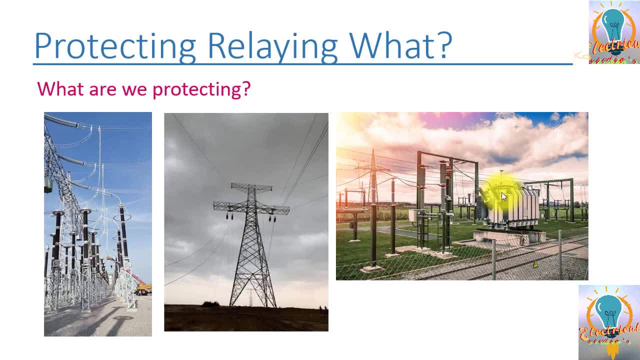 transformer winding is keep on heating up and then finally there is a fault and start burning. we are just tripping it before before and we are limiting the fault and limiting the fault. so these are some examples. basically, the idea is that we are protecting all our equipments using these relays and we 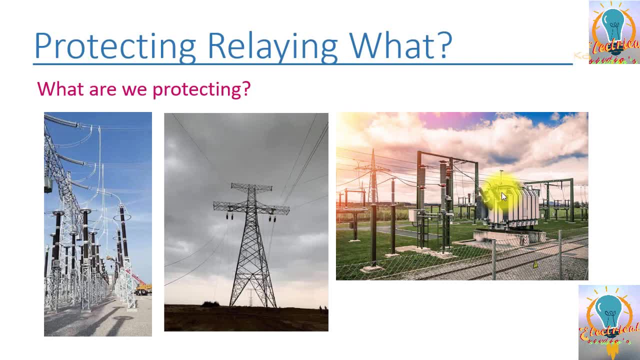 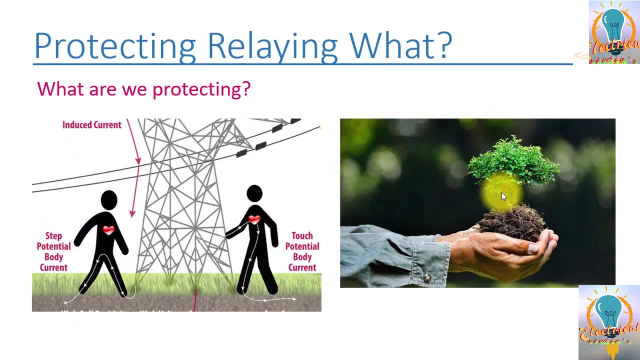 were. the aim is to have a better selectivity and isolate the faulty portion only in case of fault. so this is an example of we are protecting to protect the equipments. so another relaying, a production ideology also in this relay coordination, relay studies and short-circuit studies. 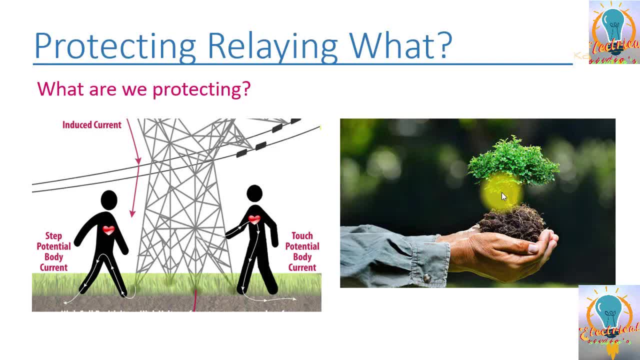 we are doing the calculations of, we are taking care of human safety also, because humans has to work in substation on or the transmission lines. so we have to take care about the humans. so in this specific sheet you can see there is a calculation in which we have to calculate the as per design substation or the transmission line. what 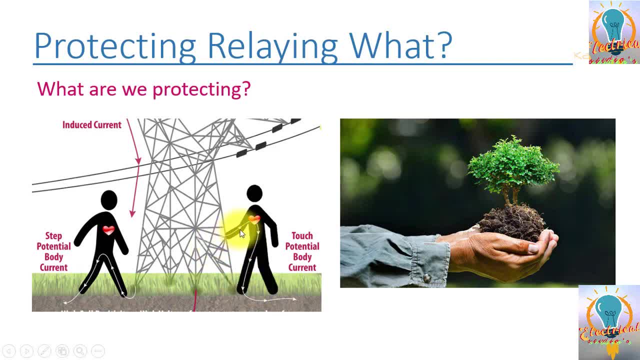 is a step potential and what is a touch. potential is what somebody is touching the tower and they will be when. when the conductor is is basically passing and it is energized, voltage will be there and there will be some kind of induced current. so if somebody is touching this, 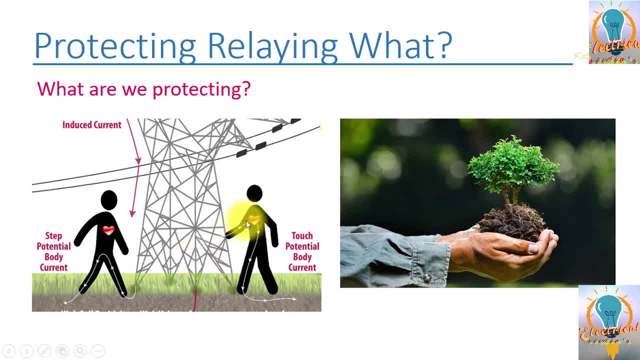 transmission line, how much current could pass through its body and if somebody is walking through near this tower, and how much could be the voltages between its two steps. so it is called a step potential because of because when there is a fault, conductor will lay down and there will be a voltage gradient in it and 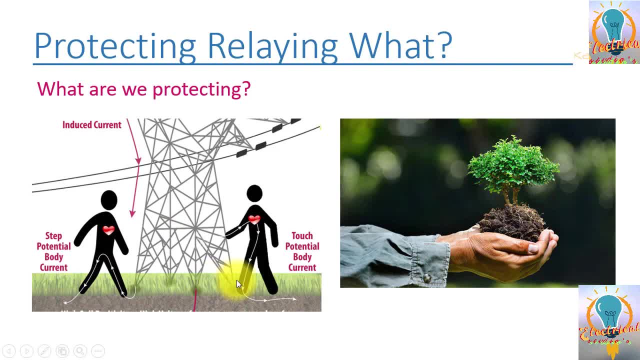 there will be some step potential which is dangerous for human. also there will be touch potential. so we have to do all these calculations. so the other perspective of production system studies is to protect the humans. so humans also, we have to take care using a protection system studies. the next thing that we 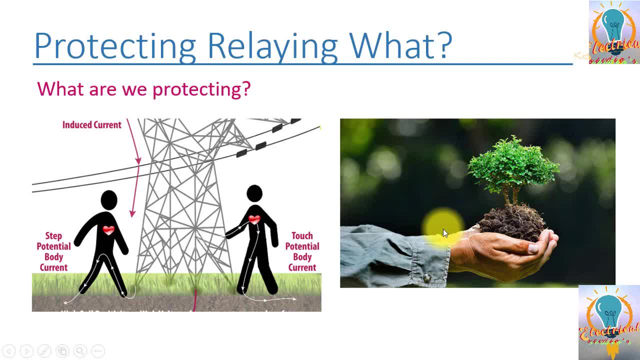 need to study is basically the environment. so what is the effect of environment and how we can improve this impact? for example, what is the impact of certain power plants and and certain substation on the environment nowadays? just an example: that if you choose, if you have to pass a transmission line to a forest, so if you 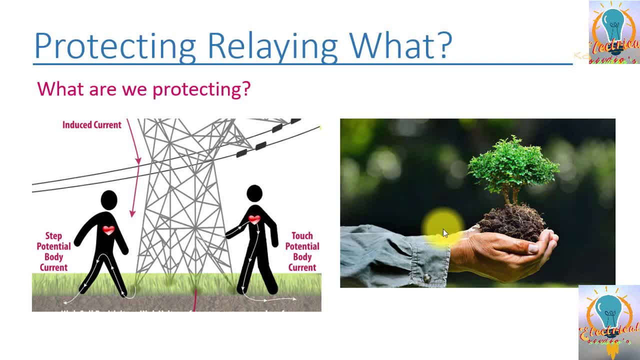 select as a study. to take this matter also, if you select an AC substation, AC transmission line, it will take, it will occupy a more area than a DC transmission, which is slimmer and smarter. So it means that you need to cut less forest and 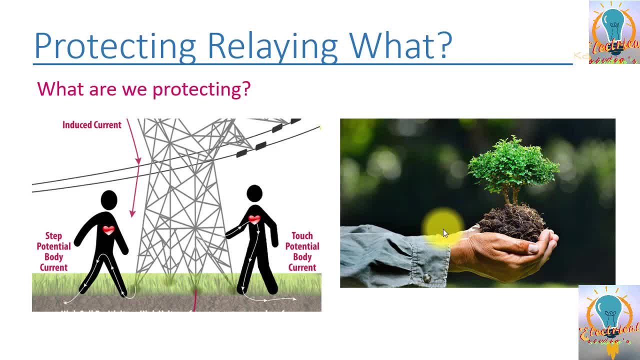 you have to take care also of this aspect when you are doing the relay coordination system studies, system design. that what is good for environment. We should take care also of our environment when we are doing power system protection studies. Now the new problem are, for example, could be in the environment. 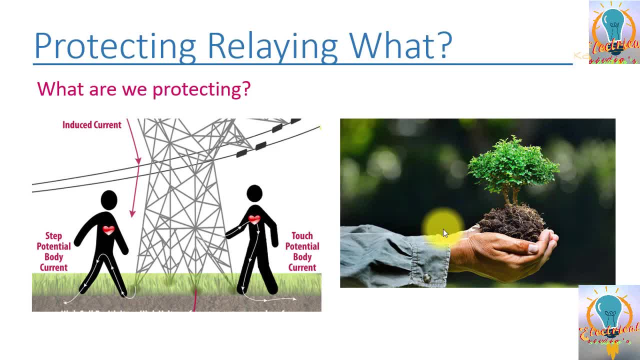 we can count it as an electromagnetic interference. So the DC transmission lines, AC transmission lines, when power flows through the electrode stations, they can cause an interference in the network which might result in disturbance of telecom signals. So this will also impact humans in some way. 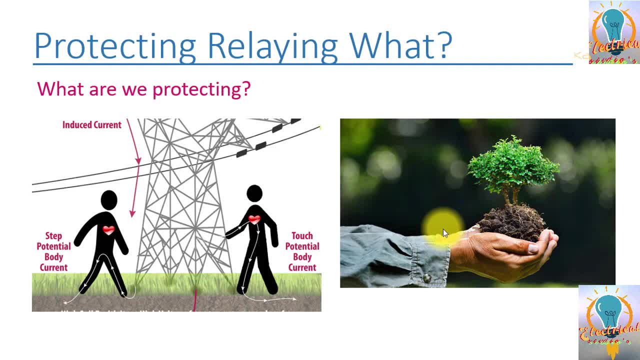 So we need to consider and design a system that should have minimum interference, should create minimum interference in the environment. So these are the factors that we need to consider. Thank you very much. Hey, friends, now in this section we will move forward and we will study. 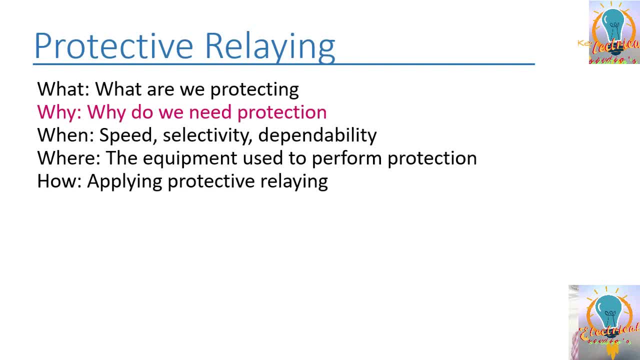 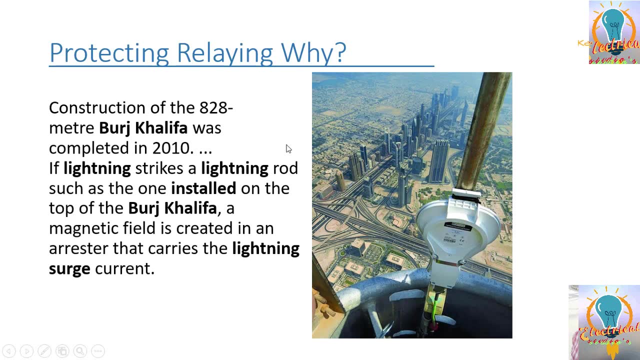 that why we do need to protect. So what will happen if we are not doing a protection in a proper way, if the relay coordination is not correct? what could happen? So protection relaying why? So I will give an example of Burj Khalifa. 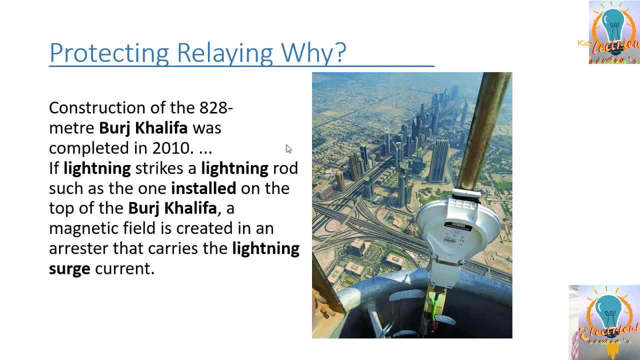 The total height of Burj Khalifa is 828 meters. It is the world tallest building And it is in Dubai. Everybody knows it. It was completed in 2010.. And on top of it you can see they have installed a lighting protection. 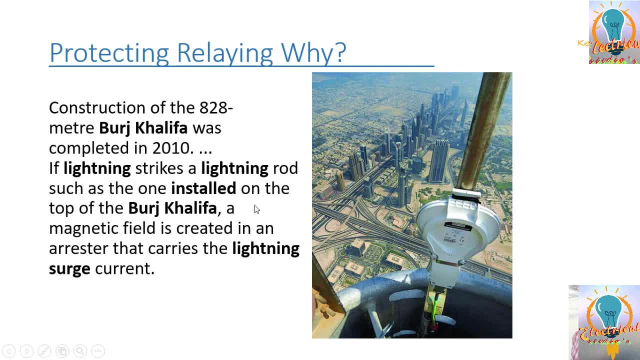 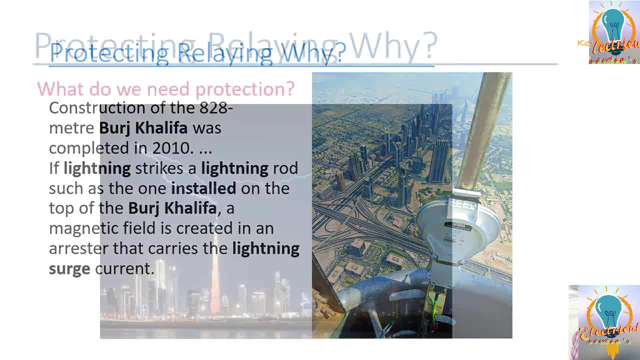 So they have installed lighting protection. If lighting strikes, so this lighting is effectively grounded to the earth, So it is protecting a light. because the building height is so high, so it is prone to lighting strokes, So they have installed a lighting protection on top of the. 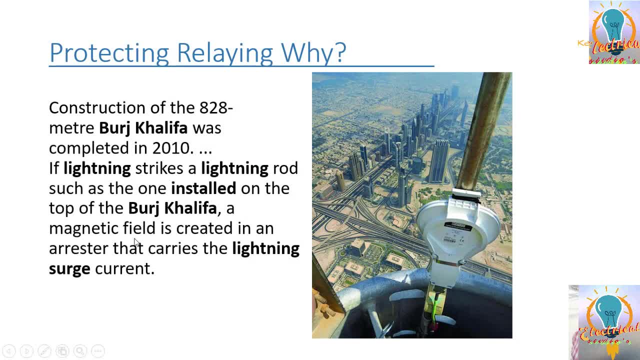 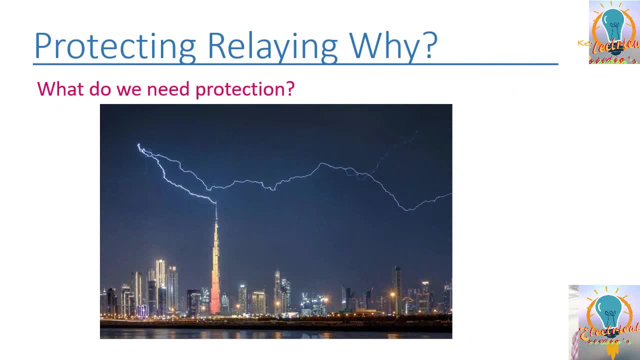 Burj Khalifa. So a magnetic field is created in a resistor that carries the lighting surge current. So in this way, when there is a lighting strike on the rod here you can see a beautiful picture of Dubai. You can see there is a certain pattern of lighting and lighting. 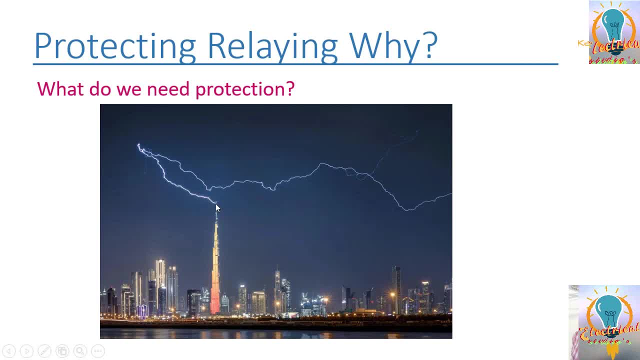 striking on top of the Burj Khalifa where they have installed this lighting protection. So if they have not installed this lighting protection, this lighting would strike and it would certainly damage this high-rise building. So you can see, we need to install the lighting protection on especially. 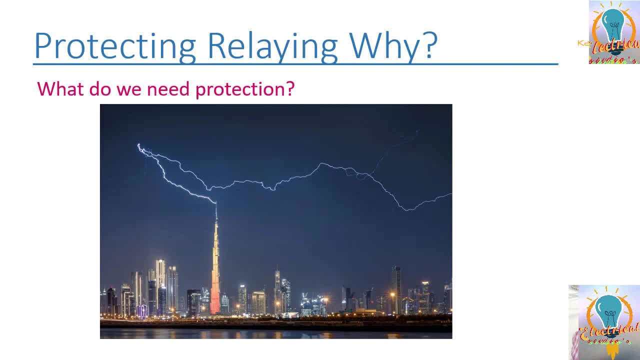 high-rise buildings, all the substations, power plants, transmission lines. If you know about these substations, they have a lighting protection installed on them. So on each transmission line there is an overhead shielding wire which is protecting the tower and transmission line from the lighting. 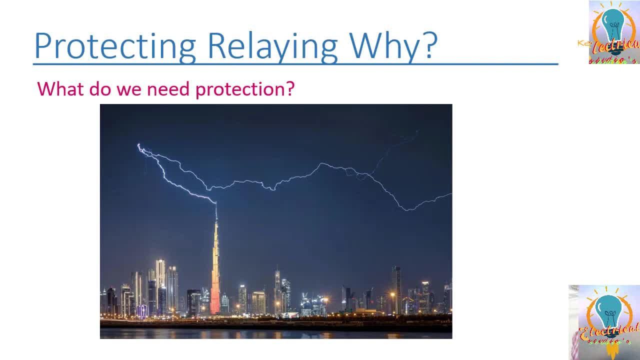 Similarly, on each substation the lighting sensors are installed in such a way that they are covering complete substation area. So lighting protection installed on everywhere in the network. So we need to provide the lighting protection on the buildings. So, similarly, lighting protection. you can see. 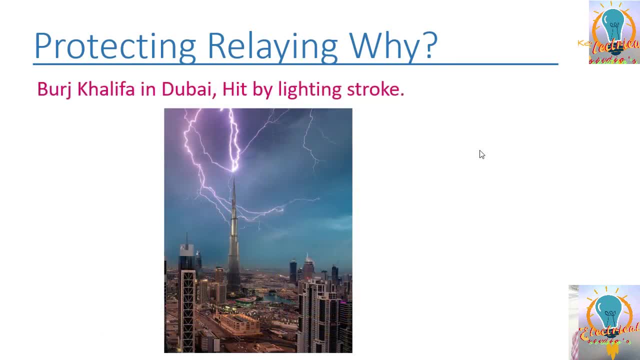 another example. So this is another very beautiful view of Burj Khalifa, where lighting is striking on the top of the building And here on this top, the lighting protection rod installed which is effectively grounding this huge electrical charge or power to the 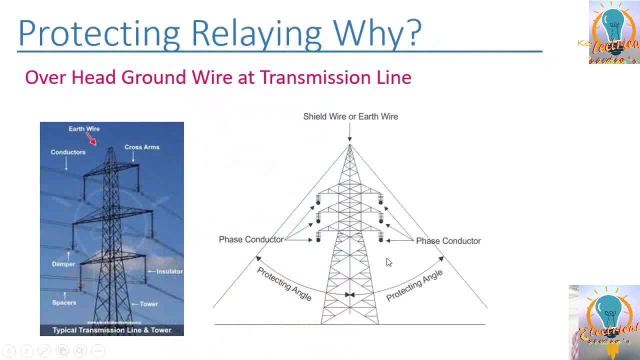 ground effectively. So here you can see in this picture you can see that there is basically a transmission line. On top of this line you can see this wire. This is called a shield wire or earth wire or overhead ground wire. You can find this wire on each. 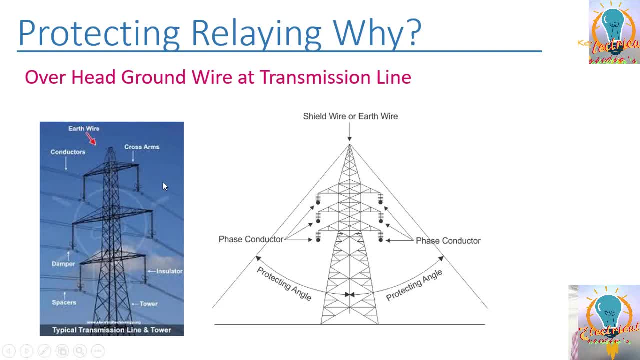 tower. So if you are passing through a transmission line, you can observe there is a wire on the top of the tower that is protecting basically the line from the lighting strokes. So here you can see the presentation of the graphical presentation diagram. So each shield wire. 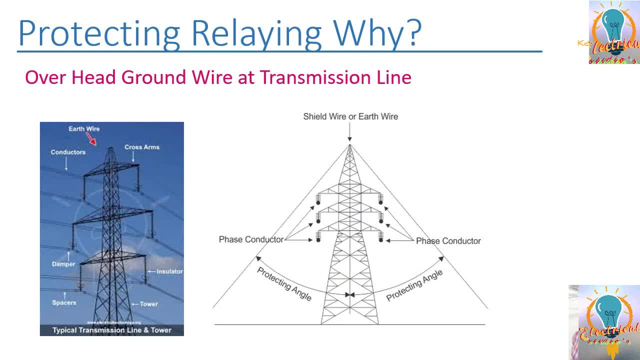 or shield rod has its own protecting angle. So when you are designing this shielding, you are calculating this angle and this angle should cover the protected object. For example, you can see now: this is the transmission line, and shield wire is not installed here directly, It is installed. 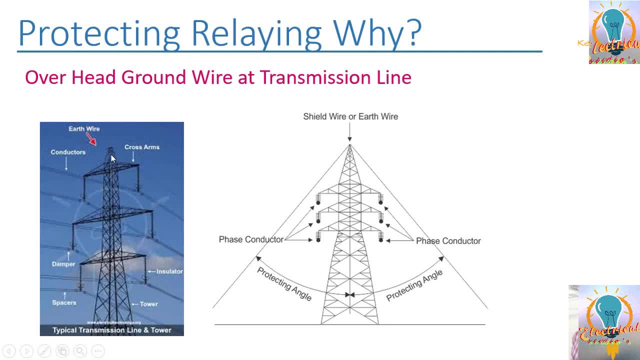 at certain height. So this height is given to cover all the wings and all the area of transmission line. If you install this line, for example this shield wire, here, not on the top, but here, For example, if I am trying to install this shield wire downside, 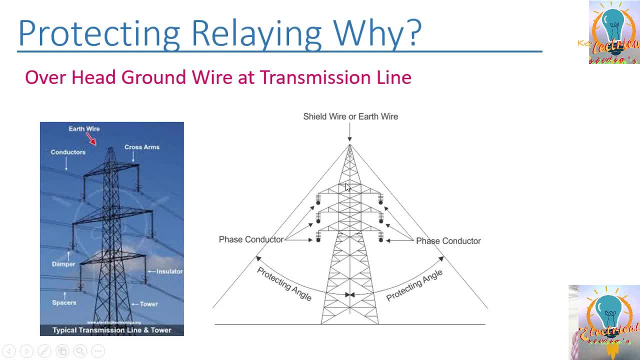 then this wings this area. if I draw this angle from here to here, for example, then this area will be unprotected. So if I am not doing this guide wire to little bit height, if I am putting my guide wire here- So I have put my guide wire here- 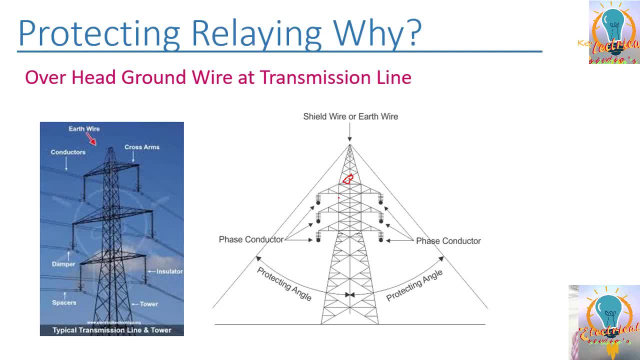 So from this point, the angle will be some kind of this to this. So it means that this area, this complete area, is now no more protected to the lighting. So my angle is: this is my protection angle. So if I want to cover this area, 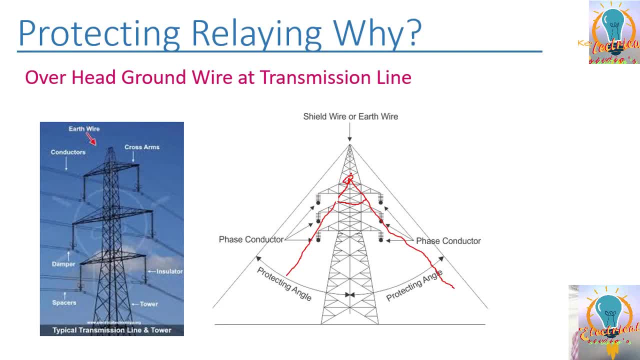 then I have to increase the height of ground wire to the certain level, For example. here I have taken this new point. Now I have done the calculations and I have now covered the complete tower plus I have some margin of error. This much is my margin, margin of safety. 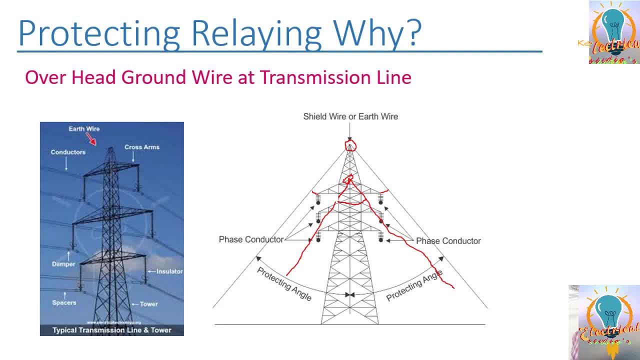 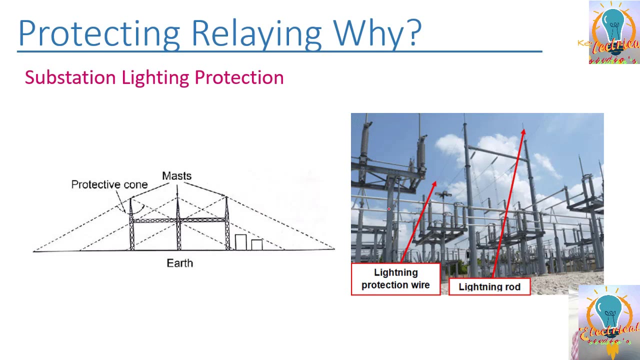 So that's why I have taken the ground wire little bit higher and then I have covered this Basically. this is just some introduction about the ground wire, how ground wire works. So this is another example Here. you can see that this is basically the overhead ground wire. You can see and 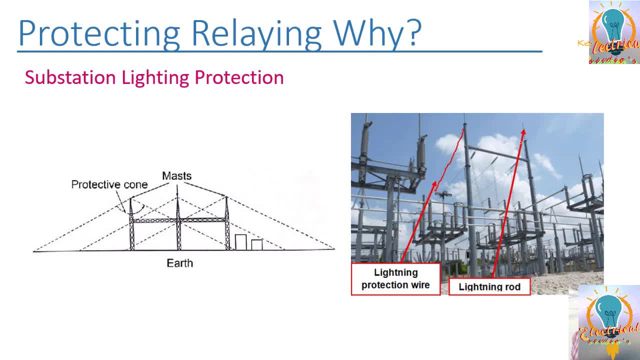 this is basically the lighting raster rod. So in the substation you will find lighting raster rod and also the shield wire. Both are combined to protect the substation from lighting strokes. So this is example of lighting. This is just. I am briefing, So 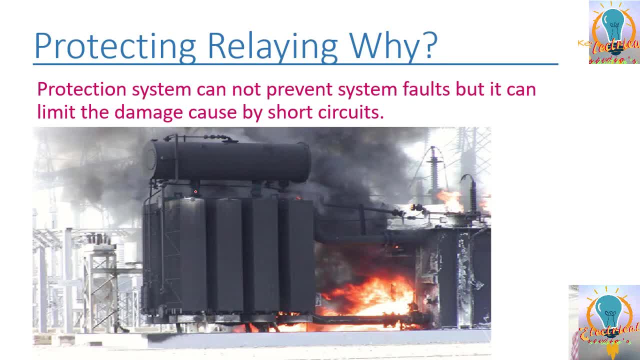 this is an example. You can see there is a fire in the transformer. So we need to have good protection. if you want to limit the faults, If you want to eliminate the faults, you need to have protection. If protection is not properly working, result could be like this: that 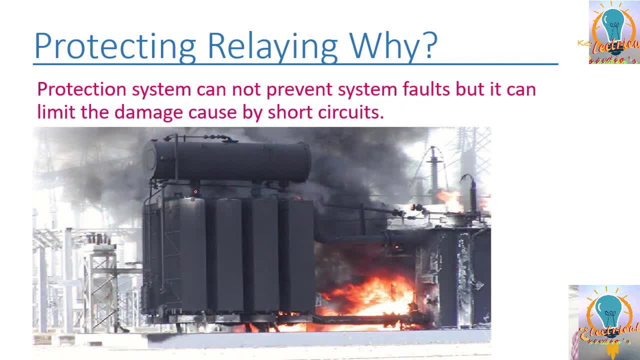 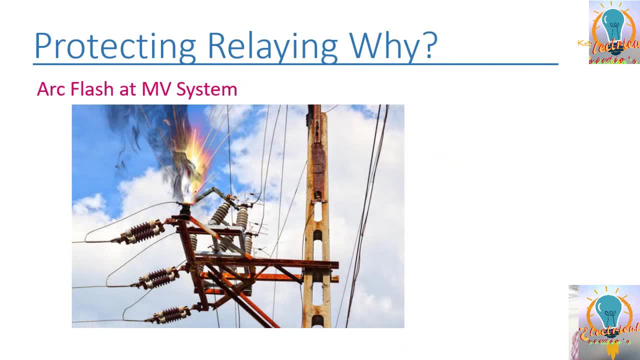 the equipment can damage And this damage can cause by short circuit, by overheating, by flash hours. You can see there is a flash over, So the system is not all the time smooth. System is dynamic and it is subject to environmental conditions, ambient temperature. 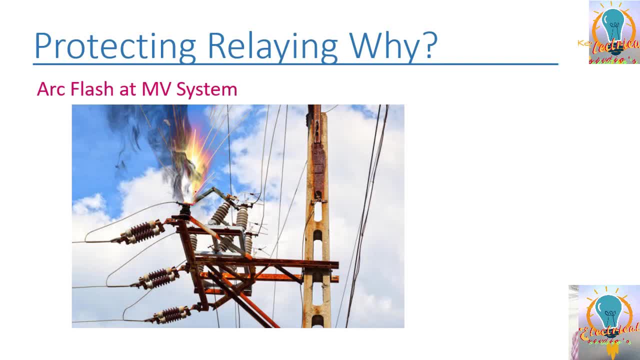 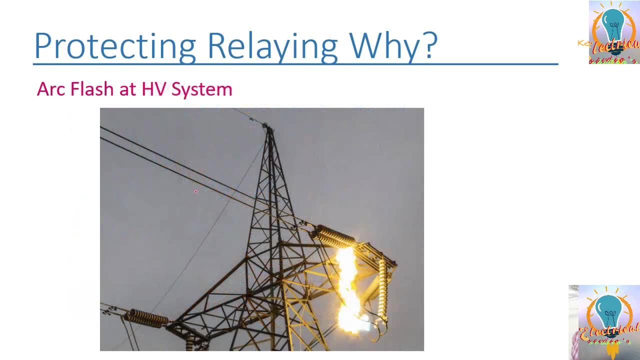 flash overs: moisture, humidity, loading conditions, voltage stresses, lighting stresses. So these all things it has to be. That's why we need to have protection Here. you can see there is a flash over on the MV system. There is a flash over here. 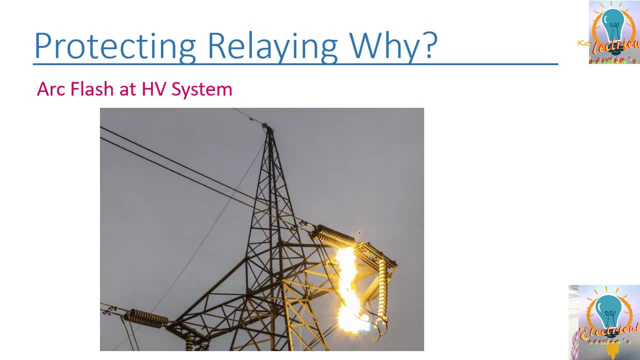 This is basically the disc of the transmission line. It is called a disc insulator and you can see this is the shield wire And here you can see this are basically called as a damper. These are dampers because in transmission line, due to 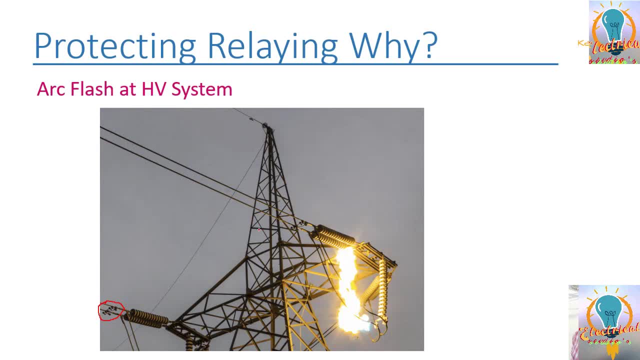 air, there is a vibration in the line. So in order to damp the vibration and protect the structure, so these dampers are installed And here you can see there is a flash over And it means that here the conductor is grounded through arc. Arc has a low impedance. 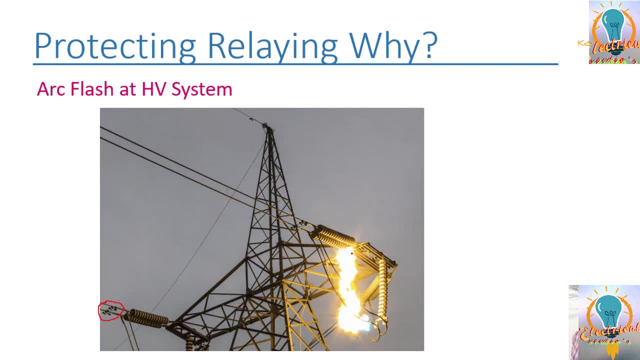 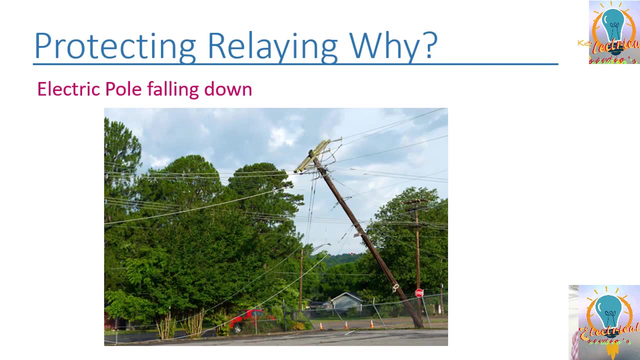 and with arc is formed completely, it is creating a short circuit, heavy short circuit. So in order to protect the system from these failures, we have to have protection. So here you can see another example. In this one you can see that transmission tower. 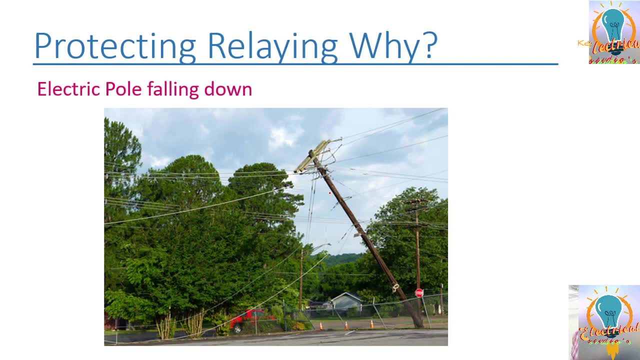 transmission line, which is in fact the medium voltage, has fallen down because of any reason, because of climate changes, heavy winds. So we need to. in such cases, when there is a falling of line, we have to immediately cut off that specific portion to save. 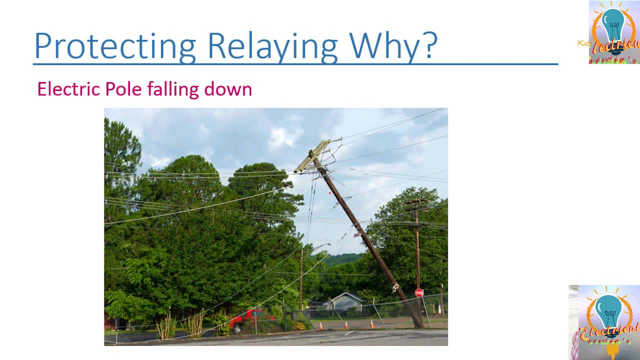 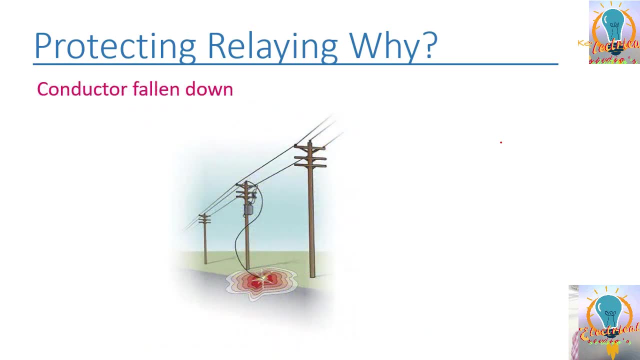 the equipment to save the human life here. So this is another example. So you can see, in this example the conductors has broken and it is now touching the ground. So in this case also, you need to cut this power supply, so you need to have a protection. 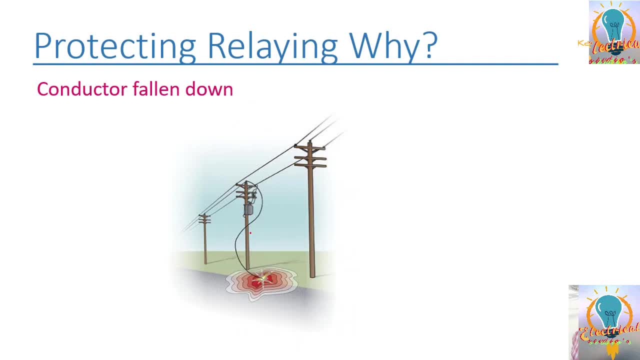 who can sense this fault and immediately, with a power tucker, it should cut down the supply of the line. You need to have a breaker installed which really can give command and it can isolate this specific area of the substation. So here you can see they have. 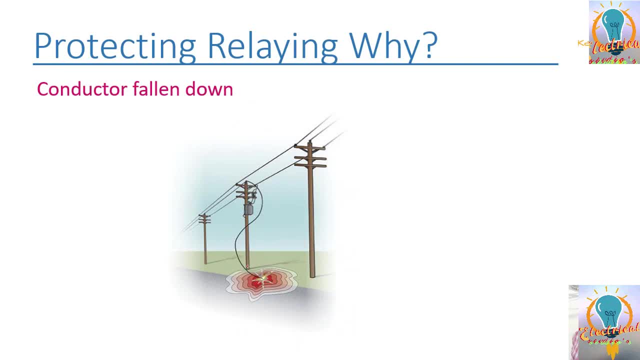 formed the layers. This is just an example for your knowledge that when the conductor- any high voltage conductor- fell to the ground, it's not simply that the voltages are on the conductor but, for example, if the line is 33 kV near to the line, there will be 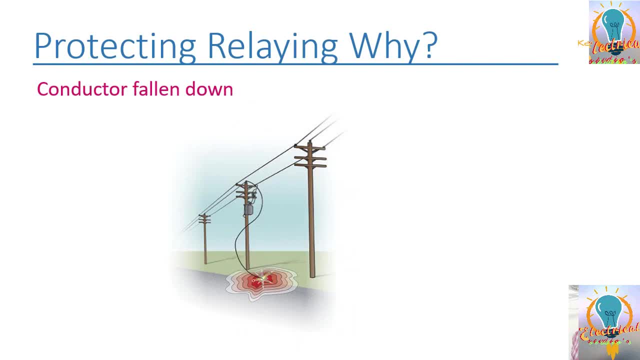 33 kV. after some time it will be 30 kV, then 27 kV. next layer will be 24 kV, so voltage will be in the form of gradients. The voltage will be in the form of whirlpool. 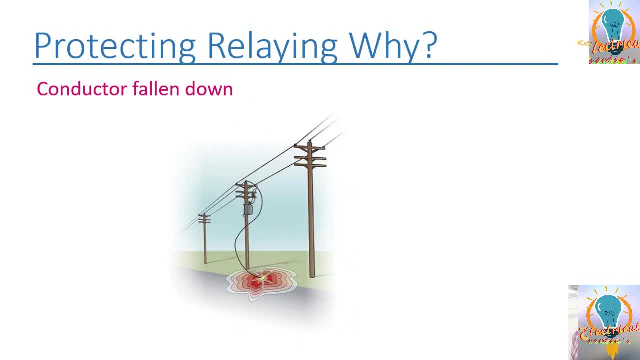 So it means that if somebody is standing or wants to come near to this high voltage line, if standing here person is coming and standing here, one foot is on this and another foot is here, so you can see there will be effective 5 or 6 kV. 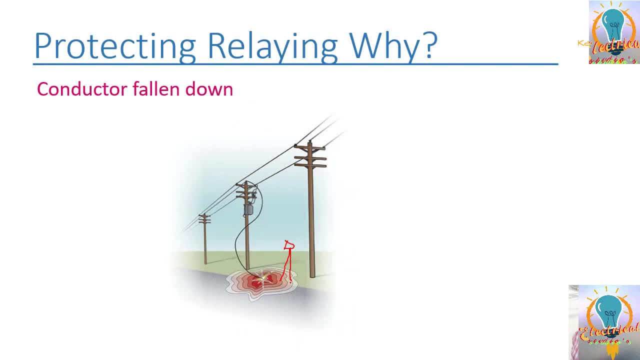 of voltage difference between these two legs, because voltages are not straight. these voltages are in the form of gradient, They are decreasing gradually, decaying gradually to the fault points. So this guy, this is called a step potential and this guy can easily be killed, or 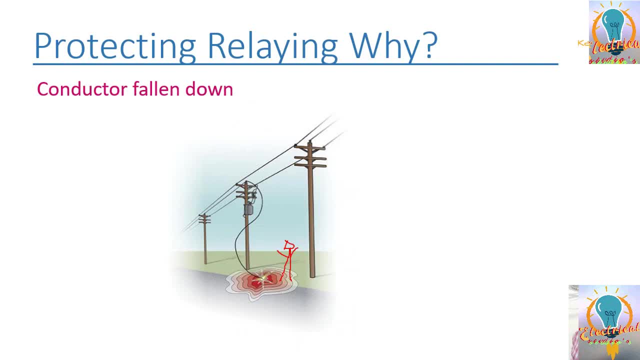 can die by these step voltages. So just for your information, that whenever the high voltage conductors fell down, never try to go near to this conductor, or if it fell down near you, then you have to join your two legs together and then you can jump and come out of. 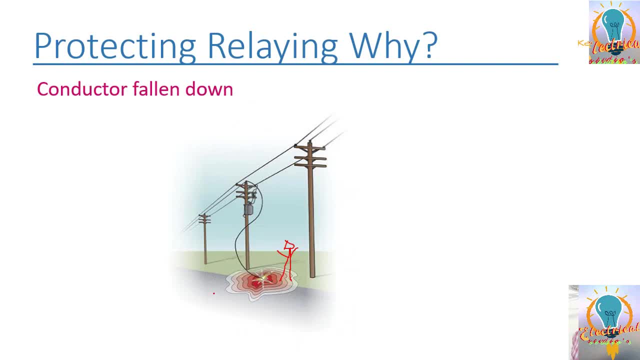 this area and you should not fall down. if you fall down, then your hand and your legs, your current, will pass through your heart and body and then it will be fatal. So that's why it's important to cut this line when the conductor fell down, for human safety, for the equipment safety. 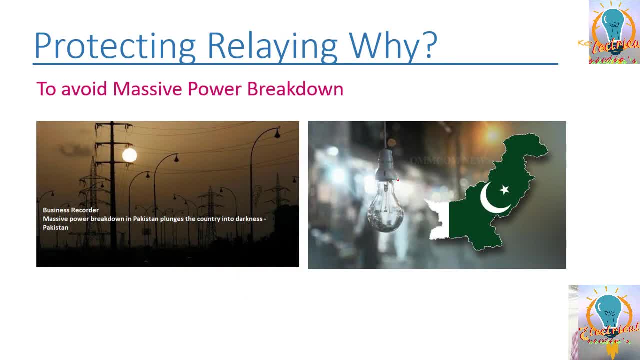 so that's why we need protection. So we need a good protection and relay coordination if you want to avoid the power interruption, if you want to avoid the massive power breakdown. So in recently in Pakistan, what happened is that there is a fault on a line. 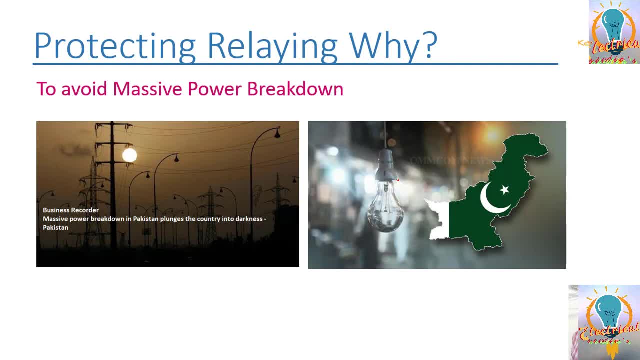 the line was grounded by a portable temporary ground. so basically portable temporary ground is a temporary grounding connectors and these are simple wires that you are connecting to the conductor and then you are grounding it and when they switch it on, the portable temporary ground was connected and the fault only that line. 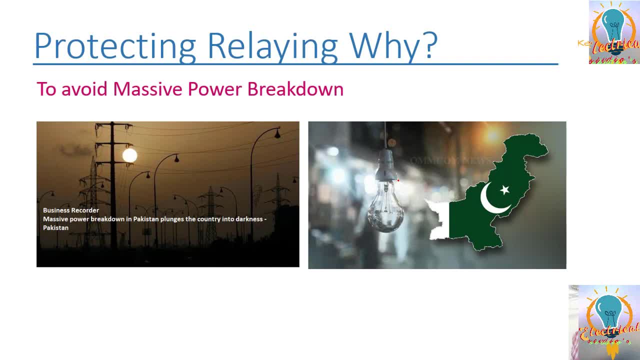 should trip, but instead of tripping that line, whole networks came down. So if the protection system and coordination has been done properly, a specific line could have been tripped and we can save all the systems. so you should have a good protection system installed so that it can. 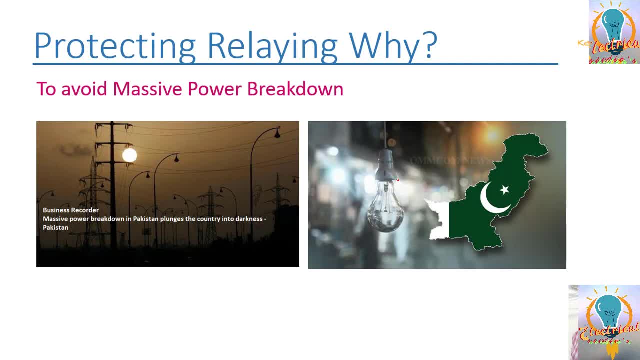 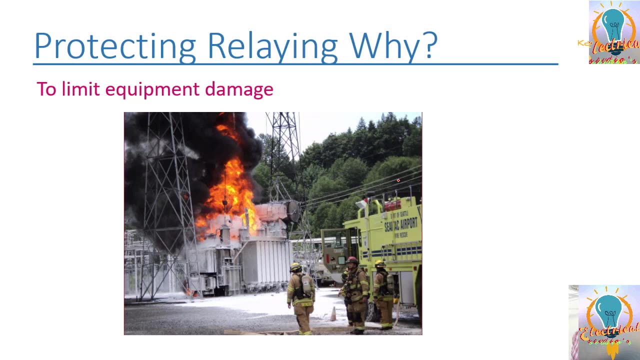 it can only cut off the specific area where it has a fault instead of shutting down whole the system. So you need to have good protection system. So another example is: if you cannot avoid the faults, you need to limit the faults. For example, here you can see there is a fire. 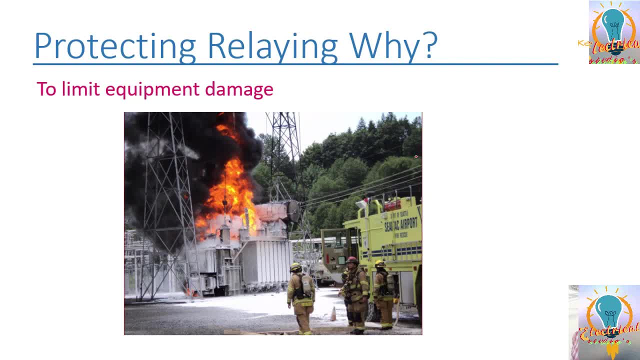 in the transformer. Nowadays, there is a new system which is available and in which the gases when basically the gases, because when there is a fault inside the transformer, gases will form and when the gases will form, this system will be activated and it will inject the nitrogen. 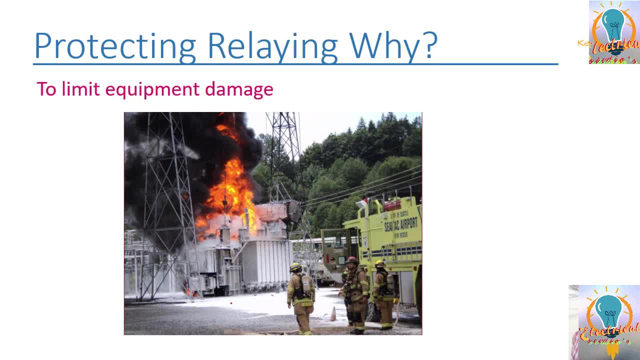 inside the transformer. it will trip the transformer immediately and inject the nitrogen and it will take all the gases, flammable gases, out because it will compress basically the nitrogen will, it will block the basically oxygen and it will allow the all the gases to go outside of the. 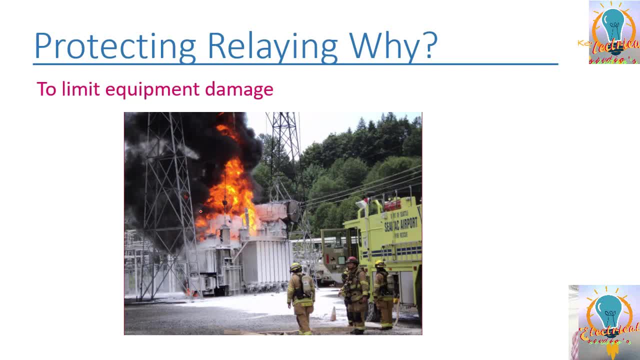 transformer and also so the fault has occurred. but it will try to limit the fault Here. limitation has not been done and you can see the fire has been started. So we should have a protection so that we can we can limit the damage to the equipment. 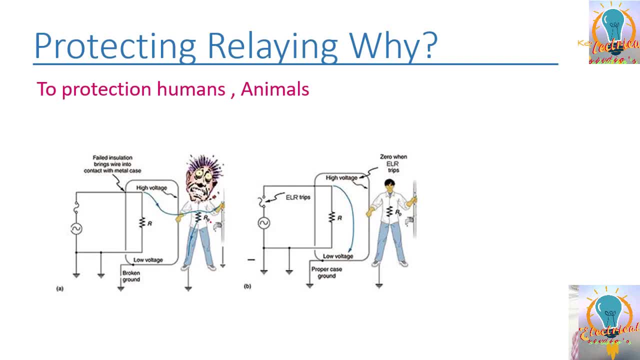 So again, this is the example earlier I have show you. there is basically a thing which is called as touch potential and another thing which is called as step potential. So we should have normally, just for your interest, all the substation, all the power plants we are. 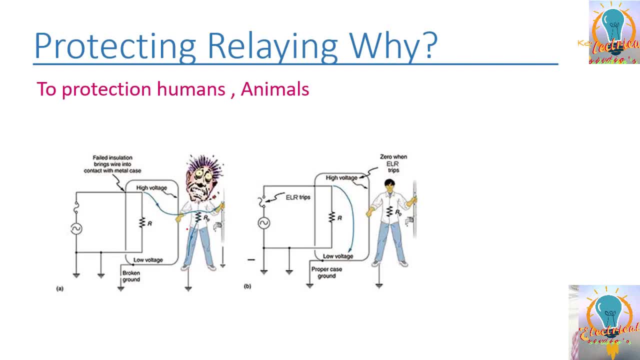 calculating. when we are designing the earth mesh, we have to calculate the touch potential and step potential. So if we are putting first step is to check the ground resistance, ground resistivity, and based on this we have to put some parameter: permissible, basically current, permissible, basically short circuit level. 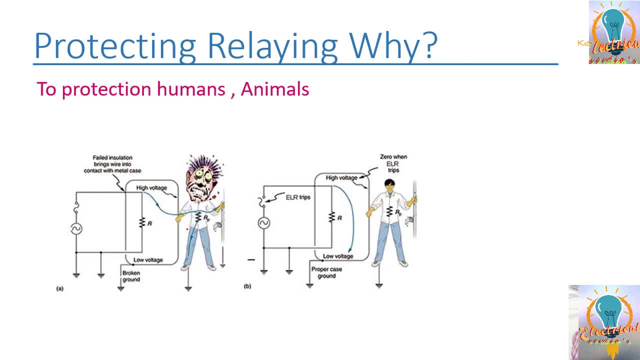 we have to put in it, We have to put the short circuit duration, and then we have to calculate how much we are laying, basically, copper mesh inside each substation and the power plant. so then, when there is a fault, and this charge will be grounded effectively and 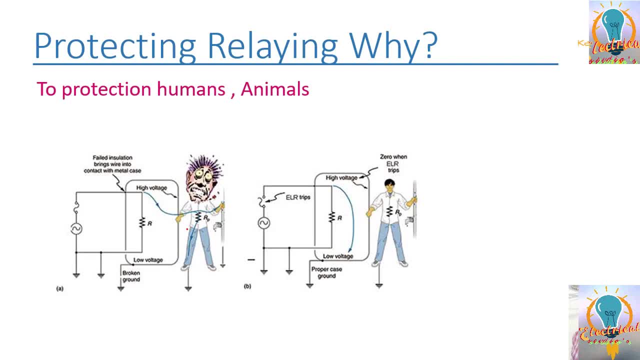 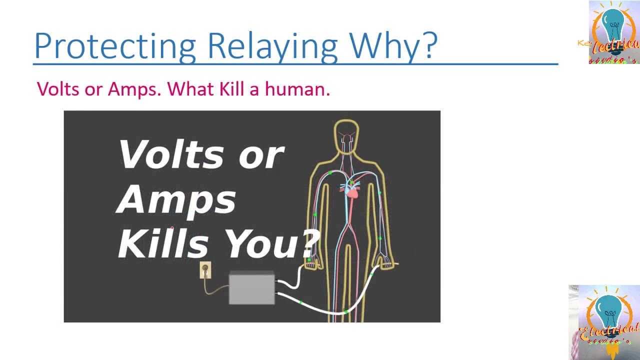 the touch and step potential has to be within the limits. So we have to do all these calculations, we have to do all, we have to design a protection system to protect humans. So another thing is when very famous question is that, basically what kills the human? 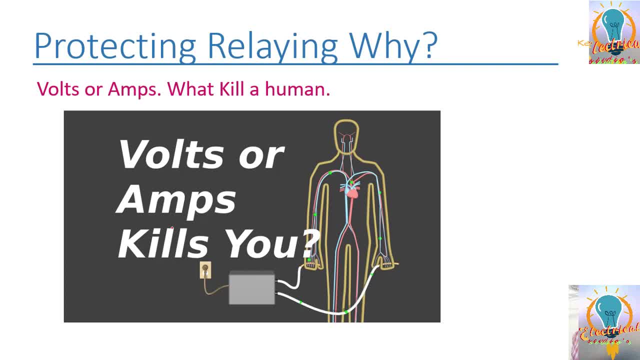 Basically there are two things: one is voltages, one is amperes, but the thing that kill a person is not voltage, is basically when the thing that kill a person is the amps passing through the body of the human. So that's important thing, so we need to. 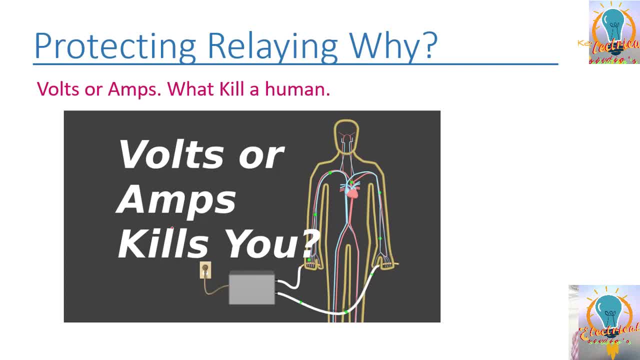 limit the current passing. if you cannot limit the voltage, then you have to limit, basically, the current passing through the body. So that's why the example is: we are using gloves. so if you are working on low voltage, if you are using insulated gloves, there will be voltage. 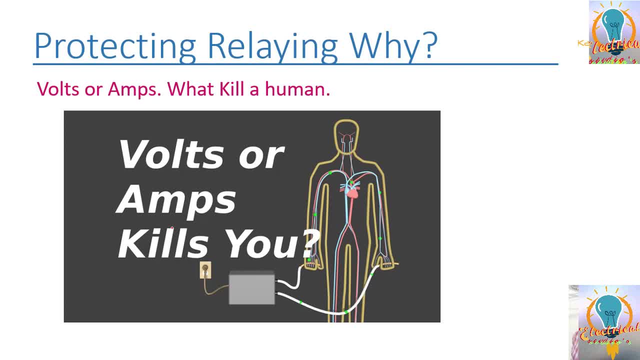 but because you have now high resistance gloves installed- insulated gloves, resistance is in mega ohm or giga ohms- there will be a very less current passing through your body. so in this way you are controlling the basically the current. The another example is basically the gravel which is installed. 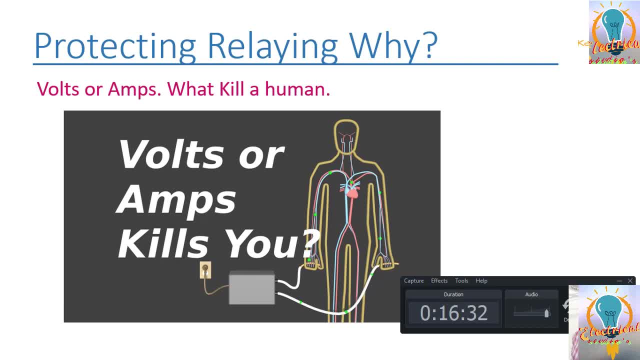 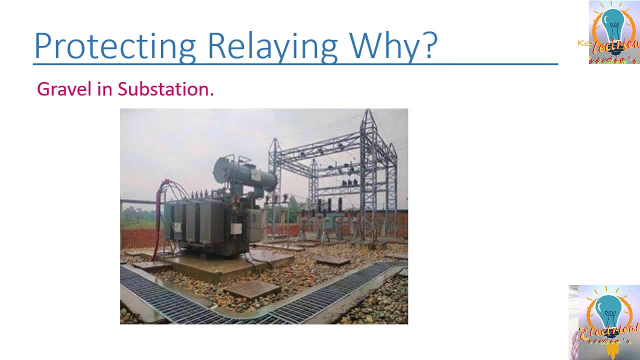 in the substation. So the example of controlling the: if you cannot control the voltage, control basically the resistance is. the other method is to increase the resistance so that the less current will flow through the body if somebody is coming in contact with the voltages. So here: 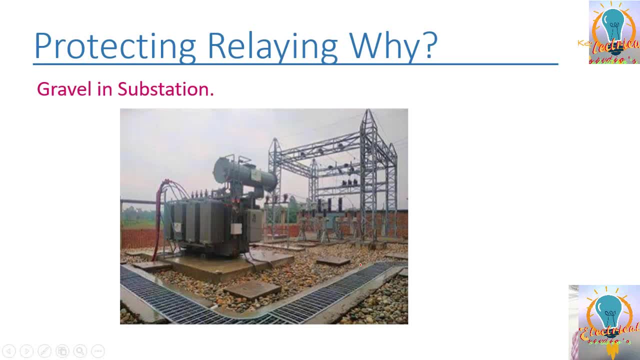 you can see the gravel is is placed in the substation switchyard. so reason of placing this gravel is to reduce the touch voltages and the step voltages, to reduce the basically touch and step voltage impact because this gravel has a high resistance. now if, for example, if somebody is stretching 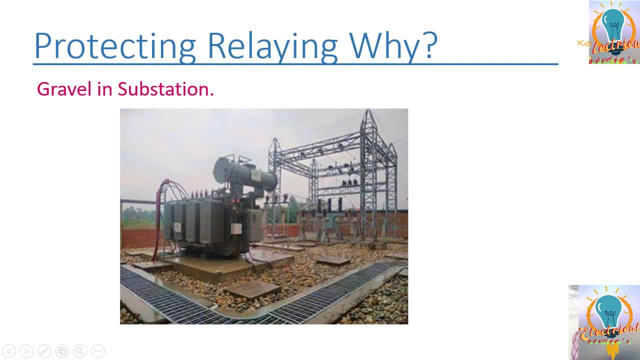 this tower, then this body resistance plus the resistance of its. somebody is standing here and foot is here and stretching, basically the tower. so what will happen? for example, this is the tower and if somebody is stretching, then its body resistance plus the resistance of the gravel, both will come in series. 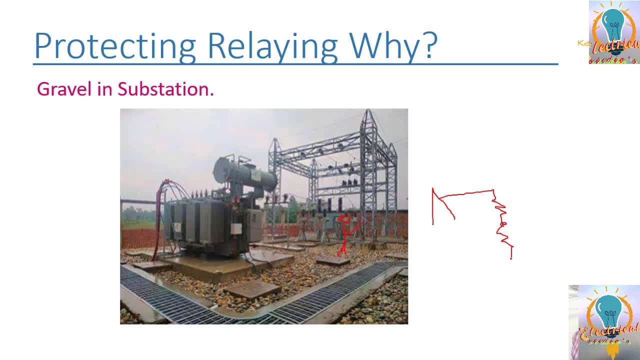 so this is the resistance of gravel, for example, and then ground. so in this way the current flow through the body will reduce and it will somehow will come into within the permissible limit. so this gravel has. you will find this gravel on each substation. this is put with. 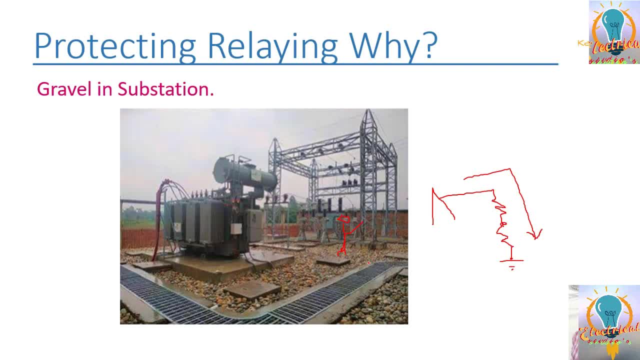 purpose, in order to increase the resistance and in order to control the current flowing through the body in case of touch and step potential. so the type of gravel and the thickness of the gravel is very important, because if more will be the thickness, more will be the resistance. so 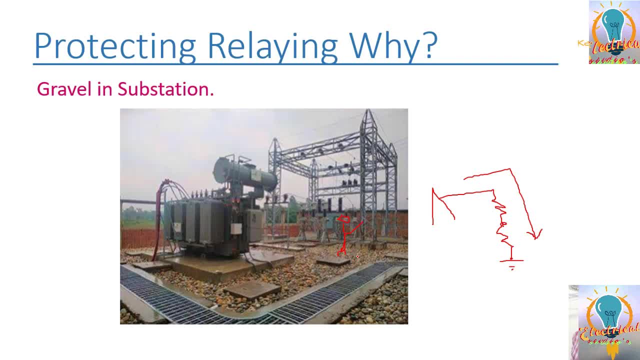 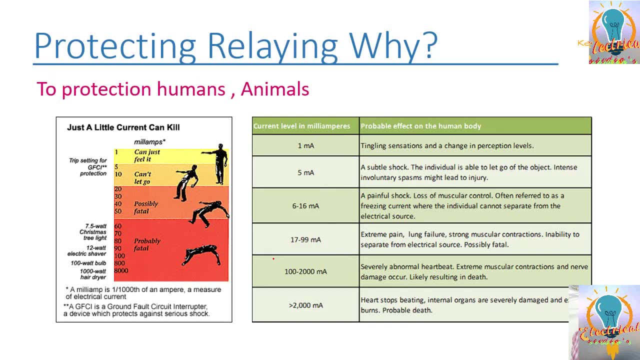 this thickness is when we are calculating step and touch potential. we are keeping this thickness in the calculations. so here you can see some, basically, basically a chart. so they have shown here that some current has passed through the body and what is the impact on it. for example, if one milliamp current 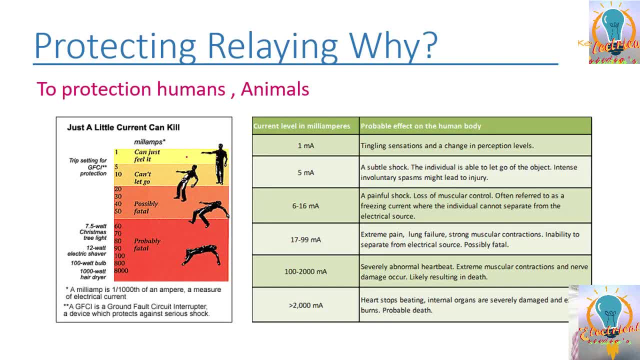 is passing through the body, a person can just feel it will have some sensation. it has a tingling sensation and change in the perception level. so if five milliamp is passing through the body, a subtle shock, the individual is able to let go of the object. intense. 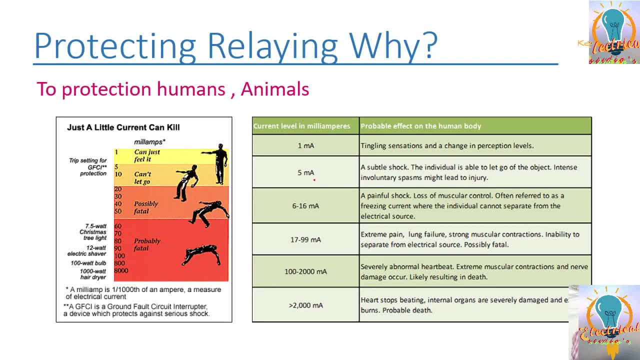 involuntary spasism might lead to injury. so five milliamp is you can remove your hand but it can injured. so six to sixteen milliamp. it has basically a painful shock. muscle control will be lost and often referred to as a freezing current, where the individual 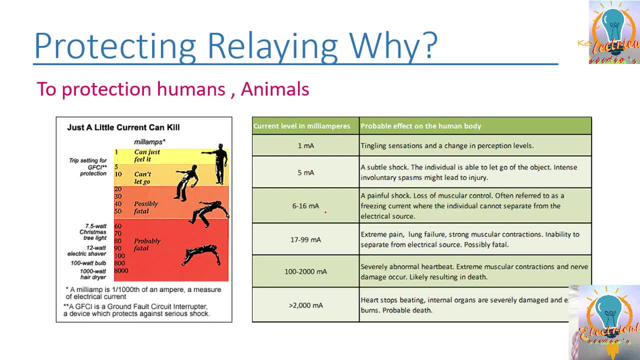 cannot separate from electric source. so basically all the body is operating through electricity, by small electric pulses. so if you have external electricity, then your pulses from the brain will not work. so ultimately you cannot take your hand out of it and the result will be really bad. then we have 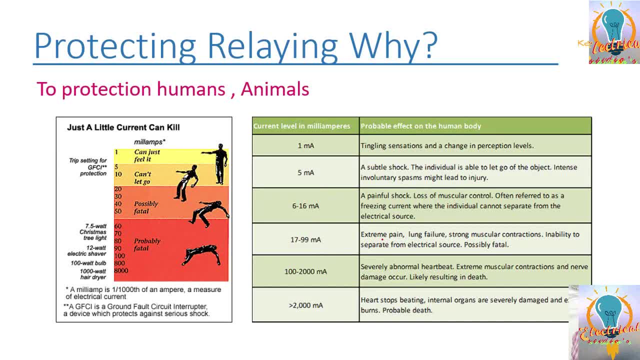 17 to 99 milliamp and then it is extreme, painful also lung failure, strong muscle contraction, inability to separate from electrical source, possibly fatal. fatal is starting here. then we have 100 to 2000 milliamp, severe, abnormal heat burn, extreme muscle contractions. 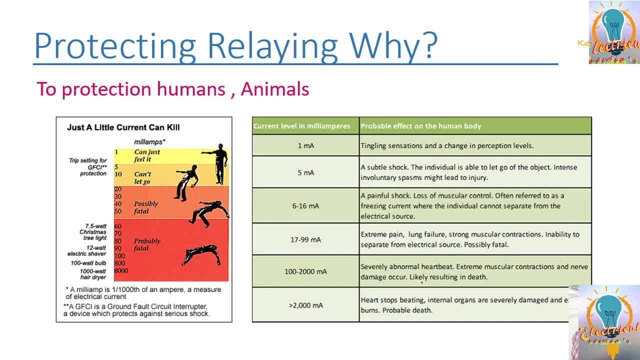 and nerve damage occur. nerve damage occur, likely resulting in death. so greater than 2000 milliamp or 2 ampere heart stop beating, internal organs are severely damaged and extreme burns probable death. so this is example of the current passing through the body. so another thing is: 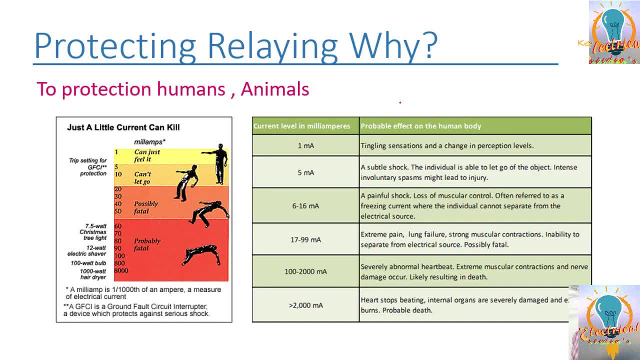 which current is more dangerous, ac or dc? so just for your interest. ac: you know already that it has a frequency 50 to 60 hertz, so every time it has passed through zero. so when it is passing through zero there is a chance and you can remove your hand. 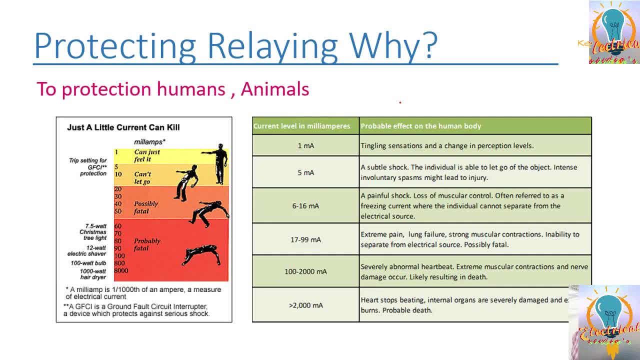 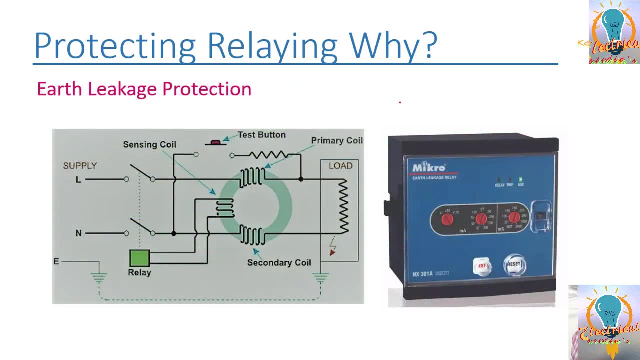 even though the current level is little high. but for dc it is a straight, so it will be difficult for a person to take his hand off. so this is just an example when the current passing through a body can damage, so we need to control it for protection. 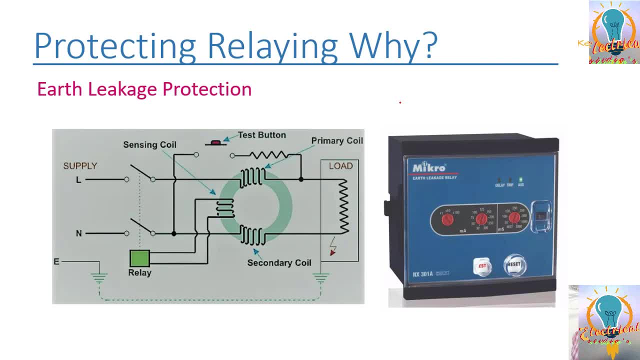 for such. in such cases, there is a protection which is called as earth leakage protection. you can see this diagram and this is I have put one relay, for example. here you can see set this time. here you can see when the earth leakage is 30 milli. 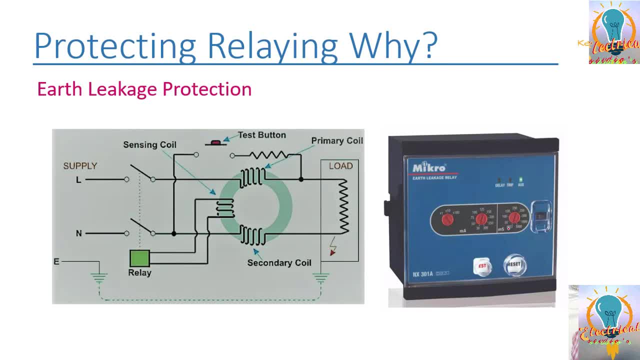 we are keeping always 50 or less than 50 milli. the settings and the time is also mentioned. we have kept here instantaneous. we can keep 150. if it is keep on tripping there might be some leakage at other place. so this protection relay we can install. 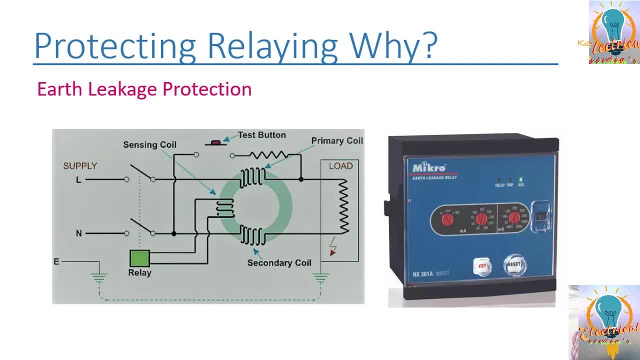 normally, this is always a good idea to install earth leakage circuit breakers or earth leakage relay in homes so in case of any person is touching any fire immediately, this protection will isolate the house and it will save that person from electric shock. so this is an example of 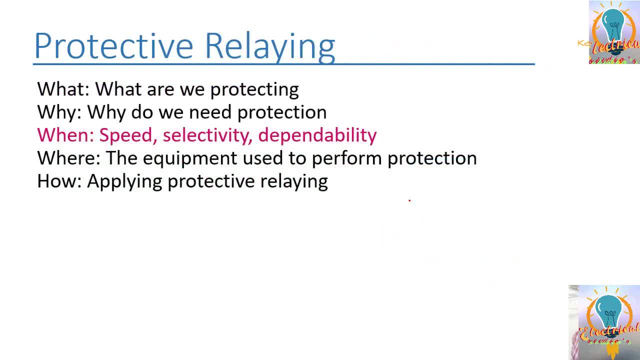 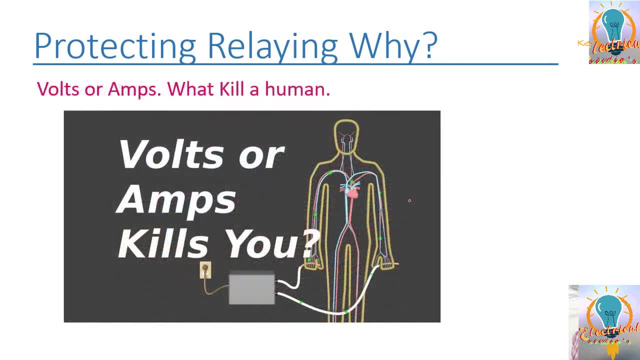 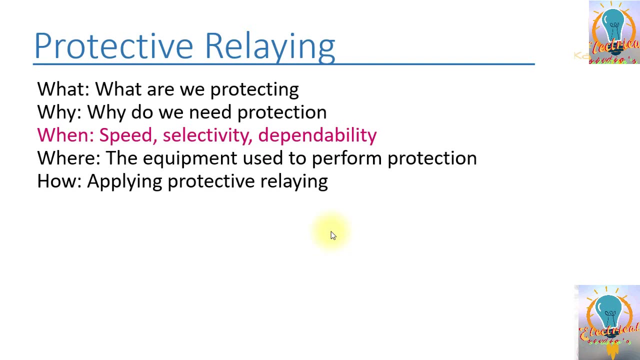 how we need protection relaying. so next we will move on to our next topic. so thank you very much. I hope that you enjoy my lecture. hello friends. now in this section we will discuss and study about some good characteristics of protection system. I have put here as an when. 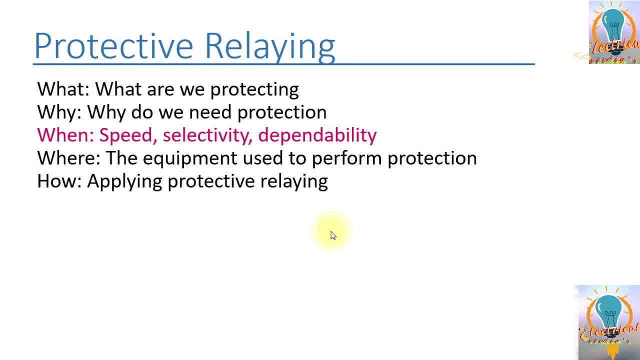 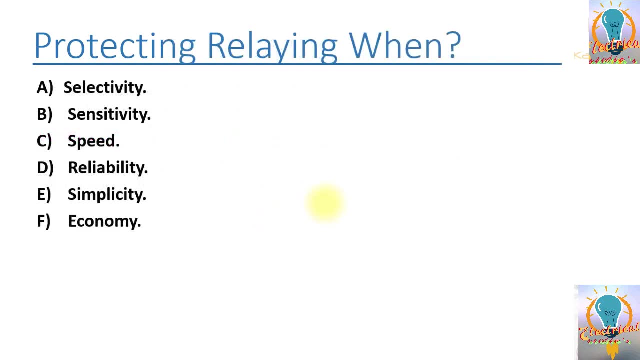 so when you are designing a protection system, what things you need to consider and what a good protection or ideal protection system should have. so we will start our topic. so a protection system should be selective. so the characteristics of the protection systems are selectivity number A, so its kind of 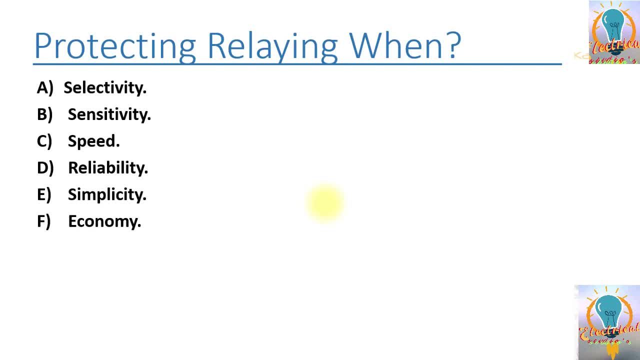 isolate only that area where it has a power, instead of isolating complete region, city or an area. number B is sensitivity. it should be sensitive enough to sense the fault. number C is speed. the protection device should not delay the fault for a longer duration, because in this way the backup protection will operate. 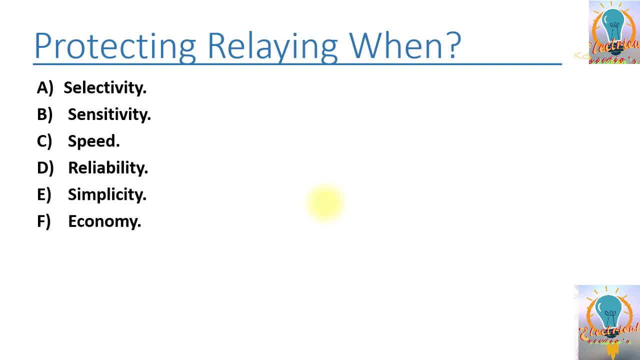 and the result will load shedding or shedding of power on the bigger area. so the characteristics of the protection system should have: it should operate in right speed, then it should be reliable. so the protection system should be reliable, so its considered that whenever there is a fault it should operate. 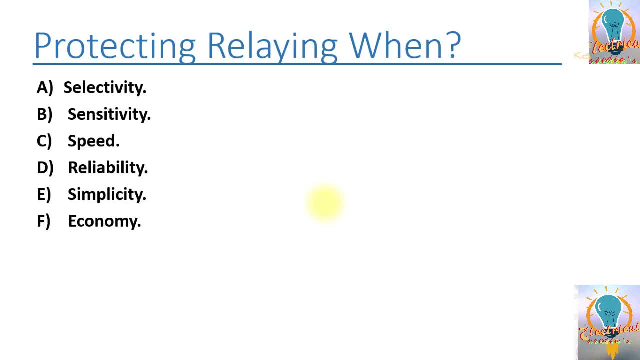 next thing that should be in the protection system is simplicity. so the protection system or, for example, protection relay or scheme, should be simple enough so everybody can easily understand it. or, in case of fault, you can also easily troubleshoot. so there should be a simplicity in the 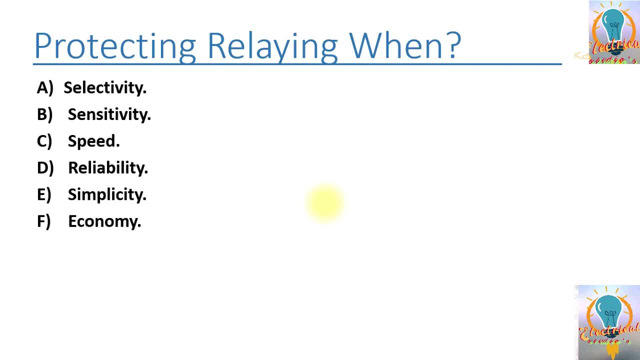 protection system in point of, also from point of maintenance, the protection system also be able to protect properly, and when we are doing maintenance then you should have enough space and it should be easy to maintain. then the economy the protection system should have should be economical. so we will start with our first. 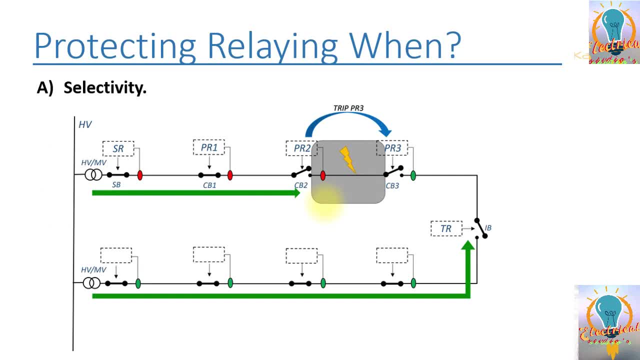 topic: selectivity. hey, friends, now we will start our topic. its called selectivity. this is one of the most important characteristics of properly designed protection system. so lets consider this example. so here you can see. this is we are denoting bus power by a line. so you can see. 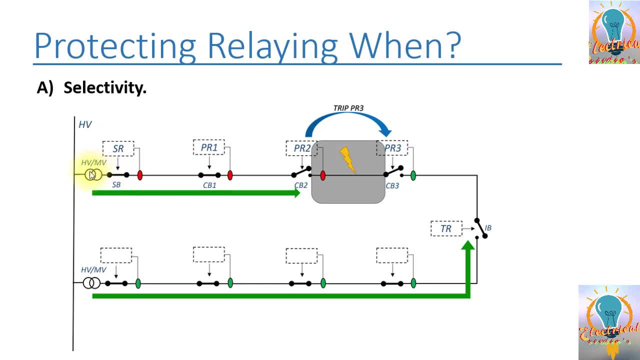 a two transformers. this is symbol of transformers. two transformers are connected to a bus and both are feeding. you can see a network. so basically, you can see it is called as a ring. so you can see it is a ring. and here you can see, and there is basically 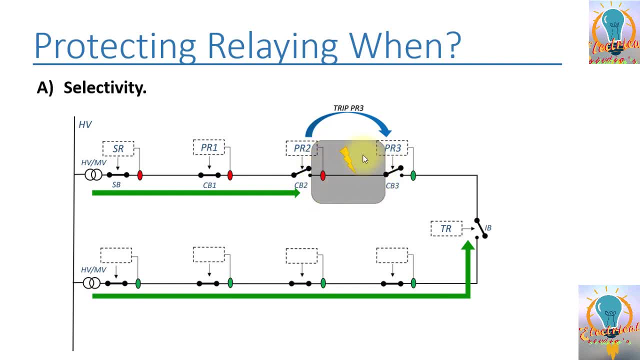 a fault in this section. there is a fault here in this section. so- and at the moment you can see that the coupler is open- this is a coupler which connect the two networks which are forming a ring. so, if there is a fault here, that an ideal network. 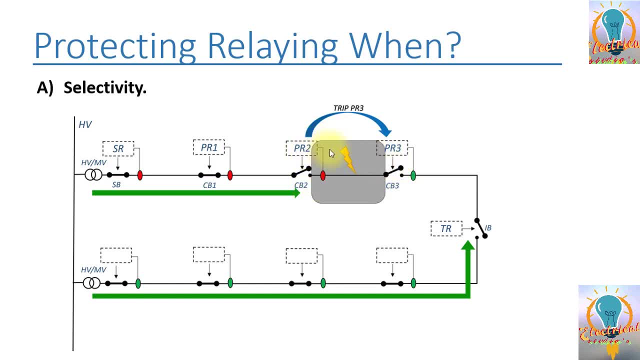 this breaker and this breaker we are to, and PR3 should open, should trip, and if they are tripping correctly and right time, then this fault is isolated successfully and all other networks will be keep on running. so the more better protection could be the tripping of these two. 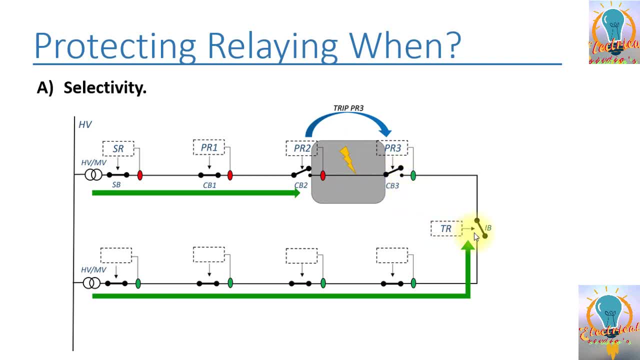 breakers and then reclosing of this tie breaker. so in the second step, first of all fault will be isolated here and this: when this breaker is closed, the tie breaker is closed, then the supply will be restored up to this point. so you need to. this is kind of. 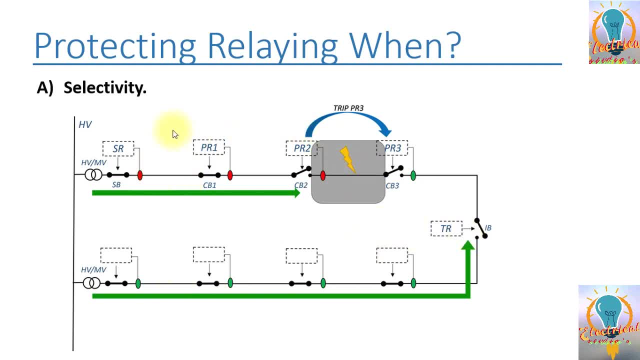 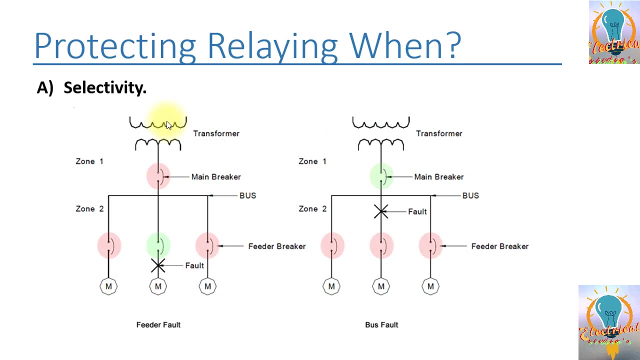 called as reclosing. so this is a good example of selectivity. so the purpose is that you need to select as minimum portion of the fault did area as possible to isolate the fault. so this is one of the main characteristics of the protection system. so here there is another example. 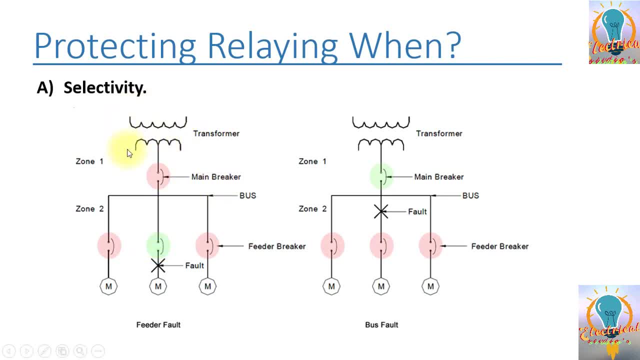 so here you can see this is a symbol of transformer and you can see this is the zone one. later on i will explain you how zones of protection are designed. so this is just an into protection. this is the main breaker, which is called as incomer, and there are three. 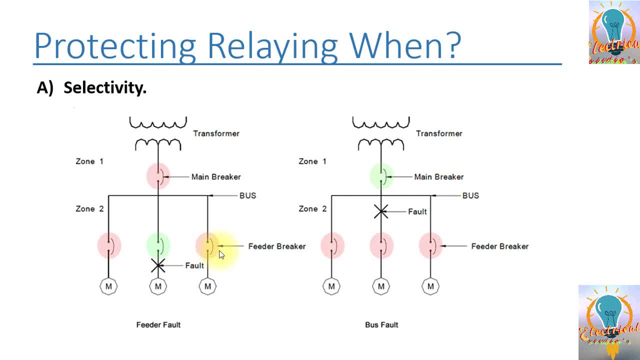 outgoing feeders and the case, consider case- that there is a fault on one of the line. here is the fault. you can see there is a fault on one of the line, so this breaker only should trip. so if this breaker trip, it will isolate the fault and the remaining system will be. 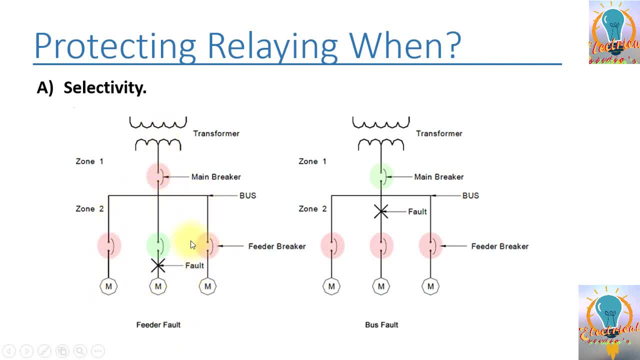 keep on running as it is. so it means that fault is isolated properly, faults selection is done correctly and only the faulted loop has been correct. so another example of the fault is now: the fault is on the bus. if the fault is here and if this feeder 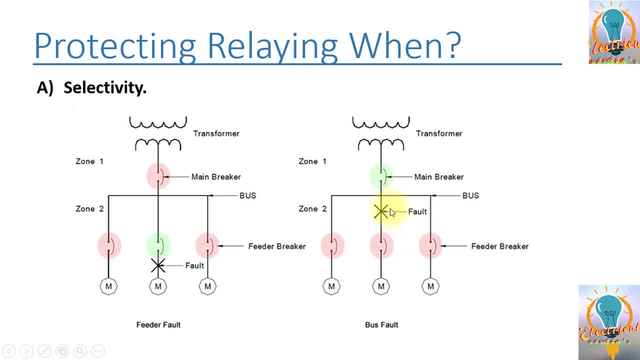 is tripped, it will not isolate the fault. so, in order to isolate the fault now, this fault is feed through this transformer, so we need to trip this breaker. so in this case, in order to isolate the fault, we have to trip complete bus and we have to trip. 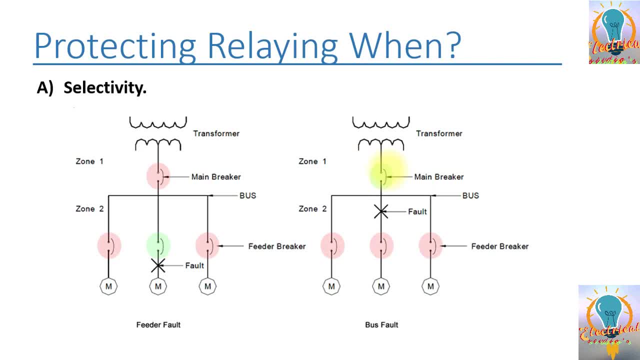 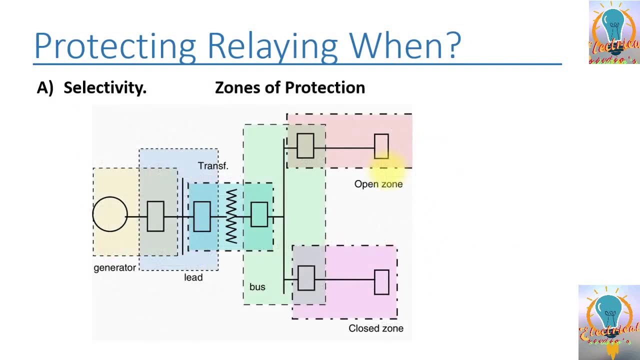 the main incomer. so this is example of fault and how to select, how different areas are selected. so here you can see an example in which we have generator. we have a breaker of the generator which is connected to a bus. this circular symbol is for generator and this: 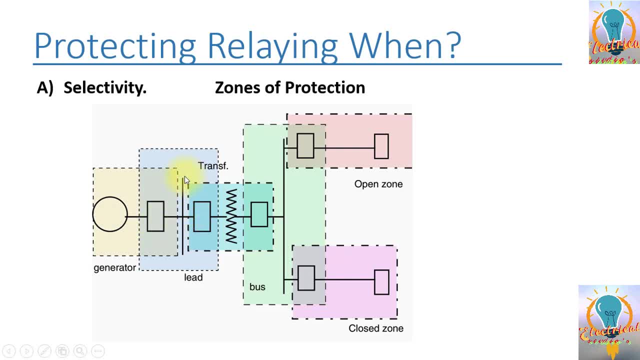 bracket symbol normally used for breaker rectangle, and this straight line here is used for the bus bar, showing the bus bar. and then we have breaker, feeder breaker here, then we have another transformer, then we have another breaker and then we have another bus. so you can see that voltage is step. 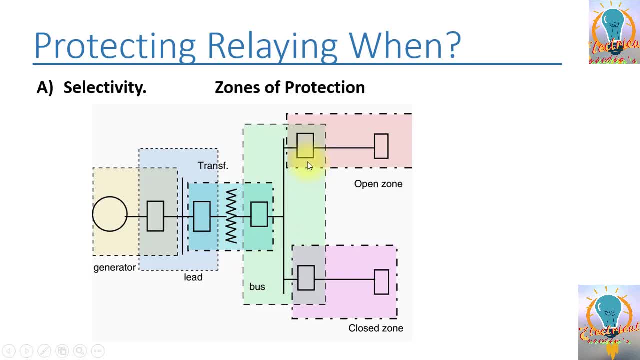 up or down using this transformer and it is connected to the bus and then it is connected to different lines. so all the protection systems is divided in zones and it is important that each area of the protection system should be covered at least by one zone. no area of the protection. 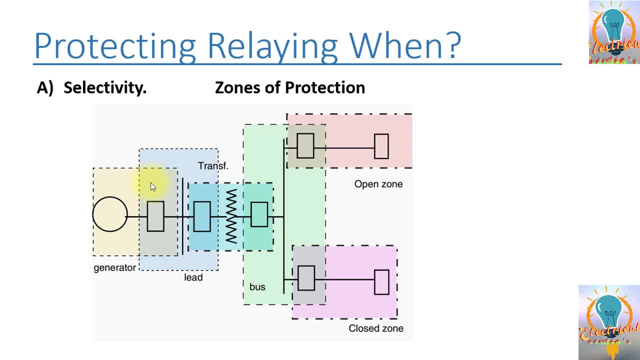 system should be uncovered or it should be exposed to faults. so you can see, this is the generator zone, zone of generator, and this is the another zone you can see which is covering the bus and the two breakers, this area. you can see this area, the zone, generator zones and the 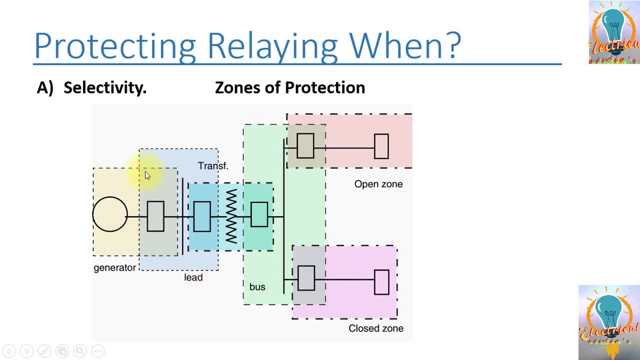 lead protection zone. both zones are basically overlapping so it is called as overlap zone. so in the protection systems you will see lot of overlapping. so advantage of overlapping is that that if for example here the lead protection did not operate because of any reason, the back and the protection 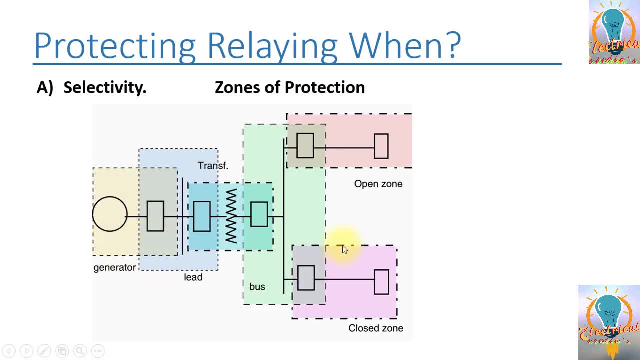 of generator will operate and it will isolate the fault. so this is called as loop overlapping, zones overlapping and these are different zones. so this is example of, and we are forming the zones to have a better selectivity. more zones means more, better selectivity. so if the fault 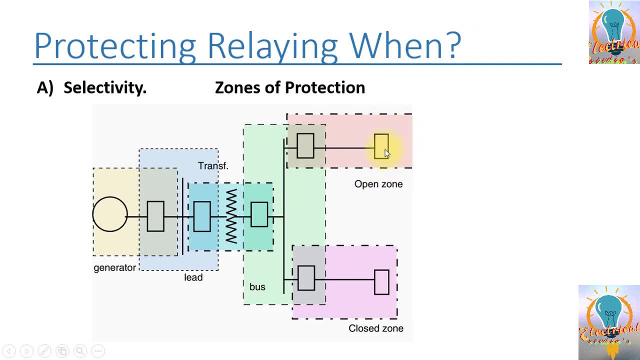 is in this zone here open zone, so it will tripped and this is an example of closed zone. so what is the difference between open and closed zone? just for your information, an over current protection has an open zone and differential protection has a closed zone, because any protection 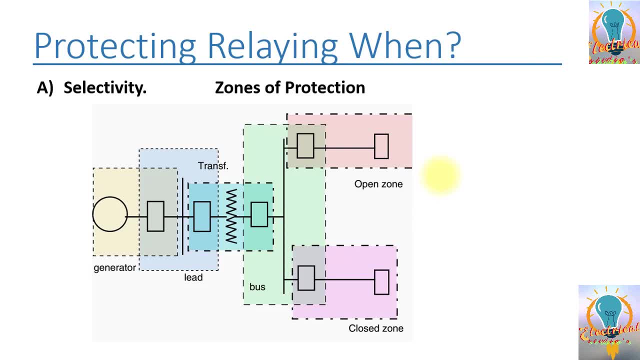 which can only, which operate only when the fault is within its zone, within within a predefined area. if there is a fault, if a zone really will operate, example is a differential protection, then it is called as a closed zone protection. so let's show you something. so, for example, 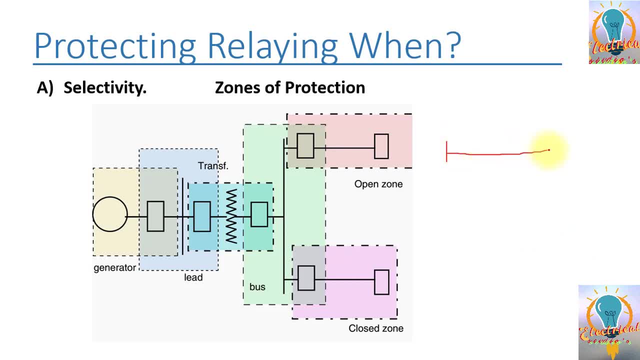 if we have a line, station A and station B, we have CTs here, we have another CT here. so, for example, here one relay is installed, 52 over current relay, and another relay is installed here, 87, which is called as a differential relay and differential relay. 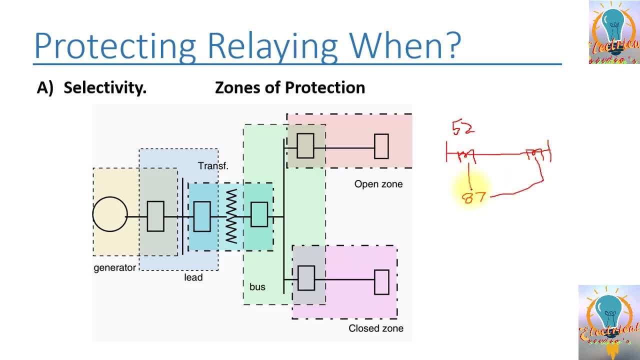 is feed by this CT and this CT. it is checking difference of both CTs and with over current relay is feed by this one and CT only. so, for example, if there is a fault on, this is station A, for example, and this is station B, this station C. 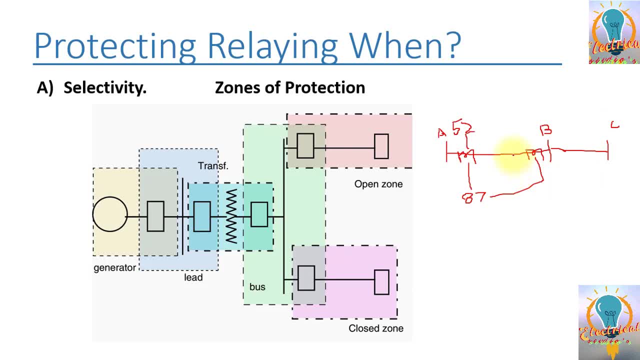 if there is a fault here, example in zone fault, there will be a fault current feeding from this to down and there will be no fault current here because, for example, here source is only connected this side, so this will be feed to the 87L and 87L will operate. 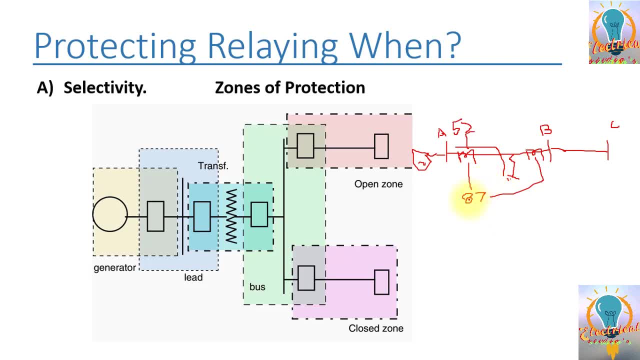 in detail I will explain you later, just for example to show you what is open and close zone means. and also differential relay will pick up because of this fault. ok, so this will. because differential has instantaneous time distance will trip first. 50 protection- 50 is basically backup protection. 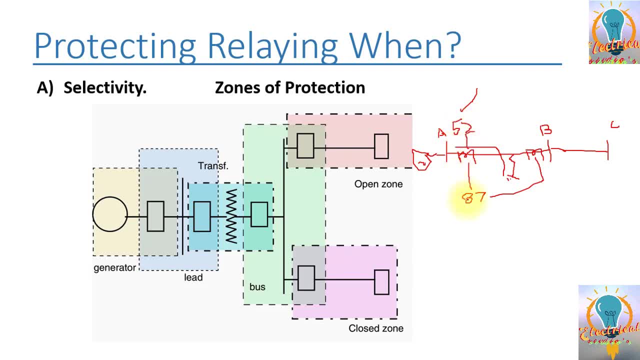 so it will be, it will trip if 87 is not trip after some time delay. so but if there is a fault outside between B and C, there will be a fault current from station A to ground. so here you can see the differential current in and out. both are same. 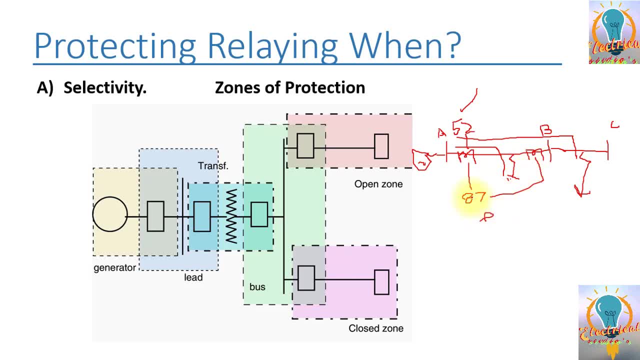 so differential current will be 0 in this case. so differential protection will not operate. where is there will be fault current and 52 will be feed by this CT only, so it will send some current. so we can say that differential protection is a unit protection and what is operating only. 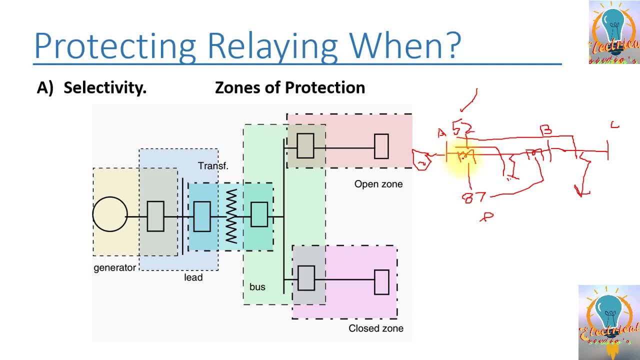 when there is a fault between a given point A and B, between these two CTs, where, as over current protection is kind of open zone protection. so that's why over current protection is used. benefit of using over current protection is that it can be used for graded protection. 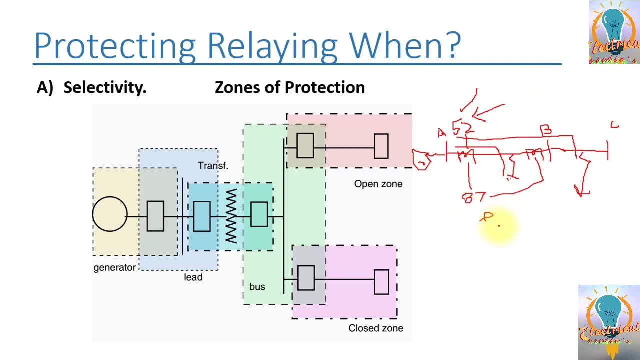 where, as 87 is not used as a graded protection. so lets on, and later we will explain you in detail what is a graded protection. for example, if this breaker fails to trip, if the protection, for example DC supply, is fail here, in that case this protection will trip after. 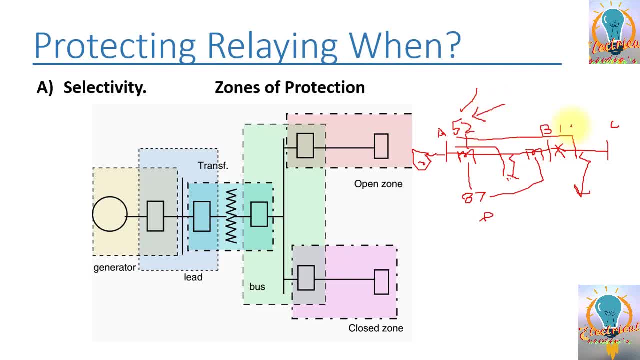 if we set this tripping here in 1 second, for example, I can set it here 1 seconds and here I can set it 2 seconds tripping in 2 seconds. so if this relay fails, then this relay can trip. so we can have concept of 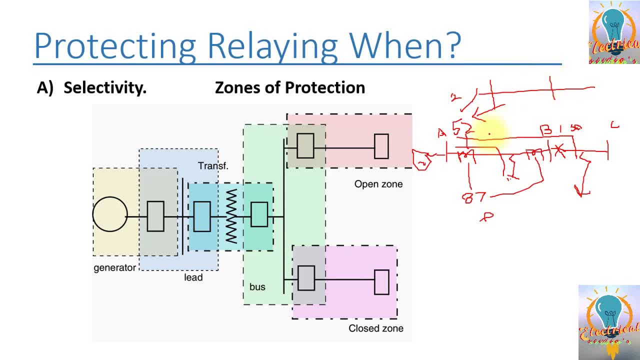 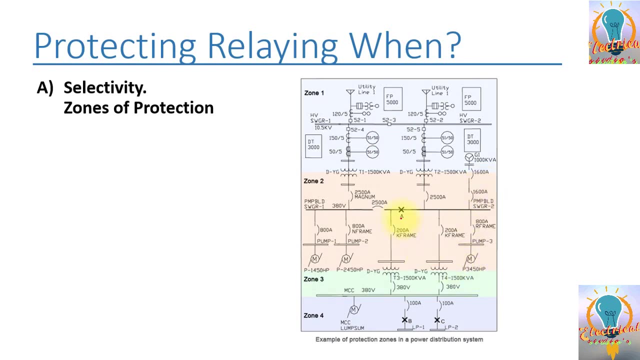 graded protection. so 52 can be open zone can be used for graded protection, where as 87 is used for unit protection. so this is some example. so here you can see another example of selectivity. so we have divided the power system into 4 zones: zone 1, zone 2. 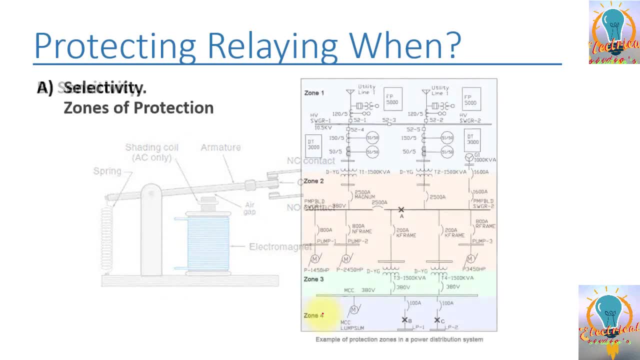 zone 3 and zone 4. so in this way now we can understand that power system is always divided into zones. and we are dividing it in zones so that we can selectively tripped faulted portion only, and if the faulted portion protection fails, then it should be tripped by the backup protection. 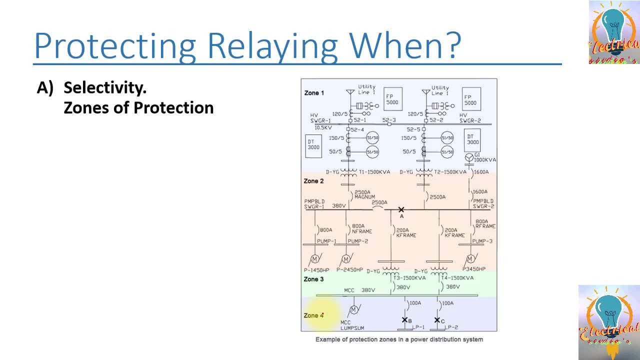 so this is example of selectivity that we should have. so we can define selectivity as simple as that. this is the ability of protection system to select correctly that part of the system in trouble and disconnect the faulty part without disturbing the rest of the system. a well designed and efficient 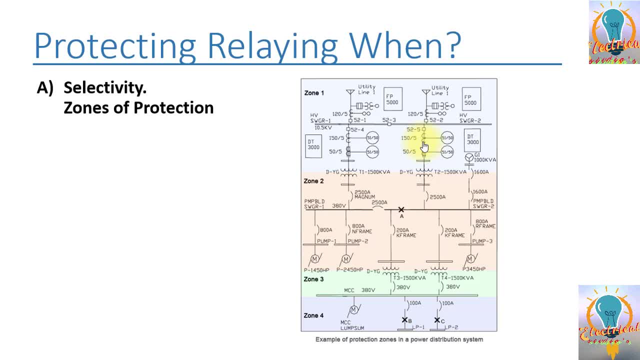 relay system should be selective, that is, it should be able to detect the point at which the fault occurs and cause the opening of the circuit breaker closest to the fault, with minimum or no damage to the system. in order to provide selectivity of the system, it is usual to practice to divide. 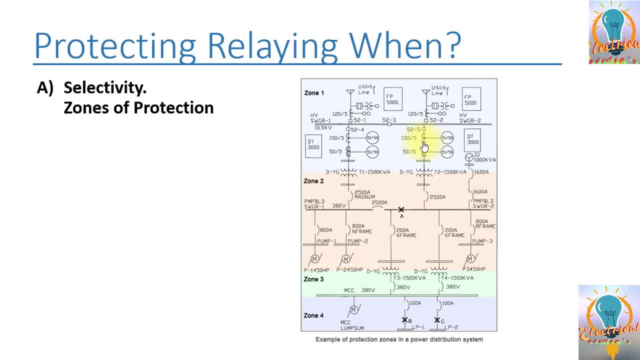 entire system into several protection zones. when fault occurs in a given zone, then only the circuit breakers within that zone will be opened. this will isolate only the faulty circuit or operators, leaving the healthy circuit intact. the system can be divided into several zones, just like protection zones. 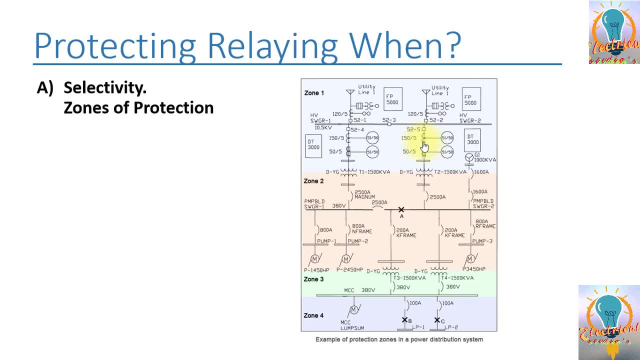 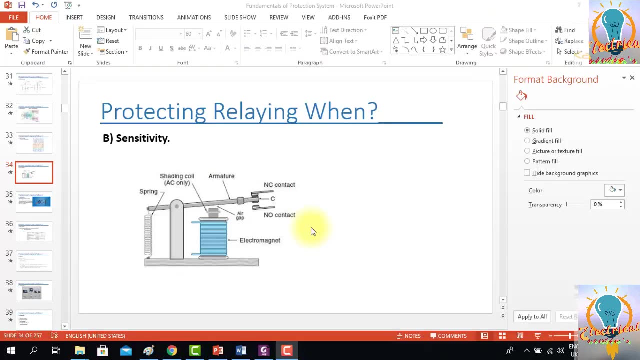 for generators, power transfer, transmission line, hv switch gear, etc. so this was a little definition for selectivity. i hope that you understand the lecture clearly. thank you very much. so the next important thing about the relay characteristics is the sensitivity. the sensitivity is- we can say that it is an ability. 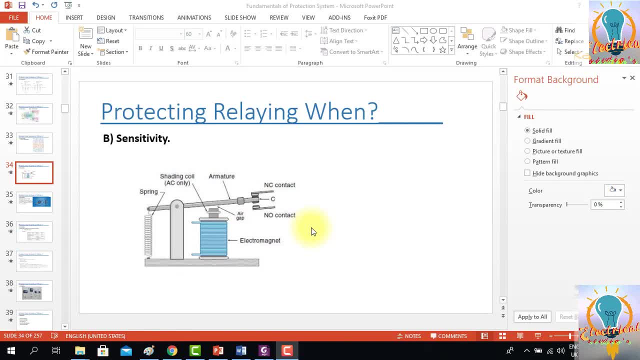 of the relay to operate with low value of actuating quantity. so actuating quantity can be voltage, can be current, can be impedance, frequency, etc. sensitivity of a relay is a function of volt amps input to the coil of relay necessary to cause its operations. the smaller the voltage amps 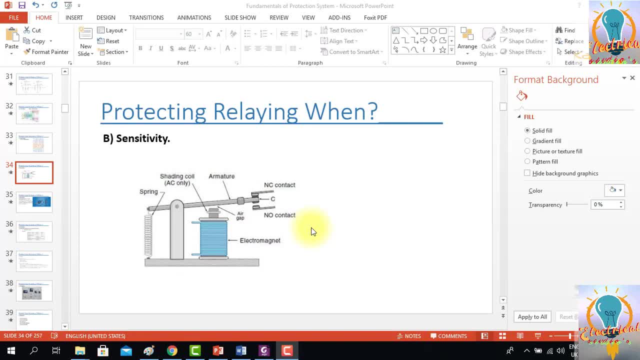 into required to cause relay operation, the more sensitive is the relay. thus a 1 VA relay is more sensitive than 3 VA relay. it is desirable that relay system should be sensitive so that it operates with low value of volt amp input. so it is very clear. 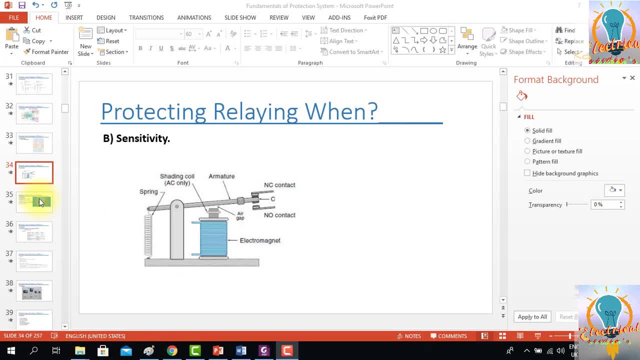 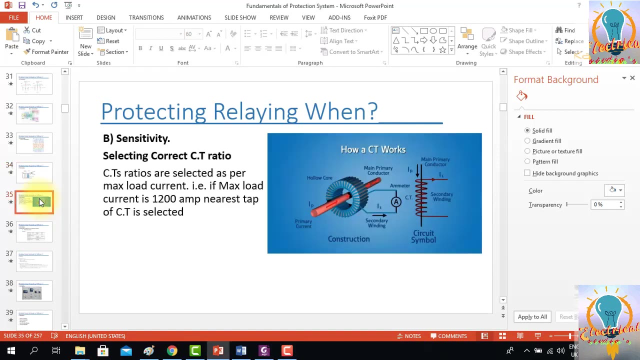 now that if a relay is drawing more power- basically more VA means is drawing more power, so it means that it need to draw more power to operate, so it means less sensitive. ideally the relay should be very sensitive. it can sense a smallest, basically quantities, so that it can operate. 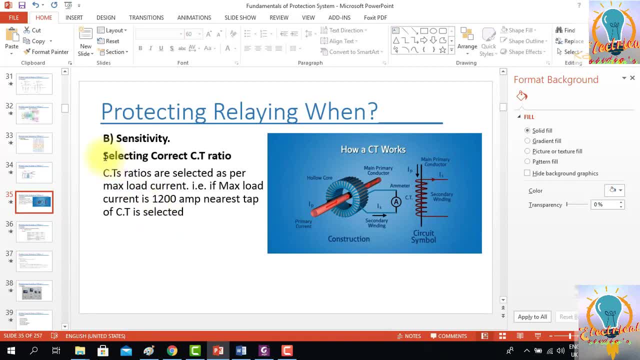 easily. so the next thing to improve sensitivity is selecting the current correct voltage ratio. so normally the voltage ratios of, for example, if we take an example of a feeder, are selected. how much load is supplied, remember if the maximum load is 800 amperes. so mostly we are selecting. 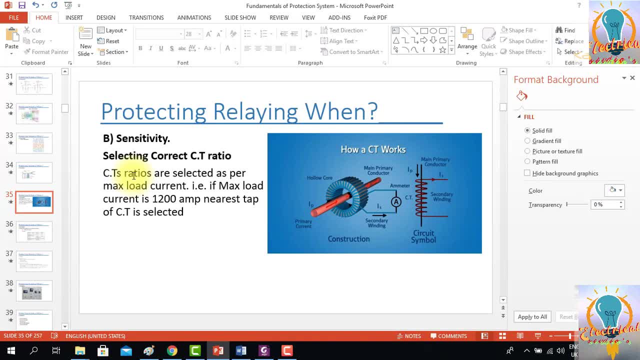 the ratio near to 800, like 900 or 1000, always allowing 110 to 20%, we are considering as an overload. so but if, if we are not selecting the correct CT ratio, for example, if the load is 800 and we are selecting ratio like 3000, 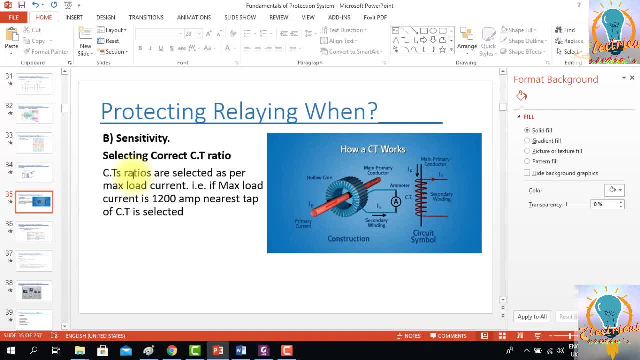 by 1 ampere, so it means that the sensitivity of the system is compromised. so, for example, if we are selecting 3000 by 1 ampere and full load, even we are getting 50% of load is flowing, so then it's like 400 is flowing. 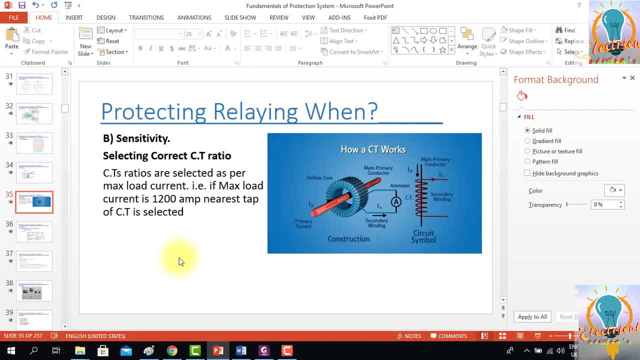 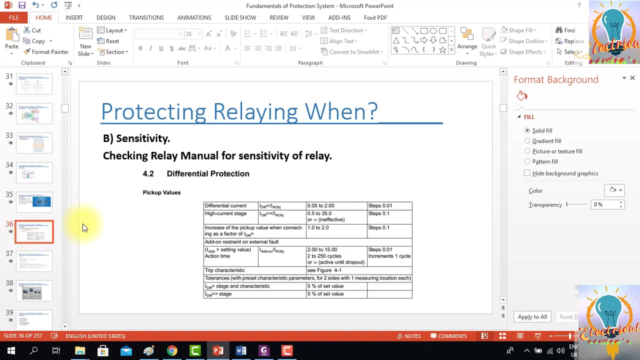 divided by 3000, so the current secondary current will be 133 milli in that case. so you need to select the proper CT ratio if you want to have the correct. basically, ah, improve the sensitivity of the system. that's always very important. so how? how you can find out the 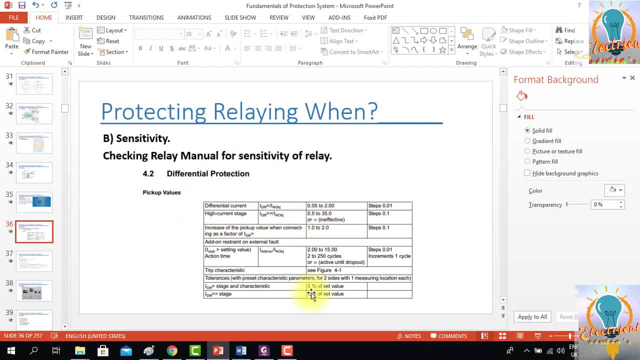 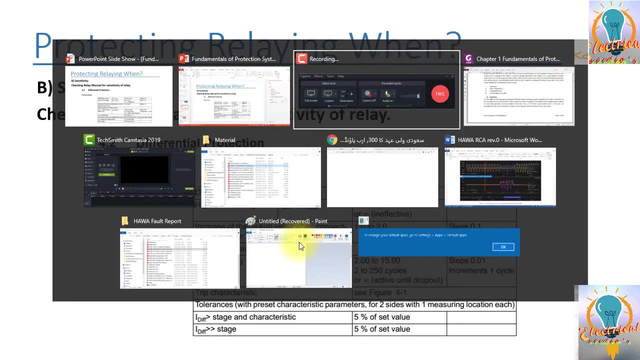 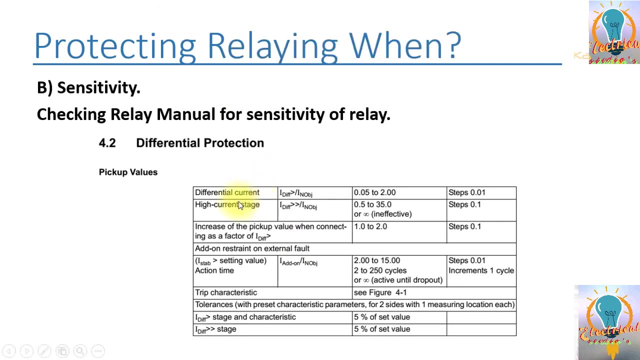 sensitivity of the relay. so here I have shown a snapshot from the relay manual of differential protection. so this is a snapshot from the differential protection. ah, here you can see they have shown some values in the chart. so let me show you that they have shown that differential protection. 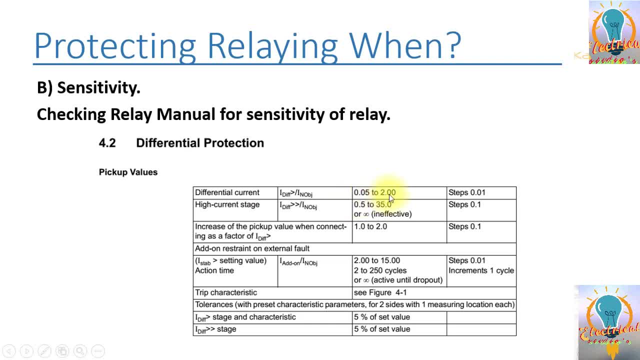 can operate. the operating range is 0.0532 with the step of 0.01, so this relay can sense increase of 0.01 amps. so this differential protection is very, very sensitive. so you can see it can detect smallest change in the current and 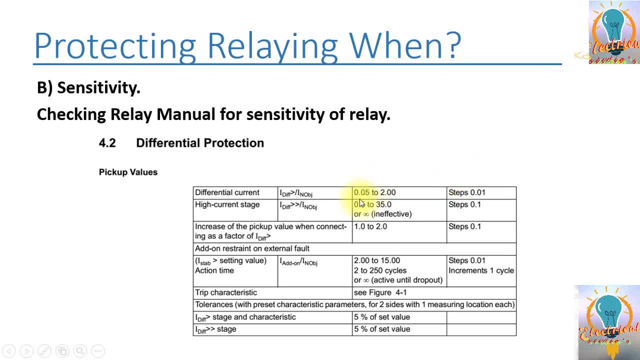 the minimum current it can detect safely and operate is 0.05. so you can say the relay is very sensitive to detecting the smallest quantity and also to detecting the differential smallest differential step. so other thing you can see. other setting is high current stage in the differential. 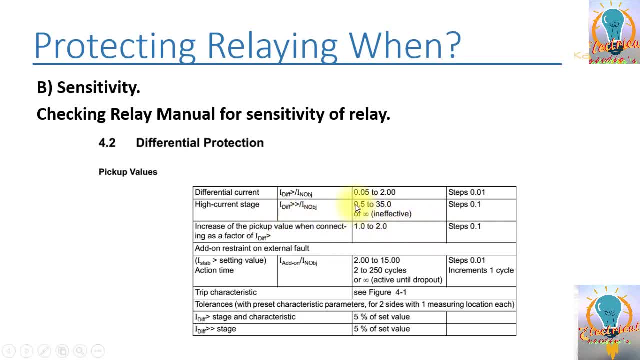 this is the second stage of differential, so you can see the pick up is less sensitive because it is second stage. so it is 0.5 amps to 35 amperes and step size is 0.1. so because this step is designed to detect. 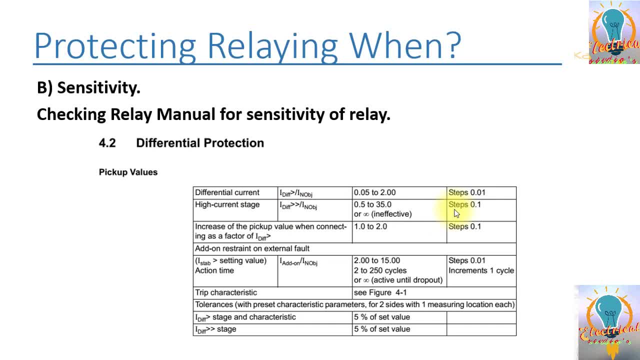 the severe faults and heavy faults, with the fault level can reach up to 20 to 30 times of normal load current, so we don't need that much of sensitivity here. so they have set this sensitivity step is 0.1. so you can see this. 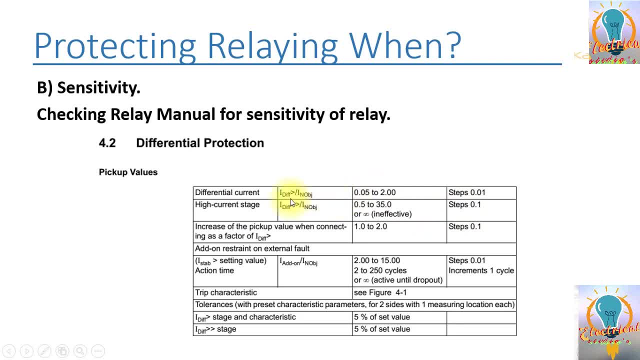 example of differential protection sensitivity. so here you can see some other tolerances are given here. so this is an example how you can check, because basically you have to go to the relay manual and check how the relay is sensitive. so another thing that we can see here is: 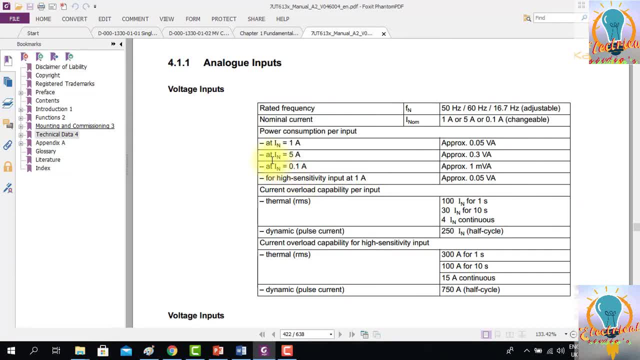 so normally another thing that we can see here is that normally the relay which are used in power system production have their secondary, basically rated current is either 1 ampere or 5 ampere. that is normally used. so in the previous days and the old days the relay was up to 5. 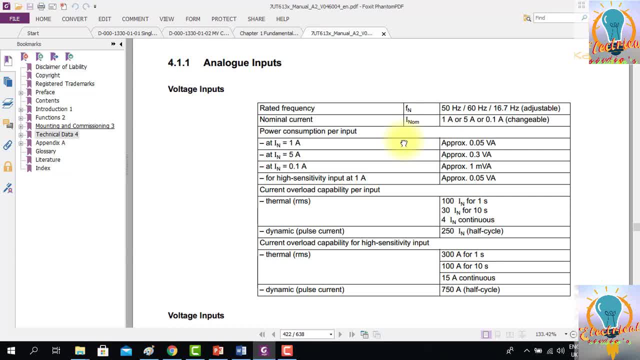 ampere, but in order to reduce the burden, because 5 ampere relay has a higher burden than 1 ampere relay. so here you can see here also that this is 1 ampere and 5 ampere. you can see the burden. this is the burden that we were discussing. 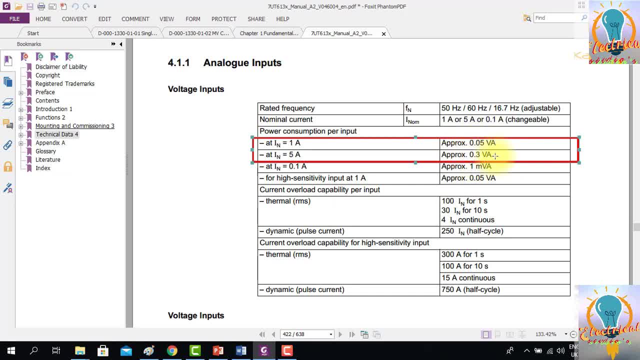 in our previous lecture, the VA. in this lecture that we are discussing that similar to the VA. more is the VA, more is more the sensitivity of the relay. so it means that in the relay there is a previously there used to be NC protect plug settings. so if you 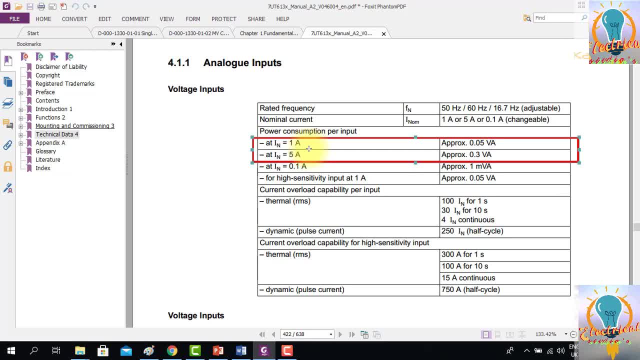 open the relay from the back side, you can change the plug settings and you can change current settings from 1 to 5. so, okay, you have done it. but things that you need to consider is that you need to also consider that now the VA burden of the relay has increased. 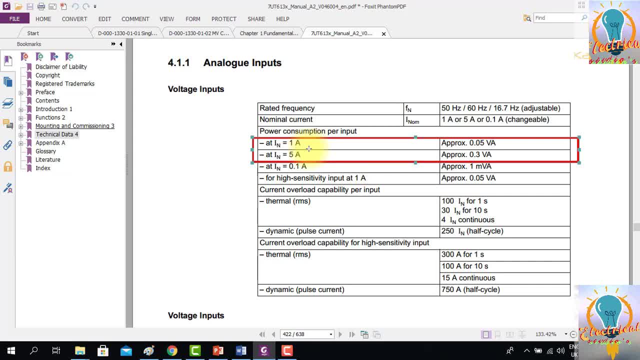 so there is a CT sizing calculation. normally that is performed on each substation, so you need to. you need to recalculate the CT sizing calculations because the VA burden connected to a CT- basically this is the burden on the CT- should be within the limits so that the error should be within the limits. 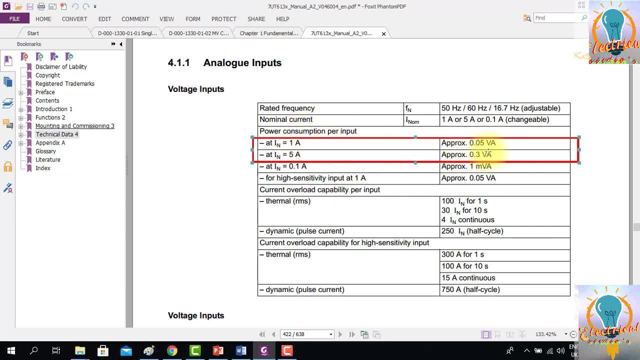 so here you can see the same relay. if you connect it to 1 ampere and if you connect it to 5 ampere, the VA burden is increasing. so here you can check the VA burdens and you can check the sensitivity. so, 1 ampere, same relay. 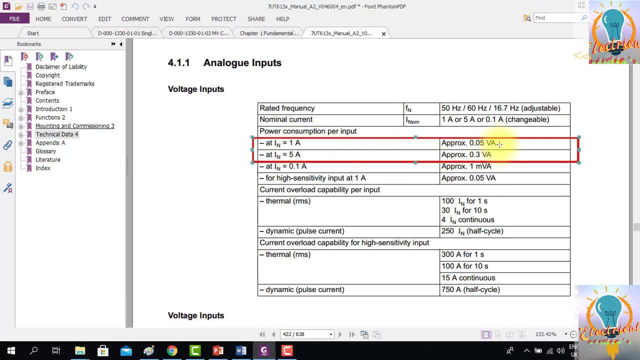 if you select it at 1 ampere, the VA burden is less and the relay will be considered to be more sensitive than the VA burden if you select at 5 ampere, so the relay will be considered as a less sensitive. so if you select the 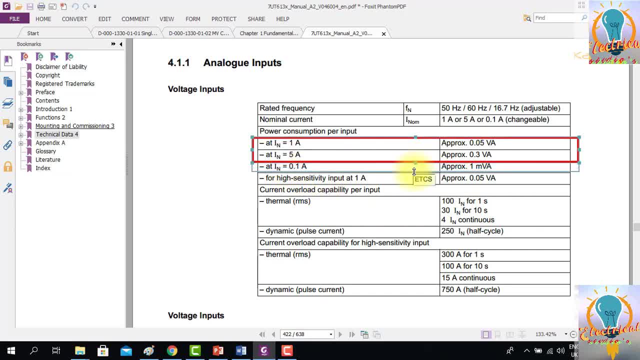 ratio as 0.1. this relay has option of 0.1 also. so the VA burden you can see is even more less. so the relay is very, very sensitive and you can see, for high sensitivity input at 1 ampere there is separate input in the relay for high sensitivity. 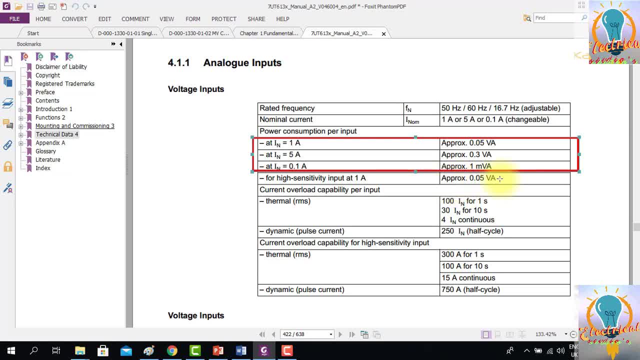 you can see, at 1 ampere it is 0.05 is basically the VA. so this is an example that how you can basically check the VA burden and what is the impact of VA burden on the system. so basically, CT current transformer in each substation is connected to the wires. 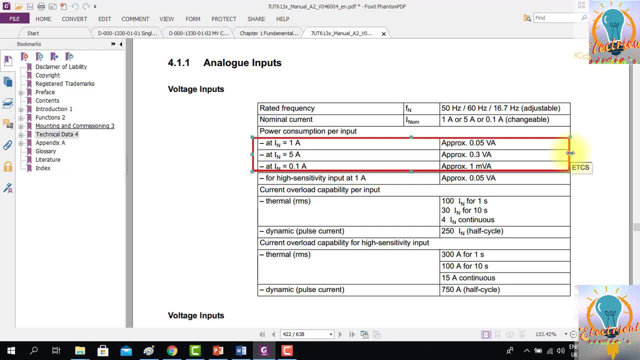 and connected to the relays, and each relay has its VA burden and each wire. if the length of wire is more and the dia of the wire is less, the VA burden will increase. so all the VA is calculated and then, based on this calculation, CT size is calculated. 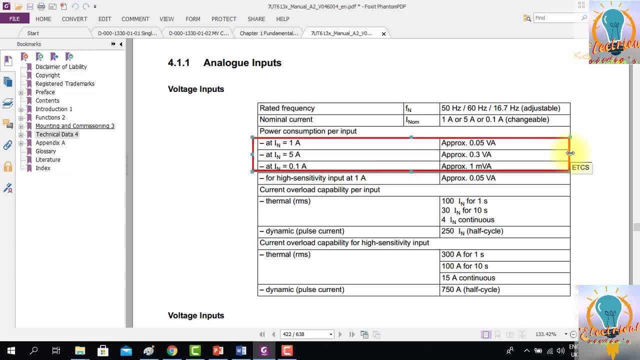 so if you are using relay, which is cheaper but it has more VA burden, so at the other end you have to select the CT of a bigger size which can support the VA burden. so you have to take care all of these things in the substation while you are designing. 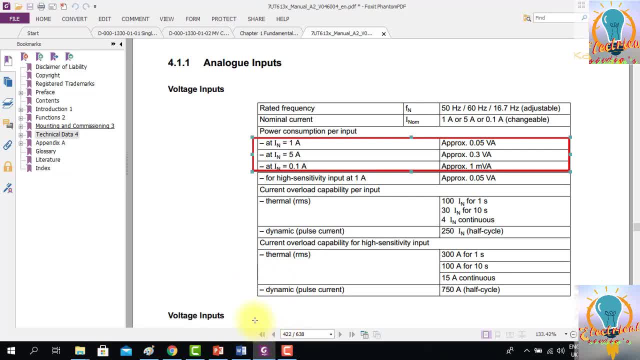 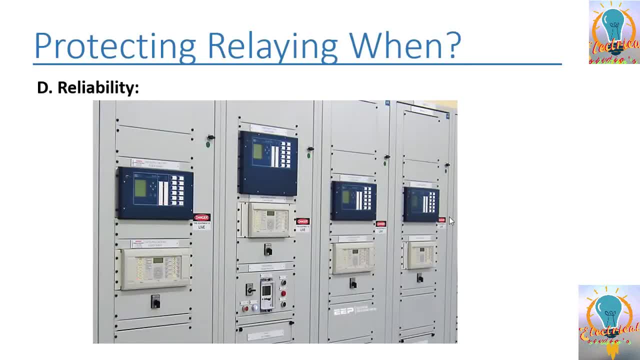 so this is some concept about the sensitivity. so I hope that you enjoy my lecture. thank you very much, Hi friends. next topic is reliability. the system should be reliable enough. it means that in case of fault it should always operate. it should not happen that sometimes the relay operates and 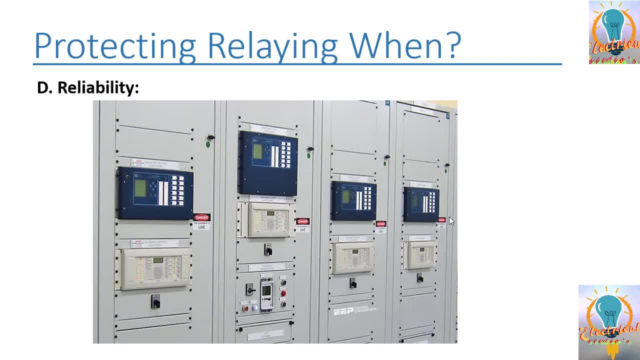 sometimes it did not operate. so reliability is one of the key factors. so what is a normal practice of utility is that whenever an vendor is bringing, or manufacturer is bringing its new relay, if wanted to use in a network, so they are keeping this relay as an- you can say- duplicate. 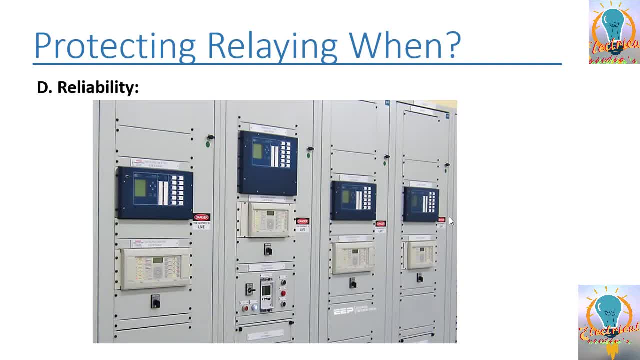 protection with existing feeders, which is prone to frequent faults, and then they are checking the performance of the relay on this feeders and after years, they are giving the approvals to use this relay on the network. so it's a lengthy process and that's why it's very important. 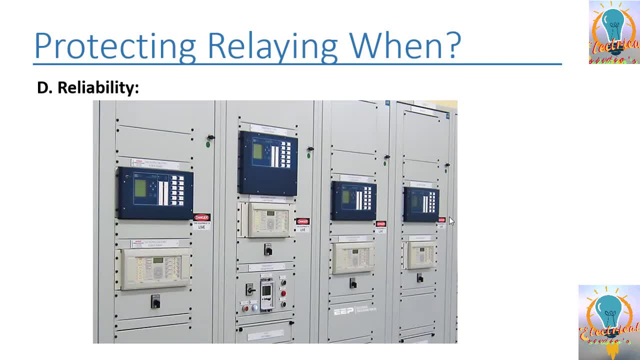 to have reliable protection relays and the scheme also should be reliable enough to work properly in in the system. it is a reliability of the relay system to operate under the predetermined conditions. without reliability, the protection would be rendered largely ineffective and could be could even be become a liability. 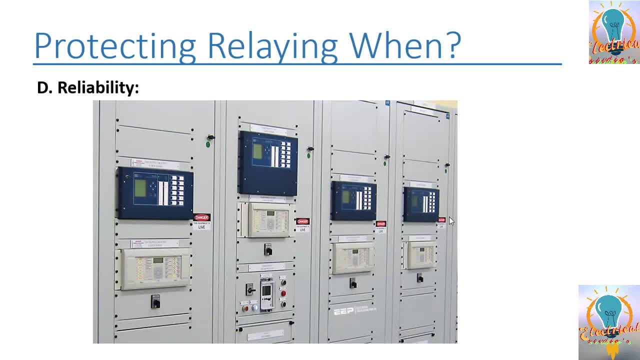 so the reliability is always a key part. so in order to check the healthiness of the relays- that's why, each year or as per prescribed maintenance plan, annual maintenance or five-year maintenance relays are keep- we are retesting the relay to check the healthiness. 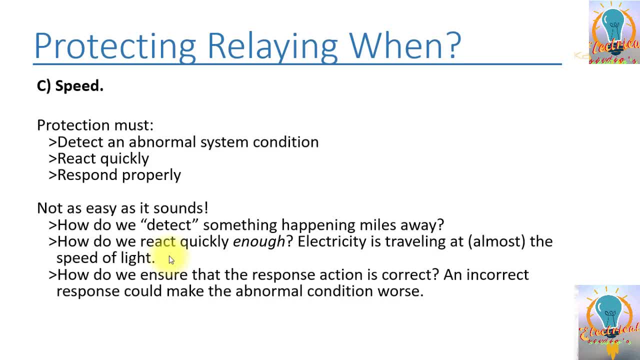 of the relay. thank you very much, hello friends. now the next important characteristics for the protection relaying is basically the speed. the relay should be fast enough that it should detect the fault and the deduction should be as fast as possible. then it could be basically react. it could. 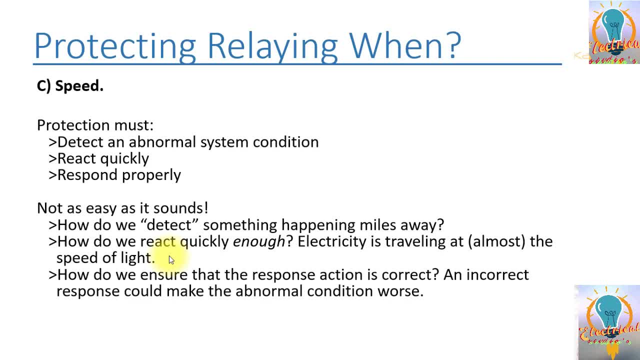 quickly decide and then respond properly means. first step is basically each relay speed with the some actuating quantity like voltage, current or frequency, etc. and then the relay basically converts this analog quantity. now, modern days, relays are converting this quantity into a digital quantity and then, after converting it into 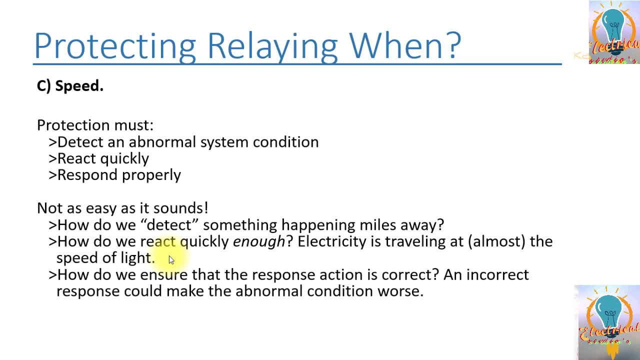 digital. they are using some comparators and then checking. they are checking the set value versus actual value, and if the limit is, if the observed quantity is more or less than the predefined set limit, then it has to take the quick action. so the relay then issues alarm. 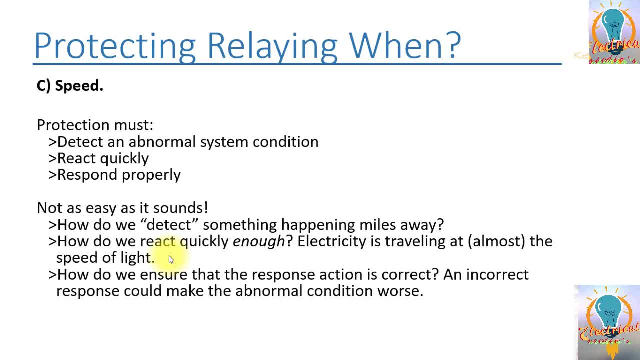 trip commands or LED indication as programmed, and then this is called another speed. so the speed is very important. if the relay is slower to act, then the backup protection will operate and that will result in tripping on basically the major area. so fault will not be localized. so more region. 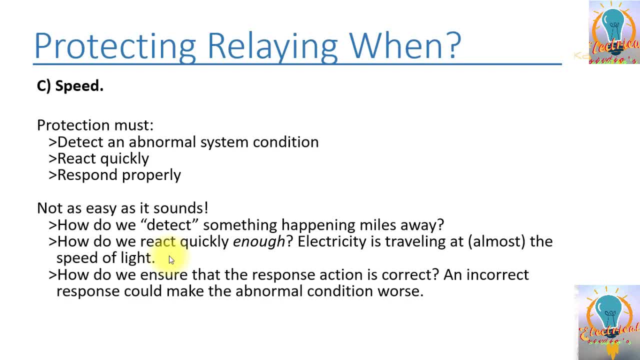 will trip. so this is always important to check the speed of the during commissioning time. what we are doing is that we are putting the setting in the relay- for example, in distance protection, zone 1 is instantaneous- and then we are simulating a fault in zone 1 and then we are checking the time. 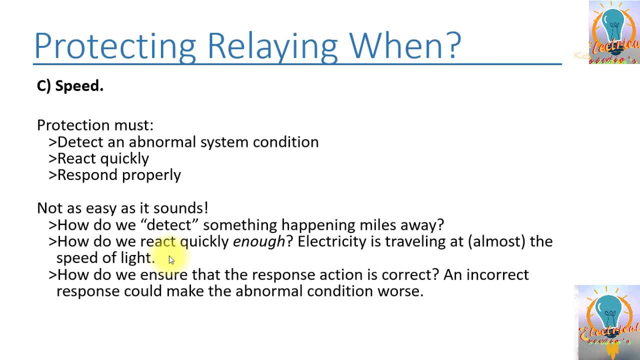 of the relay that how much time it operated, and we need to check this time in which the relay operates. it should be within the predefined limits or within the tolerance. so this tolerance you can find from the relay manual. each relay manual is giving the tolerance of the 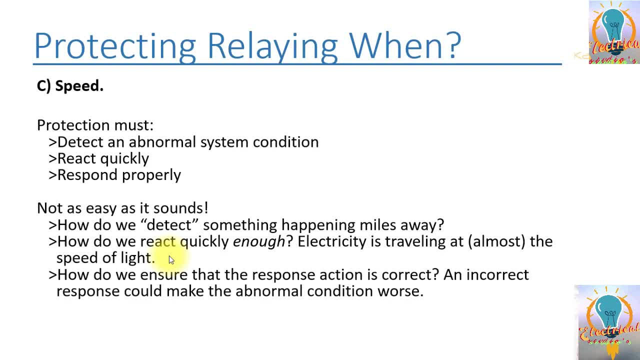 relay. if the fault operating time of the relay is beyond the tolerance, then you need to replace the relay. basically, but it's not as easy as as you think. how to we detect something happening miles away? how do we react quickly enough? electricity is traveling at almost at the speed of light. 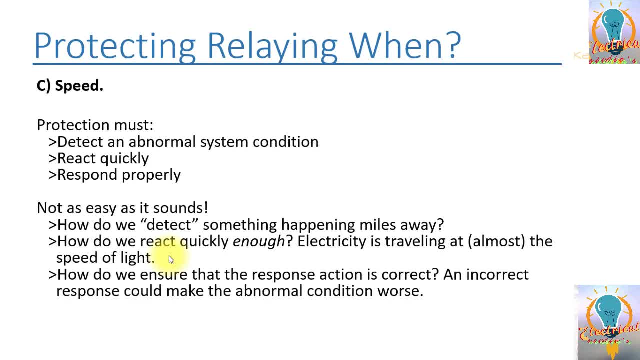 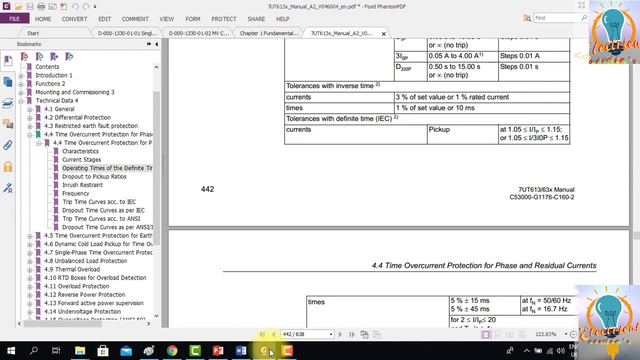 how do we ensure that the response time is correct, and incoming response time could make the abnormal condition worse. so some of the questions i have already answered, so now i will take you to the relay manual. so here you can see this is the over current, protection over current and. 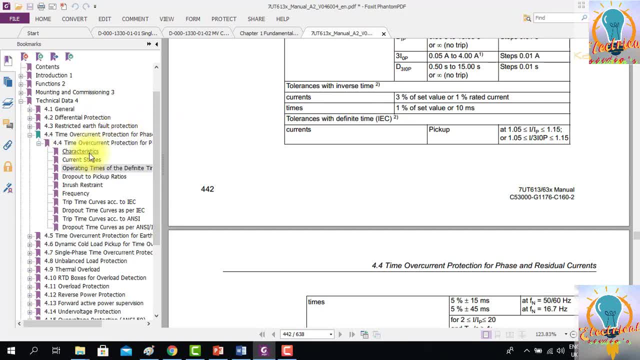 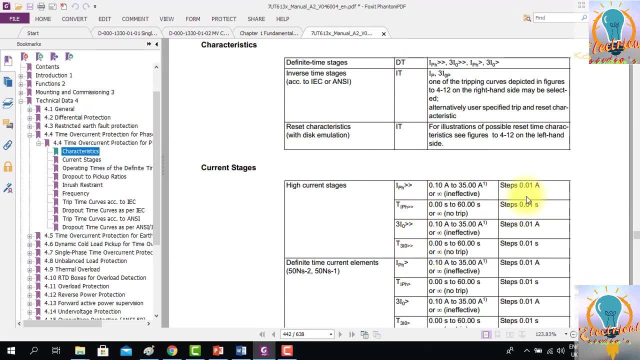 phase residual current protection. so they have defined here some characteristics. as i told you, they have defined the steps in each step. you can increase the pick up and this is the step for time: 0.01 seconds. so you can increase the time also. then we have current stages. 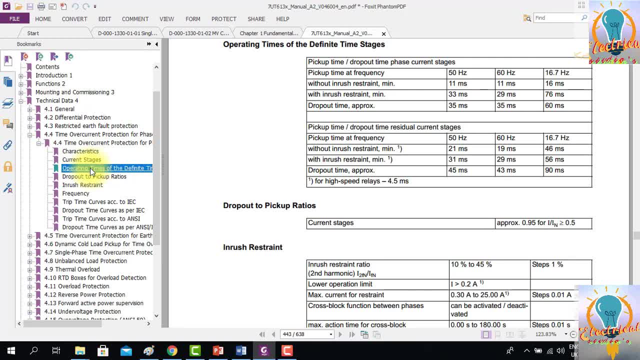 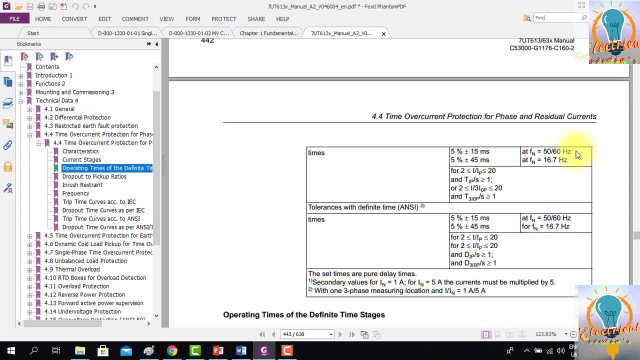 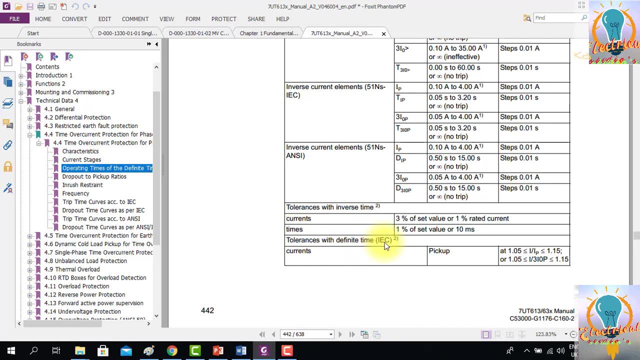 then we have operating time of the definite time. so here you can see they have defined the tolerances with definite time as per IEC. so these are the tolerances are within the IEC defined standard. so the pick up current they have shown should pick up. 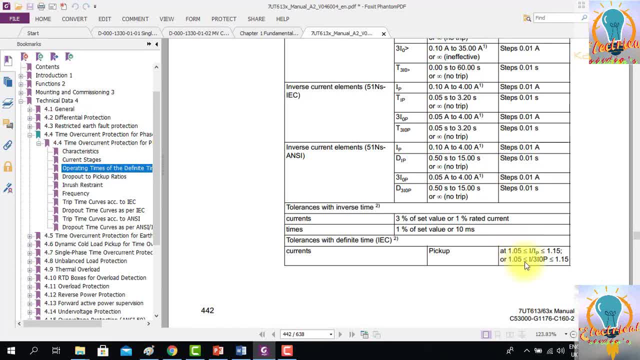 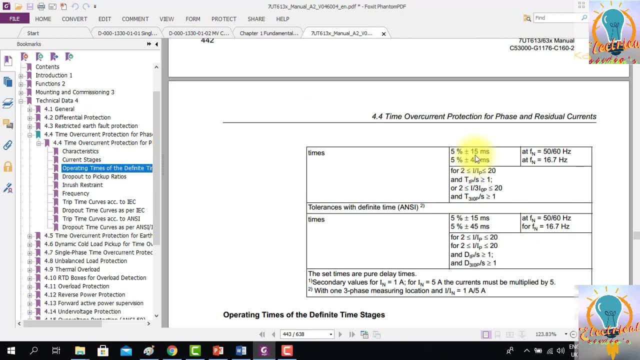 at 105 times the set value means 5% to 15% relay should picked up and this is the time tolerance. so 5% plus minus 15 milliseconds is the time tolerance and at frequency of 50 to 60 hertz and if the frequency is 16.7. 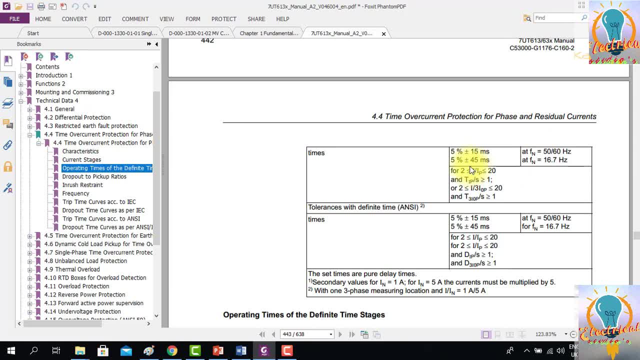 hertz, then tolerance is 45 plus minus 5% of the set value. so this is basically the tolerance. the result should be within this tolerance. so you can find all these tolerances in basically the relay manuals and this should be as per IEC relevant standard. 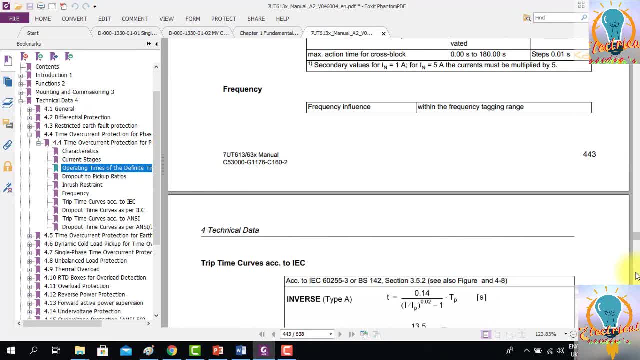 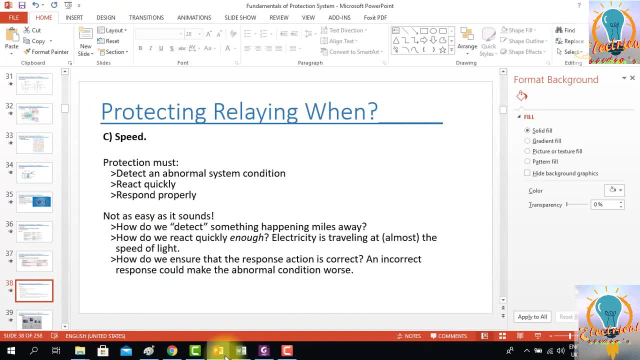 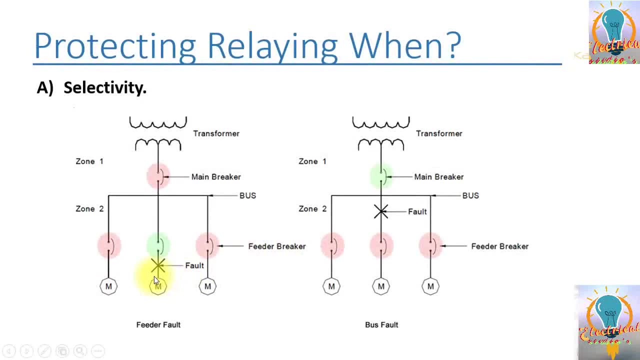 IEC2. so let's go back to our slide and if you can see here again the example: if, for example, there is a fault on the line and the trip time of the relay is 100 milliseconds of this, this relay has a trip time of, for example, 100. 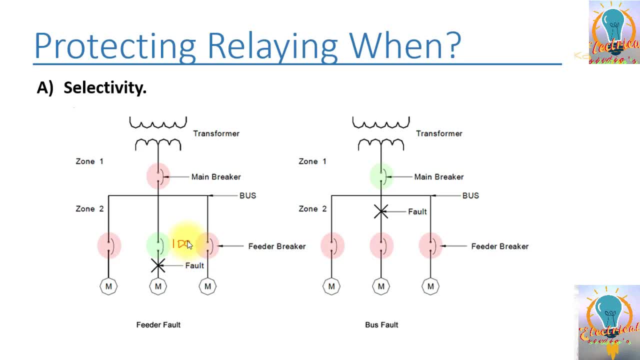 milliseconds and this relay has a trip time of 200 milliseconds. ok, so now there is a fault here. so if the relay is operating fast, so it will trip within this time. so let's see: this time plus relay operating time the relay, for example, will trip. in this case is even. 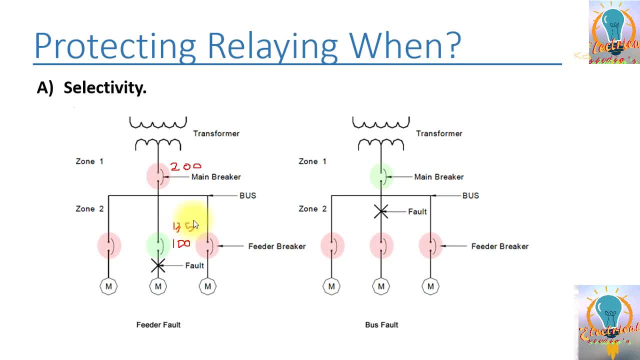 35 milliseconds. so 35 milliseconds relay takes the time to trip and 100 milliseconds is the preset time delay. so relay trip it in 135 milliseconds. and the timer of the encumber was 200 milliseconds. so the encumber will not trip and the outgoing feeder will. 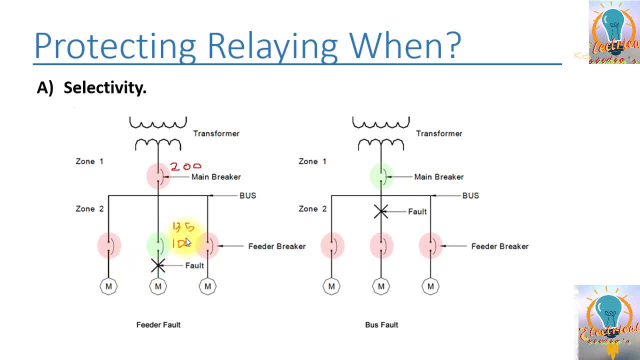 trip. now consider example that relay is slow to operate so there is some problem in the relay so relay take, instead of 100 milliseconds, 35 milliseconds. relay took now 300 milliseconds to operate so there is some issue in the relay software so relay is taking 300 milliseconds. 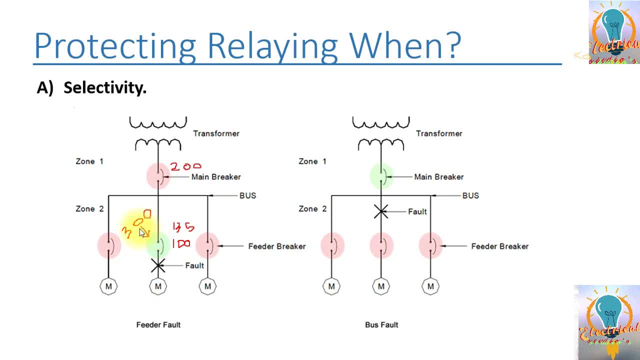 relay is slow, so only it's slow by. you can see 200 milliseconds. so you can see encumber setting is 200. relay is tripping in 300 so encumber will trip fast. when this encumber trips you can see all this area will be shut down. 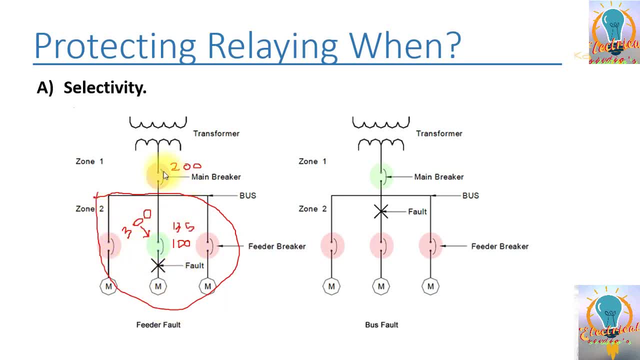 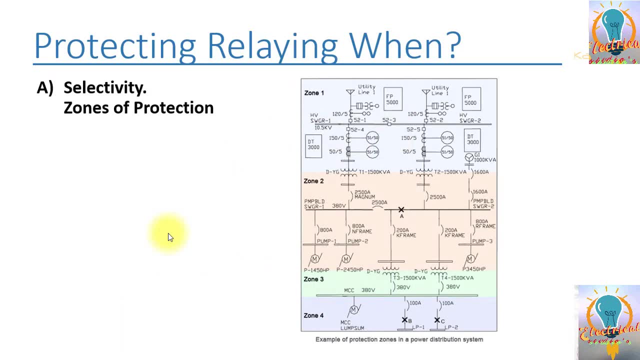 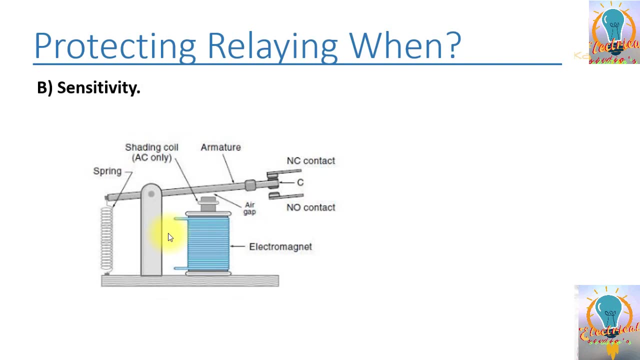 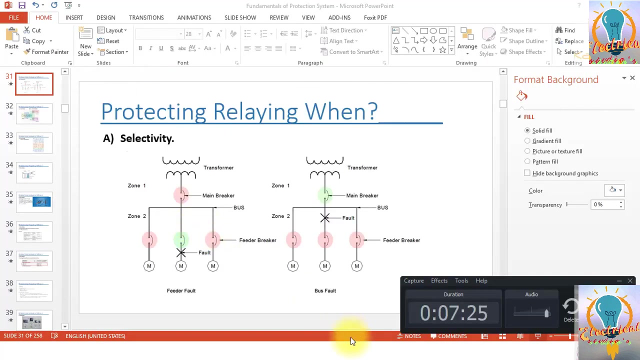 so the speed of the protection is very important. it should be coordinated and speed should be good also. so this is an example of speed that you need to consider. so now we can move to our new topic. thank you very much. thank you very much. another key factor: 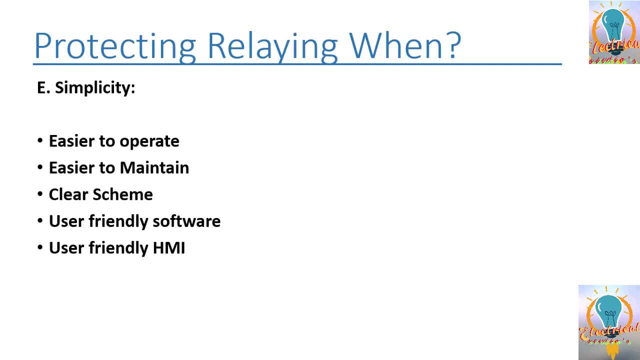 for the good protection system is simplicity of the protection relays and protection systems, so it should be easier to operate. for example, in a utility, I have experienced that they were preferring a specific type of relay by a specific manufacturer, even though it was expensive, because they used to say: 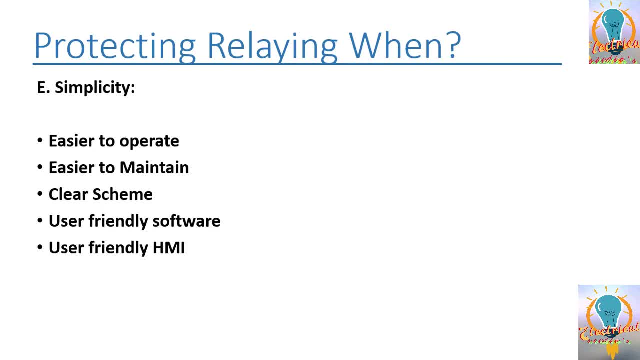 that it's very easy to operate and very easy to maintain. so simplicity is one of the key factors, and it should be easier to operate and easier to maintain. for example, if a vendor is providing a transformer or a GIS, that is very perfect, very reliable and cost effective. 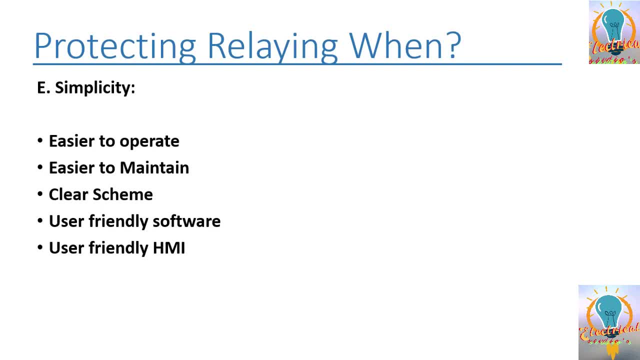 but it's difficult to maintain means if you have to do the maintenance, you have to open lot of parts and even there is no access to some parts of the transformer or GIS, so you need to dismantle complete base to access certain parts. so maintenance point of view, 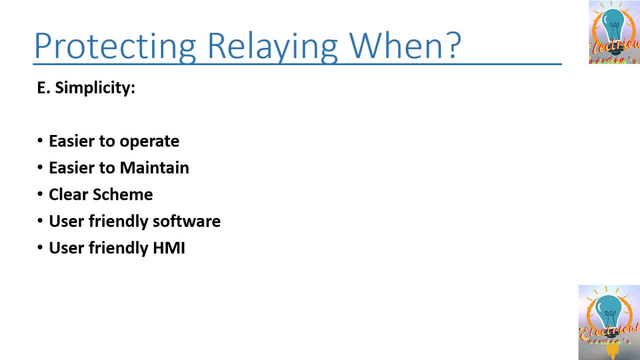 the simplicity also should be there. scheme should be very clear and easy to understand. some of the production schemes in my career I have gone through and I find out that these are very complex schemes and during commissioning it will increase the commissioning time, obviously, but for 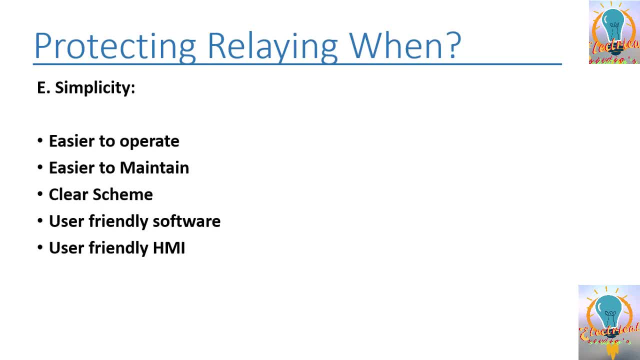 maintenance point of view. if there is a fault and if you need to troubleshoot, then it will be. it will increase the time of fault troubleshooting and rectification and analysis. so the scheme of the production scheme should be as simple and as effective as possible. the softwares nowadays 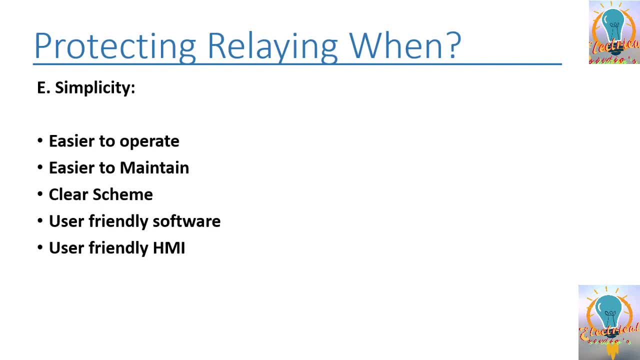 most of the relays are numericals and even the softwares are used to communicate, send the settings and receive the settings from the production relay, even to download the fault records, the software. now there is a concept that software should be user friendly and easier to operate. so these are all. 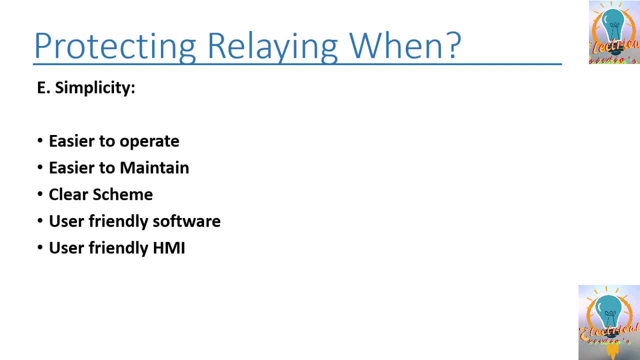 the requirements nowadays from the new utility also the user friendly HMI. HMI is basically: if you are facing a numerical relay, there is a display on the HMI. it's really nowadays. the display should be user friendly. if you don't even have a laptop, it should be easier to operate. 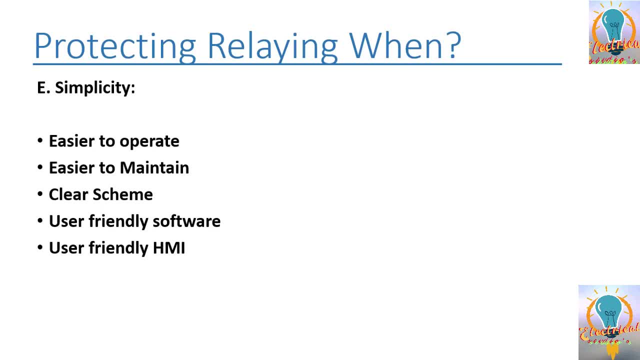 and you should be able to easily see the fault records and the events and alarms and the settings. if you want to change the settings, you should be able to change the settings from the HMI itself. so these are all the basic requirements nowadays for a good production. 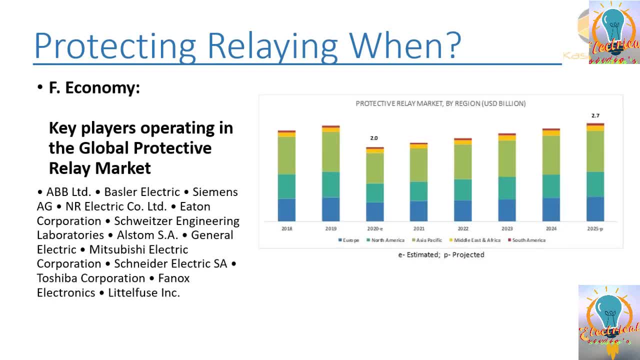 systems. thank you very much. nowadays there is a lot of competition in the market and market is becoming more and more competitive, so the cost is always one of the big, big component whenever you are selecting a production system or production relays or production equipments. so economy is one of the key. 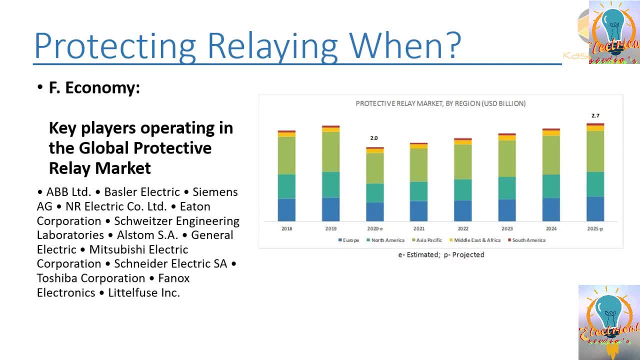 factors. I have gone through certain clients that they are preferring a new relay even though that the new relay is not that much user friendly. but they don't have a big budget so they are preferring the new relay because it's cost is price is less, so the 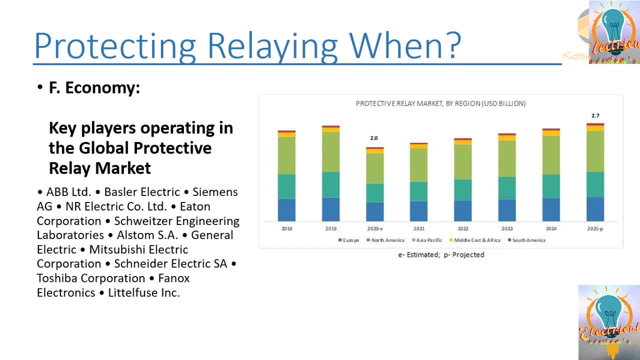 price is always a key factor, the ideal production system that we should consider and design a production system, we have to also consider the issue of price and the cost. so nowadays the key players in the global market which are very famous in the production system are ABB. 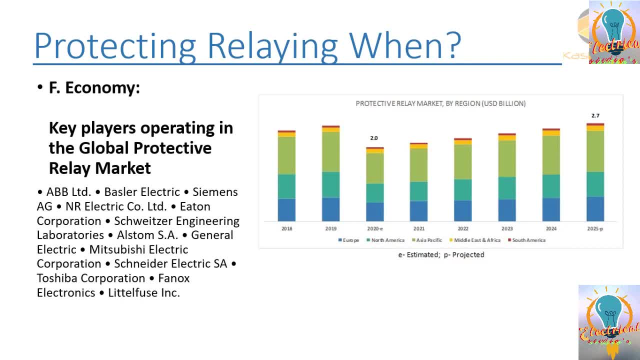 for example, Besser Electric, Siemens AG, NR electric company, Eton, SCL relays are very famous: Alastrom, General Electric, Mitsubishi Electric, Schneider Electric, Toshiba, Fanox, Littlefuse. I can see the estimated basically and the projected. here you can see the productive relay market by region in US dollar. 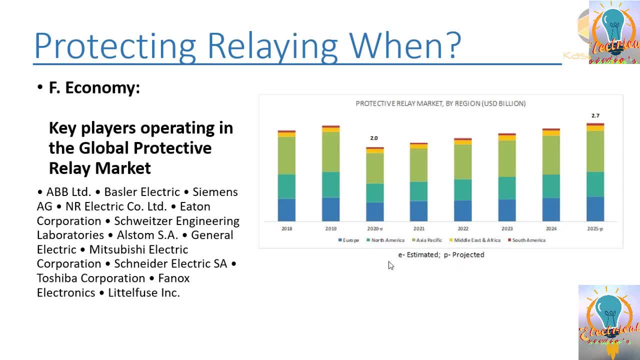 billion US dollars. so each region is shown with different colors. so here you can see: Europe is shown by blue, North America is by this cyan color, Asia Pacific is green, Middle East is yellow and South America is red. you can see easily. the asia pacific is is basically the highest at the moment, where 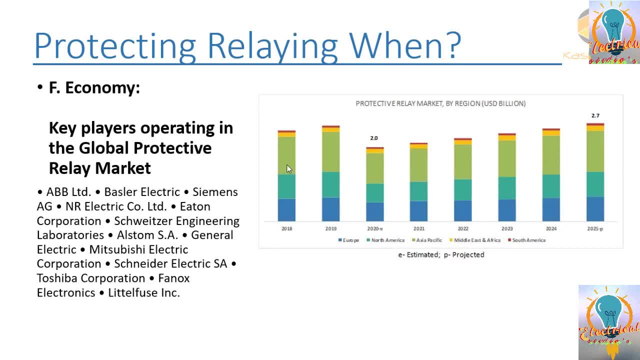 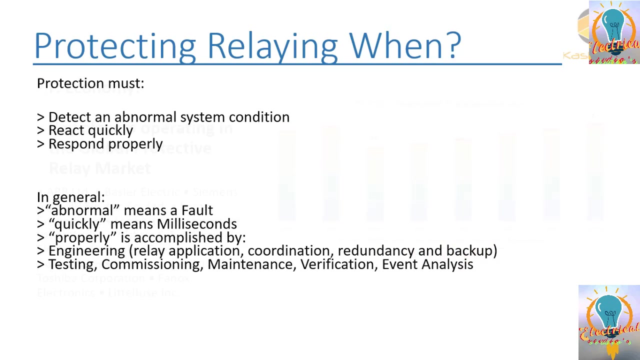 the highest investment is being done in the production systems. and then it's north america and then europe. this is yellow color is the middle east market and this red is south american market. so this is a serious business and it's one of the very important aspects of this energy. so this is 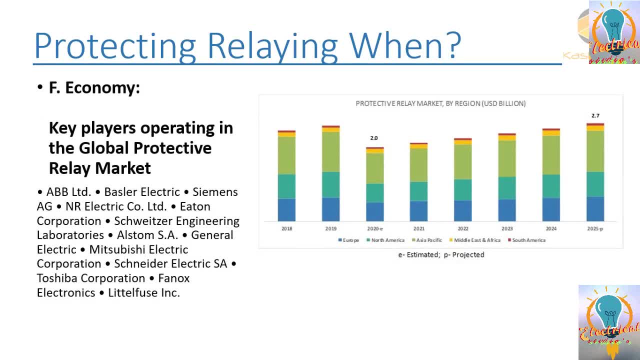 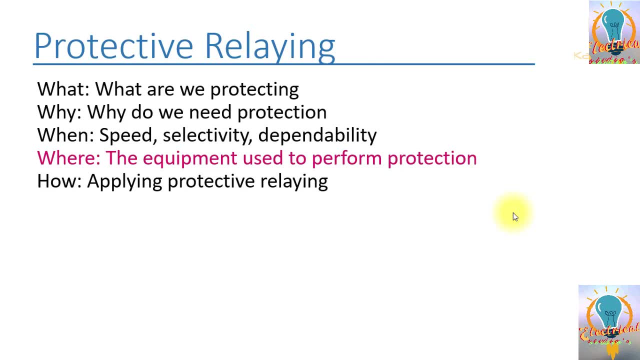 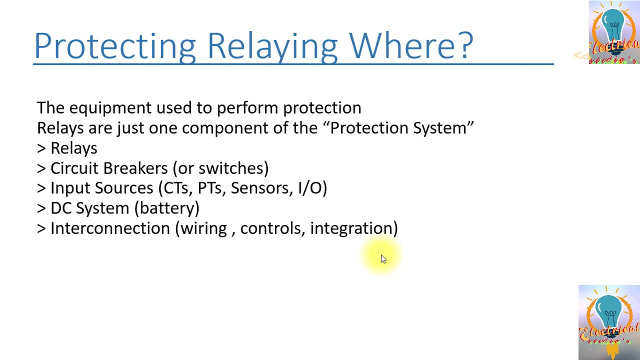 also an aspect that we need to consider when we are designing production system: the cost. thank you very much, my friends. in this section we will discuss that: what equipment is used to perform protection. so let's start. so the equipment that's used to perform protection. relays are just one component of 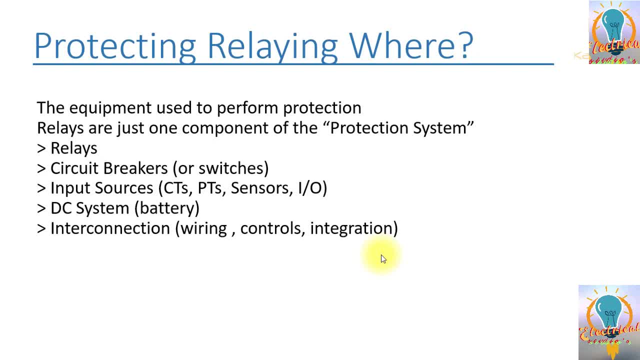 power production. so the relays are just one component. so there are other components also that we are using, just like we are using of uh that then release our circuit breakers or switches. basically we are using switches, we can say isolators, we have bus parts, so we have. 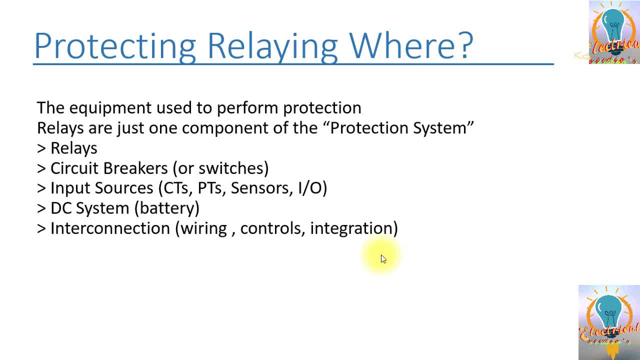 silencers, lighting resters. we have input devices like cts, current transformers, potential or voltage transformers, sensors, input and output devices. we are using dc system batteries. we are using interconnections, we are using wiring control integration. there are a lot of more factory devices, control devices that are being used. 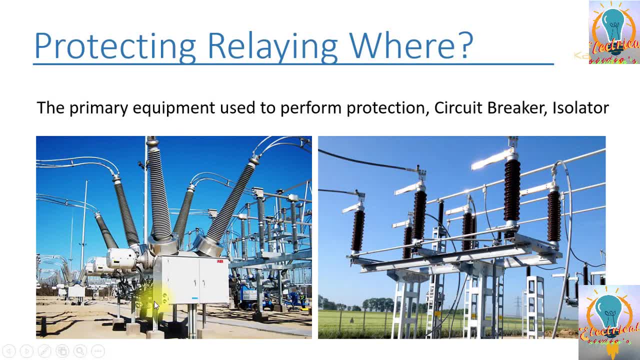 so here you can see, this is basically the circuit breaker and it is an uh air incidents substation. it is an ais- this area we are calling as a switchyard, and this is basically the box near to the circuit breaker where the mechanism and the terminal interconnections are installed. 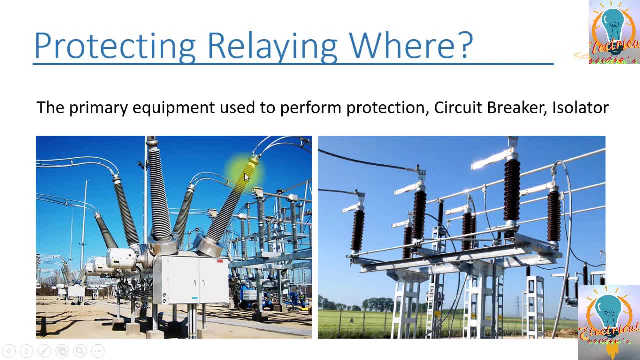 in it. this is called as a bushing of the circuit breaker and this is the tank of the circuit breaker and this is basically a picture of isolator. so these both equipments are used in protection systems. isolator is used to isolate. if you want to perform maintenance, you are you. 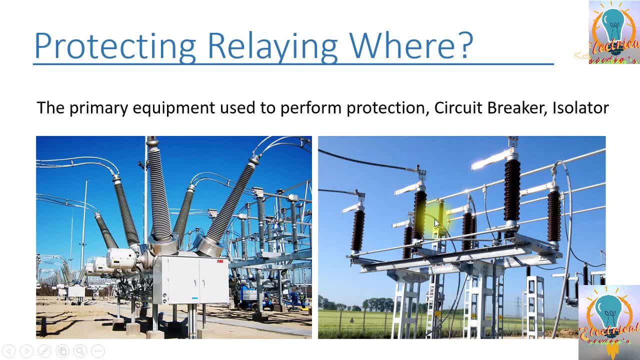 have to first open the breaker and then after that you are forcing. the isolator reason is that in the breaker you cannot see physical movement of contacts and the separation is not enough to perform any maintenance. so that's why, always with the breakers, you will find isolators where you can. 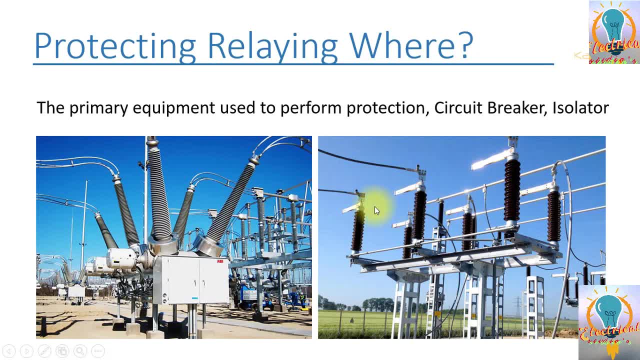 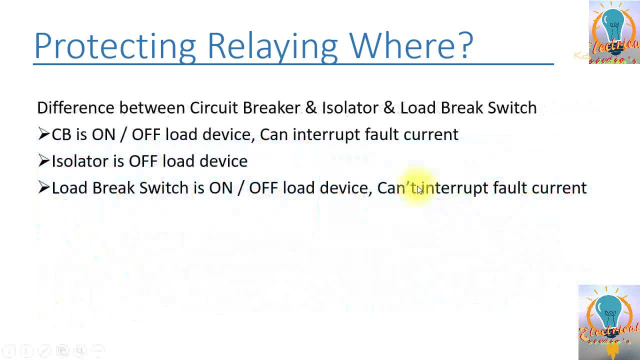 perform. if you want to perform maintenance, you have to open the isolator and then you have to connect the earth to the relevant portion. so what is difference between circuit breaker, isolator and load break switch? so we will discuss now. basically, circuit breaker is on load off load device. it can 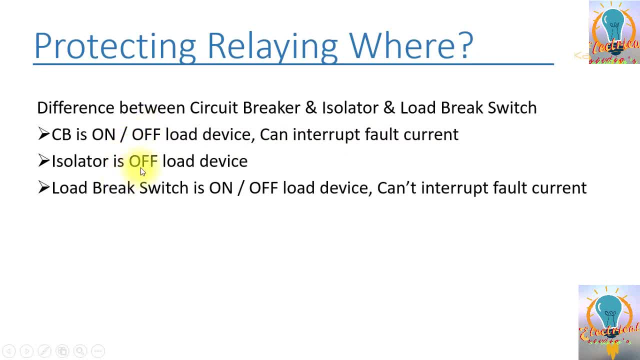 also interrupt the fault turn so and there is the isolator device. means you cannot operate isolator if there is a current flowing through the circuit. then there is a load break switch, load break switch which is on load or off load device but it cannot stop the 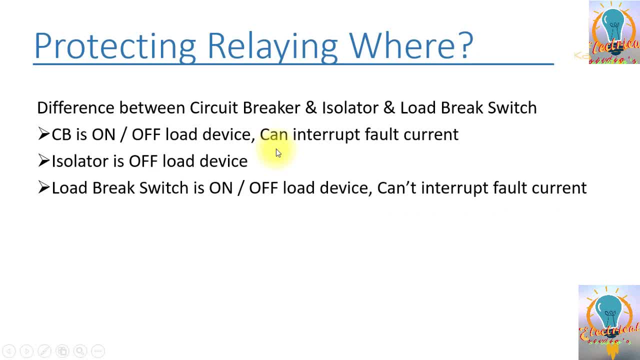 fault. so circuit breaker basically, whenever a circuit breaker can be operated without loads, which load and also it can interrupt the salt grant, circuit breaker is basically also dare it to commands automatically in the case of all from the release and there is a fall level, fall fault is directed from the release, it is the trip command. 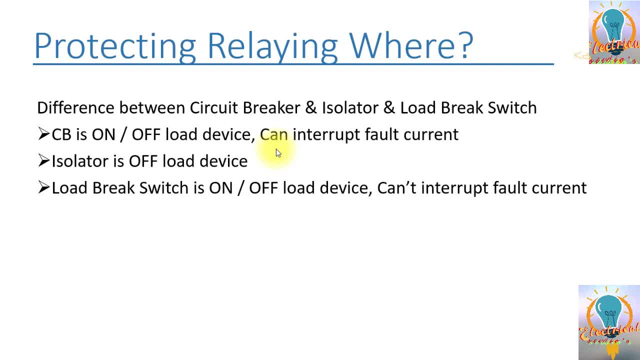 relay will issue the trip command, it will be received by a circuit breaker and the circuit breaker will open and it will interrupt and it will break the fault current whereas load breaks, which is basically, you can operate it offload, you can also put it on load, you can break the load, current load, current level. 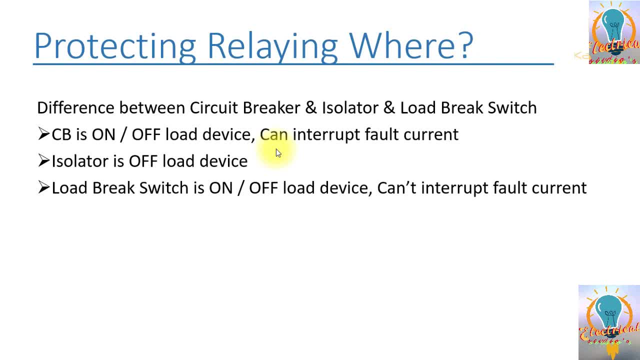 is always is limited. for example, it could be 10 ampere, it could be 50 ampere, 100, 200, 500 amperes, but whereas the fault current level is always very high, mostly in kiloampere, so the load current is designed as per load and it can break the load current. 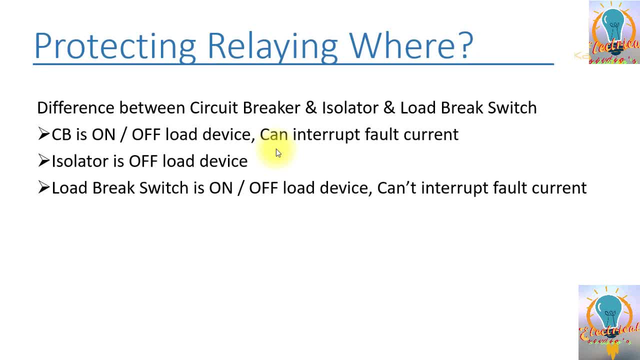 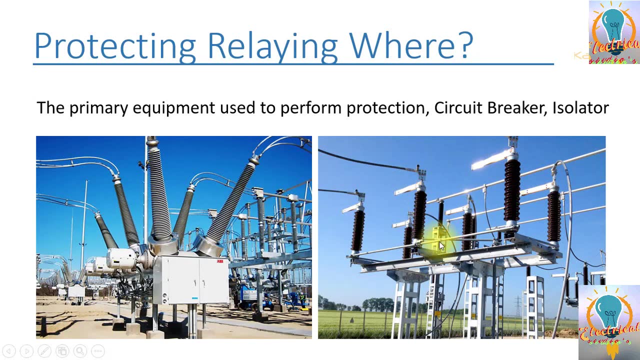 but it cannot operate automatically. it cannot interrupt the fault current until the fault appear in the system. so normally each substation, if you want to operate the isolator, it is necessary that first of all you have to open the breaker. if the breaker is open, then only you can operate the isolator. 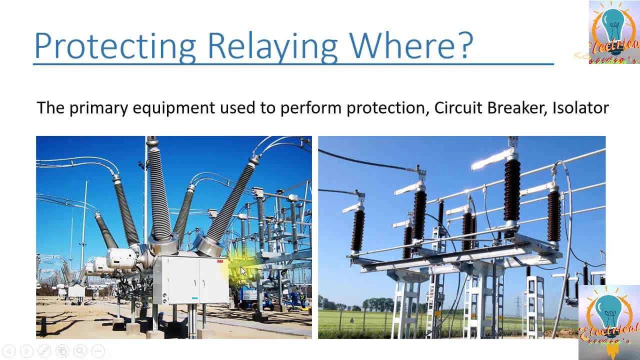 so there is a interlock available between breaker and isolator. there is an electrical interlock. there is auxiliary contact of SoC which is wired up through the control circuit of isolator. if the circuit breaker is closed you cannot open the isolator. so there is a interlock in between them. 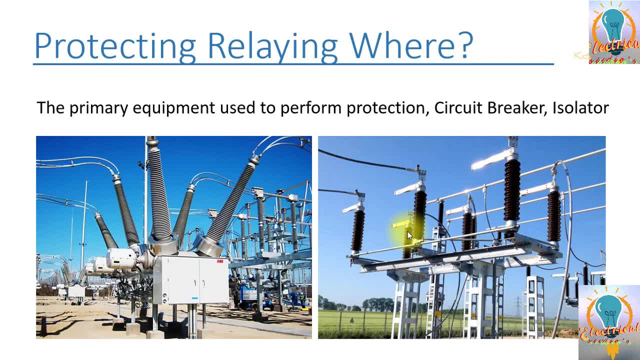 so that's the difference. little difference about circuit breaker Granule de Betten, Unknown breaker isolator, and the load break switch, The switches we are using in our house to switch on and off. the lights are example of load break switch where you can use it off. 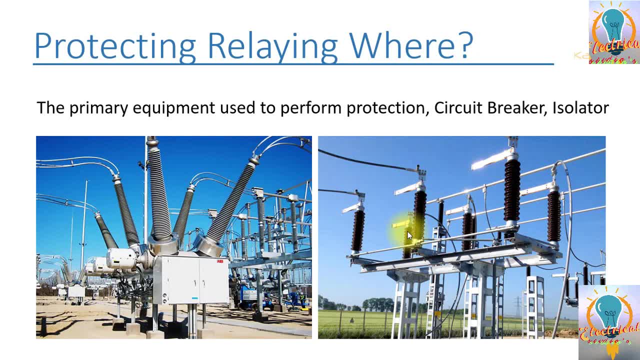 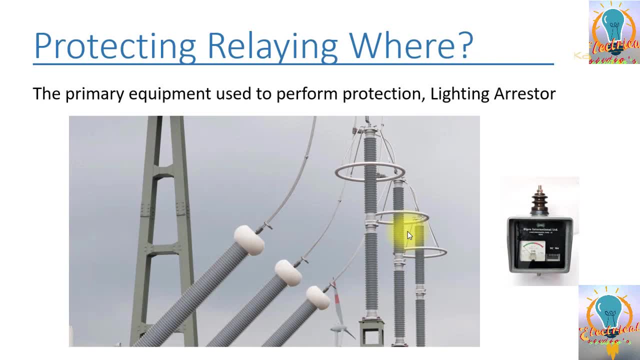 load. you can use it on load, but it will not operate automatically. You can also break the load current. Here you can see another primary equipment that is used to perform the protection. It is basically the lighting arrester. Here you can see, this is the picture of lighting arrester which is stored on a post, on the post pole. 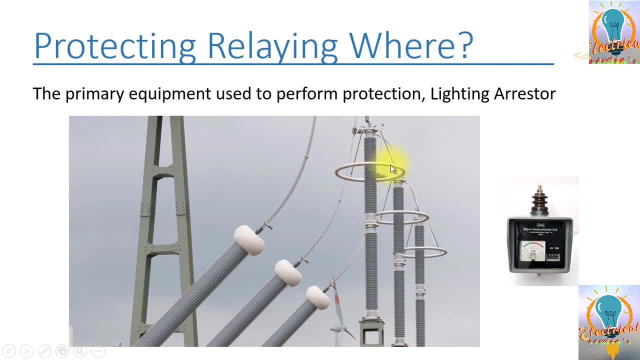 and this ring is basically the corona ring and the purpose of this ring is to distribute the voltage across this disk equally. If we are not putting the ring here, there will be more stress on the upper disk than the lower disk. So this disk 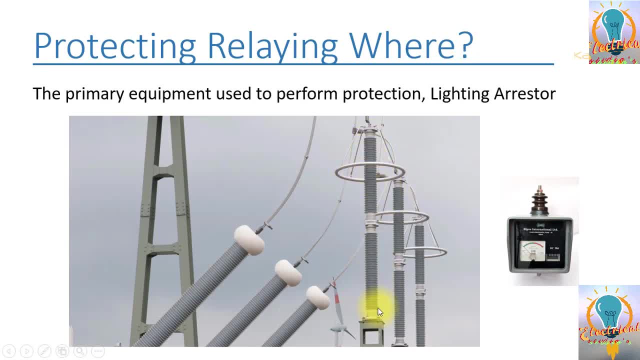 is distributing the voltage stress equally over the charger arrester. So this is the purpose of this disk and you can see this one. This is basically the counter search counter Here. you can see in this display. this is showing the leakage current in milliamps. 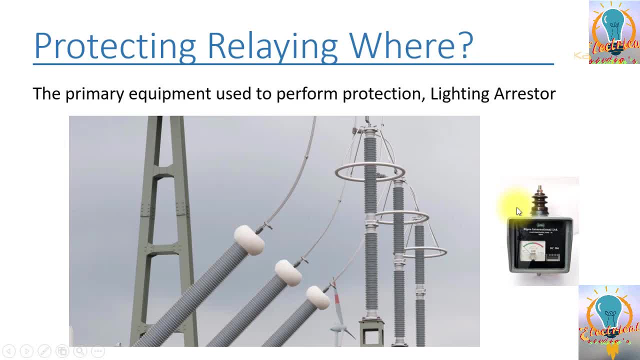 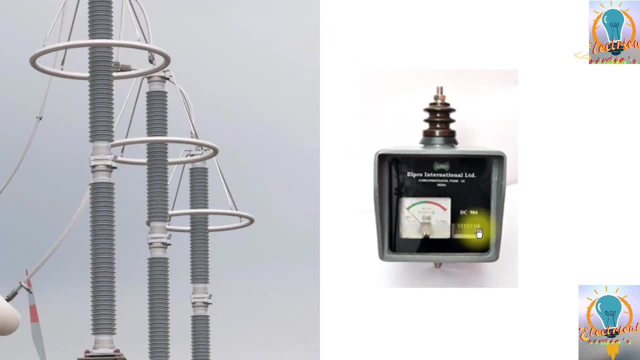 and this is the counter which is showing basically. This is basically the search counter. You can see how many of surge are grounded through this And this portion will be connected to the reopent side and the downside portion will be connected toу earth board, As you. 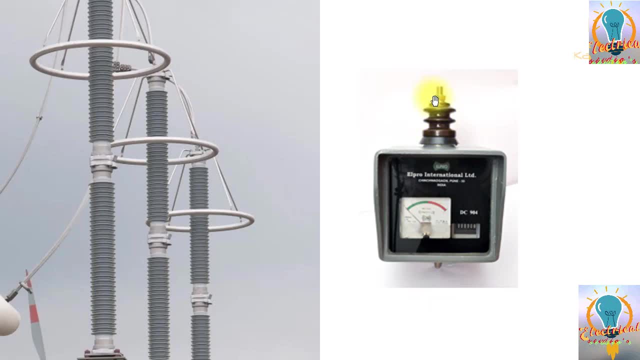 can see, you have to connect an insulated wire from this terminal to the心oprent. If you are not using insulated wire, do not connect any of them. To connect the connected the, you have to connect the two wires on the driver side And the arm Cafray went away aswell. ai note. 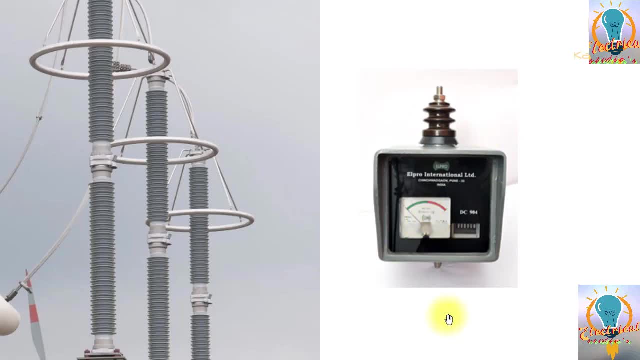 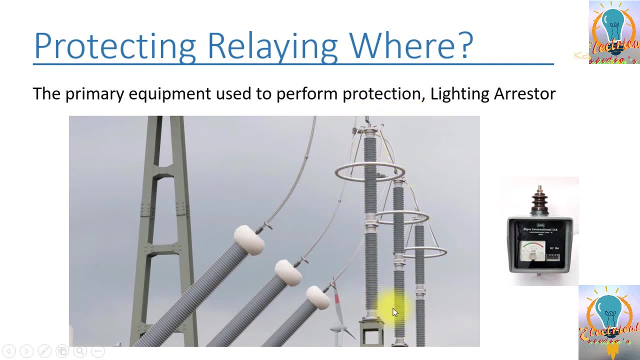 wire, the surge will be grounded directly and this counter will be bypassed. so what is the purpose of surge resistor? basically, surge resistor is nonlinear resistor. it mean at the low voltage it have infinity resistance and at the high voltages- extra high voltages- resistance is reaching to minimum and it is then. 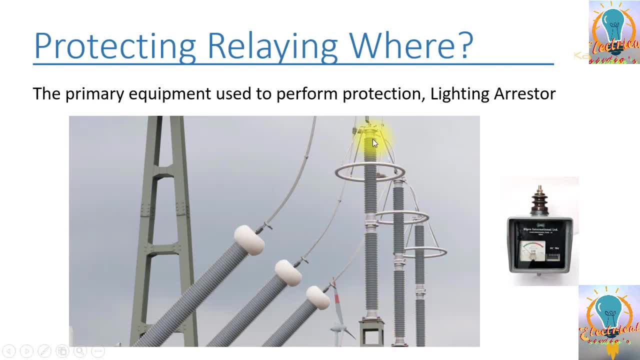 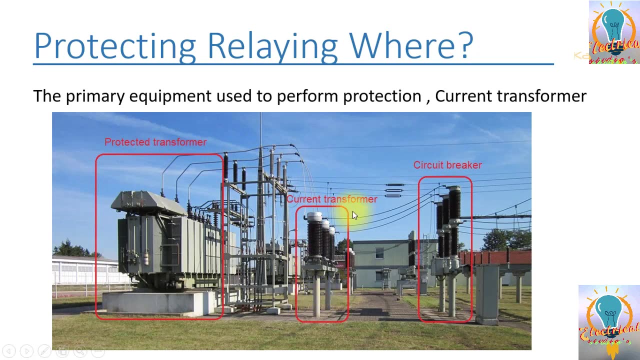 grounding the surge. so this is a very important equipment to ground the surge. normally it is made up of, you can see, by zinc oxide. here is you can see the other equipments. this is the current transformer that we have discussed. if you go to the substation you will see the current transformer and the 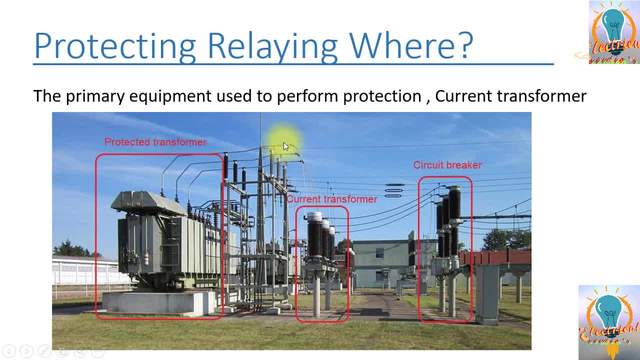 current transformer will be look like this. so how you can differentiate it, you can see there is a one cable coming in and one cable coming out, so current transformer is always put in series. so this is the connection of current transformer. so this is basically our input is providing an input to protection relays, control relays and 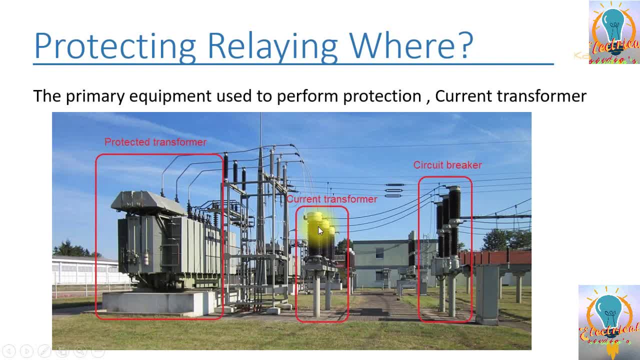 measurements. the current input will provided through this. this is the circuit breaker you can see. one is connecting to the top, another wire is connected to the bottom and in between there is a interrupted unit. there is a moving contact. so they have provided enough space and this. you already know that this is a transformer, which is used to step up and 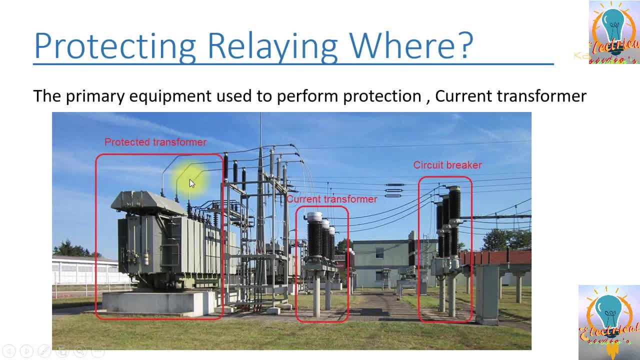 step down the voltages. so here you can see, this conductor is a hollow conductor and this is a force insulator. and here you can see they have installed here again the suggestors and through the CT, this wires are connected. this is an another example of the equipment that we are using for the production of substation. here you can see on the 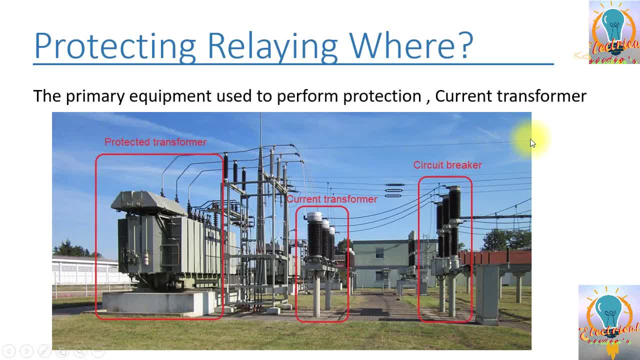 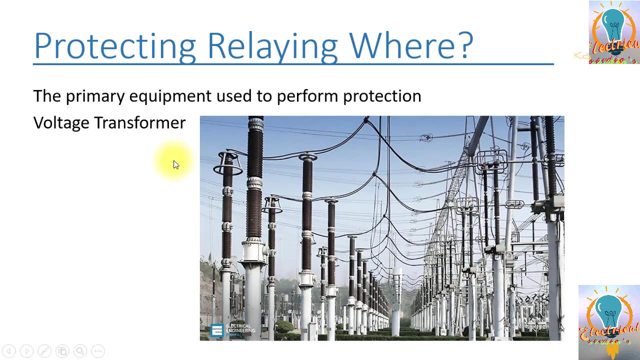 right, this wire is available and this, this basically lightning must. it is protecting substation from lighting. this is overhead shield wire and here this rod you can see is basically the lighting rod. it is protecting the substation from lighting also. so this is another protection. so here you can see the primary equipment: the voltage transformer. this is 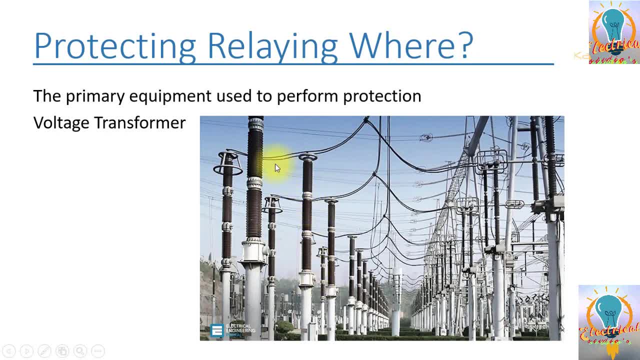 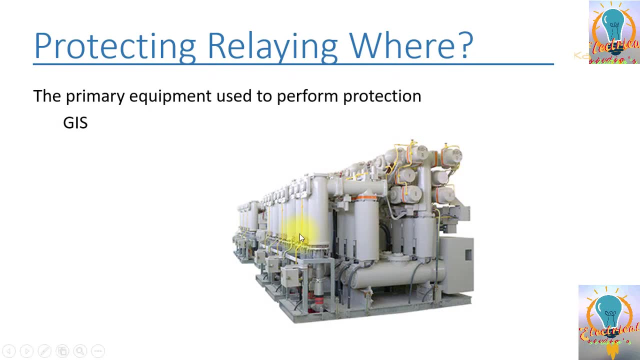 basically the voltage transformer. this one. these are the VTS connected in the substations and this is I have shown you our gas insulated substations. in this one, all the equipment that we have seen previously was outdoor. it was a air insulated AIS, but this one is gas insulated and we are normally using. 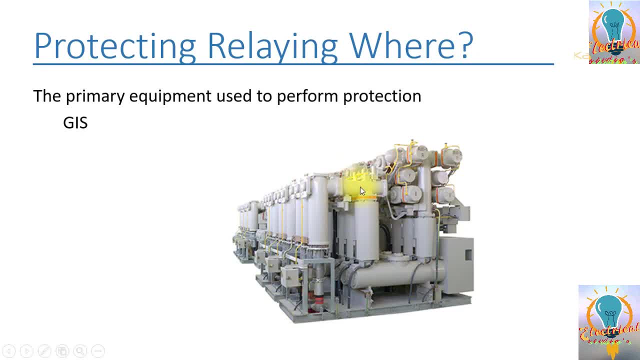 SS6 gas in it. SS6 gas has good properties of insulation, so in a small space you can have a big GIS or you can have a big switchgear installed. so the GIS is prepared over places where land is very expensive and also the maintenance cost of GIS is. 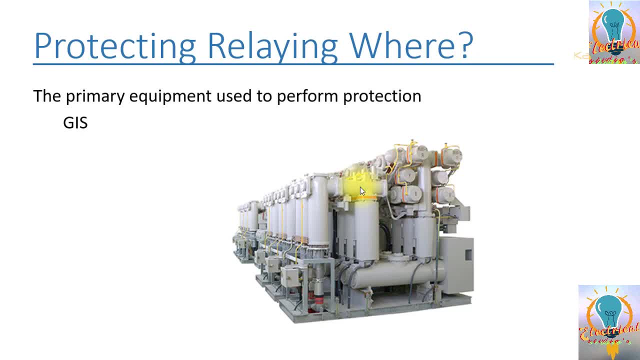 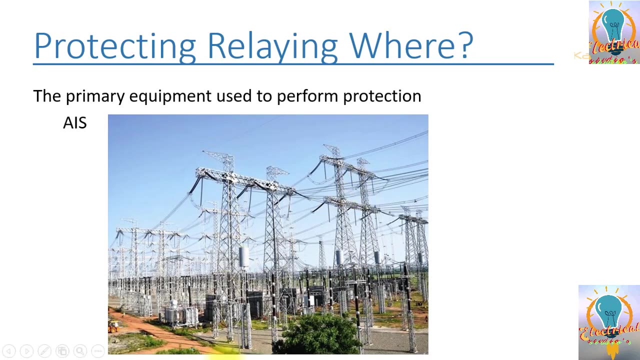 very cheap and very less maintenance is there on the on the GIS, so occasionally you need some maintenance, so that's why it has an added advantage. then you can see a picture of AIS. you can see how much size is required. here again, you can see this is overhead shield, overhead ground wire, shield wire. 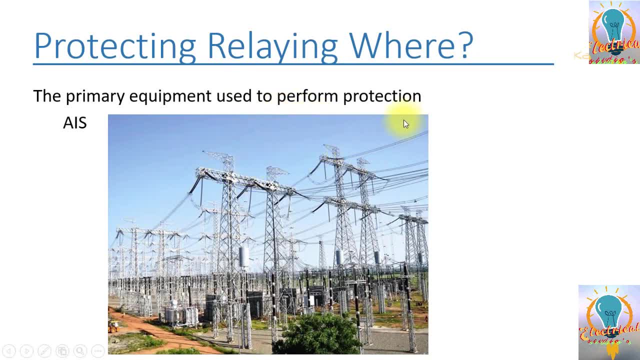 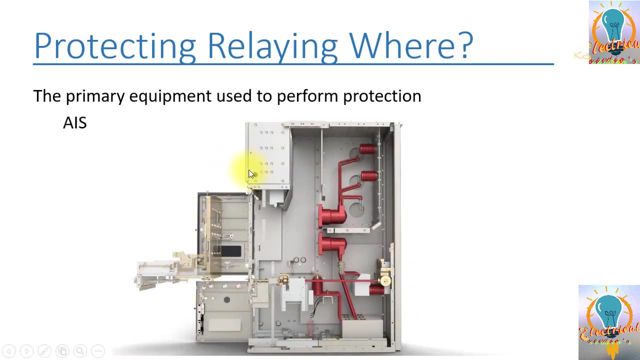 on the tower for lighting protection. you can see another shield wire here and you can see the gravel here. basically I have explained about the gravel previously. this is basically the cutout of the medium voltage switchgear. I have a separate training about the medium voltage switchgear so if you are interested you can join my this training also. 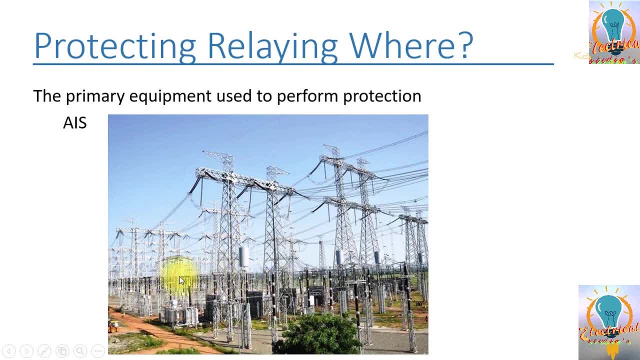 if you are interested about how you are doing the at the time calculations of a gassing substation, I have also a separate training in which you can learn about this, and if you want to study some relay coordination, you can also join one of my training about the relay coordination. so this is the MV switchgear. this is also. 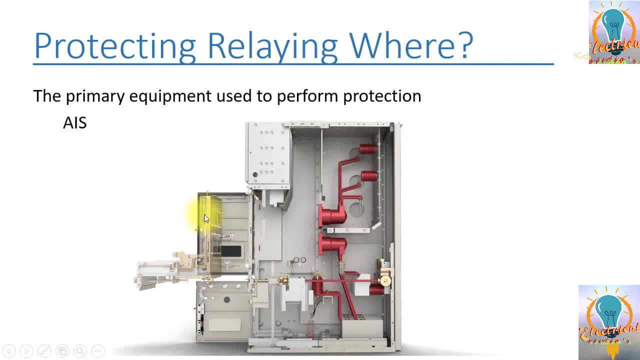 used for perform the protection. so this is you can see this is here you can put the trolley and operating mechanism of the circuit breaker will be installed. this is basically the bus path. here you can see, CT and VTs are connected. protection relays are installed in this cabinet. 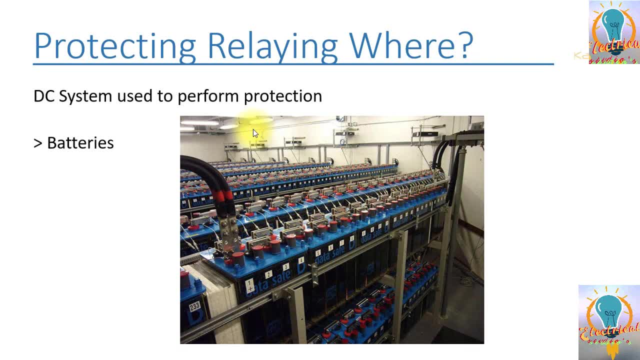 here and then you can see the battery systems, why we need basically the batteries of option A you have in the substation. in order to protect the system, you need the release and in order to operate the relays you need the power. so if you choose an AC power to operate them, if there is a fault, the supply will also go. 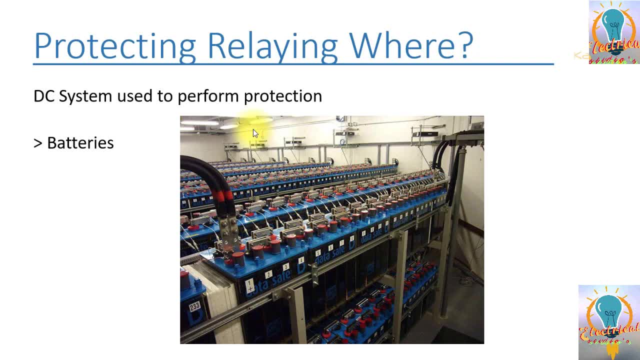 off with the fault. so it might be a fault where the whole substation is black out, so in that case there is no power. so normally in each substation you will find these batteries. so this is just like in your houses nowadays. you have seen a solar and you or you have seen a UPS in which 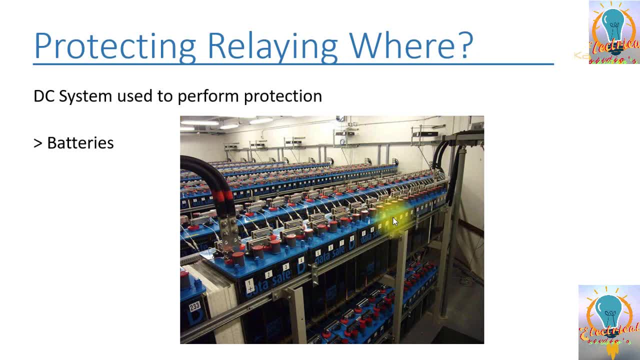 you have installed a battery. if main supplies fail, then you are supplying your home through this battery as a backup. so in the same way, the substation, all the protection system, control system, is on the DC and it is backed up by. normally this DC supply is provided by the chargers battery. 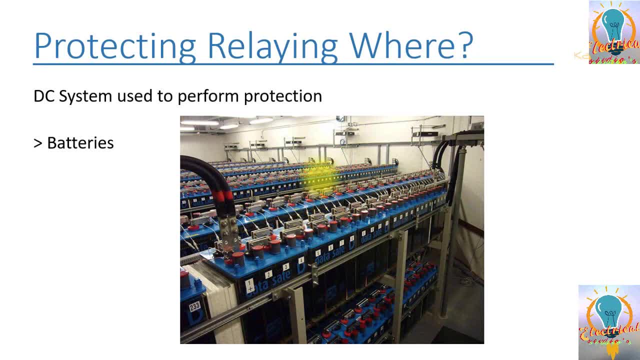 chargers and battery chargers are converting AC supply to DC and then they are supplying to the relays, control and protection systems. when the AC supplies fail, then the charger, these batteries, will feed basically the relays and protection control system as a backup. so that's why in each substation you will 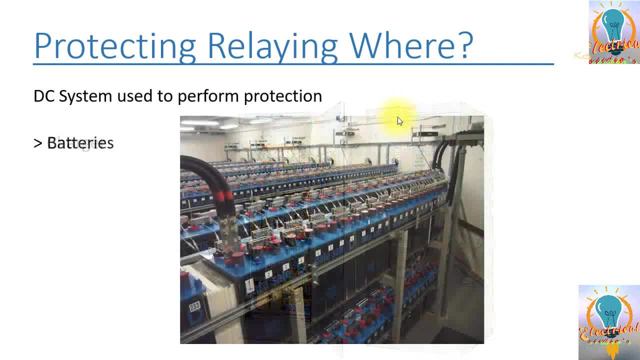 find the batteries, and normally there are two batteries, two back up two batteries, two back up up two banks in the in the substation, bank one and bank two. you will find two banks in each substation to protect, so if one, even one bank is failed, another 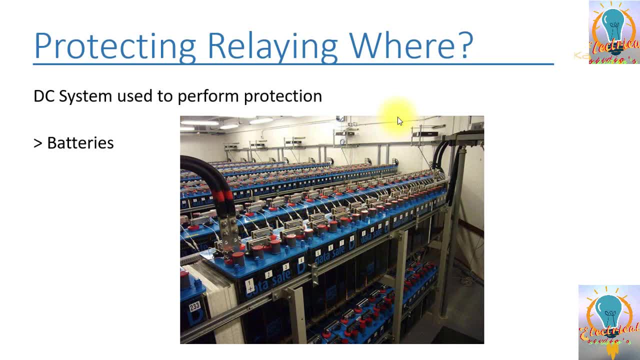 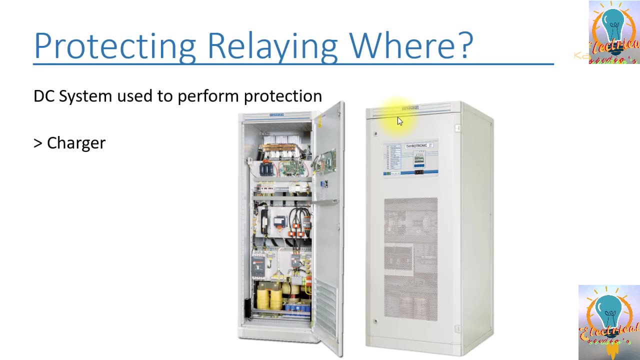 bank is can supply and also, if you have a to protection protection system one and two, normally production system one is connected with bank one and then there is a charger, so the batteries- this is from very famous brand name, so the battery is a supply- is connected to this charger and output of this charger is 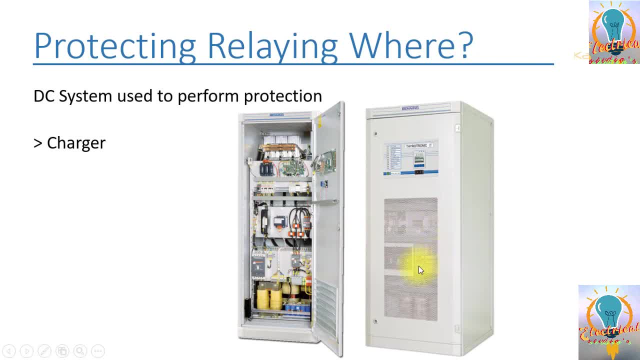 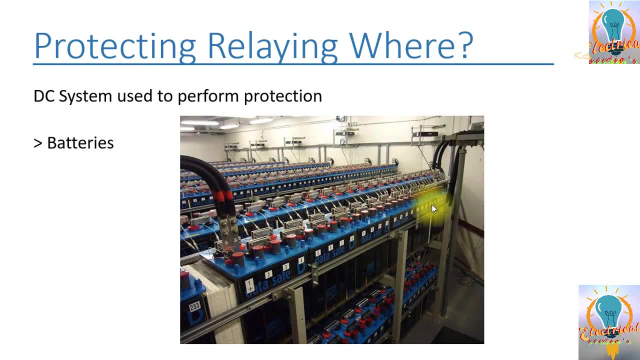 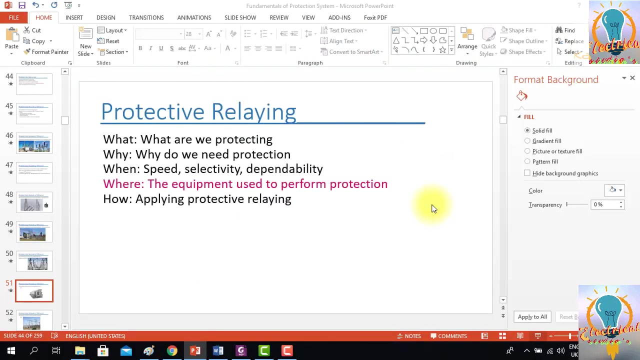 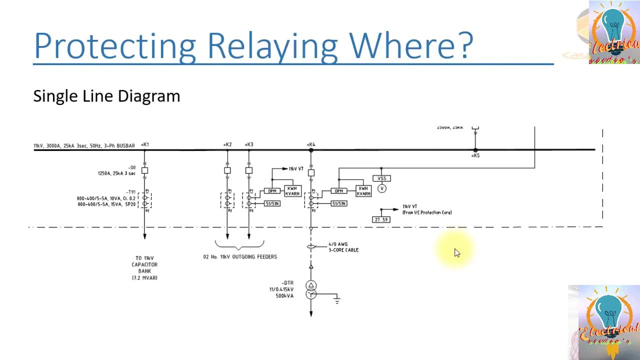 decent. so the output is connected out to the batteries and this charger is charging the batteries and also the load is connected through this charger. so this is basically some introduction of smart nuray Сегодня Containment. thank you very much. hey, friends, now I will just introduce you to single-line diagram which is also. 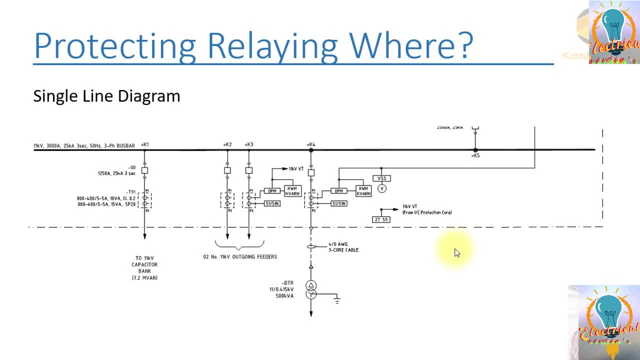 a key document for protection and control systems. in a single-line diagram all the information is shown on the high level and mean that you have to show a very basic of our system. for example, here you can see this dark line is showing here the bus bar. this is basically 11 kV. you can see the voltage level is mentioned here: 11 kV bus bar. 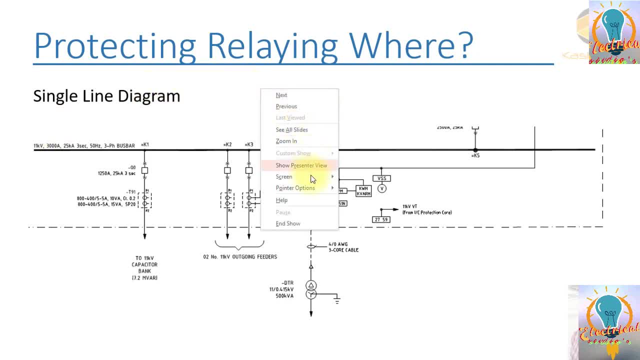 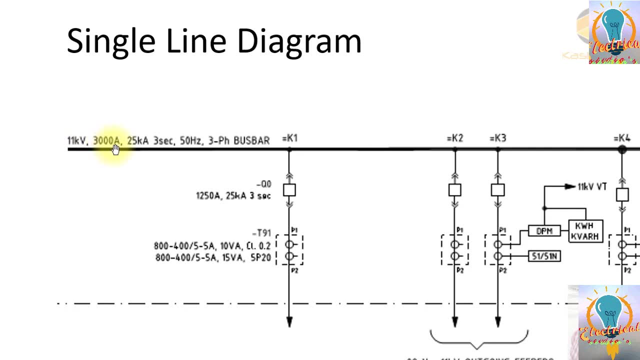 so the information about the bus bar is mentioned here. the continuous rating for the bus bar is 300 ampere. it means that this bus bar can conduct the load of 3000 ampere continuously without the temperature rise. short circuit capacity for this bus bar is 25 kA. 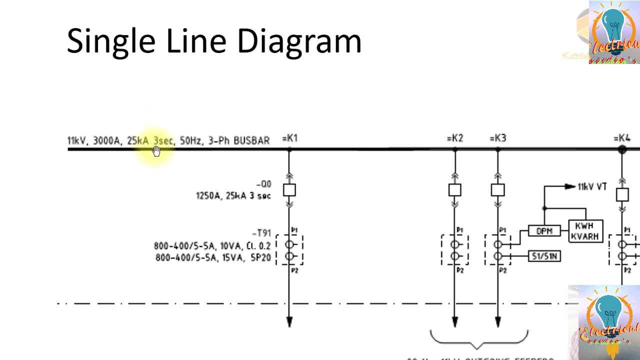 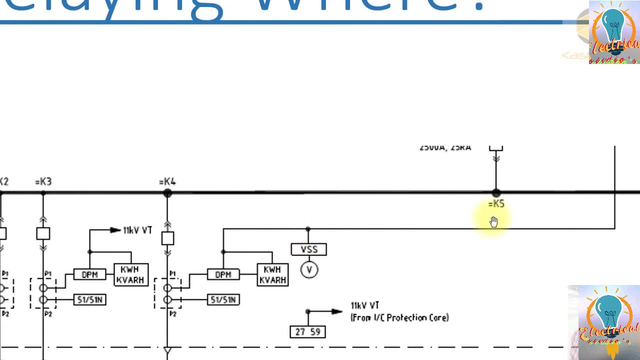 and the duration for this is for 3 seconds. it can bear 25 kA. 50 Hz is basically the frequency, three phase bus bar and here further you can see it has an incomer, k5, which is supply, the feeder, or the, which is connected to the. 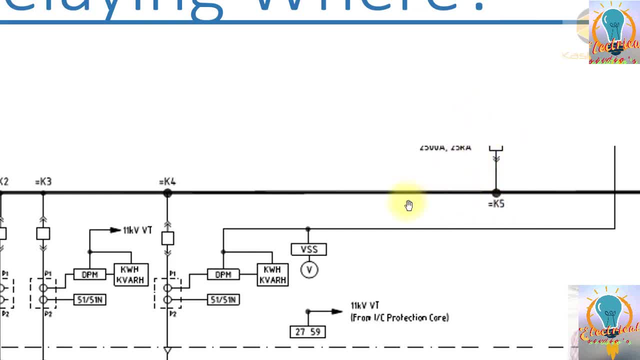 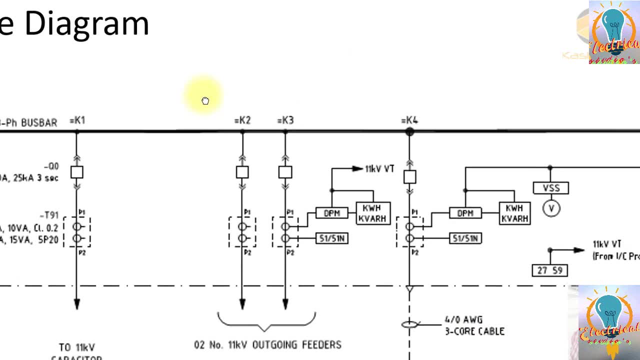 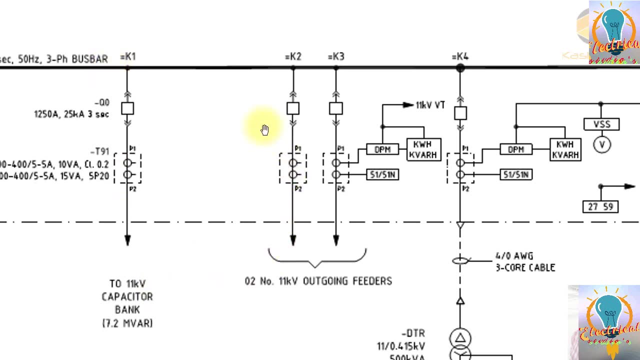 bus bar and supplying the power to its called incomer. so this is incomer k5 and it has then four outgoing feeders: k1, k2, k3, k4. k1 is the capacitor bank. here you can see each and everything. here is basically three phase, but for simplicity all three phase are shown by a. 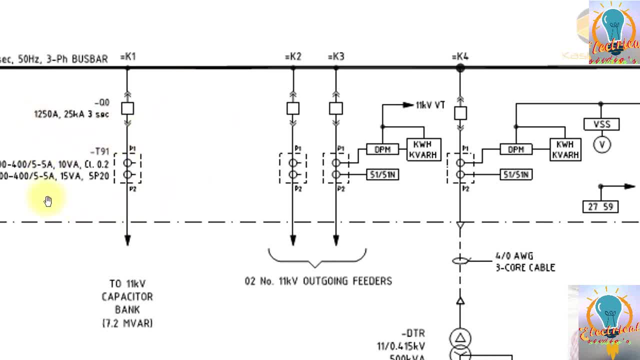 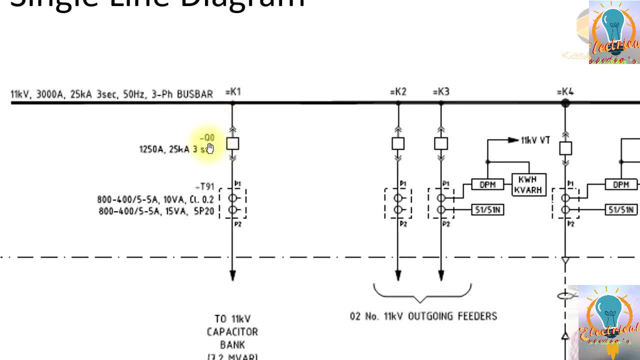 single line. that's why it's called as a single line diagram. you can see here, this is the breaker and this is the 11 kV surge gear that I have shown you already. and this is the breaker. and this double line means this is: this trolley doesn't have an isolator, but you can. 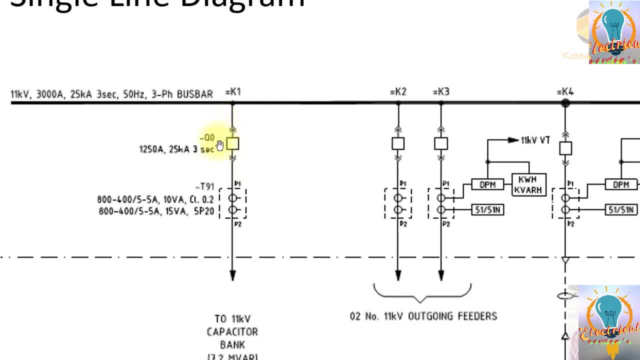 very long Play hard to study. any spoke stiff Concerning the positive inhabitation of this specifications important. Π1-P2 2: this is the name of CT and you can see the CT ratios are mentioned here. this is the basically class 0.2. this is for metering. this is protection, class 5p20. 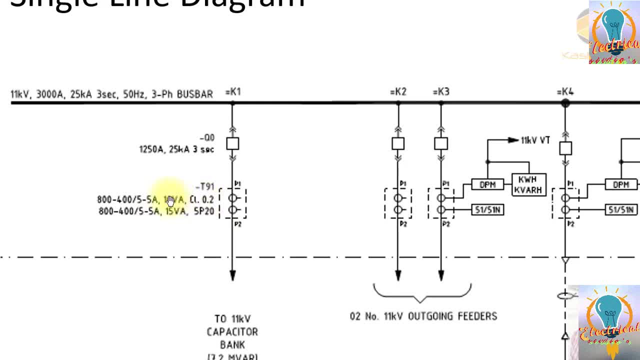 and this is the rating of the CT which is in VA- 10 VA, 15 VA- and this is basically multi ratio and multi core CTs because it two ratios can be selected- 800 and 400- and and it has two cores secondary side, so both are marked at 5. 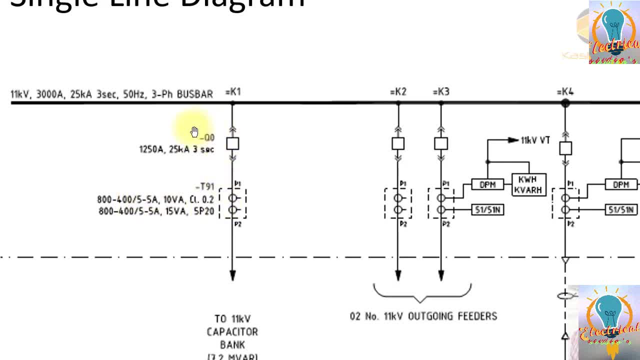 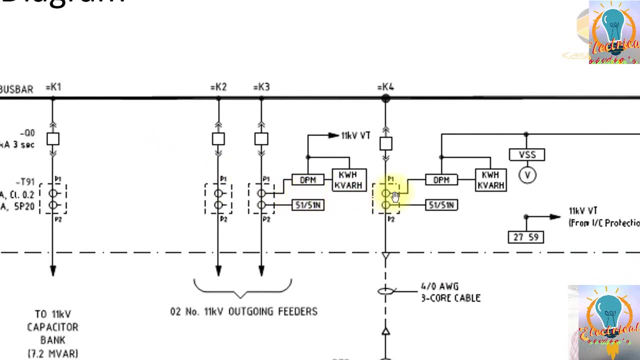 dash 5 breaker is shown by Q naught and the rating of breaker is 1 to 5, 0 amperes, which is less than the busbar rating. short circuit rating is same as the busbar, so all the other feeders also have the same rating. here you can see. 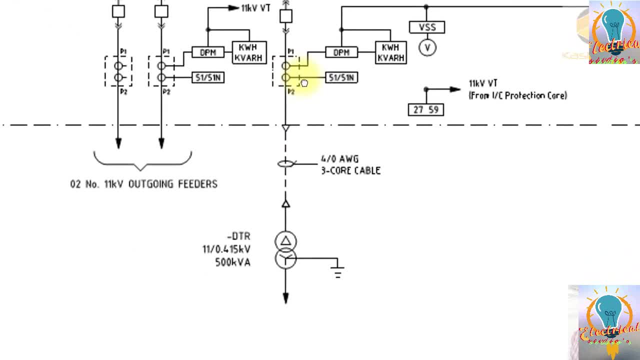 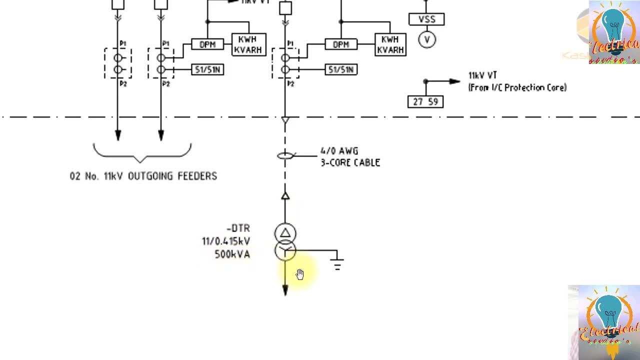 they have shown. this is a feeder k4 which is connected to the auxiliary transformer of the substation 11 k by 415 volts and it is supplying power to the substation- AC power. here you can see this is showing as an a cable ceiling and cable is. 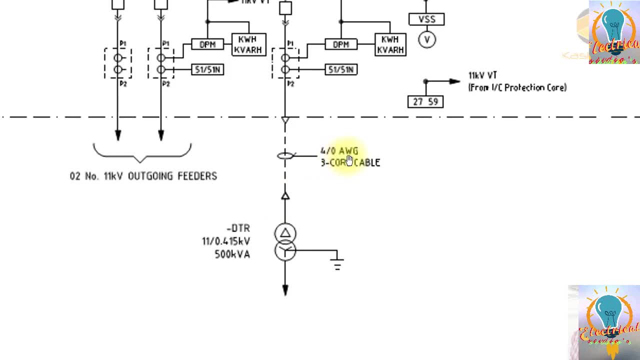 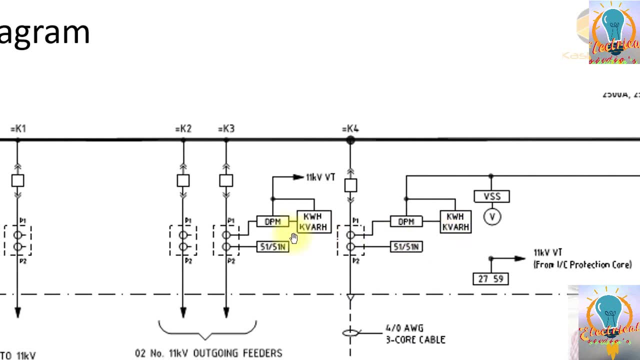 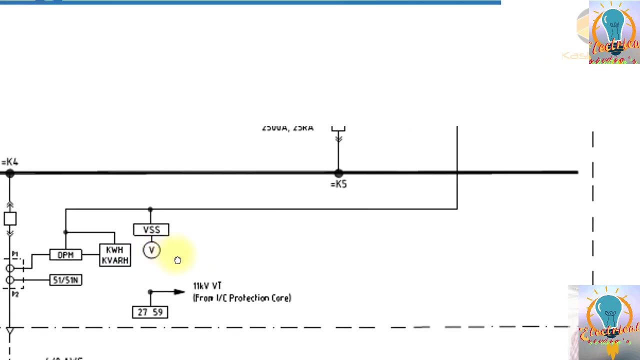 connected. it is connected to the cable and it's it's basically for AWG 3 core cable and here you can see the digital power meter, kwh meter, kvr meters. so all this information. you can find high-level information on single line diagram. so if you are more. 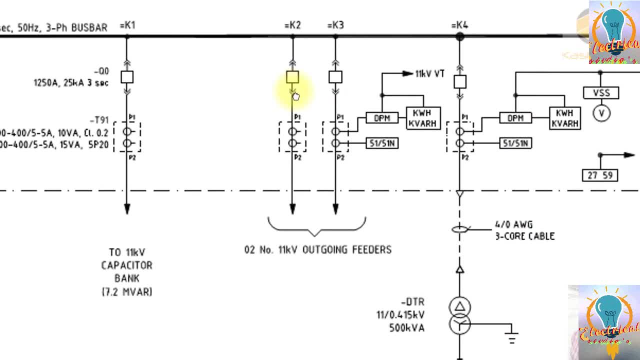 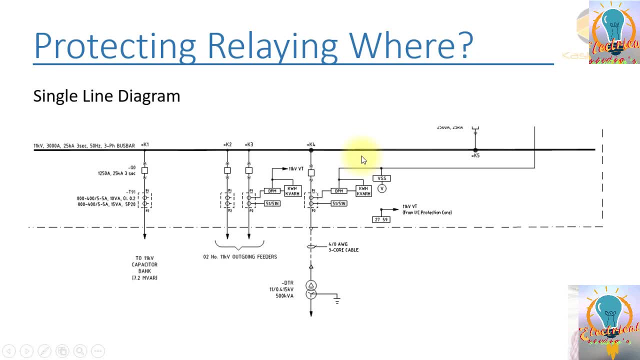 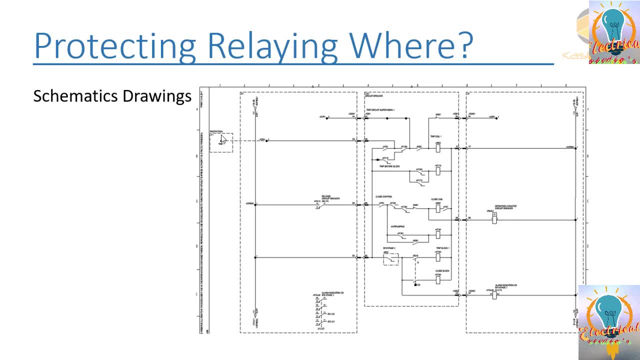 interested to learn about this, you can enroll in my course, which is explaining the single line diagram in detail. so I hope you, you will. you are this training. thank you here, friends. now I will show you another drawings which are called a schematic drawings, or we are calling them also as a detailed drawing. basically, each 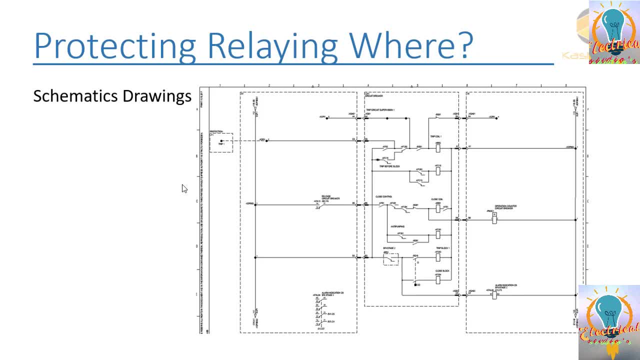 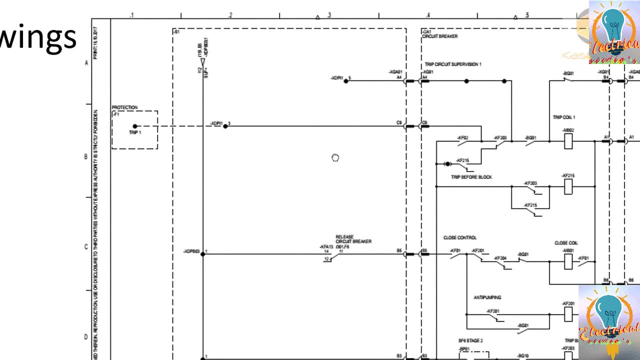 substation. I have shown you a single line diagram and then this which is showing the high level information. then we have a detailed drawings or schematic drawings, which are showing a detailed information above the protection and control schemes. so let me zone, so here you can see, this is the detailed drawing. 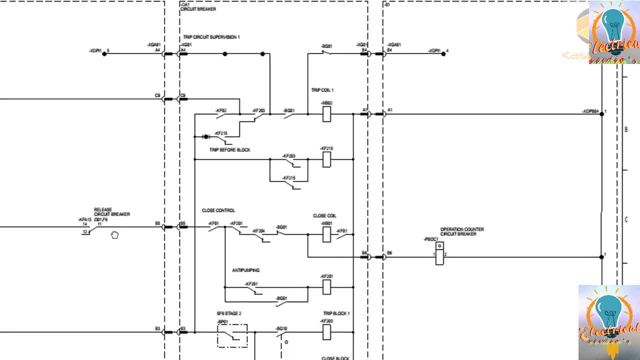 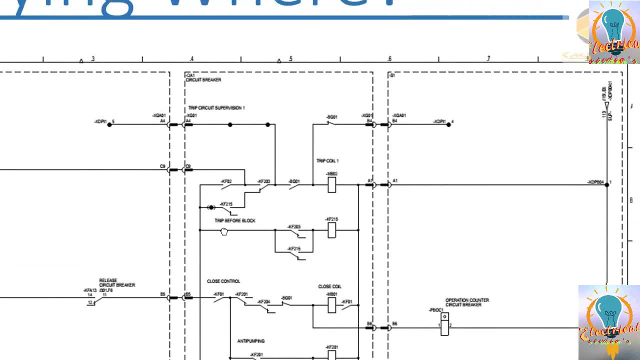 so digital schematic drawing look like this. so here you can see some information, data information. for example, I have selected a drawing of a circuit breaker to one. it is not a single line diagram. it's showing each and every wire separately. for example, here you can see: this is basically. 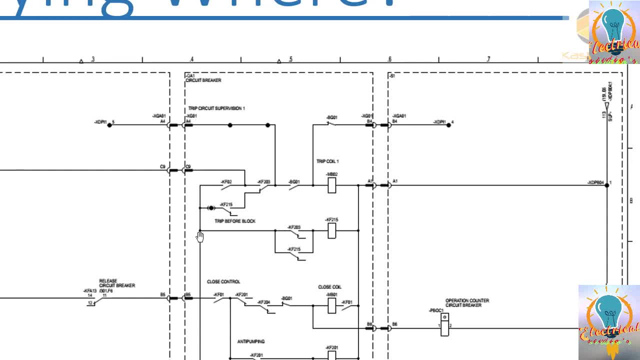 circuit breaker compartment. this is when this, this light behind the neck we called CD chord, this line comes sauce like this. so here you can see this. theseательно they are making*******************************. you can see, this is specifically such unit breaker, this line showing that this is 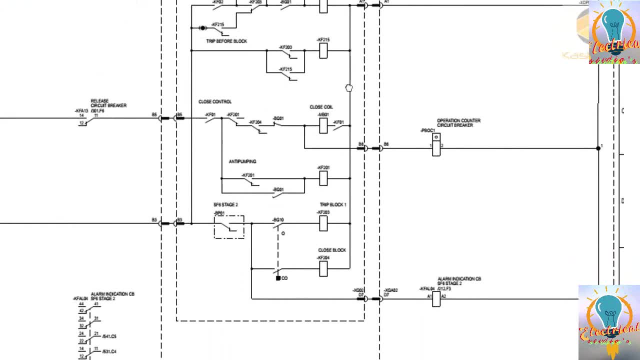 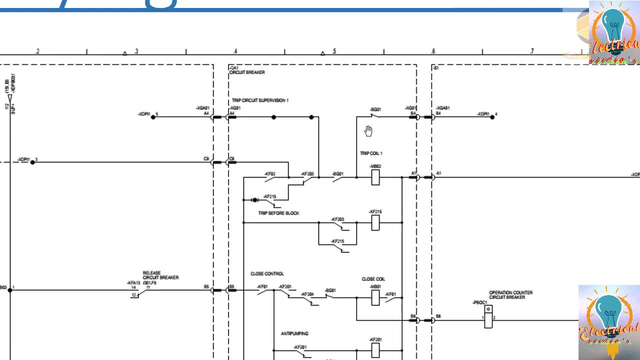 It's showing each line diagram. it's showing these two like a single line diagram, another compartment. this doesn't belong to the same drawing that we are looking in and we are at present looking in the drawing of line control cubicle. line control cubicle LCC is installed in front of GIS that I have shown you. 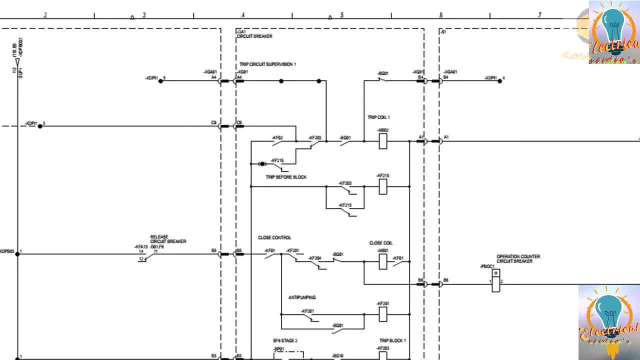 recently, and here you can see this is the tripping coil one on M 602 and they are also some contacts and then it's. you can see this point. this is basically the male and female contact of a hardening plug. it's basically a plug, it is shown. 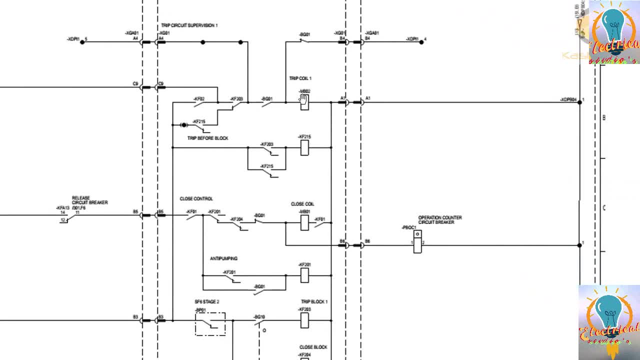 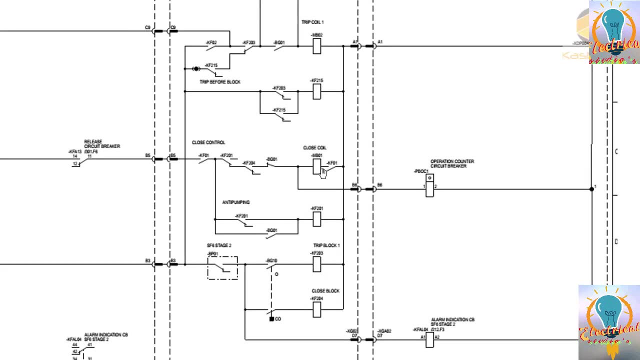 here like this: this is the tripping coil one and this is basically you can see tripping coil two. this is sorry. this is the closing coil which is shown here and this is the count point. whenever breaker gets a pulse for closing, the counter will operate and 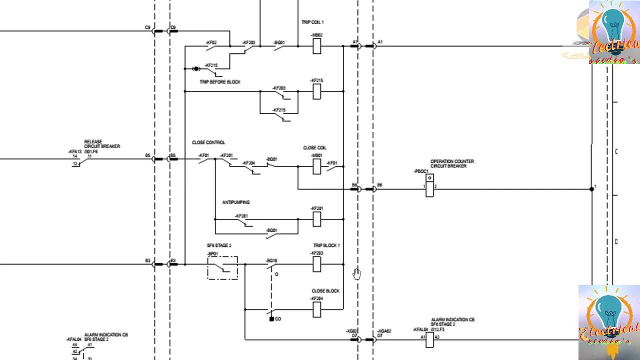 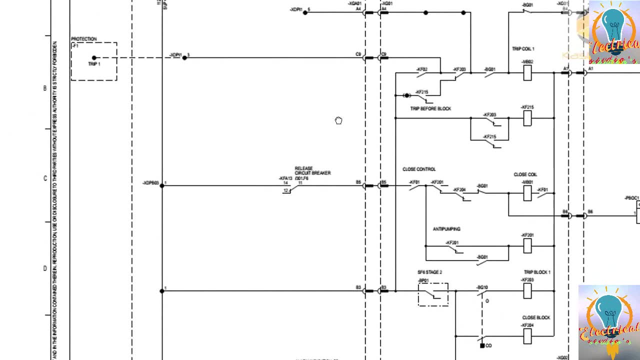 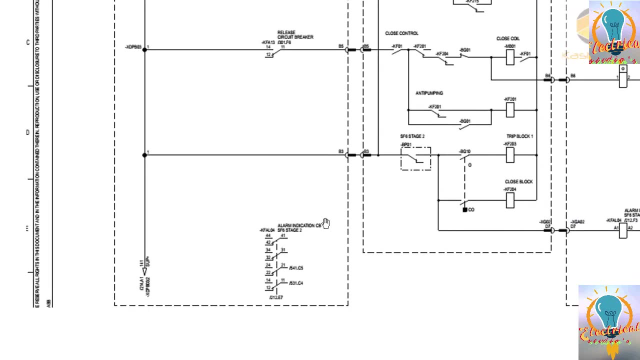 will operate, the how many times the breaker is closed. so each substation is provided by detailed drawings. all the control protection panels, alarm indication panels. they have similar schematic drawings. these are basically the auxiliary contact of the relay SSX. stage two relay are shown here, so this 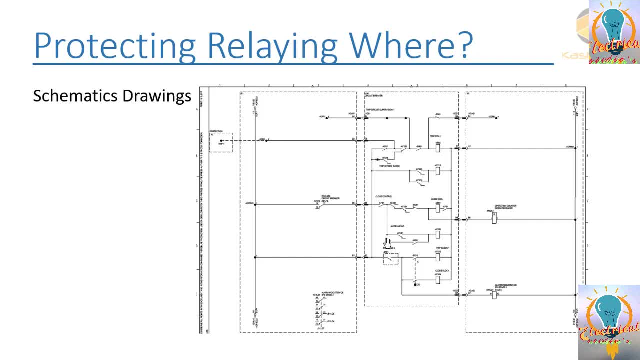 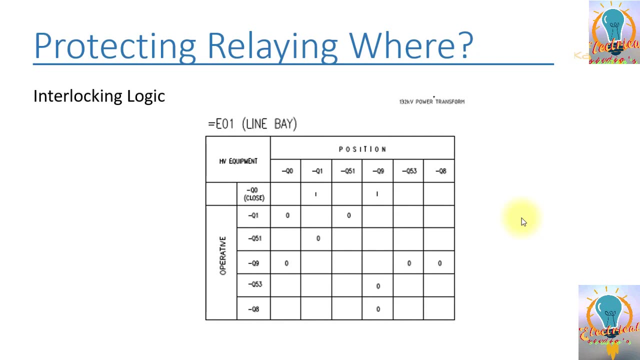 is a little introduction about schematic drawings in the substation. so I have separate trainings on these. so if you are interested, you can check these trainings in my profile. thank you very much. welcome friends in my. in my previous training I have shown you that there is an interlock between different 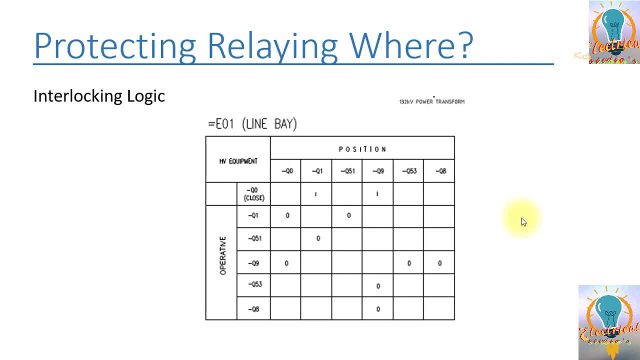 components of substation and this interlocking is to prevent the mole operations. the mall operation could be like closing of a live line or while the archetype switch is closed. so such practices are avoided and we are trying to make the system foolproof and for this we have to do the electrical interlocks so, and an example I have- 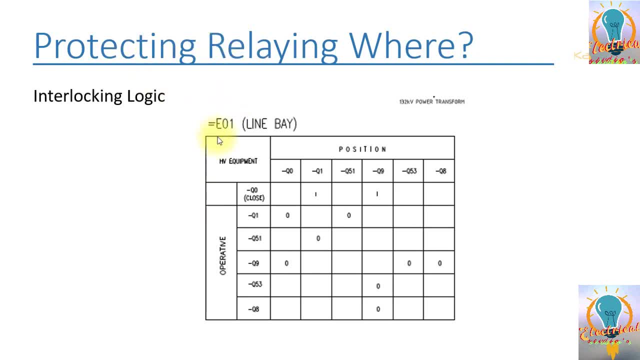 shown you a table. okay, in this table you can see, and there is an equipment, electrical supplements present in the electric appliance. so we have toそうですね, we can see, and there is an equipment e01 line way and it has some components like this: is the breaker q00. so this breaker can only be. 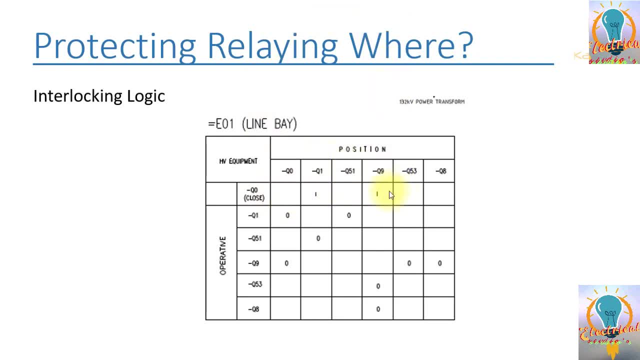 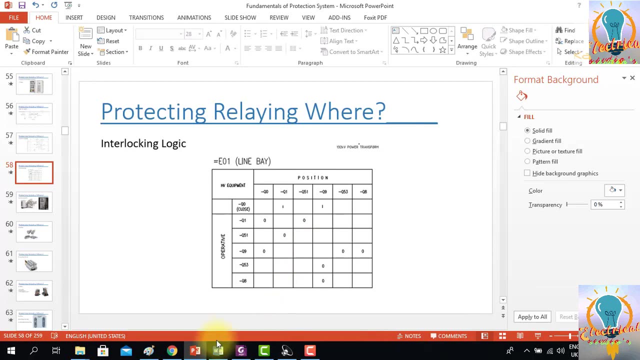 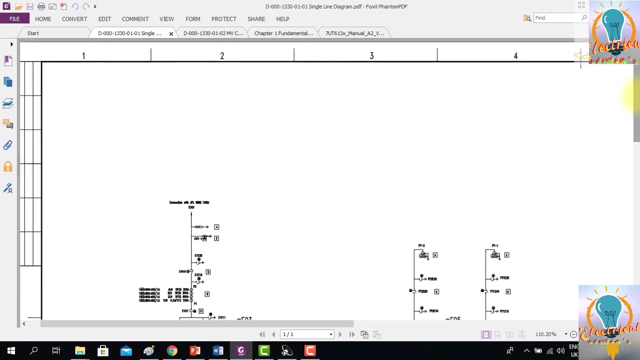 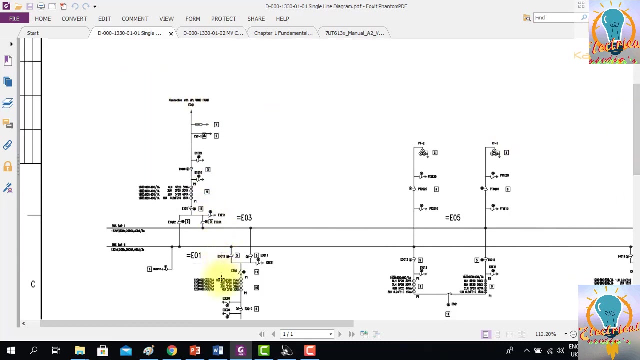 closed when q1 and q9 are closed. so let's see what are these components. so let's go to e01. this is e01, so i will zoom in. this is basically the line breaker. so this is basically the configuration of the substation. it has 1132 kv line as an incoming. 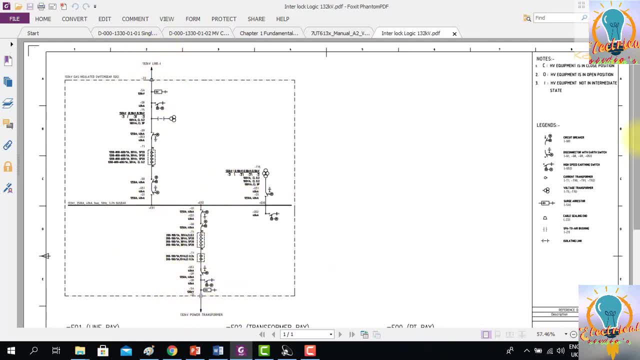 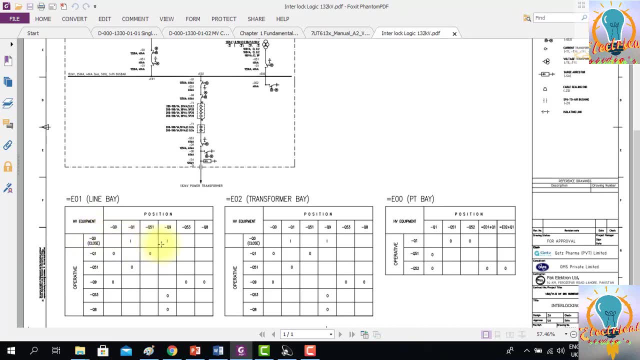 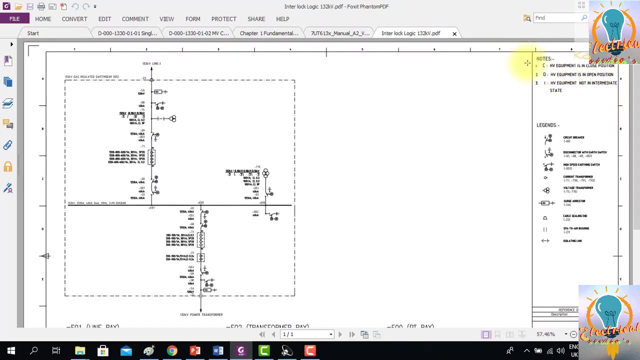 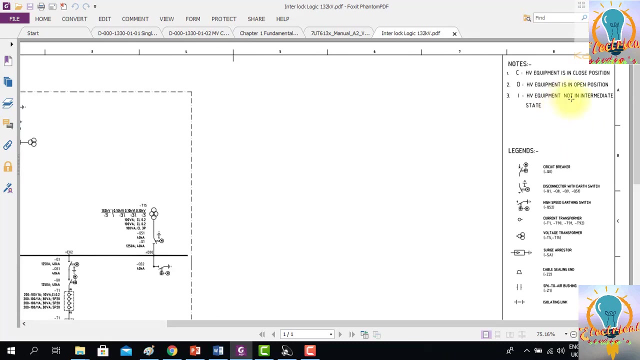 and one 132 kv line as outgoing, so it it has only two lines. so you can see, i can operate the breaker only when q1 and q9 both are one. one means here, you can see, one means equipment, hv equipment not in intermediate position. i is basically i. i means it should. 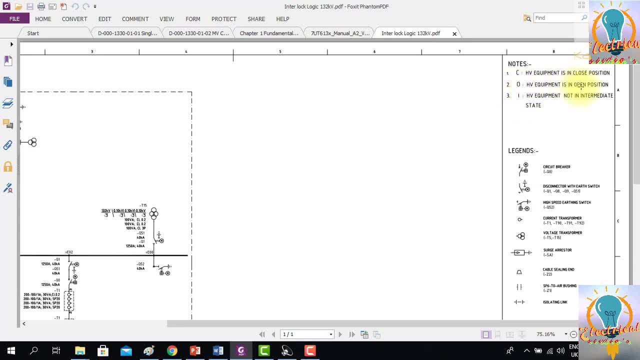 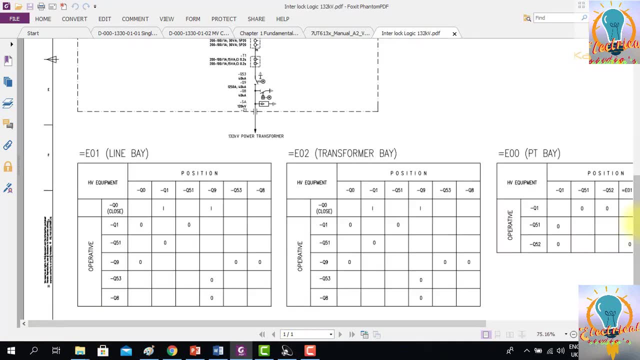 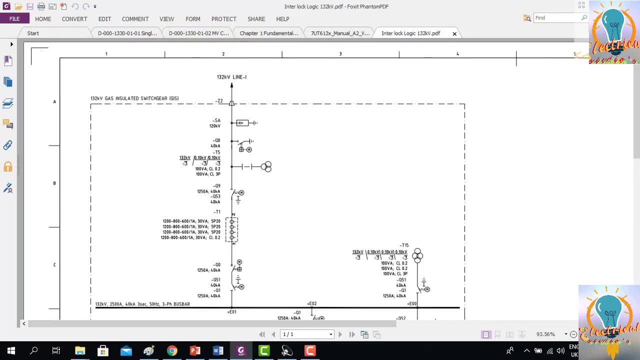 not be intermediate, uh, zero. o means hv component is open position, c means hv component is in close position, so i can operate the breaker. this is my single line diagram. this is 132 kv line bay. this is my breaker. q naught, uh sorry, this one is my breaker. 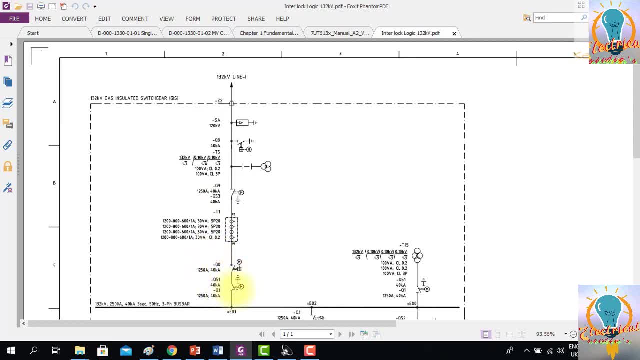 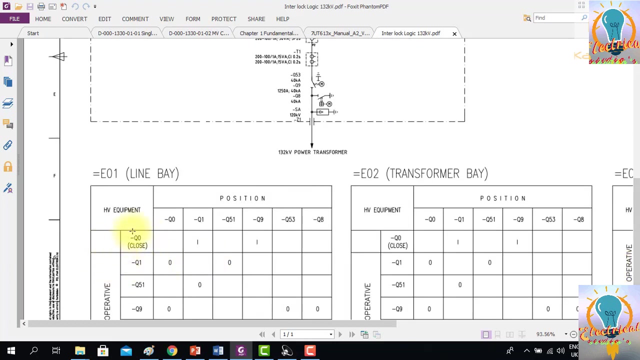 q naught. this is the bus ice refrigerator q1. this is the bus bar. this is the earth switch to ground the breaker. then you will move forward. this is q9 is the line isolator. q8 is the liner switch. so i can operate the breaker- line breaker q9- if my line isolator and 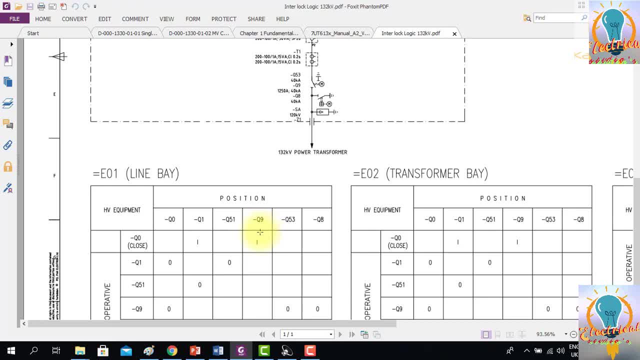 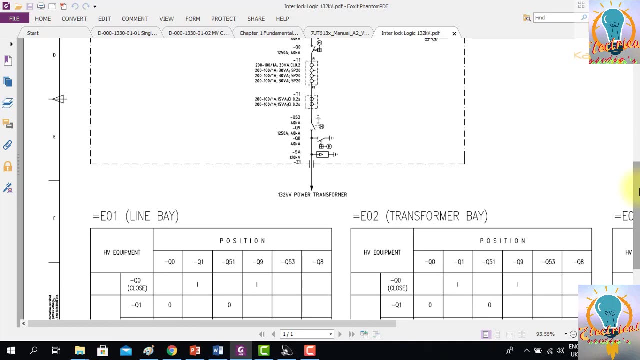 birth isolator are either fully open or fully closed. i cannot operate breaker when the isolator is intermediate position. so reason behind is this that, as as i told you, that isolator is basically a offload device. if it is in in intermediate position, it means it's not fully closed and 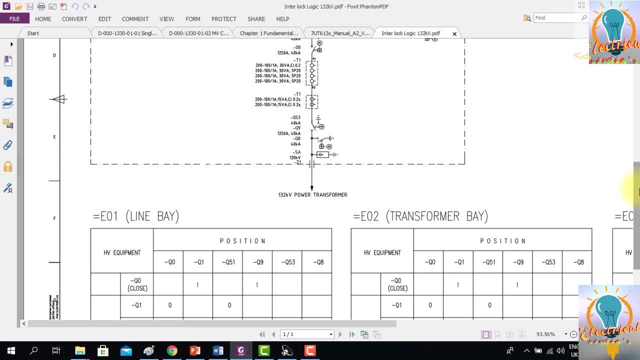 if i close the breaker, then what will happen? that there will be, uh, arcing will be started between these two contacts which are not still closed so and and there will be damage in in the isolator. so that's fine to protect. i can either operate the breaker if both of the ice. 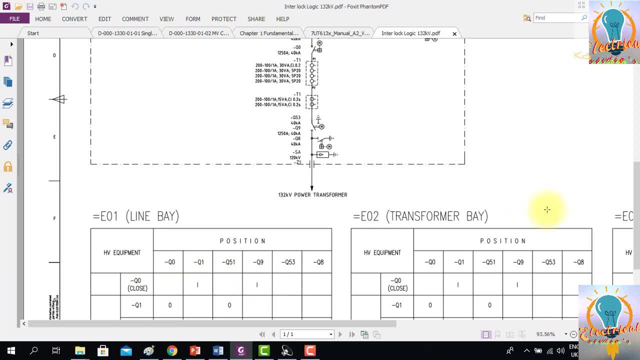 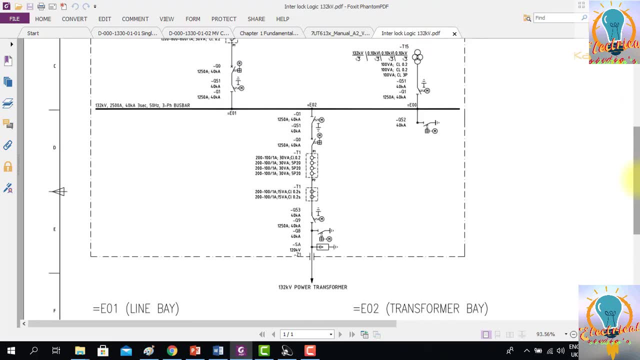 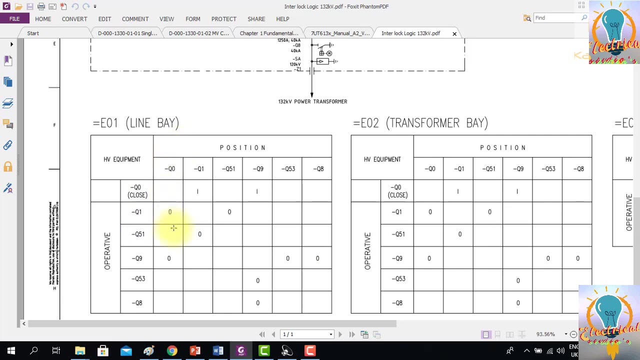 later have completed their operations. they should not be in intermediate position. so this is an example of uh interlock table. okay, we'll see how can i operate. i can operate bus isolator q1 if breaker is open. q naught is my breaker line. brain breaker is open and q51 earth switch is also open. 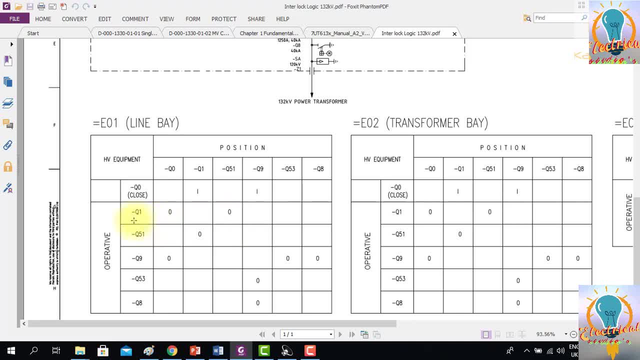 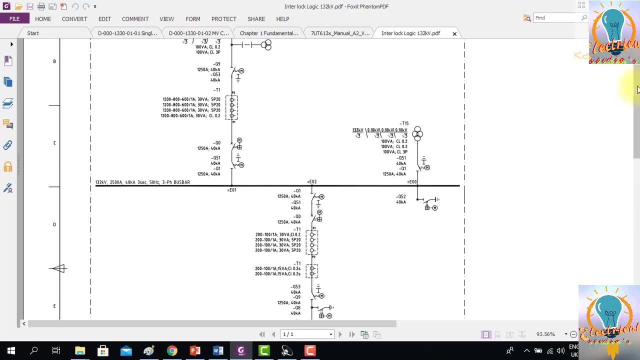 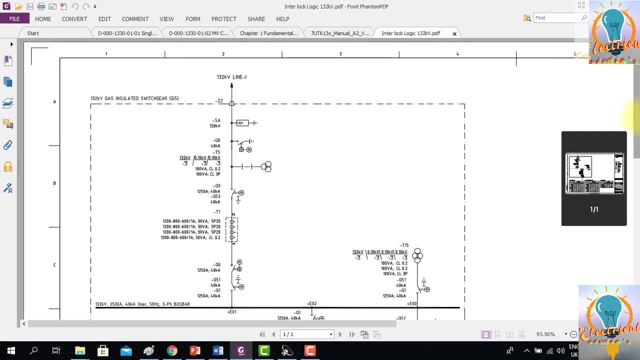 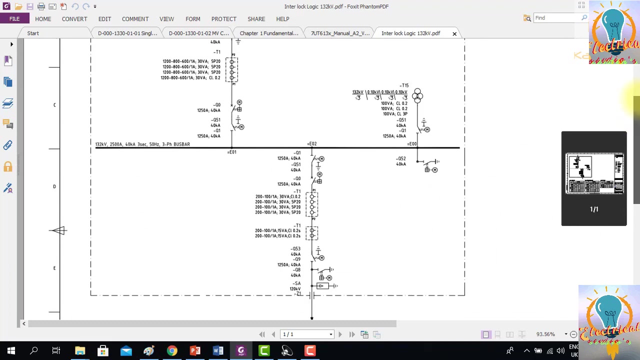 so this is the requirement to close the isolator. so isolator should never be closed where the earth switch is connected and when the breaker is open and it only be closed. so this is an example of interlock locking and this is interlocking table. so in detail i have explained this one in my another training related to single line diagram. 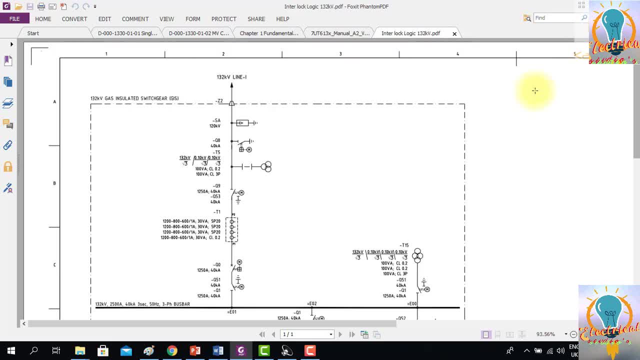 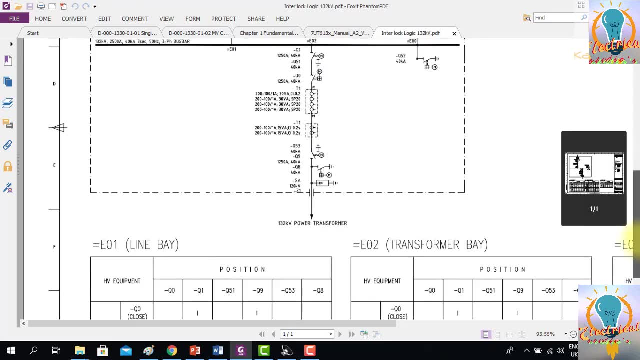 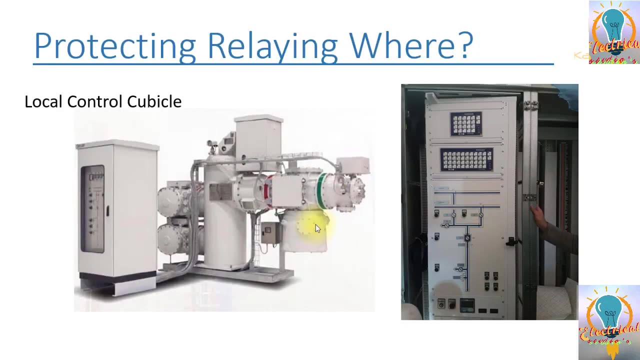 and quotation to single line diagram. so if you want to have this, you can join this training, okay. so i hope you you understand some basic information of how interlocking is working. thank you very much. hey, friends, uh, here i we will discuss about local control cubicle in my 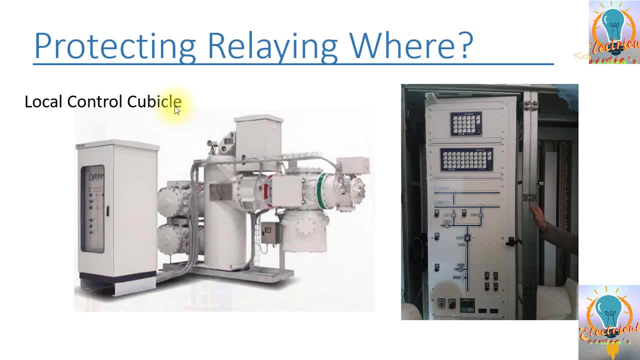 previous lecture i have shown you the drawings or as a sample of local control cubicle. basically this is our gis and i will explain you a little bit about it. this is basically the current transformer here. this is the ct. if you visit the gis with experience, you will know this. 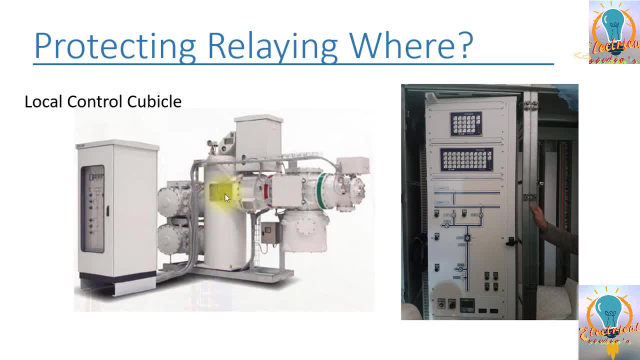 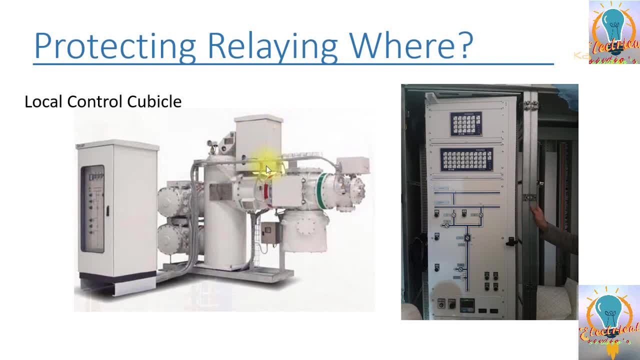 the gis is the high speed r switch. this one is the isolator. you can see it's line isolator. and this is the mechanism box for the circuit breaker. and here you can see the gis. uh, the gas uh is filled in the gis, but all the gis doesn't have have one compartment. so for the sake of 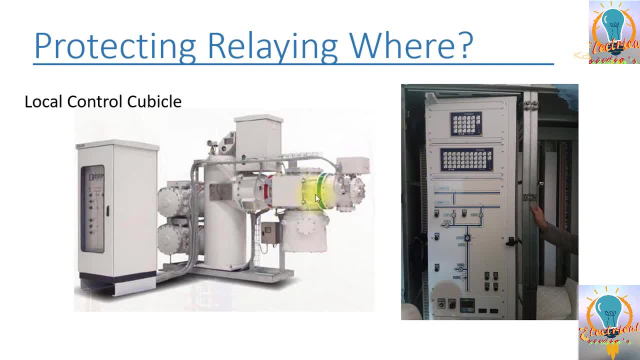 GIS is also divided in different compartments or parts, and each part is gas- is separated from another compartment, for example. here you can see, this is shown by a red color, this is shown by green color, so, and the red color means this part, this complete part, this is one compartment and here another. 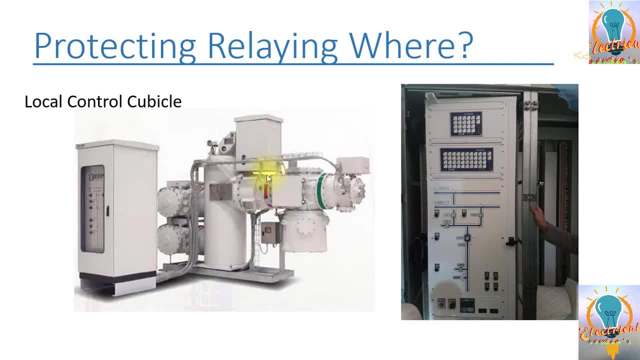 compartment is starting. this is a gas tight seal is installed in in between this. so we we have to fill gas here and check the pressure and the gauge will monitor only the pressure of this area. so the green means permeable gas for me will get compartment. so it means that here the gas is not tight and it mean 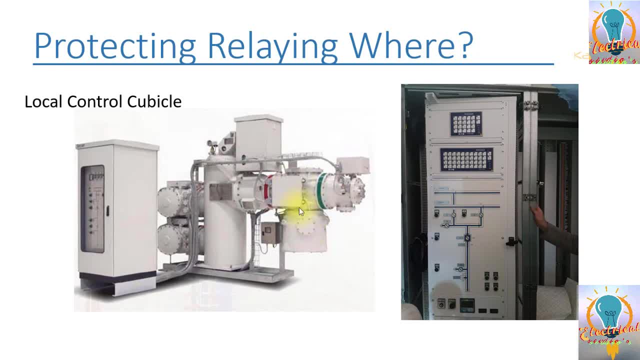 that this vt and this uh isolator and this earthing switch- these are all in inside. it has one compartment. it has only one gas, whereas you can see here the ct and the circuit breaker is also one gas compartment and one gas is filled, or one one. our one gauge will be installed uh on it, so each gis is divided. 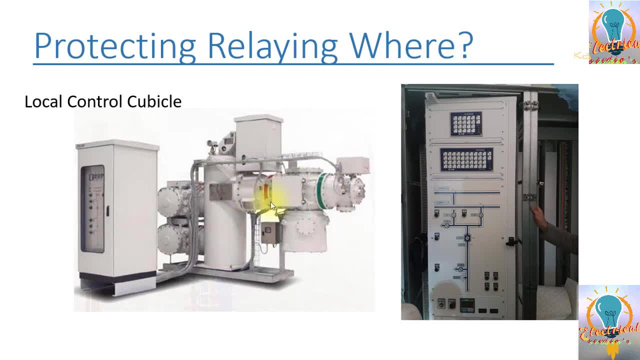 into several gas compartments and they are shown by this color- red and green- gas type or gas permeable, and each compartment is then monitored by a separate gas as a gas monitor, and here you can see the bus bar also has a different compartment, which is hidden behind. 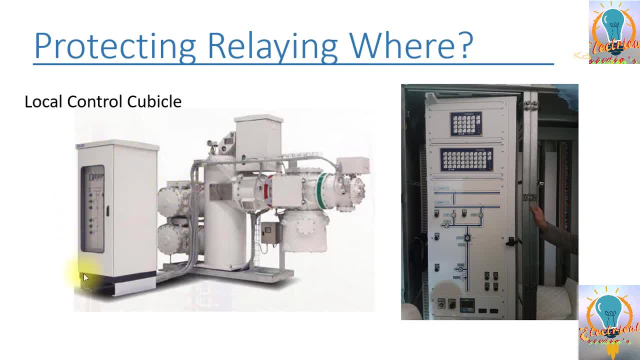 this and you can see this is basically the control cubicle, which is called as local control cubicle, lcd c, and here you can see this lcc and this area. especially if you see from the front, you will see the lcc like this: and this area is basically the scholars mimic and here you can see the 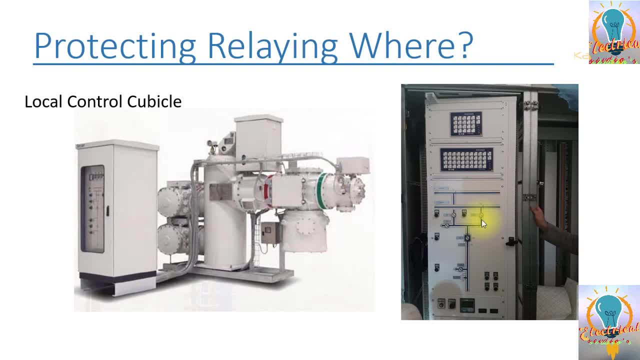 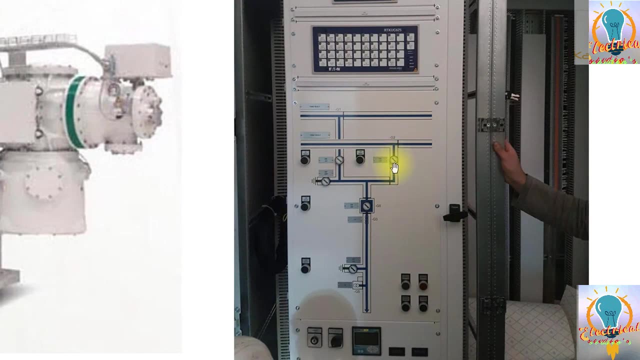 symbols, as i shown you. single line diagram. you can see the symbols of this is basically the called as sema four indications. so these are called as sema four indications at present. uh, they are in the middle state because this supply is off. when you switch on the dc then you will get the actual status of isolator if this line is in line with the. 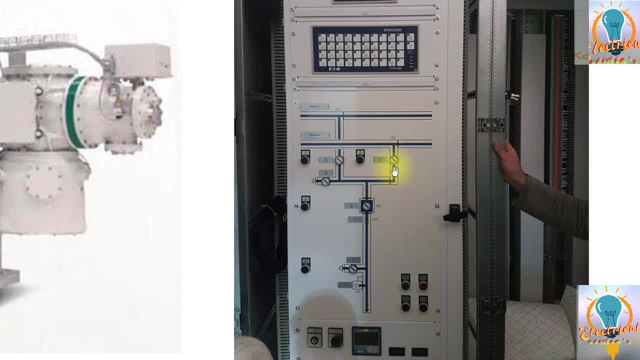 this may mean mimic line. the sema four is in line. it means isolator is closed and if this is perpendicular to the mimic line, then it means the isolator is open. so you can see, this isolator symbol is shown by circle. there is a breaker symbol and this is the isolator symbol and this is the 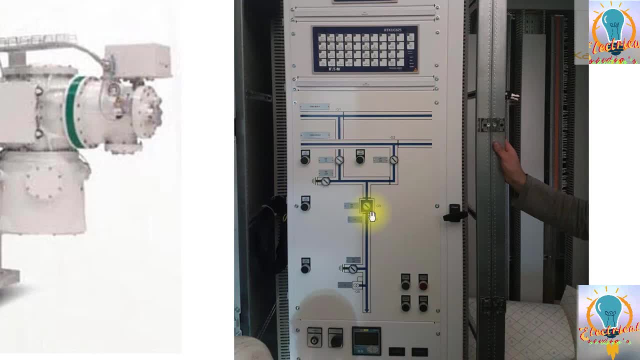 sema four indicator and this is the isolator. the sema four indicator is shown by circle. there is a breaker symbol is shown by a square And you can see. this is the earth switch and this is the voltage transformer connected here at the line and these are the bus bar. 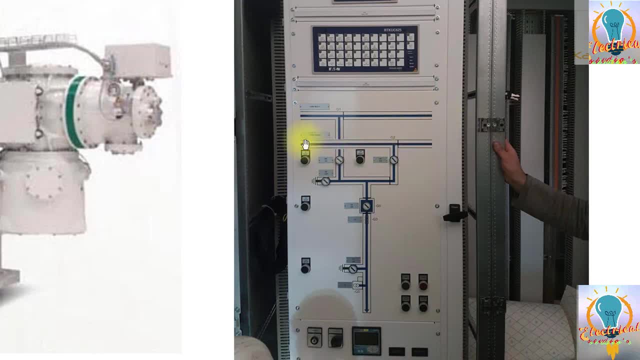 You can see this is bus 1, this is bus 2.. If you see further in detail, you can see they have written here G3 and G5. So these are basically gas compartments. So this is the gas compartment number 1, which is G5, and there is another gas compartment. 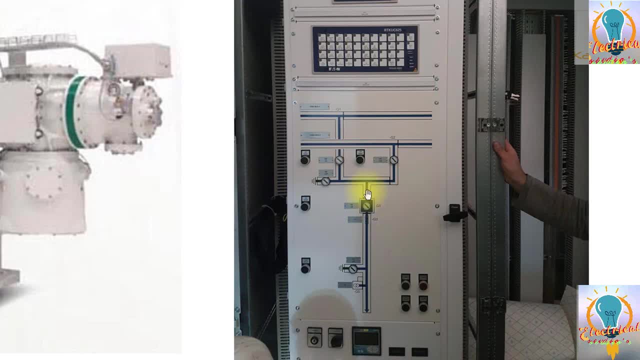 which is G3, as I have shown you, in which there is CT and breaker R in the one gas compartment. It is G3.. Another compartment has a VTE and the earth switch is in the another gas compartment. here, And in the same way, you can see the bus 1.. 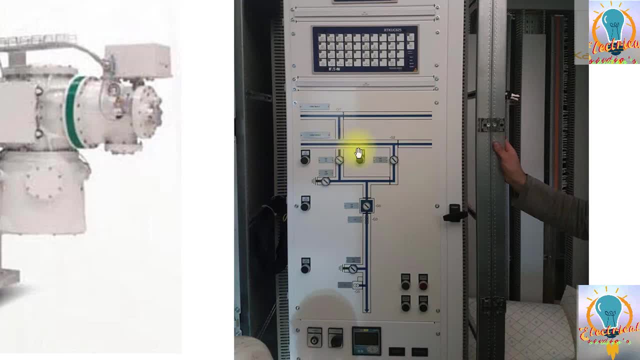 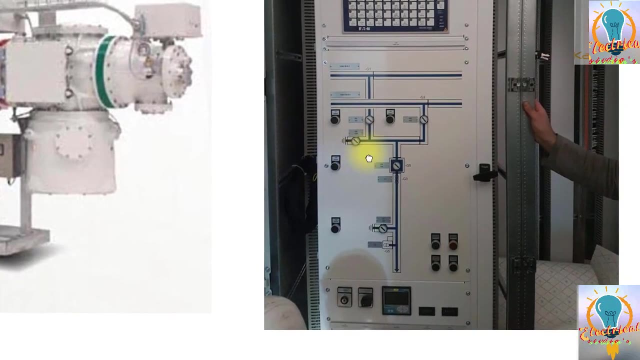 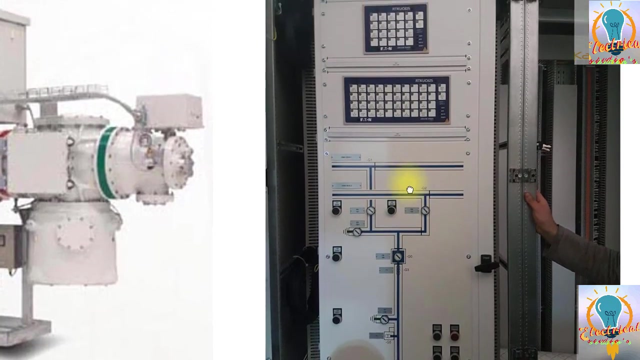 Bus 1 is shown in one gas compartment, G1, up to this point, and another bus is shown in G2. So normally you will see a gas diagram for the GIS which is showing different compartments. They are also drawing this gas diagram on, like this one on the Mimic. 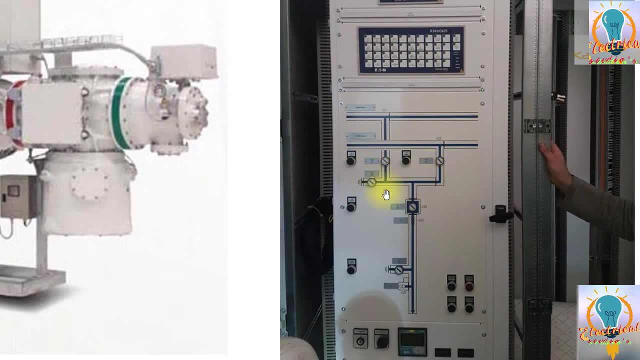 So if you want to do the maintenance of, for example, bus, bus, bus bar, you have to close you, you have to close this switch and then you can close isolator. the other ways you can close: there is a bus bar. I think switch is installed on each bus, so you have to isolate, come all the data interlock. 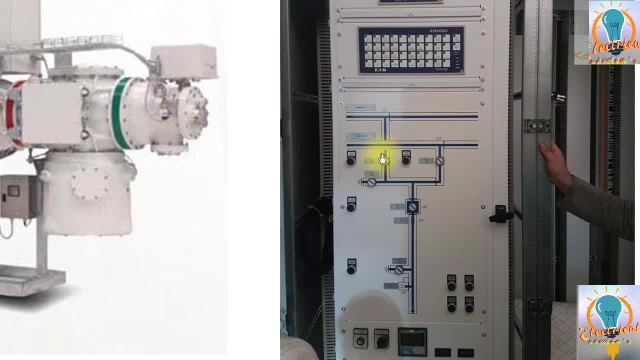 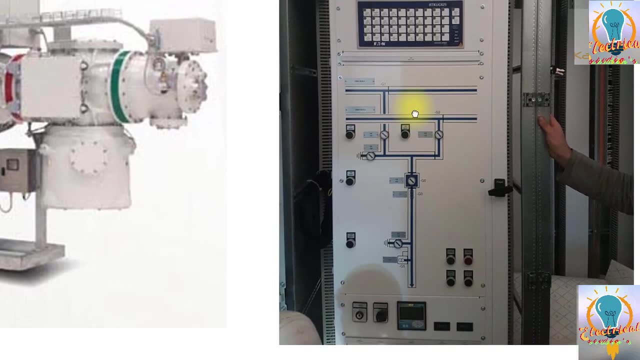 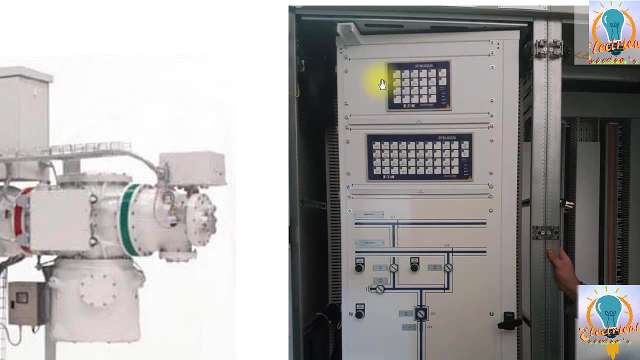 between the bus power switch and the bus isolators. so you have to open all isolators. then you can connect the bus power switch and then you can do the maintenance on it. so on the top you can see two annunciators. so one annunciator normally in LCC feed by AC supply and one is feed by the DC supply. so if DC 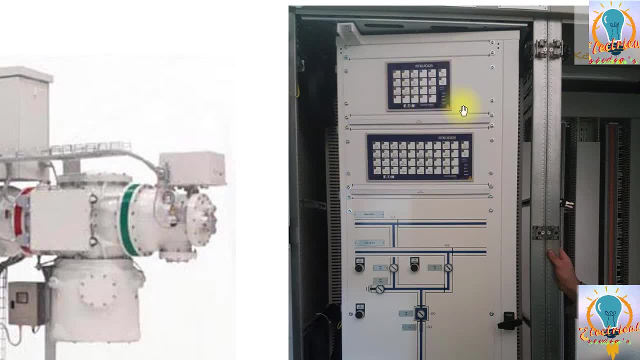 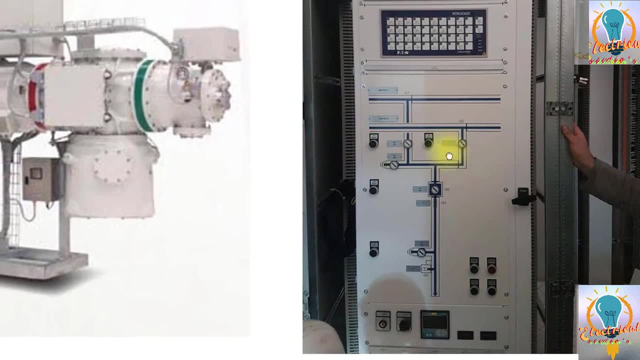 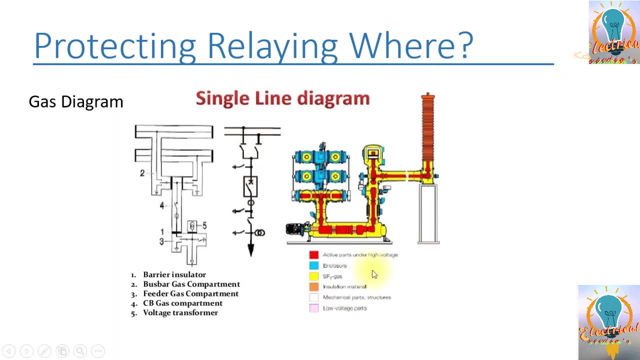 supply fail, the alarms will appear by AC and if the AC supply is failed and alarm are normally shown by the DC. so here you can see, and this is basically the single line diagram of the GIS, this is double bus bar and single breaker scheme and they have shown this. 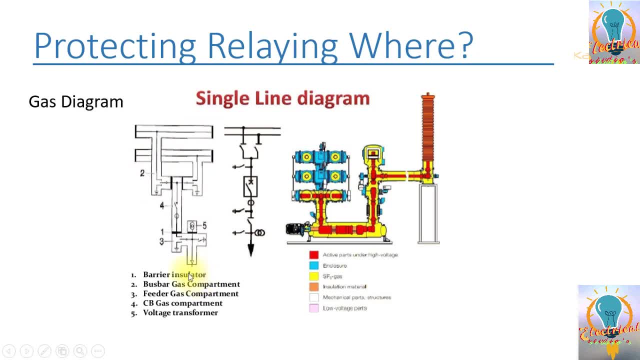 is called as a gas diagram, in which they have shown the gas compartment. so you can see, this is the gas compartment number three, feeder gas compartment, which has the VT, as we have seen just now, and it has the earth-like gas compartment and the gas compartment number three, feeder gas. 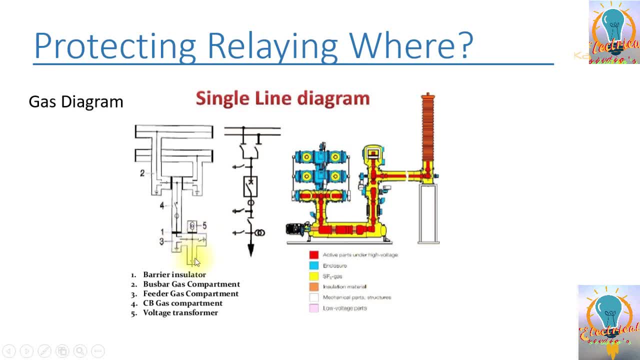 switch and and cable compartment. everything is in one compartment. this double door, this dark color line is showing basically the gas tight element. so you can see the voltage transformer has a separate gas compartment in in this case. so we have one, two, three, four, five gas compartments here, so one gas 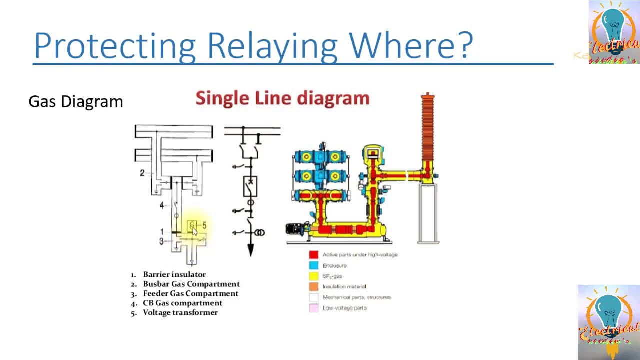 compartment is VT and the gas compartments are shown by a normally orange color, which are gas tight, and the parts which are not gas tight, for example, they are not shown by any color, or you can use a green color in that case. so this is. this is basically single line diagram. this is 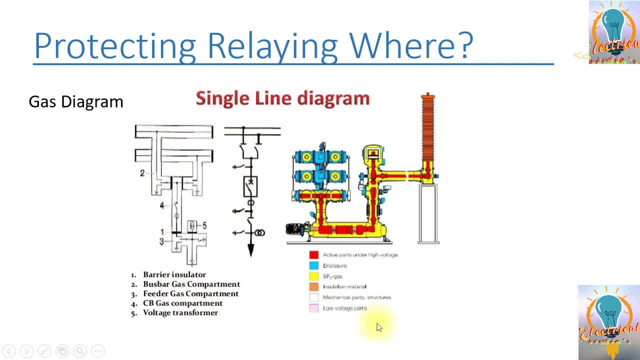 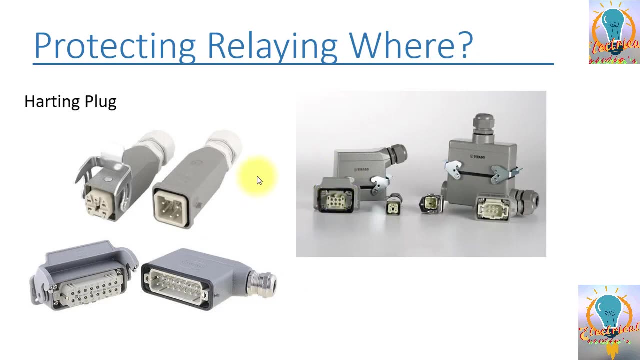 the is called as gas diagram, gas compartment diagrams, and this is basically the cutout that we have shown of a circuit breaker. just for your understanding. thank you very much. hello friends, in the section I will just go through some basic components which are used in the protection systems. this is basically an harten plug you can. 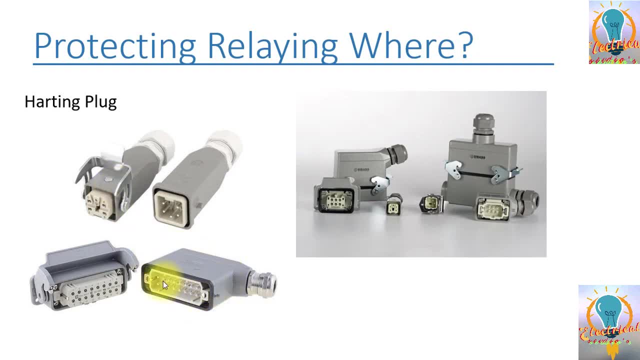 see, it's a plug. this is a main part of the harten plug and this is a female part. the main part is connected- here you can see- to the cable and instead of connecting wires to a terminal block, you can just plug in and plug out. a reason for using this type of hard in plug is that 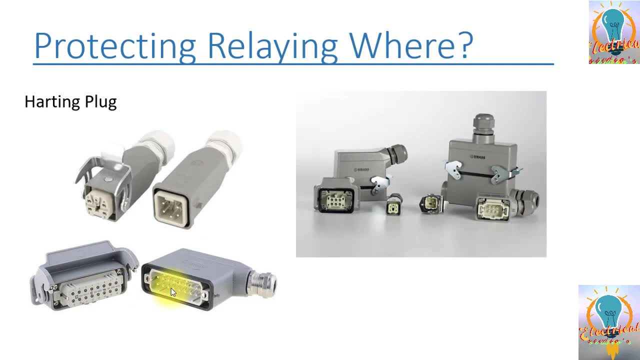 normally sometimes require to do maintenance and and you need to remove some of the component of the GIS. so if there are terminal blocks, and then it's, you will remove the wire one by one and then, after finishing the commissioning, when you put the part back, you have to connect it back one by one, so which is a 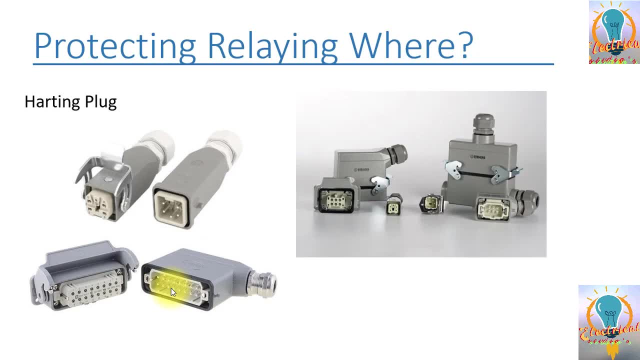 lengthy process. the second advantage of using this hardening plaque is when, during commissioning, for example, when the GIS is delivered outside, you just have to plug in these plugs. plugs are supplied along with the GIS and just you know. you should know the correct cable and the plug number, and then you 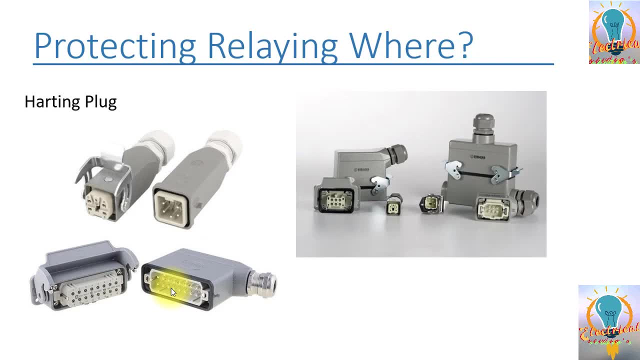 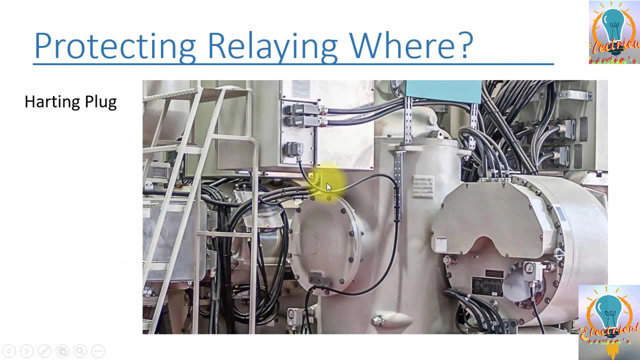 can insert the plugs and then you can switch on the hard thing, switch on the GIS. so these are some different types of hardening and commissioning processes: plug. so here you can see this hard plug is installed. here you can simply plug in the cables instead of connecting one by one to the terminal block. so you will. 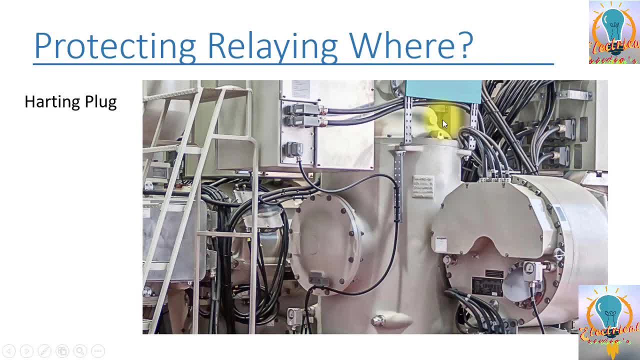 find this hard in plugs. everywhere in the GIS you can see this is basically this side is the local control cubicle and this is also connected by a hard thing: plug, so it's easier to operate and connect and remove. so it's very, very basic and good tool. further here in the GIS you can 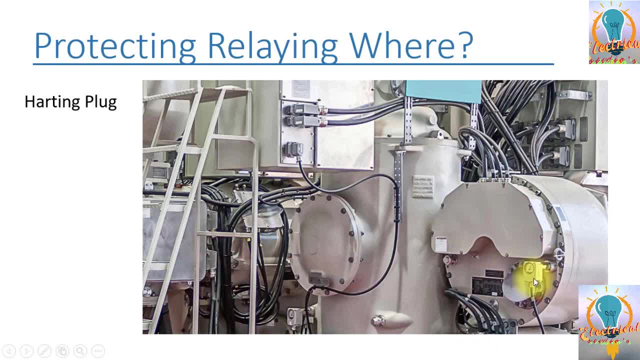 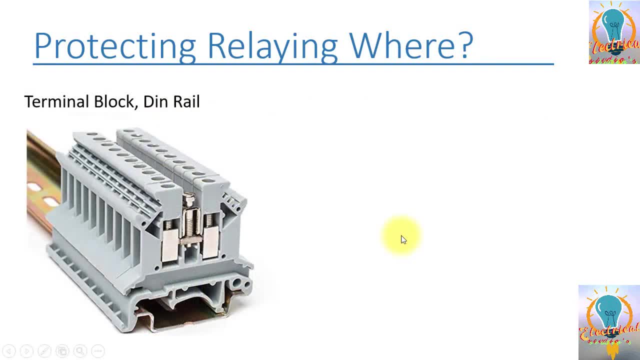 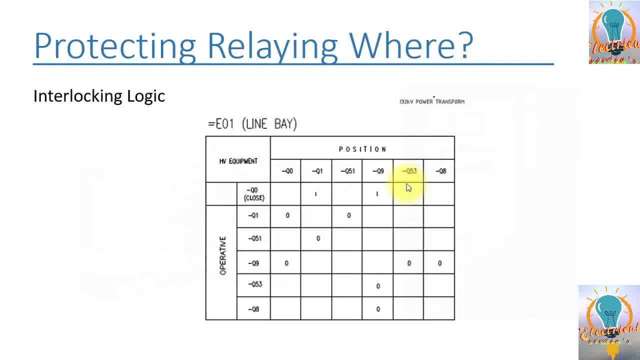 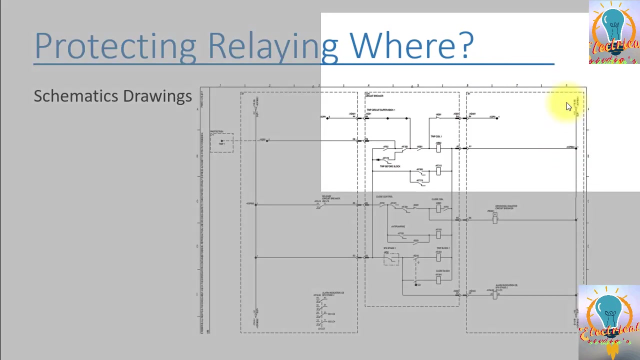 see. this one is basically the SSX gauge monitor, which is monitoring the SSX of this gas compartment where VTE is installed. so how does this hardening plug look like in the drawing I have shown you previously? let me take it back again. so this, this is the drawing of LCC that I have shown you previously, so you can. 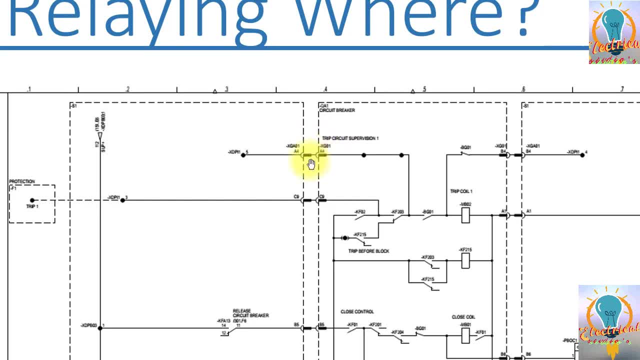 see here they have shown the hardening plug like: this is the male part and this is the female part. so they both of these compartments as one, and Q and circuit breaker- both are connected through the hardening plug. so in the drawing they are showing hardening plug like this: hey, friends, let's start our new topic and it is related to the hardening plug. 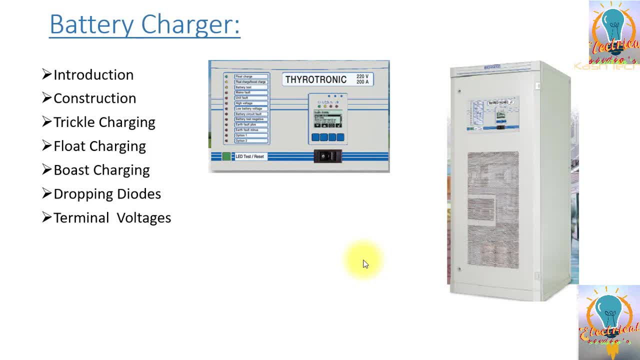 one of the main voids, based on the pinpoints which we successfully accessory to love making the best. so it's the small pinpoints of our finally interesting and very problem. we will refer U Hi array. this is just to build the tools сотrary, alternative and thin continuous output provinces to the Rock Tech storage, to the battery, charging rather than. 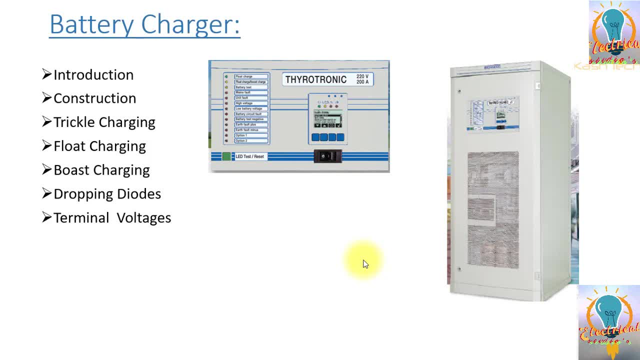 of battery. however, when the batteries get fully charged and their voltage reach at set value, the flow of charging current through the battery is stopped. the, the mains power source is derived from normally available AC source which is rectified by the charger. typically connection as shown in the figure. we will see this figure in the next. that how they are showing the connections. 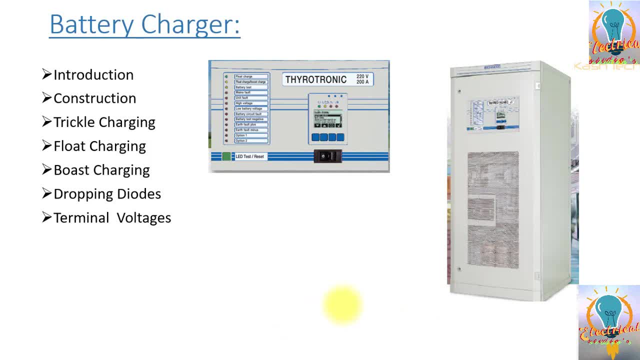 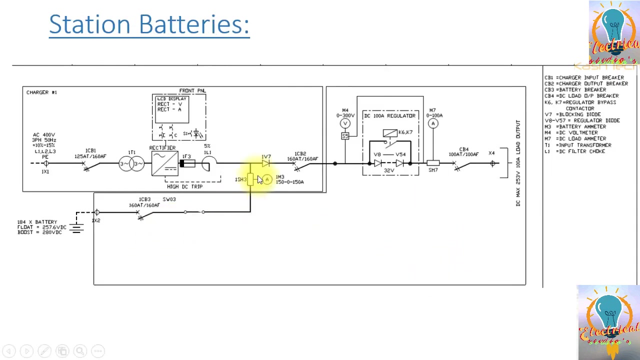 so then the function of this there. there are some functions available in this battery. one is trickle charging, one is floor charging, one is both charging and one of the dropping diodes and one of the terminal voltages. so we will discuss that later and we will also discuss these things one by one, and this is basically the single line. 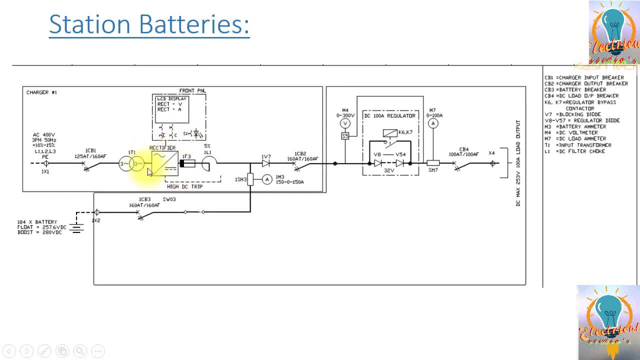 diagram of the station charger. so here you can see three phase AC supply is coming in and then there is mcb of 125 ampere and is basically then it's going to another three phase transformer and then it's going to rectifier. from after the rectifier also, there is basically a fuse. you can see fuse installed, okay, and then they have. 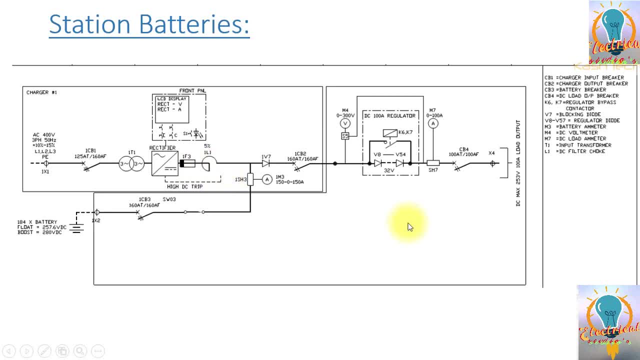 put a limiting reactor. so this il1 is a dc, this is a dc filter shock. so if still there is any ripples after the rectification, this shock will remove this ripples and then you can see one connection is coming and at this point the voltages. this is that terminal of the rectifier. 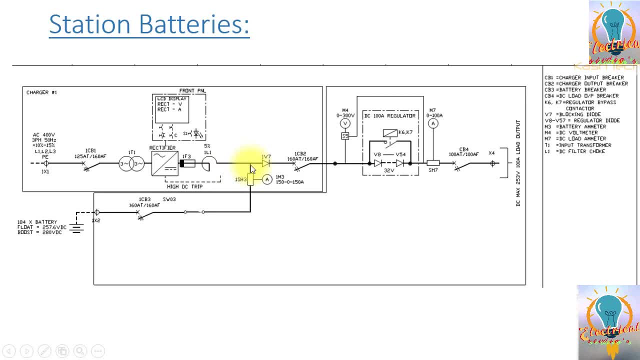 we can see, and the voltage available here will be called as a terminal voltage. so you can see then through ish3, which is basically a cutout fuse, and they have also installed a meter here and these voltage are fitted to that battery bank. so here you can see a 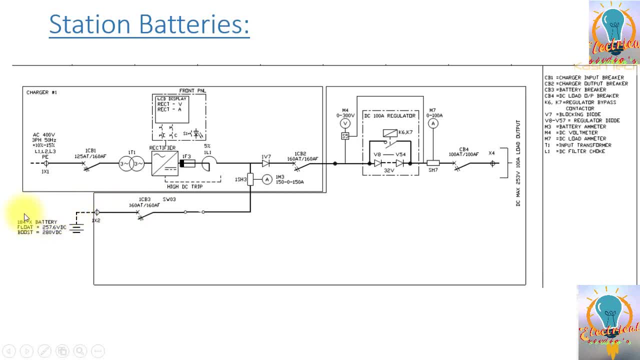 little voltage going here if we connect ish3 to it. so this is for normal cut off the. there is no in here worried about어. this is an soort of from a voltage package or there is not care battery bank installed and in this there are total 184 batteries and in during. 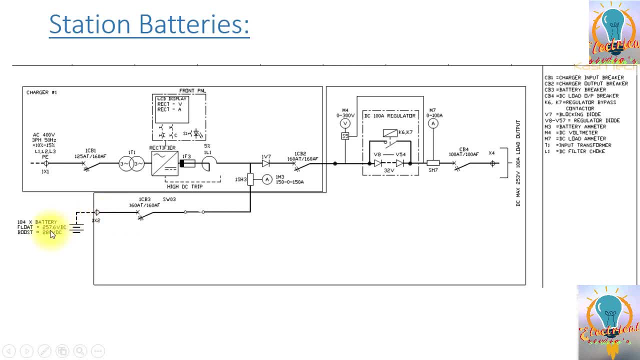 the float the charger will supply 257.6 volts and the float condition and in the boost charging the charger will supply 280 volts DC total. so there are the float and boost voltages in the charger. you need to set total number of voltages and the float and boost voltage per cell. so if you calculate here the 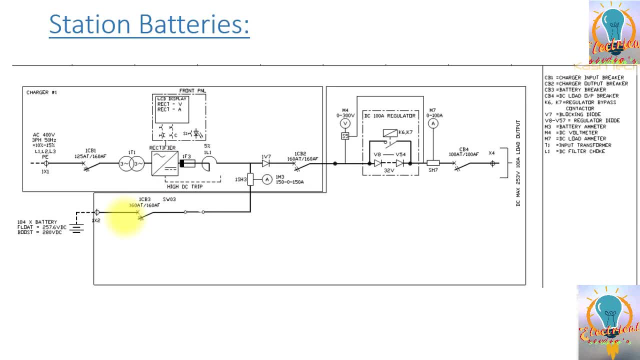 per cell voltage it would be float will be 257.6 divided by 184. so the float voltage per cell are here 1.4 and boost voltages per cell are 1280 divided by 184. so 1.4 is the current voltage per cell and the boost voltage per cell is 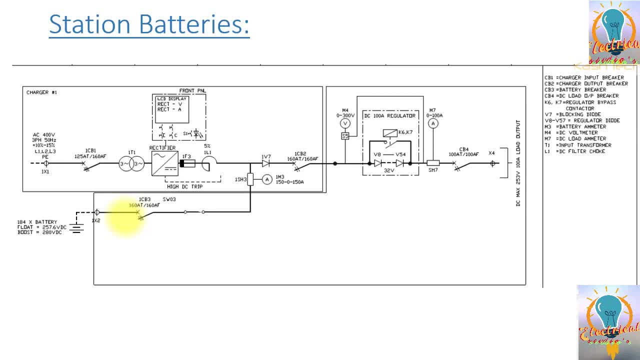 252 is the boost voltage. where is a battery rated voltage is around about, because it's a nickel, cadmium, so the battery rated voltage around about 1.2 volts. so you can say, normally the battery remains on float mode and when battery is discharged more or then it is, we are changing it to the boost mode. 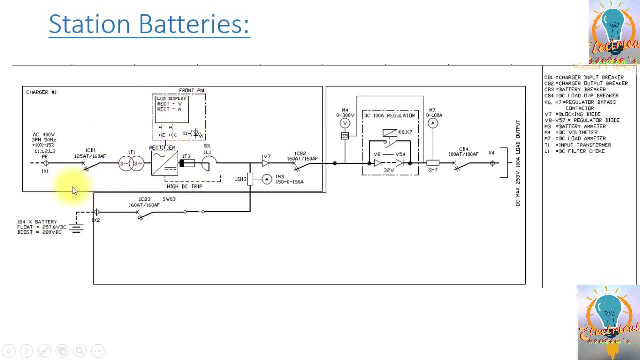 there is also automatic option in which the charger will check itself and it will convert the battery from float to boost automatically. you can see, and then from here the another connection is going to, basically here you can see, going to this trapping diode. so here you can see v7. here is a. 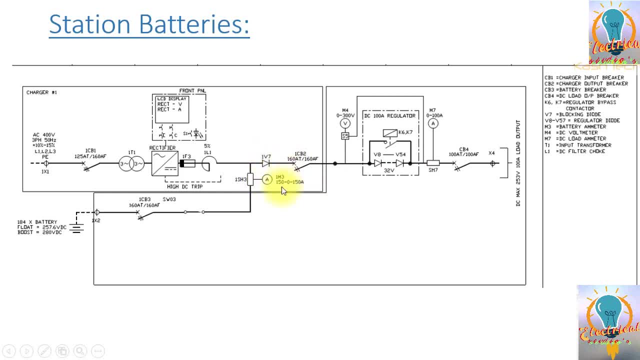 blocking diode. this is the blocking diode v7. so what is the purpose of this blocking diode? it's basically blocking any feedback from this side. okay so, and then there is a basically another MCB, and then you can see, these are basically the regulator. we are calling it as our 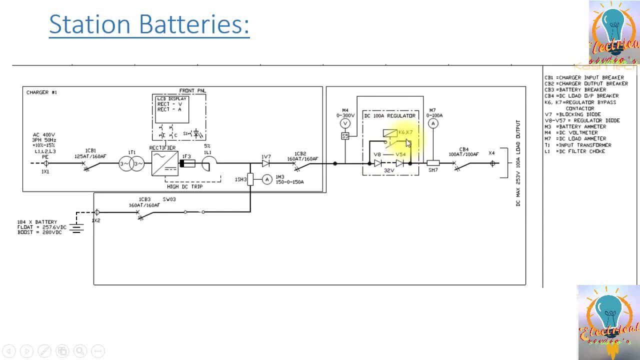 dropping diodes and this has two steps. you can say there are two contactors- use k6 and k7- and, for example, if k6 is closed some diodes will be bypass and if k6 is open, this diode will be in into the system. so when you are ordering any charger, you need to see that how. 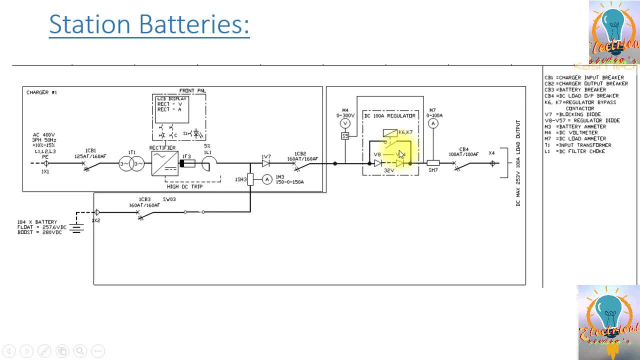 many dropping diodes are used and how many steps they have provided to control the voltage is, so more the steps. it mean that more regulation is possible and more the number of diodes between the total bandwidth will be more. and then here you can see, this is further connected to the DC distribution board. so 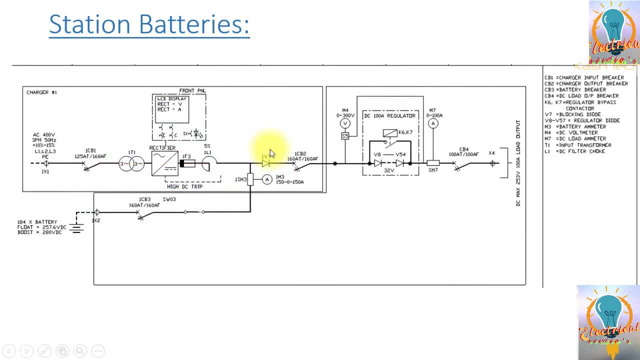 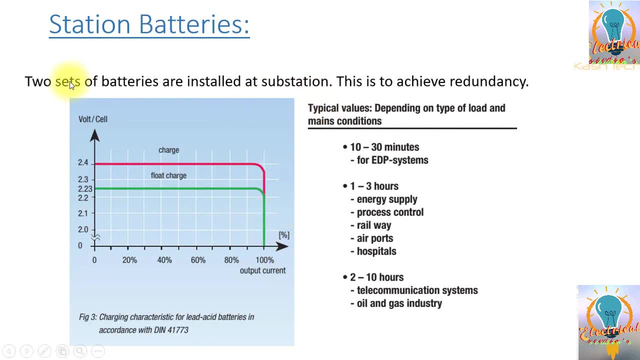 this is one of the very simplified diagram for the DC charger. here we have shown you two sets of batteries are installed at the substation. this is to be achieved at a latency. so always we are installing two sets of batteries and two set of chargers sometime. I have seen there are three charges installed in the 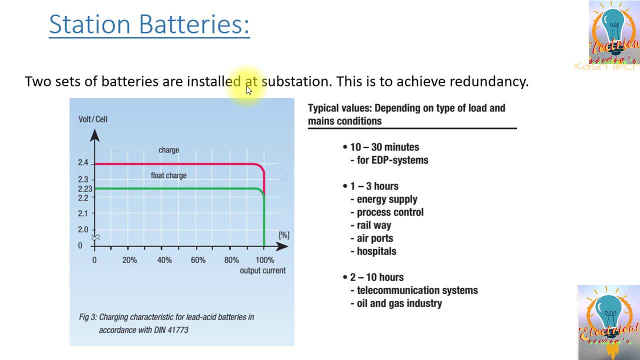 substation. so one charger is kept as a backup. so if one charger is failed, so another charger comes into the action. so here you can see. these are the chart which is showing shown for lead-acid batteries. so the float charge is for lead-acid batteries is 2.23 and the boost charge is 2.4 volts. and here you. 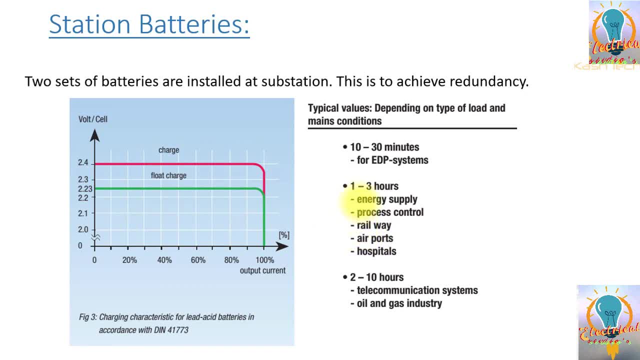 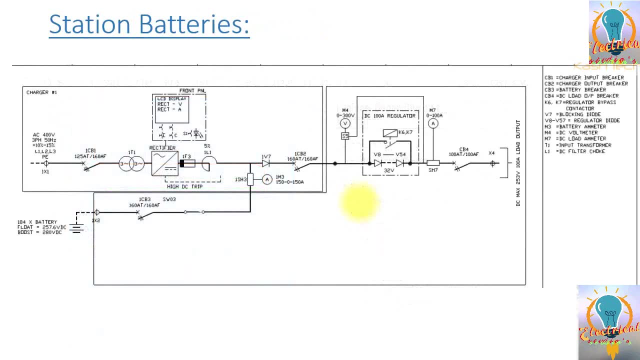 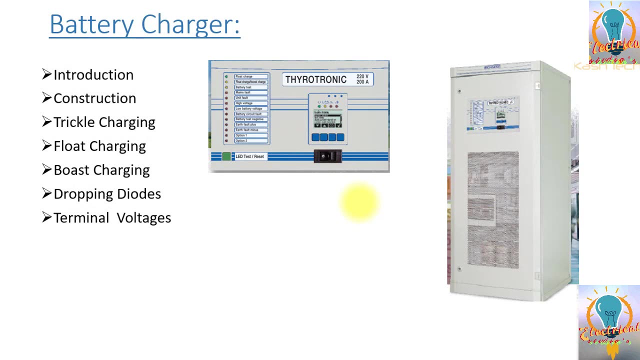 can see, there are some typical type of charging time for different type of systems. so this was a brief introduction about basically the the battery chargers. so now we will go through some definitions of float chargers. float charge and both charge and dropping diodes. so the float 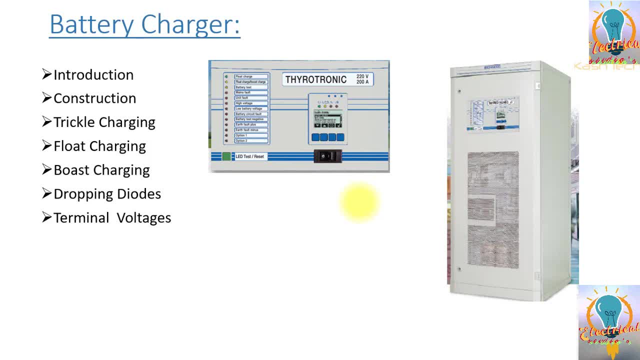 charge is keeping the voltage applied to the battery at the manufacturer specified float voltage per cell, which is normally 2.25 for lead-acid and 1.35 for nickel cadmium, multiplied by number of cells. such setting adjustment, which is normally available in charger, is carried out before. 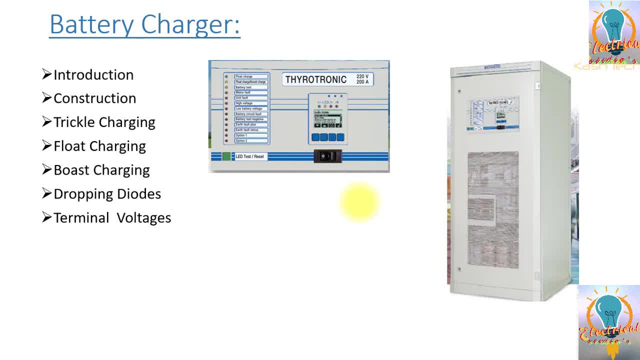 connecting the battery with the charger. this will this therefore maintain a constant voltage across each cell and the battery bank as whole. this method is usually adopted in conjunction with supplying continuous variable DC loads from the charging equipment, as should, as would typically happen for substation batteries, the load in a substation normally 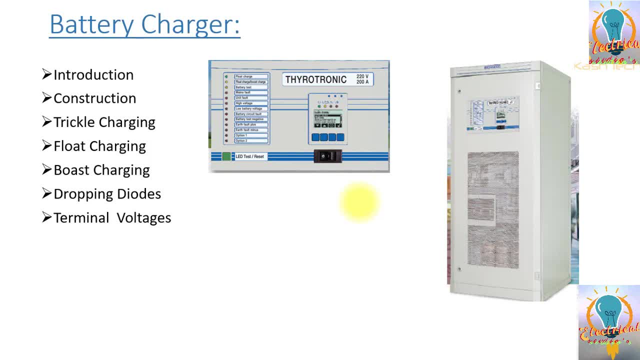 comprise of small continuous load consisting of pilot lamps, relays, etc. and momentary short time load of comparatively high values, such as those for circuit breaker, tripping and closing operations, motor spring and so on, since the charger battery and loads are all connected in parallel. the continuous 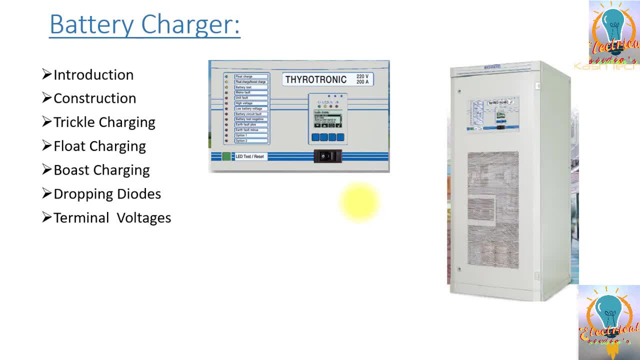 load is carried by the charger at normal floating voltage and the battery draws its own maintenance current at some. at the same time, any load that exceeds the charger capacity will lower its voltage slightly to the point where the battery discharge to supply the remainder if there should be complete. 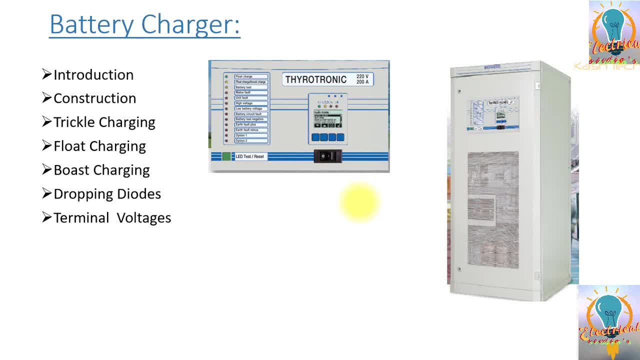 power failure, the battery will supply entire load for a period, depending upon ampere hour capacity and the load, until AC power is stored and then automatically starts being recharged. typically, float current will be in range of 30 to 50 milliamps per 100 ampere hour operated capacity. 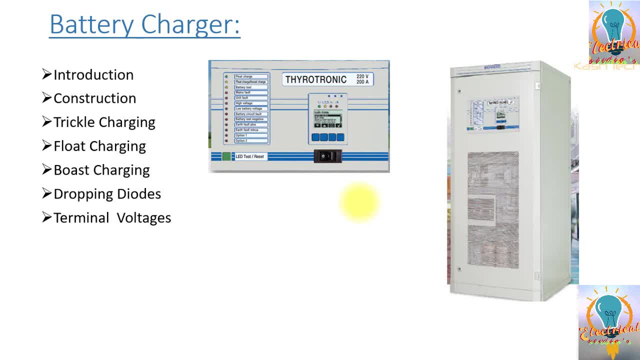 increasing to about 10 times towards the end of battery life. so boost charging. boost charging is a fast charging process through which relatively high voltage is applied across battery, which causes higher charging current to flow. here also, applied voltage is, in accordance with the manufacturer's specified boost voltages per cell. similar to float charging process, the battery bank boost voltage is: 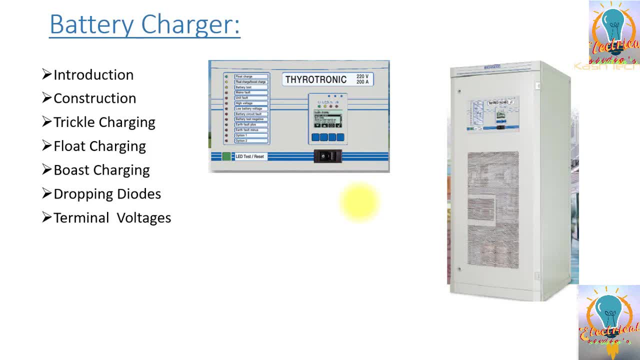 also adjusted in the charger. the process is normal, normally adopted when battery is sufficiently discharged due to supply or charger failure, however, battery manufacturer recommend to carry out process after some appropriate intervals- may be about six months- even if there is no any charging source failure. this improves serviceable. 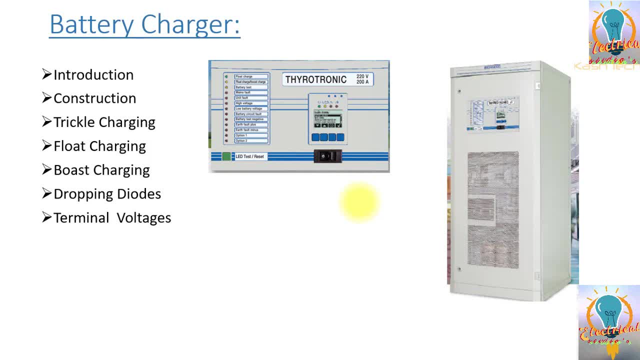 life of the battery. trickle charge: trickle charging is a method of keeping the cell in fully charged condition by passing a small current through them. the correct trickle current is that which does not allow cell to discharge, does not allow cell to discharge gas and does not allow a specific gravity to fall over period. The cell voltage will be. 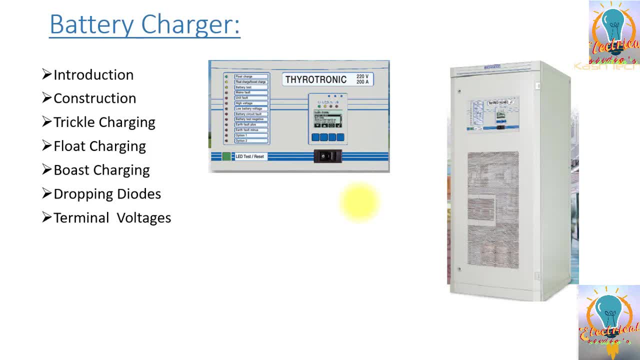 approximately 2.25 volts for lead acid battery and 1.35 volt for the nickel cadmium batteries. So these are some definitions and some theory that I would like to share with you. So I hope you enjoy my lecture. Thank you very much. Hey, friends, in this session we will see the two. 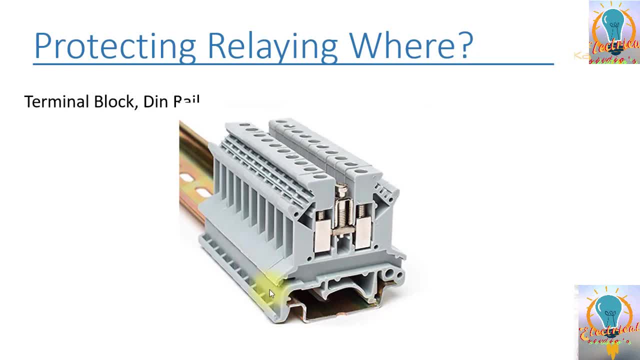 different components. One is terminal block, another one is general. Basically, you can see, this one is a terminal block and it is installed in almost in each and every protection and control panels, And this metallic U-shaped bar is basically called as a DIN rail. So this terminal block is locked. 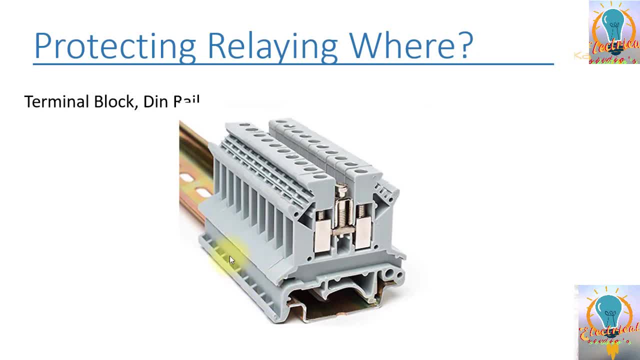 on the DIN rail and it can be removed also And the DIN rail is mounted on the panel. You can see this area where you can put a screw and then you can mount it on the any panel wall. So how terminal block look like in the? 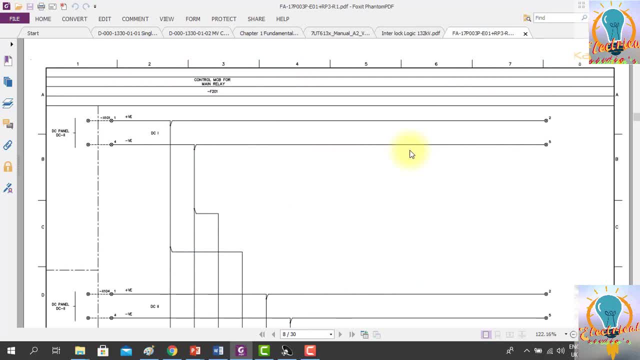 rail And another one. we compared this to a higher terminal block. This OFF Lamina, is the one which is not on the panel wall, that is, it's the same as the other vehicle You can use or, If you use, It's opposite neighbors, as in real- lets call it with surgery. You can see. 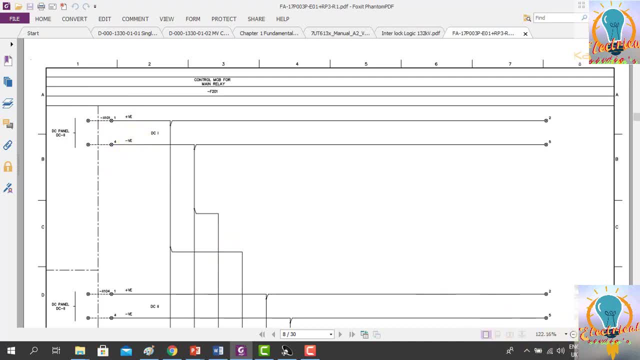 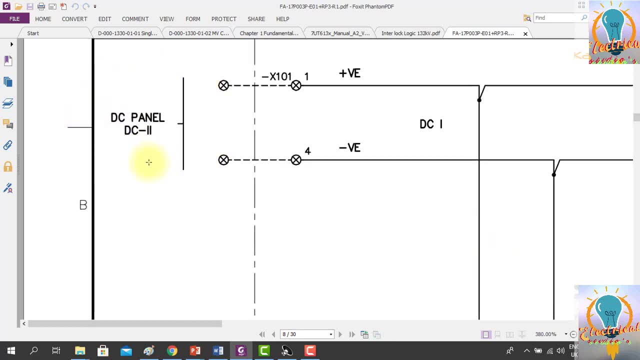 this here. As you can see on example, it is a terminal block. If you're going through the terminal Automotive � demo, look at this. This terminal block depicted here after only the type of직 huin the terminal block Press UI Screen wheel when going through the terminal U-S szyb Cream wheel drive. so let's open the drawing for the sample so you can see this. they have shown a terminal X, 1, 0, 1àn and 4. this is a positive and negative terminal. here you can see a deep minus for a DC power supply is coming from external. 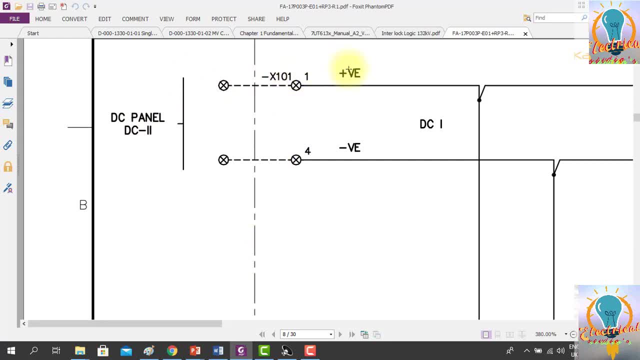 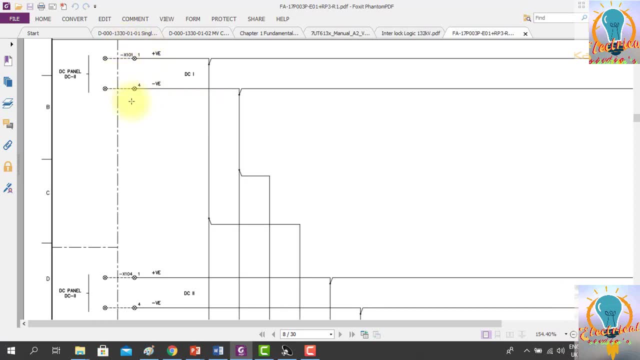 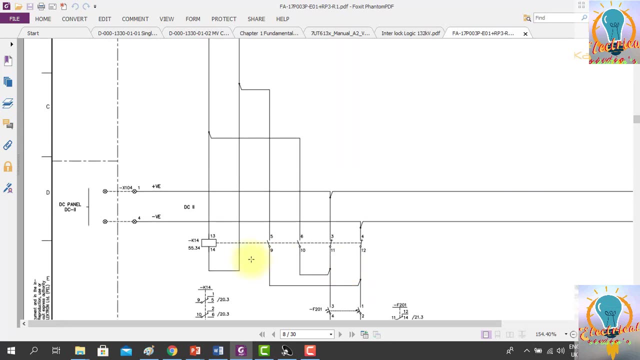 and it's coming to the terminal blocks. x101 positive and x1014 negative is coming, so the terminal block are shown like this in the drawing. then another supply is connected here. also here you can see dc panel, dc2, x1041 and 4 is connected. 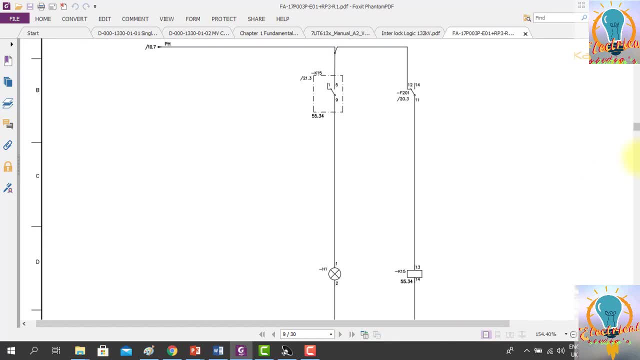 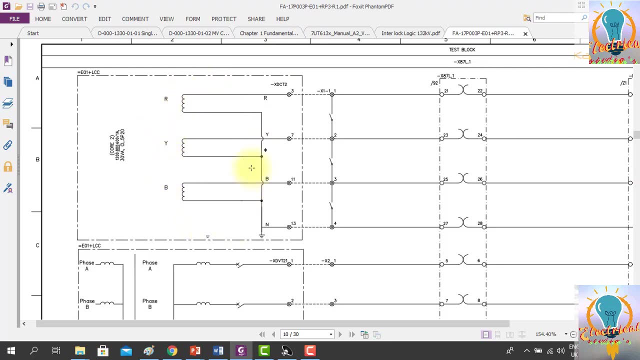 so this is how the terminal blocks are shown in the drawing. so we will see further. go through the drawing. you can see, and this is the cd circuit and it is coming from core 2 of the ct and then it's connected to the terminal first x. 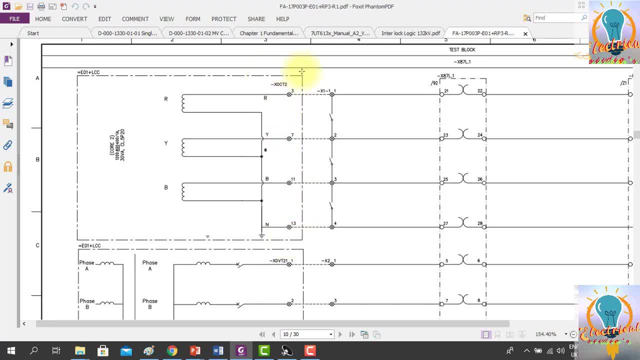 3, 7, 11 and 13 of xd cg2. and this is this terminal is in the lcc. you can see this is lcc panel e01 lcc. and then it's coming to this protection panel r03, r1, to the terminal x1-1: 1, 2, 3 and 4.. so this is a little introduction about the terminal block. 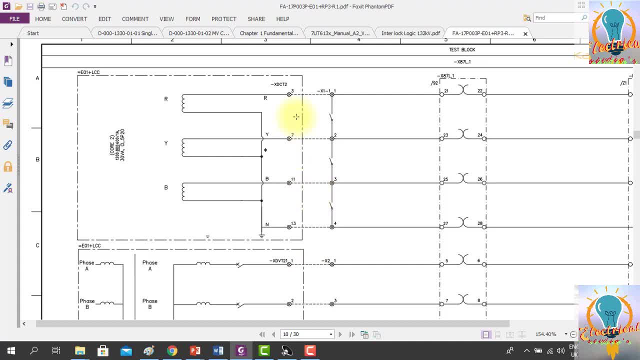 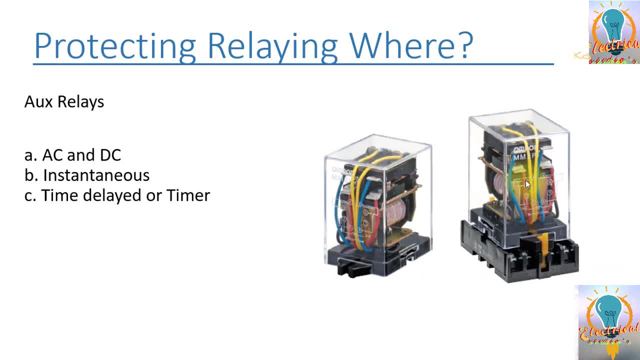 and if you want to know in detail so you can check another on my other trainings on the production systems. thank you very much. hello friends. in this section we will study about auxiliary relays basically. auxiliary relays are basically used to prepare a schematics, control and production schemes. also, these are used as a supporting role. 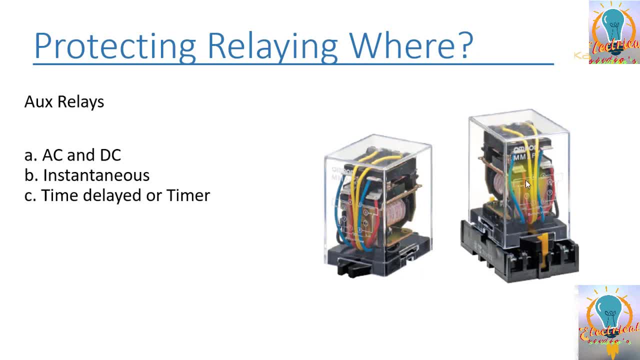 to the main relays. alarms, indications and sometimes trippings are also connected through this auxiliary release, interlocking. if you want to make an interlocking circuit you need to have auxiliary relays to perform different interlocks. so all these relays are function as an addition to the main. 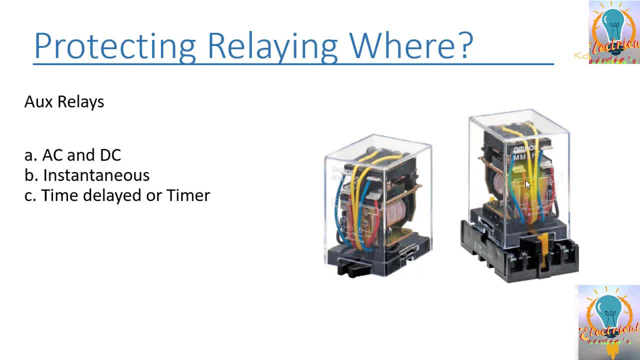 relays. so main production relays are basically sensing the actuating quantity, voltage, current, frequency etc. and then they are comparing it with the preset value and then they are making some decisions, alarm stripping etc. whereas this auxiliary relays have a more of kind of supporting function and and these are used in this, in control and production. so there there could be 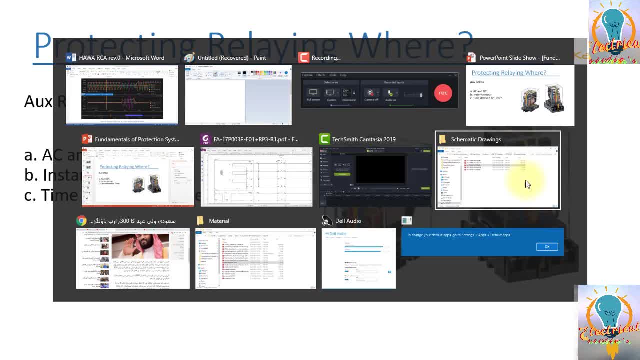 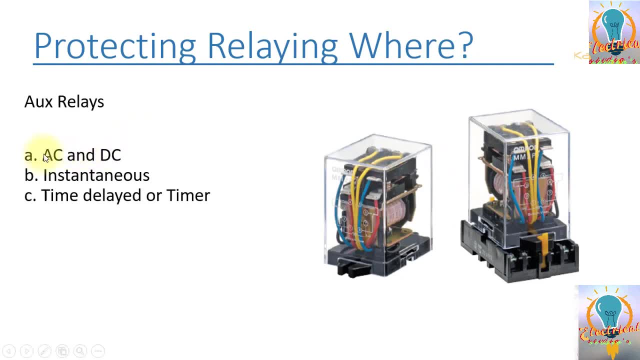 a few types of auxiliary relays, so one could be one could be auxiliary, could be ac or dc. it mean that there are auxiliary which operate on ec supply, whereas there are some auxiliary relays which are energized and used on dc system. so then we have 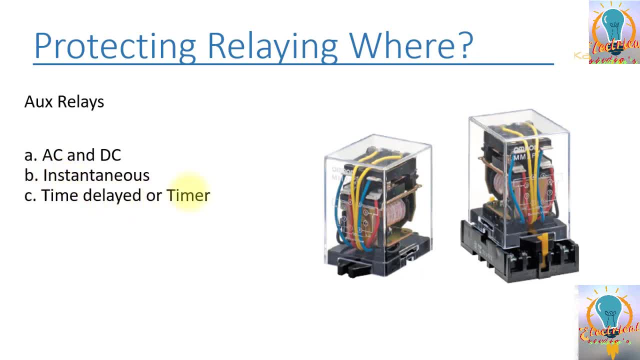 can be classified as instantaneous or time delayed or with timer. so always have can be instantaneous. type when mean as soon as you energize and auxiliary it will operate. or it could have an a timer, so as soon as it is energized the timer will start and after preset time it will operate the contacts. so here you. 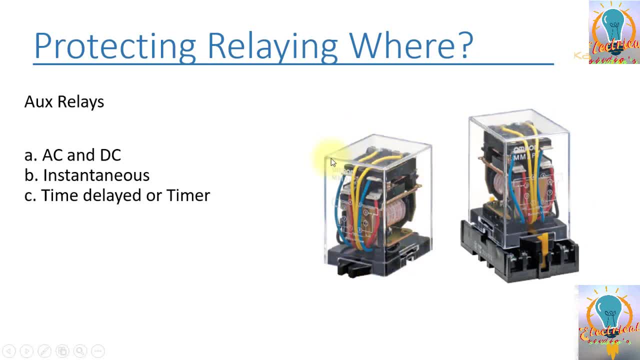 can see in auxiliary relay. this is basically auxiliary relay and this black color downside is basically that it is called as a base of auxiliary. so the auxiliary relay, here you can see, is connected to the base and it can be removed from the base. here you can see the auxiliary, another type of auxiliary. 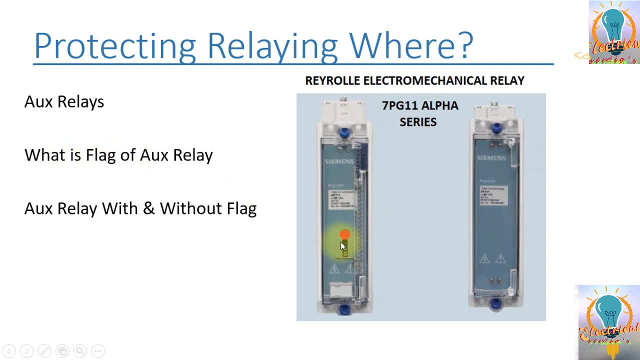 relays which are with flag, and this is one is without flag. basically, each auxiliary can have flag or cannot have flag, depending upon your ordering. so some auxiliary relays have that have flag. it mean that when this auxiliary relays are operated there is a flag that appear. so when the condition is reset, this flag 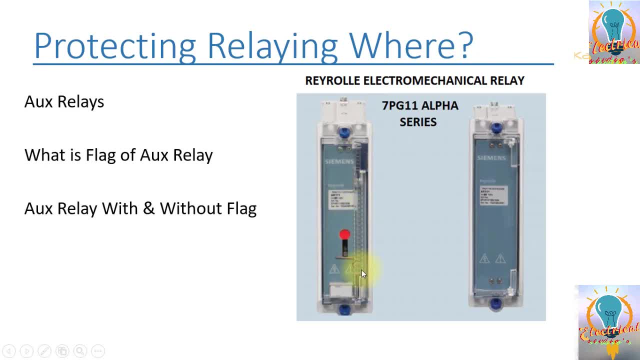 will not reset automatically. so you can see this is they have given a reset button here. you have to push it and then it will will be reset. so there are some auxiliary relays which are self resetting and which flag is will be reset automatically. but there are other auxiliary relays you have to reset a. 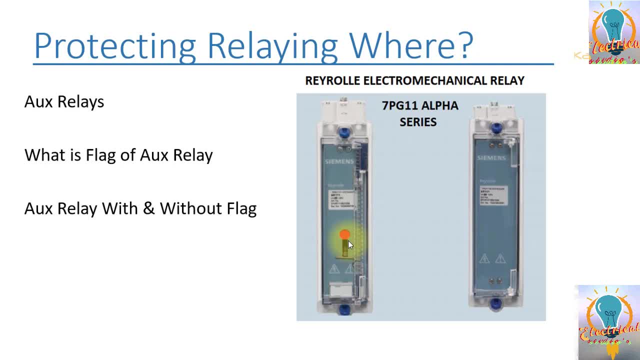 manually but there is a flag when the relay operate. the flag comes. for example in this case, if the relay is connected to some monitor, the DC supply. if this is a player file, this flag would come and you need to read, reset it manually and this relay is coming without any flag. so you can see here another type of 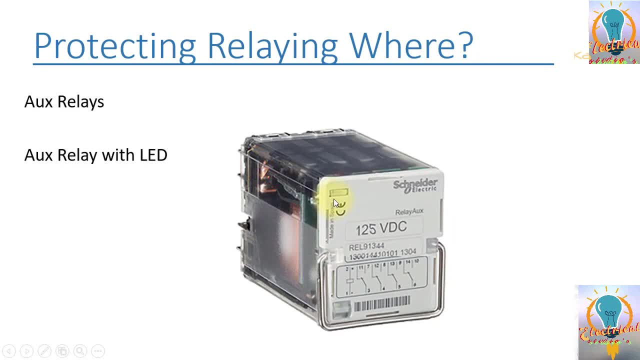 auxiliary relays. so this type of- obviously, when this relay is is basically power on, it has an LED or when it's picked up, this LED will be on. so by checking this LED itself you can, you can check and you can confirm that the relay is picked up and energized. here you can see there are some contacts. 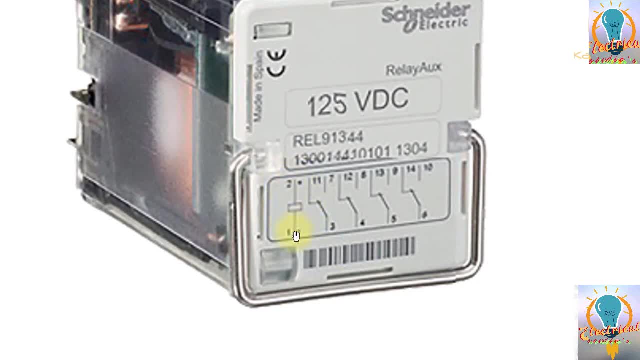 they have shown. this is basically the coil of the auxiliary relay, and one you have to connect to negative and two to the positive. this is a DC supply relay and these are the contacts of auxiliary. so you can see when these contacts are drawn, when, when the relay obviously is considered as de-energized. so you can. 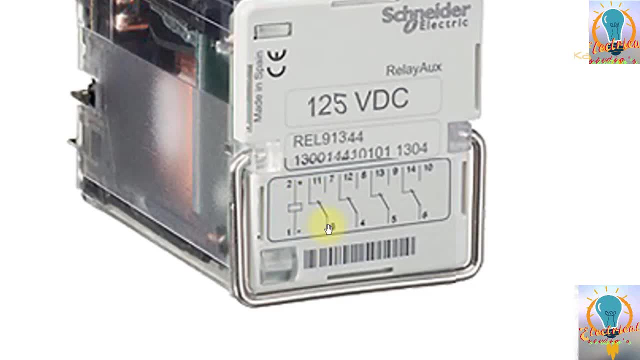 see here that it has one, two, three, four change over contacts. so three and eleven is, you can see, a normally close contact and seven and three is a normally open contact. so normally close contact is contact when the relay is de-energized. this contact is closed. so you can see it is closed at. 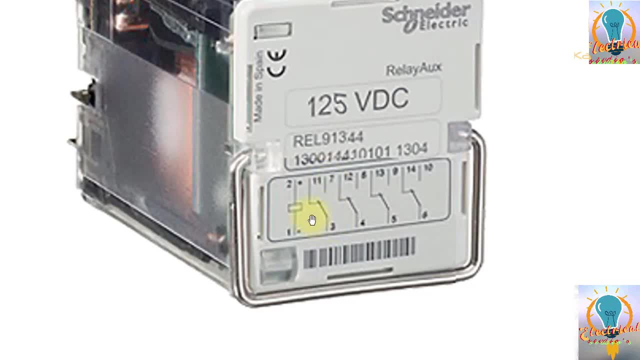 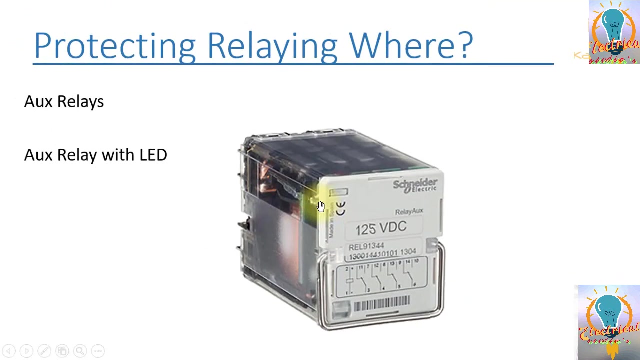 the moment. and 713 is normally open means when the relay is de-energized, this contact is open. so this is a little definition of normally closed, normally open contacts and these are change over contacts. you can see this contact changes position from 11 to 7 so you can utilize these contacts for interlocks, alarms in the. 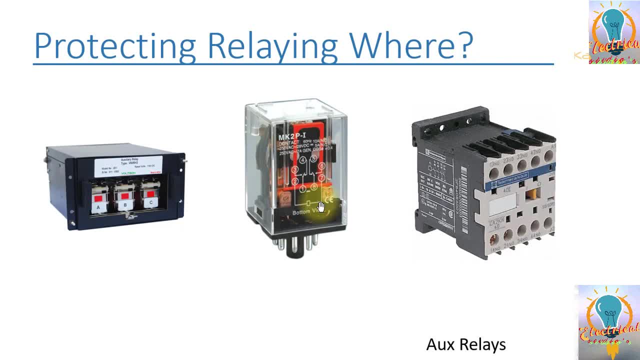 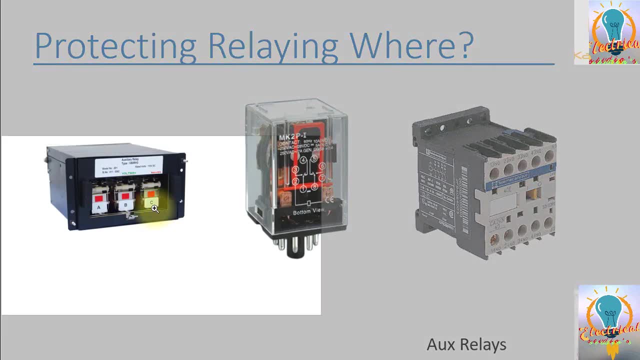 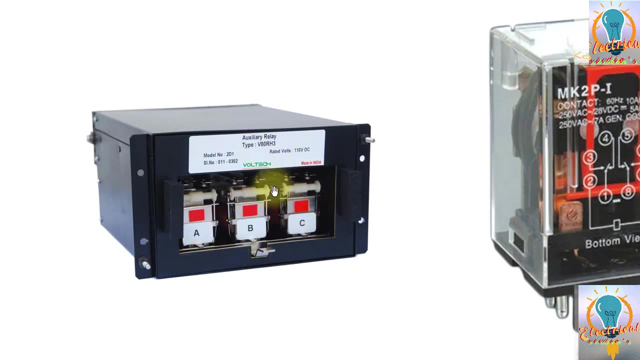 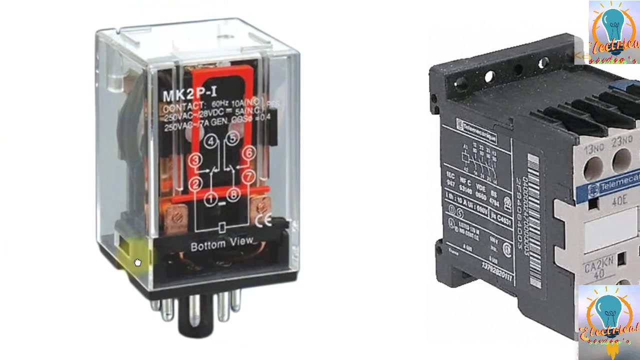 scheme. so here you can see more other types. this is another auxiliary relay and you can see this is type is V80 RH3. so you can see it has the flag. as soon as it operates it will give indication. here you can see this is another auxiliary which is will be mounted on the base as I have shown you. 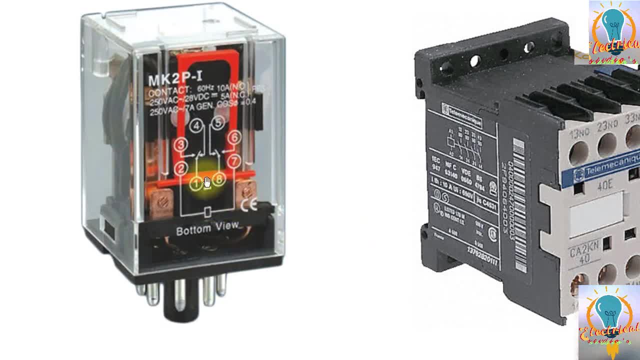 previously and they have shown here. you can see, they have shown it has to change over contacts. so and the supplies connected to two and seven. the supply of this coil is connected to two and seven and it has two changeover contacts. so you can see here that normally close contact is at 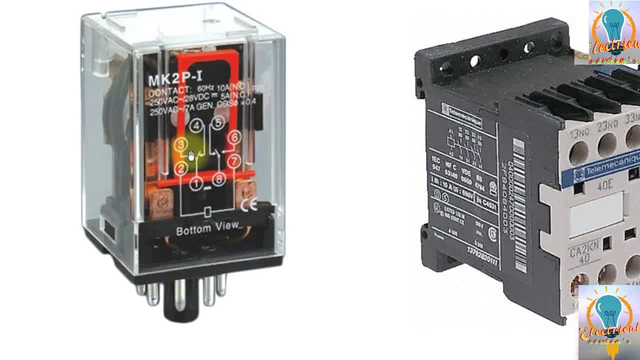 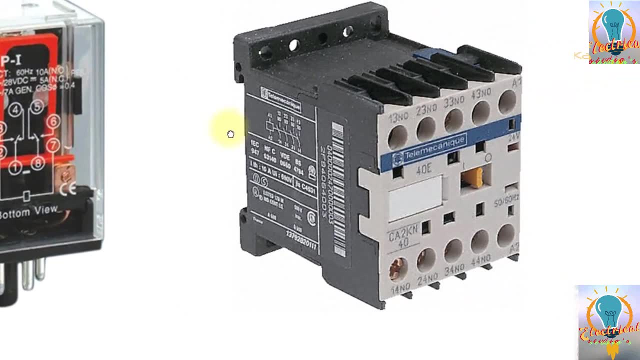 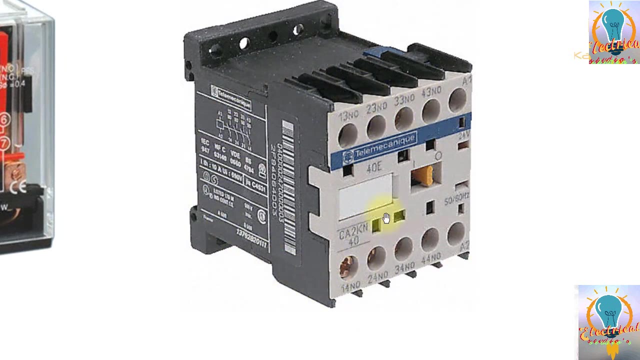 one and four and normally open in the one and three, similarly normally close contact. another is at five and eight and normally open is at eight and six. this is basically a this also auxiliary, but we are calling it as a contactor. typical trunk for this type of device is a magnetic contactor or a contactor. 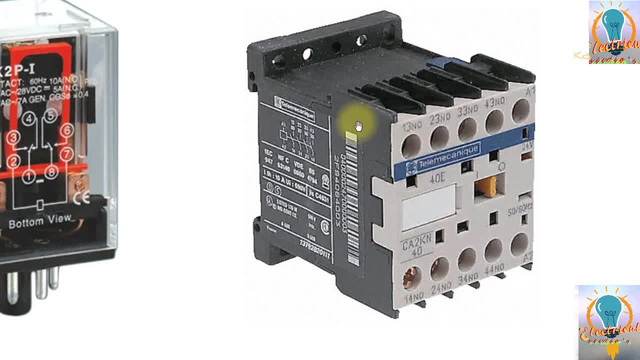 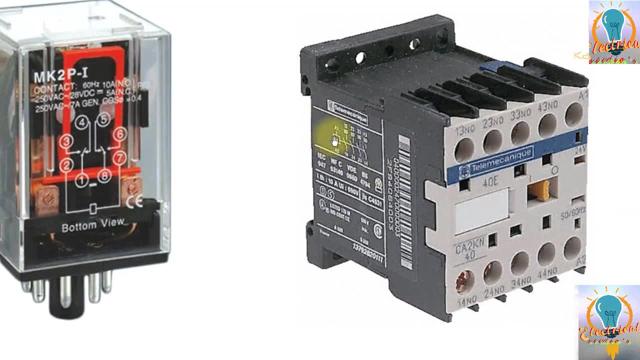 this is heavy-duty. it has a more capacity, current carrying capacity, than this, this small relief. so here you can see. they have also shown the coils a1, a2 and they have shown the contacts available in this contact. it has one, two, three, four. normally open contacts are available for this. 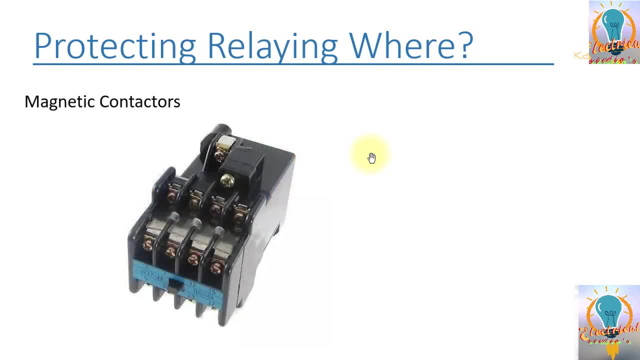 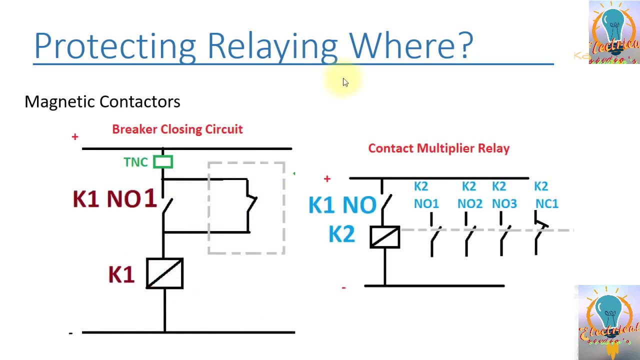 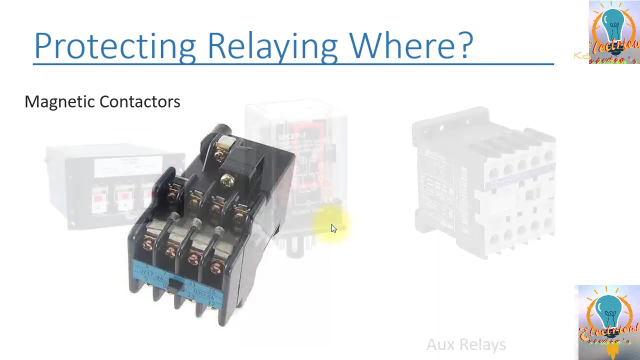 you. this is another lecture for the magnetic contactor, so here you can see how the auxiliary is drawn on the circuit. so this is basically auxiliary and it has these contacts. when the relay operates, this contact will change its position. so this was a little introduction about the auxiliary relay. I hope you enjoy this. 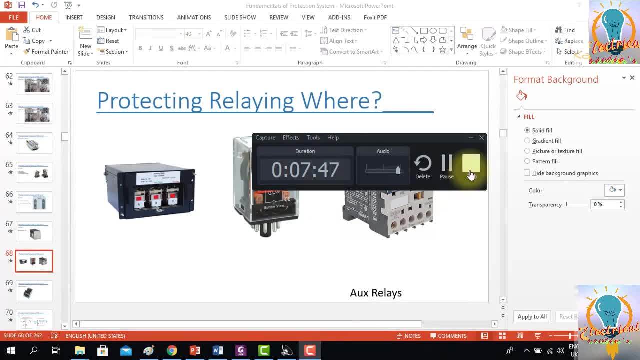 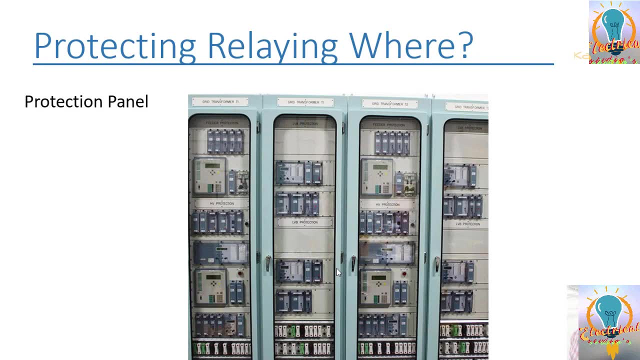 section. thank you, hey, friends, if you visit any substation you will find protection panels. and what are protection panels? in the protection panels, all the protection devices are installed which are put a protecting a specific part of the equipment of the substation. it could be any of the devices which are installed which are 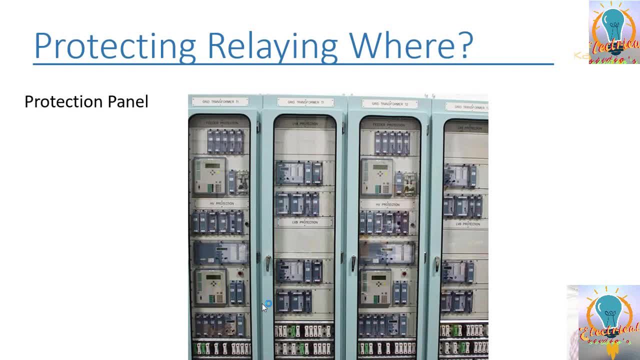 protecting a specific part of the equipment of the substation. it could be like line, it could be like transformer, shunt reactor, circuit breaker. so there are a lot of protections available. so here you can see, this is a panel where you can see a lot of protection devices are installed. so this is basically this. 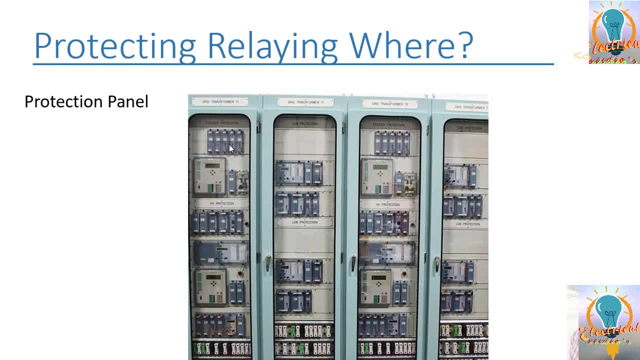 big one is the main protection relay and these are- you can see these are small- are the auxiliary relays which are installed. this is again the main production relay we are calling and this is basically the main production relay. again, this is the auxiliary protection relay. so this is the main. this is the main. 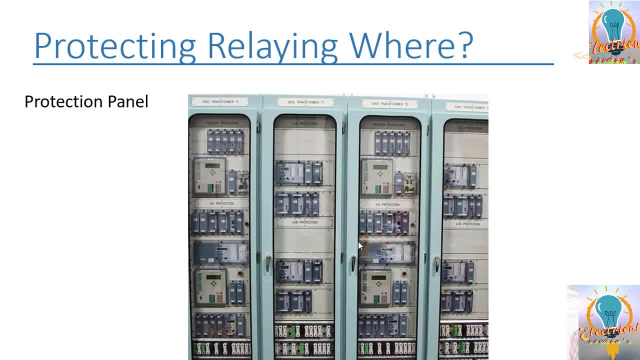 main and these are auxiliary protection relays. so a protection panel is basically. you will find the components like main protection relays, auxiliary protection relays, terminal blocks. you will find door switch, a bulb, AC socket. you will find terminal blocks. you will find external internal cables. you can. 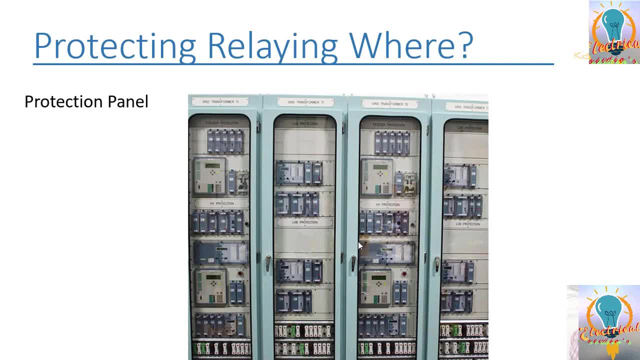 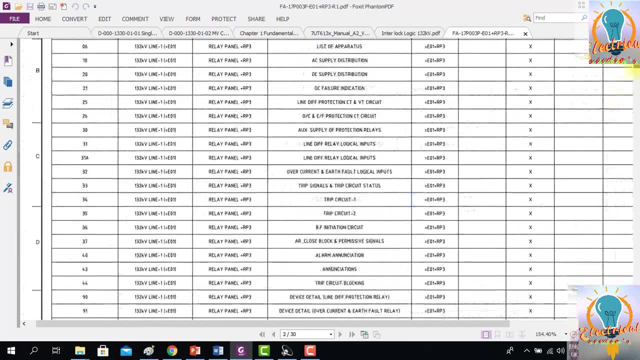 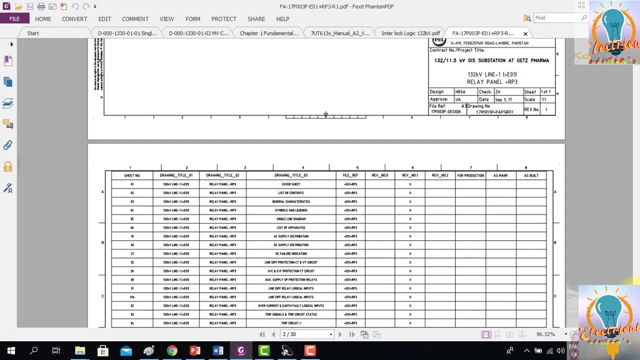 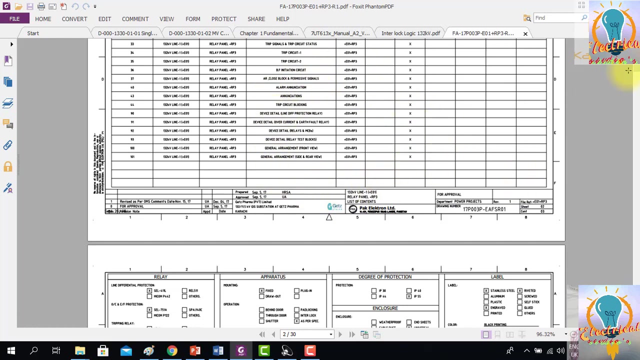 find the earthing plates and auxiliary relays. you all such stuff is available in the protection panel, thank you. so I thought worthy to show you protection secondary drawing for a protection panel. so this is how the drawing start. in the start you can see the cover sheet. it's telling you about how many pages are. 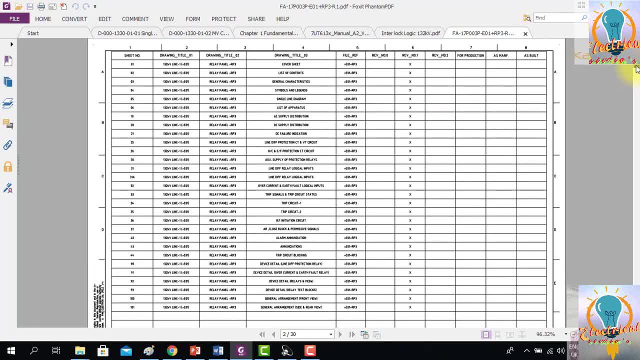 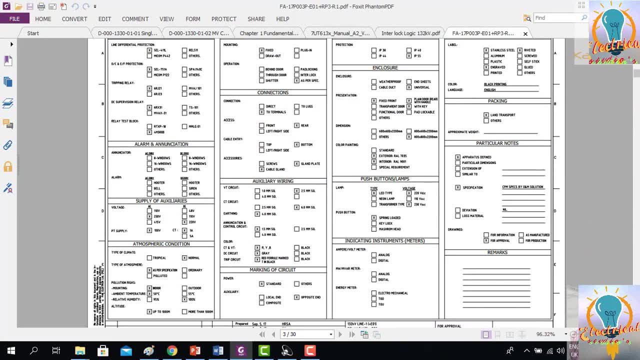 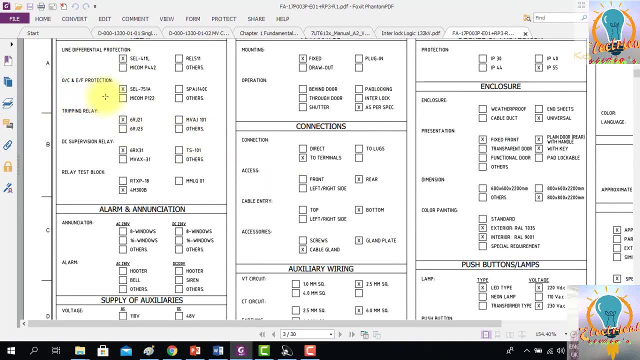 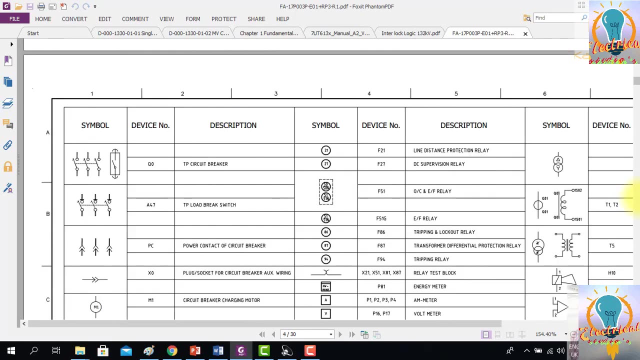 available in the drawings and what is on each sheet especially you can see. then you can find different operators here. for example, which relay is installed and the line differential is: L 411 L, over-canned earth fault protection trapping relay, DC supervision relay. so all the details are shown here. then you 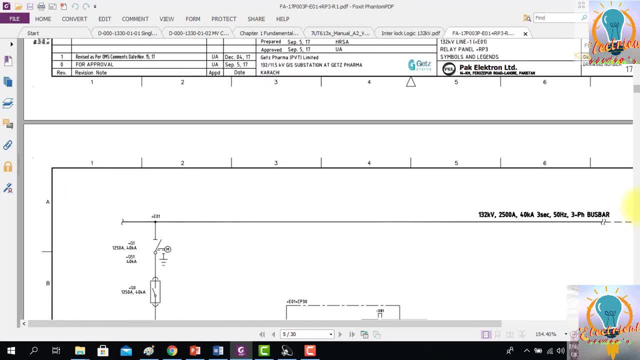 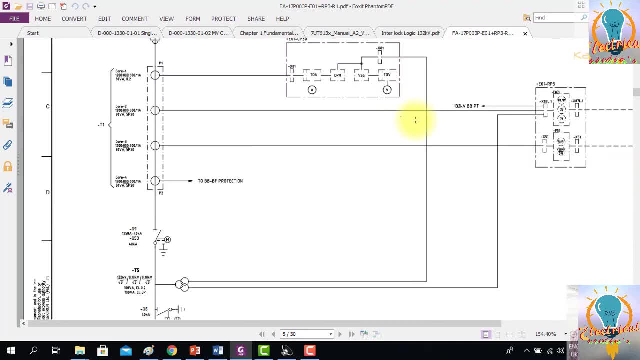 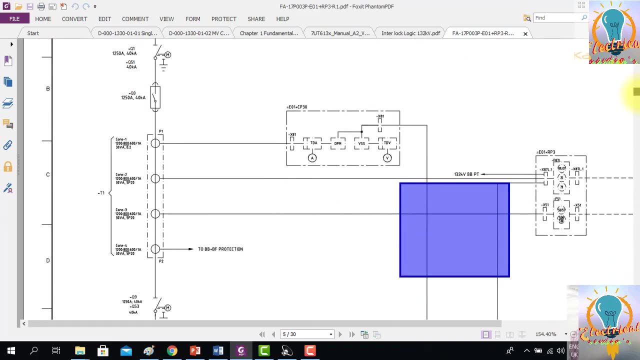 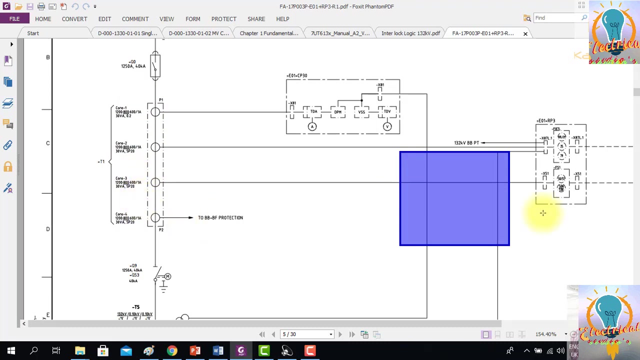 can see in this drawing. the symbols legions are shown here in this protection and control drawing. further, they have shown a single line diagram here in which you can see all high-level information like how many CDs and VTS are installed, which release are installed. you can see there today are shown the four codes. here then they have: 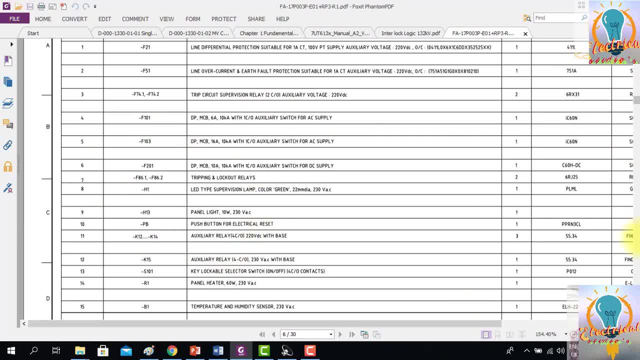 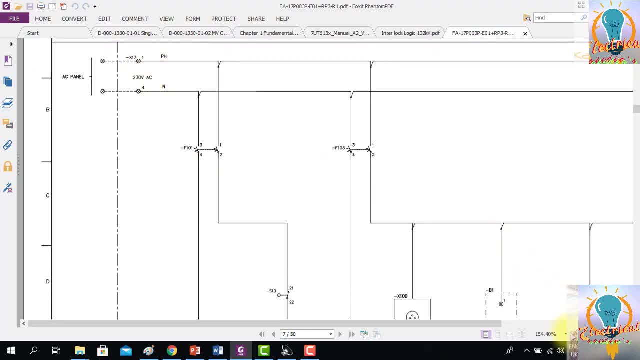 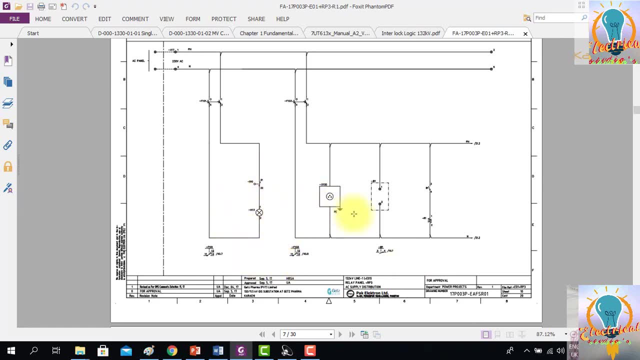 listed down all the components available in the production panel. here you can see the digital design is starting. they have shown how is supply is connected, so in each trial. this is the lamp and this is the AC socket. this is basically the humidity sensor, and here you can see this space. 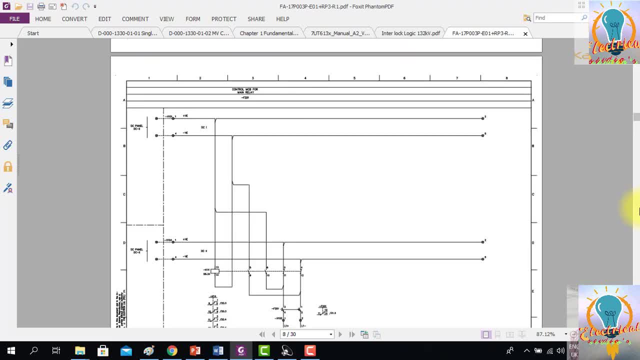 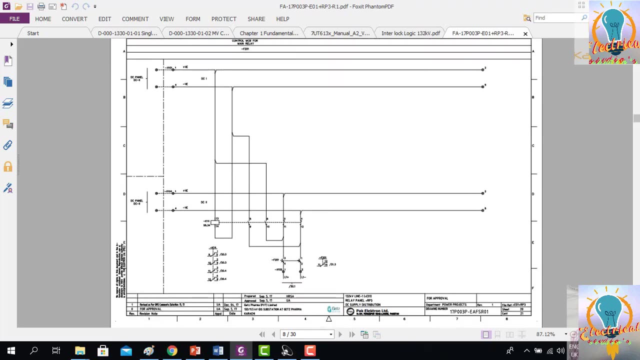 heater is installed. a space heater is installed in each protection control panel to control the moisture. so if there is a moisture, then there there is a chance of resting. so as soon as the temperature falls below the set value, the space heaters are switched on and then you can see the twenty supplies are. 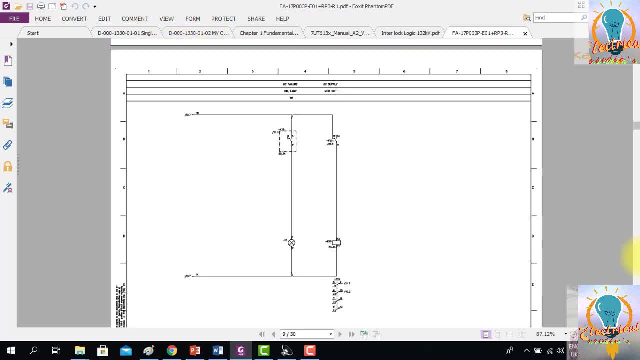 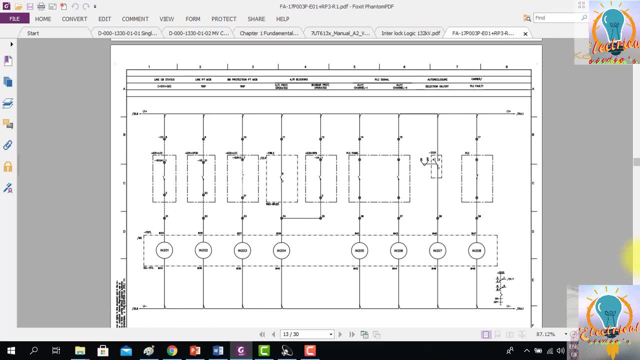 coming to the panel and this is the changeover. then they have shown basically the CT and VT circuits. I'm just taking through you very fast and how protection schemes and detail design look like. and here you can see these are binary inputs. different inputs are coming from the field, like circuit breaker. 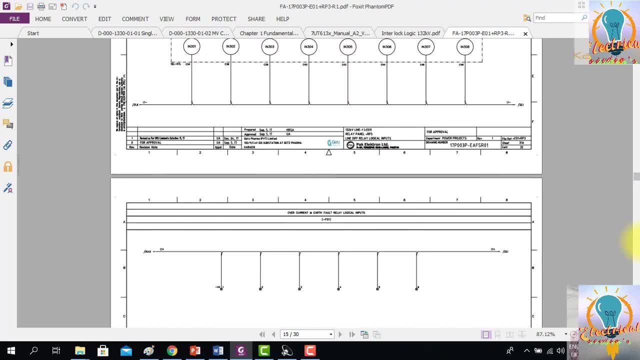 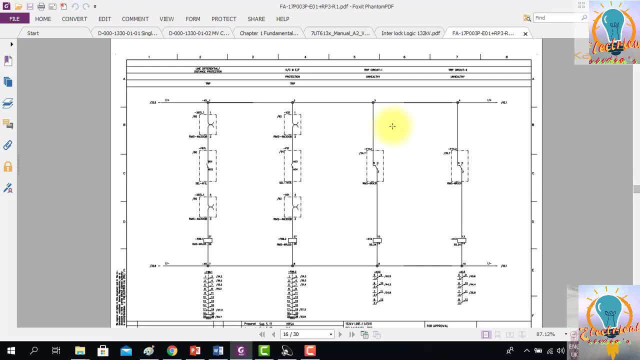 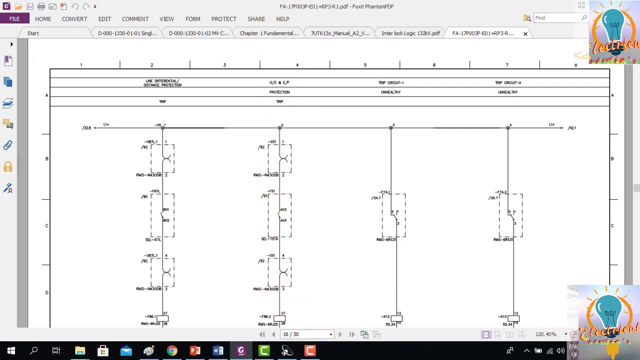 status, PLC status. then here you can see there are. these are the lockout relays. lockout relays are basically protection for the over. current protection is not issuing trip directly to the tripping coil but it's issuing trip to 86 lockout relay. and 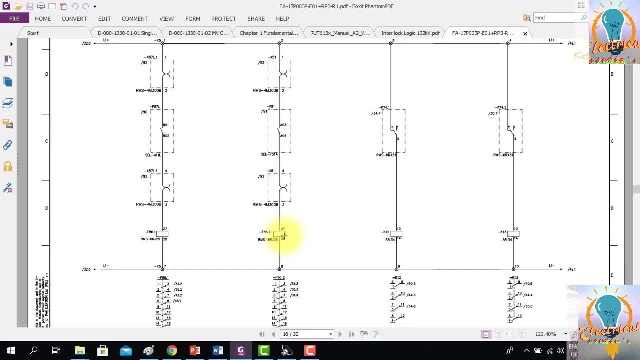 then lockout relay, further giving trip command to the LCC. this is basically to protect the relay contact itself. so in this case, if, for example, if the relay has low burden contact or if you want to save the relay contact itself, because it's difficult to, if the relay contact get damaged, it's difficult to replace a. 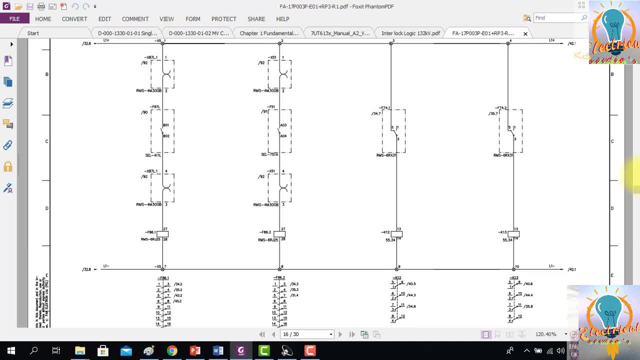 relay contact, but if you are initiating another relay through this relay contact and then this relay is taking all the burden. if this relay is damaged, then you can you can have a sphere and you can easily replace this relay. so that's why the concept is to use another relay, and here they are using. 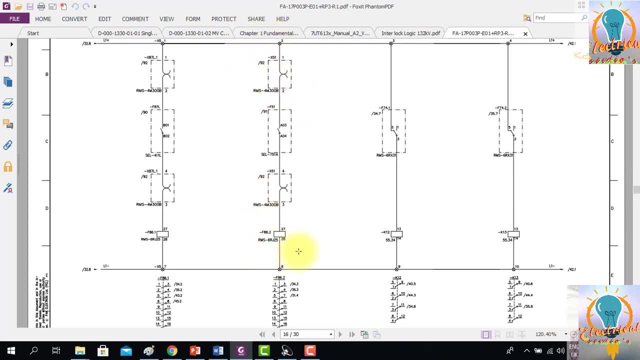 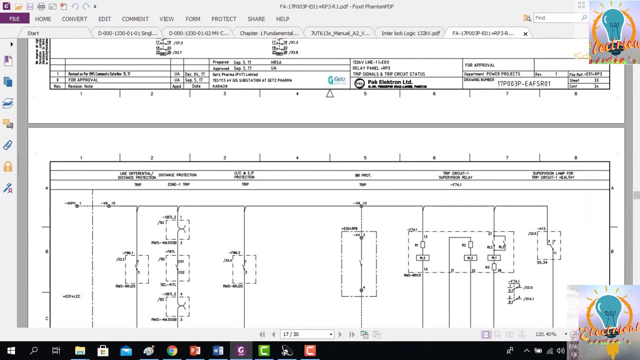 also lockout relay 86. so if this relay operate, the lockout relay has a feature that it will not allow circuit breaker to close unless this relay is reset. so this is a function of lockout relay in protection systems. here you can see trip coil one and here you can see they have installed a trip circuit supervision. 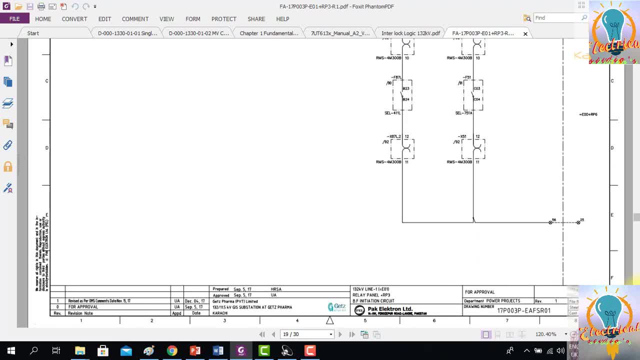 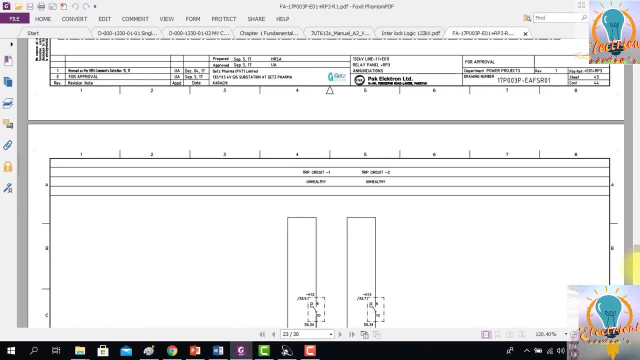 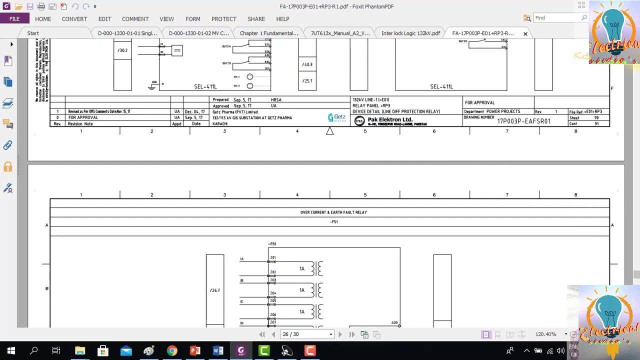 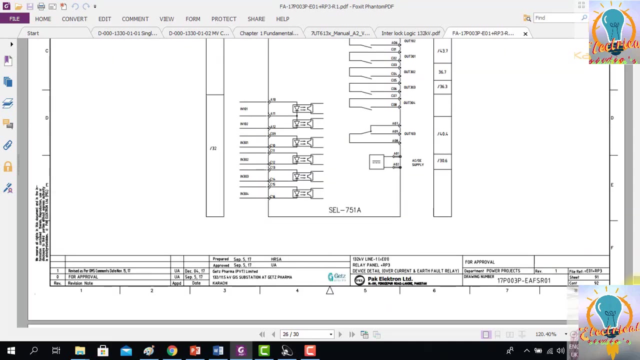 relay. so this is how this trying is looked like. then they have connection to SCADA alarms, to alarm panel, SCADA panel, and at the end they are showing the drawings of, first of all of all, the mean release. like this is acl line production relay backup over modal relay. and then they are showing the 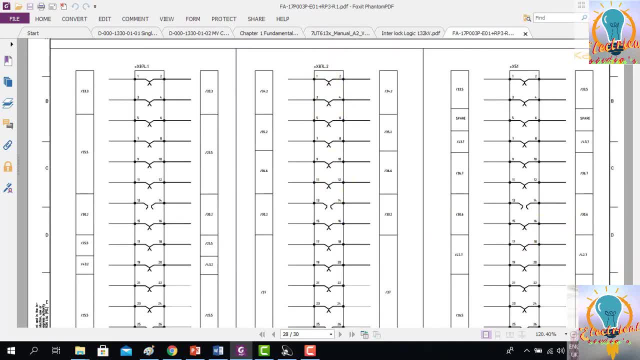 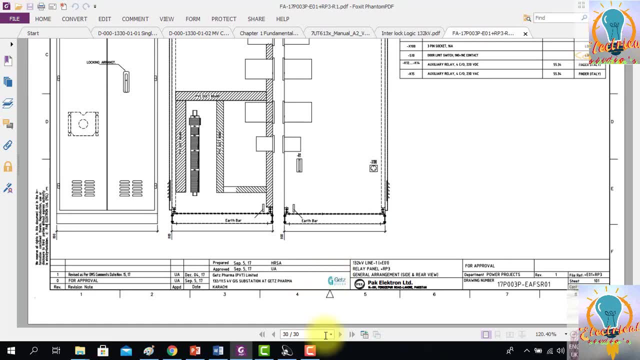 detail about auxiliary relays. after that. this is basically test plug. they have shown and they are at the end. they have shown the layout. so this is how. this is how the protection secondary turn looks like. so I hope you enjoy this portion. hello friends. previously we have 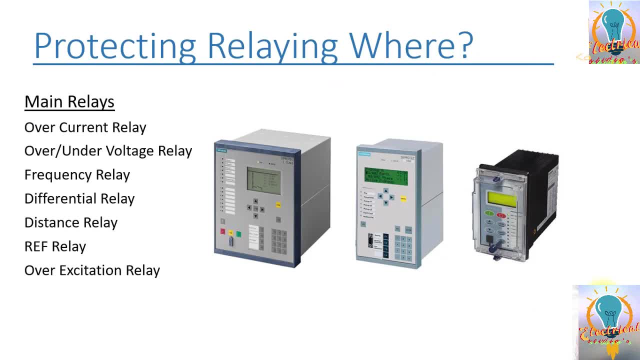 discussed a little bit about the auxiliary is now we will discuss about the main relays. so main relays, basically all the CT and VT inputs, current transformer and voltage transfer inputs are normally connected to these main relays and these main relays are basically the main devices which are 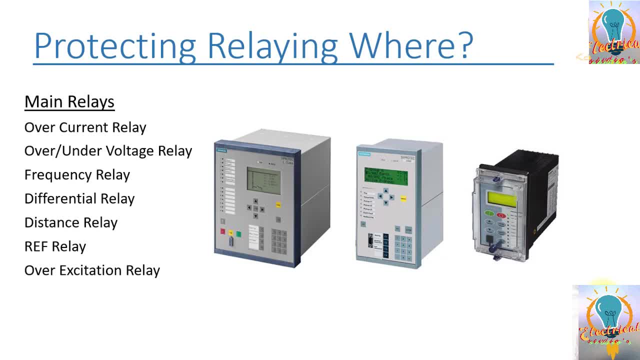 monitoring different voltage and current and impedance parameters of the substation or the power plants, and they are also called as a brain of substation or a power system. and what we are doing? we are putting the settings in this relays and they are continuously comparing the set value with measured 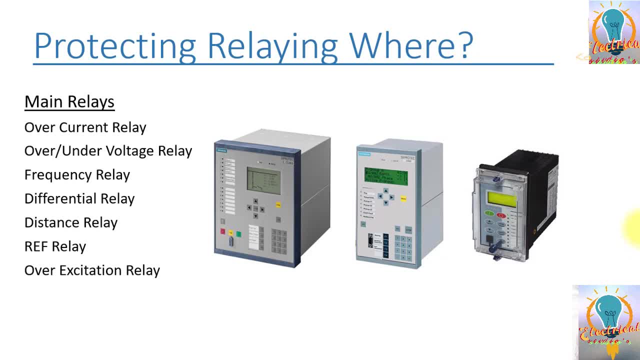 value and they are making all the decisions. and if it's necessary to trip the breaker, and they are also making the decision. so here you can see. this portion of the relay is called as HMI, so here you can scroll and you can see different alarms, events settings in the relay. also, if you want, 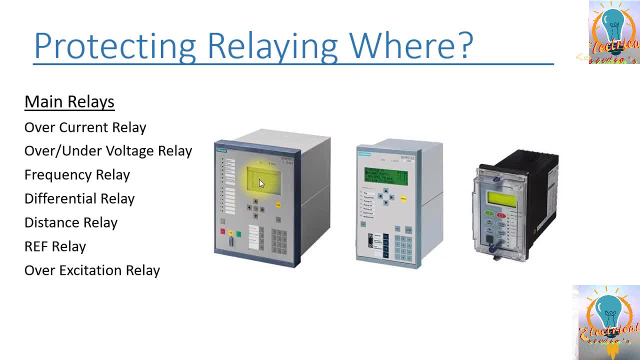 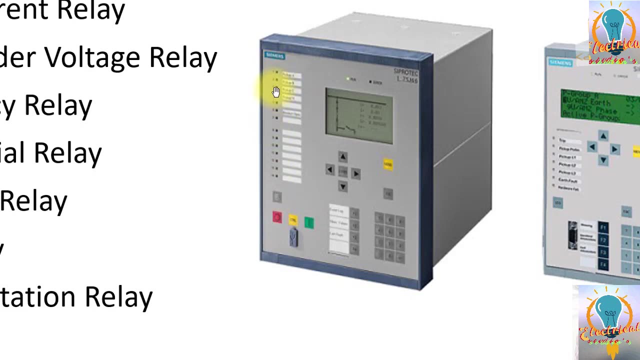 to change the settings. you can change it. you and this work. these are normally protected by the password, so all these things can be done from the front. this area- basically what we are doing here- is that the data set is being stored in the- is basically these are LED. these are the LEDs so if some event happened for 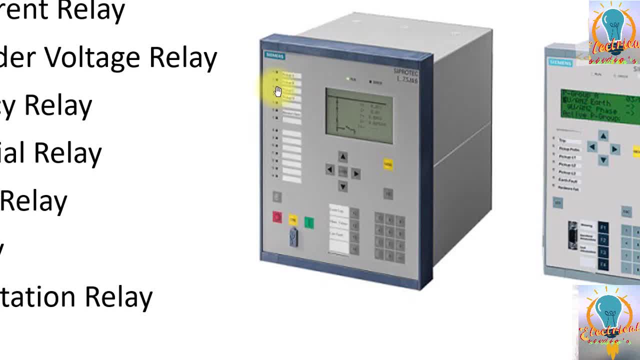 example, red face, pick up yellow face, pick up blue face. wake up, this LED will be glow and if you program is as a latch, it will be latched, it will remain and operator: after the fault, he can come and he can check which fault has which loop. 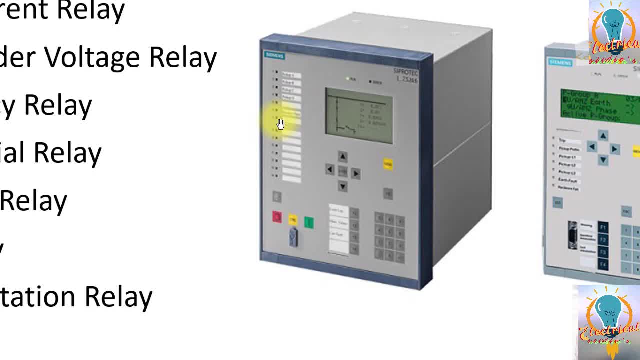 has a fault and what type of fault is it? and he can gather all the information from from the relay itself, from the front, and here you can see, this is the keypad where you can enter the values and you can scroll through this, this menu, through these arrows. so there are different type of the release I have. I'm 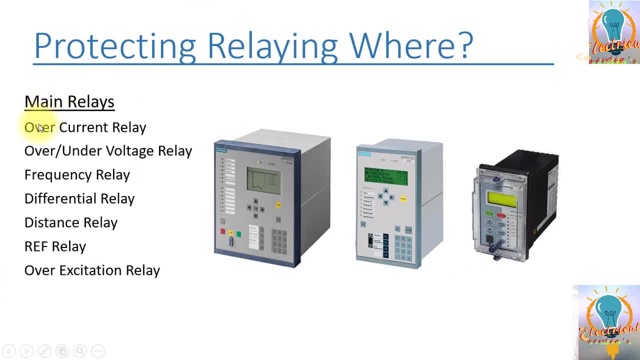 showing you: oh mean release, the release such as over control, a over voltage, under voltage, relay, frequency release, differential release, distance release, RF release or sedation release and accept and any other release. these are all example of main release. so nowadays you will see more and more microprocessor based release, as I've shown you here previously. 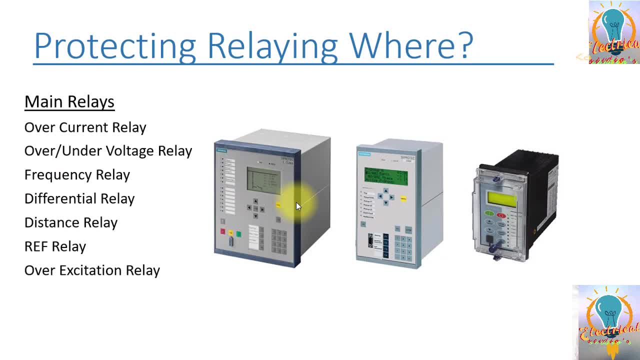 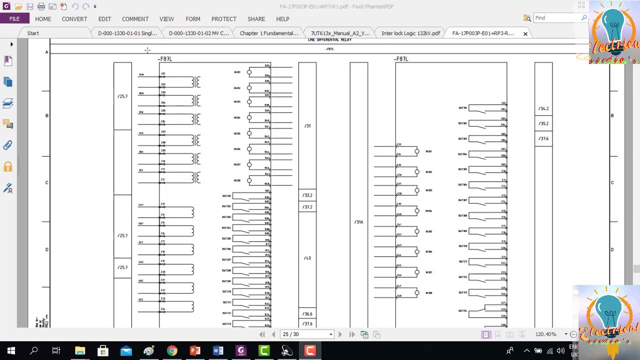 relates for electromagnetic mostly, but now you will see most, mostly the microprocessor based release. so I hope you enjoy this section. thank you very much, so here I will show you in the drawing. in this drawing they have this is our main production- differential production and distance direction. really F it is. 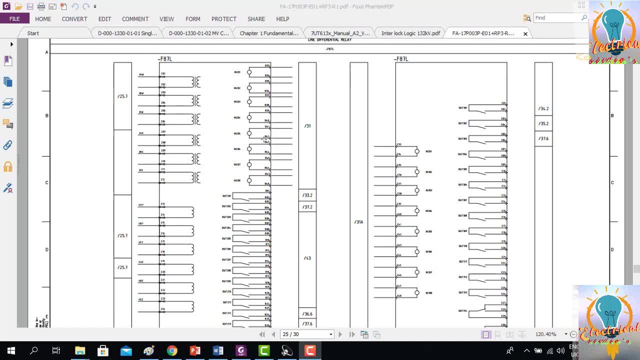 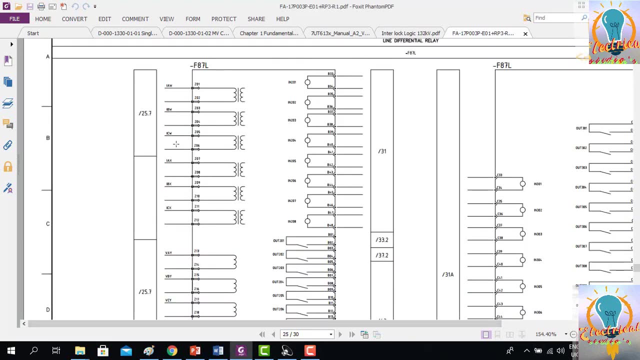 7, oh. so they have shown this relay at the end of the drawing and wherever the industry and the connections are shown, the action, the page number. for example, this is the CT circuit for the relay and shown by I aw, I BW and I C W. and if you 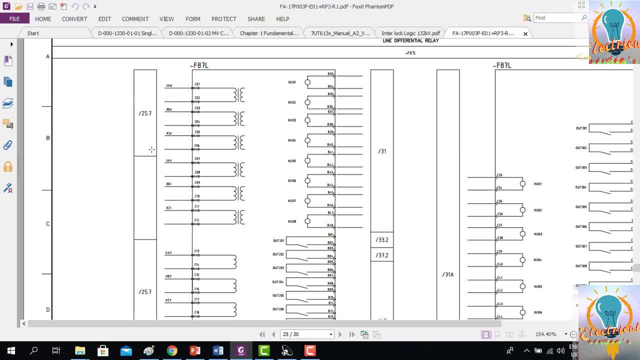 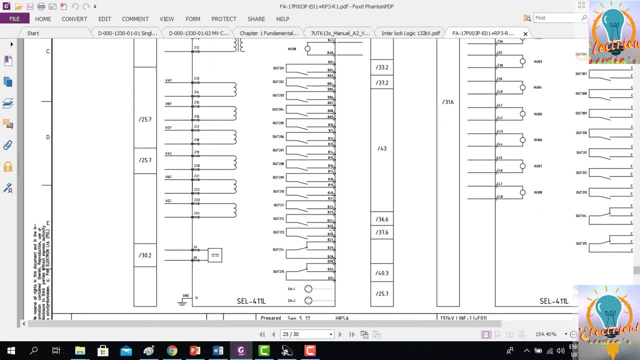 want to see where the series are to risk an connect it, you can go to sheet 25.7 and you can see the drawing of CT circuit. so this is how they have shown the CT circuit. I will show you later on. and if you want to see the VT circuit for this really VT is connected on these. 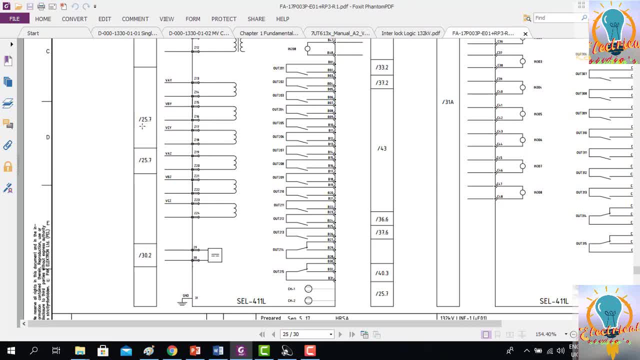 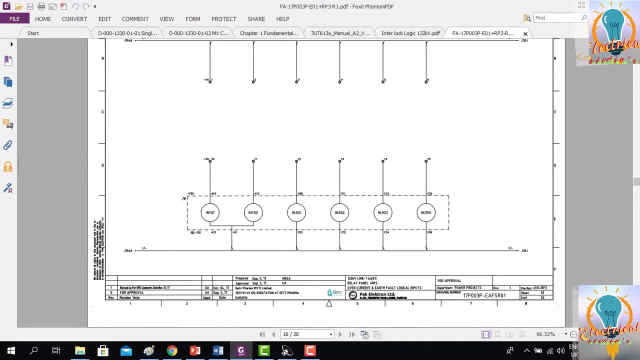 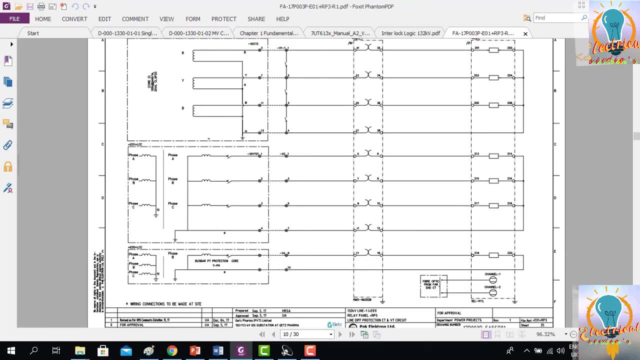 terminals of the relay and you can see from where it's coming at 25.7. so let's go to 25.7 to see CT and VT circuit. so this is basically the page which they refer. so here you can see, this is the CT. 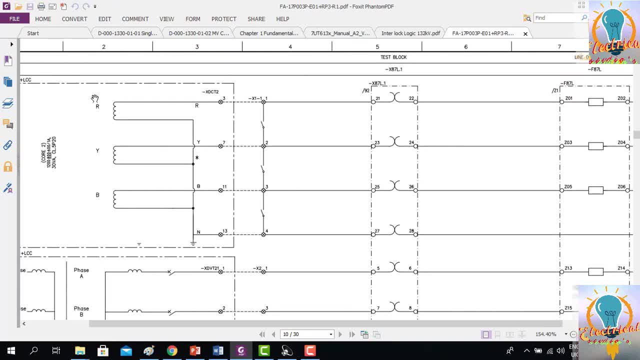 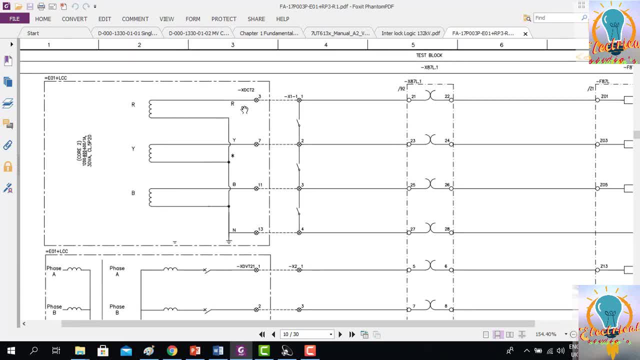 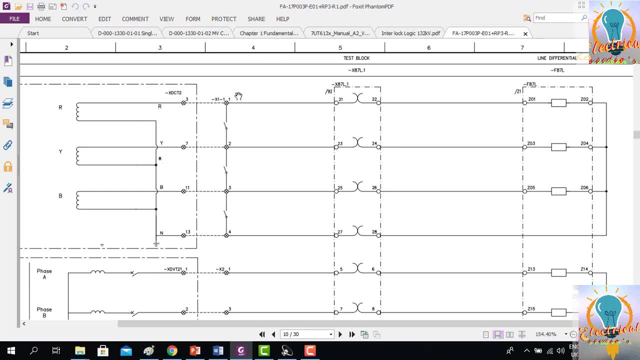 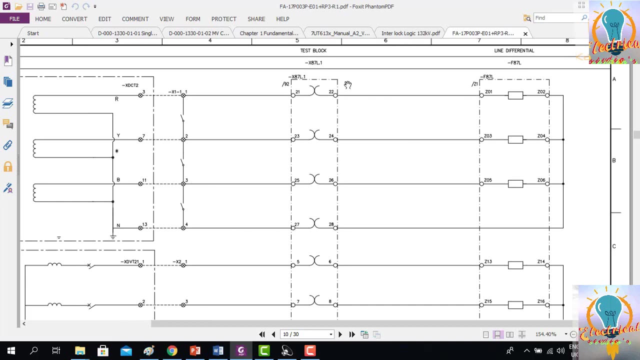 and through this- and this is a terminal blocks on the local control cubicle, then it's coming to the protection panel RP03R1 X1-1, terminal block one, two, three, four and then it's further coming to the test block. so, if you want to, 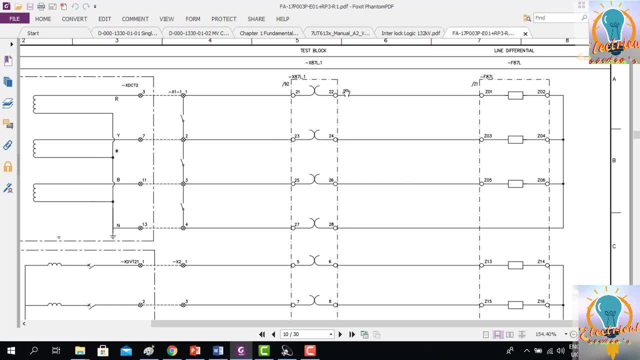 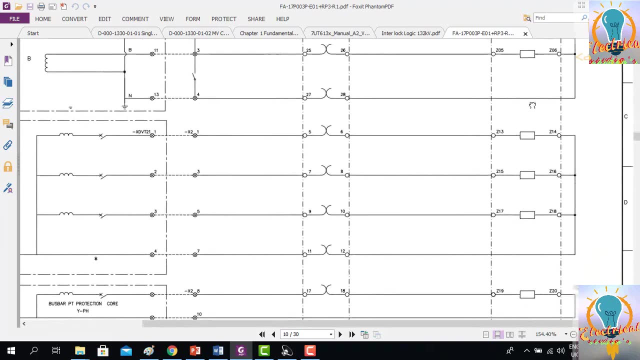 perform any testing. you can insert the plug and then you can inject current and voltages here. here you can see this old side is switchyard side and the even side is the relay side and you can see the CT is connected to the relay and this is the VT circuit. in the same way VT is connected, so you can in. 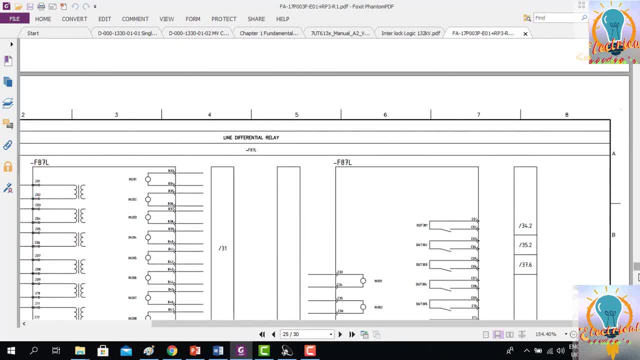 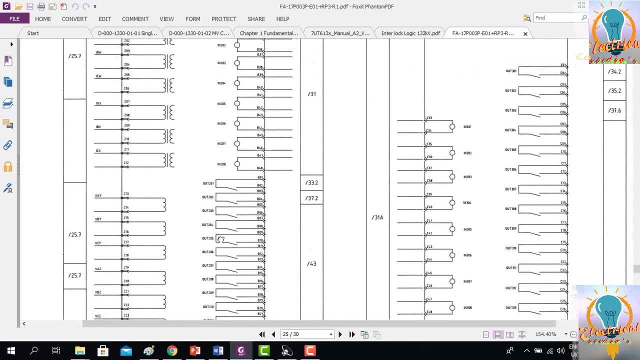 the same way you can find all the information of the relay. if you want to scroll and you can see further, you will see the power supply. this is the power supply is connected at 30.2. these are the binary inputs: IN201, 202, 203. these are all the inputs that are connected. 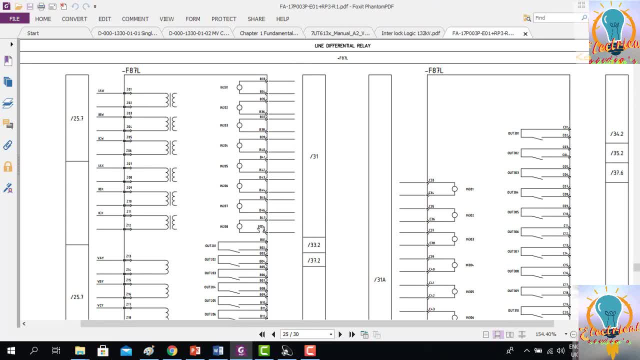 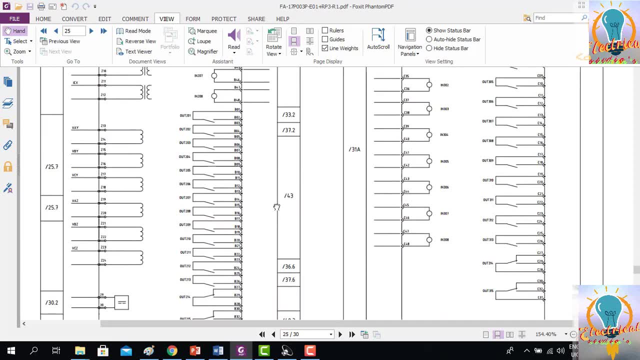 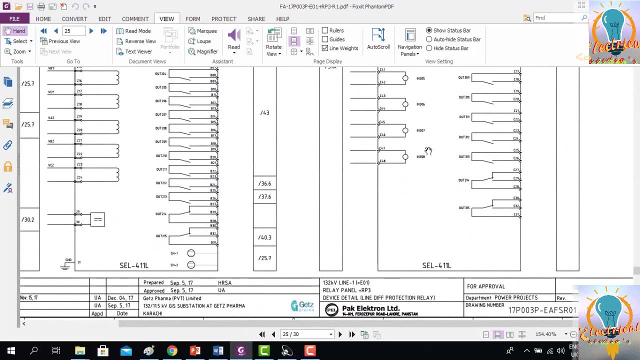 all the binary inputs you can see on the sheet number 31. these are the binary outputs, so if the relay sends a fault it can issue the trip alarms and it you can see these are used on different sheets. this is the communication channel because it's line differential relay. 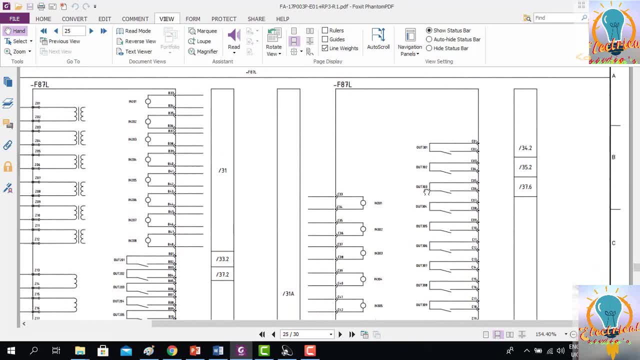 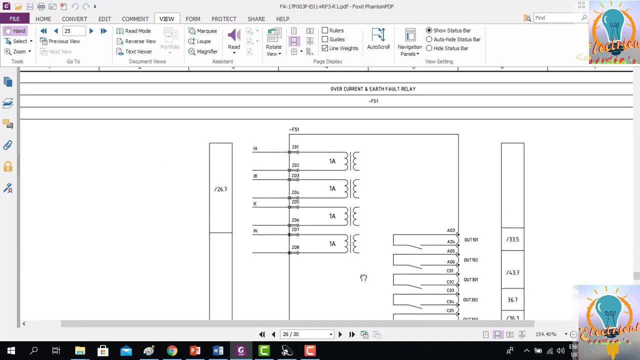 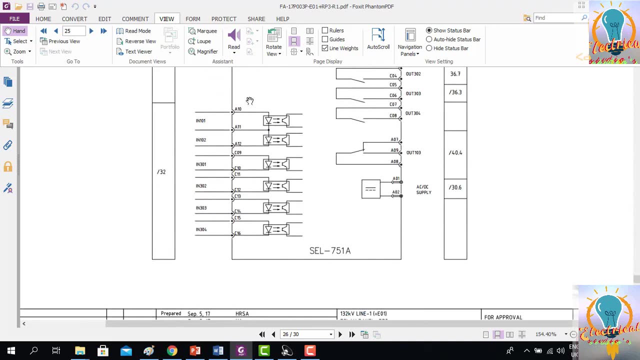 so it is communicating also to the remote end. so these are all our input outputs are shown here in the same way. all we will see another. this is the F 51. this is basically over control a. this is the current input, this is the voltage input and these are the binary inputs. this is the power supply. this 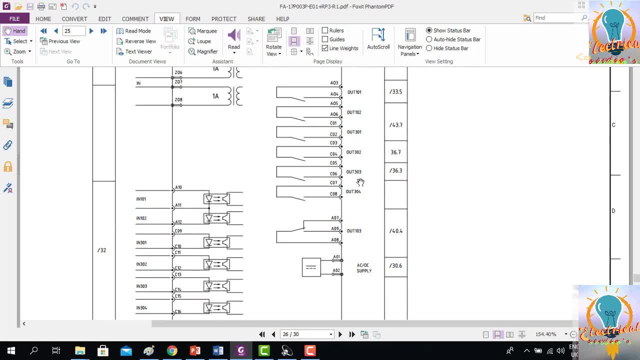 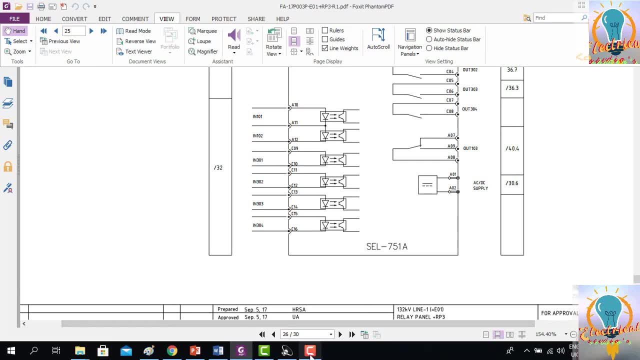 here you can see, this is the change over contact and this is the normal contact. so this is the difference between change over and normal contact. so this is how, then, these relays are shown in the drawing. thank you very much here, friends. let's start our new topic: the burden. the burden is: 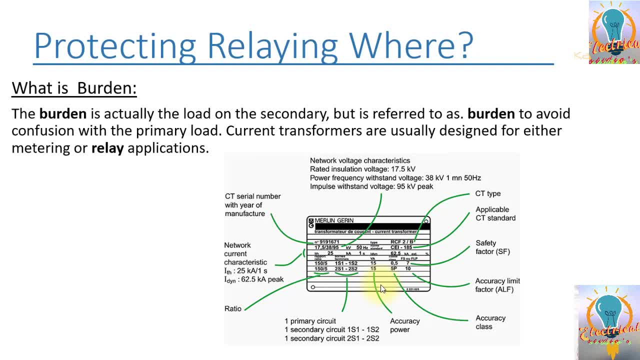 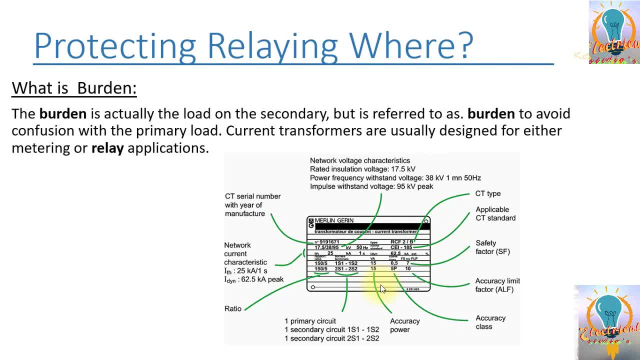 designed for either metering or relay applications. so basically, whatever on the CT secondary and vt secondary, there especially, we are using a trump burden. if, for example, if you, if you connect a relay to the CT secondary, so it means you are adding a burden to the relay secondary. 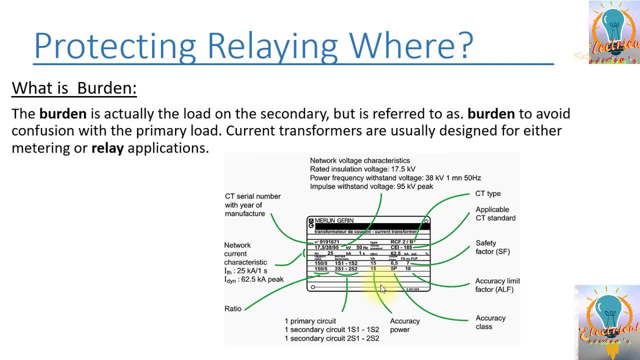 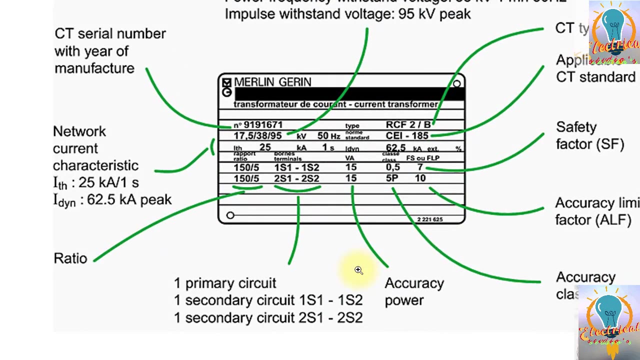 read all the CT and VTS. their rating is shown as VA. for example, CT VT can be shown as 20 VA or 30 VA. it's called as basically the burden rated burden for the CT, if you you connect more, if you connect more load or if you connect more. 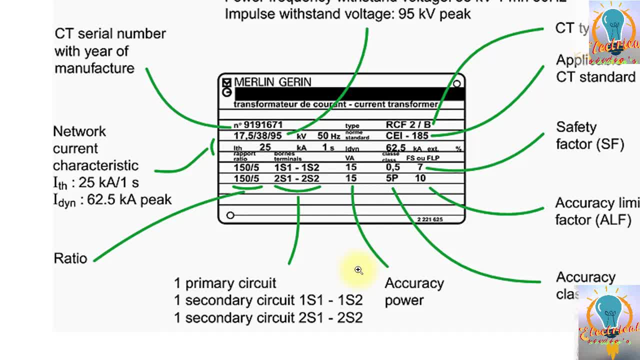 burden, then the rated one, it and then the accuracy of the CT will be compromised. so here you can see, this is an input of a CT and you can see, and this is the rated VA. so, if this can, this CT has basically two different course. so this one as one as is showing secondary, and one is showing that this is the core. 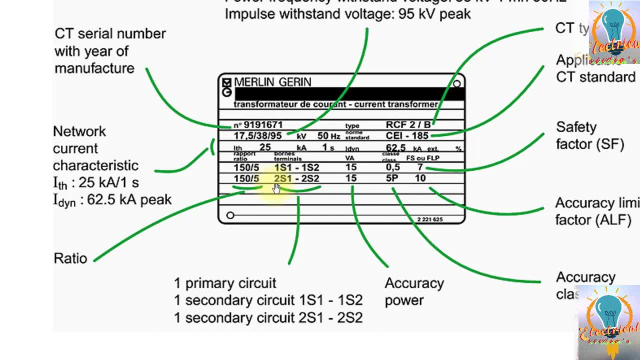 one and two is showing it is a core two and one is showing that this is the core one and two is showing it is a core two. and this is the secondary side terminal. one and two. so this CT has a two core. primary is rated at 150. if 150 ampere is there, the secondary will have a 5 ampere. 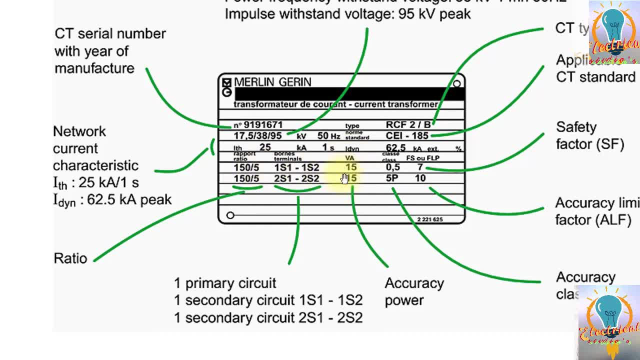 at the secondary side. so the rating of this both course is 15, 15, VA and class. here you can see the accuracy class is 0.5 and it mean this type of CT has an error of 0.5 percent. and here you can see this accuracy class for this protection class for this CT is: 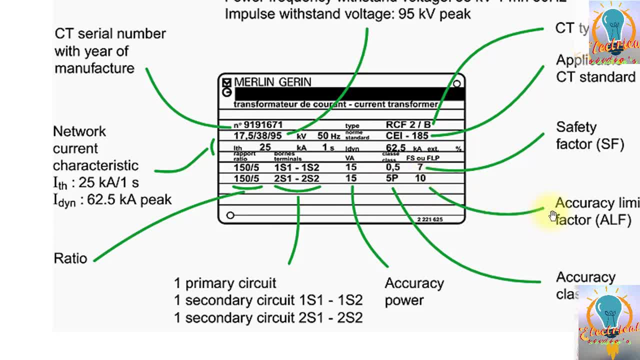 5 P 10. so here 10 is basically accuracy limit factor and 5 P is basically the accuracy class. it's mean that if this CT I have 5%- could have 5% error if the current is 10 times the rated current. so rated current is 150. so if 1500 ampere, 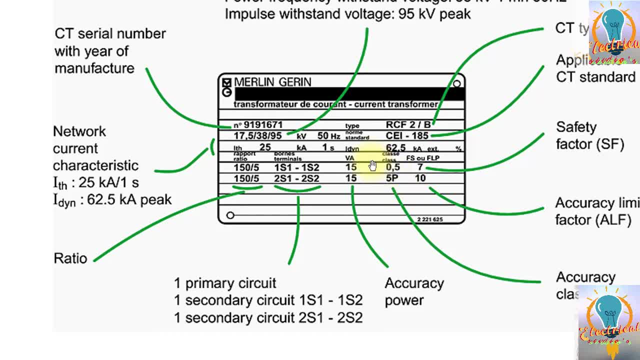 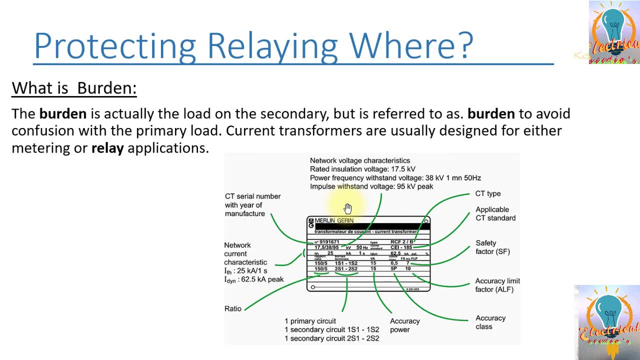 is flowing through this CT, then the current is 10 times the rated current. so rated current is 150. so if 1500 ampere is flowing through this CT, the ratio of the error could be 5%. so we are basically measuring the rating of the CT with VA and all the basically relays they have mentioned. 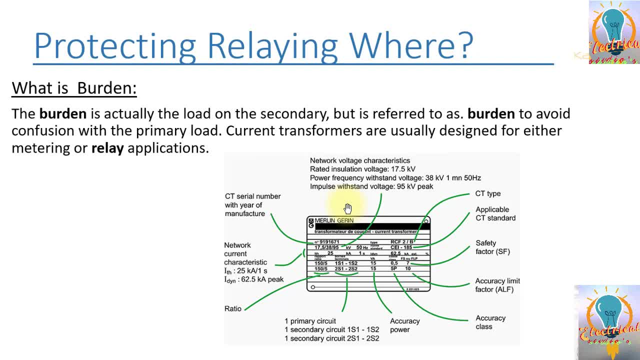 that what is the burden of the relay itself? so previously I've shown you if you use a relay at 1 ampere and 5 ampere, the burden increase at 5 ampere then then a 1 ampere relay. so this from burden especially used with CT and VT in the power system production. so I 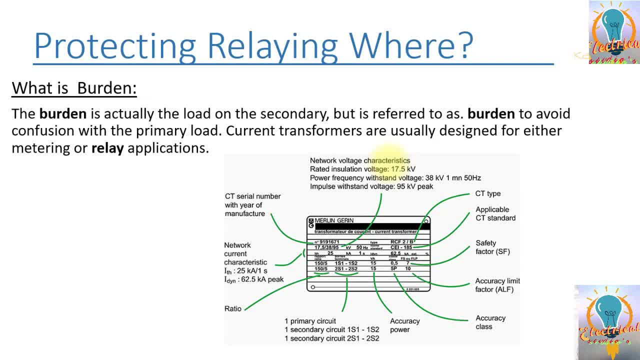 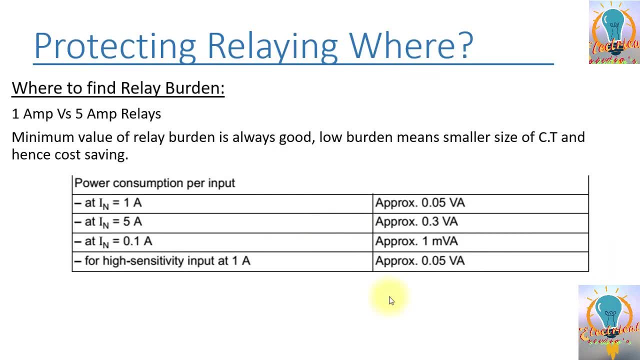 hope you enjoy this small topic. so we'll move to the next topic. thank you very much, hi guys. whenever manufacturers is supplying any relay and then it's also supplying that, what is the burden of the relay? you can also measure the burden of the relay by applying the rated voltage, and then you can use a clamp on to. 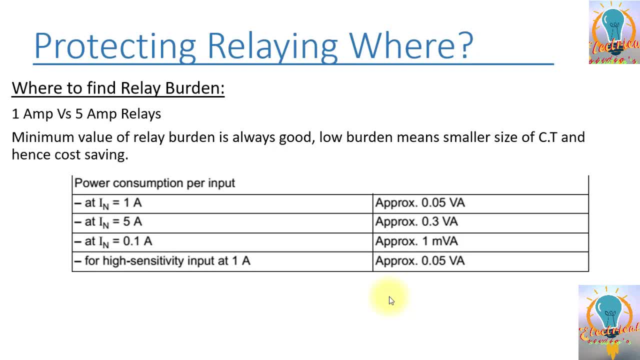 measure the current. for example, if it's a basically a CT circuit, then you have to apply the rated 1 ampere and then you can measure the voltage across this relay. then you will be able to measure the VA burden of the relay. so here you can see. I have shown you. you can find the VA burden of the relay in the relay. 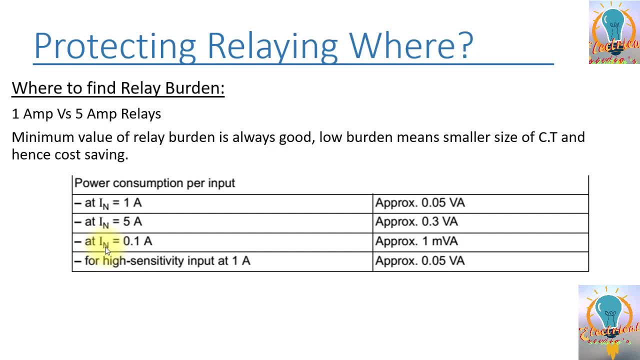 manual which is provided with the relay itself. so in this manual I have shown you that there is a relay which is 1 ampere or you can also choose it to to be connected at 1 and 5, normally on the, if you remove the cover, there is a basically jumper is. 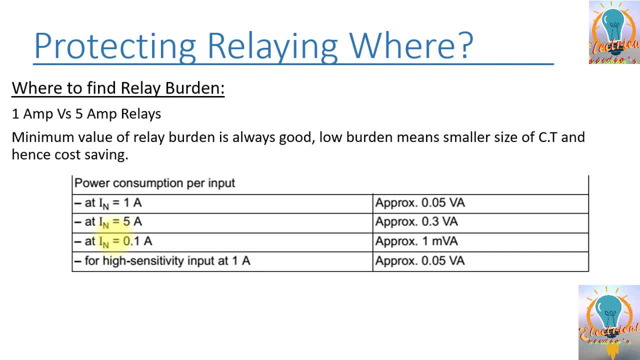 provided, and if you change the setting of the jumper, you can convert the rate from 1 to 5. but the remarkable difference you can see here is that if you change the relay from 1 to 5, the V rating, the burden, is also increased. so 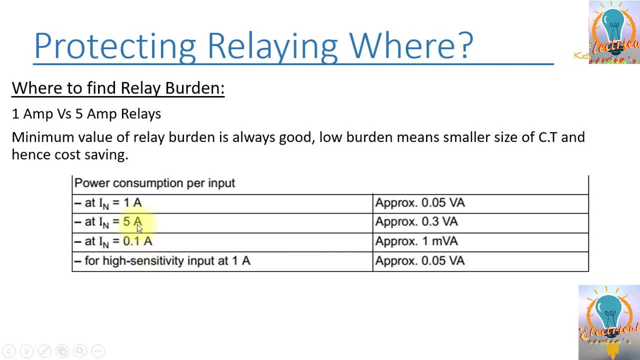 in. previously the practice was to use 5 ampere relays, but in future, in order to reduce basically the burden- mostly now everywhere you will find mostly the one ampere relays- because if you use a 5 ampere relay so we might save some cost, or 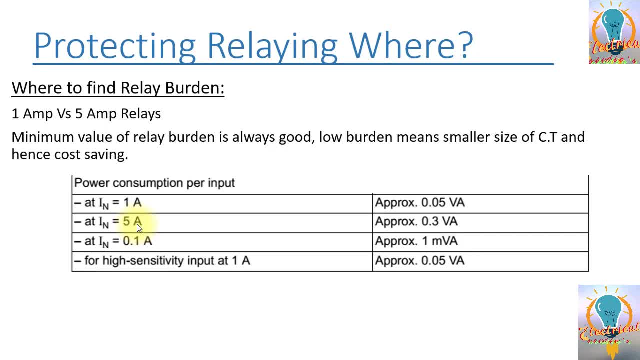 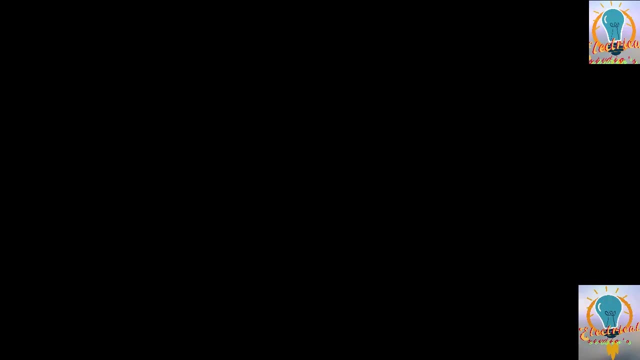 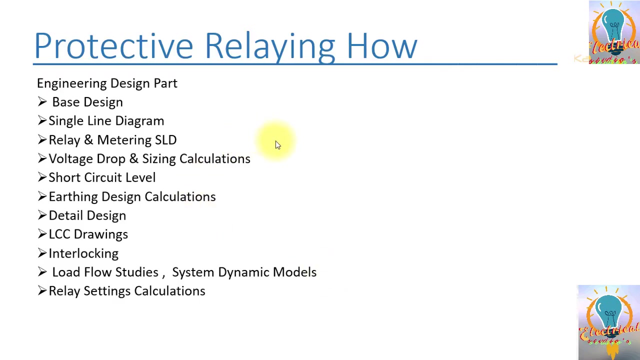 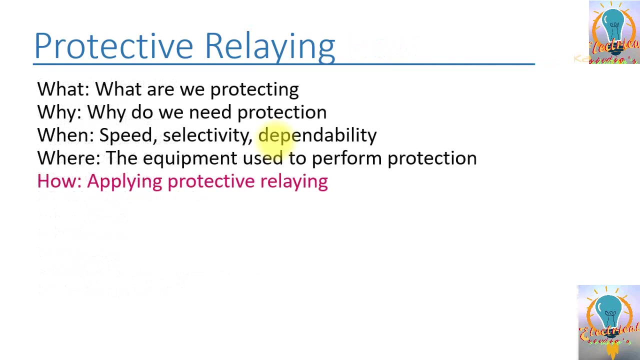 if you, but the burden will increase, and then you need to increase the size of CT. so that's why it's always you need to check each and everything before designing the system. thank you very much. you hello, friends. in this section we will move to the next topic, and that is how. 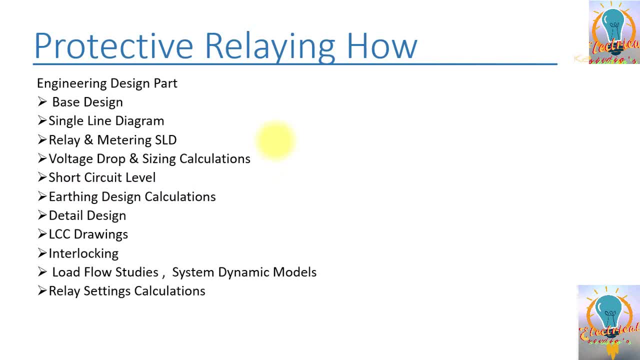 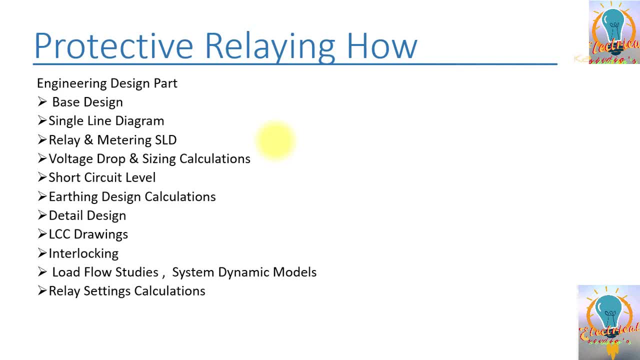 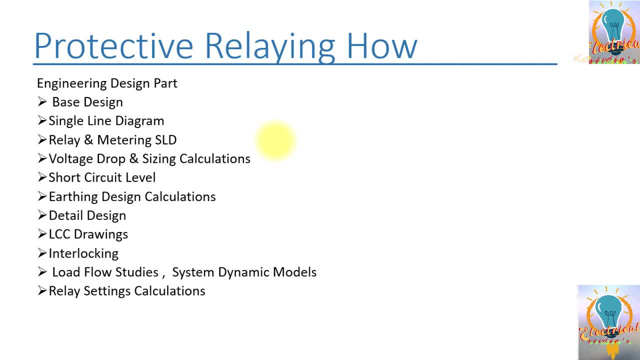 one-and-a-half breaker scheme. all these things are finalized in the base design stage and then single line diagram is prepared and single line diagram is showing all the high-level information, how many seats and VTS are used. after we are finalizing the single line diagram, 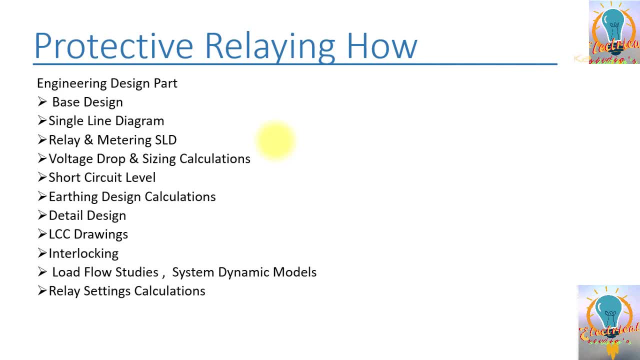 rain meeting SLDs are prepared and rain meeting SLDs are showing which protection will be used and how many GT codes will be used. what is the specification of CT codes? and all this information is finalized further in this design stage is the first phase of. 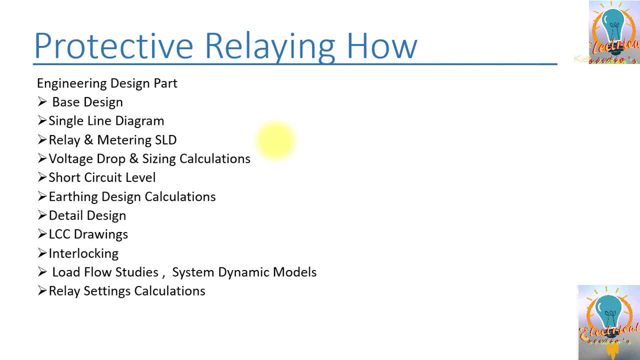 design stage, voltage and drop and sizing calculations are done for the CT and for this AC and DC circuit. city sizing and sufficiency calculations are also done in this stage to check how what is basically the size of city required, adequate for carry the burden of relays and also the cables length in the burden. 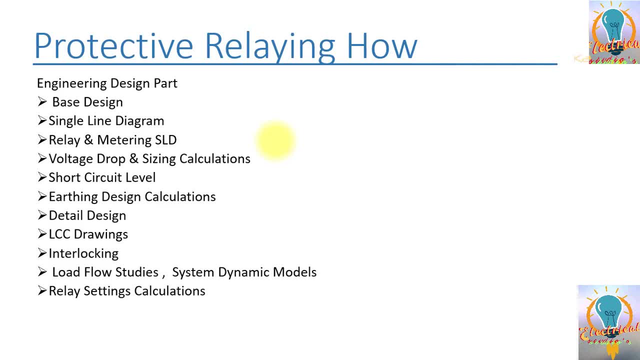 on the city depends on the length of the cable. the cross-section of the cable and the burden of the then short circuit level is also confirmed and this is very important also. so short circuit levels you are. it is a main input for designing the mesh, earth mesh and also for pick during the high voltage equipment. each. 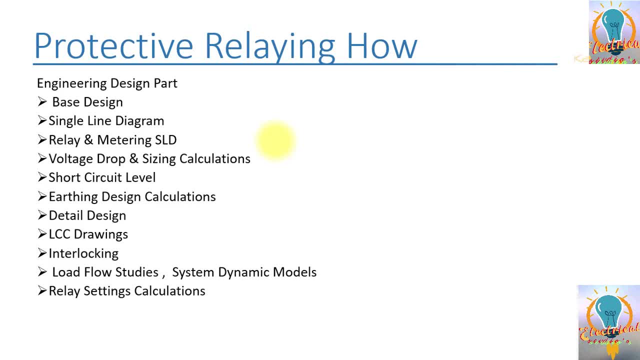 equipment is rated for certain short circuit for a given time. then you have, I think, design calculations. you have to do design the earth and we will calculate all permissible values, like allowable touch and step potential, allowable voltage rise. so each thing should be under control. after doing all these things, we are proceeding to the digital. 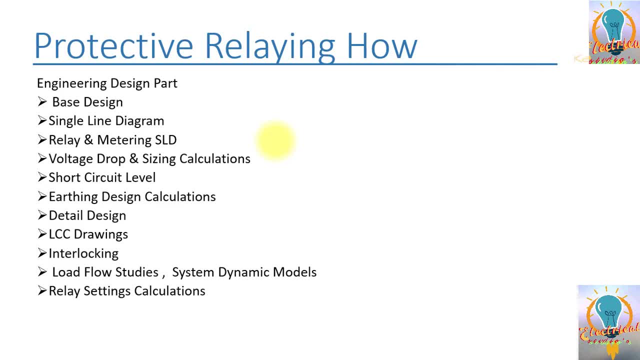 design stage in which we are preparing the detailed design of different production and control systems. so after detailed design is completed, then it's such a time to go manufacturing, go ahead. so then, similarly, LCC drawings are finalized, which are local control cubicle drawings, interlocking are. 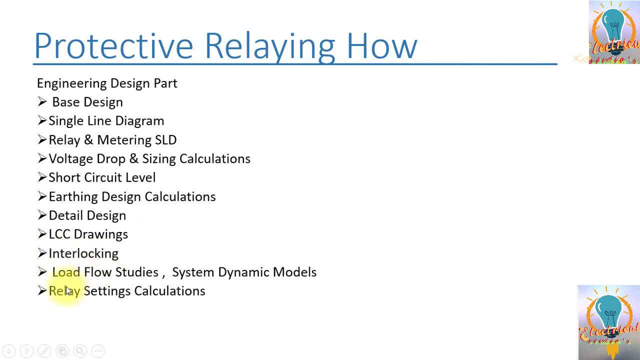 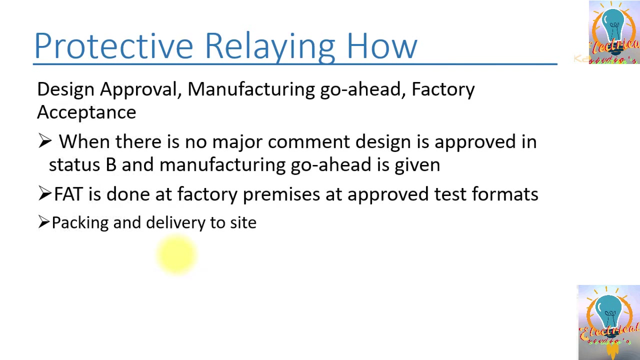 also finalized and reviewed in this stage. if you are doing the planning of adding a new power plant, then you will have to do the load flow studies, you have to simulate the dynamic models. so these all things are done at the engineering part of you. similarly, relay: all these things are also prepared. they are based on provided data. so after 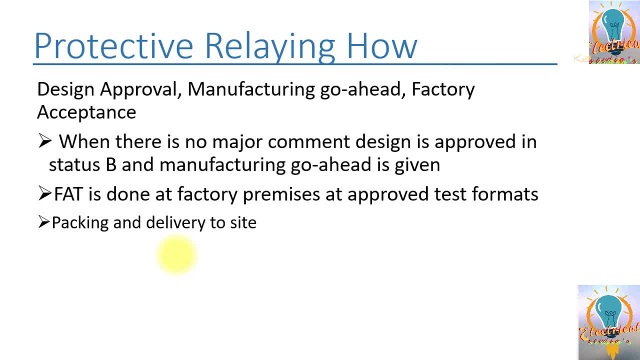 design approval manufacturing go ahead is given and when manufacturing go ahead given, manufacturer start preparing the equipments protection panels and GIS. and when the GIS is ready, FAT factory acceptance test is done at factory premises at approved test farmers normally. the third possibility is to use a third-party inspector or you can also client. 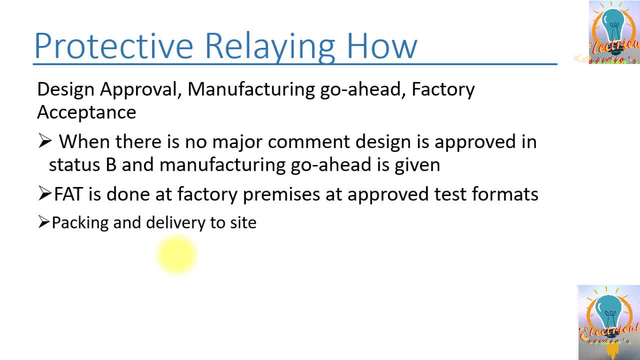 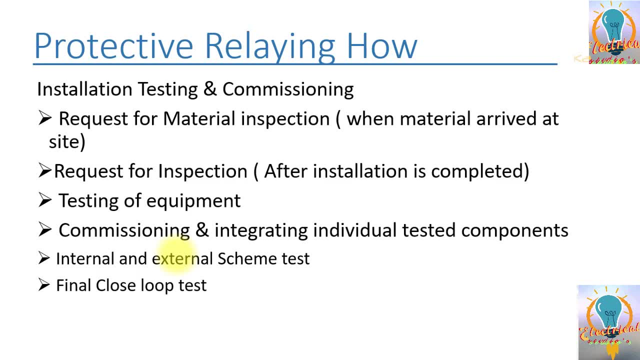 sometimes also want to visit so you can visit himself and we have a packing list and delivery to the site. when the equipment is delivered at site, normally process starts a request for material inspection. as soon as the material arrived at site, RMI is issued and the material inspected. it should be not. 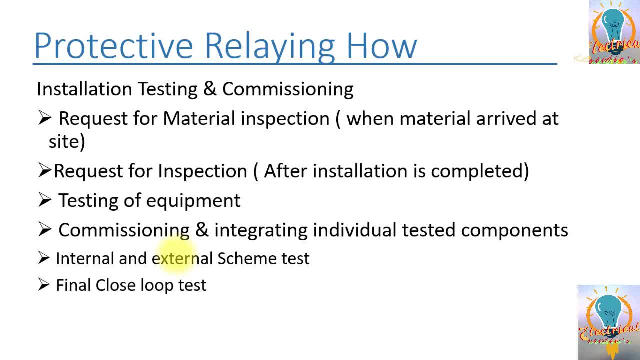 defective during transportation. it should be as per the drawings bill. of quantities is also checked after material is inspected and the next phase is to do the installation. for this, one request for inspection is done. in this inspection the stall equipment is checked and if there is any comment is. 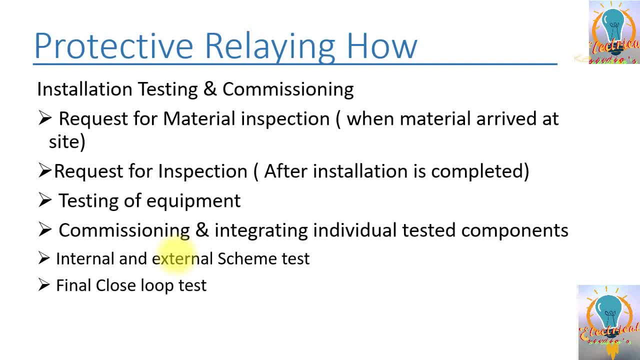 passed on and it is corrected. after installation is finished, the next phase should start the equipment testing. usually each equipment like CT PT generator motor are tested individually and the results are recorded. when the equipment testing is finished, then next for process to start the commissioning and integrating individual components, components together, so this: 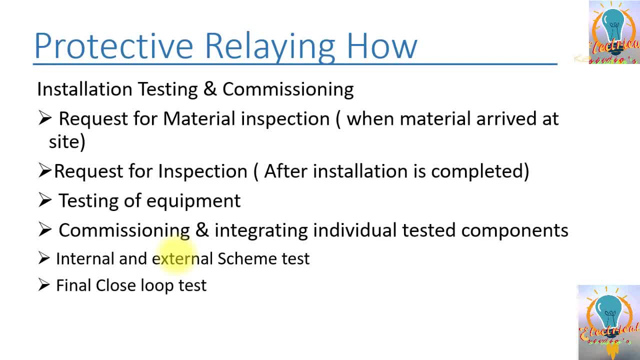 process when is complete, then the final process is basically checking all signals, trippings, command operations of the complete system internally and with externally to other panels. finally, the closed loop is done, in which all the alarms and signals are tested from first of all locally at local substation which 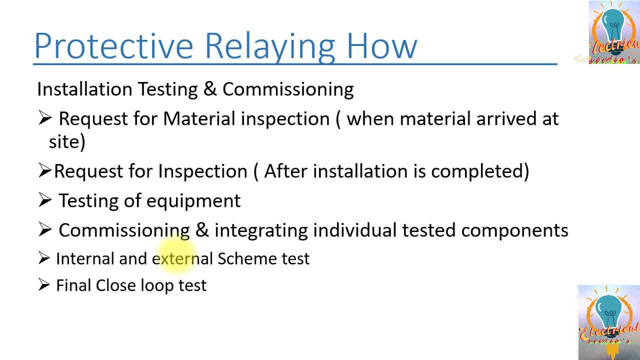 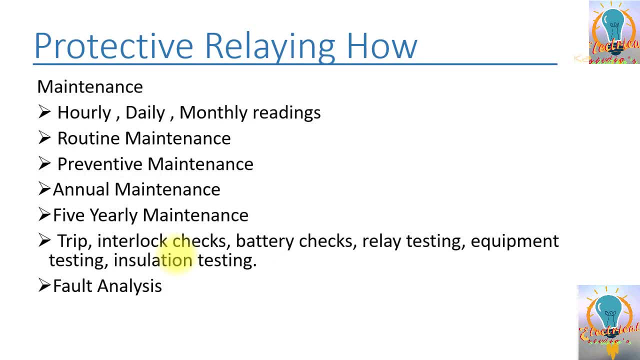 is called as local closed loop, and from next from the remote substation, remote control center, which is called as remote closed loop. so when system is commissioned successfully, after that it comes the part of being the maintenance. so maintenance first of all. in doing operation and maintenance, the one part is to 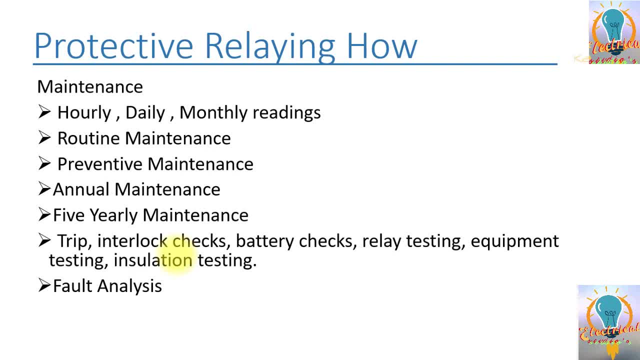 take the hourly, daily, monthly readings as per the decided frequencies, to do the routine maintenance, to do the preventive maintenance, to do the annual maintenance. also, there are some tests which are committed by manufacturer to do it in five yearly basis during maintenance. we are checking chip, we are checking. 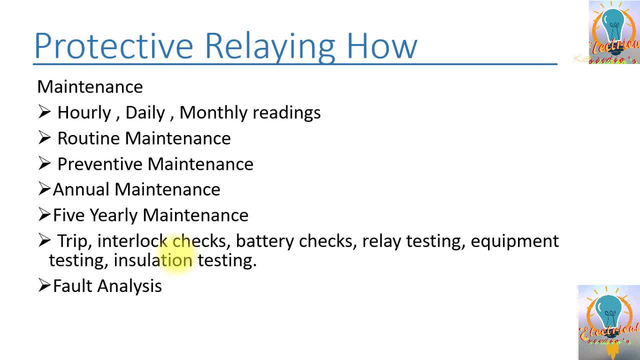 interlocks, we are checking batteries, relay testing, equipment testing, installation testings. all I have performed. now we have ready to go out and basically pull off the during an animal maintenance testing, then we have. if there are faults- we should have any fault- then these faults are analyzed and finally, root cause: 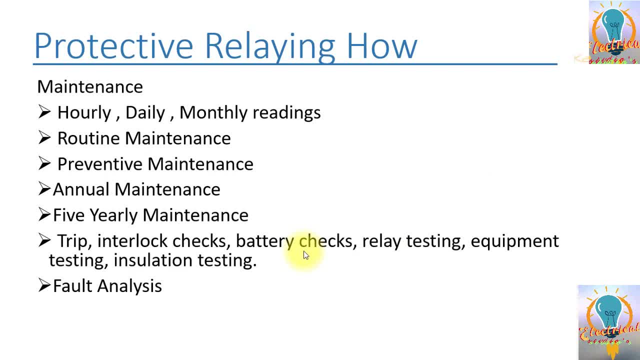 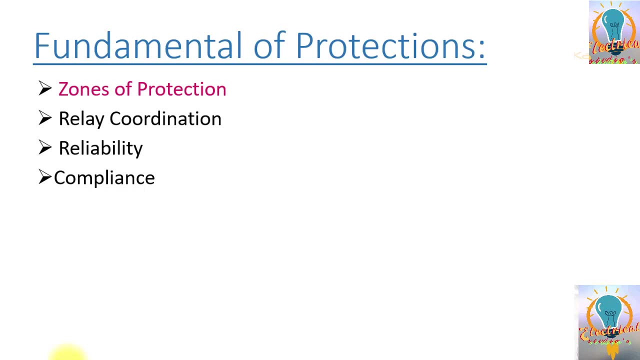 analysis report is issued. so this is basically the process by which we are continuing the protection system from start, and thank you very much. hey, friends. now start our new topic. that is about zones of protection. in previously we have studied that zones of protections to make zones of protection. 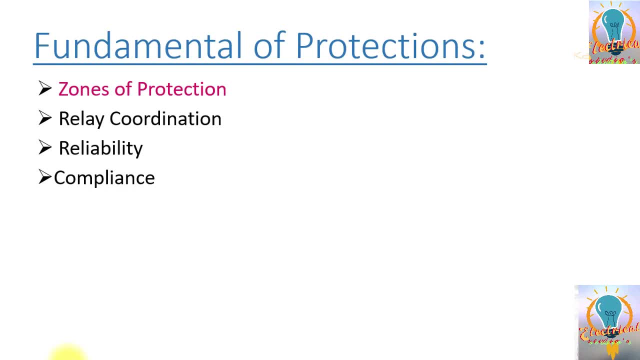 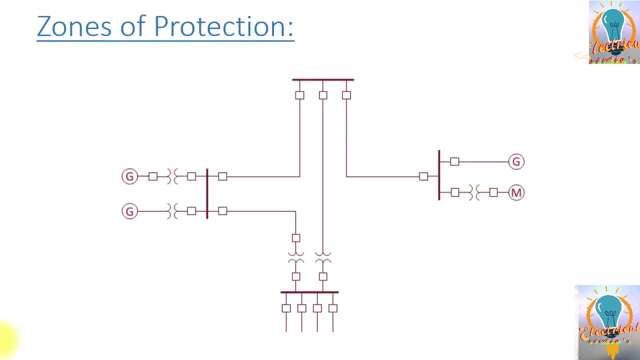 is very important in power system protection. this will help to localize the fault and only that portion of the protection system will be out which is basically feeding the fault. so this is basically the concept. so here you can see we have a protection system. just consider the case where we have two generators which are feeding the 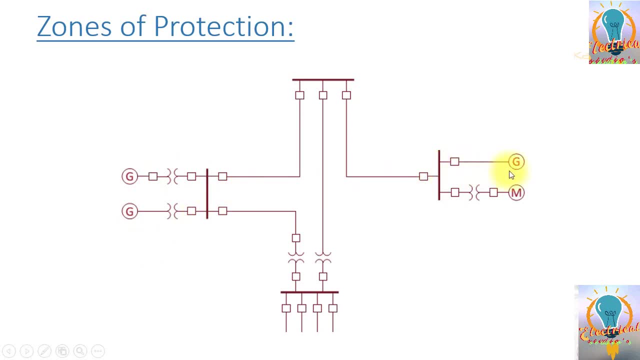 protection system. on here you can see, on the left side and the right side we have one more generator, we have one motor and we have one substation which is working as to make a ring. then we have another substation where we have four outgoing feeders and two incoming feeders. so here I have to start to make. 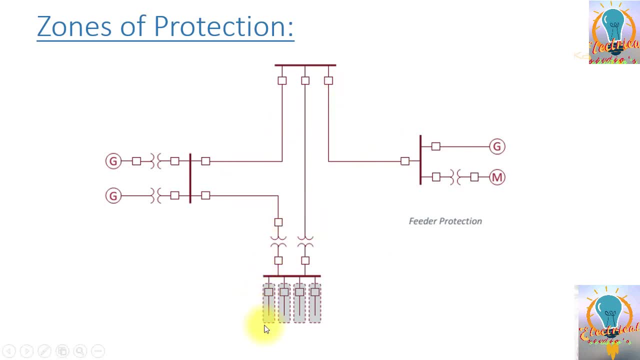 zoning. so first of all I will start to make the zones on individual feeder itself. so I started with four feeder protection zones. so if any fault occur, and only this feeder should trip. if the fault is on the feed itself, this square rectangle is actually showing a circuit breaker. this is a symbol of transformer. this dark line is: 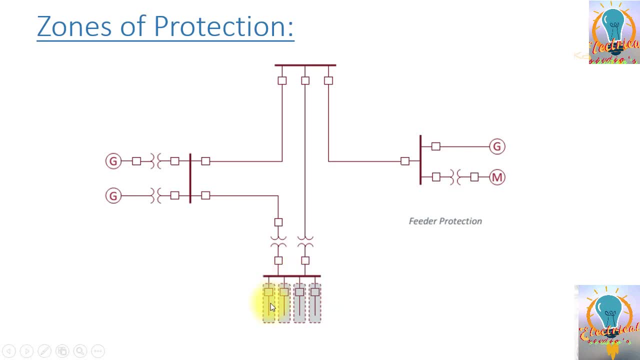 symbol of a bus bar and this is line is showing a feeder, basically. so i in the stage one, i have prepared the zones for feeders. stage two: uh, we can mark also here: uh, zooms. i have make a separate zone on the motor and i have included the breaker. it means if there is a fault on the motor then the breaker. 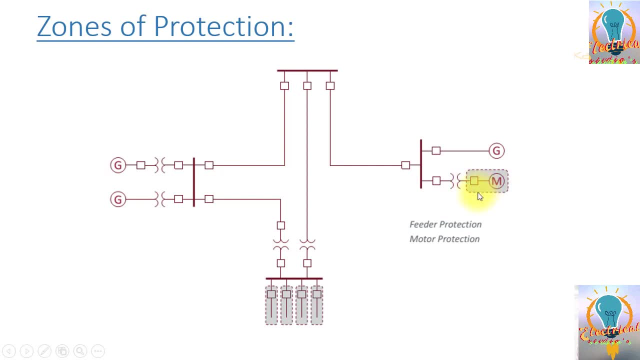 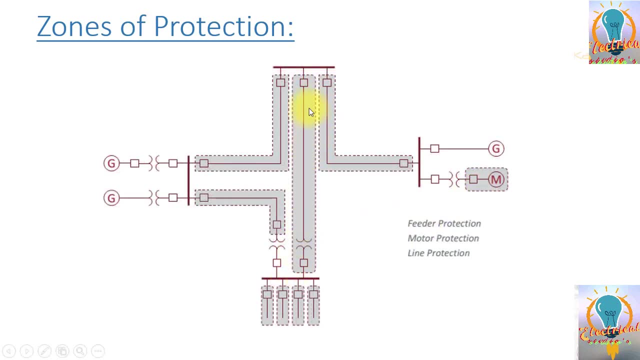 uh will trip and it can isolate the fault. so let's now start making another zones. okay, now i have made a little further zones. so this is the zone one between this and this breaker. this is another zone. this is another zone. this is another zone. so these are. you can see this, could. 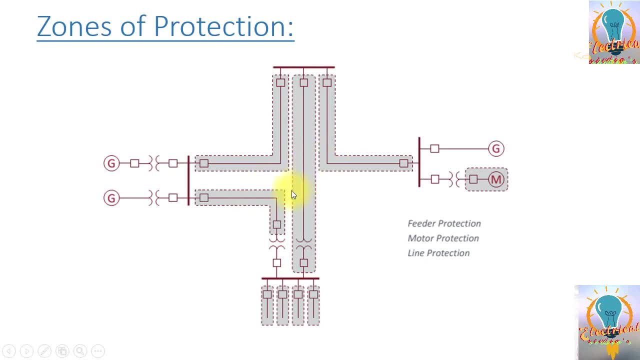 be regarded as basically the transmission line protection. so we consider them as a transmission line. so each line i have make a separate protection zone. so here you can see- uh, one difference here you can see: this transmission line has a breaker at one end and the other end is directly connected to 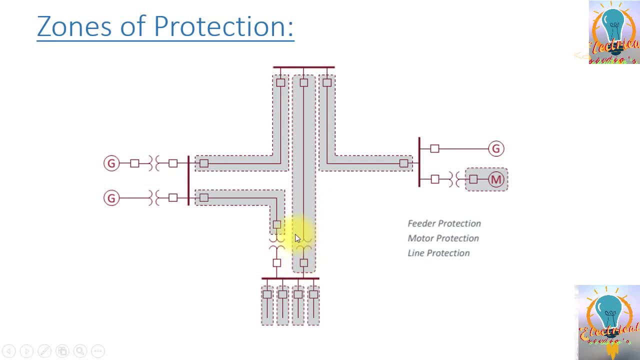 the transformer. so i have- you cannot isolate, uh, this part of if there is a fault. you cannot isolate the line itself, because it is connected directly to the transformer, so i have to include the transformer and the breaker. so if there is a fault, in order to isolate, i also have to isolate. 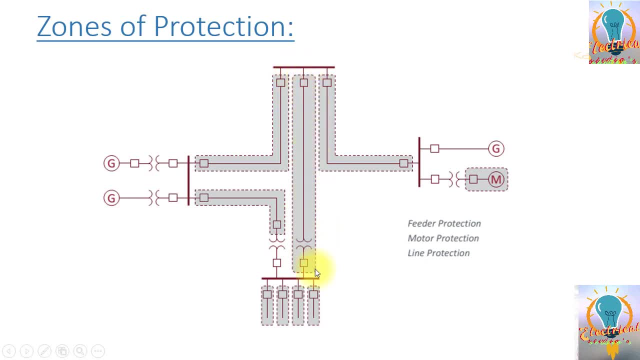 transformer itself. so i have included this transformer and breaker in this zone. in this case, you can see i have two breakers: one is before transformer, one is after transformer. so i have make a zone where i have included the breaker before transformer and the line breaker. so if there is any fault, i will prefer to trip and isolate this portion only. 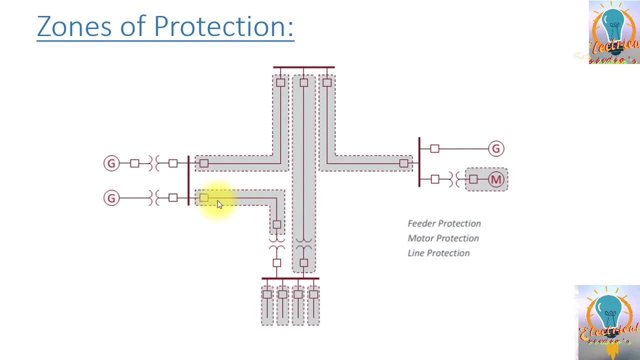 so i have this, this zone. similarly, i have make two more zones here. one zone i have make for this line from breaker to breaker, and one is zone is here, from breaker to breaker. so now you, you, i have prepared three zones so far: feeder protection, zone mode. this is the feeder protection that we have created first. then we have 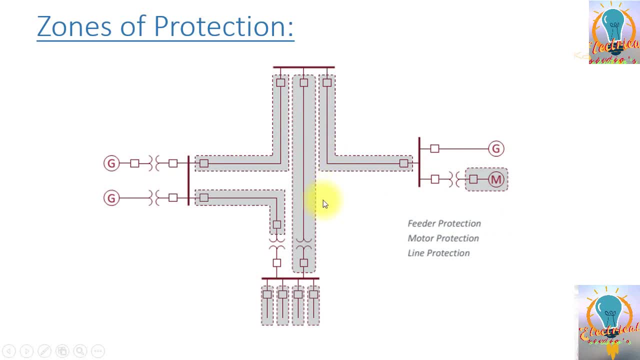 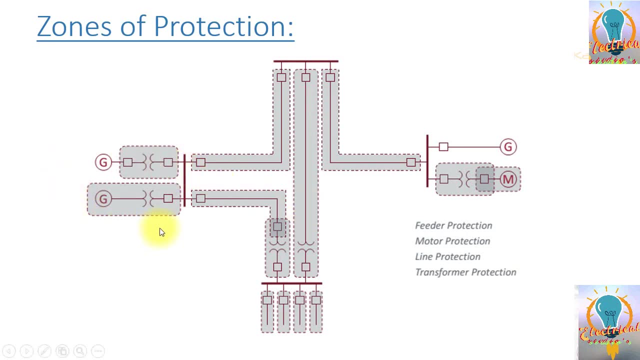 created the motor protection and then we have created the line protection number three i have created and the zone for generator protection. so i have created two zones. in zone one, you can see, i have taken a complete generator and i have taken a breaker and in this zone i have facilitated twice. if there is a fault here, for example, i will trip this breaker and this. 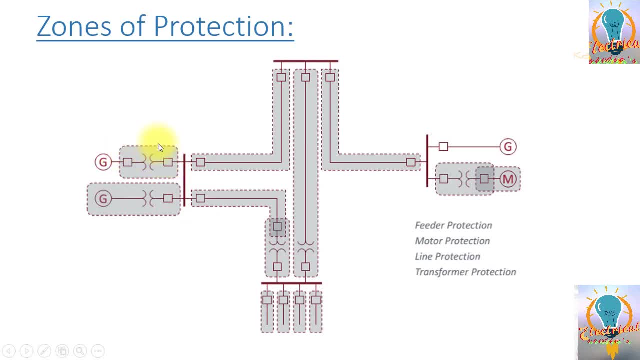 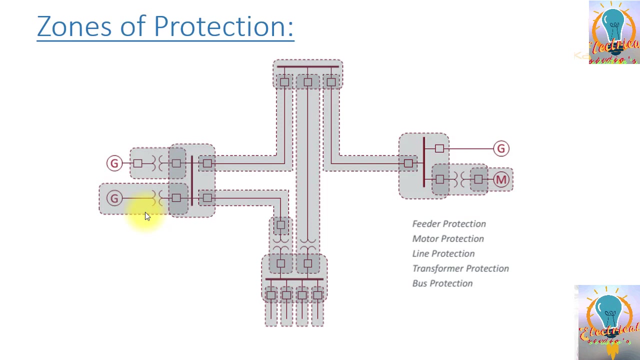 breaker. so i have made rather a small zone here. so the zone should be as small as possible. so this is to improve the selectivity. but here i don't have an option to isolate the fault, so i have taken the knitter together. so here now i have taken another three zones which are called as a bus bar protection. so i have drawn. 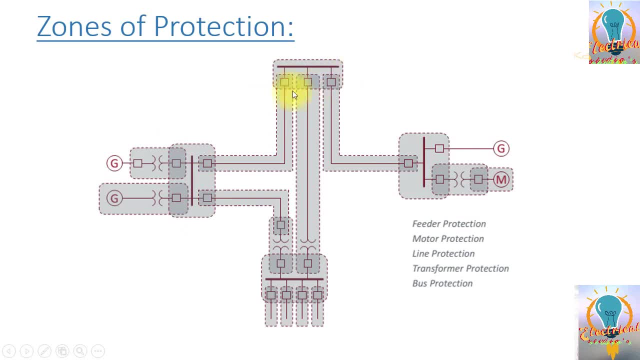 a zone here. this is one zone, this is another zone on the bus bar and this is another zone on the bus car. so if there is a fault on the bus and then the bus for protection will operate. and now here you can see, there is overlapping between these zones. so now this area is protected. 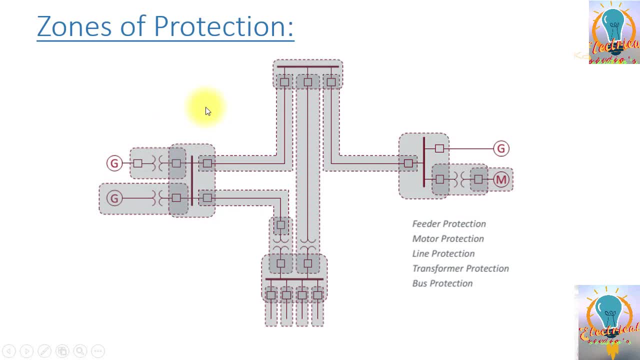 by two different zones. so overlapping is always good. all the protection systems should at least covered by one protection zone if and and it could be also covered by more than two protection zones, so over. normally, in order to protect the system, overlapping is done. so in this case, for. 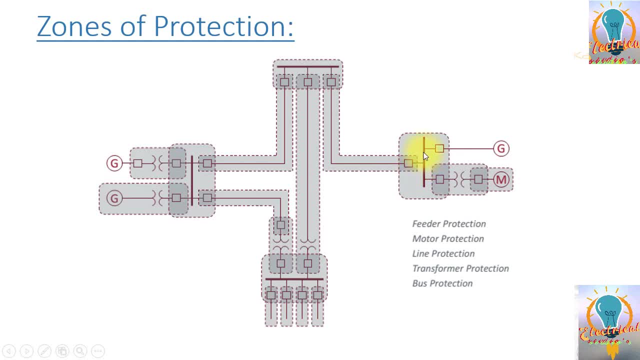 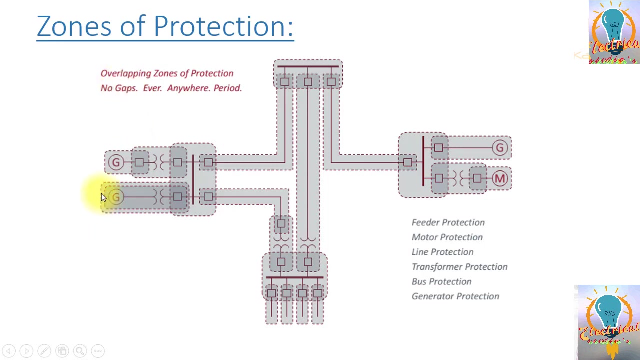 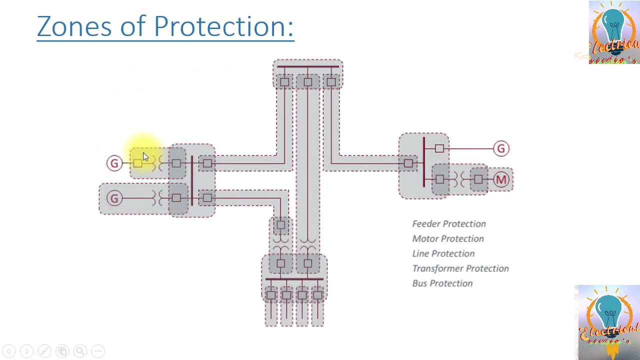 example, if this is a fault on the bus, bus per protection will operate. if the bus per protection fails to operate, then you can see this zone can also operate. now I have added here. you can see I have added as a native production here, so I have covered this part here. so I have added the denier production previously. 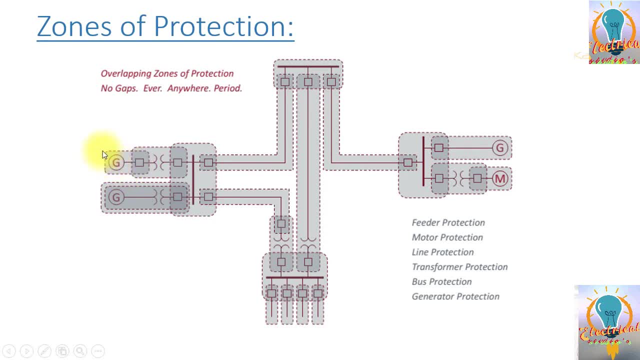 this was not there. so I am now deciding the zones. so I have added the native production here. so all the things you know, production, no gaps, every anywhere in the period. so no area of the protection system should be without covered covering, without any zone. so this is an example. so now we 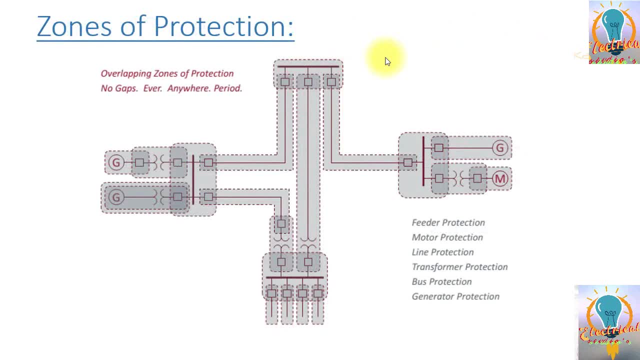 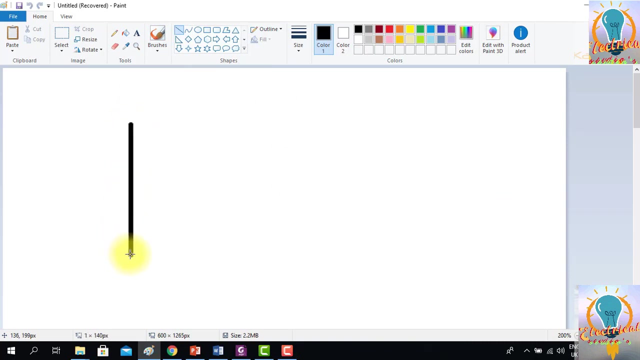 will discuss zones of protection. so let's have another example i will draw for you. so let's draw a busbar. so, for example, this is thinking, which is usually time when you're charging right now- so this is not the bus bar, okay, and this is the line, okay. so I will draw here one breaker. 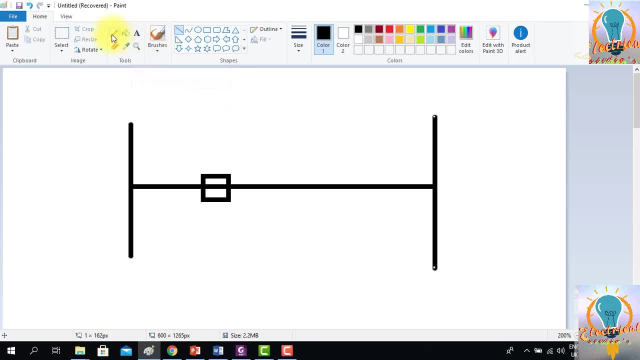 so this is representing station E, for example. this is the substation E. this is substation B. okay, and we have breaker here. we also have a breaker here and one CT is installed here. for example, we have one CT here and we have one CT after the breaker. 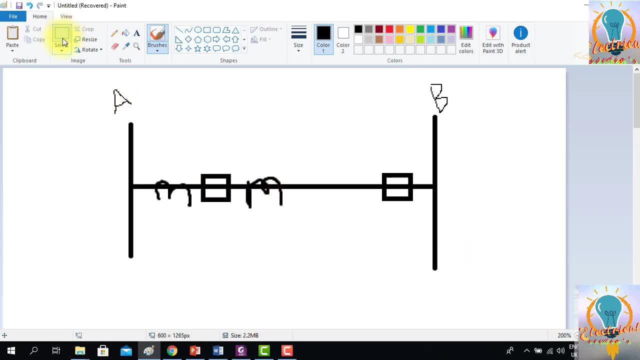 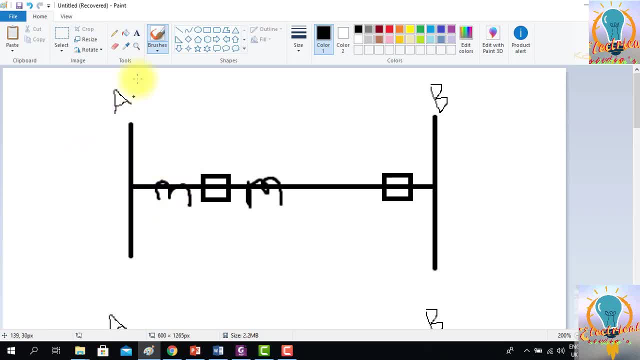 if you take a scheme like bus bar protection, if I take bus bar protection from this CT protection, if I take bus bar protection from this CT protection, if I take bus bar protection from this CT, so zone of protection will be kind, so zone of protection will be kind. 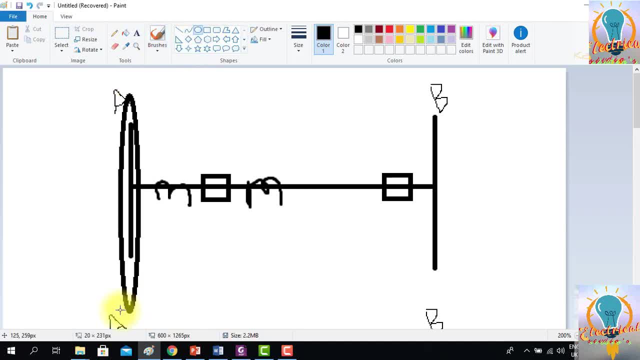 so zone of protection will be kind of this. so if I take this CT for the bus of this CT for the bus of this CT for the bus bar, so this is my bus bar zone and if I take a the line CT from this and I have another CT here if I take line differential. 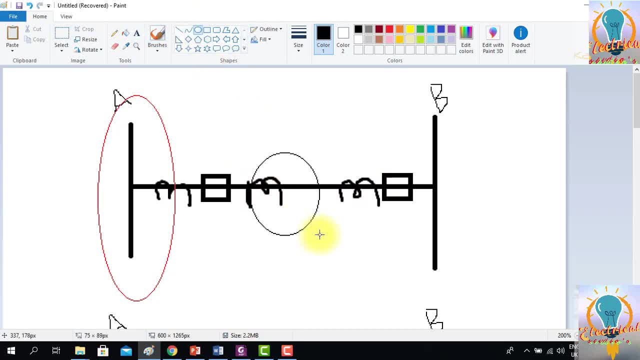 protection between these two CTs, then my zone will be kind of this: this is an example of doing the CT selection and it's another CT and if I take this CT on the busbar, so this is my middle. so now if I make such selection, so you can. 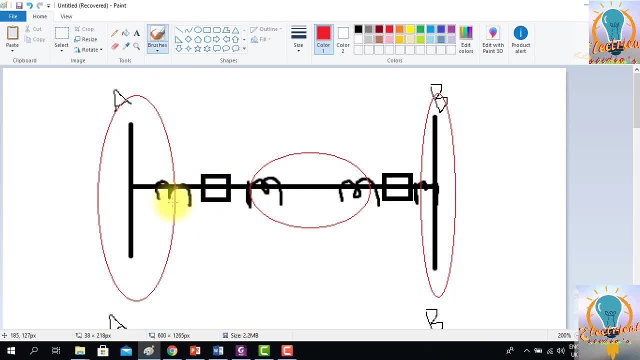 see this area. this area is basically not toward by any usable. there is a fault here. this is wrong 해. for example, if this is true and if this is happen, part so neither this zone will operate nor this one will operate. so this is an example of bad. 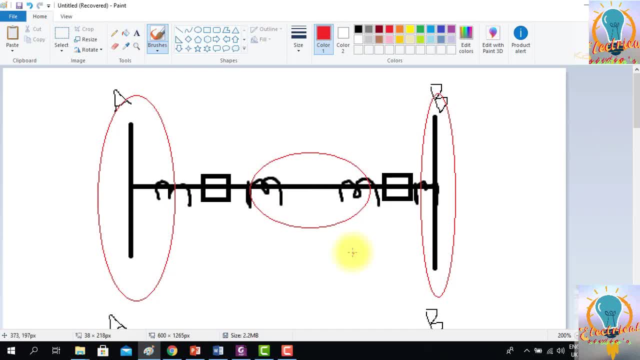 protection scheme. so what should i do? i will prefer in order to cover this area. i have the cts, same series, if i apply same ct and if i want to cover all the area, because this all area, which is not covered by any zone, is unprotected. so i have to change my skin here. so what? what i can do? 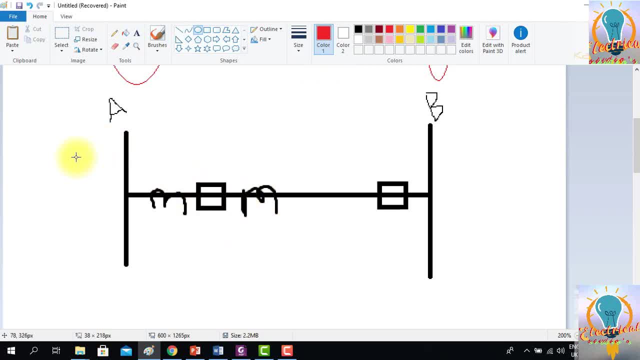 so i will select this ct for bus power. if i select this cd for bus power, so it means my bus power zone will be increased from here to here. so this ct will feed in the bus power. so my bus power zone now extended from this to that city. and let me draw this one will take the short ball on. 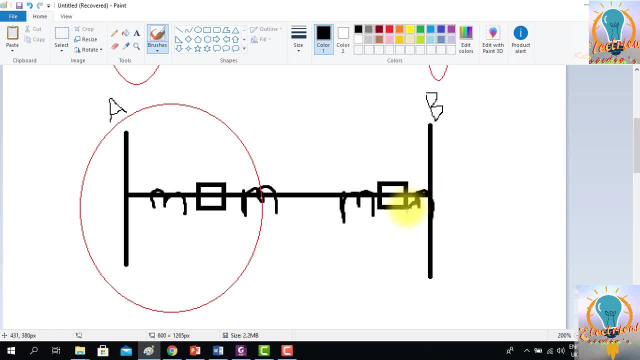 once ct here and one ct after ct after breaker, and if i take my line differential ct from this ct to this ct as well, any ct before breaker at the both ends. so now i have covered the line and also this area. similarly, at the other station i will choose the ct after the breaker for the bus power scheme. 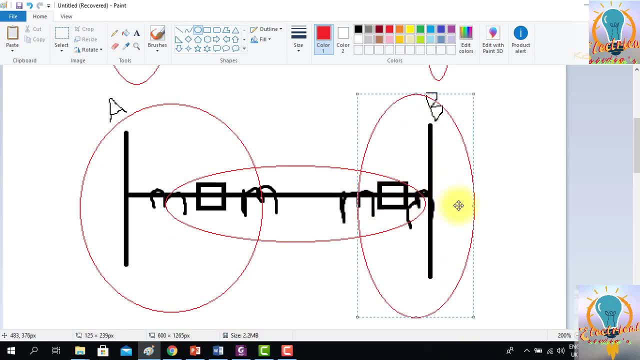 so now you can see in this way i have covered all the parts of the substations. so basically, from where you are connecting ct we are taking ct to the protection relay is deciding the boundary of that protection. so here you can see if there is a fault here in. 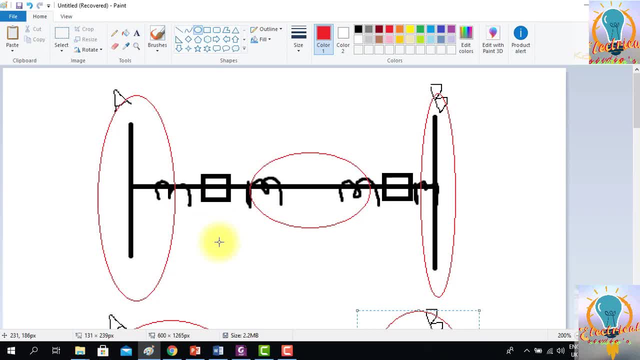 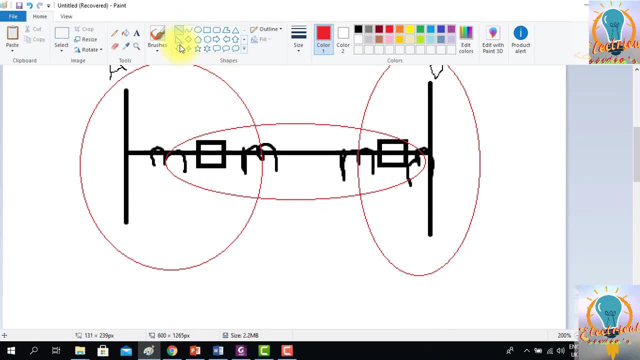 between in this area is there is a fault, so neither of the bus, by protection, nor the line production will work. but now, if i inject the fault again, if we consider a fault here again, this point, if it is a fault there is a fault here, this point, then buffer production can also operate. 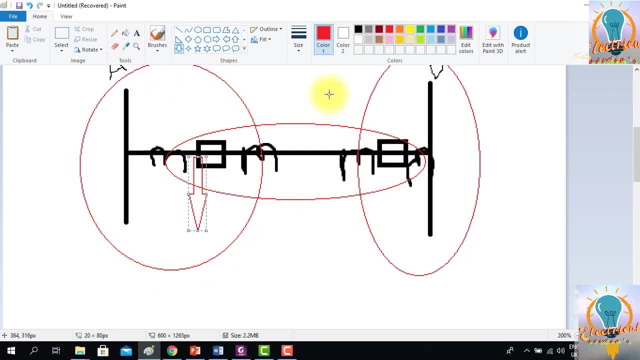 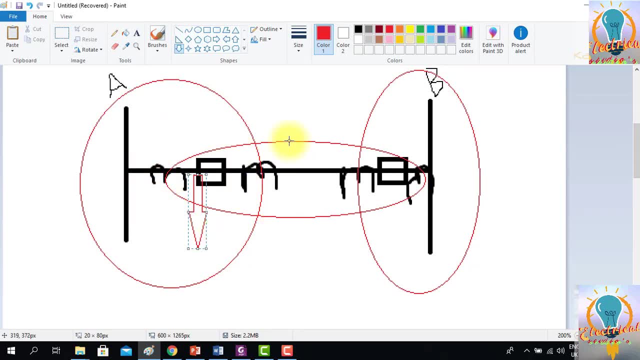 here and also the line production can operate. so line differential will also operate here. so this is an advantage and the forward will be immediately located and cleared. so i can do here one more thing: if there is a fault, for example in this area, so i can trip the breaker and isolate the fault. 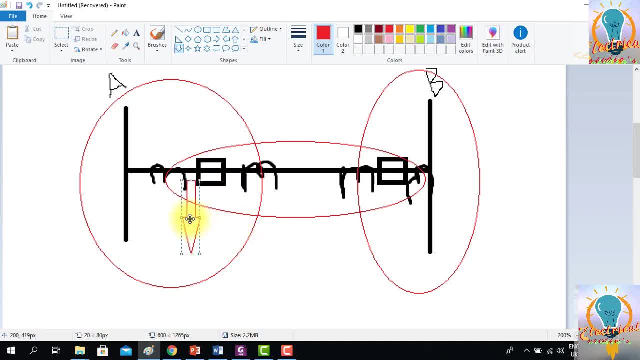 because i have the facility and if the fault is before breaker i can trip the bus bar immediately so that, because the fault will be kept on feeding through the bus in the breaker is opening through the other feeders. so, for example, if there is one more feeder here, 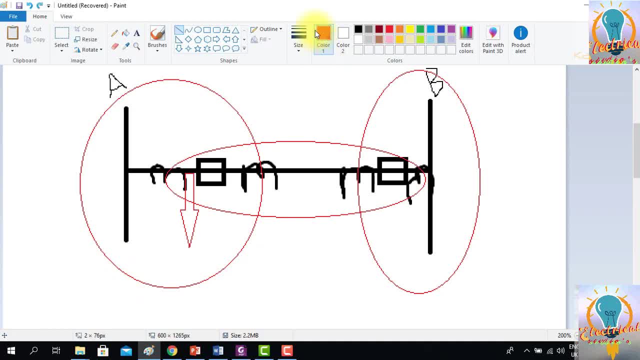 i think you know, i think linden deserved a couple more opens, not to say my right can't pick up a weapon, but there's absolutely nothing wrong with the way he's going. if there is one more here, then this will keep on feeding the fault. so this is this. 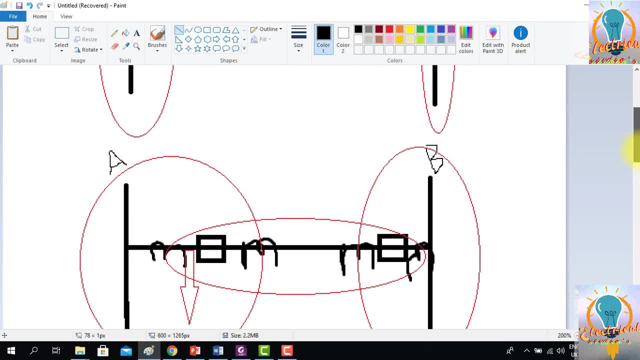 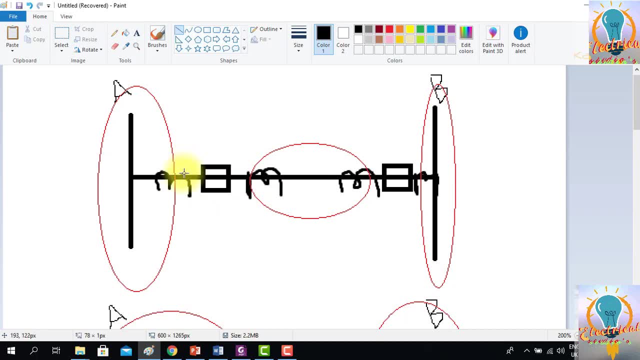 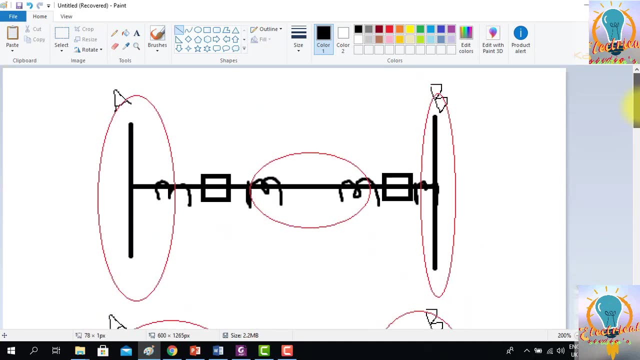 is an example of showing you that you need to cover all the area, this area, in this bad example of zoom selection, and this is the good example of zoom selection that i have shown you. so in this way you can increase the system stability. you can also increase the selectivity of the system. 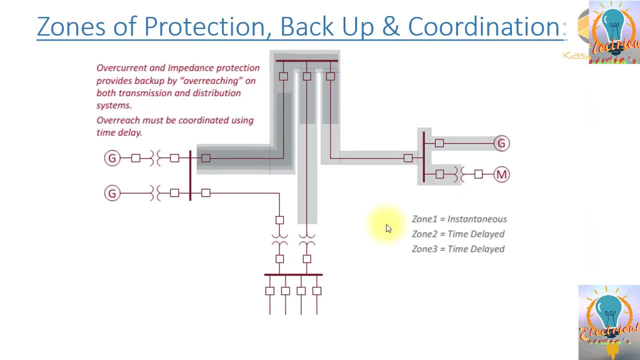 thank you very much. okay, guys, now we will see that how we have we can create backup of given zone protection. for example, we'll see, uh, we have installed a distance production here, so the distance production zone one is normally 85 percent. uh, so you can see, this is the line from this station considering. 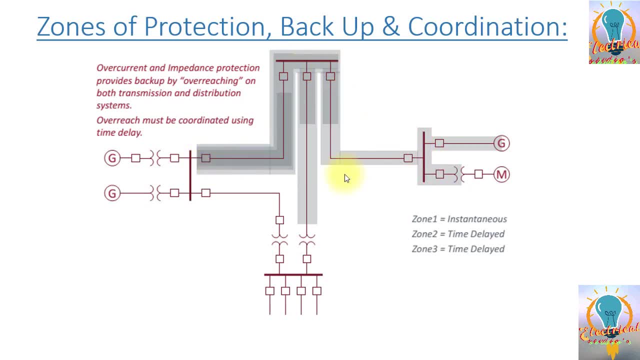 is that station a, this station b and this is station c. so here you can see, in zone one, discovering the 85 percent to 80 percent of the line. so time of zone one is instantaneous normally. uh, zone two: here you can see it has covered almost 120 percent to 30 percent of the second line. 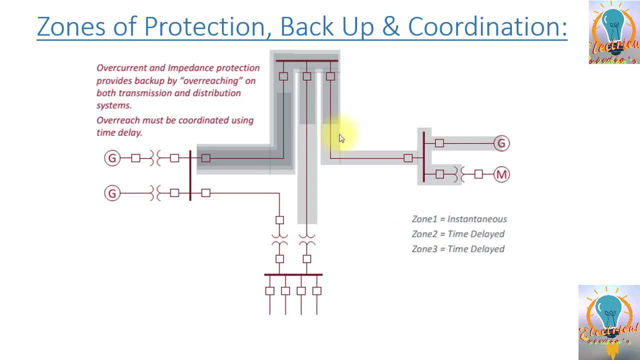 so time of zone two is normally 300 to 350 milliseconds. and then zone three, you can see, is covering here, uh, 225 percent or something to the shortest line or the third line. so here you can see if there is a fault here. for example, if there is a fault here in zone two, this is, it is the zone one of this relay. this relay should trip. 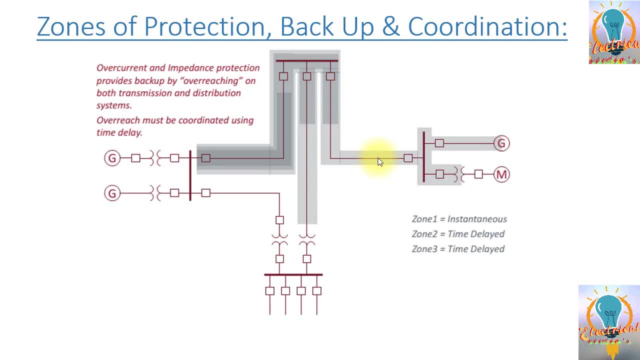 in zone one. okay, and if this relay has not tripped in zone one, then you can see this relay, it can trip in zone three. uh, with the zone three time delay, approximately seven milliseconds. similarly, if there is a fault somewhere here, so this relay should trip in zone one. 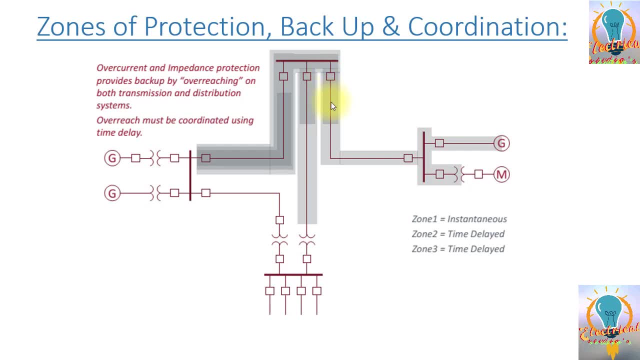 instantaneous, but if it is, it is not tripped in zone one, then this relay- it is zone two of this relay- will trip in the given time of 350 milliseconds. so in this way and the backup is provided for the protection systems. so here you can see this: protection zones and their backups. 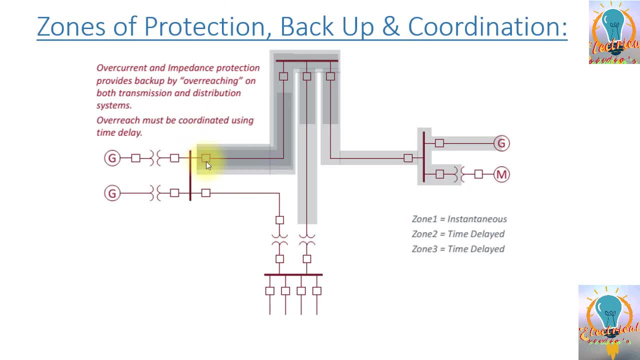 so similarly on each station with the distance relay and backup and protection is also installed. so on the same station, backup production is available as a backup over time with the distance, for example, if this one operates, if there is a fault here and distance should operate. if distance is not operating, then there is a backup of uh open production. 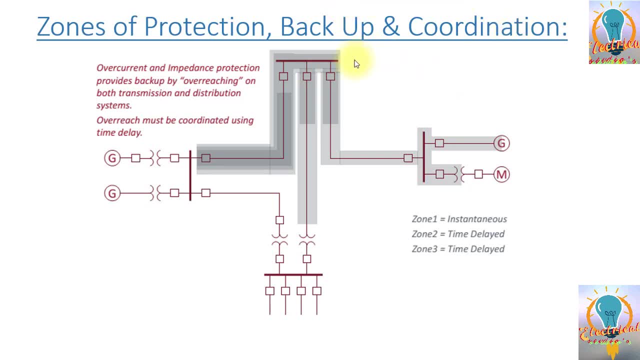 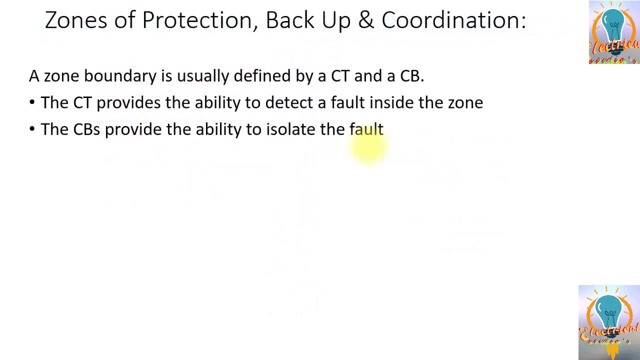 is there also. so backup should operate. so one backup operation is installed at the same point, another backup is being done by at remote and by the other protection. so in this these zones are created and these, these are backing up. so zone boundary is usually defined by ct and a circuit breaker. the ct provides the ability to 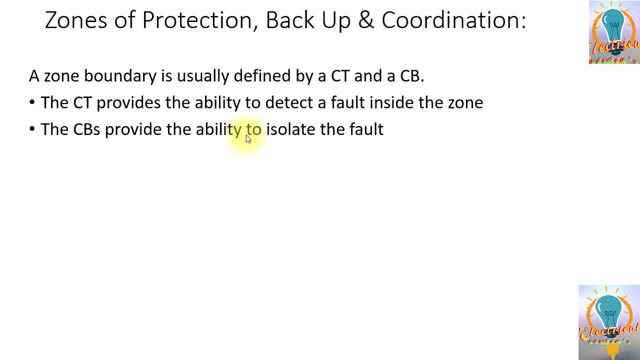 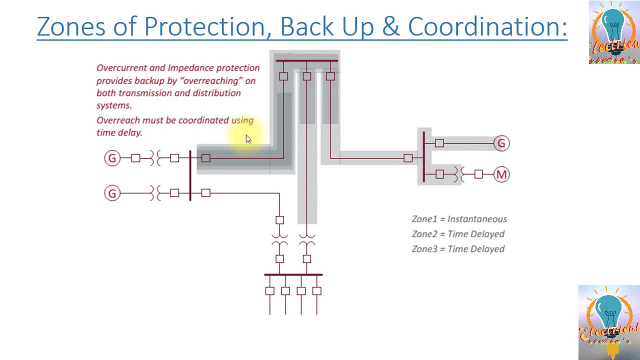 detect a fault inside the zone, the circuit breaker provides the ability to isolate the fault. so this is little introduction about the backup and how we can do the backup and how we can do the backup and how we can create a backup and how we can build a backup. 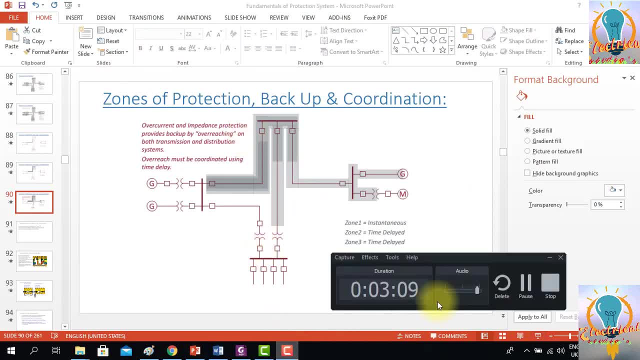 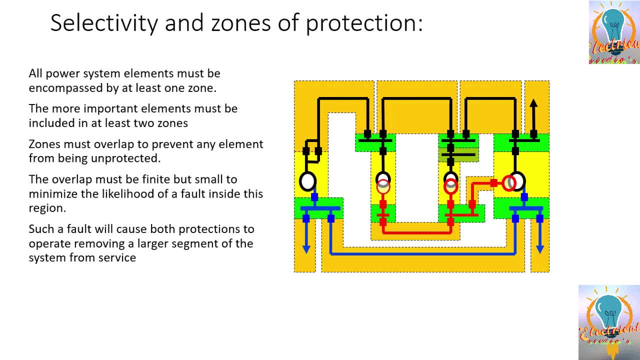 do the coordination. thank you very much. hello friends, here we will go through a little conclusion that all the power system element must be encompassed by at least one zone, and we have seen example that all the power system should be at least covered by a single zone of protection, but it could be more than one. 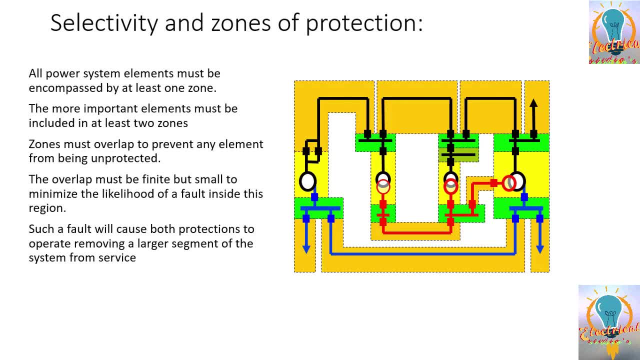 zone of protection, which is called an overlapping. the more important element must be included in at least two zones. zones must overlap to prevent any element from being unprotected. the overlap must be finite but small to minimize the likelihood of a fall inside this region. between that overlap should. 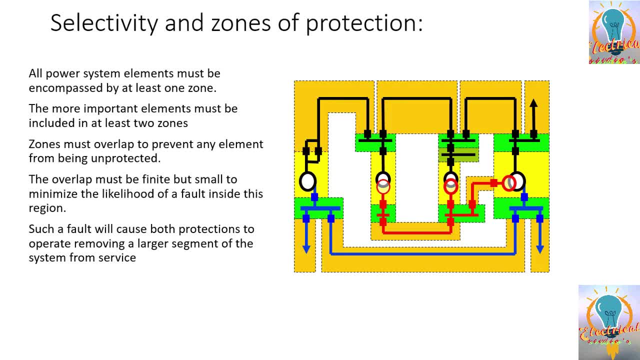 not be unlimited, so it should be limited to a certain portion. such a fault will cause both protections to operate, moving a larger segment of the systems from the service. so overlapping is good, but the disadvantage overlapping is that both production could operate in. that specific is for the current that. 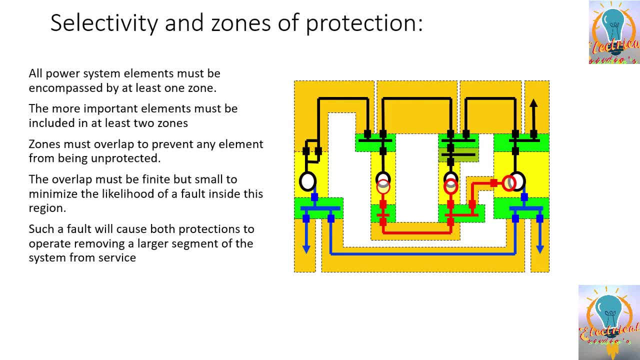 specific area, as I told you. if, for example, I have covered a region with the bus bar and the land production, so any financial protection is the for liquor, both will operate, so it will result in outage of a bigger area. so we need to consider, or each and every aspects before going forward. so here you can see. 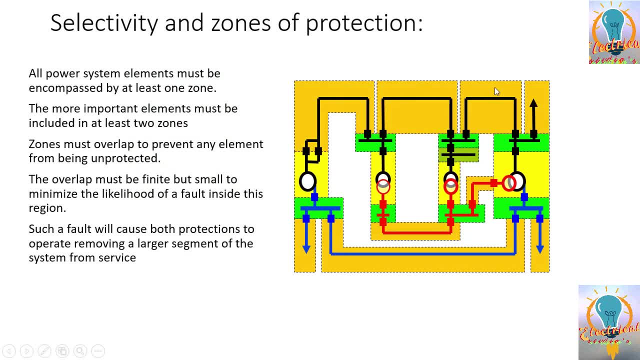 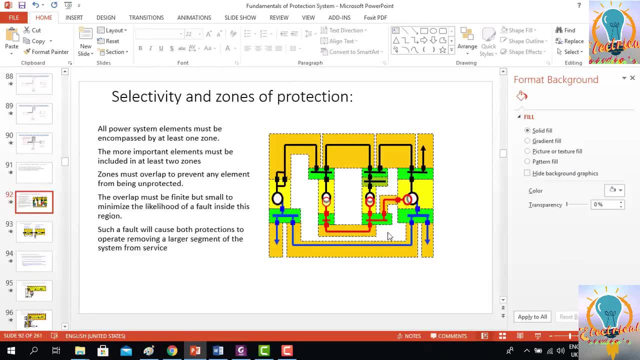 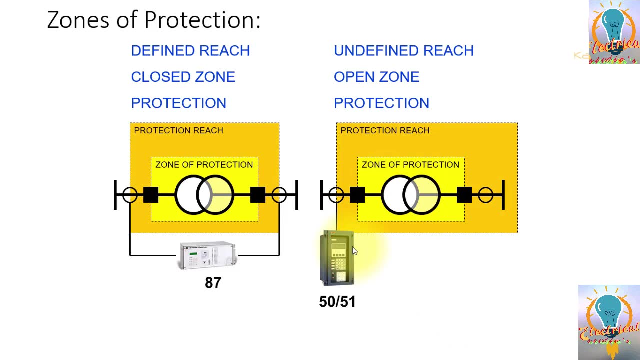 a power system. we have created some zones. so this is another example of so much. thank you very much. hey guys, now we will consider a case of zones of production which is created by work and really FN time, instantaneous or by a line difference protection, really basically nine differential production really is. 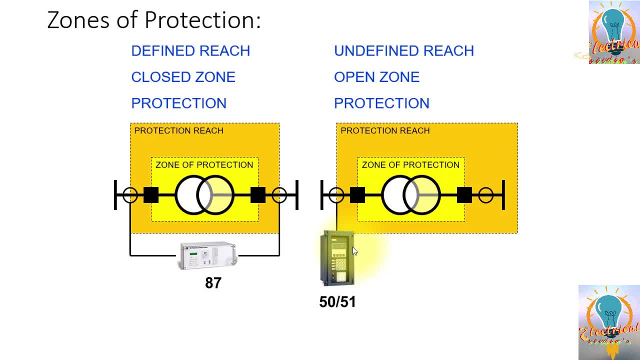 called as a unit production. this it means that it will operate if there is a problem on a specific given unit, whereas the orchard protection is operating, whereas work and production is basically operating based on the current only. so, for example, this here you can see this is: 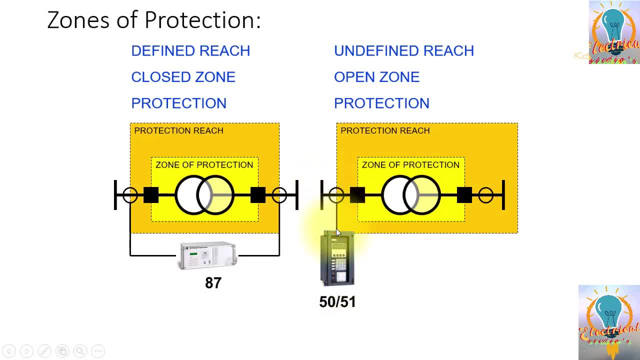 the work and protection and it's speed by only one CT, whereas the line differential protection, here it is saved by two different cities and if there is a truth, if there is a fault within this two zones, within these two cities, within this zone, then this differential protection will operate. if there is a fault outside of the 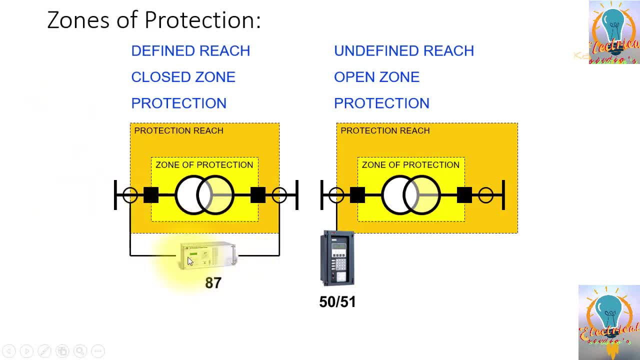 zone, then this differential protection will not operate. if there is a fault outside of the zone, then this differential protection will not operate. if there is a fault outside of the zone, then this differential protection will not operate, because if there is a fault outside of the zone, the current in and out of the 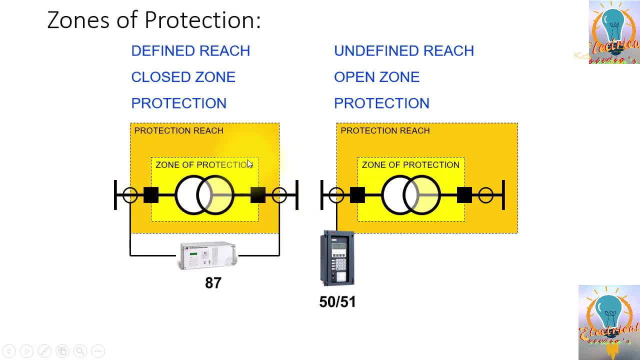 CT will remain same, but if there is a fault inside of the zone then current entering and leaving will not be the same and different production will operate. so the different production. it has a defined reach. the zone is is closed here. so you can see: zone is closed, zone of production is this. it is. 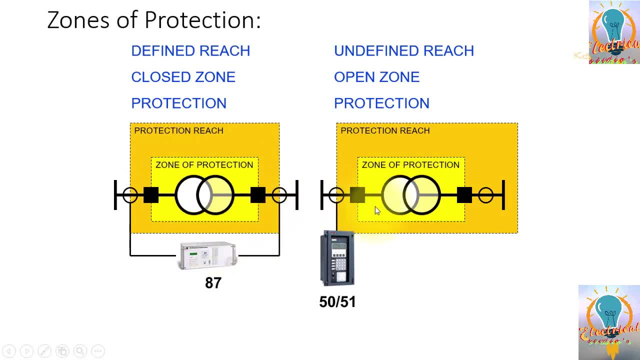 closed and reach is defined, whereas the work and protection is fitted by only one CT. if there is a fault, for example, here, the relay will operate. if there is a fault on another station, here the fault level will be lesser, but still the current will be filled by this breaker and then 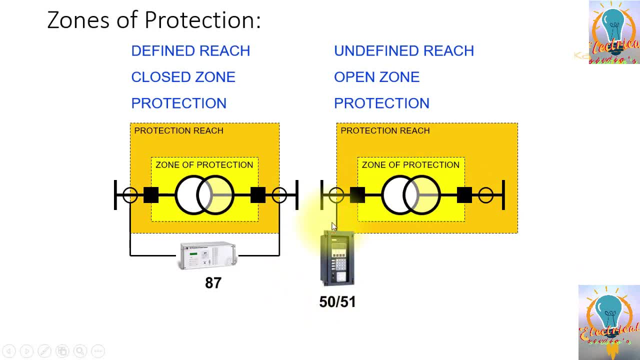 this protection, differential protection will operate. so this is an example of two different protection schemes. so let's consider again. just consider here: if there is a another feeder outside and if there is a fault here, so this fault current will be feed by this bus. you go to the ground and this current will go to the relay in the secondary side and the 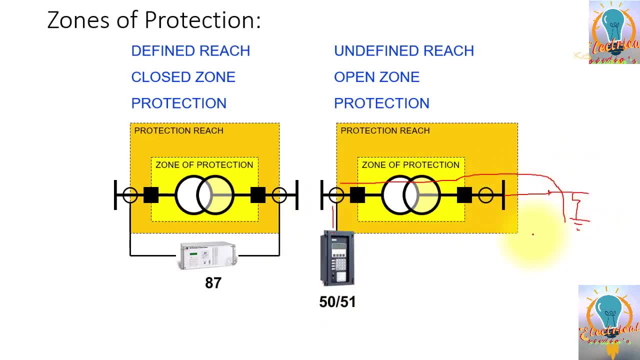 relay might pick up and trip. so this is still in the reach of the over current relay and, for example, if there is a fault here, the fault is now, at this time, near to the source. just consider that we have a source here, we have the net installed here, so again, the current will flow. 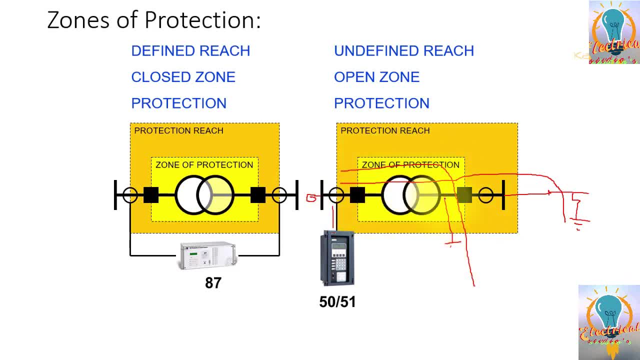 from here to here the current value of current will be more, because now the conductor length is increased, but the fault current will be feed through this and then again the current will go to the relay. so the zone of this relay is not very well defined, so its zone is open, okay, whereas in 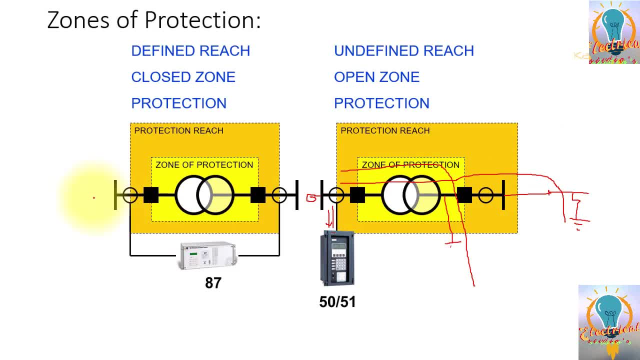 this case. just consider, for example, if we have line here, if there is a fault here. okay, 100 ampere sentence, for example, is flowing from here to the ground, so it mean 100 ampere current is leaving from here and a 100 ampere current is entering here in hadn't amp rape and it is also leaving. 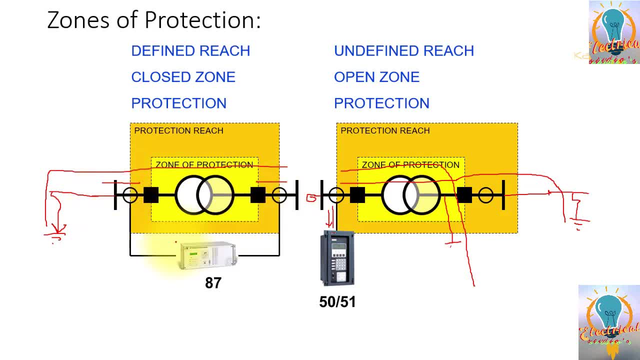 from this. so current in and out, both are same. so differential current here will be I. differential will be zero. okay, so differential current in this case will be zero. so we are calling a fault which is outside our differential zone. we are calling it as a through fault. this is a terminology that we are using in a 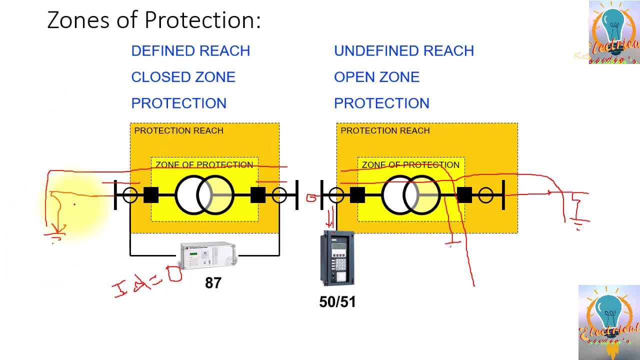 protection system. so the differential protection should not operate on the through fault which is outside the zone is closed. the zone of this protection is between these two cities. okay, so this is a protection reach. so now we consider another fault. for example, the same fault come here, the refuse to ground fault here, now current. 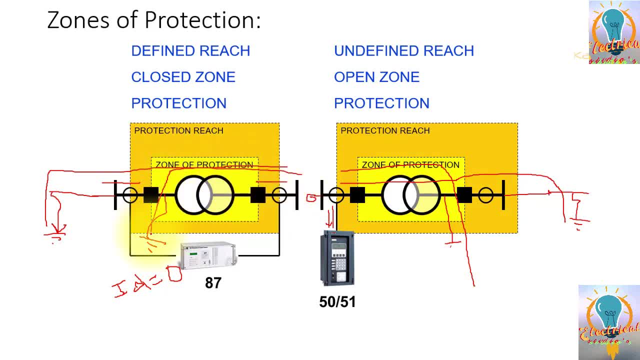 occurs. you can see the path of current from here. it will go to ground and then back to the generator. so here you can see here that 100 amp current is now again flowing here. for example, this ct is 100 by one, so one amp current will be here, one amp will be entering the relay and this relay there will 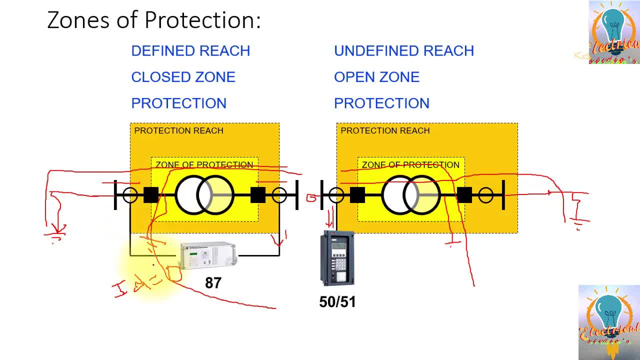 be no current, because all the current is bypassed and flowing to the ground now. so differential current will be equal to, in this case, for example, one ampere, and if we have set the relay settings to 0.5, for example, this relay will operate and trip the circuit, these two circuit breakers. so 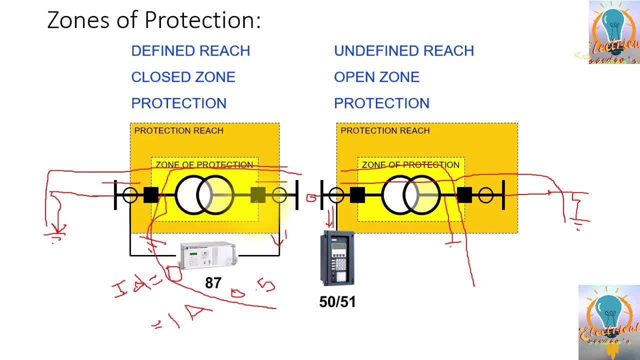 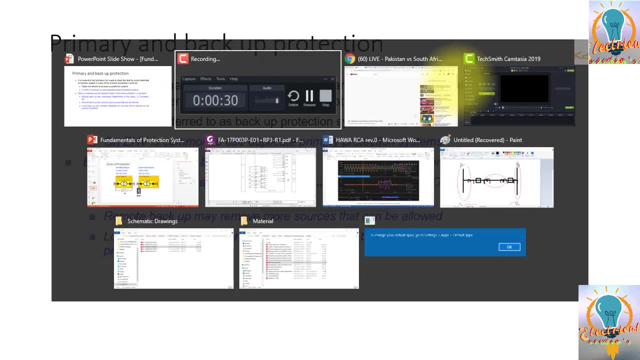 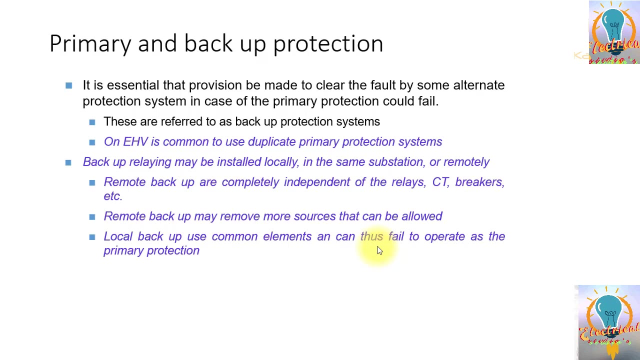 that's why we are calling a different production as a closed zone and over current protection as an open zone. so i hope you have an idea about this and different type of sections. thank you very much. hey, friends, now we discuss the concept of primary and backup production. so why? 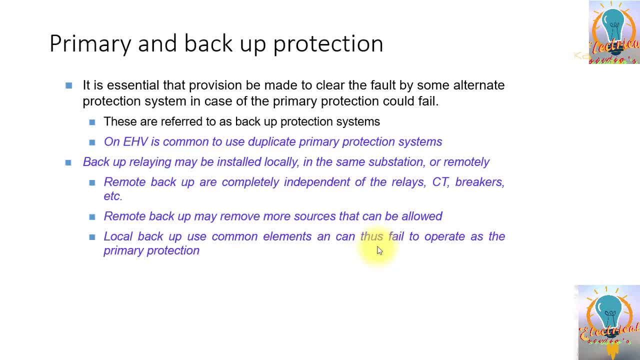 we need a backup protection. so backup protection is required, basically to in order to if the fact that if main protection fails, there should be a backup production available so that it can operate. So another concept in extra high voltage is to use a duplicate protection scheme on the lines. 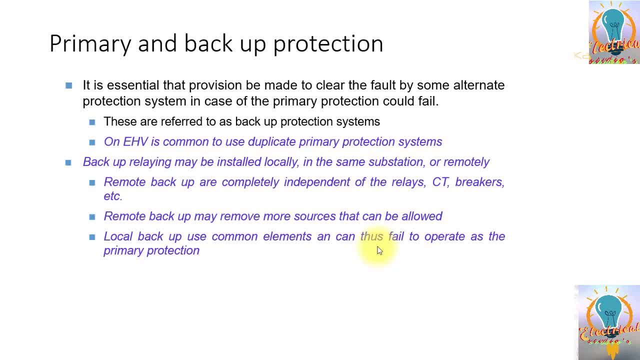 In extra high voltage. we are using two distance protection and two backup over current protection. So each distance protection is fed from a separate CT core and it is also connected to a separate DC bank in a substation. So each distance protection is also giving tripping command to a separate tripping coil of the breaker. 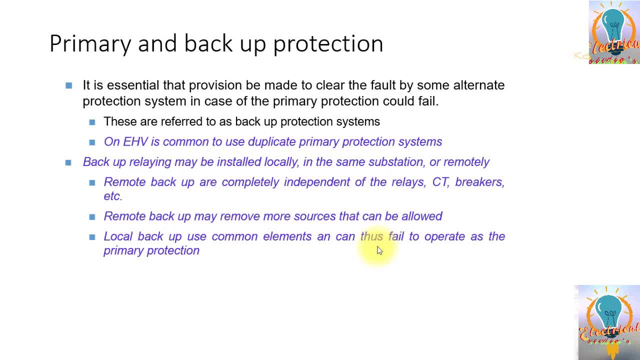 So in this way, the concept is to create a redundancy. So in order to create a redundancy in a substation, two DC supplies are normally placed and installed And two protections are installed on the extra high voltage And there are two trippers And there are two tripper coils available on 132kV and above levels. 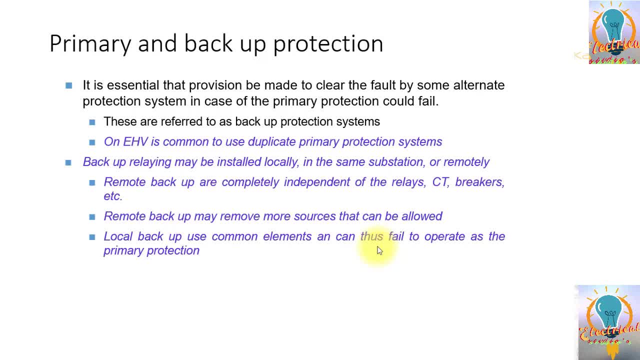 So if one tripper coil fails, another tripper coil is still available to trip and to the breaker and isolate the fault. Apart from duplicate protection, duplicate protection has the same timing as it is as the main protection, So we can call this protection as main 1 and main 2 in our extra high voltage. 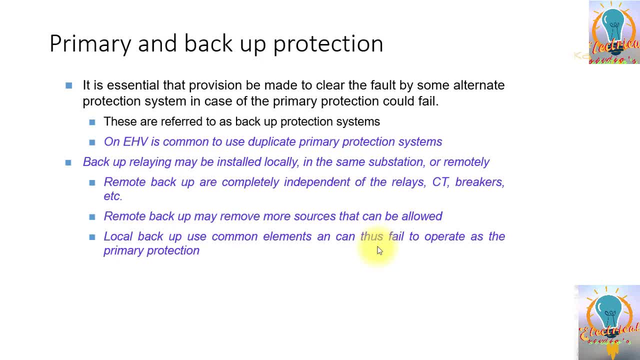 Whereas the backup protection has. The backup protection has delayed tripping. So if main protection duplicate 1 and 2, both are failed, then the backup protection should operate. So backup protection. there are two types of backup protection. One, backup protection, is installed in the same substation, just like installing a backup over current relay to a main distance relay. 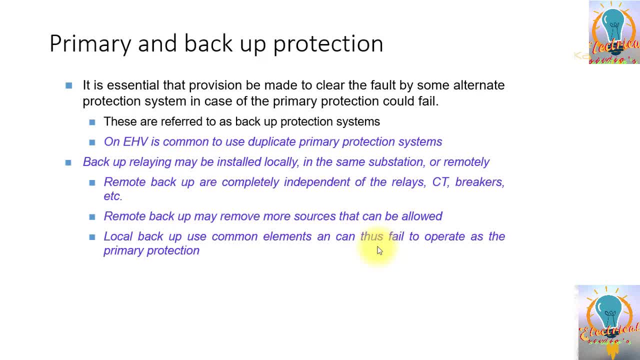 Or other option could be to install backup at the remote. So if you are installing backup over current relay to a main distance relay, So if you are installing a backup protection at the remote station, it means you have completely independent relay. You have completely independent CT breaker. 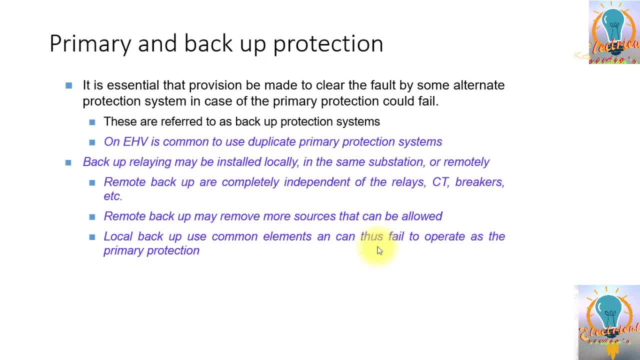 You have completely independent DC system and everything, Whereas if you installed a relay- a backup relay- on the local end, Then it means that the backup relay will also be feed from the same CT. It will utilize also the same DC supply. So there are more chances that if the main relay fails, the backup will also fail. 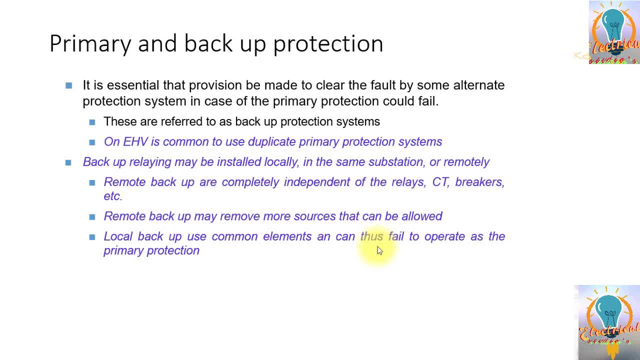 But the remote Disadvantage of remote relay is that there could be more than one remote relay is installed at different location, Because one location of the one substation could be feed from more than one sources, So each source will be. Each line would have a backup protection. 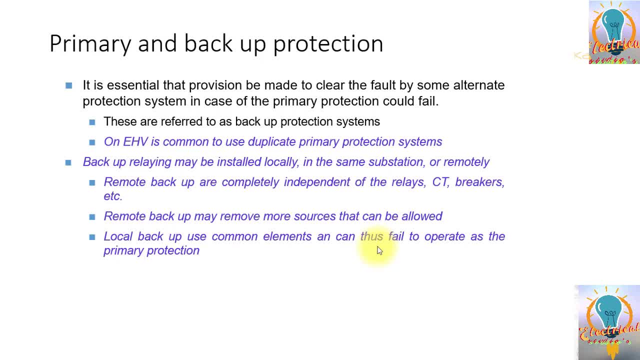 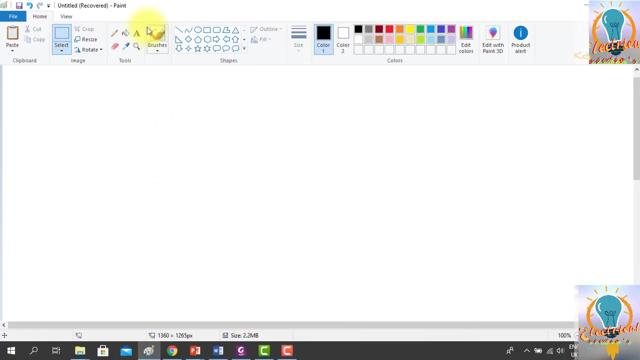 And the result could be, Instead of tripping one line, and if it fails to trip then the other backup lines, they will be tripping on more than one line, So which is not a great sight. So let's see this example, So let's make a 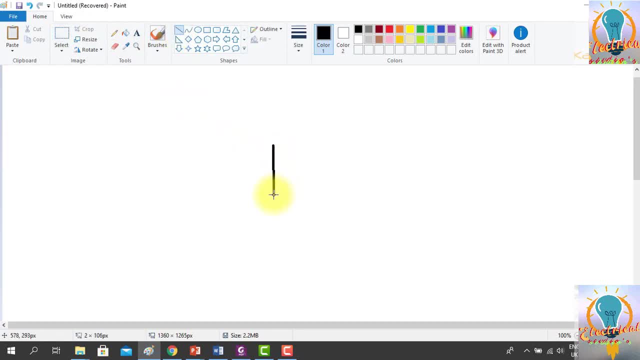 I will make substation here. This is our busbar, substation A. This is substation B. This is here. you can see substation C, Or make this one And you can see. this is the line And this is another line. 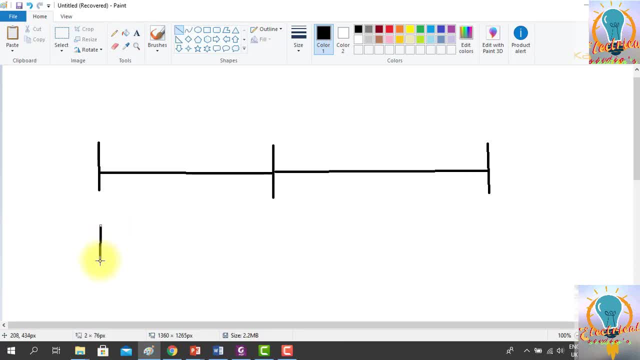 And this substation is feed by more than one source, for example. So now, for example, if we have, Let's draw breaker here also. So this is the breaker, One breaker here, One breaker here. We have one breaker here, One here. 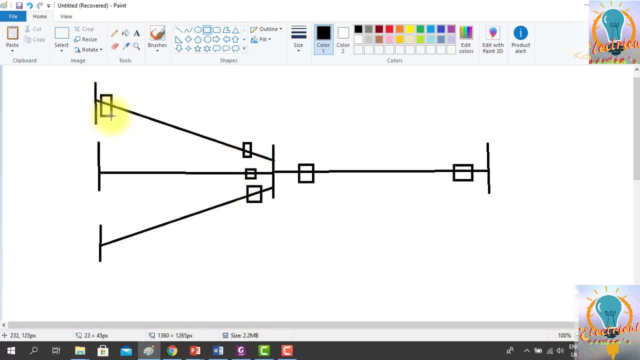 One here. We have one breaker here. One breaker here, One breaker here. Okay, So you can see now, the zone 1 of this station of the relay is from here to here. This is the zone 1.. Okay, Whereas zone 1 of this relay is from here. 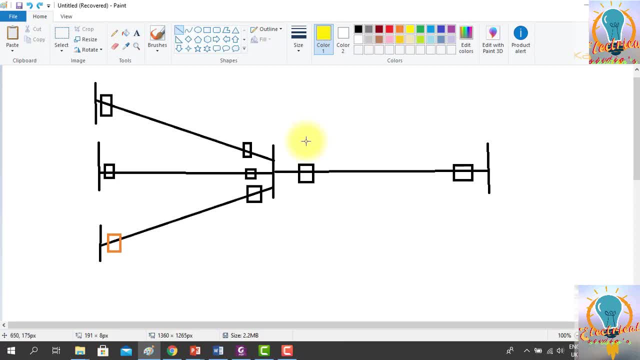 Just a minute. Let me correct this. Zone 1 of this relay is from here to 85%. Zone 2 of this relay is from here to 120%, If we consider this one as zone 2.. And zone 1 of this relay is 85%. 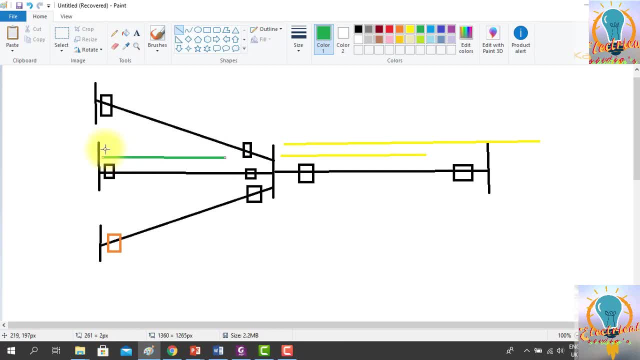 Zone 2, for example, from here to 120%. Okay, This relay, zone 1, again, here is 85%. Zone 2 will be somewhere here to let it make it another color, Make this one brown Zone 1.. Zone 2 will be kind of here. 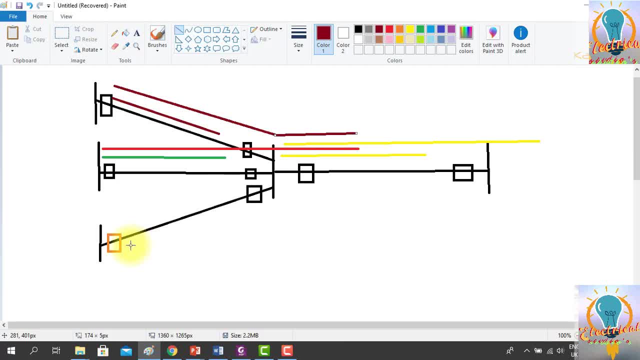 And zone 1 is 25%, Zone 2 will be kind of up to here. So we have here protection relay installed And that is we have 21 here. Okay, We have here distance relay 21.. Which is a distance protection? 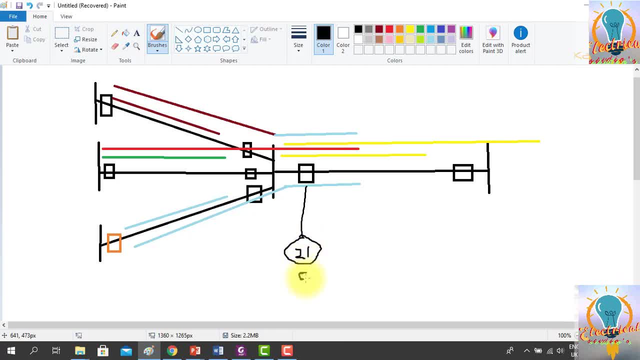 And we have also 51. Or we can say 50. Definite time over current. Here we have also 21.. Distance protection, And here we also have distance protection, And here also we have distance protection. So first of all we consider the case here that if there is a fault here, 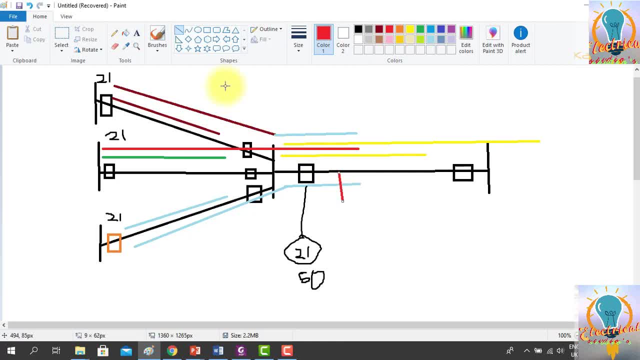 In the line. there is a fault here. Okay, There is a ground fault here. The line is grounded here. Okay, Let's draw a better presentation. So line is somehow grounded here. So it means that fault current will be feeded from all three sources to the ground. 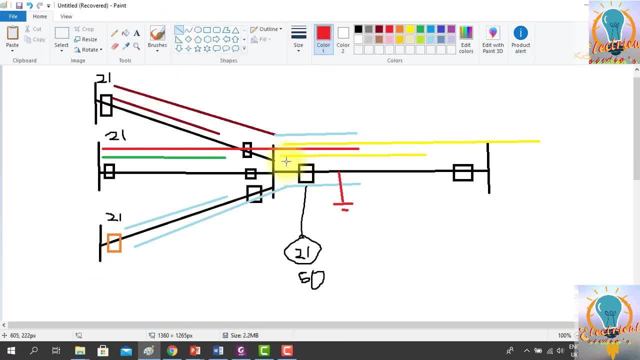 Fault current will be all three sources to ground. It will be from here, So let's choose another color, like blue. The fault will be flowing here to here. Also, the fault will be feeded from this source, This source And this source. 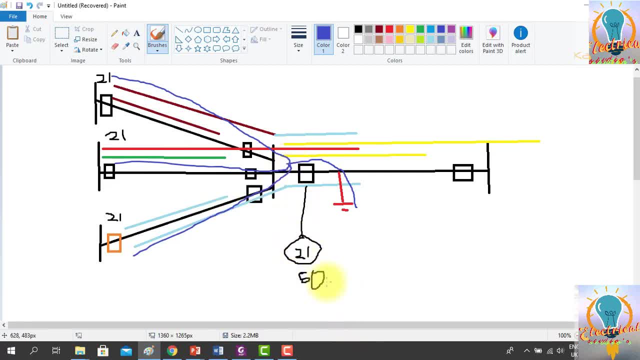 So let's suppose the distance protection should operate Here. you can see distance protection Here we have 21. And 50. Over current protection. So distance protection should operate here. But for example distance protection should operate in zone 1. Zone 1: time here is instantaneous. 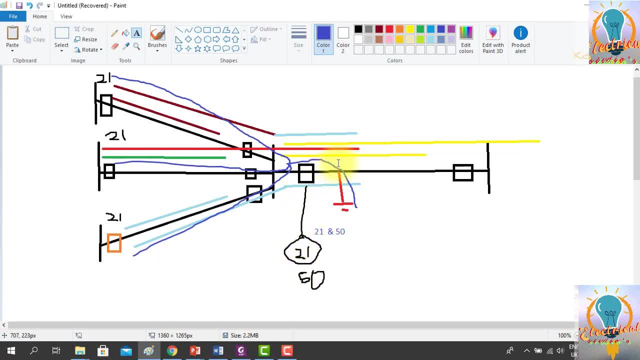 So ideally zone 1 of the distance protection operates And it will open this breaker And it will send signal to the remote end also, And then the remote end breaker will also trip by teleprotection. So this is an ideal scenario. But if, for example, distance relay fails, 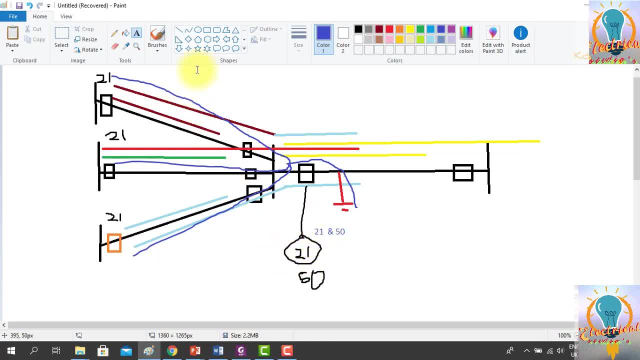 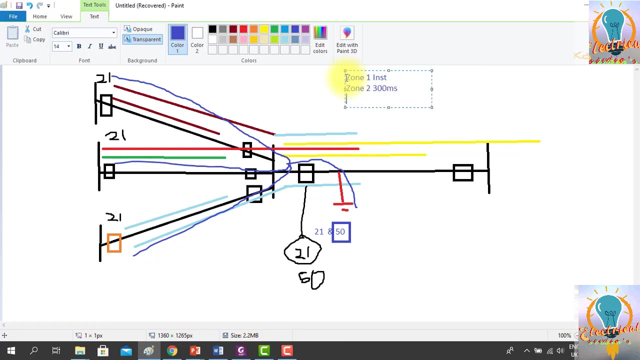 So if distance relay fails then it has two backup. We have one backup protection installed, The same substation, which is 50 over current relay. Okay, So if we normally the timing of zones is defined here as zone 1 is instantaneous, Zone 2 is 300 milliseconds. 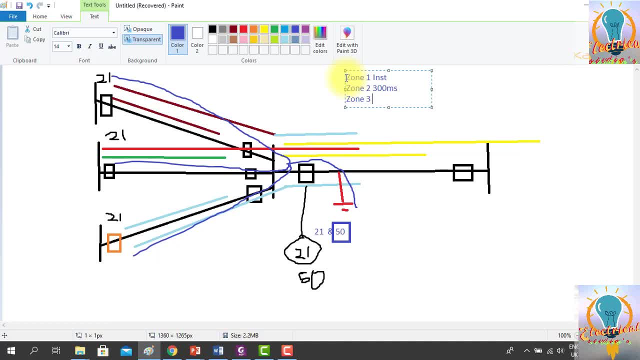 Zone 3 is, for example, 700 milliseconds, So this is normal. We are setting these zones like this. So this is a face to ground fault. So if I set this settings here, If this is my backup over current, So it should operate instantaneously. 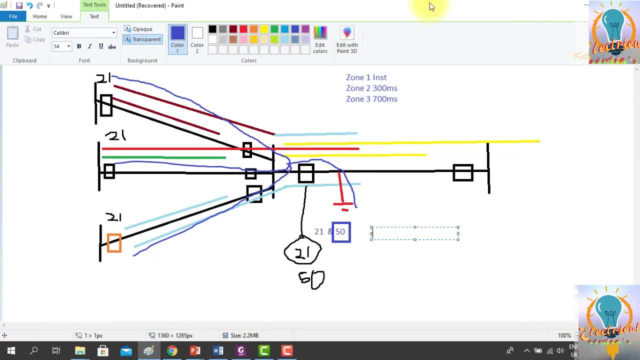 If it has not operated, Then, for example, if I have set to operate the backup over current And just before zone 2. Just like 200 milliseconds. So if I set this one, Then this backup over current here Circuit, over current earth fault, 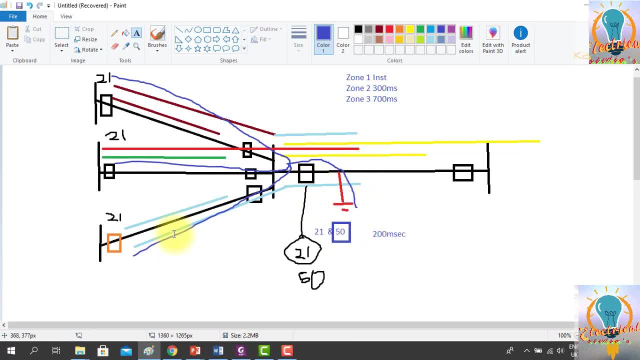 Definite time will operate in 200 milliseconds. So still these relays, all These, all three relays are picked up in zone 2. But zone 2 timer is 300 milliseconds. They will wait for 300 milliseconds before issuing the command. 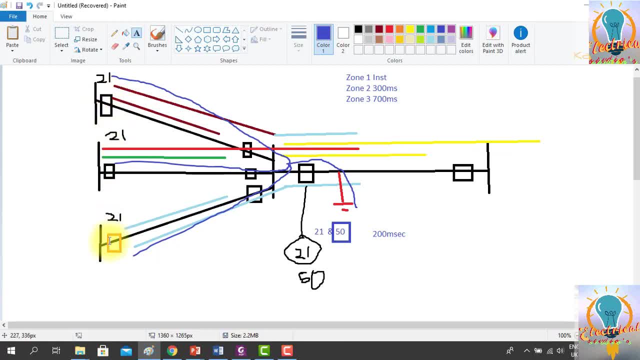 So these three relays are distance relays. These are working as a backup protection of relay here. So you can see the relays are installed at remote locations And the CT here is totally different, VT here is totally different, This power supply is totally different. 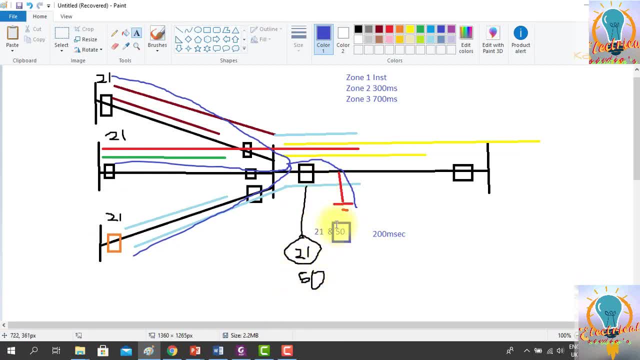 Everything is independent, But here this backup installed here. So if this protection operates, Then breaker will open And the forward current will be reset. There will be no dripping. Only this breaker will be dripped. So this is the advantage of local backup over current protection. 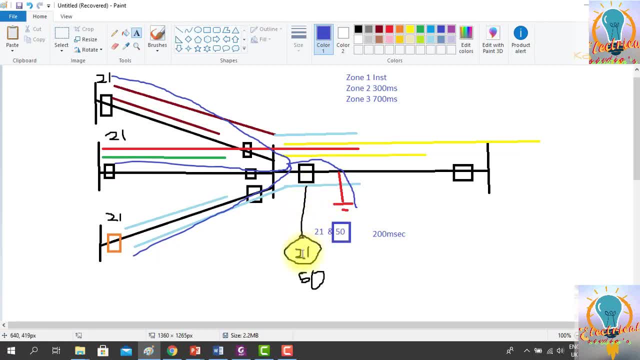 But just consider a case that VT was such as to hesitate And the over current relay, backup over current, was also feeding through the same CT, So this protection also did not operate. So now all three distance protections. Now the timer will run. 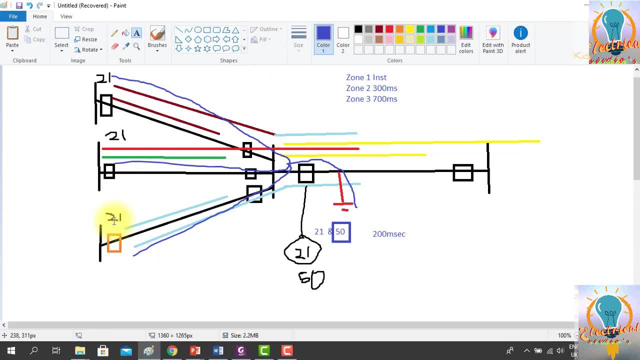 And whereas 300 milliseconds are crossed, All the three sources will drip And all three- you can see lines- will drip. Instead of dripping one breaker, The three breakers will drip. So this is a remote location. There are advantages is that everything is separate. 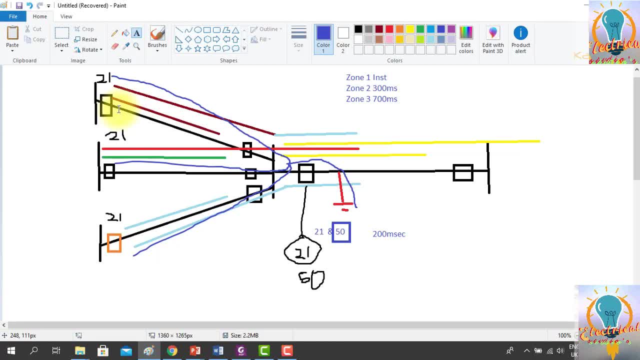 Every supply, DC supply, AC supply, Breaker, Everything is redundant here Separate. But the disadvantage is to But now because there are lot of sources at remote, So there could be lot of power shutdowns Or then one sources will be out. 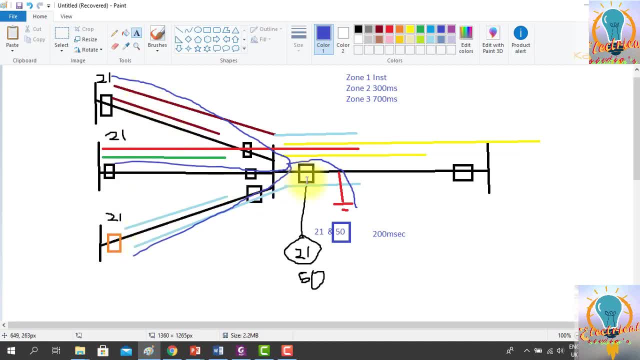 So all three lines will be out Which are feeding this line. So this is an disadvantage For this. That's why on extra high voltage Normally we are keeping two distance protection Or feeding from two different CTs If one distance fail. 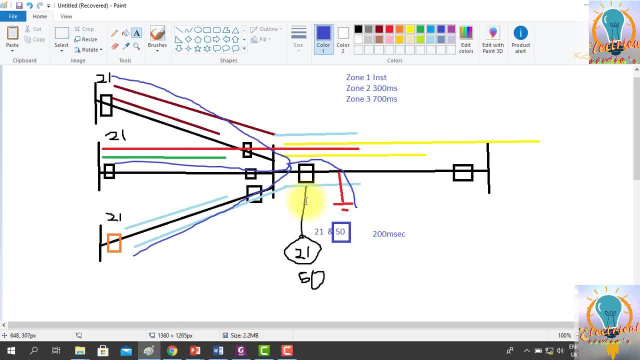 Still the chances to that other distance will drip. Otherwise You can see That normally the backup protection time is not set to 200.. It's just I have taken example. The backup protection is normally is taking as to 500 milliseconds or one seconds. 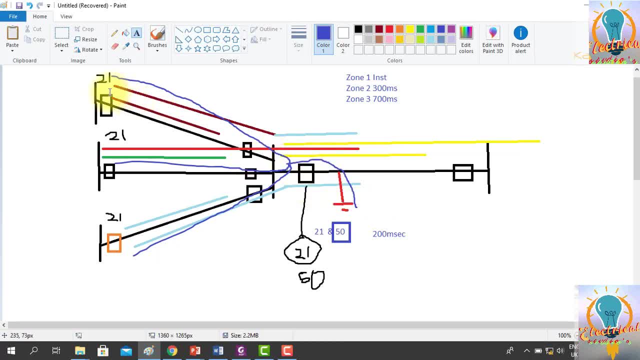 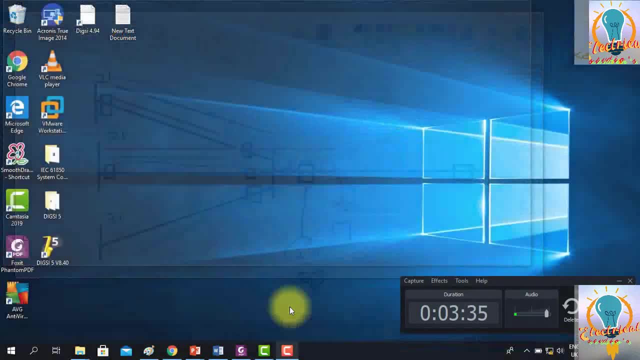 So If this relay did not drip, The other relays In zone 2. They will drip And isolate the fault. So I hope you have understand the concept in detail. So thank you very much, Hi guys In this section 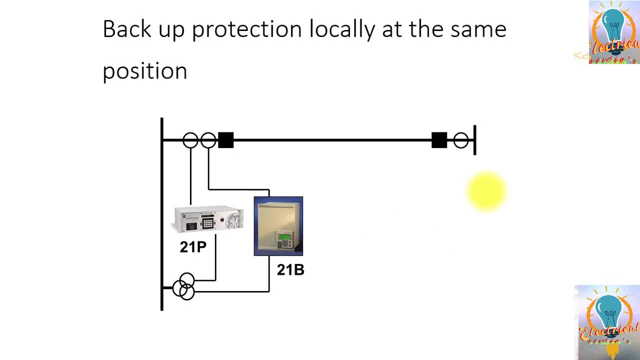 We will consider An example Where we have a backup protection Which is installed on the same substations. Here you can see There are two different CT cores. Core 1 is feeding 21B. Where is the core 2 is feeding to 21B. 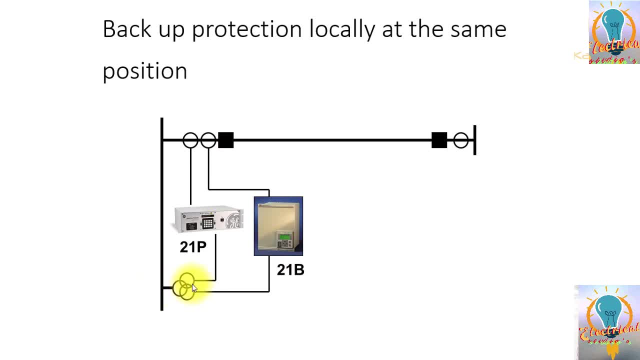 And there is a single VT, Although it has two cores. Two separate cores are feeding to Two different protections. So Each relay has a separate CT VT cores connected. So Let's see What happen If there is a fault occur. 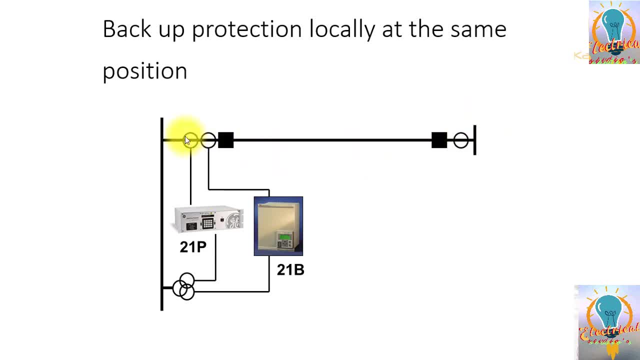 In between these stations. This is one substation, This is another substation And you can see This is the bus bar. So there is a fault here. You can see The fault is sensed by Both relays. Okay, 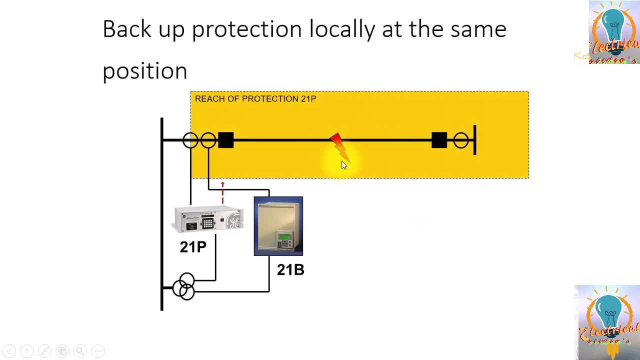 And both relays Have given trip command To this relay. So this is an example of duplicate Protection. So Two distance relays are installed here. Both have Same reach. So Both relays, Both relays, Both relays. 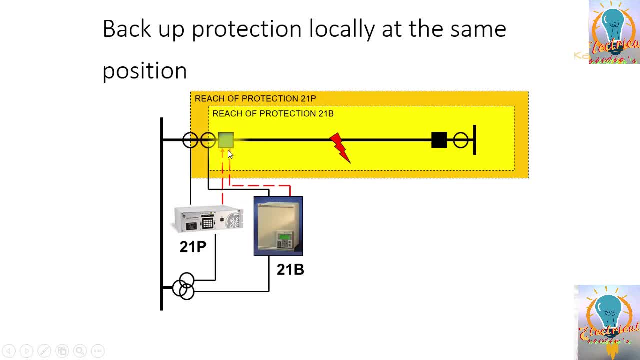 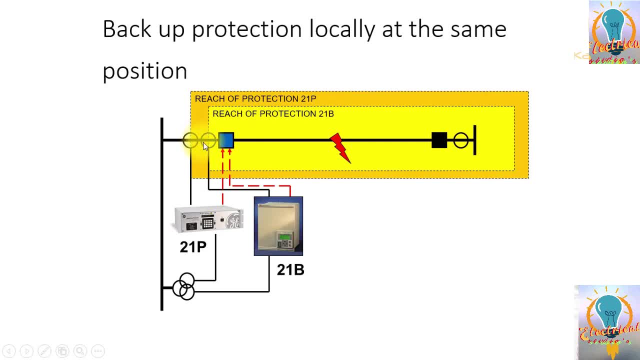 Only one has Same Reach. you can see, Only the difference is The location of CT Cores And Both are Acting to the fault. So This is an example of Backup protection And in this case, 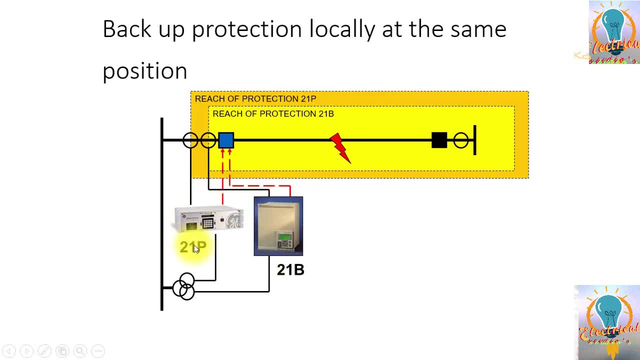 Backup protection is Available Locally, So if One of the protection Fails, Other protection Can Trip normally keep on. the substation is that, apart from the duplicate protection and backup, overprint is also installed, which is backing up these two line protections. 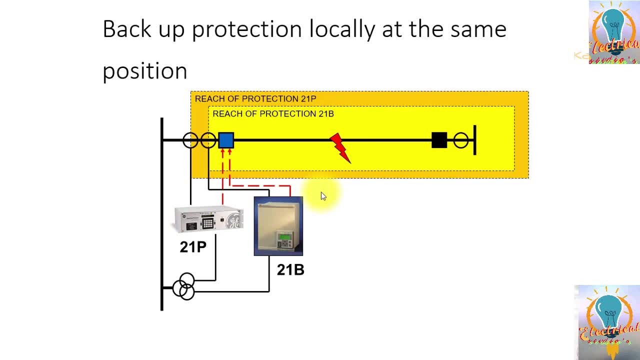 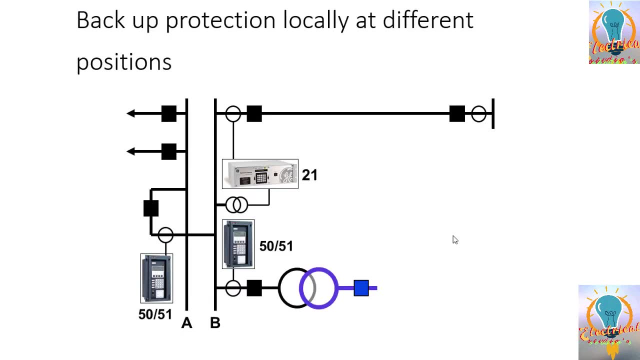 so this is example of backup or duplicate protection at the same position here, friends, now in this section we will see an example where we have backup protection or is installed at the remote locations, at the other locations. so, for example, you can see, this is basically our distance. 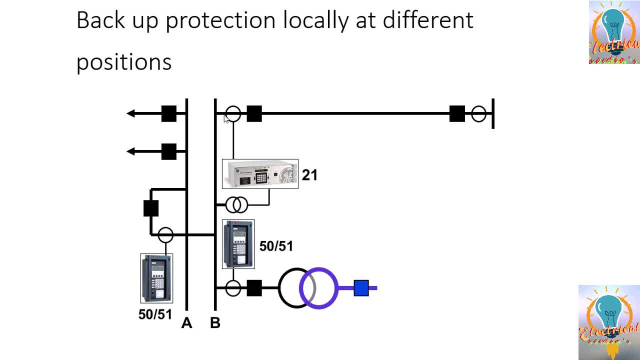 protection is installed here on this feeder, so you can see and this is the substation, so this is backup protection 21 and on you can see, on the coupler, one over control is installed and at transport summer you can see every size and another protection. it's a storm which. 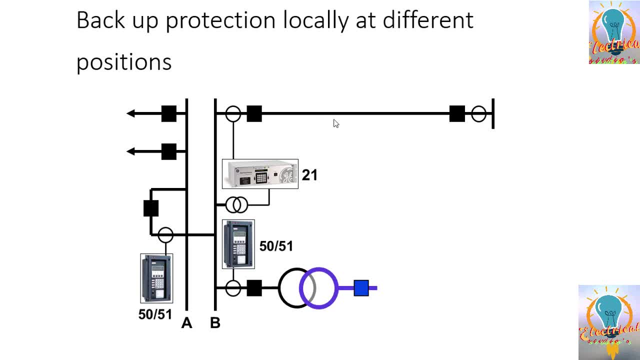 overcome production. so let's see it fall. ofistas in the fall appear here, then this production should operate. so therefore, this is the reach of this progression, is protection. ship it. if you do not care, the coupler will operate the perfect trip going to see, and it will open. the paper goes. stop to stop the. 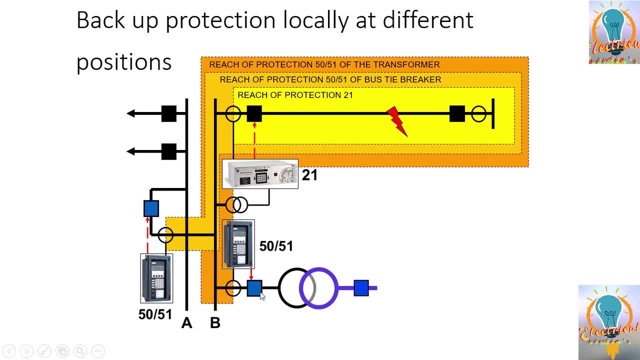 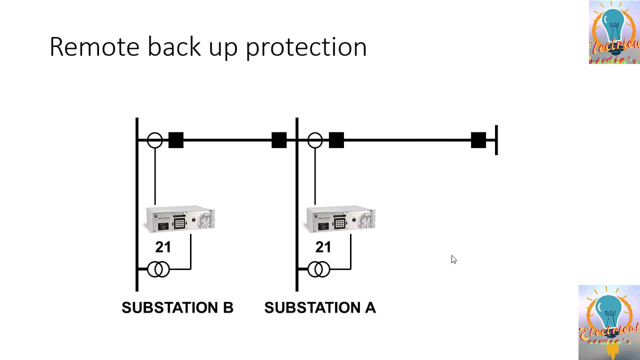 feed, the fall, the other bus, and also this transfer protection will operate. this will try to isolate the fault. so the backup of this protection of this feeder is one relay which is connected at the coupler, another relay which is connected to the transformer side. so this is an example of backup protection here. friends now, 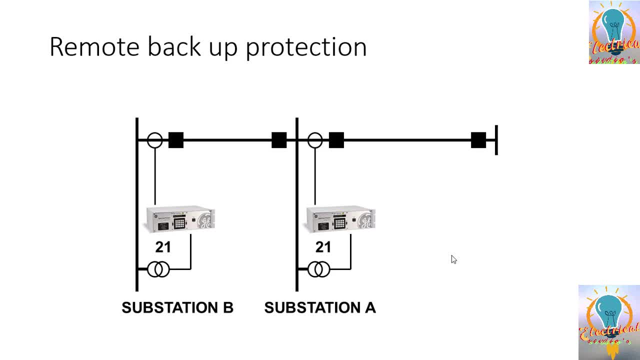 you see that how backup protection installed at remote substations works. so you can see, here we have substations A and Distance relay installed here and at substation B another Distance relay installed and we'll see if there is a fault here. station A: this Distance relay should operate in zone 1, but if this, 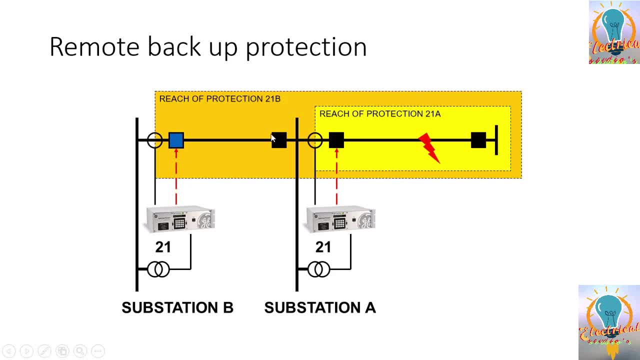 consider case that it failed to operate- the breaker still remain close, then this relay here it will sense the fault in zone 2 and then it will trip the breaker. so this is an example of protection installed at remote. so you can see. this protection should have cleared this fault in zone 1. if it has not cleared, so you can see. 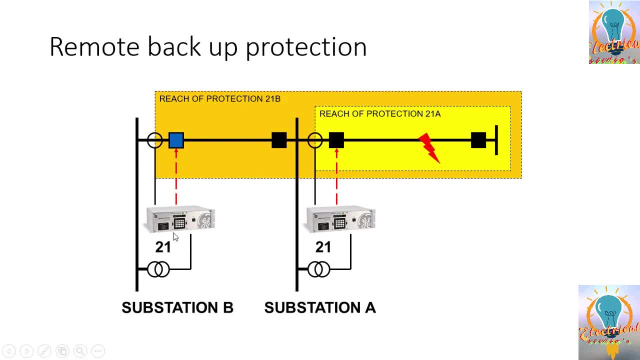 that another protection at the remote end has picked up in zone 2 and after predefined time delay of zone 2 normally, which is 300 to 350 or 400 milliseconds, it will trip and isolate the fault but the disadvantage could be in the remote protection. is remote backup protection is that, if there more 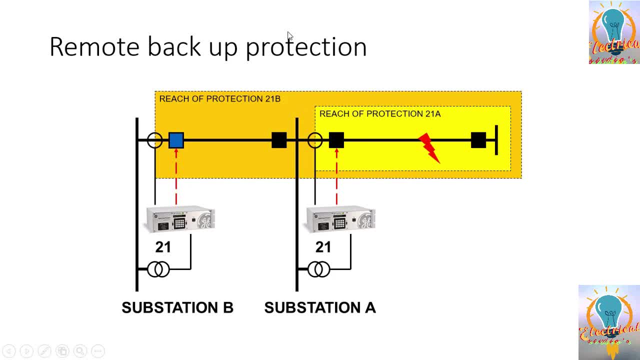 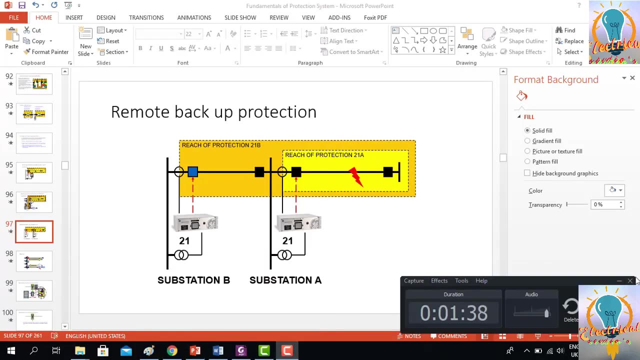 than one sources which are feeding, the fault on more than one sources, then more than one sources can trip on same fault because these all are feeding to this station. this is the disadvantage of remote backup protection. thank you, hey, friends. now we will consider the concept of teletrapping. 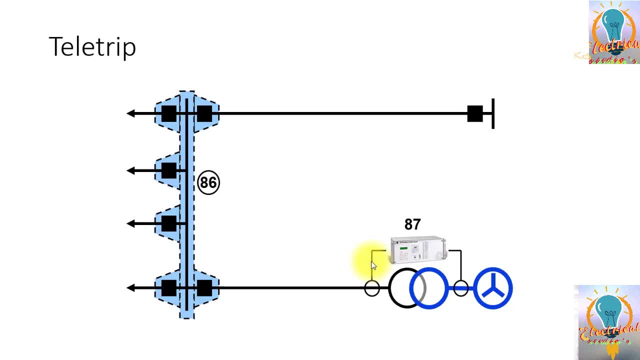 here. you can see, this is basically simple configuration. we have one generator here and we have one transformer which is then feeding to a remote station. the transformer doesn't have any breaker, so one directly cable is feeding and one there is one breaker over here only and we have one busbar and at this busbar there are several feeders which are connected. so let's. 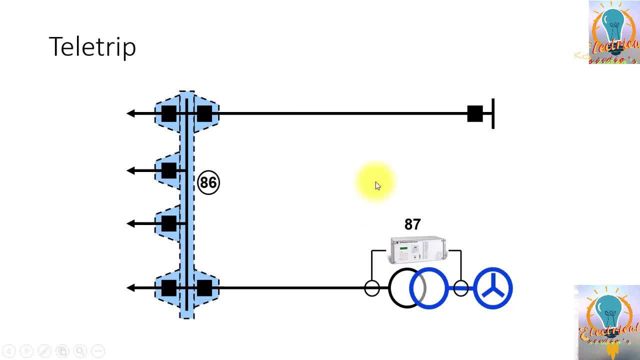 consider the case one. so if there is a fault here, so this relay 87 will pick up, because there is a fault on the transformer. differential has been picked up but there is no breaker to isolate the fault. so it will send a remote trip signal to the remote breaker to isolate the fault and 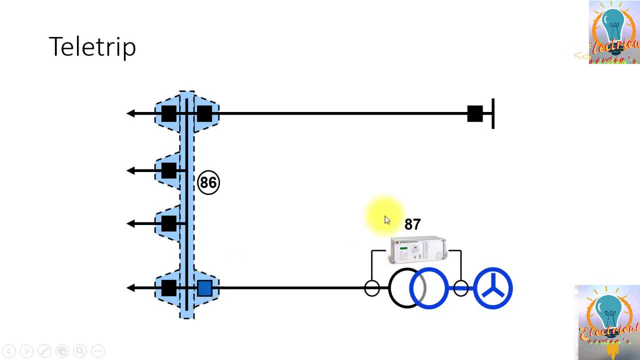 this breaker will trip. so this is example of a remote tripping. so consider the another case. so there is a fault here on the breaker. so if there is a fault on the breaker, then the protection will be above. the protection will operate and this breaker is failed to open. 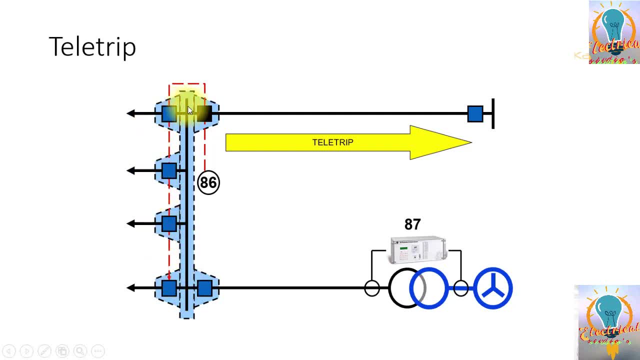 and then it will operate and trip the complete busbar to isolate the fault and also it will send the remote signal direct transfer trip signal to remote end and this remote end breaker will also feed. so if- and the concept is if- there is a fault and the breaker failed to open, all possible. 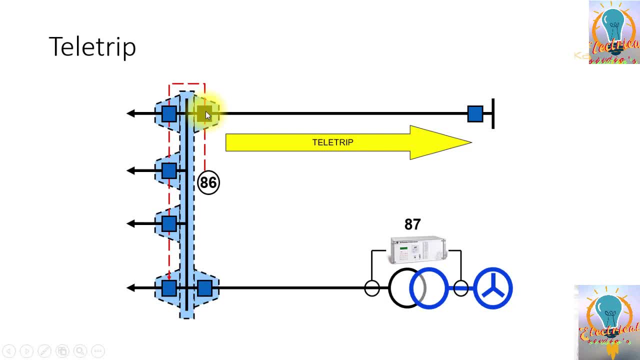 sources which can feed the fault should be isolated. so in this case, these all, all breakers which are connected to the busbar, should be isolated, and then the breaker will be isolated. and similarly, there is one feeder which is feeding the fault for another remote. so this: 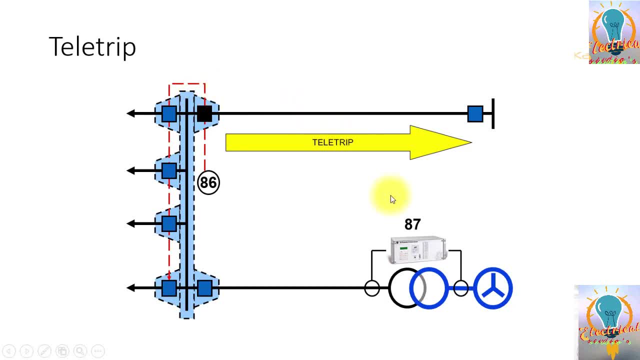 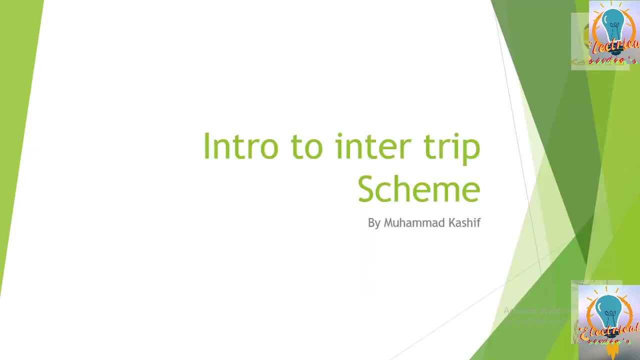 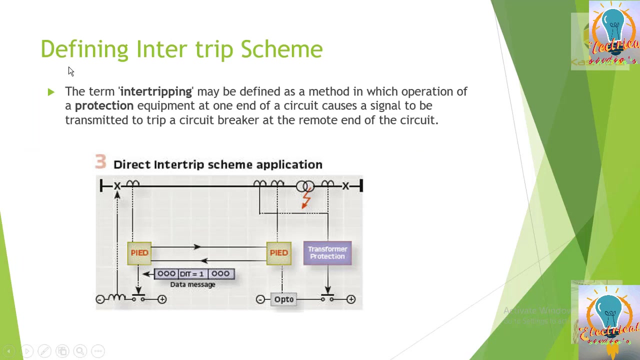 feeder also need to be isolated. so this is an example of teletrip. so i hope you enjoy this concept. thank you very much. welcome guys. now in this section we will just go through the basic concept of 있�rotrip scheme and let's start. we will define the integrative scheme first. the term inter trapping may be defined as method in. 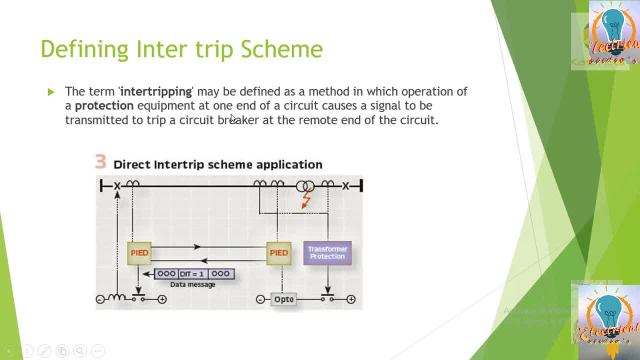 which operation of a protection equipment at one end of the circuit causes a signal to be transmitted to trip a circuit breaker at the remote end of the circuit. so the concept is really simple. here you can see there are two end. you can say this is and a and this is and. 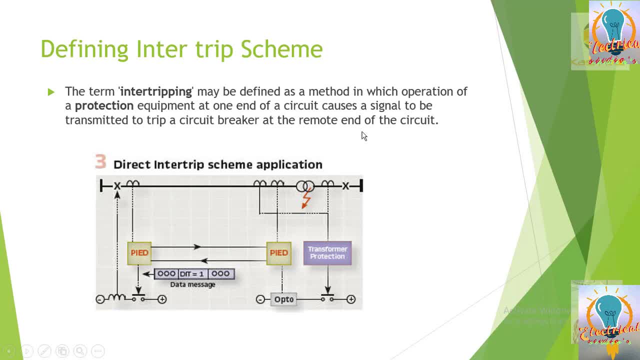 B. so this is substation a. here is substitution D. in this substitution you can see the breaker is installed here on the line and at the receiving end there is a transformer and there is no breaker at transformer. I would decide there is, whereas there is a breaker at transformer- low-voltage. 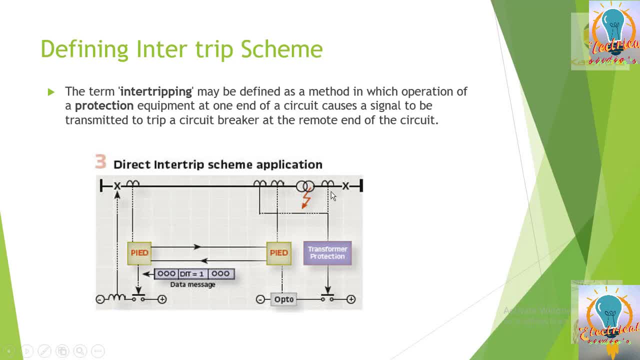 side. so it's very clear now that if there is a fault in between line here or there is a getting here, so when we run the procedure on a surface- which is we allow for its current action and now the next step will happen- we are going to find out that we are going to. 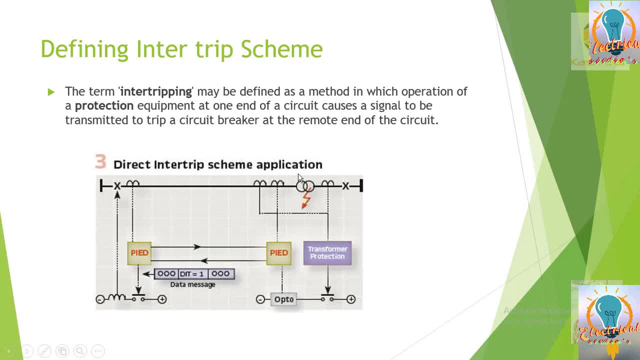 fault on transformer. so in order to isolate the transformer- it's very important that we should be able to isolate it, because there is no local breaker. the tripping has to be sent to the remote breaker and it should trip immediately. so in this condition, this type of scheme is called as direct. 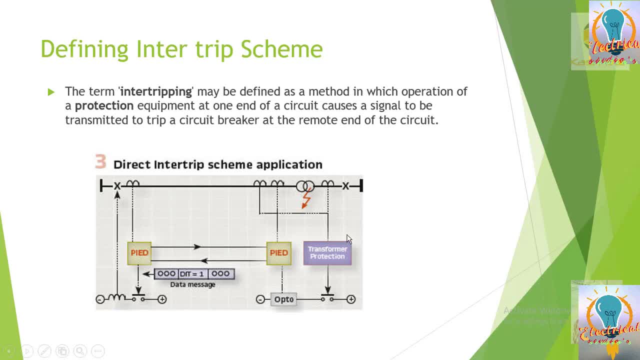 transfer strip scheme. but we will discuss this one in detail. but now the concept: if, if substation A and substation B, it is a foreign substation B and within the end there can be such a condition that if there is a fault, substation B, we, and there is no breaker here, so we want to trip immediately the 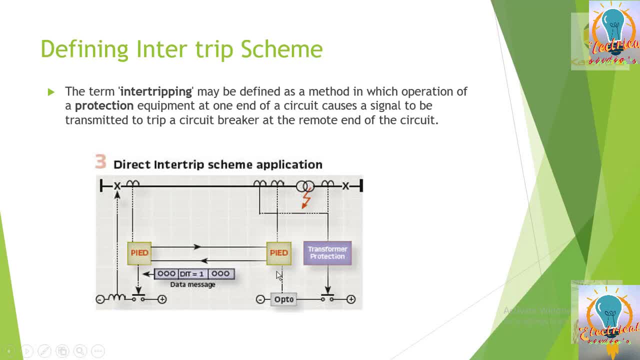 feeding and breaker at the remote station. so through this P IED they will transmit a signal and as far as signal is received it will strip the breaker at the remote end to cut the fault apart. this is the current, so this is basically the example of transfer. 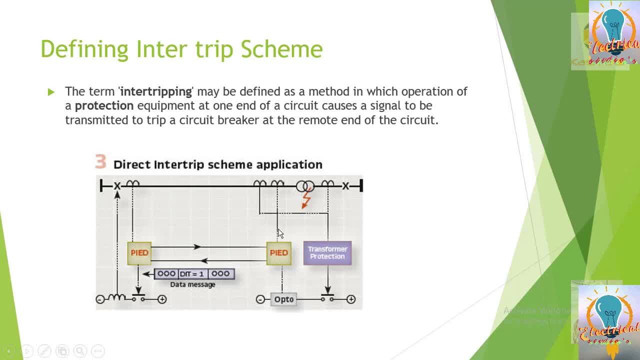 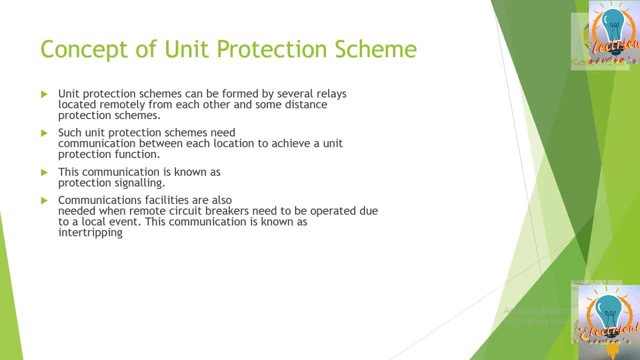 tripping. so it could be in case of a radial feeder, or there are some other applications we will study. so concept of unit protection scheme: your unit protection schemes can be formed by several relays located remotely from each other and some distance. protection schemes- protection schemes need communication between each location to achieve a unit protection function. 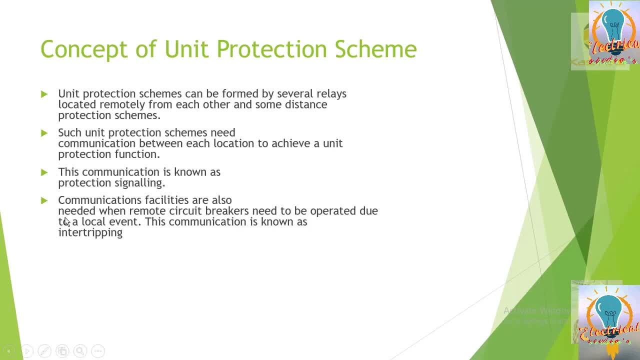 this communication is known as protection signaling communication facilities are also needed when remote circuit breakers need to be protected, operated due to a local event. this communication is known as intro trapping. so these are the basic definitions that we have learned. basically, um unit production scheme is the protection scheme. 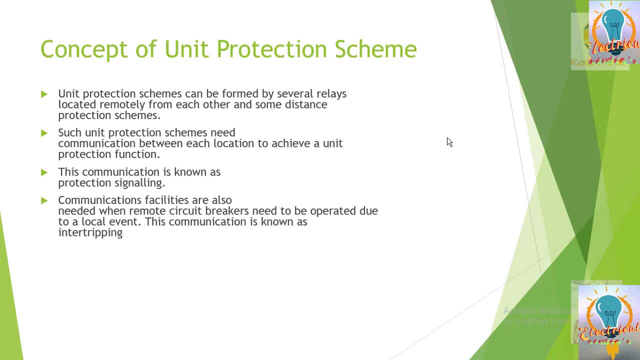 in which, uh, it is um, when there is a fault on a unit, for example a transformer, it's our unit line, it's a unit, it's. it is tripping the feeding sources or stripping the breaker at the same time. so, whereas in the grid production scheme, tripping is done. that we will learn later on. 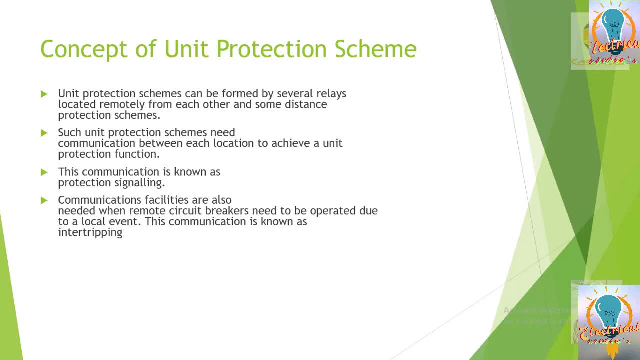 tripping is is not done as per unit but it's as per grade. for example, if you have, as you have seen, there is a 400 volt incomer breaker and there is an outgoing breaker. so if there is a fault in organ breaker first out and recover trip. 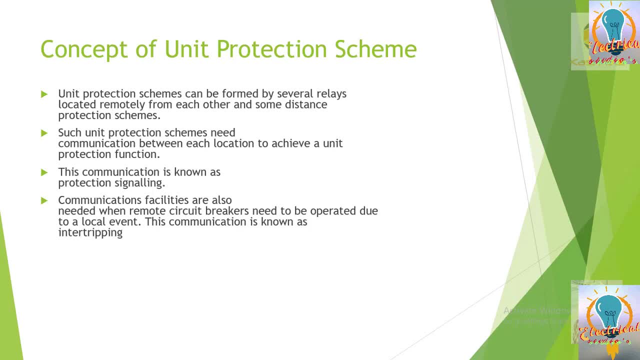 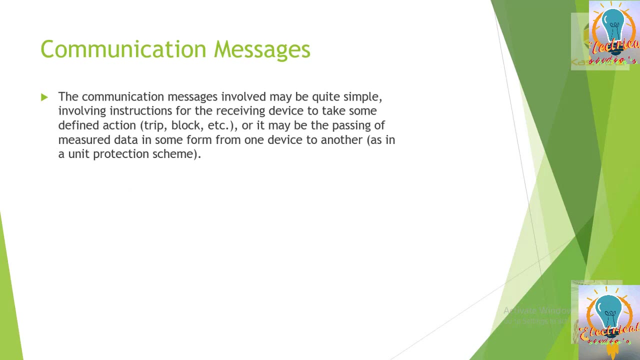 if tripping is not, uh, successful, then income or will trip. this is kind of a great creating graded protection. so we will further learn later that what is the unit production and what is the grid protection? so communication messages. the communication messages involved may be quite simple, involving instructions for receiving device to take some defined action: tripping, blocking, etc. 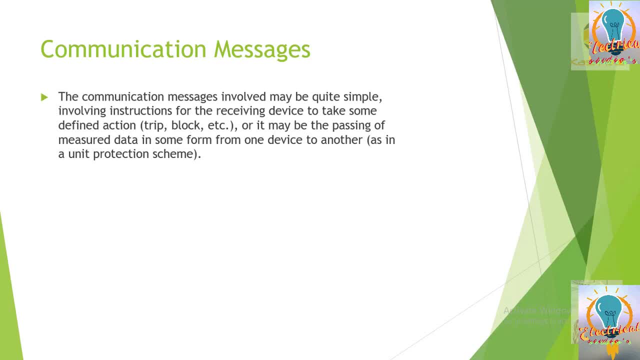 or it may be the passing of major data, in some of the form, one device to another, as in a unit production scheme. so communication messages. so you want to send communication messages. it is not necessary that it will send a tripping, it could send through a communication medium. 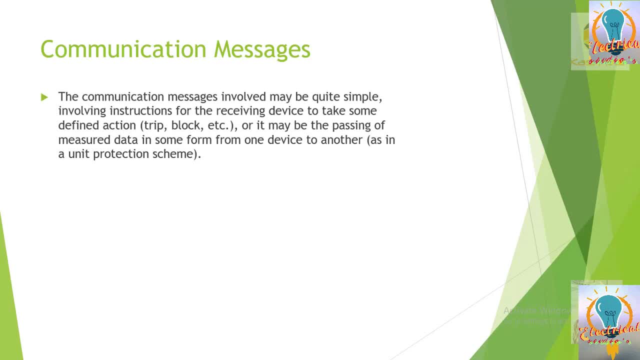 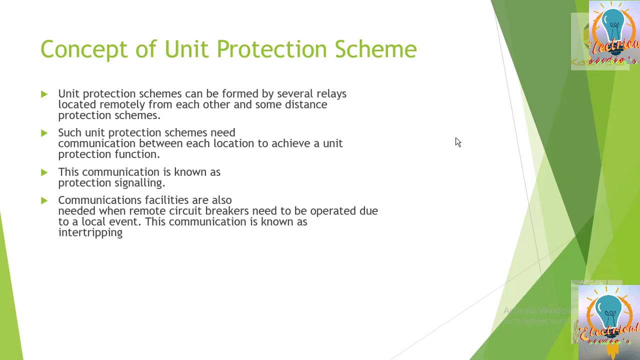 trip signal, a blocking signal, unblocking signal in some cases, like line differential production, it is sending the signal of measurements, like how much current at one end, another one and both currents are communicated. so these are example of communication messages. so this we will discuss in detail. so so far we have understand what is the concept of unit production in this section and in detail we 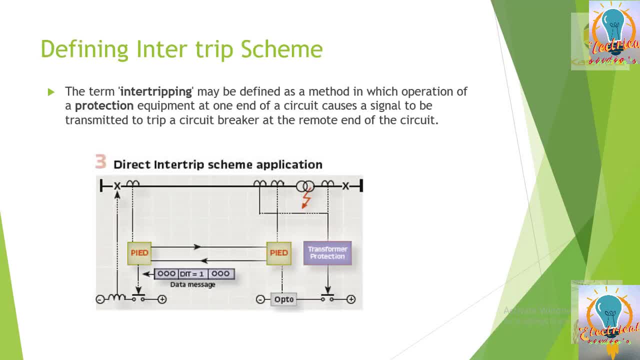 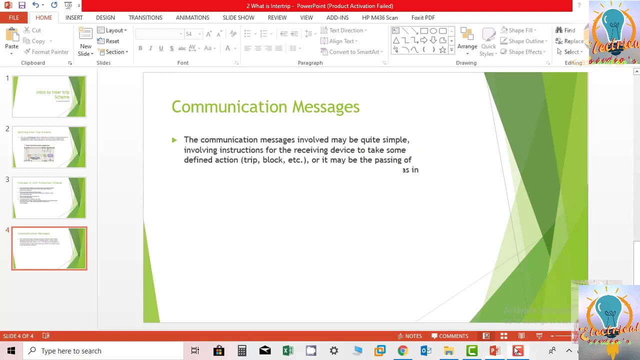 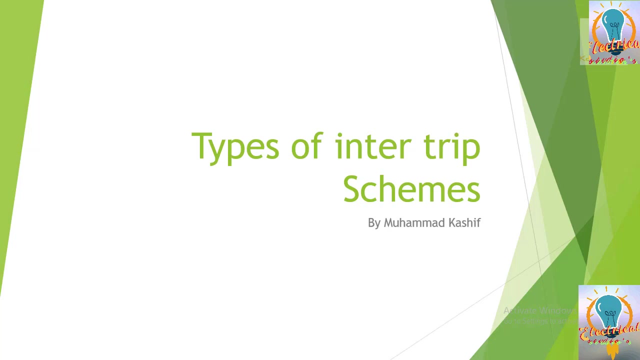 will give you the concept of graded production. we have understand about what is an interactive scheme and we have understand one example. there are several examples that we will study in the next section. so thank you very much, welcome friends. in this section we will study, uh, the detail and types of interactive schemes. 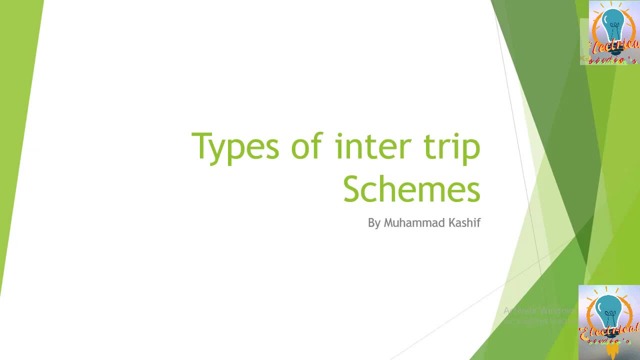 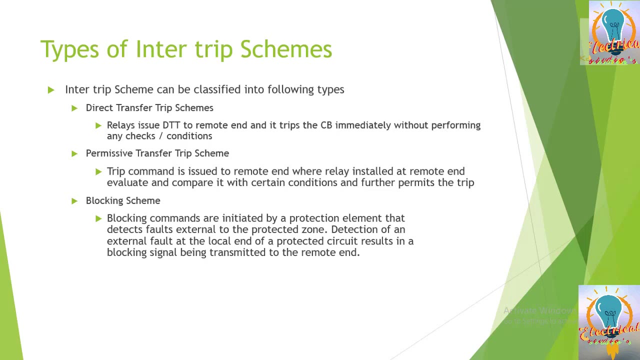 and we will discuss the basic types. so it is intro. trip schemes can be classified into following types: direct transfer tip schemes. in this scheme the relay issue trip dgt. direct transfer trip command to remote end and it trips the circuit breaker immediately, without performing any checks or 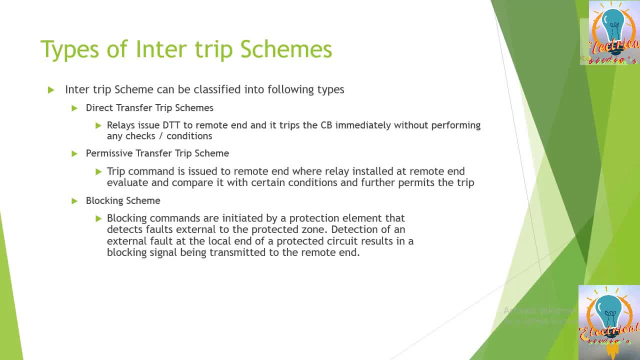 conditions: permissive constant trip scheme. trip command is issued to remote end where relay installed at remote, and evaluate and compare it with the certain condition and further permits the trip blocking scheme. the blocking commands are initiated by a protection element that detects fault external to protected zone: detection of an external fault at the local end of a protected circuit reserved in a blocking signal. 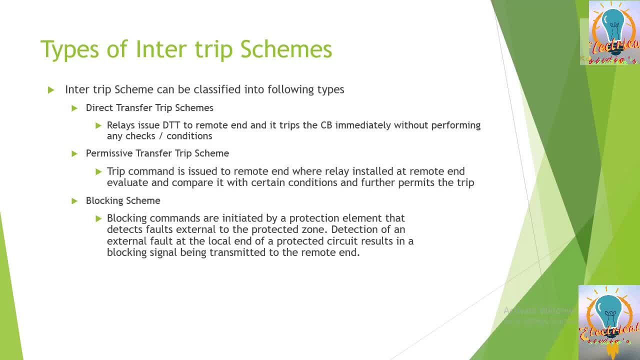 being transmitted to remote ends. so there are three types of basic protection schemes. one is a direct contraceptive scheme and in this scheme the remote end trip to the existing location and the remote end trip to the state at the remote end of the station, to the remote end to be send directly at. 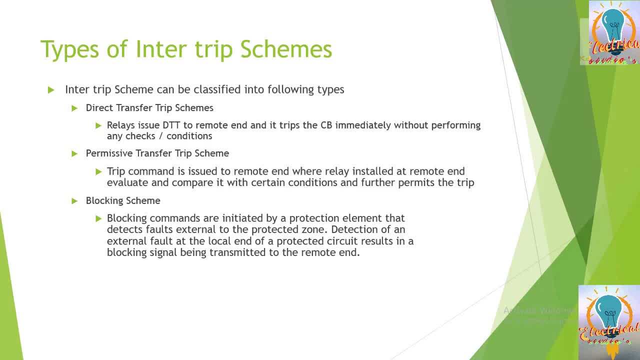 one end, for example station a, give tip command to the station b at remote end and the remote end trips immediately, without making any logical decision or without evaluating any local conditions, trip at the local and we will discuss in detail later when we will discuss this permissive scheme, that local, and will evaluate certainly the local conditions. 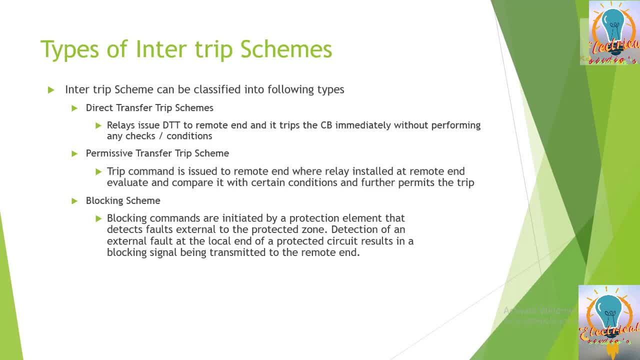 that must be fulfilled in order to release the trip signal at the remote end. so another type of scheme is blocking scheme. so in permissive scheme relay is waiting for permissive command from the remote end, whereas in the blocking scheme the relay is always ready to trip unless it receive the 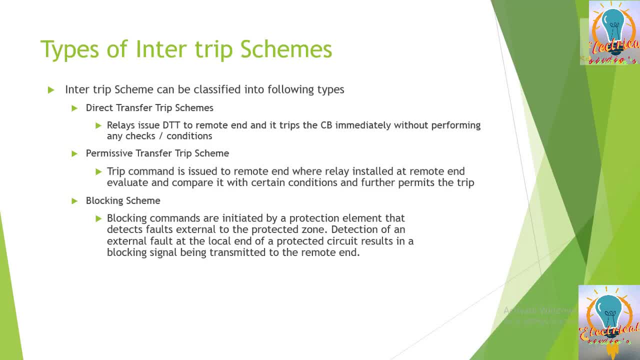 blocking signal from the remote end. so it could also be if you just apply a NAND logic or inverse logic, it could also be unblocking scheme. this is another type that we will discuss in detail. so these are some types of iterative schemes we will discuss in the next video. 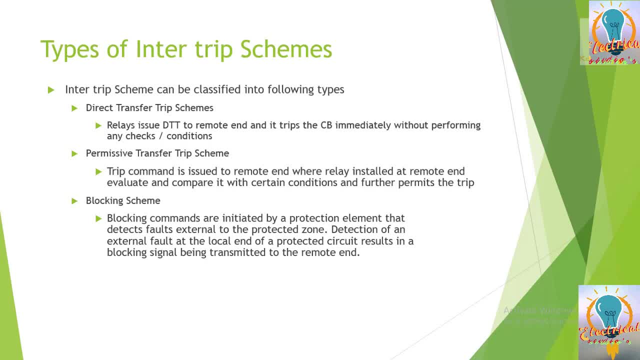 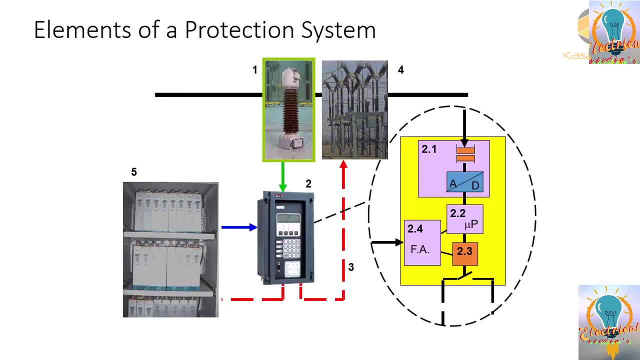 go through the schemes one by one now. thank you, hi friends. in this section we will go through briefly two different elements of power system, how these elements are connected and how these elements are operating. so here you can see, there is an current transformer and this current transformer is feeding this overcome relaythe series. second is 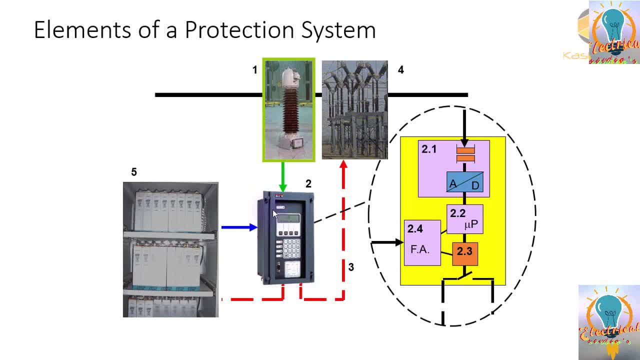 せて to this relay, so the relay can sense the current in the line. similarly, this way is power up from a DC bank, so AC supply. you know it can be failed on a substation and there is no backup of AC supply, so it's easier to convert AC into. 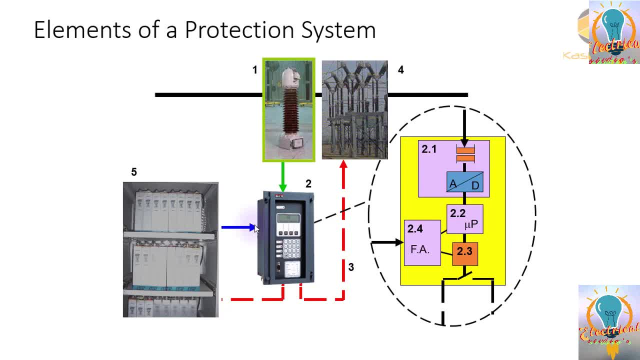 DC through a DC charger and at the same time this DC supply will be connected to all the control and protection system in a substation. and also this DC supply through charger will be used to charge the batteries and when the supply is supply fails, these batteries can supply the DC supply to. 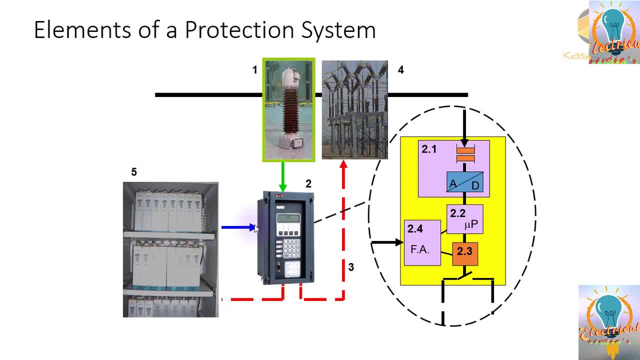 the control and protection systems to operate. so that's why you will find a battery bank in each substation or power plants. similarly, when relay gets the input quantity, it compares this input quantity with a pre set value. first of all, when the input is connected like a current, there is an analog-digital converter in each. 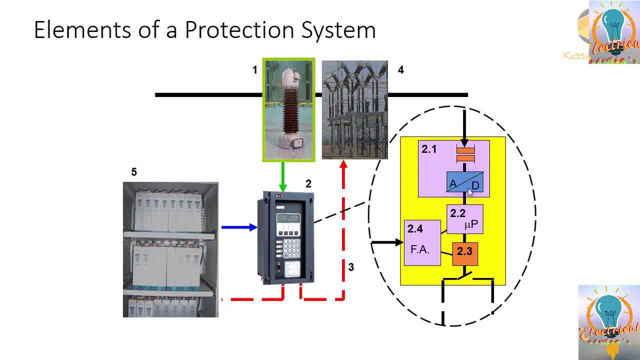 protection number equal relay. it converts thePod board 's, the quantity from analog to digital and then its used in all computation microprocessors in the relay. so relay compares the measured quantity with the set value. for example, if it is a over current relay value is if 1 ampere and if the measured quantity is 0.5 ampere, relay will not. 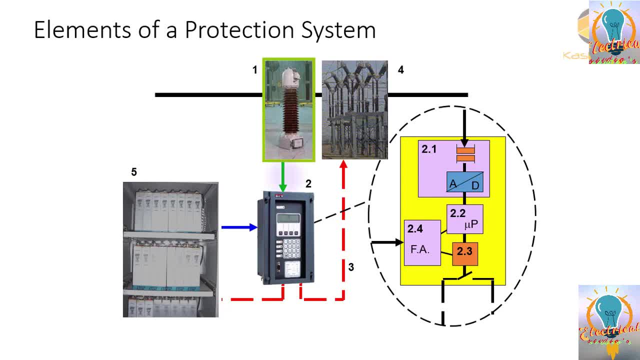 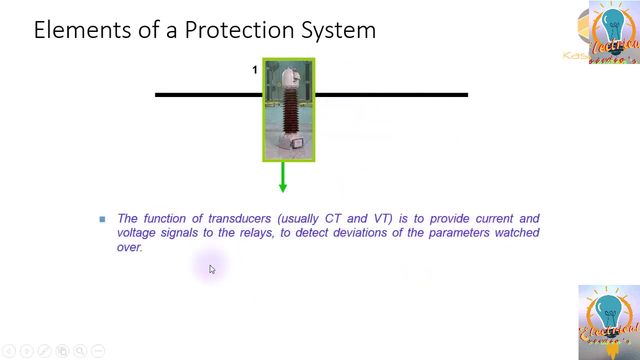 pick up and relay will not issue a trip command. but if the value measured value is more than 1 ampere, the relay will pick up and it will issue the trip command and then it will operate the breaker which in turn will isolate the fault. so this is a brief description that how the protection system works. so 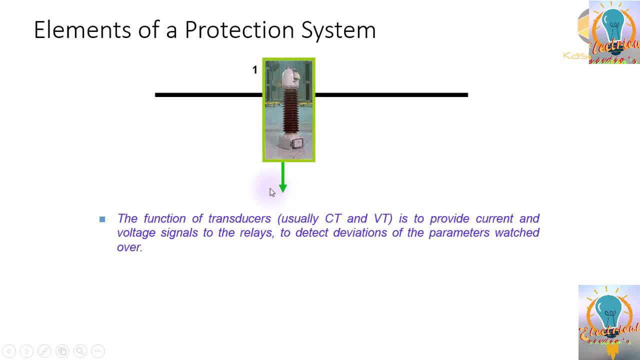 you can see, this is the item number one, which is a current transformer or voltage transformer. the function of transducer, usually CT and VT, to provide current and voltage signals to the relay to detect deviation of the parameter washed over. so CT or VT current transformer, voltage transformers are 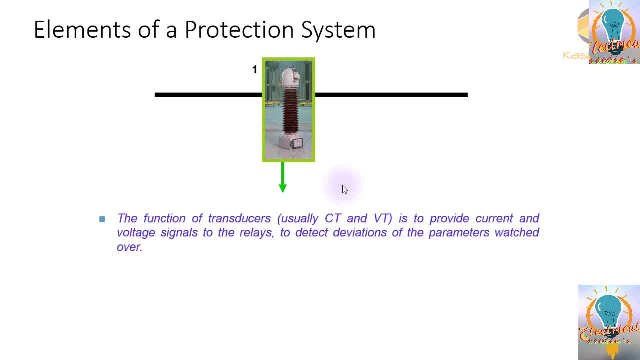 basically you can see I and I's and ears of the substation, so these these are connected to you are basically you can see I and I's and ears of the substation, so these these are connected to. so these, these are connected to relays and the relays are measuring the data from, measuring the quantities and 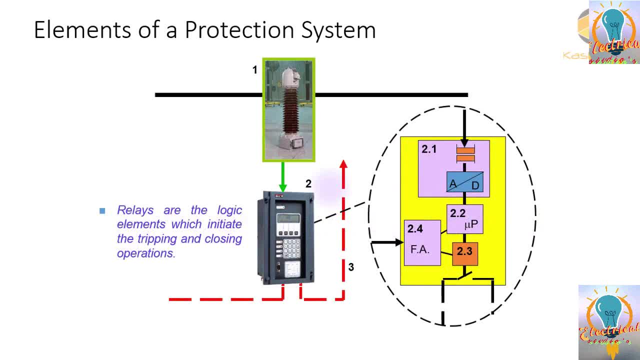 then they are making final decisions. so here you can see this CT and VT is then connected to the relay. it's an input. output from the CT is connected to the input of the analog input of the forward current relay. so relays are the logic elements which initiate the tripping and closing operations. so the relay is 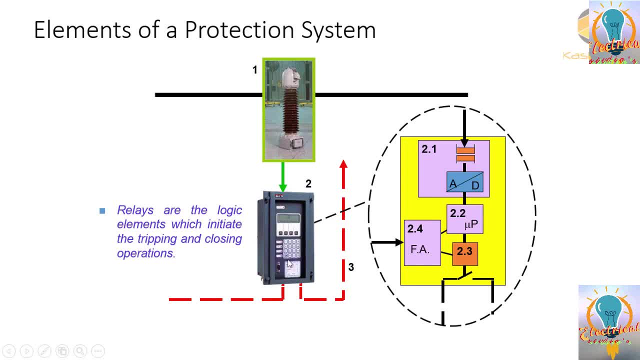 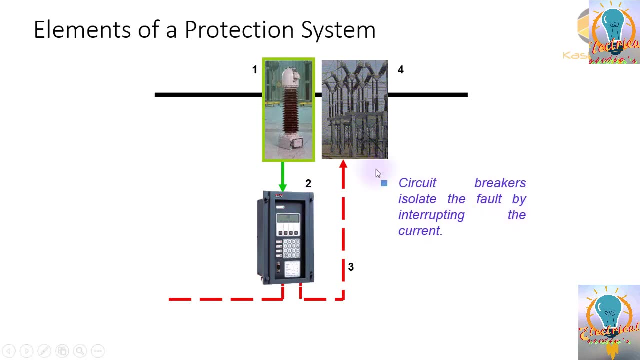 basically have the power to initiate the tripping. and there is another relay which is called auto-recloset relay. it can also do the auto-reclosing, so circuit breakers isolate the fault by interrupting the fault current as soon as relay senses that value is more. 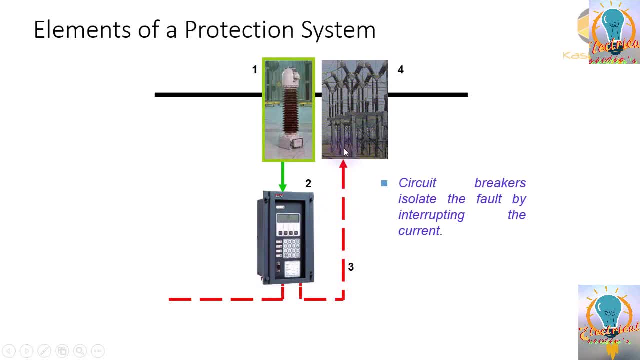 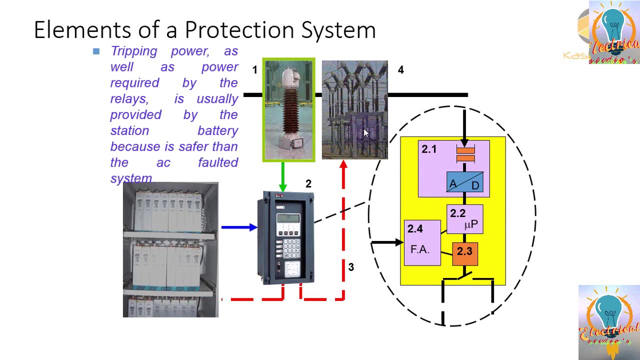 than the set value. it issues a trip command after predefined time delay and then it's giving trip command to the circuit breaker. circuit breaker and in turn the contacts of circuit breaker opens and it interrupts the fault. current tripping power, as well as power required by the relays, is usually. 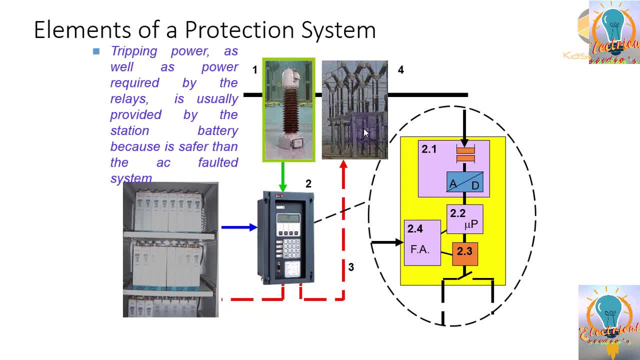 provided by the station batteries because it's safer than the faulted system. so each system you will find that each substation is feed from the DC power. so this was a little introduction again to brief you that how the system is integrated and working. I hope you enjoy this. thank you very much. 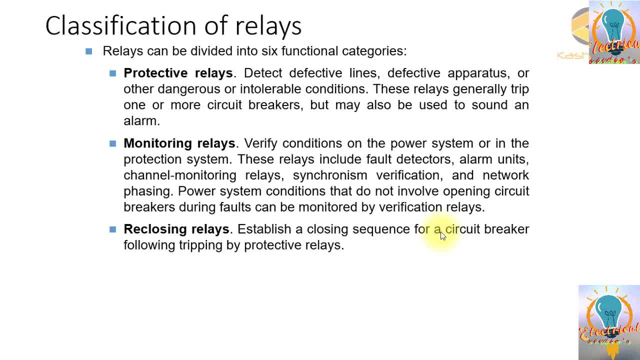 hey friends, in this section we will study about how we can classify different production relays. so production relays can be classified by different ways. so we can classify as a protective relays, as monitoring relays, as the reclosing relays, so protective relays, basically direct fault currents. 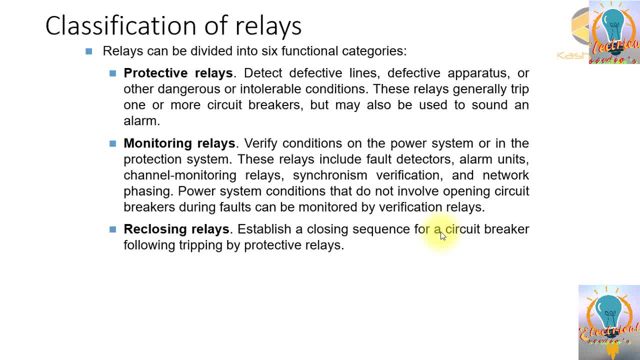 and it detects a defective operators. they are monitoring the dangerous, intolerable condition. these relays generally trip one or more circuit breaks but may also be used to sound an alarm. so example of protection relays are like we have on the line. we have a distance protection and the ANSI code of this. 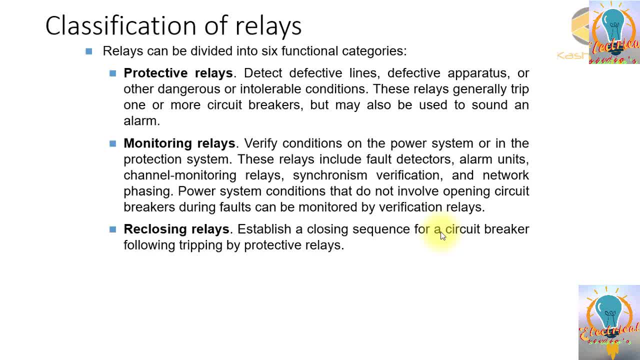 operation is 21 and we have a backup over current protection, inverse time or definite time. we have over gain, earth watt protection, we have over under frequency protection, over excitation protection. there are a lot of relays because, because these, all of these relays are named, as you can see, as an protection relays. 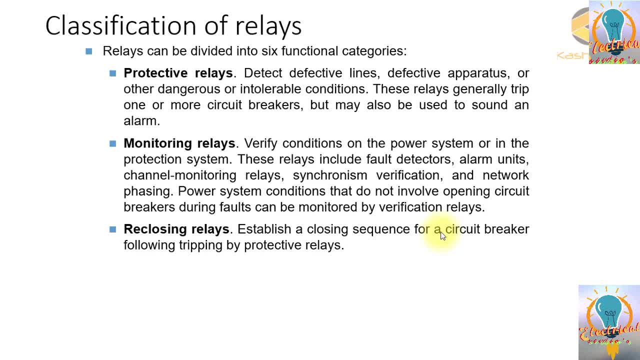 second type of relays are monitoring relays, so we are basically verifying the conditions of the power system in the protection system. these relays include, like of fault detectors, alarm units, channel monitoring relays, synchronism verification and network phasing phase system conditions that do not involve opening circuit breakers during the operation of the system. and 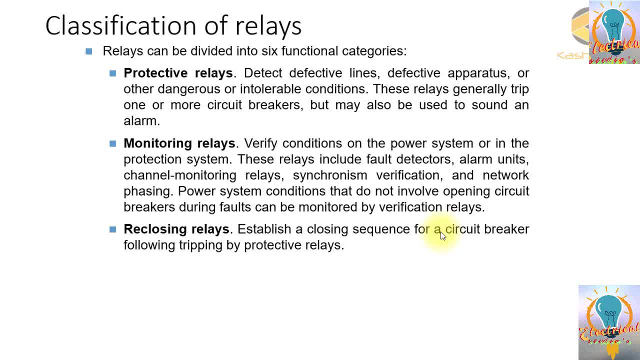 faults can be monitored by verification relays. Monitoring relays. example is, for example, for the GIS. we are monitoring ethics or the transformers. we are monitoring the winding and oil temperature all the time and we are initiating the alarms. and even the trip is initiated, then buckles relays also. 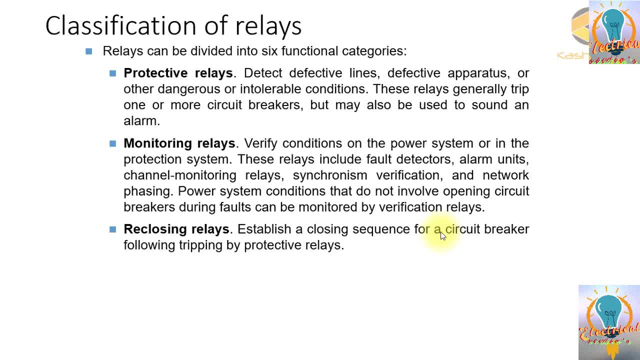 installed in the transformer which is monitoring the, any gas which is produced inside the transformer. so in SSX circuit breaker, SSX is monitored. so these are all example of monitoring release. so another type of relay is reclosing relay. these are called as譬for example after recloser, if there 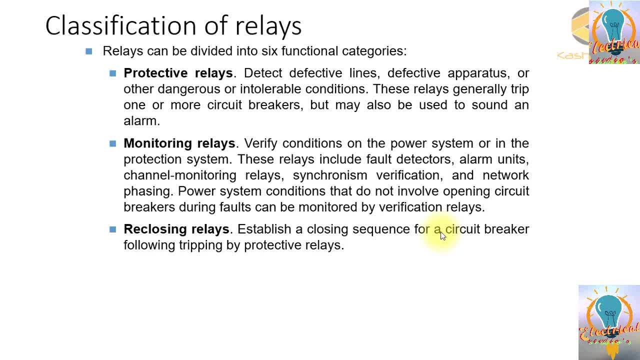 is a fault and offer temporary nature, then after recloser tried to reclose after dead time and then if it is multi-shot, then reclaim time is run and time is if the fault reoccur in reclaim time. if it is a single shot, then the second time breaker will not close. if reclaim time is passed and the breaker 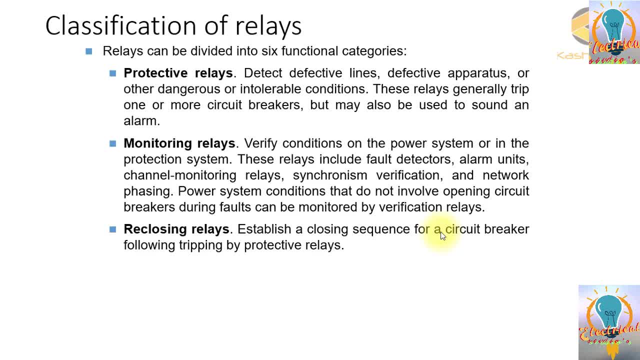 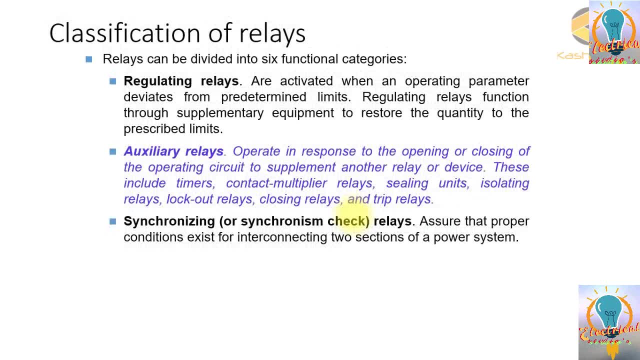 is declared as successful, then if the fault occur it will consider as a new fault. then we have classification of release like regulating release. for example, you can see there is a AVR automatic voltage regulator installed on the transformer tape changer. so the function obviously is to regulate the secondary voltage to 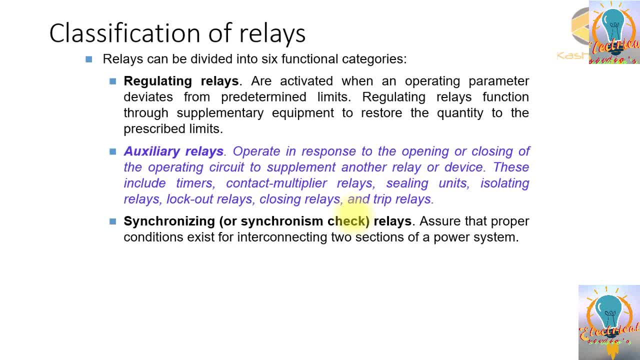 maintain the voltage. so this is example of an regulating relay. so recruiting relays are activated when an operating parameter deviates from predetermined limits. regulating relays function through supplementary equipment to restore the quality to the prescribed limits. so example: I have already told you that there is a automatic voltage. 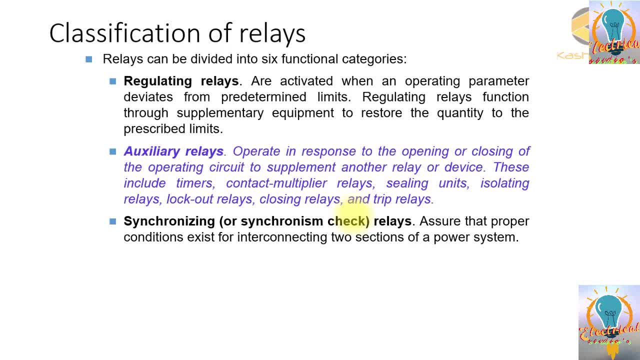 regulating relay is called as an AVR relay, and this relay is installed on the transformer and when and they, then a predefined bandwidth is defined. for example, if the voltage change more than the preset value, 1 kV or 2 kV, then the tape changer will operate and will try to bring the voltage within the limit. so 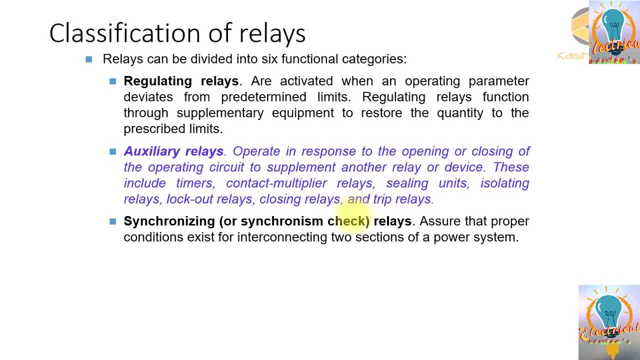 another type of relays can also be classified as auxiliary relays. so these relays operate in response to opening or closing of operating circuit to supplement another relay or device. these include timers, contact multiplier relays, ceiling units, isolating relays, lockout relays, closing relays and trip relays. so auxiliary relays, we have gone. 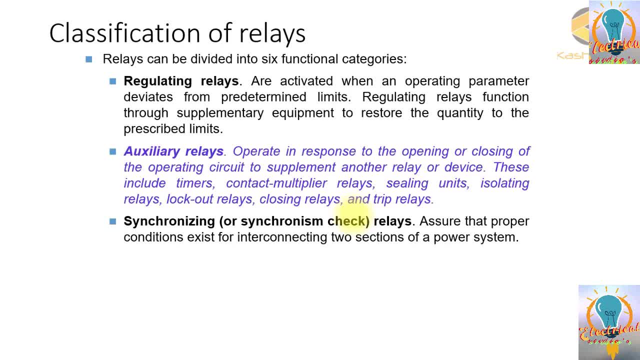 through this already in our training. so these are small relays that you will find in the substation. so for contact multiplication and for making a timer circuit, for interlock circuit, you will find all these relays. then we have synchronizing relays. these relays basically check the 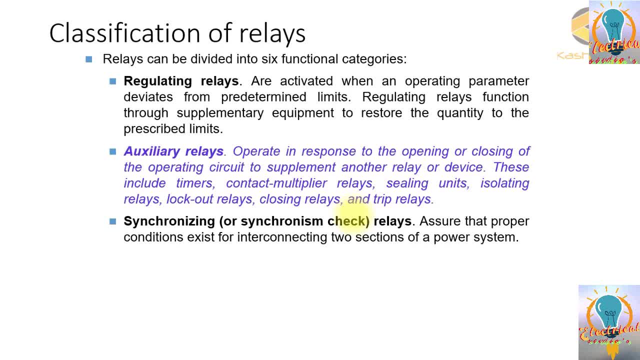 synchronous checker function. the code of for this relay and C code is 25. so what the relays they are checking? the Delta V difference of voltages, Delta F difference of frequency, Delta Phi difference of angle between two sources that need to be connected. so if condition permits, then the synchronizing relay is: 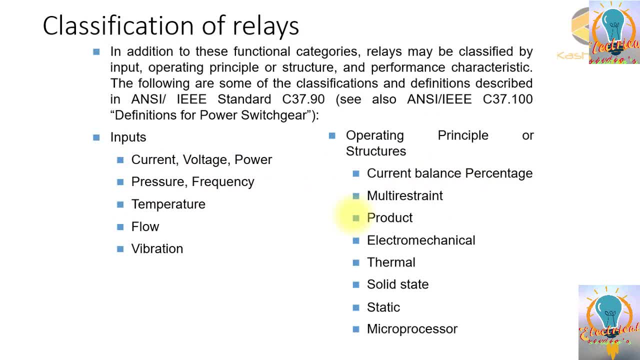 the one that will allow breaker to close. so this basically classification of relays. so in addition to this function category really may be classified by input, operating principle or structure and performance characteristics. the following are some of the classification and definition described in NC IEEE standard C 3.90. so on the basis of an input, we can classify relay into either: 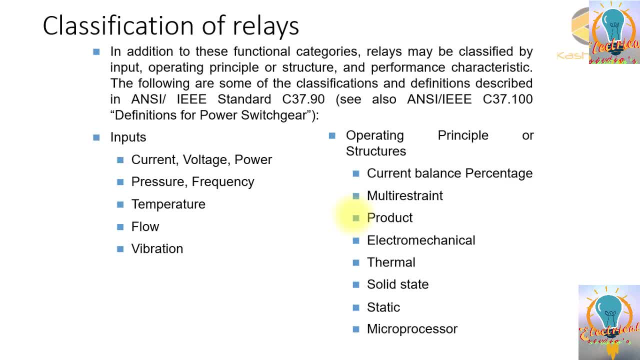 current voltage and power and current voltage and power release, pressure release, frequency release, temperature release, flow release or vibration release we are. we can also classify the released based on their operating principle or structure, just like current balance protection, multi-restrained, really product, really electromechanical really. carbon, really solid state, really statically, or microprocessor really. 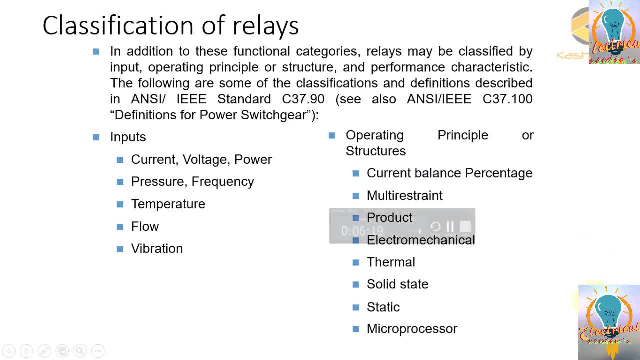 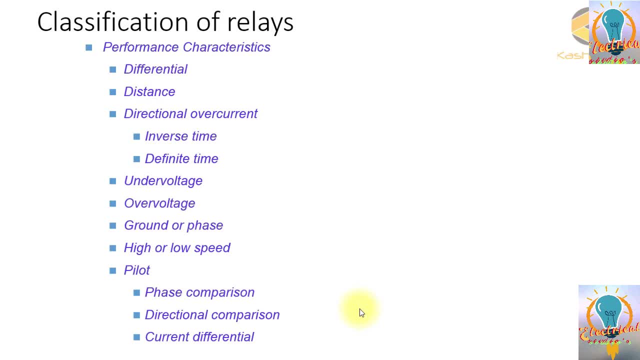 so the further classification of release can also be done by performance characteristics, just like differential, distance, directional, overcurrent, inverse time and definite time under voltage relays over voltage relays, ground or phase over current relays, high or low speed release, pilot protection, phase comparison, direction comparison, current, differential. 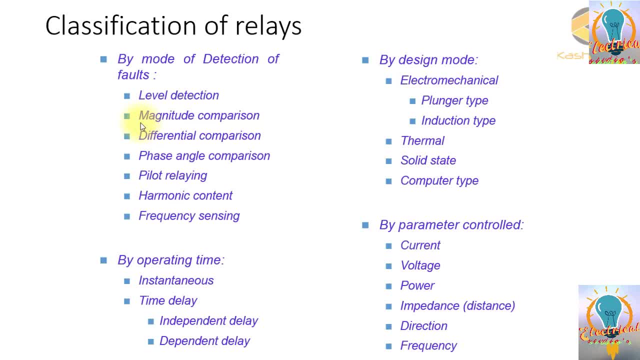 we can further classify the relay by mode of detection of faults, like level reduction, magnitude comparison, differential comparison, phase angle comparison, pilot relaying, harmonic content, frequency sensing. we can classify the relays also by operating time, like instantaneous relays, time delay relays, independent relay and dependent relay relays by design mode. 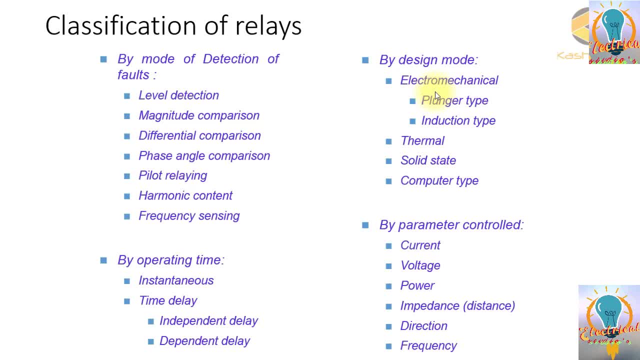 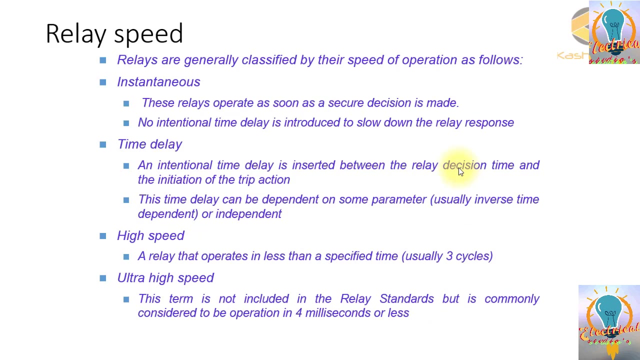 electromechanical plunger type induction. disk type thermal relays. solid state relays, computer-based, released by parameters control like current voltage, power impedance or distance, moisture, frequency, standen from the speed point of view. if you can divide and classify the relays as follows: instantaneous release: these relays operate as soon as secured decision is made. 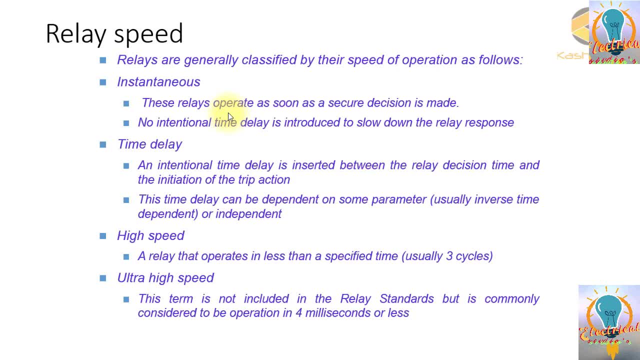 so instant relays don't have any time delay, it operates within no time. so like example of instantaneous operation is zone one where we call the word data keep their time to zero. the second type is time delay relays. an intentional time delay is inserted between the relay decision time and the initiation of trip. 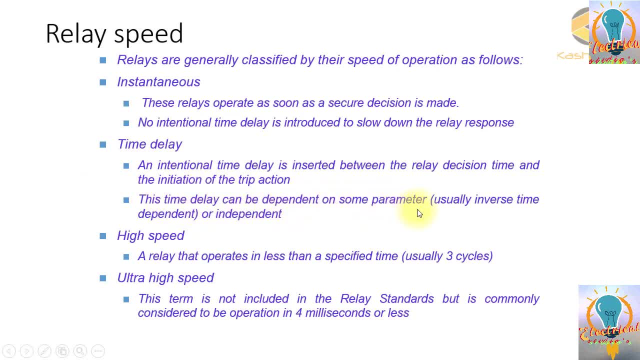 action. this time delay can be dependent on some parameter, usually inverse time dependent or independent. so time delay relays are examples are. inverse time relay is example of a time delay relay and definite time relay is also example of a time delay relay. so if you're talking about a distance zone, one is: 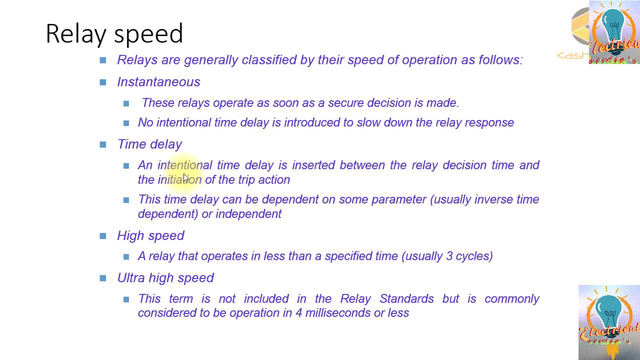 instantaneous, and various zone two and three are time delayed. so then we have a high speed relay. a relay that operates in less than a specified time- usually three cycle- is called as a high speed relay. then we have an ultra high speed relay. this time is not included in the relay. 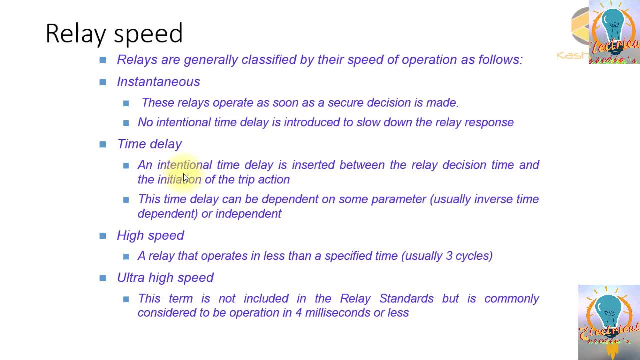 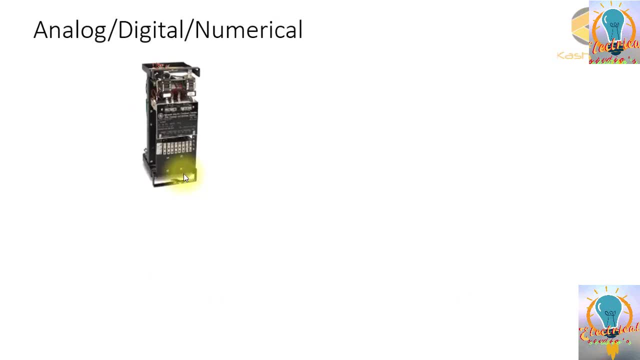 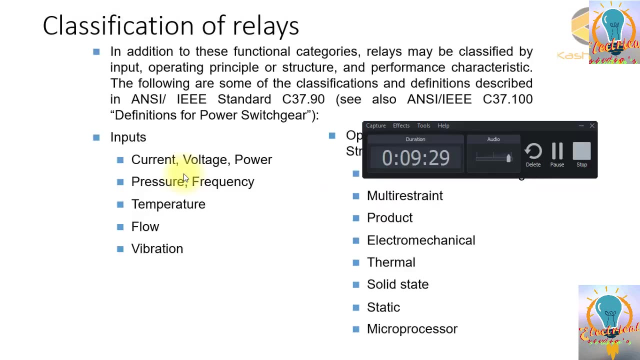 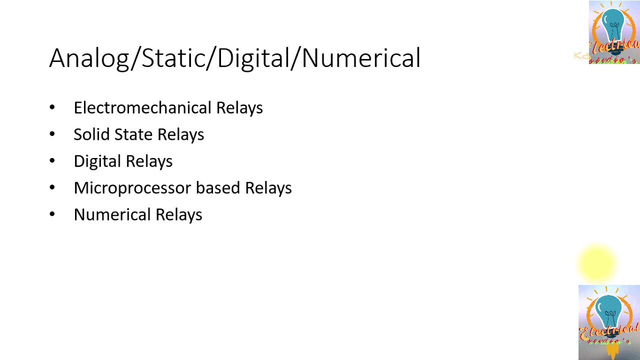 time relay, but it is commonly considered to be in operation in four milliseconds or less. so these are some relay classification as per speed. so I will conclude my this section. thank you very much. so now we will see and how the protection relays are modernized, how, how used to be the old protection relays. 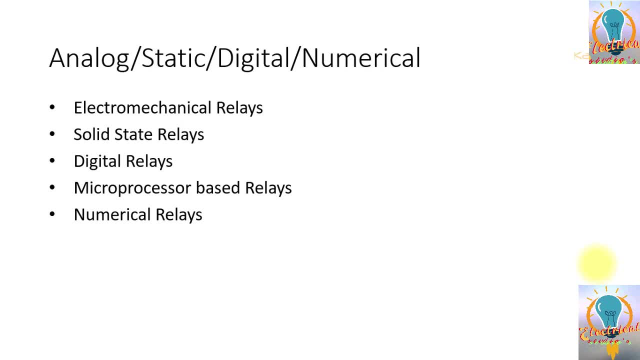 and in the start of the production era the old protection relays used to be very bulky, big in size. you will see especially really black in color with the with a transparent glass you can find relay inside and these are called as an electromechanical relays. the size of the added piece that I have seen is 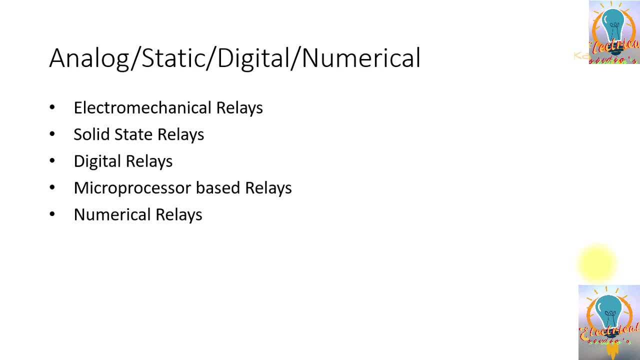 one of the very old relays that was installed is in I think nineteen eighty I think, and one of the very old relays that was installed is in I think nineteen eighty-three times in 500 kV. Jamsher was LHV and you can see the size of this relay is. 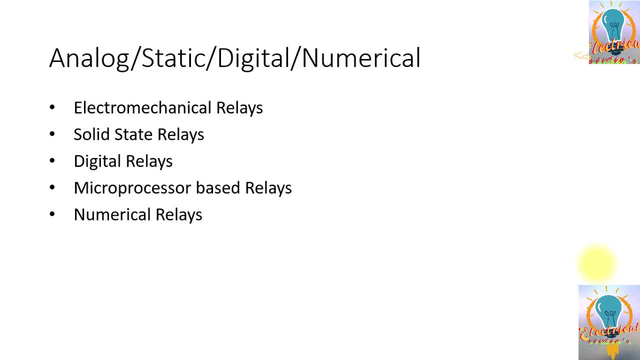 half of the cupboards. so it's a very big and bulky relay. so I can see in the relay each element separately, like you can see zone 1 element, zone 2, zone 3 elements separately. you can see a starter element. so when starter pick up you can see the starter. 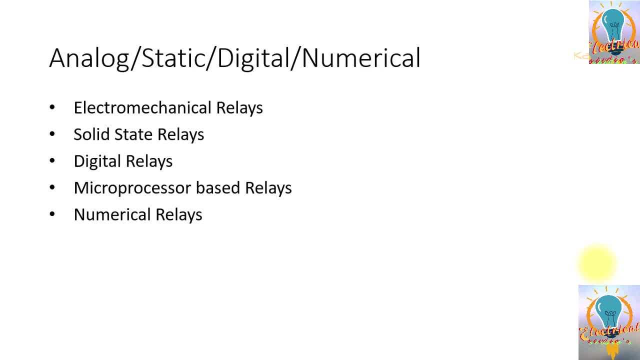 physically you can see switch on to forward element and you can see over current elements. so you can see all the elements, all the comparators, voltage and current coils. you can, if you want to try, you can locate, you can see the physical timer in these relays. so this relay, 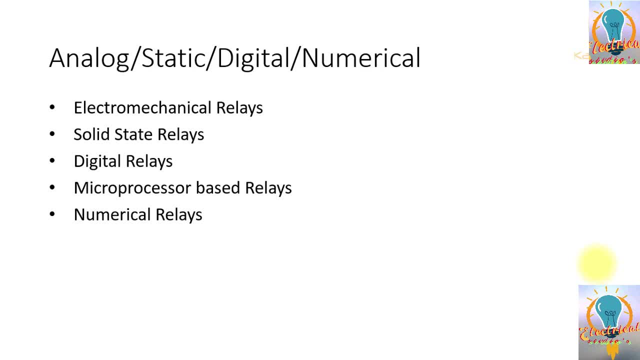 name of the relay was LHV and this relay was. I came to know this relay was made by jointly by electrical engineers and the jewelry makers in Switzerland, so it's basically a brown bovary relay. later on there is another basically big company named ASEA have a merger with brown bovary and both 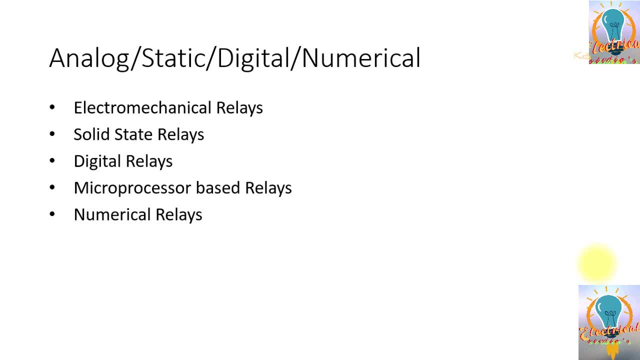 combined and they make another company, ASEA, brown bovary, and which is very famous. now it's called as ABB, so older. you can find the older relays from ASEA and brown bovary separately, but all these relays are bigger in size and We are in this לז. this is the 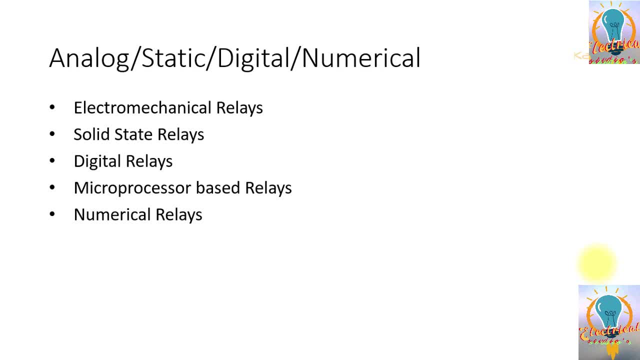 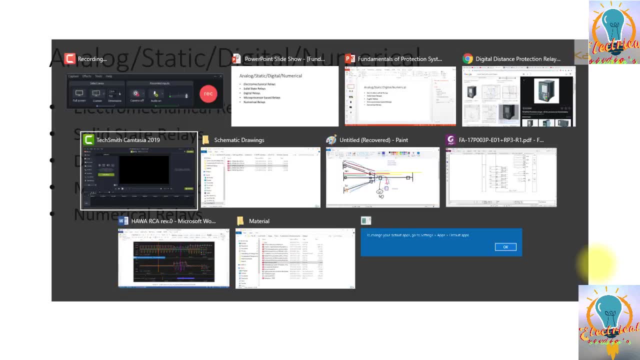 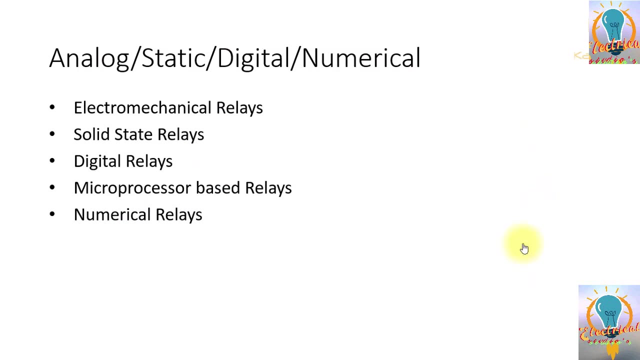 older one If you use the new one there calling ASEA S7 3.2, 4.. applications ISO t style- This one is also Jetzt. electromechanical relates are made and i have seen the timers and also these coils together and they are working together because the current element- okay, that could be performed and programmed. 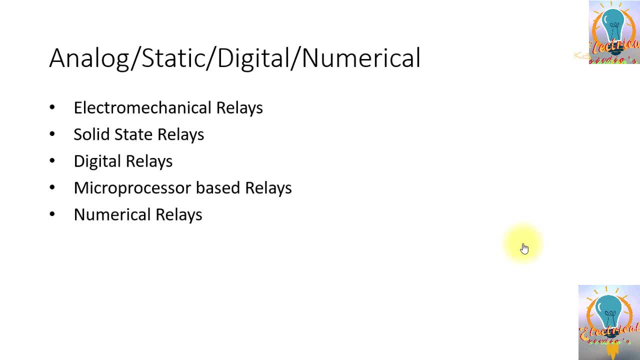 by the electrical engineers, but all the timers and all these different competitors and logics are supported and by by the watchmakers. so, uh, it was initially era and the burden of this release was another disadvantage. one is: the size is very big and these are very heavy and difficult to 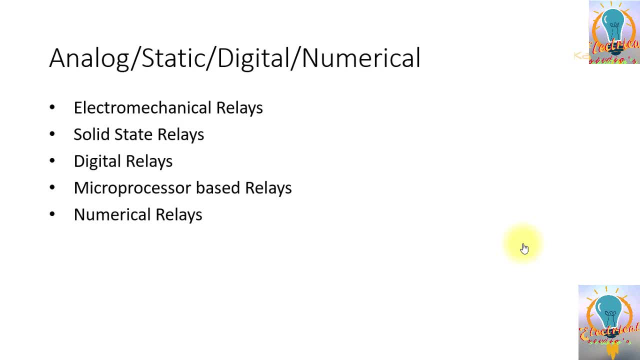 carry installed and they take a lot of space. the second disadvantage is that these relays have a high burden. the burden of the release is high, so it means that you need to have a bigger size of ct if you want to still want to use these relays in the old old time. so this was a disadvantage. 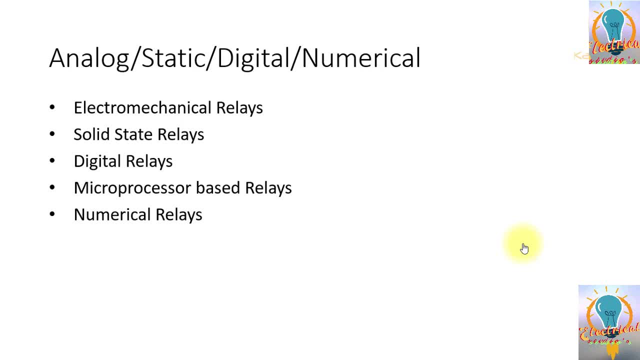 another disadvantage was the flexibility. so so if you have designed a contact for certain function, you cannot change it. output contact: if you design a input for a certain function, you cannot change it. uh, so these are the disadvantages of this huge electromechanical release, but the advantage, what i have seen for this huge electromechanical relays like cdg. 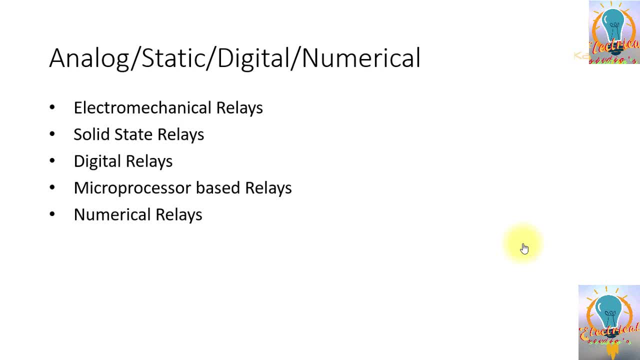 i really personally like this cdg over control. this is a really rugged relay and it doesn't need any. in our area we have extreme temperatures like 40 to 50 degrees centigrade, so even if i found this release even working fine in these temperatures, 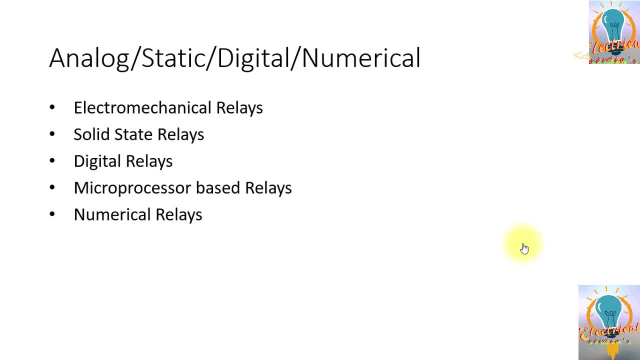 but whereas the microprocessor basically need to have an air condition and you need to need to have a clean environment to run these relays, so the electromechanical relays are rugged as compared to microprocessor release. so next era was the solid state release. these 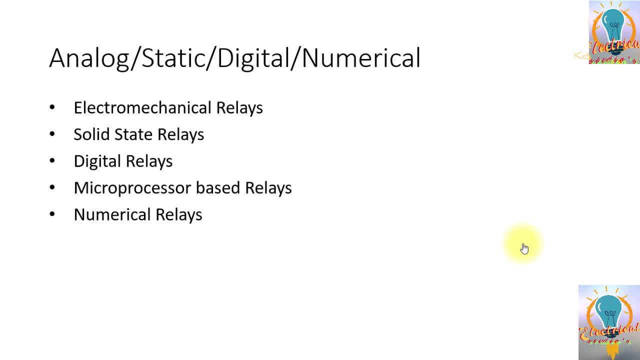 relays are smaller in size and in this release they have used basically the digital component, like capacitors, thyristors, transistors. so they have used and they have tried to use these solid state components in in these relays. and here you can select different settings by using a dip switch or a selector switch. 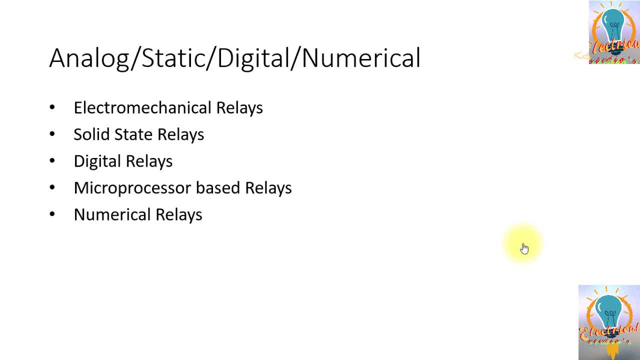 this. this was also the compact release, and in electromechanical release all the input quantities are used as it is for, whereas in solid state relays we are using some analog digital conversion. at some state, then it comes the era of digital relays, instead of using the solid state components. 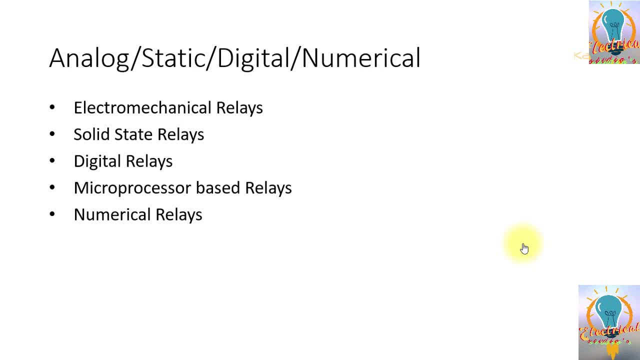 now the engineers started to use the microprocessor to do the operations, but still you have again the microprocessor installed in the background. but you cannot do the reprogramming. you can do lot of functions, the relays work same as solid state relays, but it has microprocessor installed. 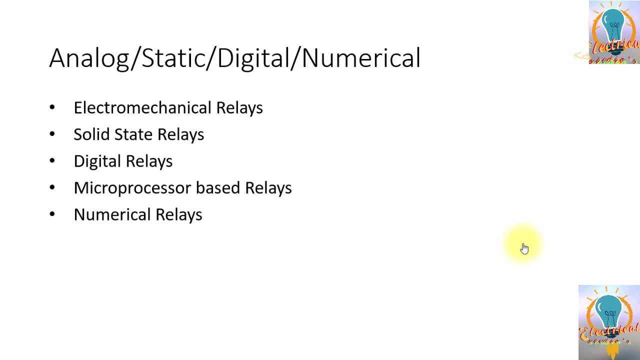 and you can do some, basically selection of settings. it's not very flexible, but in this microprocessor relays, base relays are basically digital relays. now the method of operation has changed. now these relays are converting the analog quantity like Ct or Vt, current or voltage. 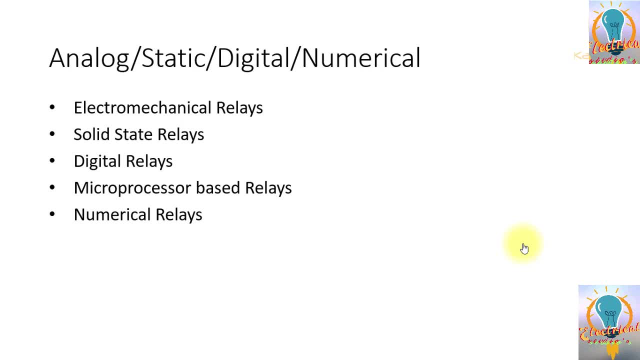 which is input to these relays, into a digital quantity. mostly they are converting first of all the input signal from analog to digital and then this digital signal is used in the relay everywhere. so these are microprocessor based relays. later came the latest production relays that we are seeing now. 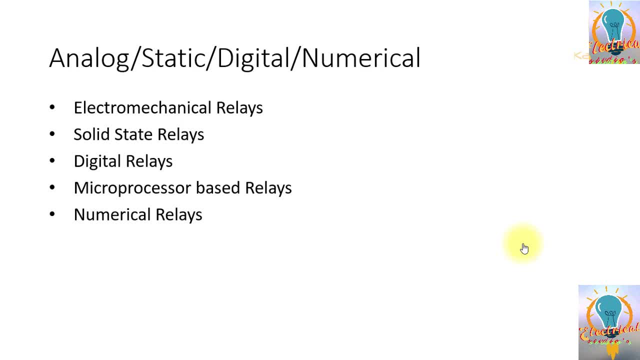 the latest production relays that we are seeing now, the latest generation, in which each relay has a user graphical interface and relay has a lot of flexibility. you can configure output contact as per your requirement. you can connect any binary input for any function and you can change the settings. 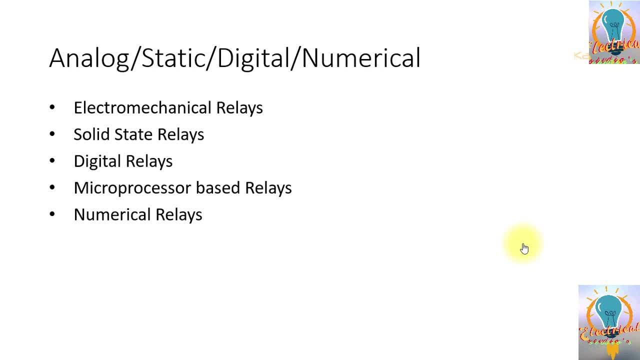 you have lot of setting groups, functionality of setting groups. you can switch on or off different setting groups. you can adopt adaptive settings just by pressing a push button. so there are lot of flexibility now in numerical relays. so this is the little background about the protection schemes. 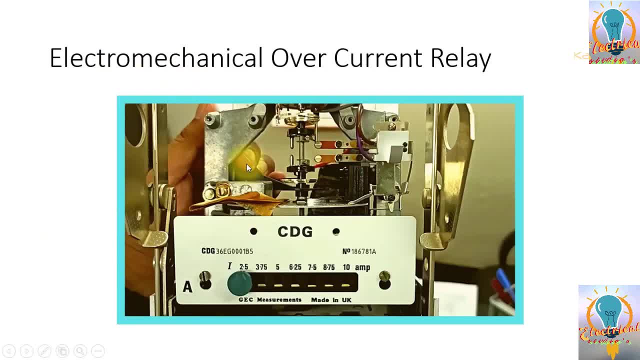 now we will go through. so this is basically one of my favorite electromechanical relays, so you can see it used to have. basically, this is called as current setting multiplier. this is a plug setting multiplier. this is a plug. that's why we used to call it as a plug setting multiplier. 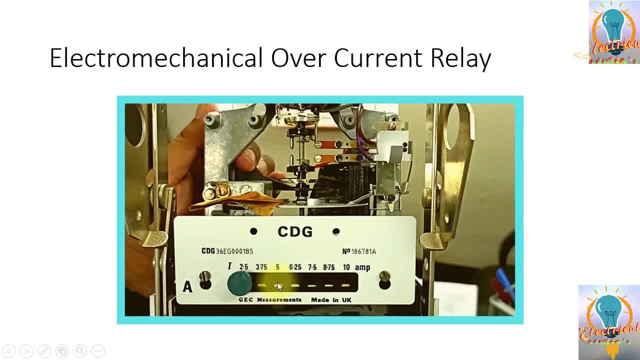 so you can have a different setting of 2.5, 3.75. so, and you can see this is a disk. so this relays works at the principle of induction disk and during transportation you can see they have put a paper so that it should not move and damage excessively. 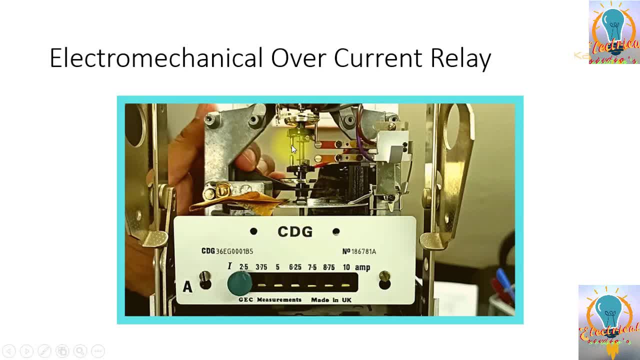 so and you can see these are the contacts when it move and hit this contact here, so it will issue the trip command. so this is basically the initial electromechanical relays that I really also favor this relays it's very simple to operate and it's very rugged relay. 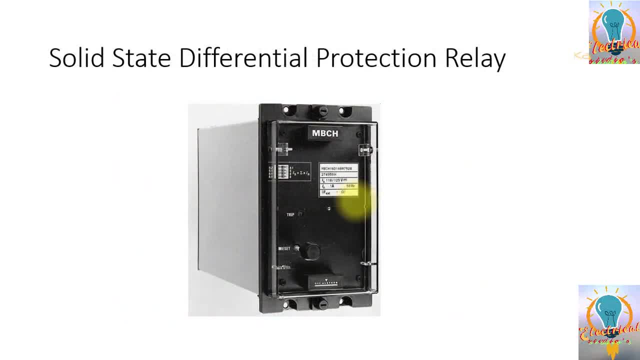 so another example of solid state relay. now, with the time passed, you can see. now the relays are changing also. so from electromechanical now we have a relay which has solid state components like diodes, thyristors, capacitors in it. so using this and you can see on the front, 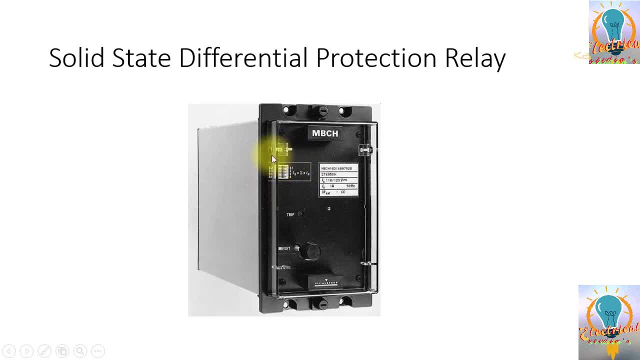 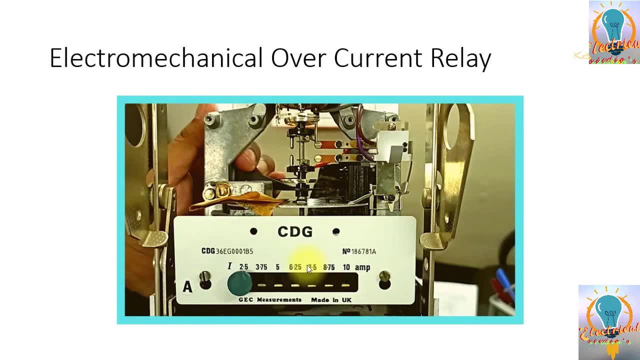 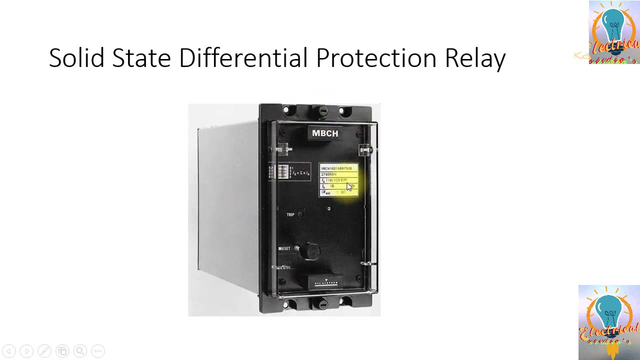 there are dip switches. these are called as dip switches in the protection relays, so you can, instead of putting a plug here, you can select a dip switch and you can do the settings as you need. this is basically a differential protection MVCH by GEC LSTOM. 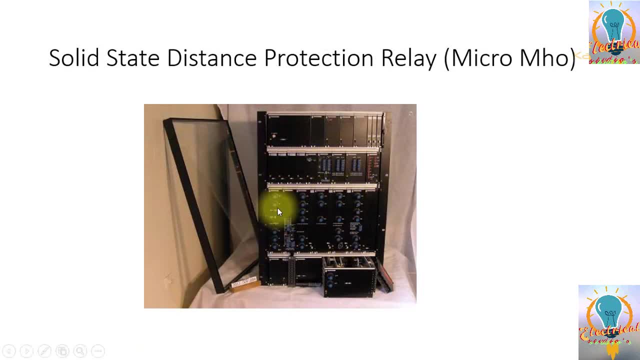 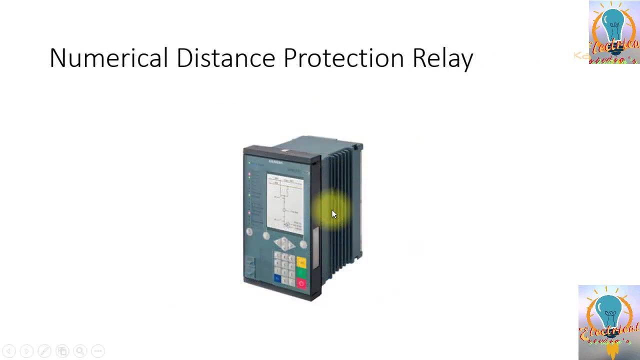 here you can see another relay which is basically another solid state relay, which is a micromo. you can see this is also a very big relay, so you can do all the settings. you can do by dip switches or the selector switches here now this is the latest relays. 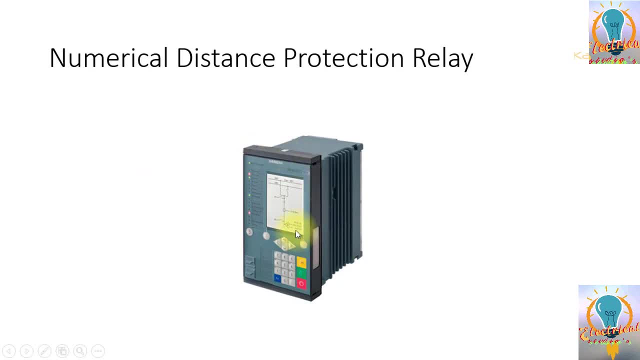 this is Dixie 5 relays and this is one of the very most modern relays. it provides you the most flexibility and this portion is called HMI- user human machine interface. so you can do lot of configuration. you can view the fall records, so this is giving you the maximum flexibility here. 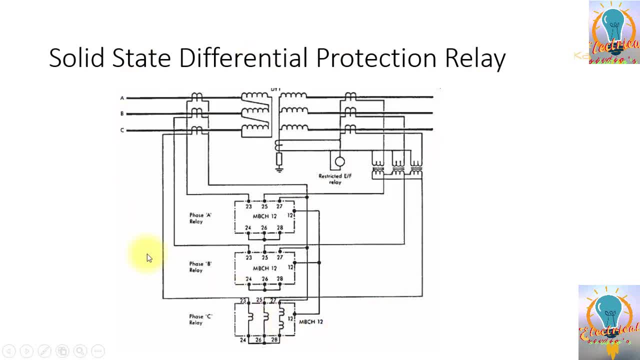 and this is basically the circuit diagram. just I have shown you how they have connected MVCH relay. it is basically here doing the differential protection of delta star connective transformers. so here you can see, in the old days this MVCH relay is the transformer differential protection relay. 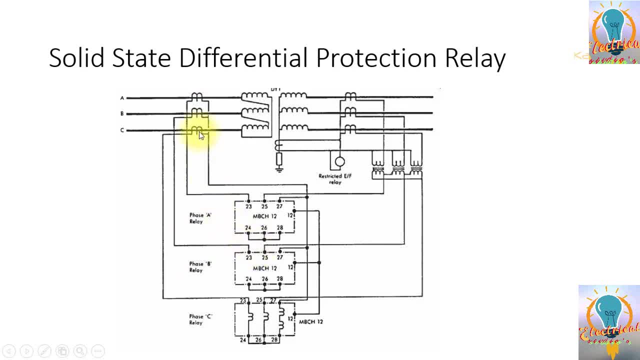 they have connected HV side to the MVCH. HV CTs and LV CTs are connected through this interposing CTs. the previous solid state differential protection relays were not able to compensate the phase shift and the ratio, the phasor and the ratio error. 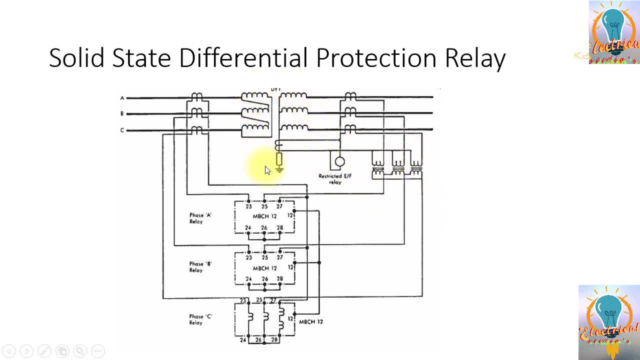 that is caused by the transformer differential vector group, transformer vector group. this doesn't have the ability to compensate this difference of ratio and angle. so what was the practice is to install one another- matching CTs. it is called. you used to call it as a matching CT. 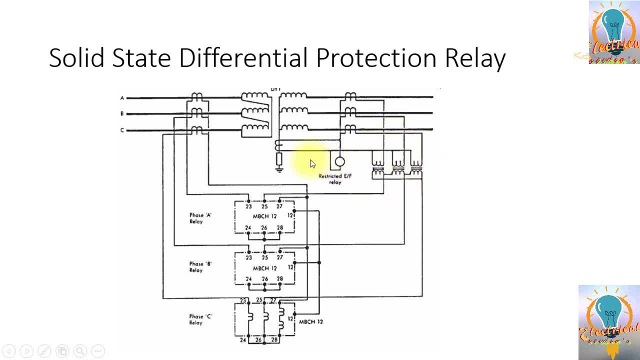 so you have to connect this matching CT in a way that it should compensate the angle and it should also compensate the ratio. so it will, so that the LV current will be reflected same as HV current. so this is an interesting fact that used to be do, used to be done. 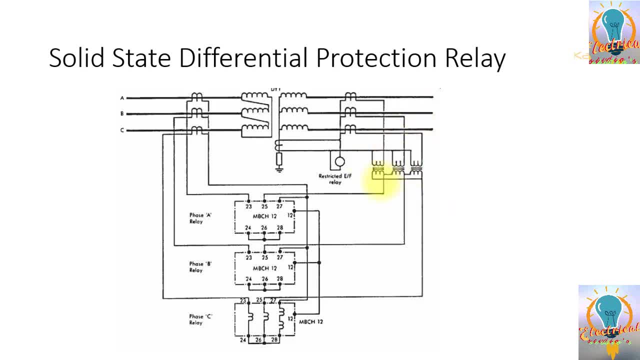 but nowadays you can see, just you need to put vector group in the numerical relay and rest of the matching will be done inside the relay automatically. so this is a good example how the numerical relay has the saved for the time and the money. so I hope you enjoy this section. so far, 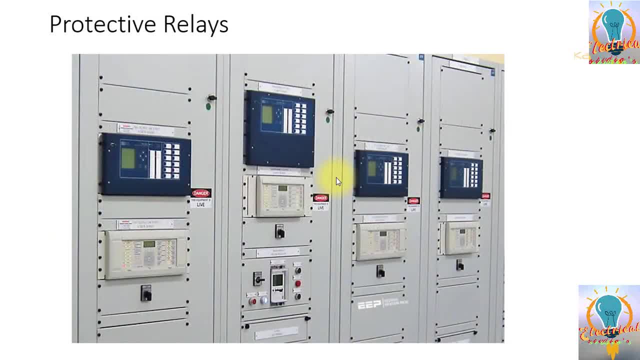 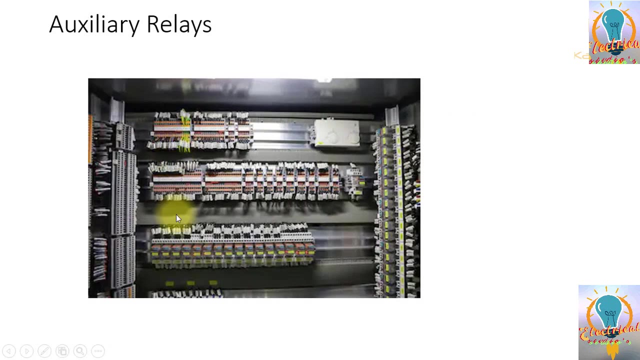 so here you can see this is a protection panel and you can see these are the numerical relays, the main relays which are installed in the panel. this is the inside of the panel and you can see these are the auxiliary relays. this is the set of auxiliary relays are installed. 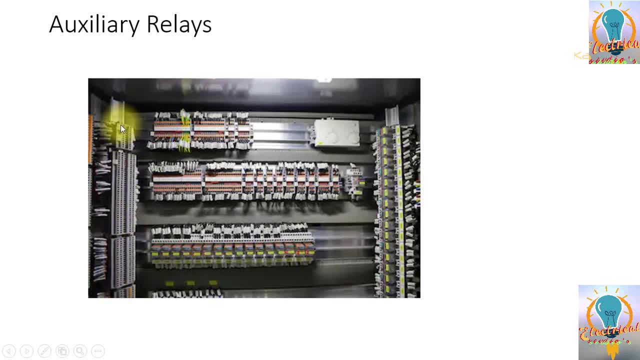 here you can see. this is the terminal block that we have seen. the back side is. you can see a dendrite and you can see normally on the left side. here the cables are coming from external side and the right side the cables are connected to the internal. 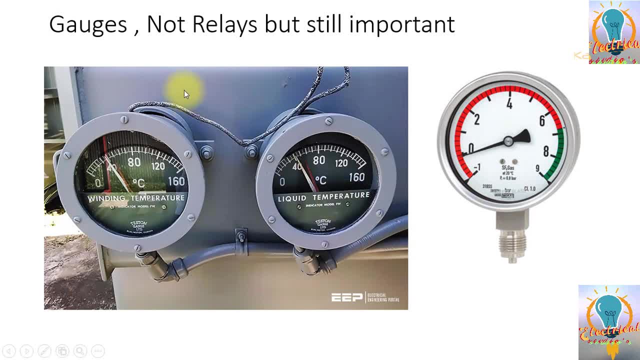 and here you can see the gauges. these are not relays, but also very important. so this is winding temperature that we have discussed. this is installed on transformer and this is the oil temperature gauge. the red needle here you can see is basically when the needle is moving forward. 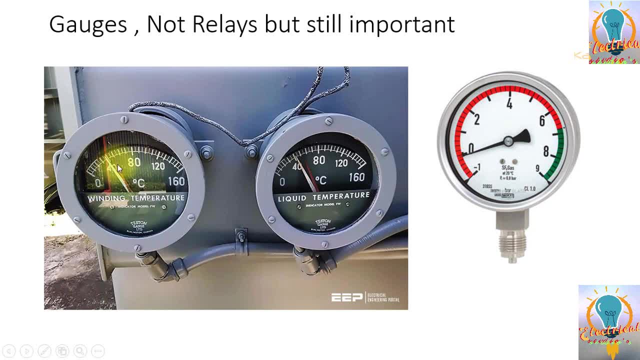 it will take the red lead with it when it is going back. it will stay its own position. so in this way you can see what was the maximum temperature has gone for the specific equipment here you can see this is the gauge to monitor the SF6. ok. 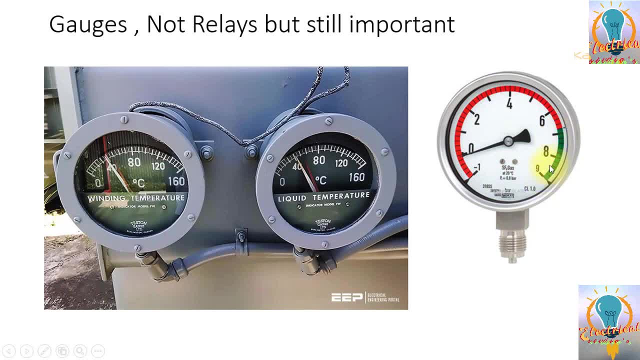 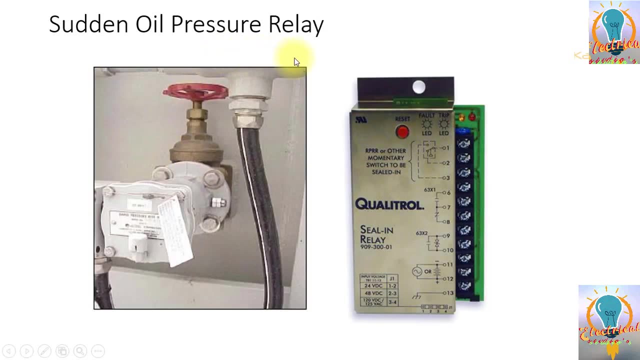 and you can see this green. it means that this is the healthy region and this normally. there is a green, then yellow means alarm and then there is a lockout region. so this is SF6 gauge. again, it is a monitoring device. then you can see a sudden oil pressure relay. 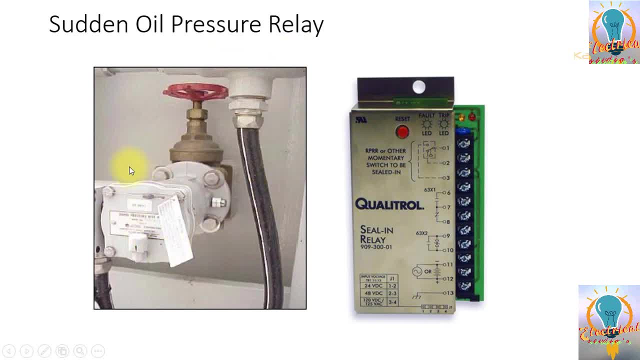 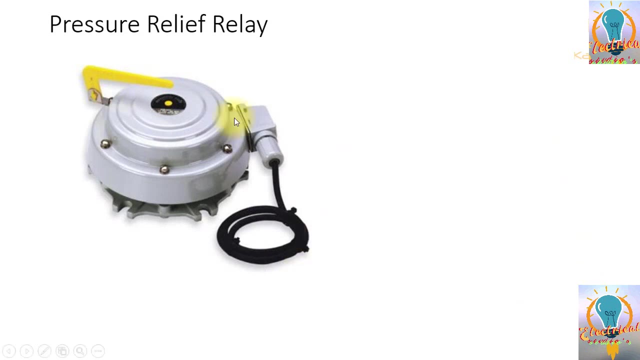 so this sudden oil pressure relay is installed, which is monitoring the pressure inside the transformer, and this is the device that is connected together. so as soon as there is a sudden oil pressure, the relay will trip the transformer. then you can see a pressure relief device. this is again a mechanical device. 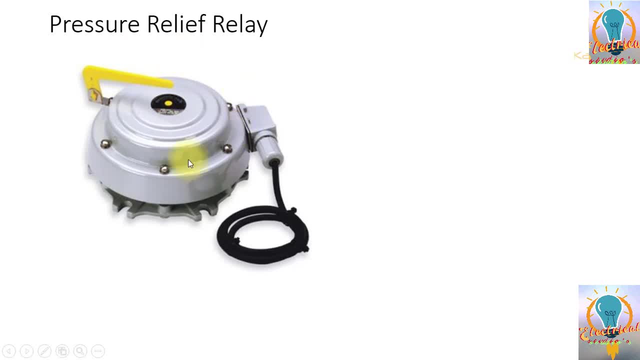 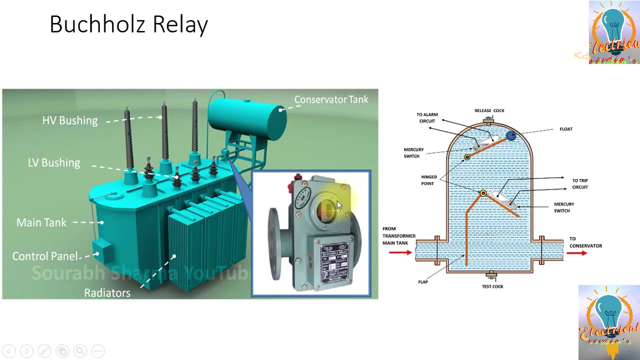 which is installed on over the main tank and when there is high pressure, this will be, pressure will be released and this contact will operate and it will give alarm and may give tripping. you can see the connection can be made through this. then we have another type of relays. 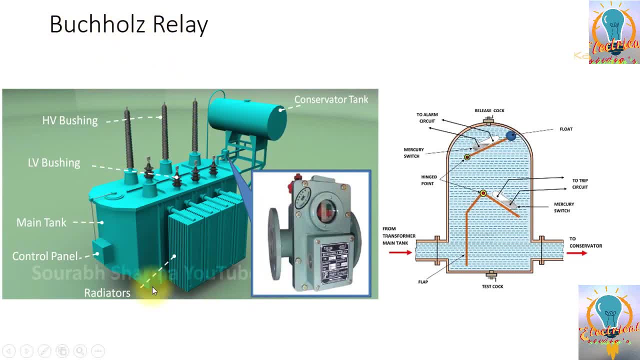 like a buckle relay. this is our transformer here. so you can see buckle relay is installed between. this is the main tank and this is a conservative tank. so you can see the buckle relay is installed between these two. so if there is any gas it will go up on the tank. 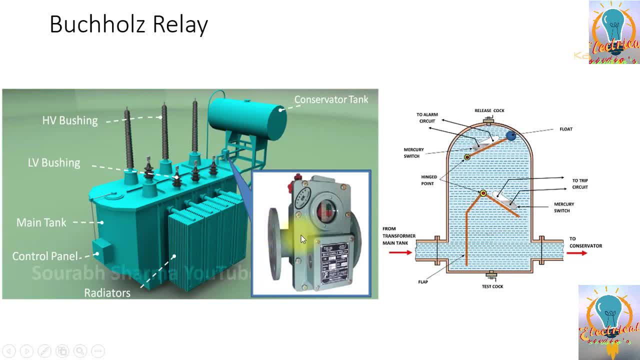 and it will go further rise. when it will come here and passes through this buckle, this gas will be trapped here on the top and it will start accumulate and in first stage you can see when this flow gas is there. this float will start to come down and then alarm will initiate. 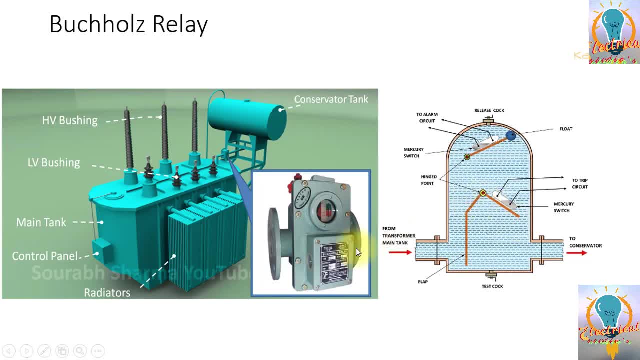 and in the second stage- this is another contact- if there is a severe fault in the transformer, then oil will be rush instead of gas. oil will be rush with such huge pressure from main tank to conservative tank because huge pressure is built up in the main tank because of the severe fault. 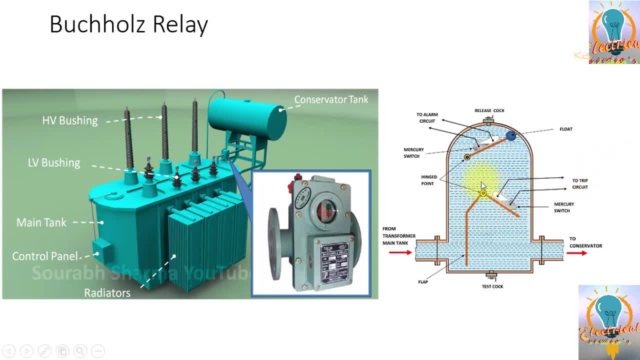 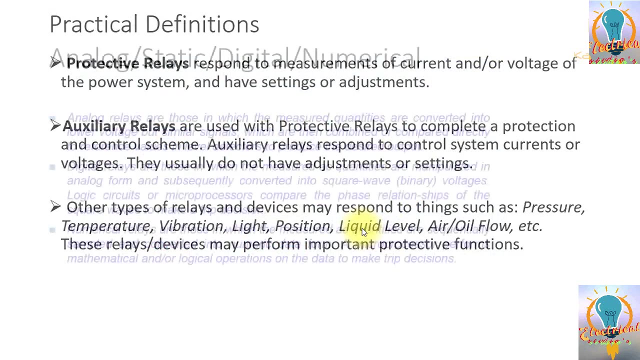 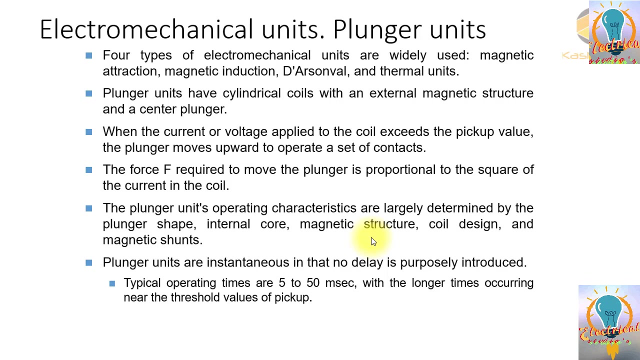 then this contact, which is a trip contact, will operate. it will trip the transformer. so this was a little introduction. so I hope that you have enjoyed this lecture also. thank you very much, hi friends, in this section we will study electromechanical different type of relays. 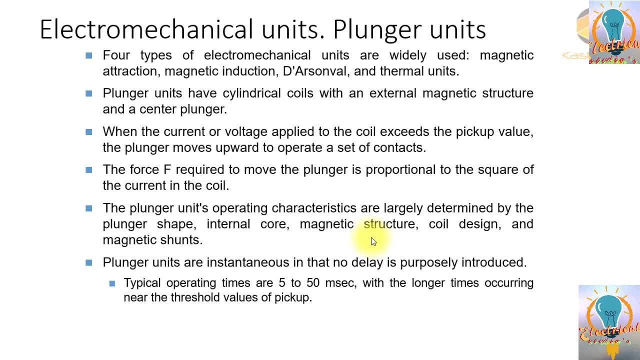 so electromechanical relays can be classified into four different types, like magnetic attraction type, magnetic induction type, de-arsenal and thermal units. so these are different kind of electromechanical relays that we can classify. so we will start and study the plunger type. 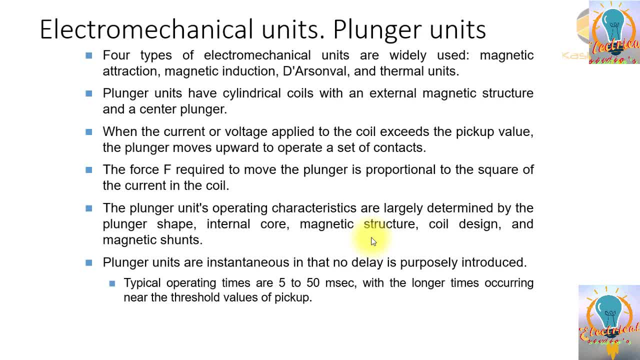 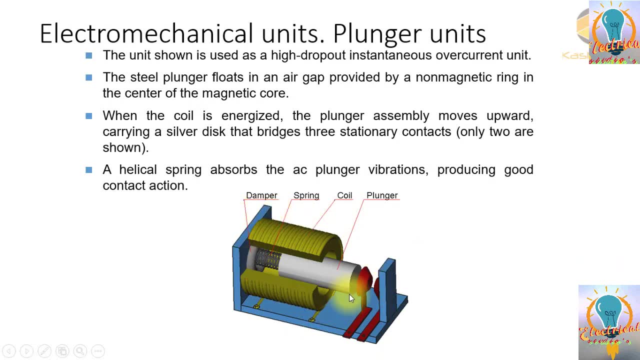 production relays, the plunger unit have cylindrical coil with an external magnetic structure and a center plunger. so you can, we can see here this is basically a plunger type relay. so this is a plunger which is- and this spring is installed, ok, so this is basically a damper. 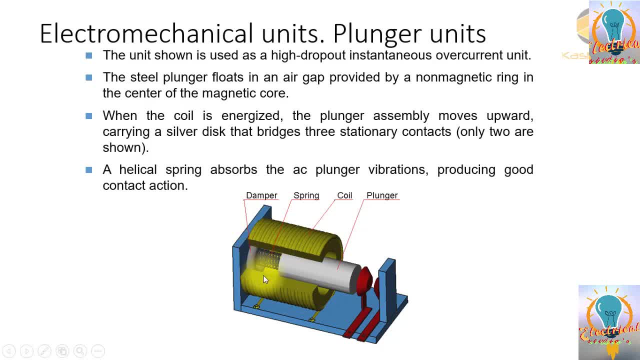 damper is also installed here which dampens the oscillations, then this is a coil and this is a plunger, and this- you can here see- this contacts. when this armature is, when this coil is energized, then this plunger is moving forward and then it will hit this contacts. 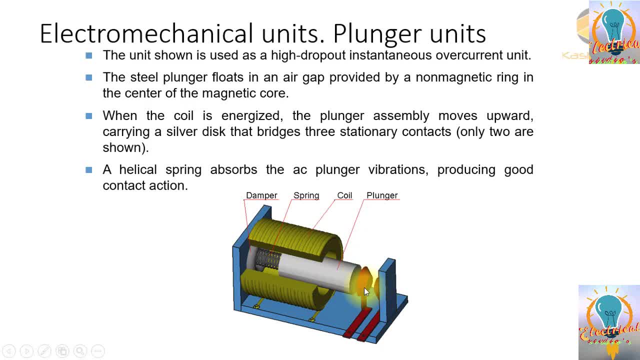 and this contacts. when it is hit, they will closed and any function like tripping or alarm or as you need, you can operate it. and as soon as this supply is switched off, this plunger will go back. so when current or voltage applied to the coil exceed the pick up value. 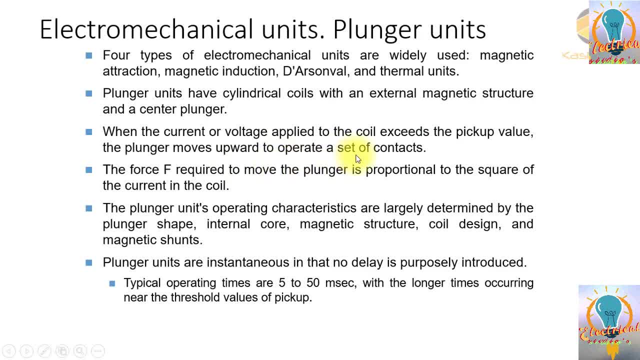 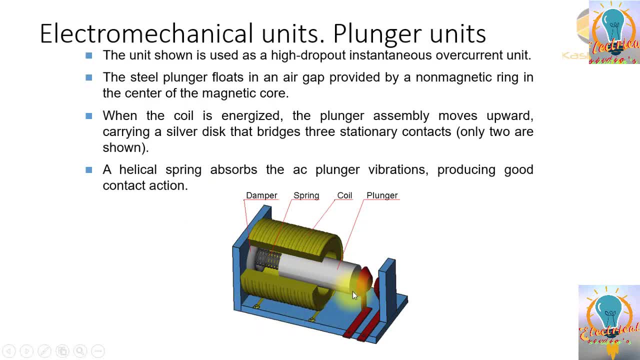 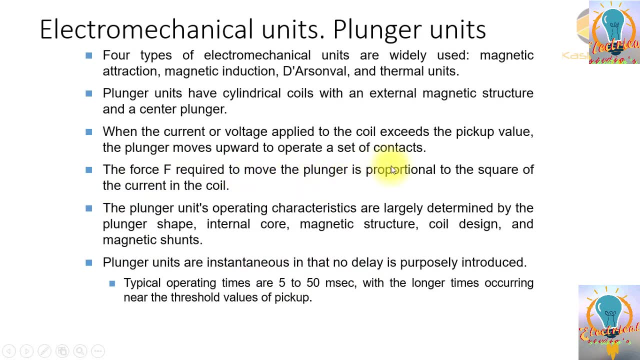 the plunger moves forward to operate a set of contacts. so you can see, this plunger will move forward as soon as this coil is energized by voltage or current and it will hit the force as required to move. the plunger is proportional to the square of the current in the coil. 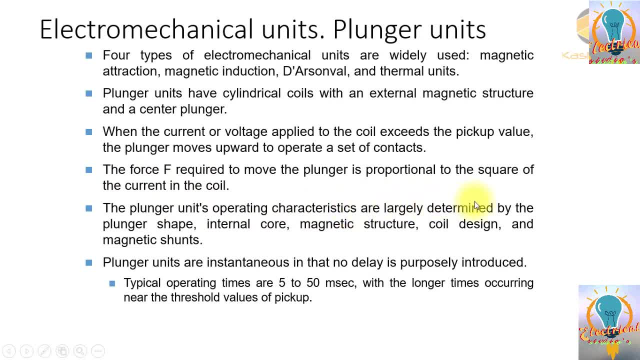 the plunger unit operate. characteristics are largely determined by the plunger shape, internal core, magnetic structure, coil design and magnetic shunt. plunger units are instantaneous in that no delays purposely introduced. typically, operating time of plunger is 5 to 50 milliseconds, with longer times occurring near threshold value of pick up. 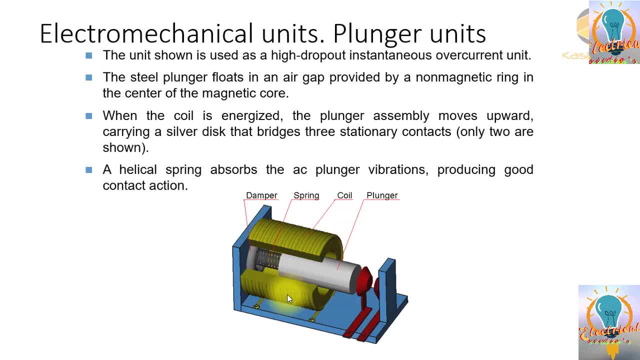 so these are very fast to operate. so we are operating within range of 5 to 50 milliseconds. these are very one of the very simple just relays. the unit shown is used as a high dropout instantaneous overcurrent unit, so here this is used as an overcurrent protection. 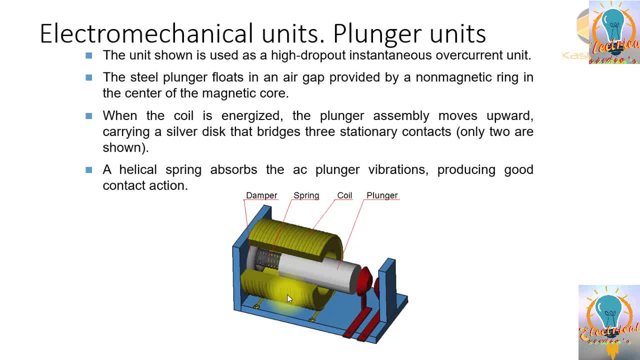 the steel plunger flows in air gap provided by non-magnetic ring in the center of the magnetic core. when the coil is energized, the plunger assembly moves upward, carrying a silver disc that bridges the three stationary contacts. only two are shown here. a helical spring absorbs the AC plunger vibration. 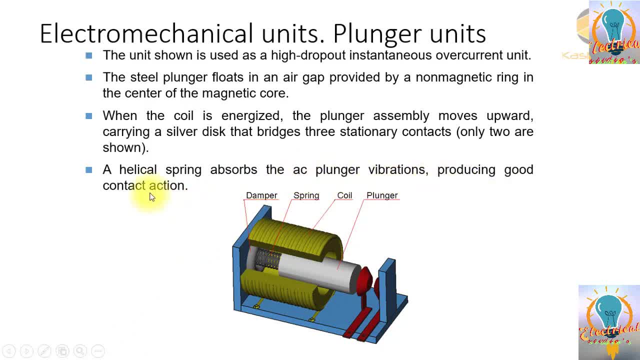 and produce good contact action. so this is a very simple plunger mechanism. all the tripping coils which are used and closing coils which are used in the protection in the circuit breaker mechanisms are basically plunger type and this coils which are used in the circuit breaker. 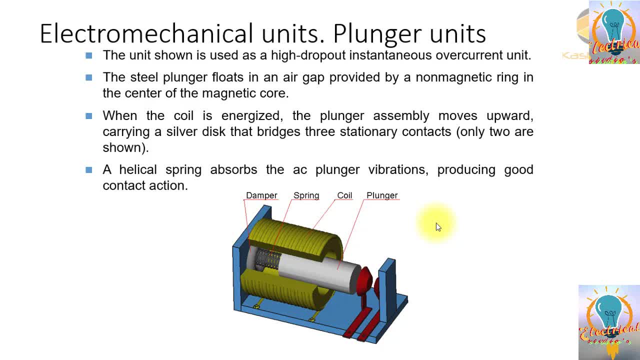 have a very small duty cycle. it means that you can, if you have to give a pulse for a very small duration of time. if a pulse is given for a longer duration, the coil will be damaged. so we have to take care while operating these devices. so here you can see. 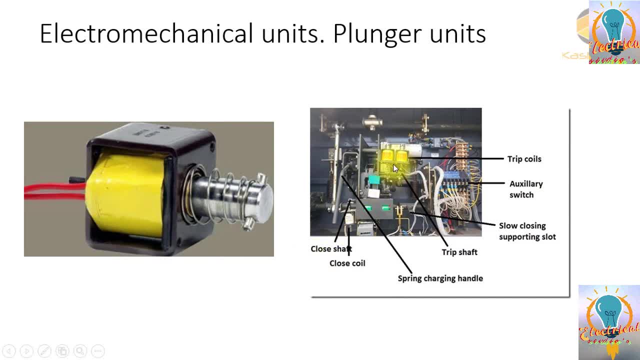 this is basically the plunger mechanism and you can see these coils are installed in the circuit breaker. this is the MV circuit breaker. so you can see this is the closing coil, which is also a plunger mechanism, and this is the trip coil. so when it is energized, 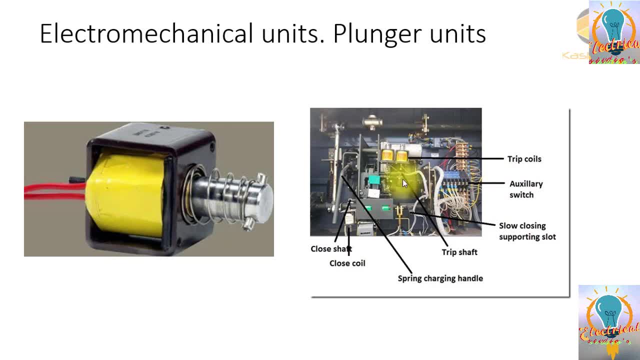 it is heating a latch and at that run that spring is released, and then the spring is release mechanism is released and you can close and open the breaker. so this was a little introduction about the electromechanical units plunger type. thank you very much, hello friends. 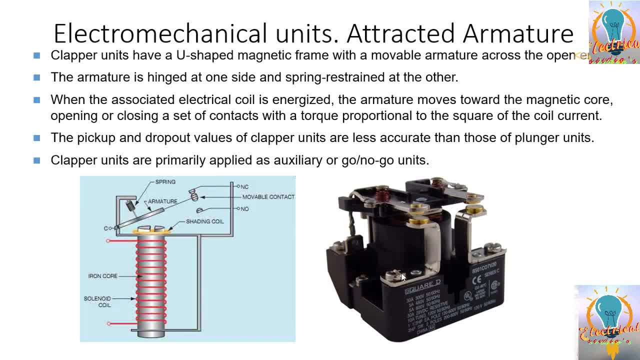 now we will start our new discussion, and that is electromechanical relay and now the type is attracted armature type, so this is also called as a clapper unit. so basically these are in U shape, magnetic frame with a movable armature across an open end. 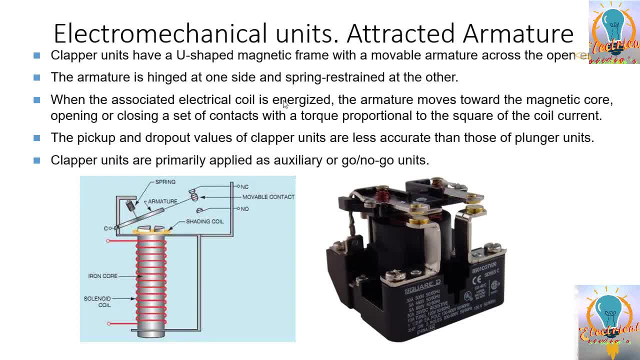 the armature is hinged at one side and spring is seen at the other. so you can see, this is basically an armature and it is restrained by a spring and it is hinged at one side and this is basically a coil, and this coil is across an iron core. 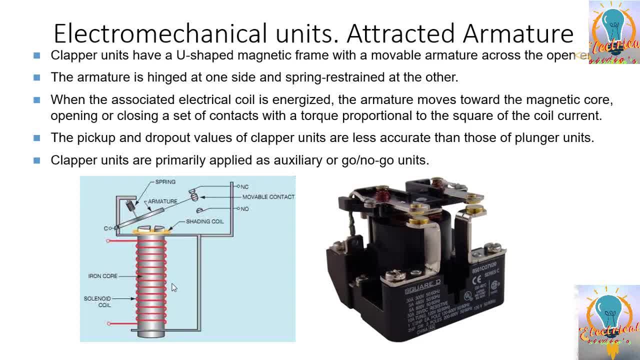 so when this solenoid or this coil is energized, then this magnetism is formed and then this magnet will attract this armature and it will come down. so this is the normally close contact. so when it will come down, this is the common contact and then it will touch this. 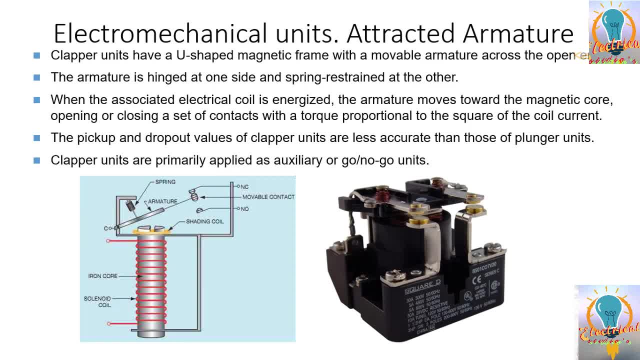 so this is the normal open contact. so when this is energized, this armature will come down and this contact will move here. so it will move from here, it will hit here at NO. so in this way these relays are operated and you can see this is. 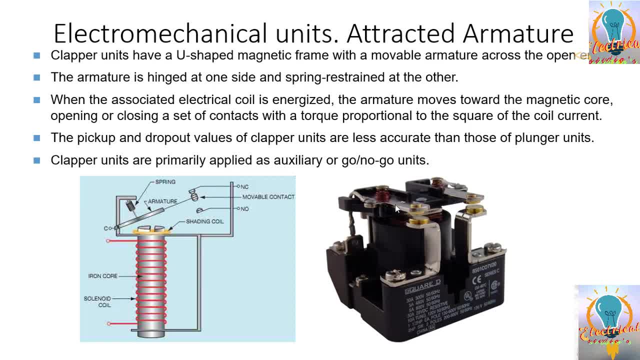 the physical shape of the relays like this. so these are kind of yes or no relays. so this is very simple logic. the pick up and drop out values of clapper units are less accurate than those of plunger units, so these are not very accurate. 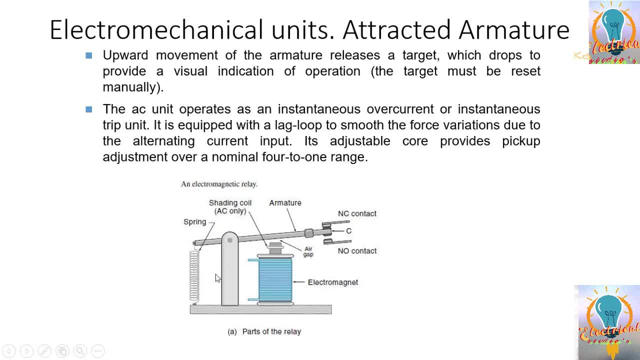 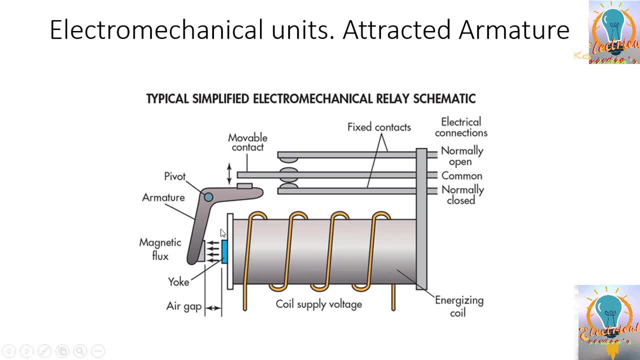 so here you can see another type of atletic armature relay. so here you can see another construction, so how this atletic armature relay is operating. this is very simple diagram once again. so when this coil is energized, okay, and this contacts, this armature will pick up. 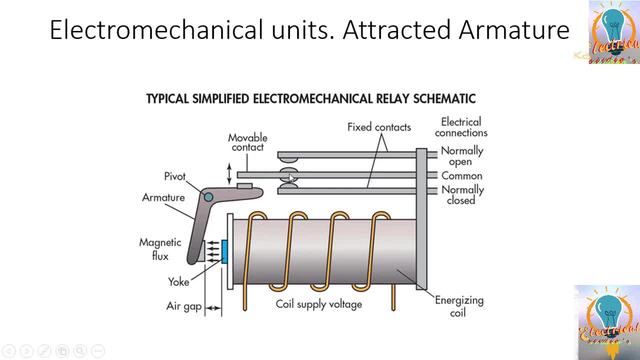 and then it will push it and then you can see this contact will change from. it's a change over contact from NO to and C2 towards NO when it's picked up. so this is basically very simple relay. so we'll move to our next topic. so another type of 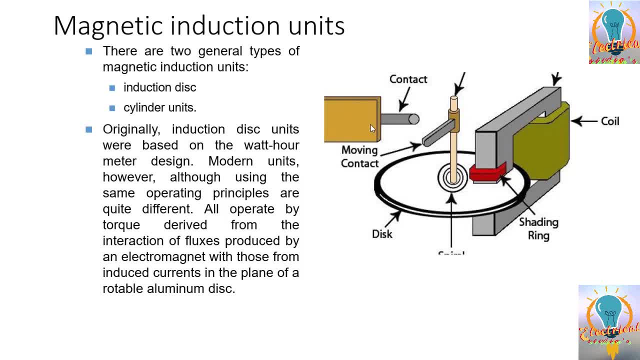 production relays are you previously used to make was on the principle of induction disk type. previously I have shown you a CDG relay which is a great example of induction disk type of the relay. induction type of the relays can be classified into two types: induction disk type. 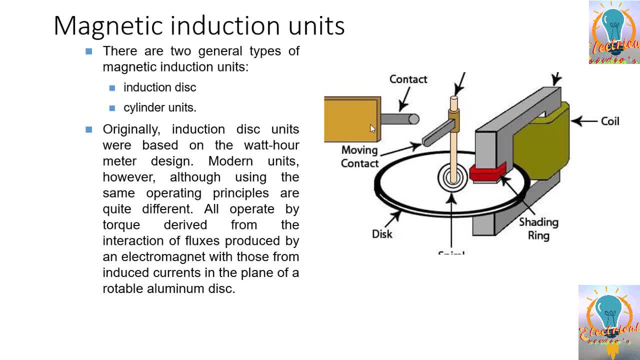 and cylindrical unit types. so how this relay functions. basically, this electromagnet has a flux. when this flux cut this, this disk, it induces the current in it and the interaction of this induced current and the flux, there is a torque that is produced. so this is how this 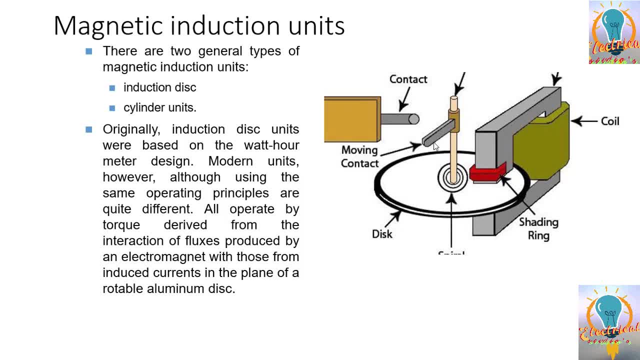 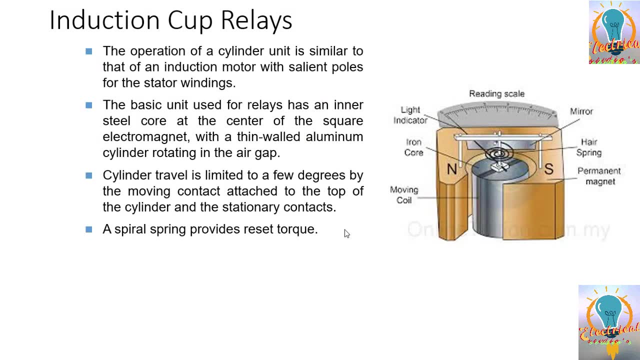 this relay works and then this disk starts to rotate and you can see at the end this contact will be made and this is a fixed contact, this is a moving contact and you can see the relay will operate. so another type of the induction principle relays are induction cup type of the relays: 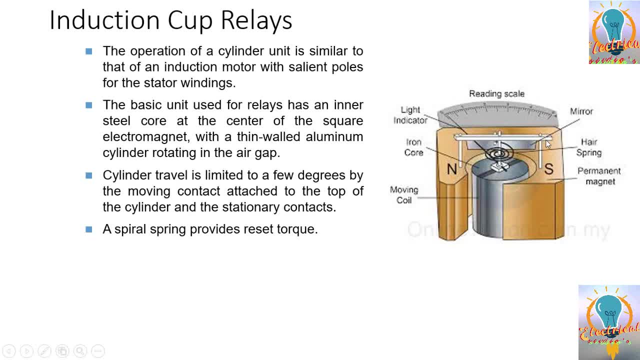 so here you can see basically the induction cup. this spring is used to reset the relay basically, and you can see this is it's forming a magnet and you can see this is basically a cylinder and in the similar way it will work as induction disk type. so you can see. 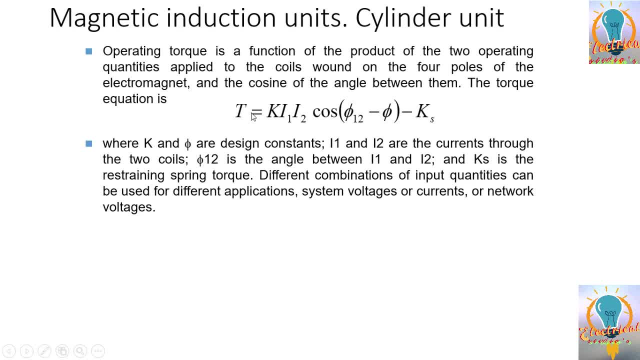 the equation of torque. so equation of torque is a function of product of two operating quantities applied to coils wound on the four poles of the electromagnet and the cosine of the angle between them. the torque equation is: t is equal to k, i1 into i2. 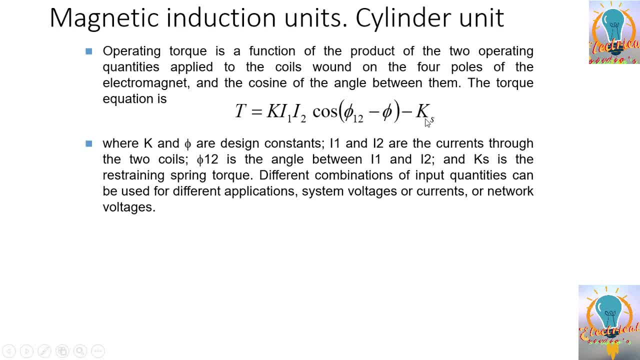 cos of phi 12 in minus phi minus ks, where k and phi are design constants. i1 and i2 are the current through the two coils. phi12 is the angle between i1 and i2 and ks is the restraining spring torque. different combinations of input quantities. 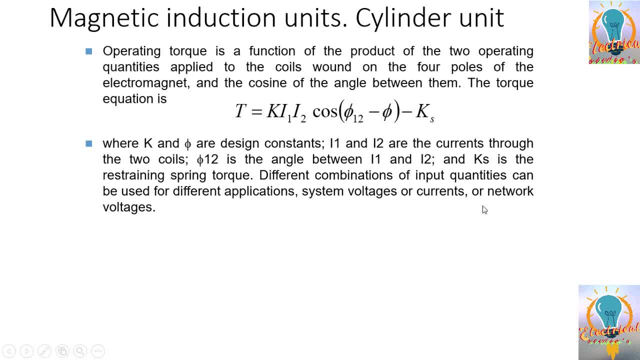 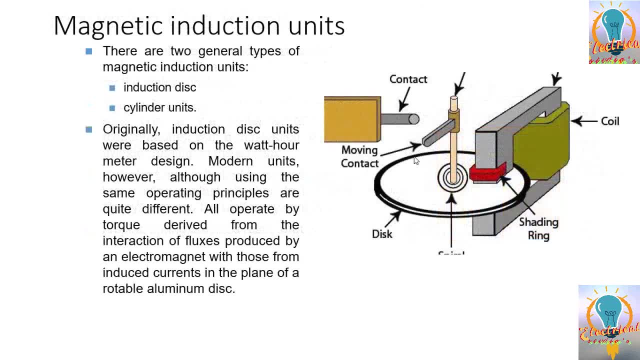 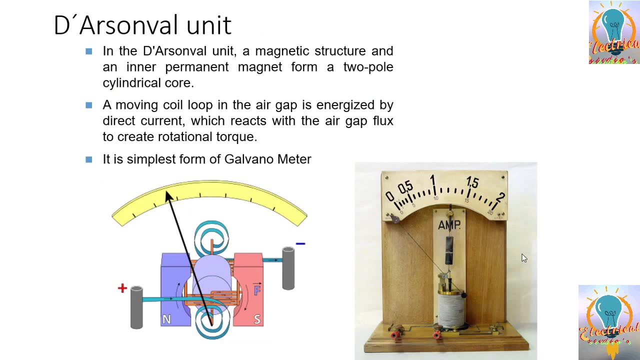 can be used for different applications: system voltages, currents or network voltages. so this was a little introduction about the induction type units. hi guys, now we will discuss another different type of protection relays that we use in the past is t-arsenal unit. we all have studied the galvanometer. 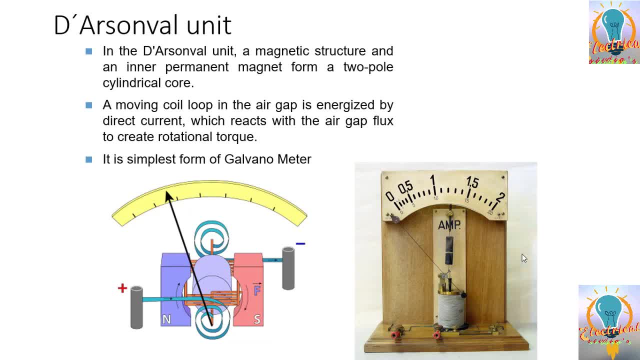 and how galvanometer works. this is working on the same principle. basically, you can see a coil, coil is placed in a magnetic field, across a magnetic field and the current passes through the coil. and when the current passes through the coil it has its own field. then there is an interaction. 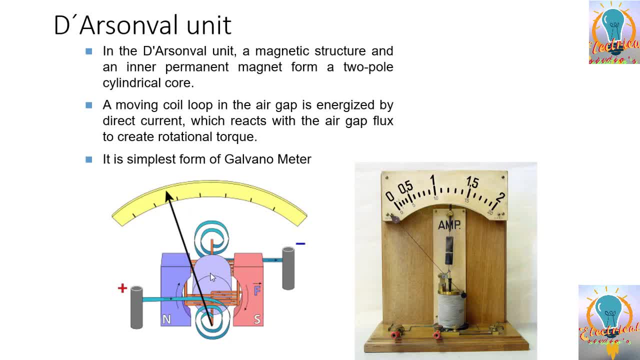 and this interaction basically causing this coil to move and this spiral springs are keeping the needle. it is taking the needle back when there is no force, so a moving coil loop in the air gap is energized by direct current which reacts with the air gap flux to create rotating torque. 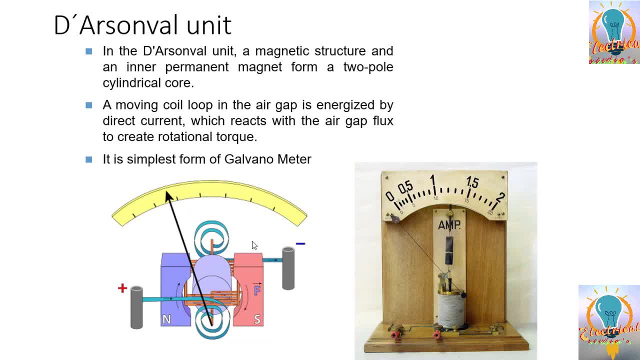 it is the simplest form of galvanometer, so this also can be used to make a protection relay. so this is another working principle on which previously we have designed the protection relays. so here you can see a very old form of protection relay, so you can do some settings. 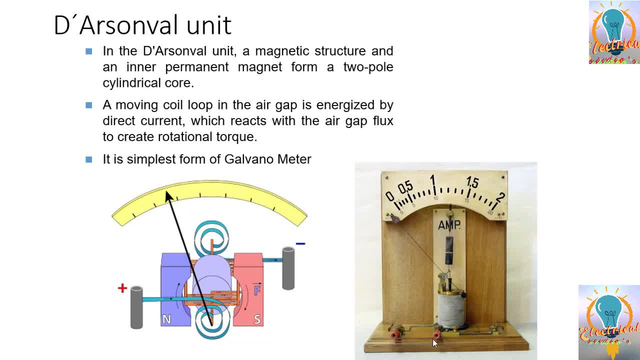 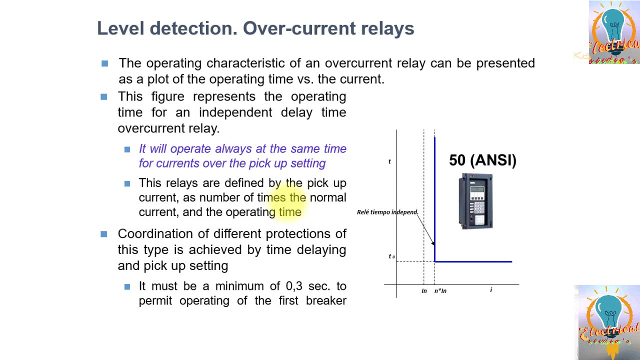 and after preset value the contact will operate and you can get here alarm and tripping. this is the very simplest form of electromechanical relay based on t-arsenal unit. so we will discuss here the level detection over current relay or you can say the definite time over current relays. 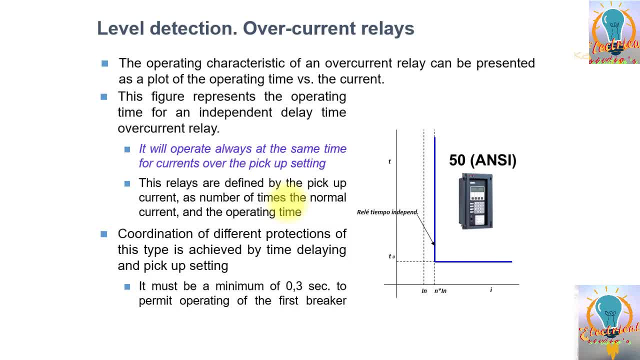 so these relays are basically continuously measuring the current and then they are comparing it with the set value: if it is just more than if it is over current protection, if it is just more than the set value after preset time relay or instantaneously, depending upon the settings. 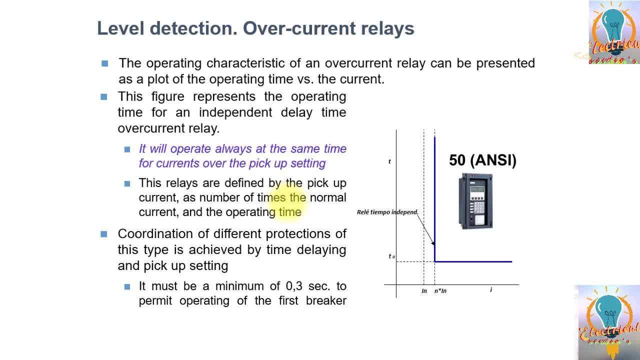 relay will issue an immediate trip command, so it is just simply checking the level all the time. so here you can see. the operating characteristics of the level detection or definite time over current relays are shown here. so here you can see this is the time and this is basically. 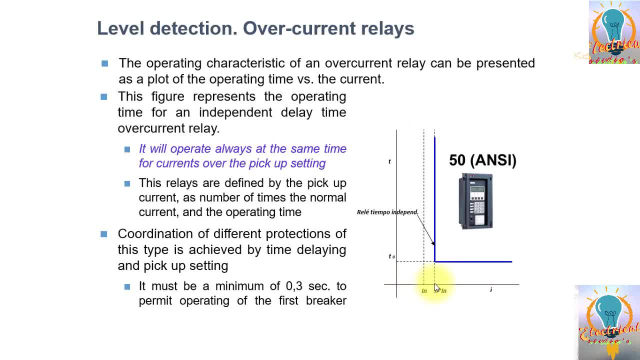 the current. when the current is increased, this is the rated current and the setting is done as multiplier of the rated current. n. so when the rated, when the current is increased more than the set value, the relay will operate, but the time of operation will remain the same. 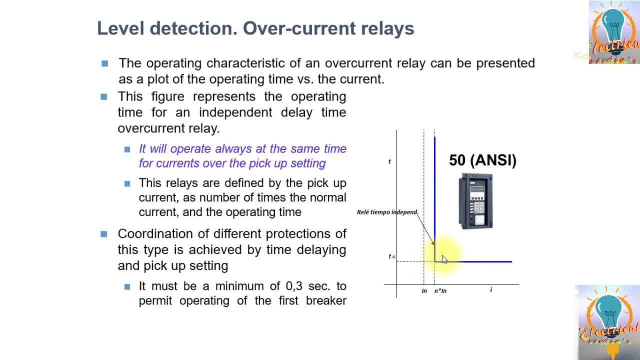 it will not change. as soon as the relay picked up, it will operate. if it is a time delay relay, then it will wait, timer will start and when the timer will complete it will issue alarm or trip. so this is used for coordination of different. protection of this type is achieved. 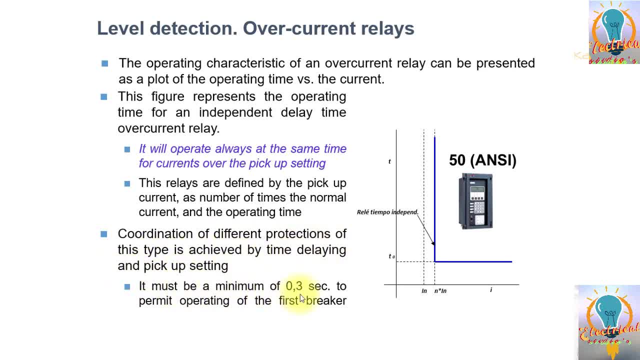 by time, delaying and pick up settings. it must be minimum of 300 seconds to permit operating of first breaker. so if you have, for example- let's take an example- if you have two substation, this is one, this is two- and one relay is installed here. ok, 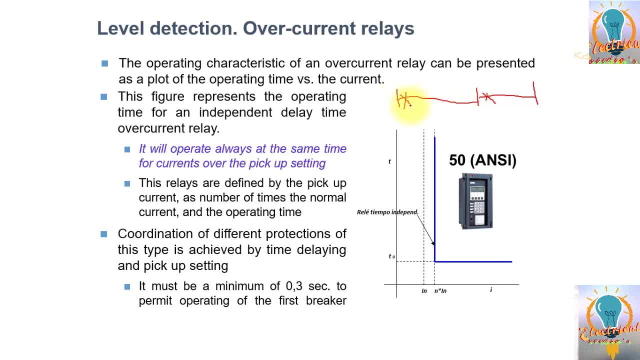 and another relay is installed here and there is a fault here. the fault current of this relay- the fault current because both are in series- will be same and we will set the time delay here to 100 milliseconds. ok, when, as soon as the relay will pick up. 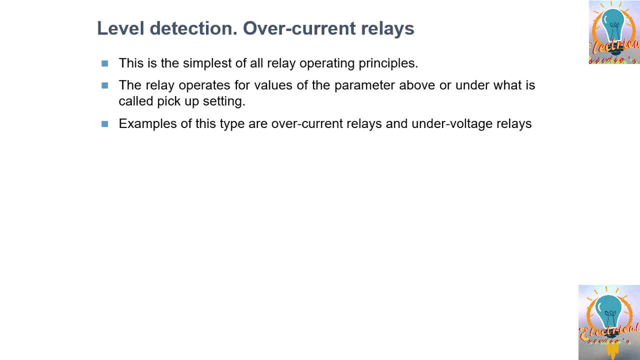 it will trip in. so in this section we will discuss different type of over current relay, the relay, how we can classify the relay by their function. so one type is level detection over current relay. so basically we can also name it as a definite time over current relay. 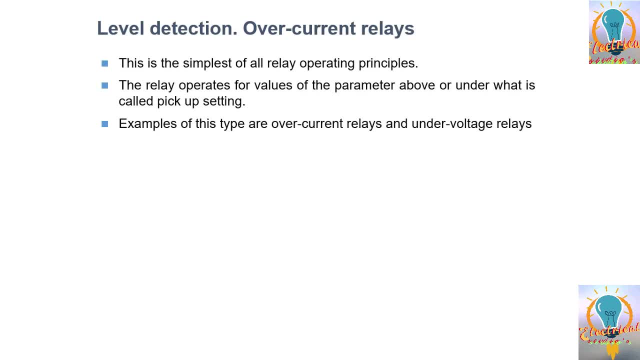 so this relay or definite time over voltage relay, so these type of the relays are continuously checking a level, certain level. for example, if you have set the setting of one ampere in the relay and the relay detects that it is now just more than one ampere, 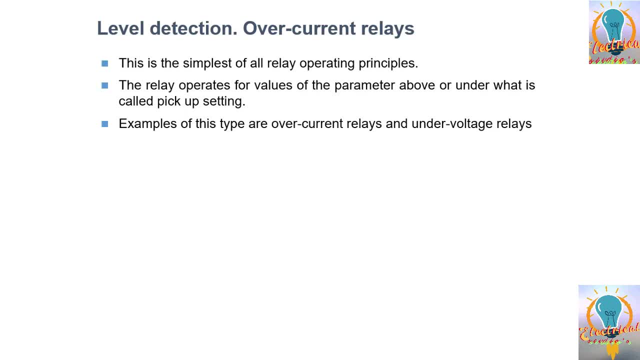 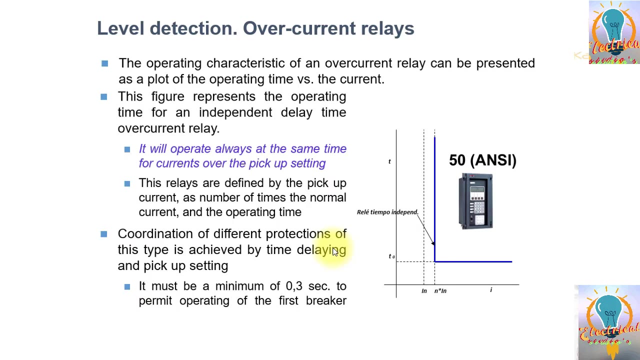 then, after a preset time delay or instantaneously as per your settings, relay will operate. it will give alarm or tripping as desired. so these are very basic type of protection relays. so we will discuss here the level detection over current relay or you can say the definite time over current relays. 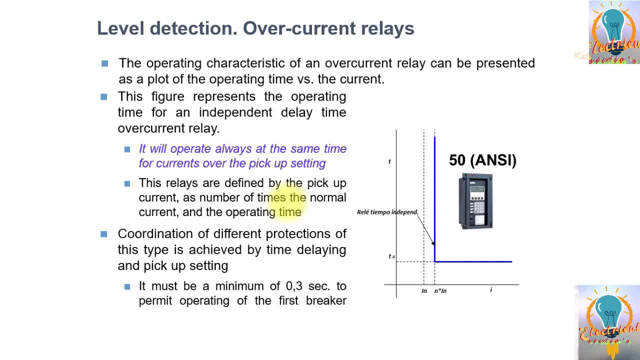 so these relays are basically continuously measuring the current and then they are comparing it with the set value. if it is more- just more than if it is over current protection, if it is just more than the set value after preset time, delay or instantaneously, depending upon the settings. 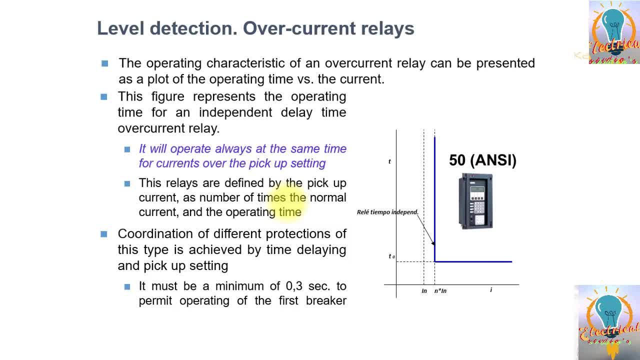 relay will issue immediate trip command, so it is just simply checking the level all the time. so here you can see. the operating characteristics of the level detection or definite time over current relays are shown here. so here you can see this is the time and this is basically. 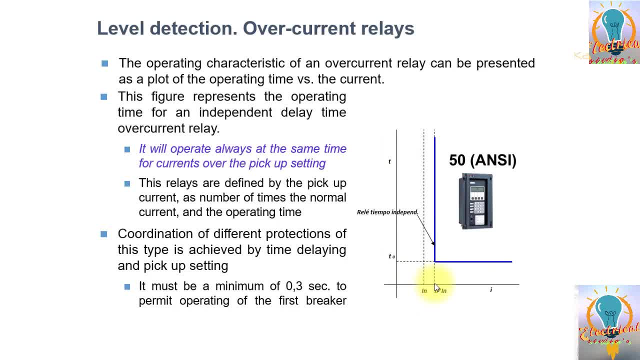 the current. when the current is increased, this is the rated current and the setting is done as multiplier of the rated current. n. so when the rated, when the current is increased more than the set value, the relay will operate, but the time of operation will remain the same. 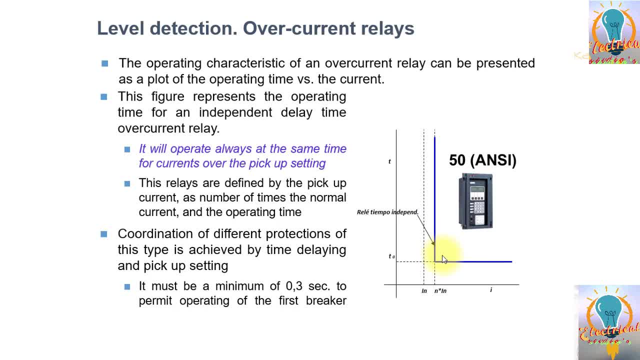 it will not change. as soon as the relay picked up, it will operate. if it is a time delay relay, then it will wait, timer will start and when the timer will complete then it will issue alarm or trip. so this is used for coordination of different. protection of this type is achieved. 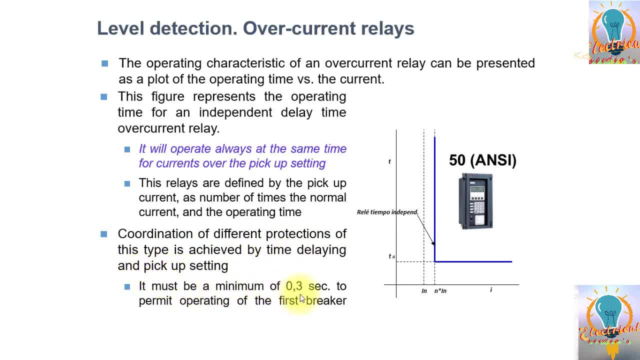 by time delaying and pick up settings. it must be minimum of 300 seconds to permit operating of fast breaker. so if you have, for example- let's take an example- if you have two substation, this is one, this is two- and one relay is installed here. ok, 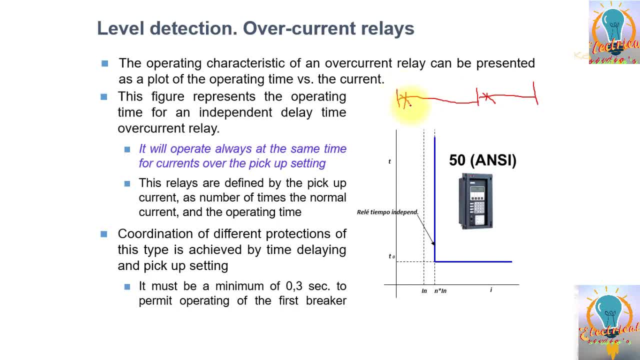 and another relay is installed here and there is a fault here. the fault current, because both are in series- will be same and we will set the time delay here to 100 milliseconds. ok, when, as soon as the relay will pick up, it will trip in 100 milliseconds. 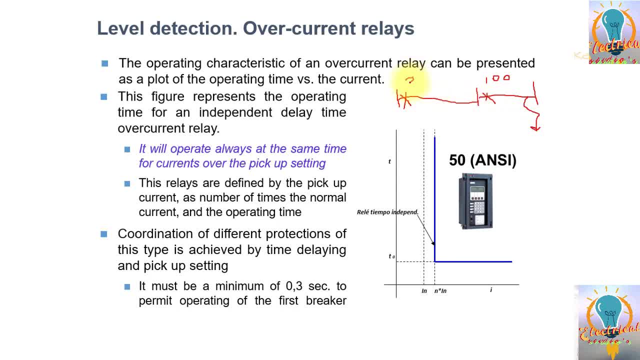 and here we can set the time delay of 300 milliseconds. so if there is a fault, this relay will picked up and it will trip the breaker in 100 milliseconds. this timer is also running. but if the breaker is not tripped by the relay because the relay is faulty, 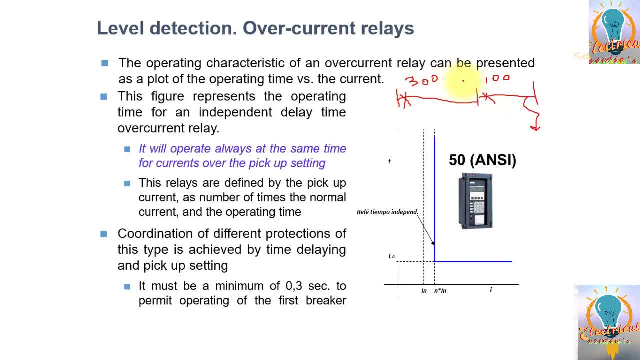 or there is no DC supply, for example, then this relay can will trip and isolate the fault in 300 milliseconds. so the level direction relay is with a given time delay. you can do the coordination studies. you can do the coordination under the thumb rule. you are keeping. 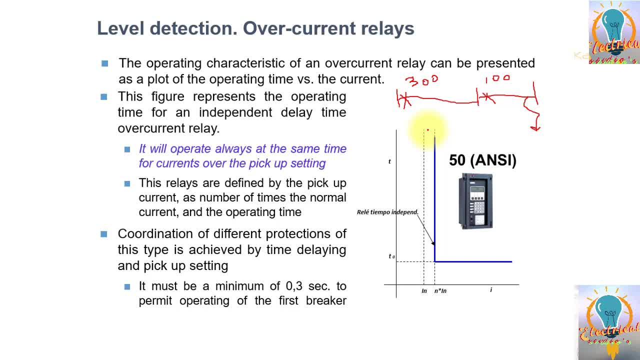 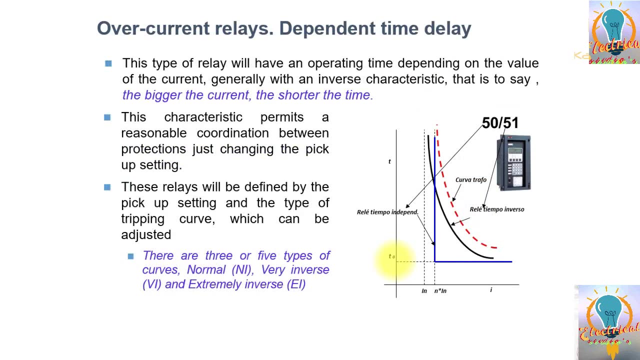 the minimum difference of time delay of 300 milliseconds to give enough time to operate this breaker. welcome friends. now we will study in this time table time dependent over current relay. these are also called as inverse time over current relay. it means that why we are calling it. 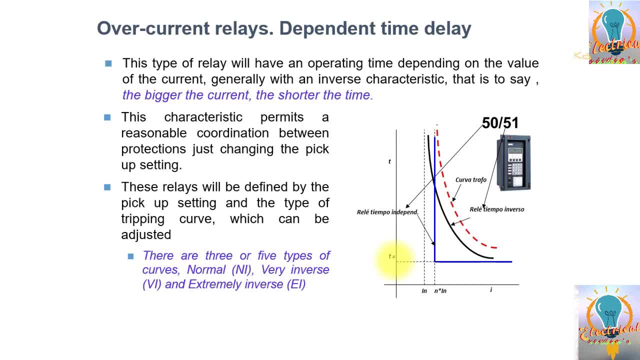 as inverse time, because if the fault current is increasing above the pickup value, more the current lesser will be the operating time. so you can see this is the curve here. ok, so this 50, 51 relay, 51 relay is basically, you can see, is inverse time. 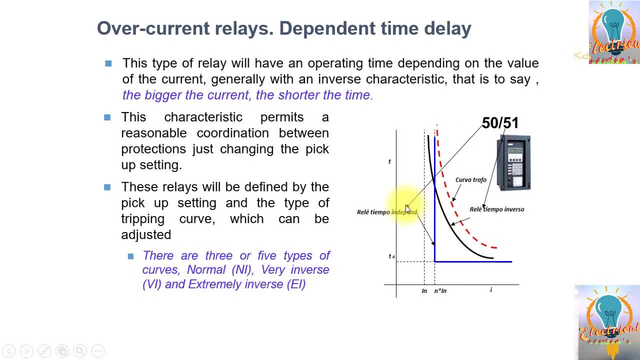 and the 50 relay is basically the definite time over current relays. so this is our pickup value. for the inverse time it is also we have set the same value, but you can see if the fault current is increasing. if the fault current is equal to n. 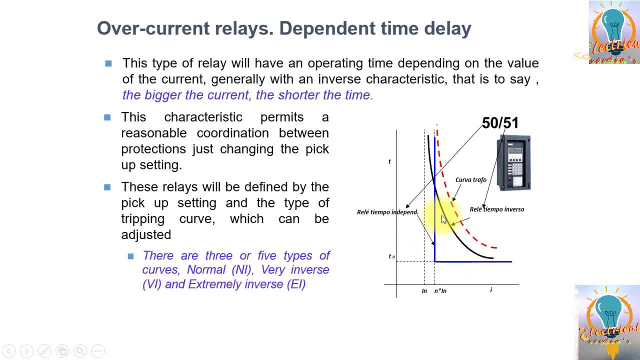 both have. this is the definite time it will trip, for example, in this time, but inverse time, as per the characteristic. the time it will take more. but if you see, if the current is increasing, you will move forward. the fault level is more. so you can see, if you see. 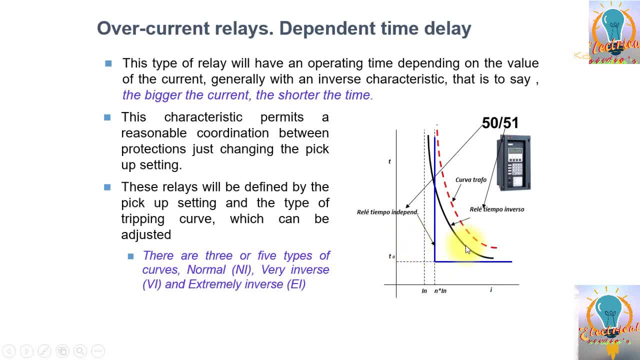 current is round about here now. the time is reduced, operating time is reduced, so similarly, as there will be more current, the time will keep on reducing. so this is example of inverse time characteristics. this is the difference between inverse time and n. from the data you can see. 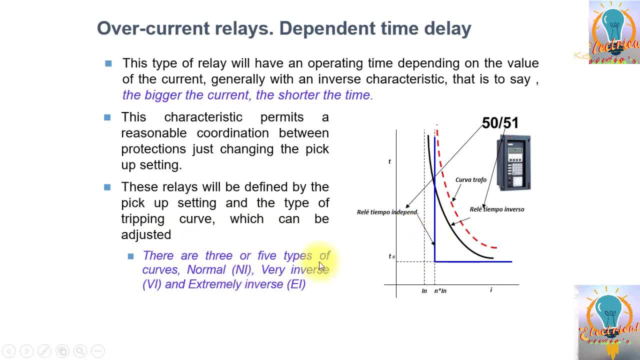 that the inverse time is the same as n, but if you see that the time is less than n, calculate this time. now I am. I will prepare a training in which I will discuss about in detail about the over current protection, all the different types and how you can do the coordination, so how you can make the 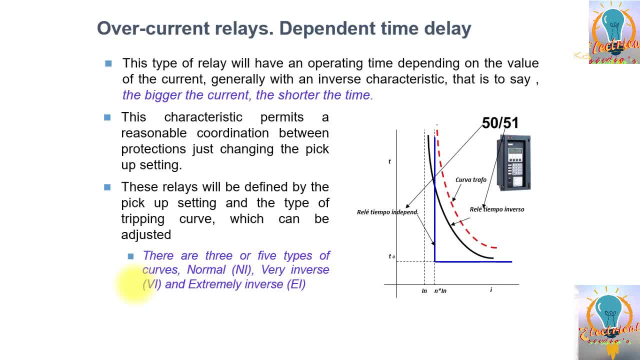 relay, coordination of an feeder. so I hope you will enroll in this training also. so this is basically, and a very simple example of all current protection that this is. we are calling it to the definite time, which is a straight line, and this is the inverse time. inverse time also has three different. 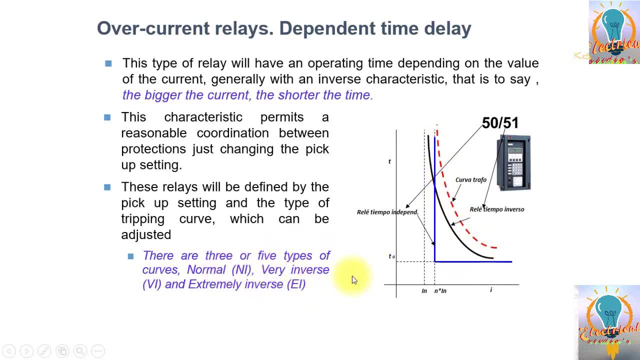 curves- normal inverse for you, most than extremely worse- and each curve time can be calculated using a formula. there are two different standard, one is there and there are two different formulas. one is NC and one is a and one is a ic. in our region we are working on ic, which is mostly used in europe, and c is used mostly in. 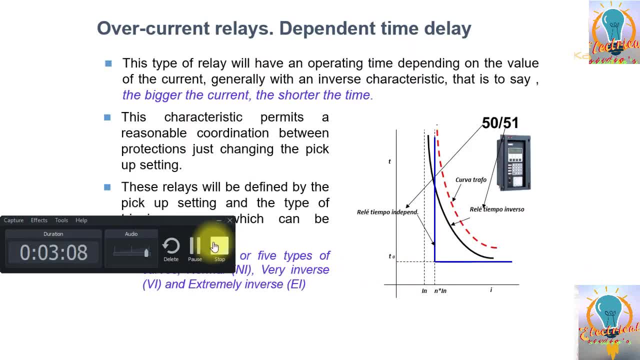 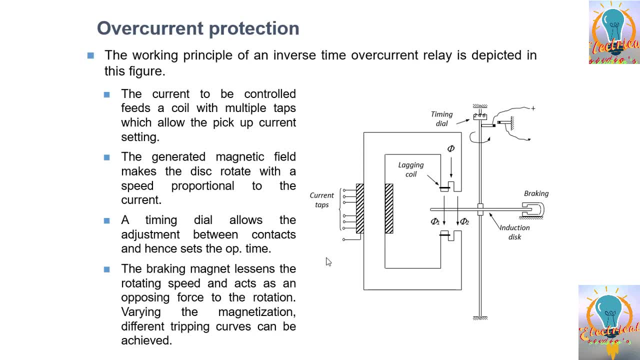 america. hey guys, now we will discuss about over current protection. uh, over current protection is a very simplest type of protection. uh, when there will uh basically like a mechanical release, then you can find a plug setting multiplier. we have just seen this picture also and you can see the. basically, the coil has provided with multiple tapes and you can. 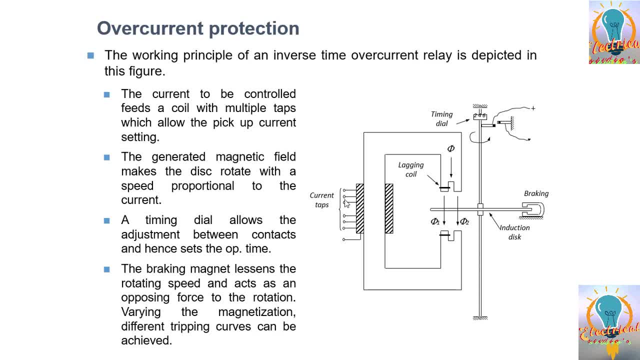 select uh, you can put a plug in between and it means that you are now changing the trend ratios and magnetic field which is applied on the disc and effectively you are changing basically here the pickup currents. so this is the induction disk type and the very famous relay is cdg relay. 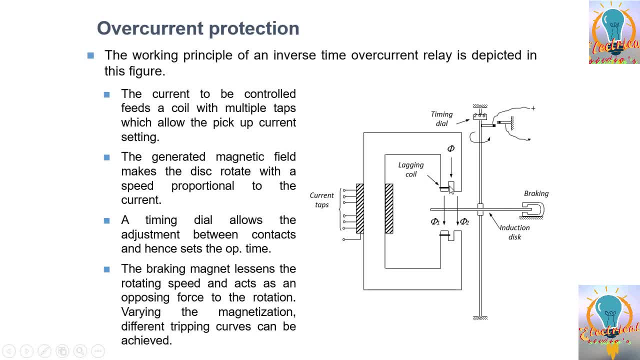 so here you can see, we have put a coil here, a lagging coil, and basically it's a coil that will make a difference of angle between flux which is going through this part and this part. so phi 1 and phi 2 will be produced. so this is all type of electromagnetic relay and you can see, this is when the disc operates. this 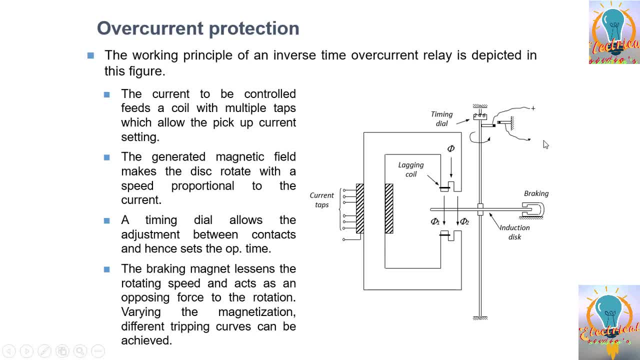 contact will make a difference of angle between the disc and the coil and then you can connect it to tripping or alarm. and this is basically where time dial setting is available, where you can choose different times. for example, if you want to have more time, then you will move the disc further and it will. it will. 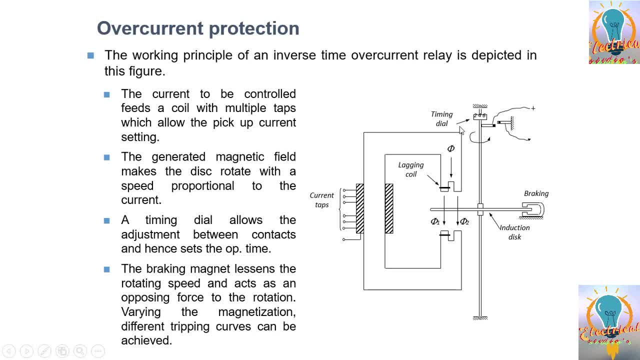 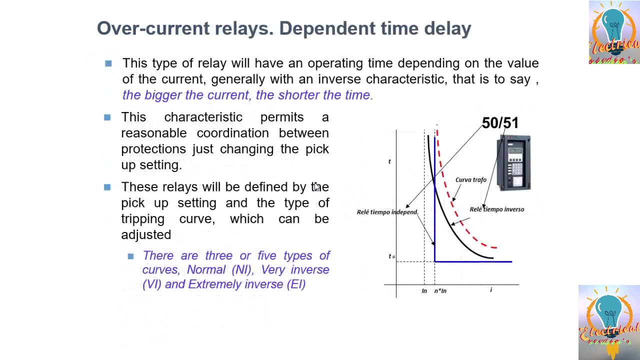 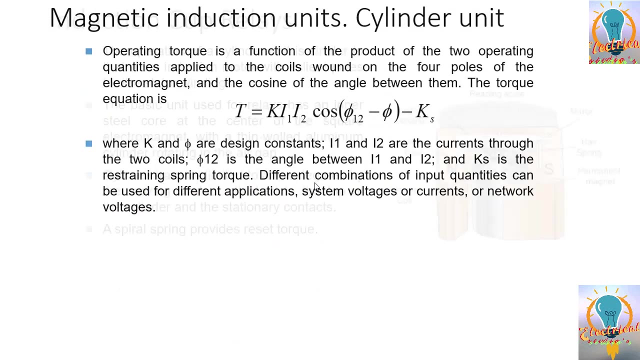 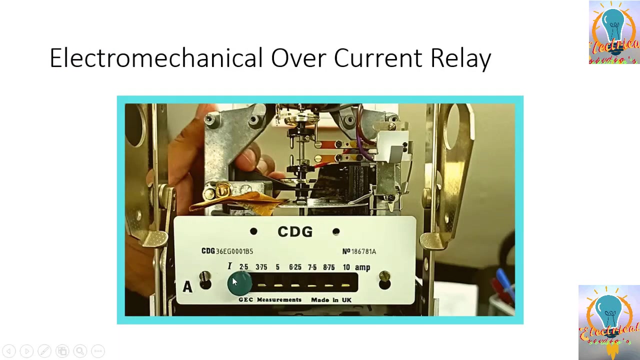 take more time to travel and then it will allow you more delay. so it is called as time dial setting and it is called as a plug setting multiplier. so let me go back and show you the cbg relay. so this is the relay that i have explained you. this is basically the 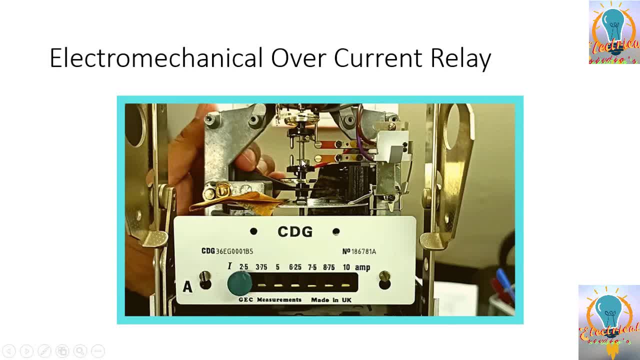 plug setting multiplier that i have shown you in the drawing, and on the top here you can find the time setting multiplier. this is basically a coil type spring which will reset the contact and reset the disc and the fault is reset and these are the contacts and that will operate. so this is basically the 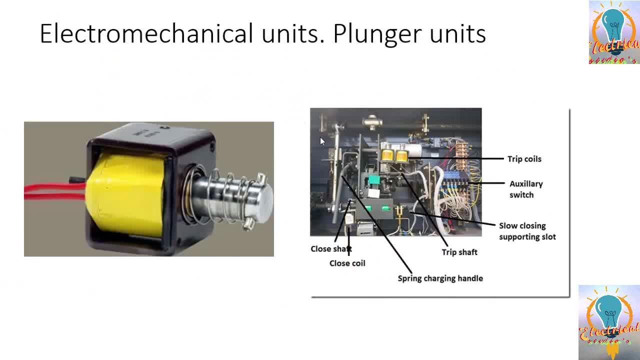 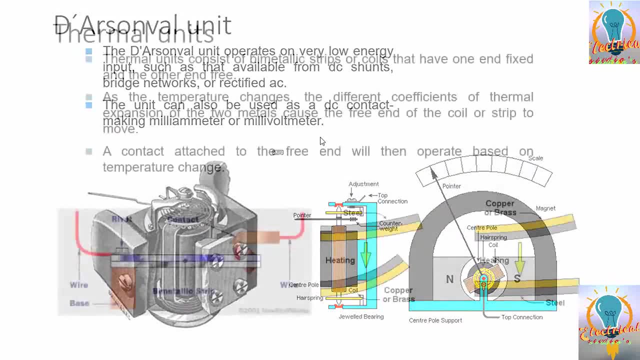 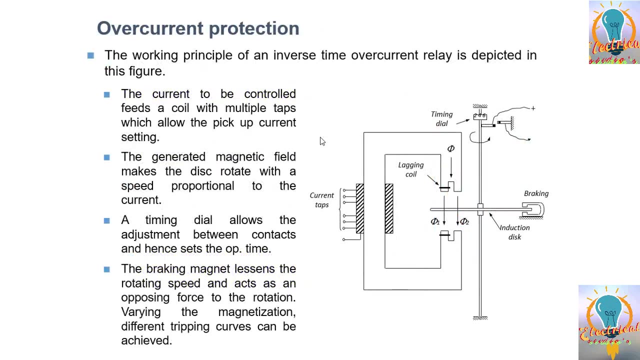 old type of relay, but nowadays the modern relays are microprocessor based relays. just have to configure in the relay, just have to put the value- pickup value- and the relay itself will do all the calculations and it will do all the trippings. and it's very 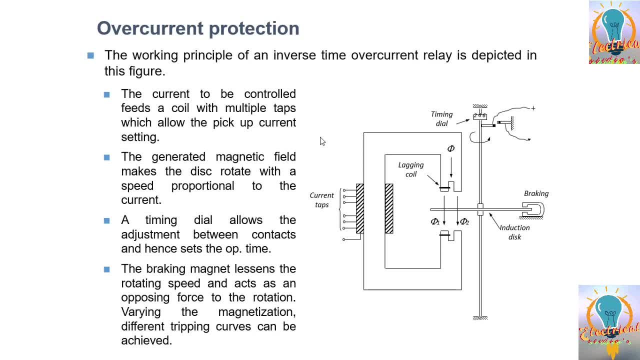 simple. so this is how the over current protection works and it the over current protection normally has two types: one we have seen, one is a definite time. one is in your spine, so inverse time, the nc code is 51 and for the definite time, the nc code is taken as a 5: 0.. 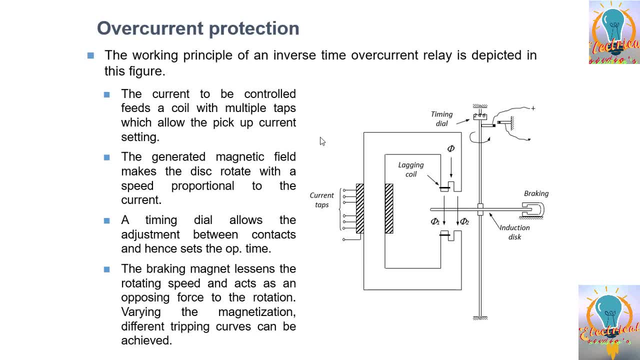 so other types of protection we can define as work phase over current. we are calling it a phase over current and earth fault over current. so if there is a phase to ground fault, the earth fault over current will operate and if there is a phase to phase fault and phase over current will pick and 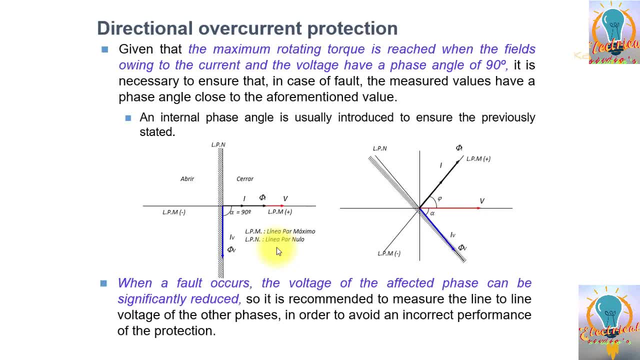 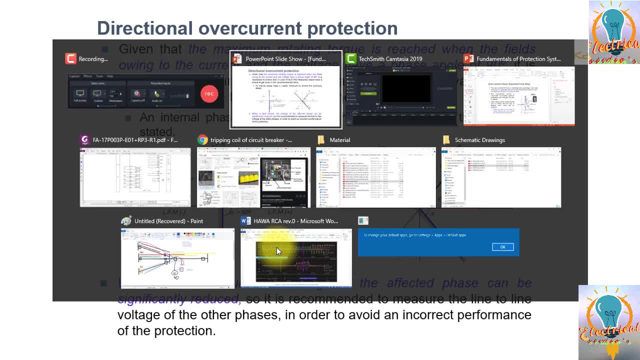 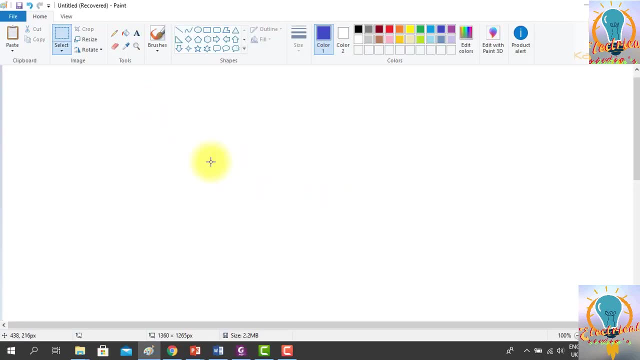 operate it. hi friends, in this section we will study a little bit about the direction over kind protection. so let's now discuss on a board: so what direction organ protection is doing? so let us understand this. this is, for example, a bus bar and this is the line. 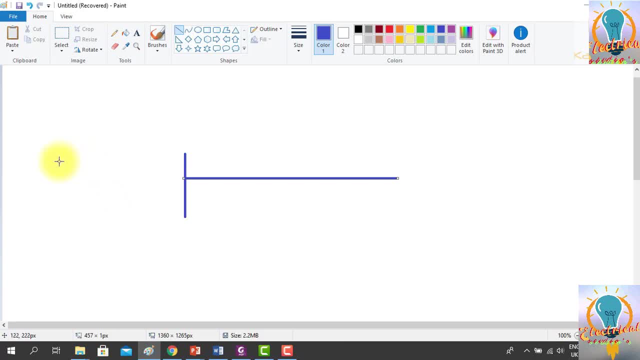 from the outside. and this is the station a. okay, and this is the station a and this is the station b. or we can make here a transformer. so, for example, here we can make a breaker. here this is an outgoing feeder, this is an incoming feeder. so if we install a, 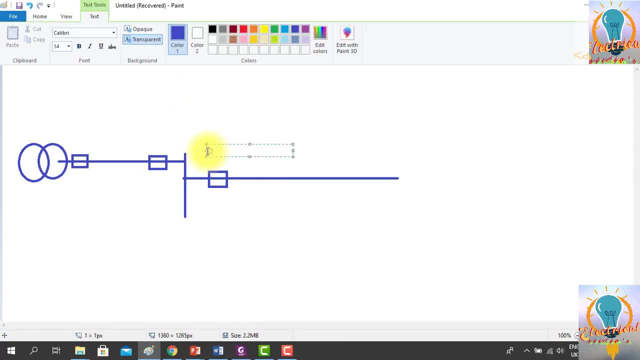 directional over current. here it is called as directional over current at fault. so what will happen? that this relay will not only see the level of current, but also it will see the direction of current is flowing to make the decision. so let's go. the setting of the relay here is zero. okay, one amp and this relay 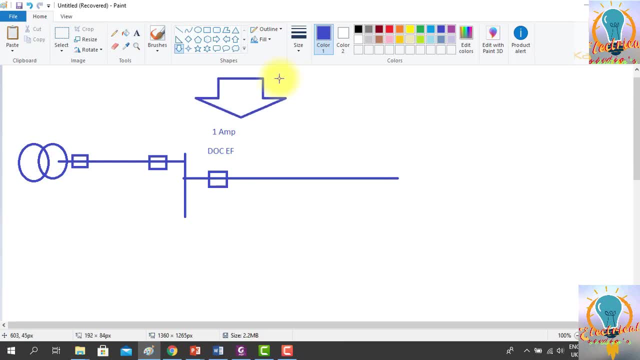 is direction of this relay is basically this relay is seeing the fault in this direction, the forward direction. so if there is a fault here, for example there is a fault here, this relay will sense the fault level, it will check. it should be more than 1 amp here. 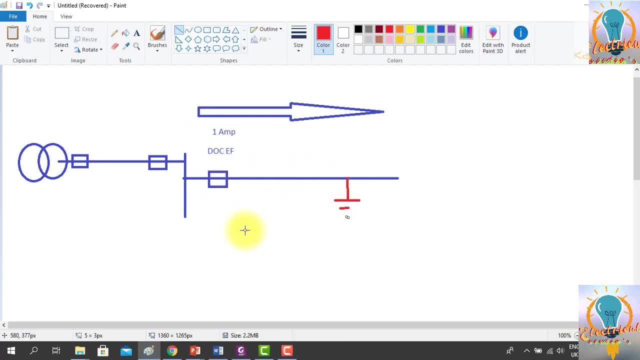 and it would track the direction of current. if it is in power direction, then this relay will operate and trip. what if the fault is in the back side here and, for example, normally DF is installed where on the generation side, so we have a generator here, so the fault 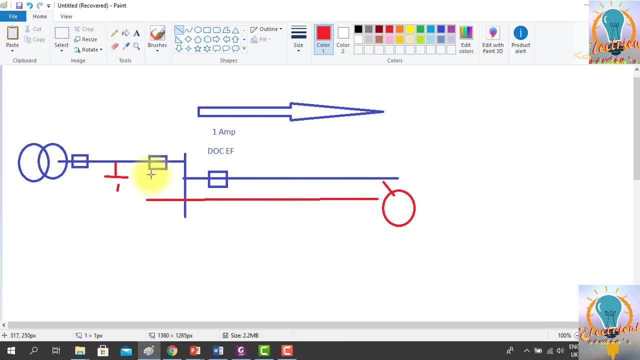 will be feed by this generator, okay, and then the current will flow through this over current relay. but now relay will sense that direction of current is not the forward but the reverse direction. current is the reverse. the current level is more than 1 ampere, but the direction of current is not. 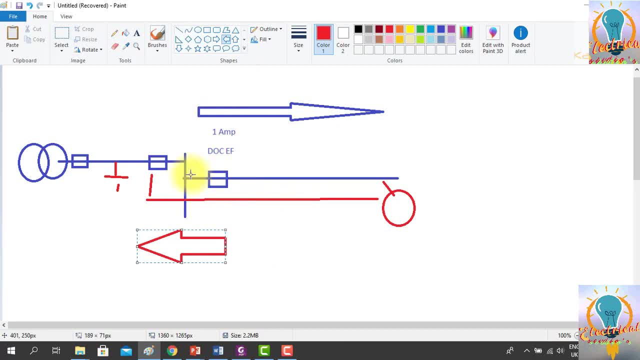 forward. so this relay will not operate and it will protect this generator too, out of network. so, for example, if we have more than one feeder here, if we have more feeder, this other field is applying to another area. so this relay will trip. okay, it will sense a fault and it will make a trip and this 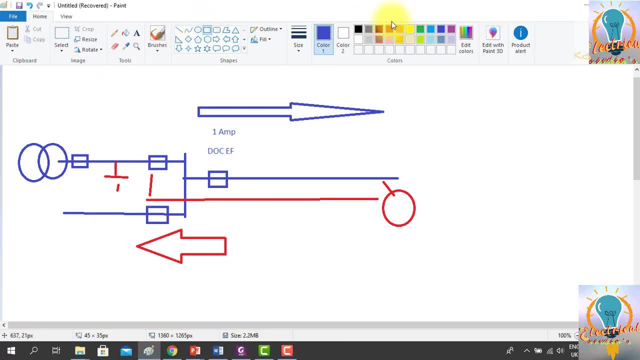 portion will be isolated. so this portion will be isolated in this case, when this trips. so this region has tripped, the breaker has open and then this region is isolated, but this generator is keep on feeding the to the, to the load, to the network. so this is a 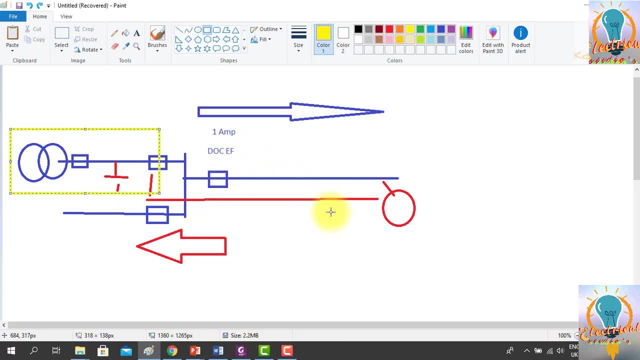 advantage of directional earth fault. so if the fault was here in the forward direction. now generator cannot feed to the network. you have to isolate this breaker. that will operate and it will isolate the network. it will trip this breaker and if there is a breaker here on this area, it will. it can. 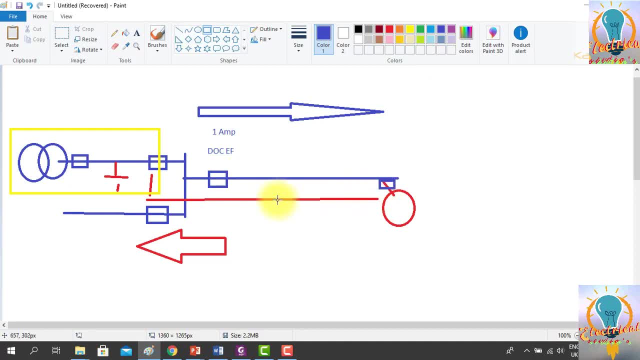 also trip this breaker by direction, by G to V, or if the depth installed here which is looking in this direction, it will trip. or we can even install here novel over country, because the direction of port will not change here. so this is basically the concept of using directional earth fault relay on the 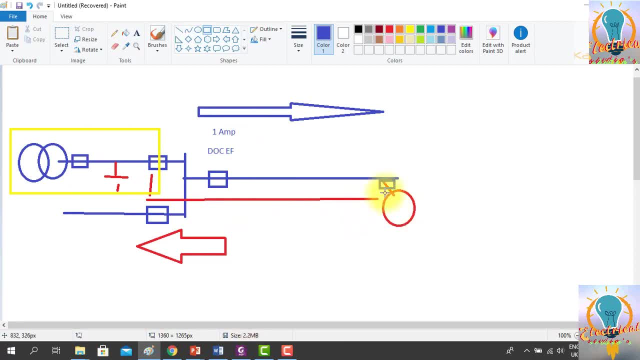 network. the advantages: mostly it is used with a out feeder that has a generation. so now there is a sense of fault, the direction of fault, either in forward or reverse, and how they relate direction. earth fault relay is accessing the part is because one input of this relay is CT. okay for. 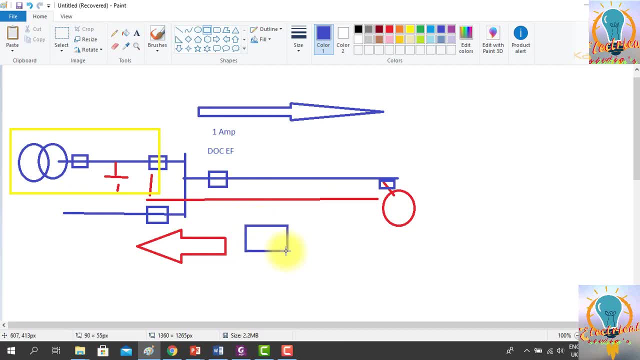 example, this is the directional earth fault relay. this is our directional earth fault relay and it is connected to a CT here and also it is connected to a VT, so it is checking angle between voltage and current- voltage and current- in order to determine the direction of current flow. So this is the working principle of DEF and why this DEF is. 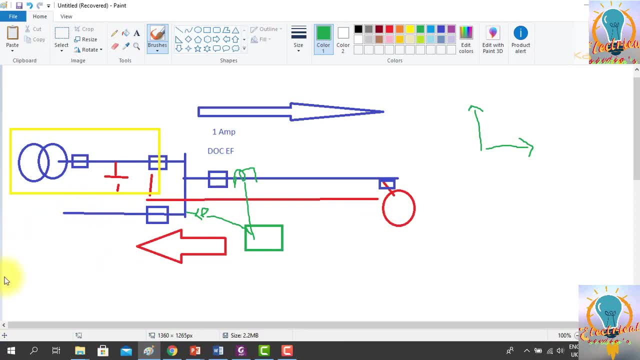 very important. So this DEF feature is similar to a distance protection 21, which also work in forward and reverse directions, but it is a cheaper solution. mostly it is installed on the 11 kV and 33 kV unit of feeders where generation is connected, So the generator should not trip. 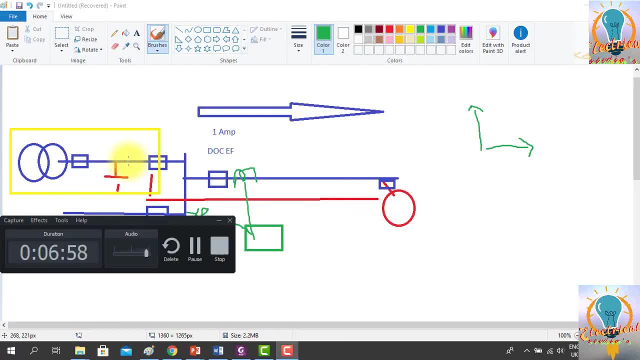 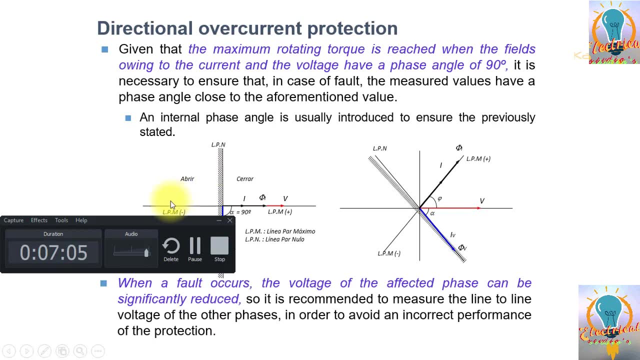 if the fault is in the reverse direction. So here we can go through some theory. Given that the maximum rotating torque is reached when the field, owing to the current and voltage, have phase angle of 90 degrees, it is necessary to ensure that, in case of fault, major values have a phase angle close to the aforementioned. 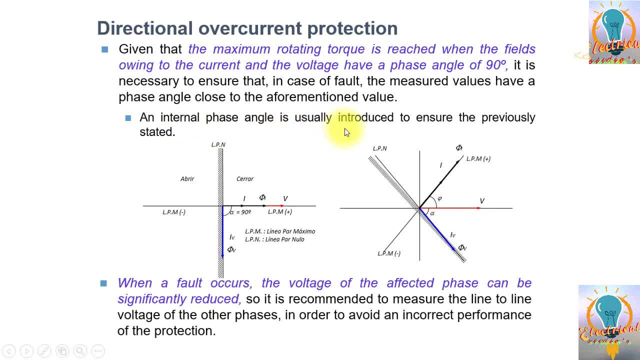 value. An internal phase angle is usually produced to ensure that was previously stated. When a fault occurs, the voltage of the affected phase can be significantly reduced. so it is recommended to measure the line to line voltage of the other phase in order to avoid the incorrect performance of the. 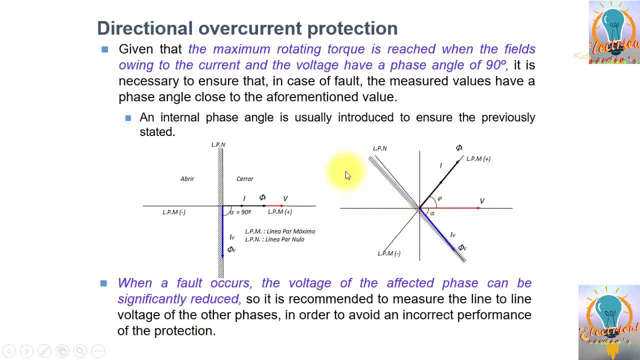 protection. So when there is a fault on, for example, red phase, red to yellow phase or red phase to ground, normally the other phase voltage is used, because the the phase which has the fault, the voltage will obviously goes down. so it is called as cross polarization and the polarizing quantity is, in this case is a voltage. 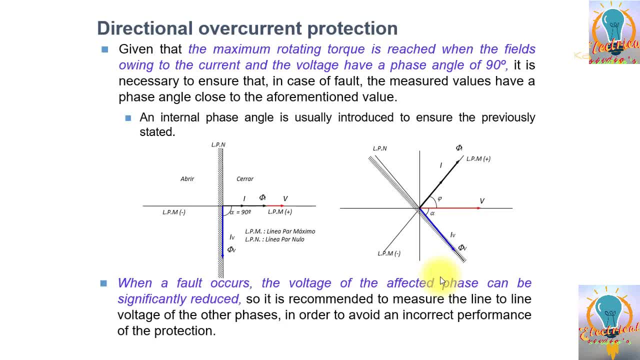 which is giving the sense of direction to the relay. So the angle at at the, at which the maximum torque torque is produced, it is called as MTA, maximum torque angle, and in the relay you can say they are doing some some day, using some method to adjust the angle to maximum 90 degrees. So this is some basic concept of 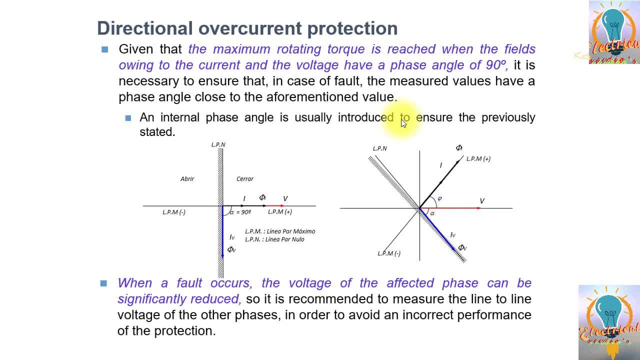 directional earth fault, directional over current relay and directional earth fault. also you have the option of using the polarizing quantity a 3V0. basically, in 3V0 you are connecting all three voltages, all three VT windings in series together. but you 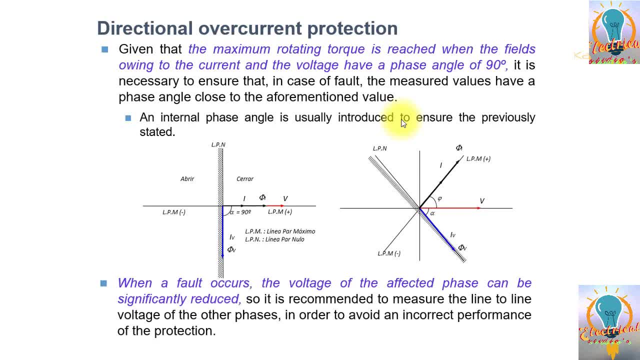 are not closing a Delta and this Delta will be connected to to the relay. so normally when the system is healthy our three phase voltages will be balanced and there will be some will be zero. so 3V0 in the normal condition will be zero. but when there is a phase two ground fault, this three V 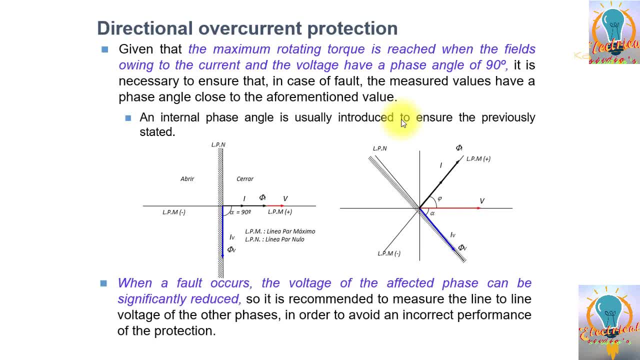 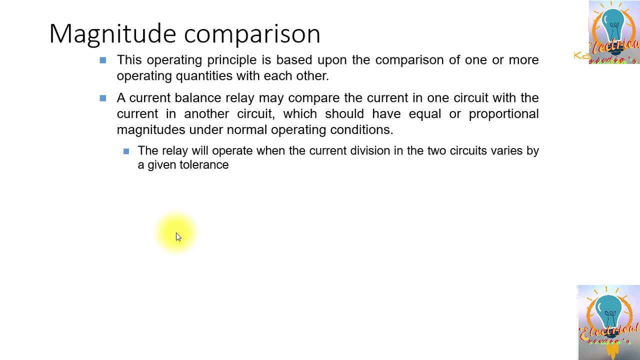 naught will have some value and it will used as a polarizing quantity for the sense of direction to the direction arc fault relay. welcome friends. in this section we will study another type of protection is basically a magnitude comparison. so basically in this, this type of protection is basically checking. 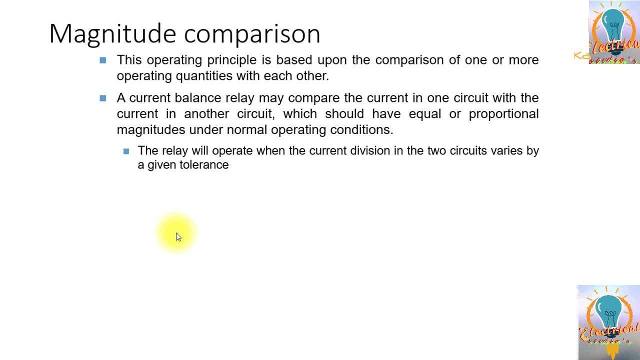 the magnitude between a and B. so the focus is on the magnitude. we are not taking care here about the angle. so the current balance relay may operate the current in one circuit with the current in another circuit which should have equal or proportional magnitude under normal operating conditions. the relay 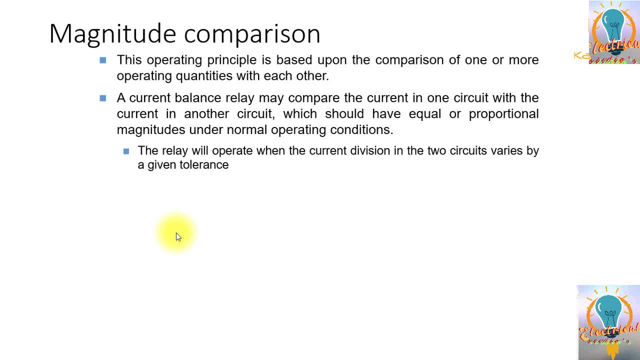 will operate when current division in the two circuits varies by given tolerance. so example could be example: if you have a three-phase motor, the normally all three phase should draw similar currents. so we can have a relay which monitor all three phases- magnitude, not not the angle, and if there is a significant, significant difference and 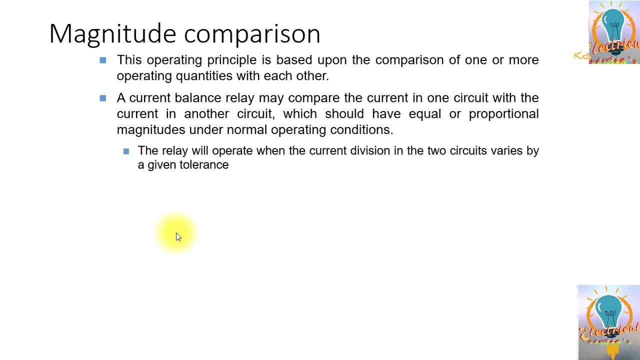 stage one, it could have relay issue the alarm, and then stage two, it will issue the trip, because if one phase is out the relay could damage same. same we can apply on the generators. so all the generators are going to be in one circuit. so the two are designed to run on certain unbalanced, if the unbalance is. 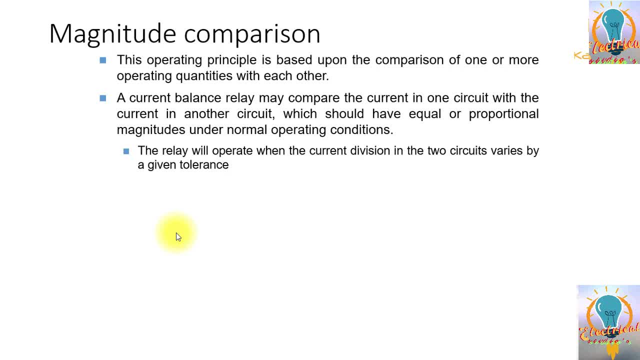 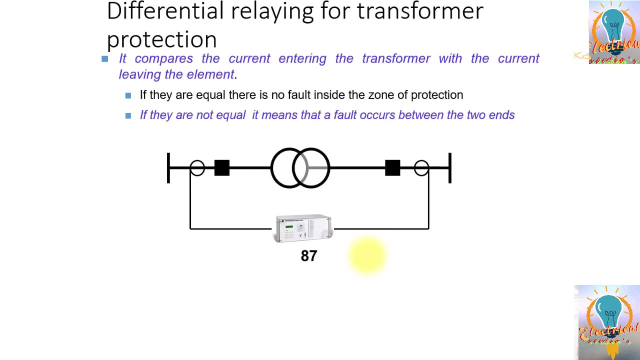 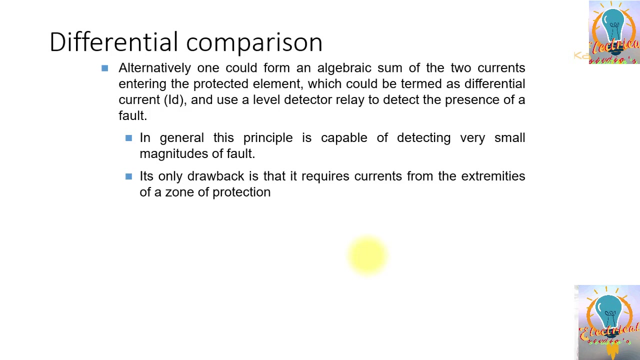 more so it it it will damage the generator. so this is the one principle of magnitude comparison units. so another type of technique that is used is basically the differential comparison systems. so in this way, alternatively, one could form an algebraic sum of two current entering the protected element, which could be termed as differential. 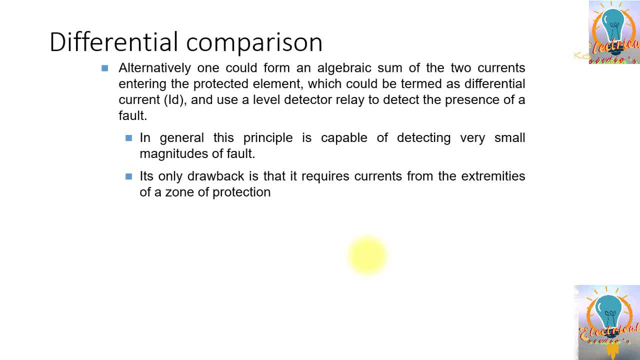 current and use a level detector relay to detect the presence of fault. in general, this first principle is capable of detecting very small magnitude of fault. his only drawback is that it requires current from extreme of our zone of protection. so nowadays, the differential protection working principle, a transformer, different production, is. 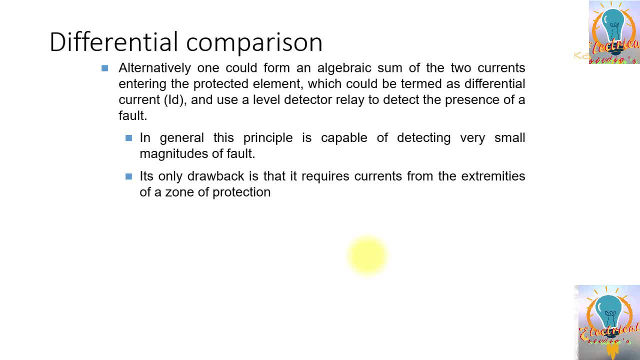 working. so advantage of transfer differential protection is that and the HPCT is an LV CDs. both are in the same substations. but if you talk about the differential protection of a line that we are talking about now, is that you once it is available at local and and other cities, available at remote and previously. 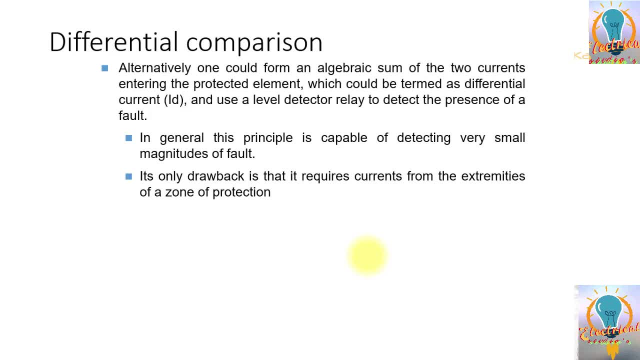 it was difficult because the release were not that much modern, but now it's also very simple. the release are both line differential. relays are connected through a fiber optic and they are communicating all the CD data through fiber optic to each other and then in the release working satisfactorily and line differential is. 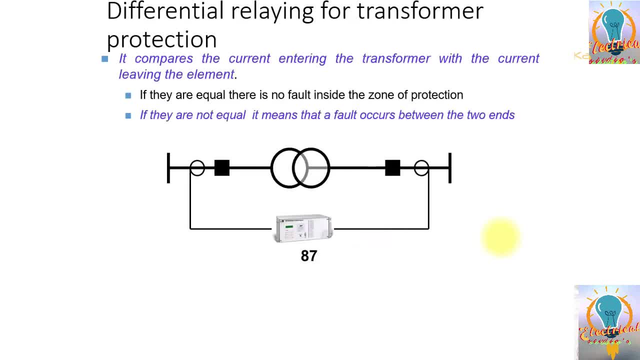 working fine. so here you can see differential protection principle for we. if you consider for the transformer, same will be the line. so it compares the current entering the transformer with the current leaving the element. if the if they are equal, there is no fault inside the zone of protection. if they are not equal, it means the fault occurs between: 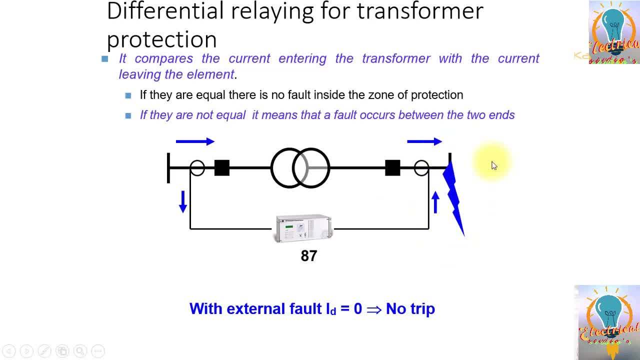 the two ends. so this is a case one. here you can see the fault is outside of the zone: current entering and current leaving. both are the same because there is only case between. so there will be a zero differential here in the relay and the relay will not operate. 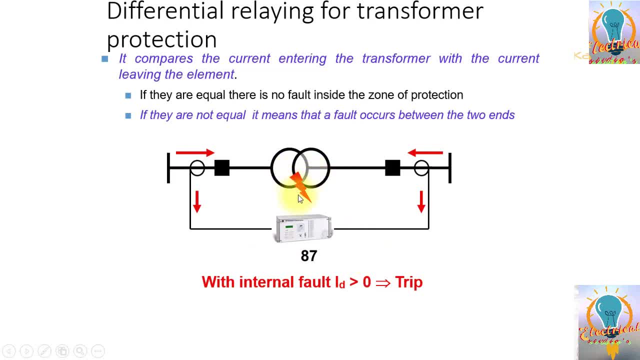 Differential here in the relay and the relay will not operate. so this is the case to. we have a fault on the transformer face to ground fault or transformer failure. so you can see, the current will enter from the both direction and it will add up in the relay. 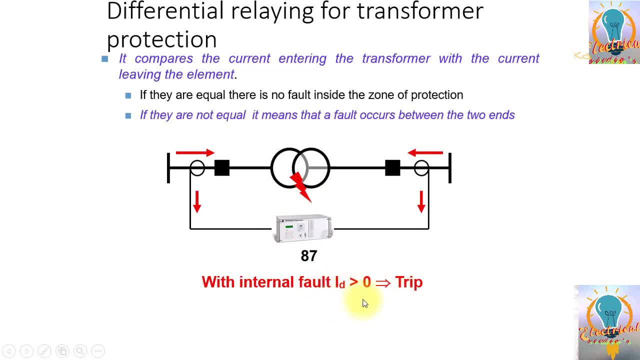 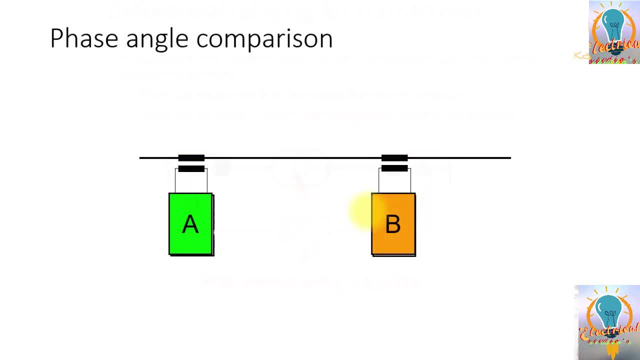 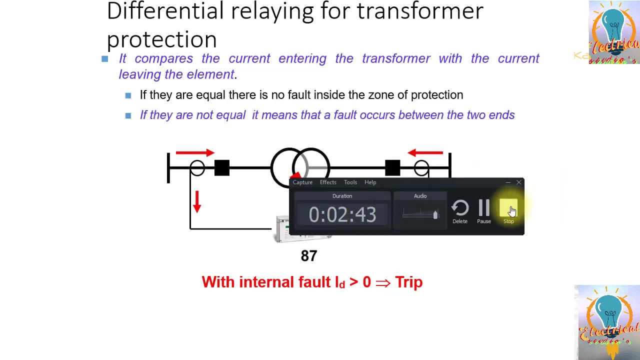 so the relay will operate and differential is greater than the zero and greater than the set value, the differential will operate and it will make a trip. so this is a very simple explanation of differential relay. thank you very much. phase angle comparison release. these are one of the very interesting release that we 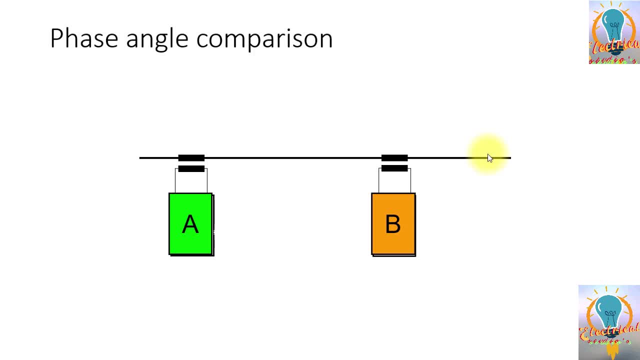 used to used to be used before, but now we are seeing lesser this type of relays in the field. so just consider: this is a station A and station B. there are two stations so the relay will check the phase angle of the station A, for example, that quantity of current with 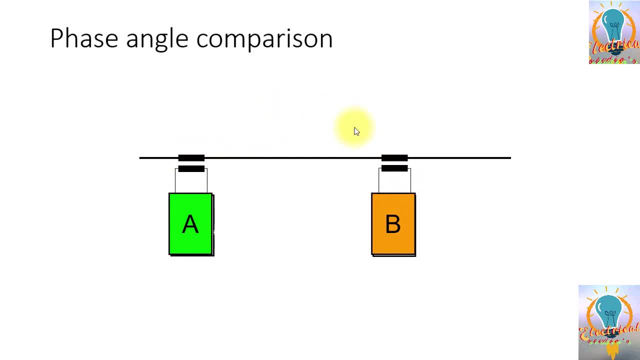 the station B current. so it will check the phase angle of the both stations. so you can see the direction of current will be from A to B and the direction of current we you can see, is in this direction, from A to B. now if there is a fault in between these feeders, the fault will be feed by both the 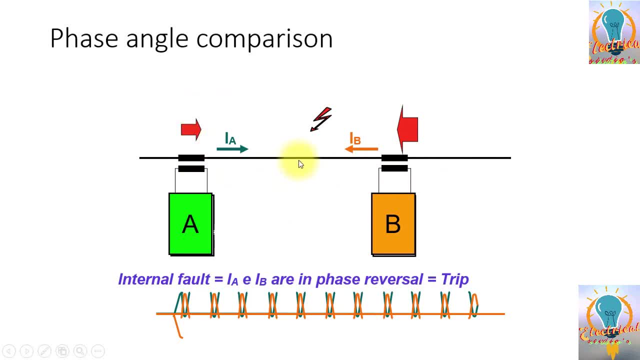 both directions. so you can see here: the phase angle will be out of phase by 180 degrees, so there is a phase reversal. the relay will sense the, the phase angle of the two quantities under observation. the current of A and B is now reversed, which means only that there is a fault. so then relay will issue a trip command. 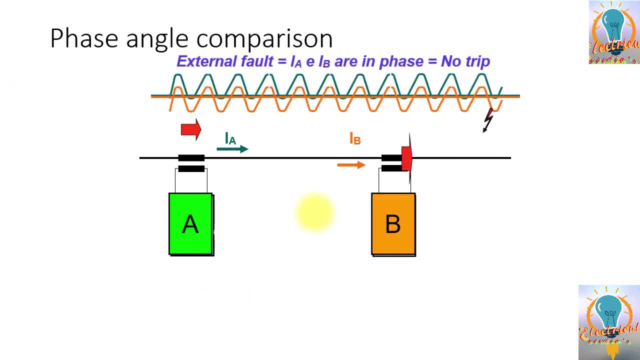 so the relay will issue a trip command. so the relay will issue a trip command. so so Now you can see if the fault is outside this zone. A and B. So the direction of current in the both station will be the same. So the fault between and and the direction will be same. the phase angle of the A and B quantities on the both. 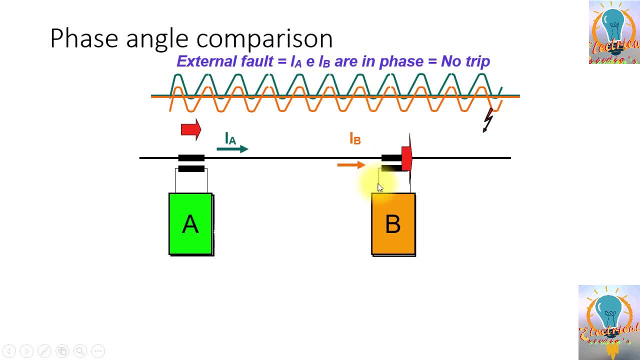 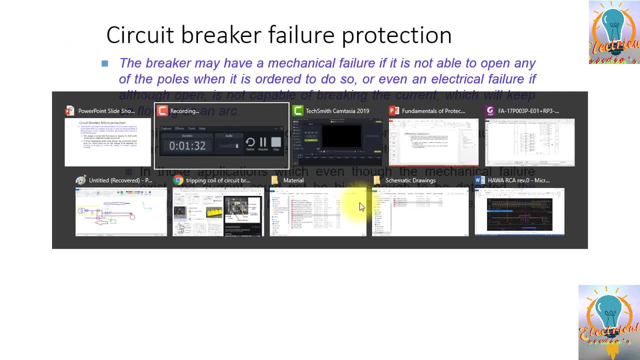 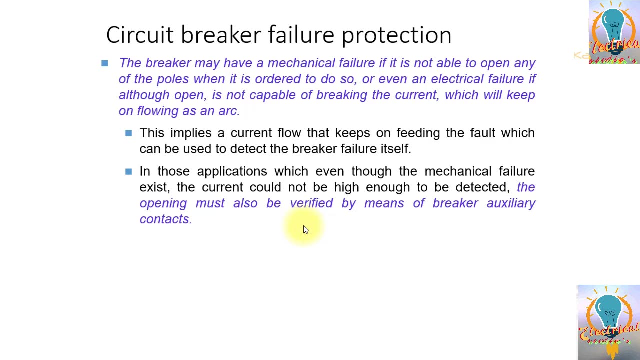 Substation will be in phase and hence no trip will be issued. So this is a concept of phase angle comparison protection release. Thank you very much, Hi friends. in this section we will study about one different kind of protection, which is called as a circuit breaker failure protection. 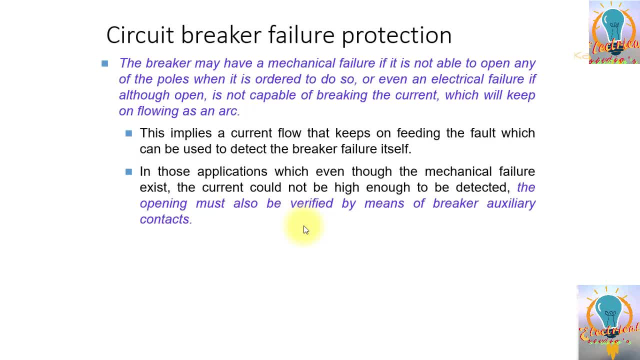 So the breaker may have a mechanical failure If it is not able to open any of the poles when it is ordered to do so, or even electrical failure If, if, although open, is not capable of breaking the current, which will keep on flowing as an arc, So another type of failure could be. 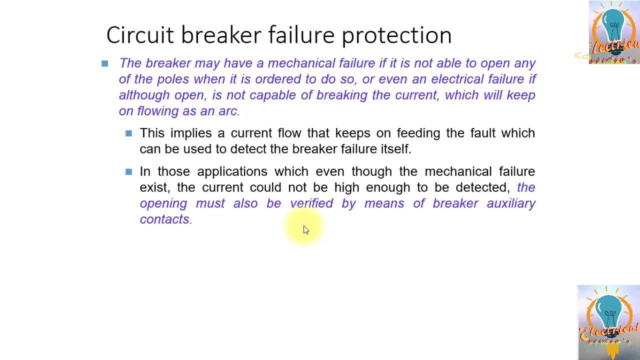 failure of SF6 lockout because if SF6 breakers, if the gas is low, stage 1, there will be an RM. in stage 2 The gas will be released more and it's dangerous to operate the breaker. So breaker will be in lockout stage. 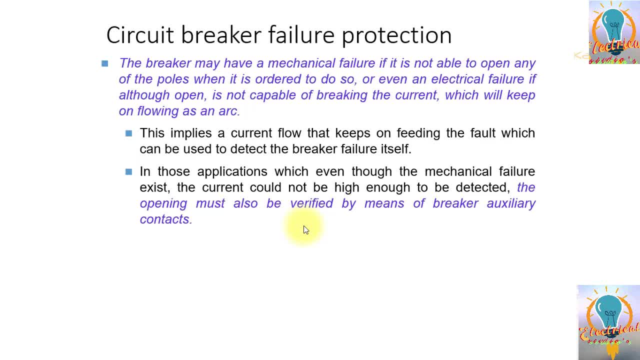 So this is another form of breaker failure protection. This implies a current flow that keep on feeding the fault, which can be used to detect the breaker failure itself. So the relay breaker field is really monitoring the status of the contact- Auxiliary contact- of the breaker and also it is monitoring the current 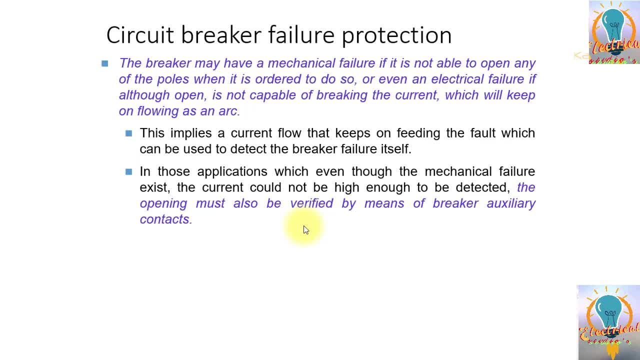 Since the failure could be electrical or it could be mechanical. It is possible that the breaker is open mechanically but arc is not quenched and The current is still flowing through the breaker. so in this case the breaker failure will detect it as a fault and the failure of the circuit breaker, and then it will in stage 1 it will try to. 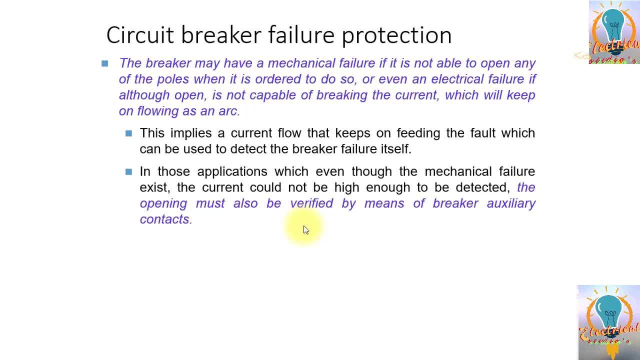 Retrip the breaker, it will give tripping commands to TC 1 and TC 2, to coil 1 & 2 and, in stage 2, It will trip the feeding sources in These. so those application which, even though a mechanical failure exists, the current could. 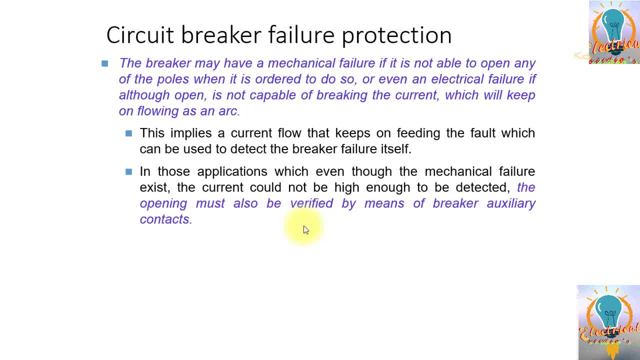 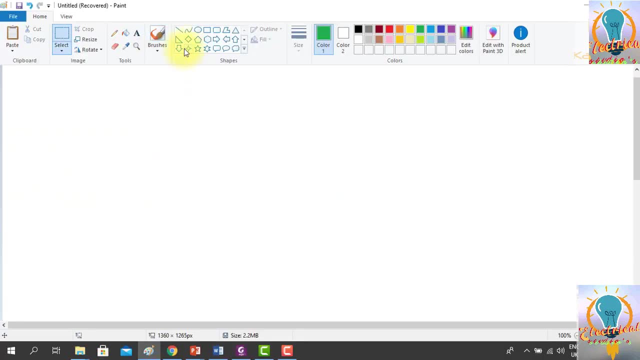 The current could not be high enough to be deducted. The opening must also be verified by mean of breaker auxiliary contacts. So let's go to our board. So now let's consider the case here. So for example, we have here: okay, I will open. can I open this? 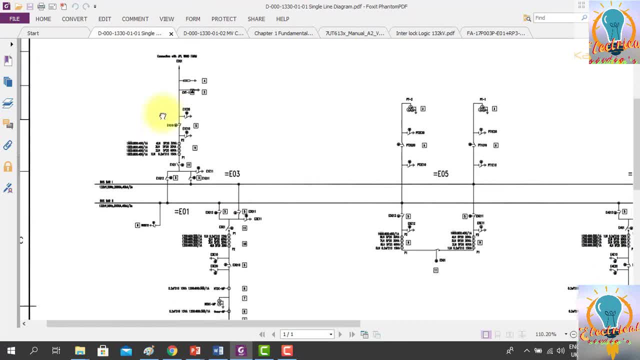 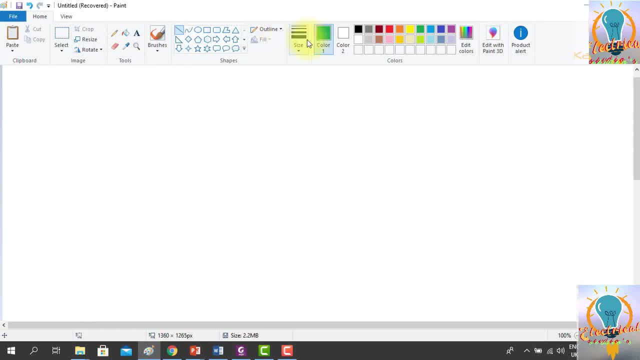 single line diagram. Okay, Okay, so better to draw on Paint. it's easier to understand, so I will select. first of all, I will draw the bus bar, For example. This is the bus bar And this is one feeder. this is, for example, another feeder connected to the bus. this is another feeder. 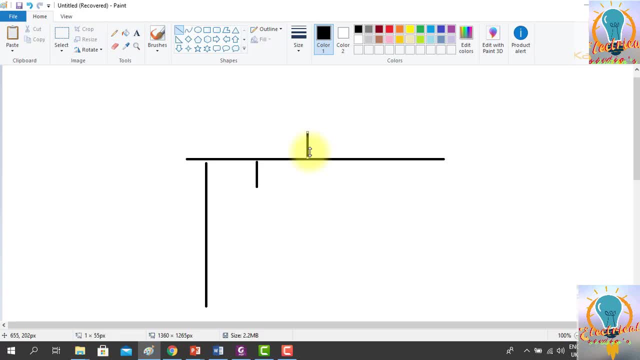 Connected to the bus. These are all feeding to the bus and we can then draw the breakers. so we can draw the breakers. excuse me for some bad drawings. I'll try to. I'm trying to improve this section also, but it will take some time. so this is basically the bus bar and it is feed. 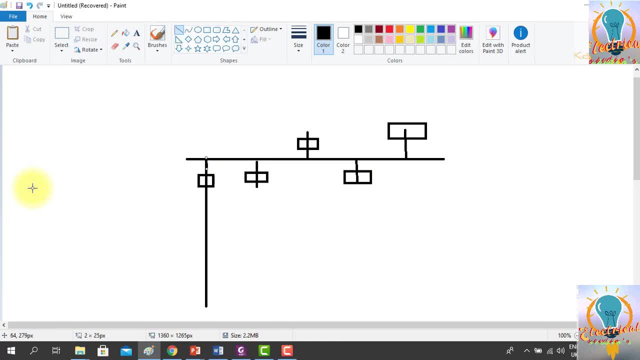 by different breakers. so we will understand you can. there is a fault, for example, here on the line. so we will consider a case where we have a double bus and single breaker scheme here. you can see this line can be connected to pass if you close. this is a later it to connect to the bus 1 and 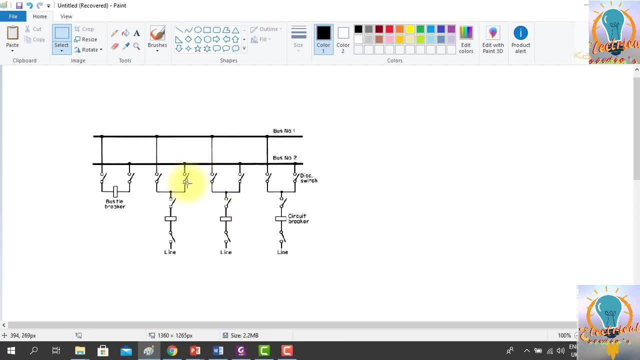 if you close, this is greater. the line will be connected to bus 2 and further. we can have different connections that we can make. so we will first of all make connections. I will connect line 1 to bus 1. so let's close this isolator. so here we have: close the isolator. 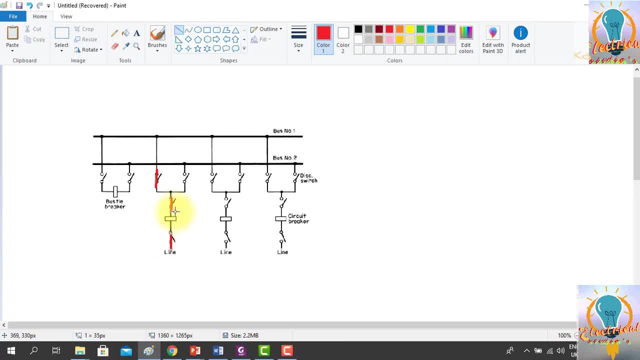 and the line insulator. so it means this line is connected to bus 1 and this line is connected to also bus 1. this feeder is connected to bus 2, line 2 is connected to bus 2 and coupler is also connected. so here I have make a initial configuration. so 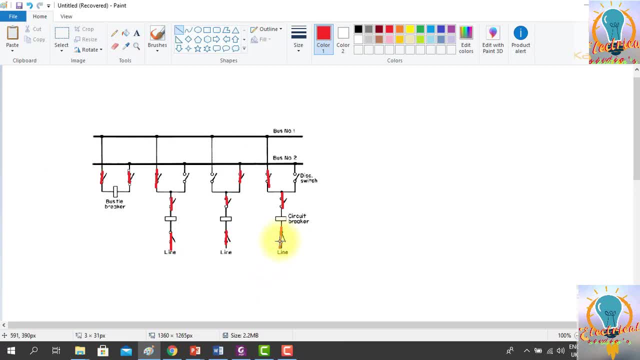 we will consider a fault on this line. okay, if we consider this line has a fault, fault on this line, this line, etc. line 3, for example, this is line 1, this is line 2 and there is a fault on line 3, we will. 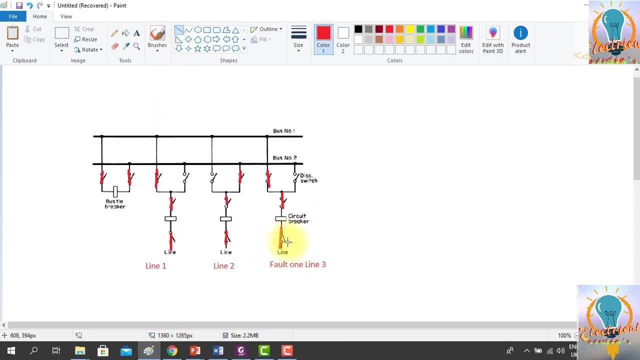 assume that there is a fault phase to ground fault here on the line. okay, there is phase to ground fault on the line and the relay of this line, line 3, will pick up and it will issue the trip command. okay, so whenever any protection relay pick up, this is our breaker failure. 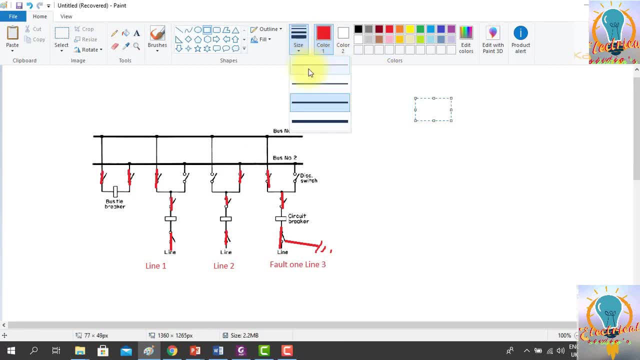 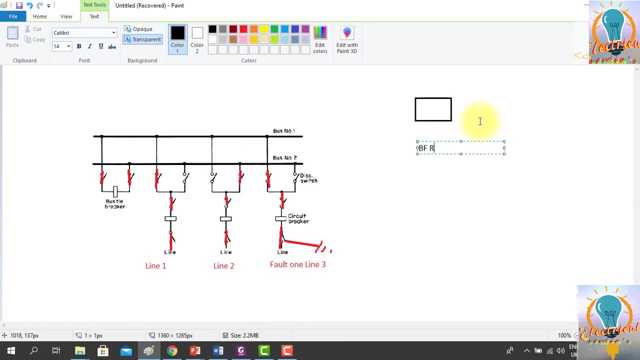 protection really. for example, this is breaker failure. also, you write BF- really, so this breaker failure. this for protection relay, line protection, relay, distance. for example, we have here distance relay which is protecting line 3, distance 21. we need to resize it. okay, this way will issue the trip command to the circuit breaker, but circuit breaker we will. 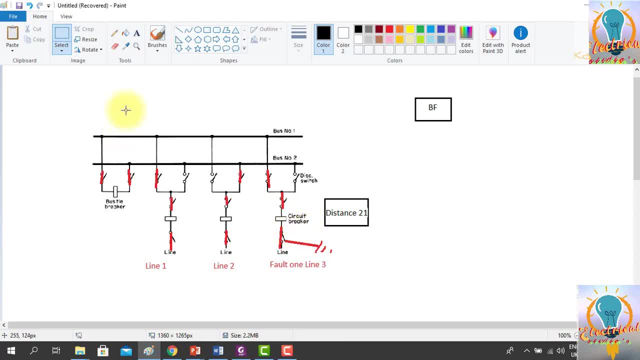 consider that this circuit breaker is failed. so it means that still fault current is flowing to the ground. so loop of the fault current will be from bus 1 to the breaker to the ground. so this is the fault current which is still flowing in the ground. it irrespective that the circuit breaker is. 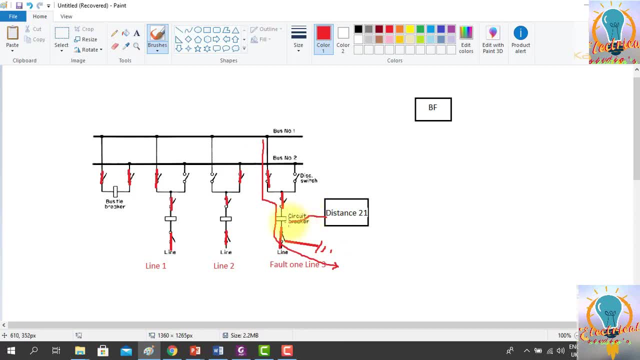 found, irrespective that distance layer has issued the trip command, the breaker is not open. so this breaker is faulty. so we will mark this breaker as faulty. so this breaker failed to open. when the protection relay gives the strip command, at the same time the protection relay also give initiation to the breaker. failure protection, really. so it will. 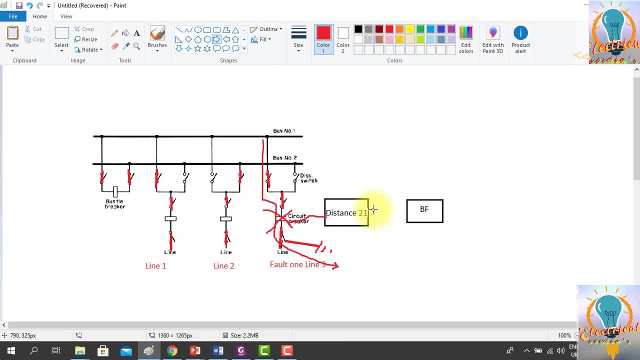 give initiation to the protection that you should be ready and start pick up when the relay breaker failure really initiate. it will get initiation signal from the distance main protection relay. it will start a timer. so it's getting a current input from the CT. so let's draw a CT here. 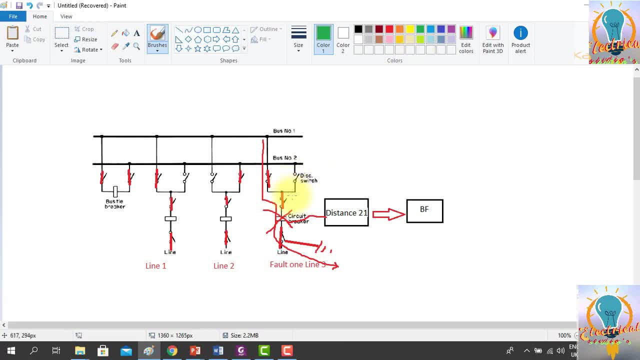 so, for example, CT is available here. let's choose a green color for CT. and CT is connected to distance and also it's connected to breaker failure and then at the end it is grounded. so now relay breaker failure relay is getting initiation signal. so initiation means at least one of the protection relay should picked up means some. 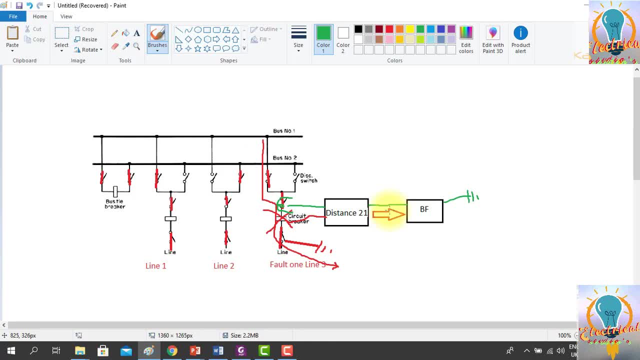 fault has happened and protection relay has operated already. so this is information, is now feed to breaker failure, relay breaker failure, at the same time monitoring the current. if the current is reset, the relay will understand that now this breaker has operated successfully and then no need to continue the timer. the timer will stop. 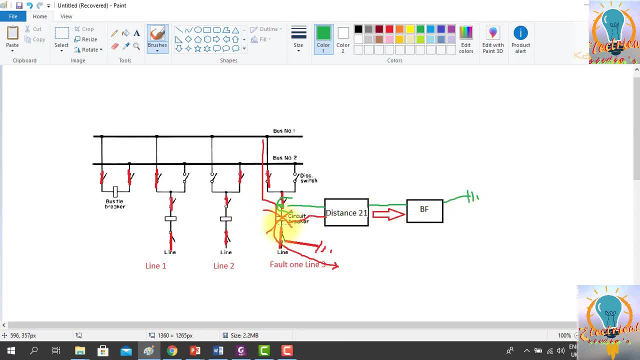 but if, for example, in our case, the breaker is failed, the current fault current is still flowing. it means the relay is also picked up. they will not reset. if the fault current is there, relay will not reset. so this initiation, BF initiation, so the one quantity is BF: any 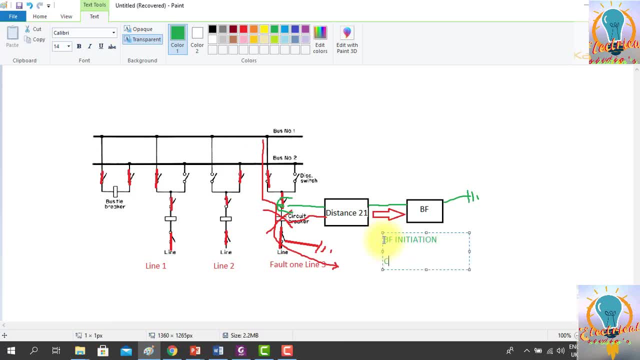 cation and current pickup. both are there, so timer will be continued, so predefined after predefined time delay, for example. so BF stage one is 100 milliseconds and BF two is stage two is 200 milliseconds. so in the stage one, in the stage one, the BF relay 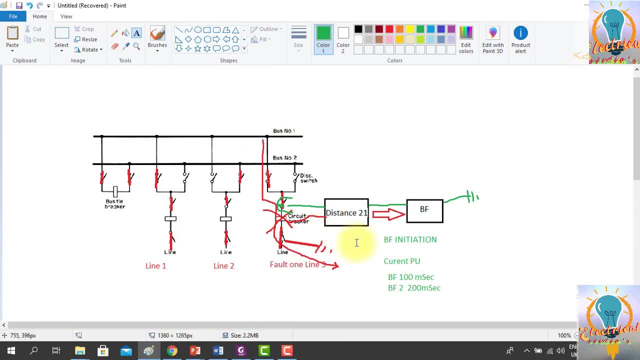 after 100 ms are passed, the stage relay could be 100 to 150 ms. the stage 1 is passed, the BF will relay in stage 1 re-trip command. it will try to same breaker. it will try to trip it again. 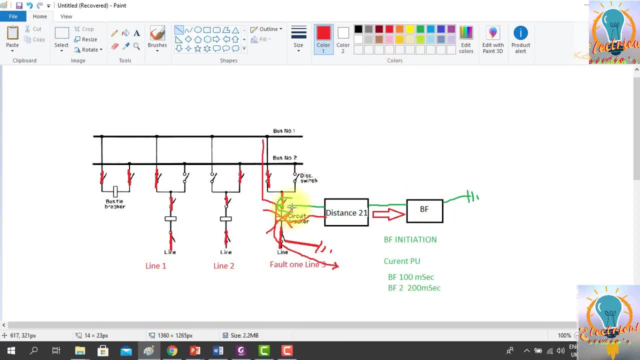 in fact, in this scheme it will send trip command to TC1 and TC2 at the same time, so it will try to re-trip the breaker in stage 1, so that if the breaker is tripped then fault will be isolated. 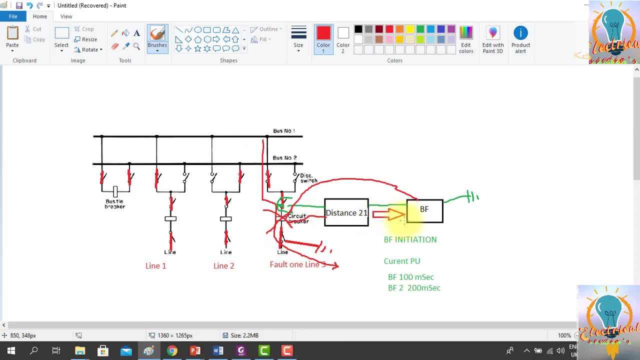 if the fault is still not isolated and the pickup is still not reset- the current is still there- then the relay will go into the stage 2, differential breaker failure, differential protection will go into the stage 2, and stage 2, what? 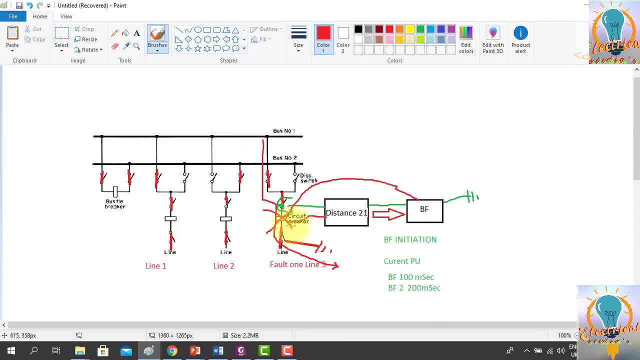 it has to do is in stage 2, the basic principle that you have to understand for the breaker failure is you have to isolate all the possible sources which are feeding the fault. so what are the possible sources? source 1 is this bus 1. 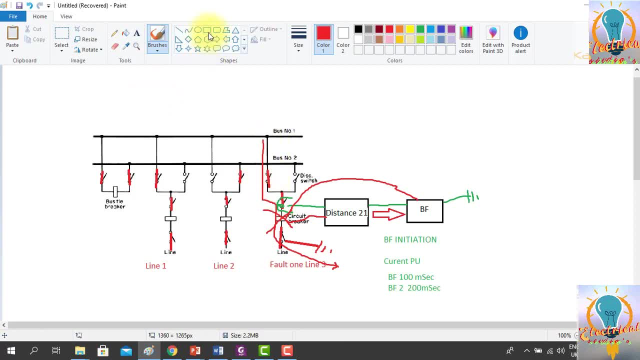 so the fault is feed through bus 1, so this is one of the source. so we will mark it. this is one of the source which is feeding the fault. so breaker failure protection in stage 2 will initiate the bus power protection 1. 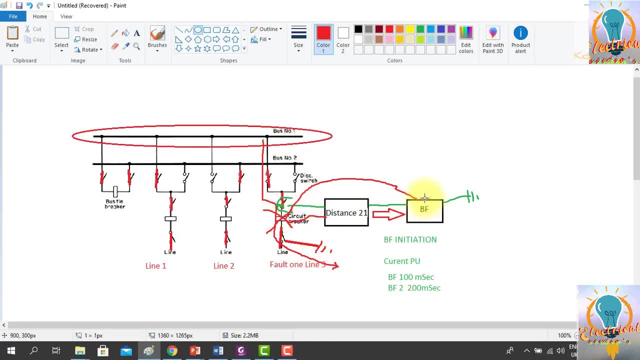 because this field is connected to the bus power 1, so it will initiate the bus power protection 1, so let's make another box of bus 1, so the relay will initiate in stage 2, it will give signal to this bus power. 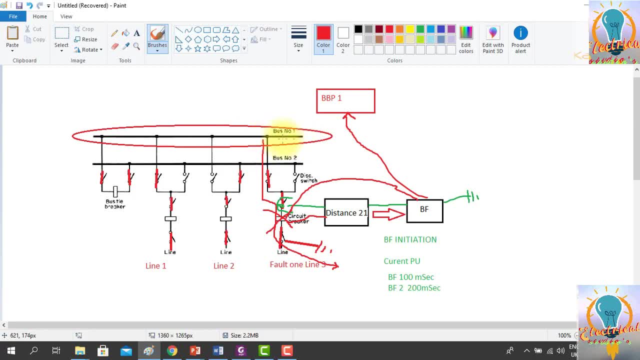 because whatever fault is feeding the signal, it will go to this bus. 1 because whatever fault is feeding the signal, it will go to this bus. power feed through this one, through this bus. so yeah, in the bus will operate. so now those feeders which are connected to this bus will be tripped. so at the 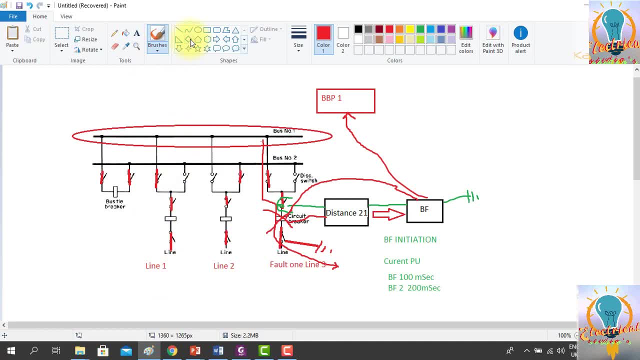 present you can see, line one is only connected which is basically feeding the fault also. so you can see the loop here from the line one fault loop is like this: at present it is going through the bus one and to the ground so the bus will trip all the feeders connected to bus one. so the this line one will be. 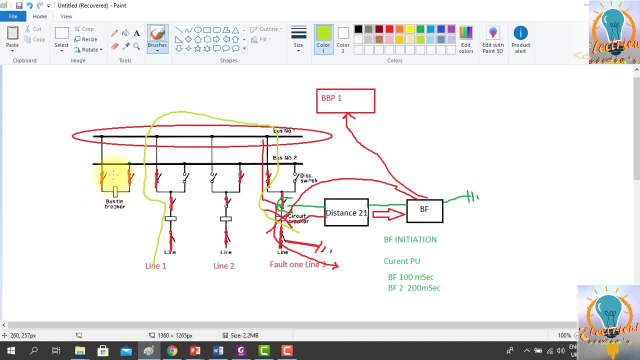 tripped and also the coupler will be tripped so so that the bus two should be isolated. so when this is isolated, this loop is isolated here. so this breaker is now open, so this is now open. also this breaker line, one breaker- is open. now there is no. 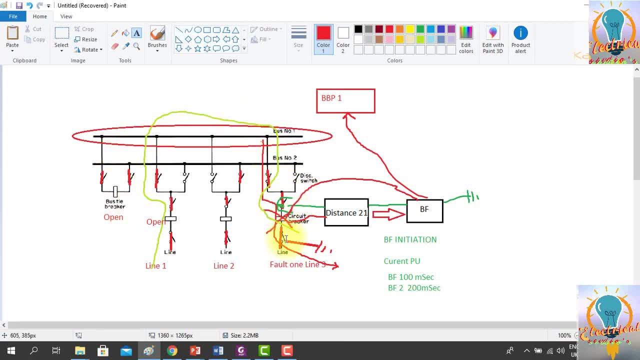 fault feeding from this end. but still there is a chance that fault is feed from the remote end. so the breaker failure in stage two operate the bus bar and also it will send direct transfer trip to the remote end breaker. so let me draw here the remote end. 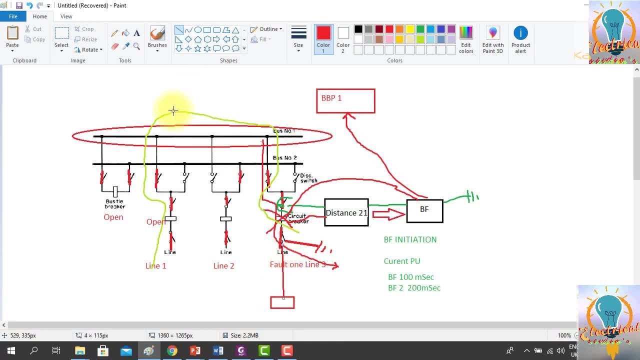 this is the remote end. so the relay will send DTT through the telecommunication systems. it will send trip to the remote end. breaker to send the command is called as direct transfer trip. it will send direct transfer trip to the remote end. so this is how the breaker failure protection is operating. 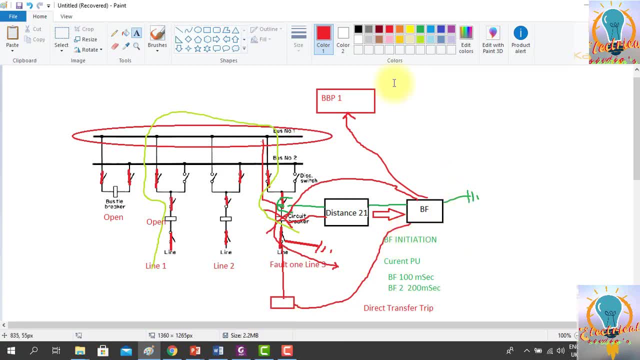 there is another function of the breaker. failure is another function of the breaker fail. for example, the breaker fail protection is connected to our transformer and there are some protection of the transformers, which are mechanical protections. so where are? there is a chance that there is no enough current in this system. 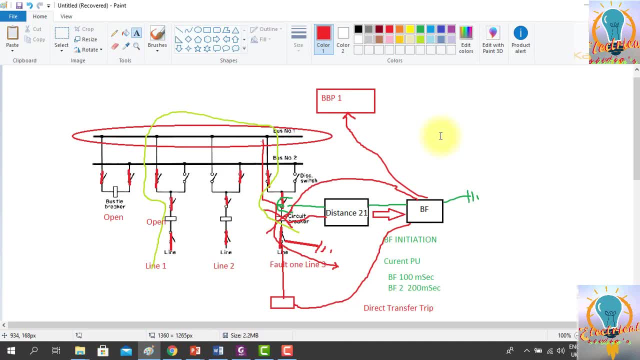 like a pressure relief, like buckles. so there is one option in the relay which is called as a local mode, and that option is enabled and also breaker status is also connected in this, in this type of low current operations, and instead of current the status is is monitored. so this is how the breaker 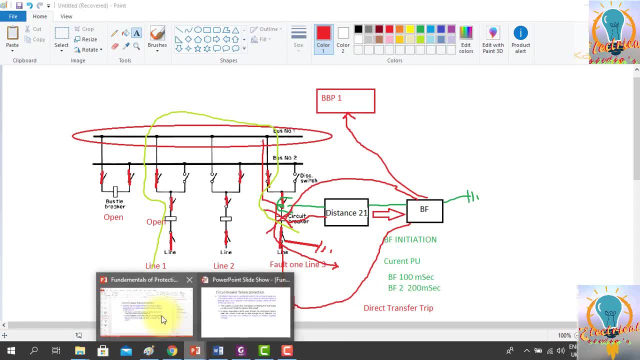 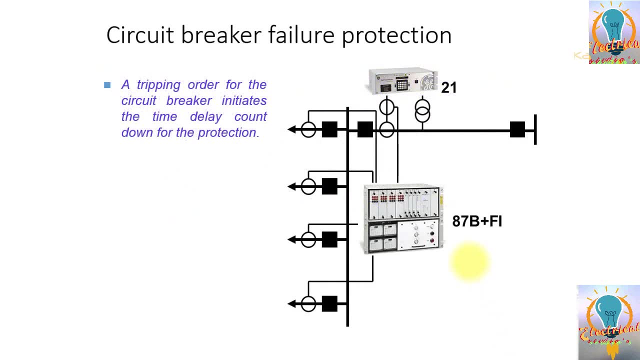 failure protection works. so I hope you understand the concept well. so we will move on to the slide. so we will see the tripping order for the circuit breaker. initiate the time delay countdown for the protection. so you can see the fault is here. the relay will issue the trip command. okay, 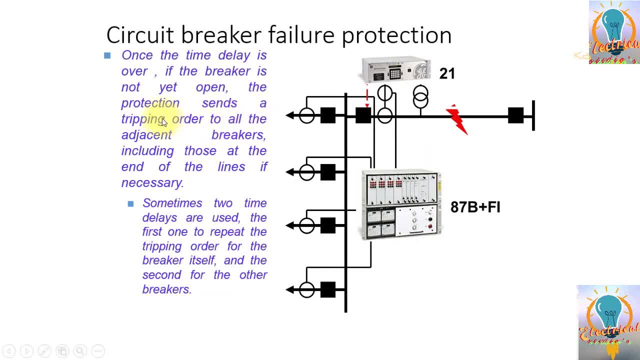 once the time delay is over, if the breaker is not yet opened, the production sends a tripping order to all the adjacent breakers, including those at the end of the line of. if necessary, sometimes two time delays are used: the first one to repeat the tripping order for the breaker itself and the second for the other. 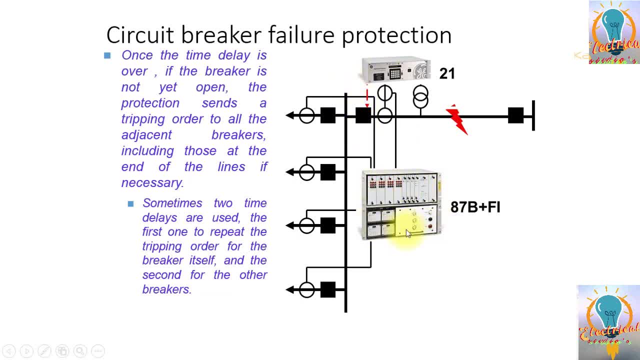 breaker. so in the stage one this is the breaker failure protection. so you can see one core is connected to CT core is connected to distance. another CT core is connected to the breaker failure protection. so in stage one distance delay will give trip command. but if the distance delay fails to trip the breaker, 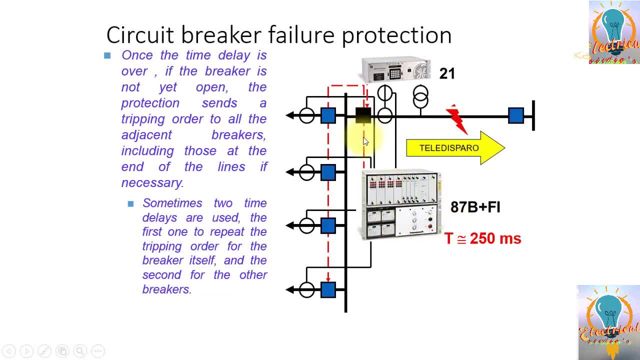 failure will issue re-trip, first of all in in stage one- it is normally 100 milliseconds, 150 milliseconds, and then stage two, which is between 100 and 50 to 250, will 200 to 250 milliseconds and it will issue trip to the bus power. 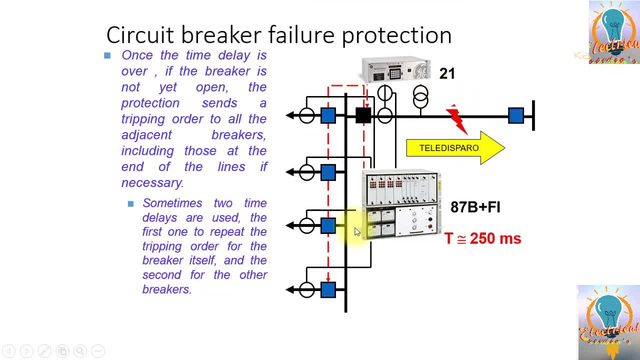 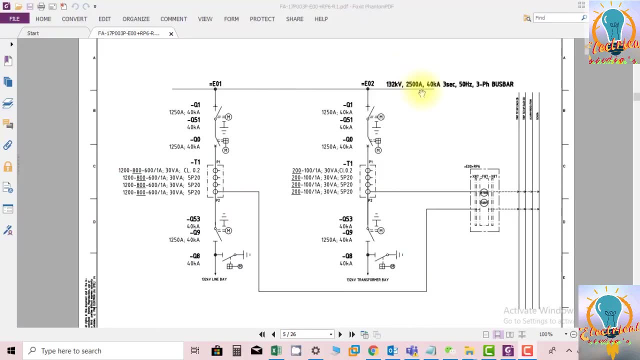 protection, all the adjacent breaker which can feed the fault and the remote end. so this was about the breaker failure protection. I hope you enjoyed the training. it is a continuous current which a bus power can carry without any damage. then it has a 40 kilo ampere for three seconds. it means it is a short circuit. 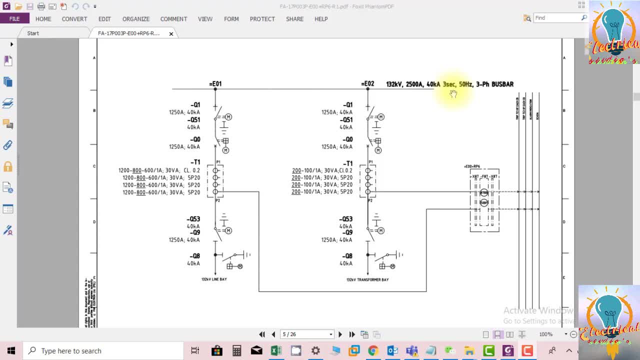 rating of the bus power that the bus power can carry 40 kilo ampere for three seconds. then frequency is 50 Hertz and is a three phase bus power, obviously, which is shown on a single line pattern. okay, then we will go to the E01, which is our bay. number one is showing: 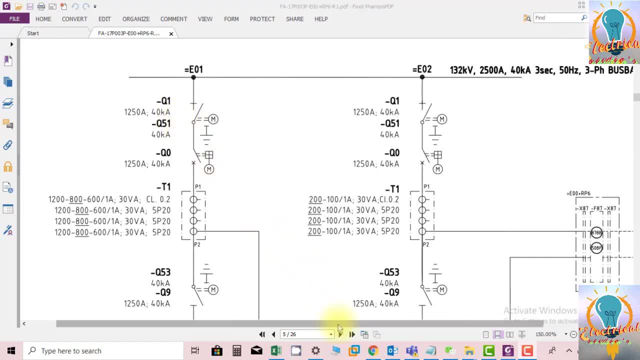 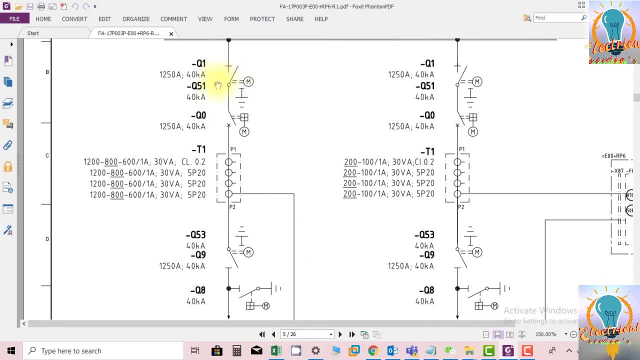 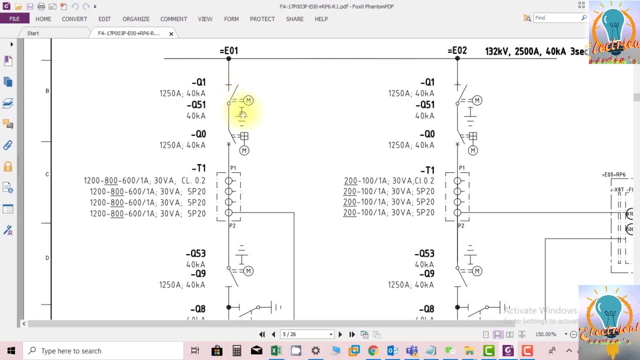 basically the voltage level for 132 kV. so here you can see this is the isolator and this isolator is called as the bus isolator and M is showing it is a mode property and it is isolator. come at switch. so it is basically a three position switch. so it is basically a three position switch. so it is basically a three position switch. 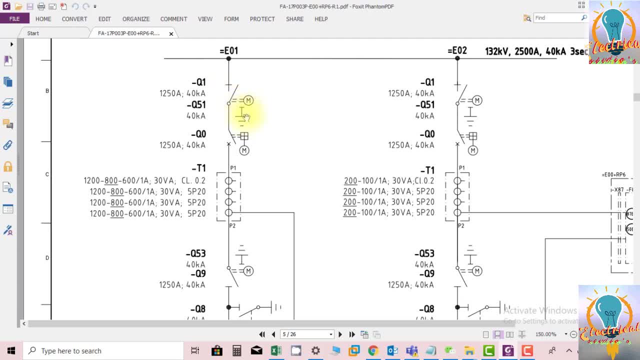 you can see like this, which is a function of isolator, and earth as well, and the rating of this isolator is 1250. so you can see the rating of the line bay is 50%, the rating of the bus power here. this is per design. then we have Q5. 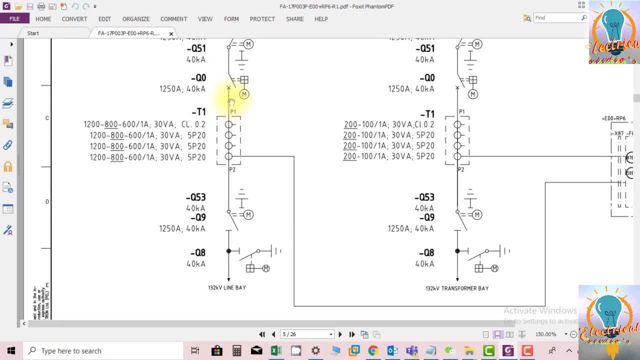 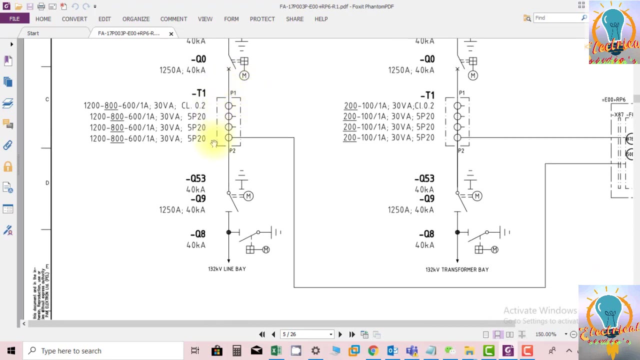 one which is basically earth switch. further, we have a breaker, and which is a 1250 AM here, which is 40 kilo ampere. so because of the more prop, credit further. you can see a maquette transformer and current transformer has one, two, three, four. these circles are showing number of cores. so it is. 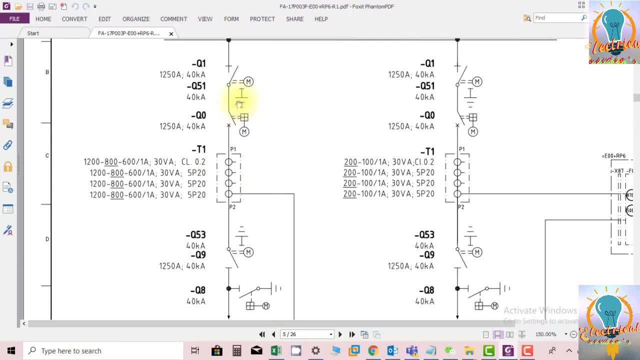 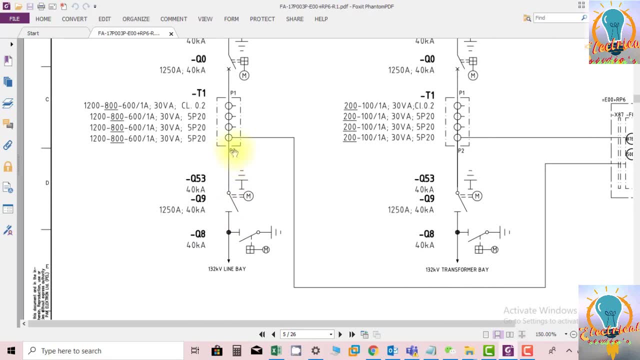 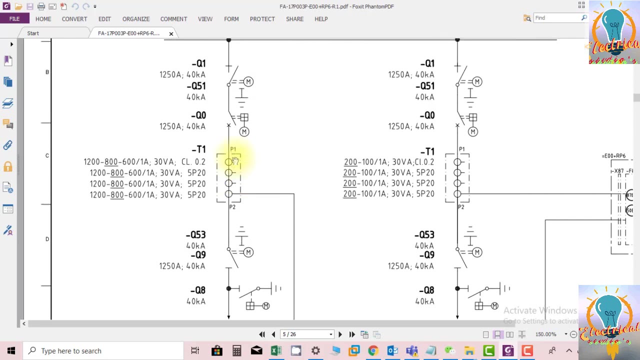 somewhere is multiple even is a polarity of expelled which is towards bus posso. ETO is a priority over CTU is towards line. so if we make a star point or we all join all the CT secondary winding at S1 side, then we will say that star point of the CT is: 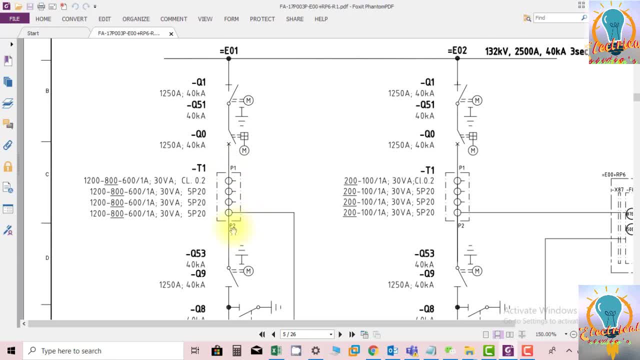 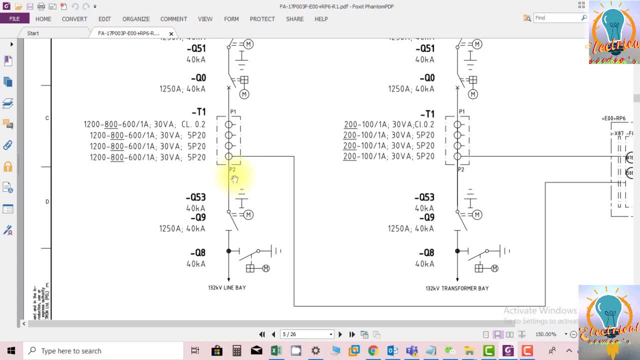 towards plus and if we join all the CT wiring coming from S2 side to make a common wire, then we will call it as CT star, point towards line. so this is some introduction that I have provided you further. you can see, this is the core number one, which is of class 0.2. this is for use for metering 3, 4 and 2, 3 and 4. 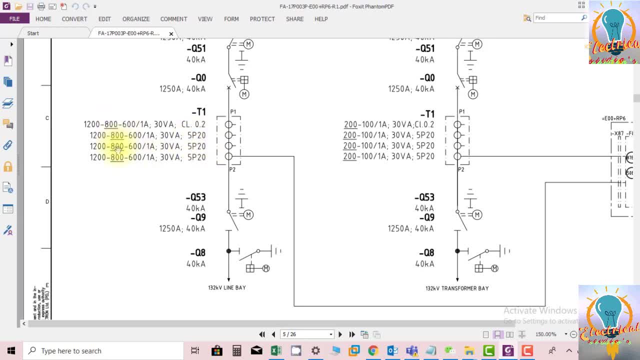 are 5P20 and they have chosen 800 ampere slash 1 ampere ratio for all the CTs, so we can call it as a multi-core and multi-ratio CT. CL point 0.2 means it is. it can have a error of 0.2 and it is class 0.2 used for metering 5P20. 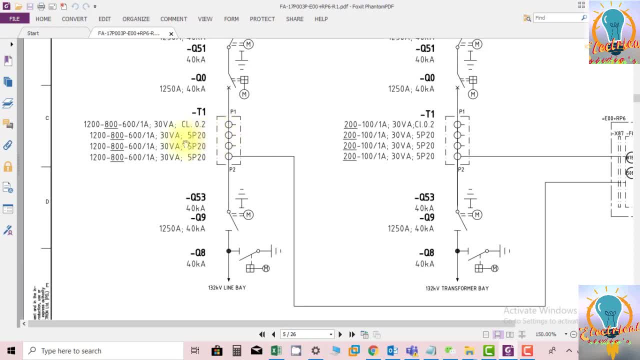 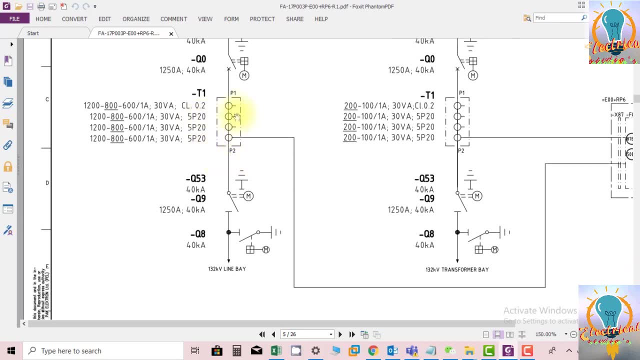 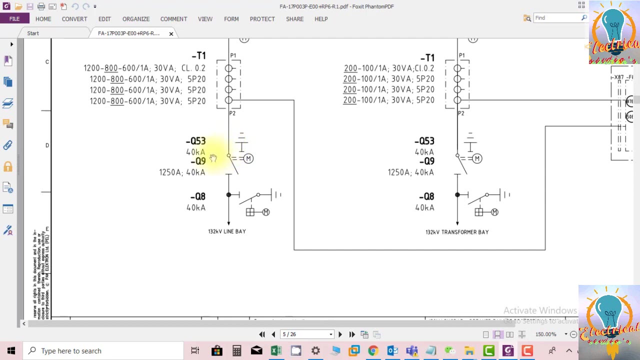 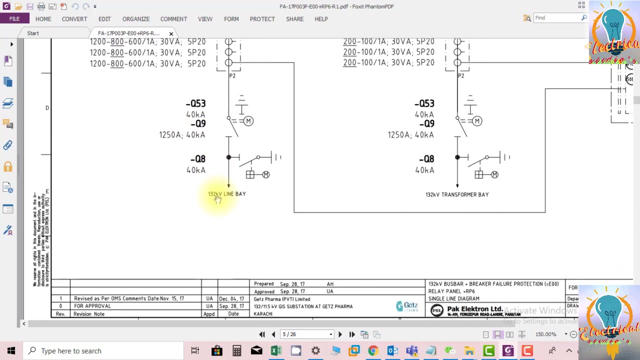 means this CT can have 5% error at 20 times of forward current. so this is the some detail about the CT. then you can find line isolator which is again motor operated, and then you can find the detail about the. this equipment, which is 40 Gi Ampere and continuous rating, is 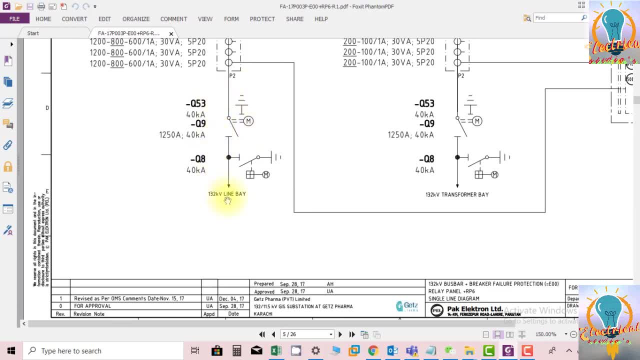 1 to 5.0. this is again the line isolator ARTR switch. further you can find QA which is 40 Gi Ampere and you can find this is basically high-speed ARTR switch for the line because line you work better on the QA and popularized wheel. 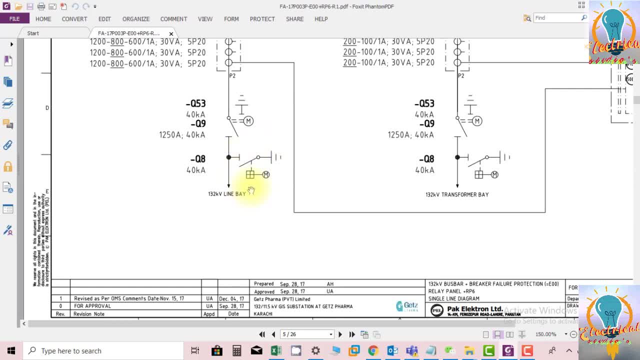 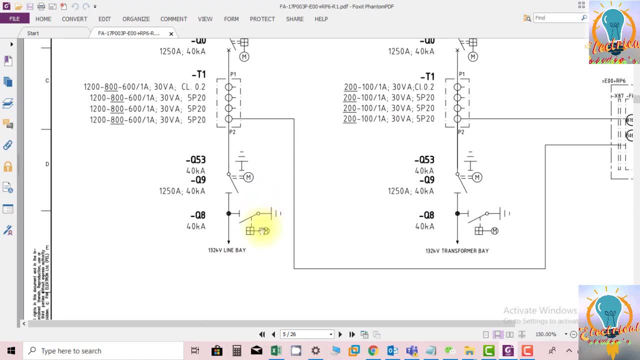 weasiw of gonna place that in your case is a cable feeder and the cable is long. there will be a large charging current and if we slowly close the earth then it might damage the contact of the earth because it has a high charging current. and when you will, 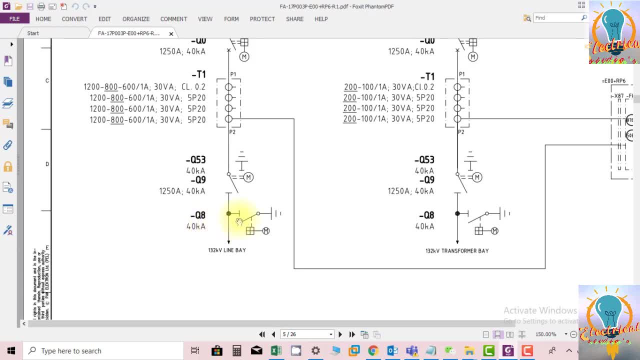 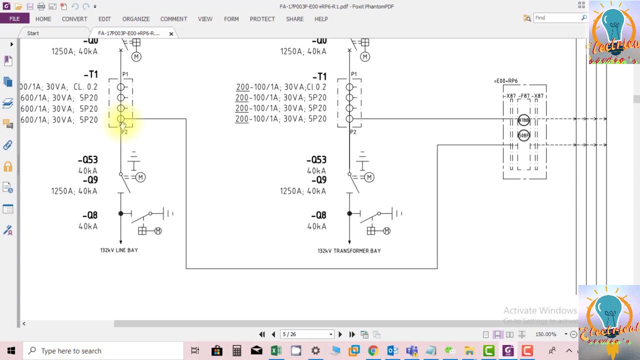 connect the earth slowly, the spark will figure and will damage the contact. so high CVS which is provided to close the earth in a fast way to protect the component. so this is basically. you can see this core P2 near to P2. this core, 520 protection core, is connected to breaker failure and bus power protection with 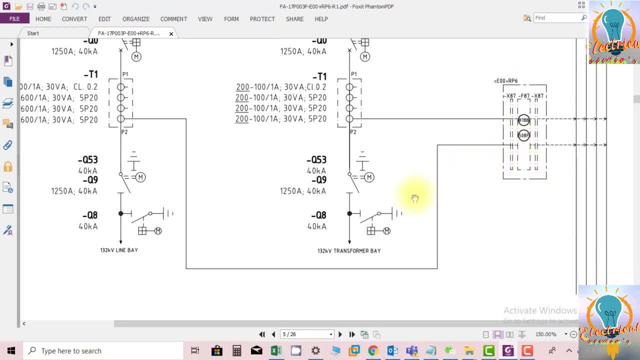 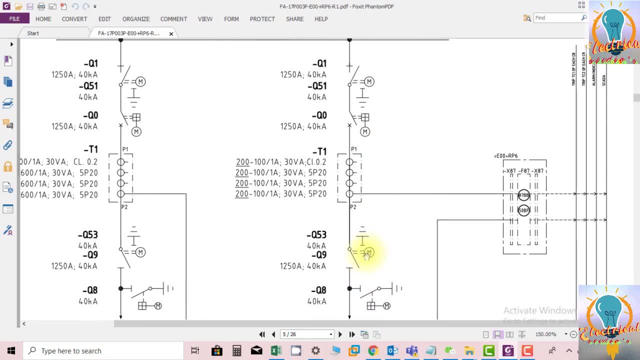 this protection has both functions, so one CD is enough for both and further you will see that bay E02, which is the transformer bay, and you can find the similar equipment here. and the CD is again, except the ratio here uses 200-1 because it is using as: 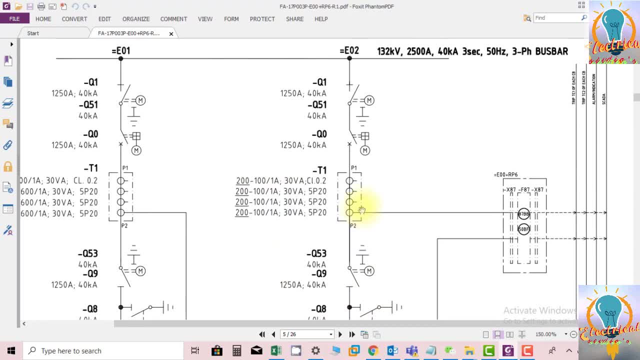 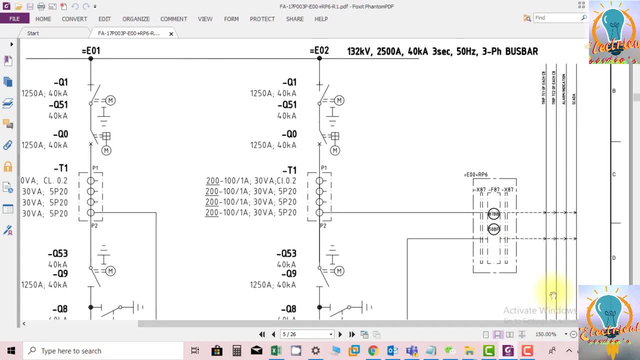 less ratio because of the capacity of transformer and the CD is connected to again the bus power and breaker failure protection relief. further, you will see that protection panel RP6, the bus power protection relief, is giving trip to trip, coil 1 to coil 2. it is. 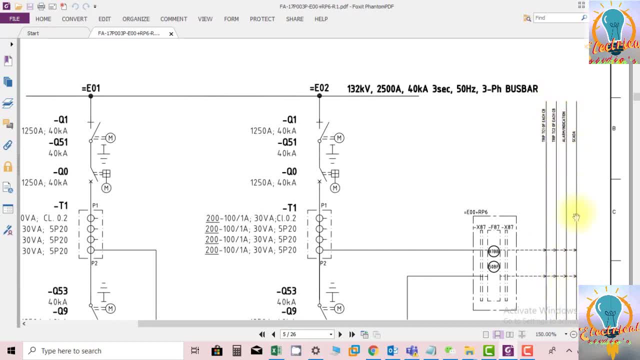 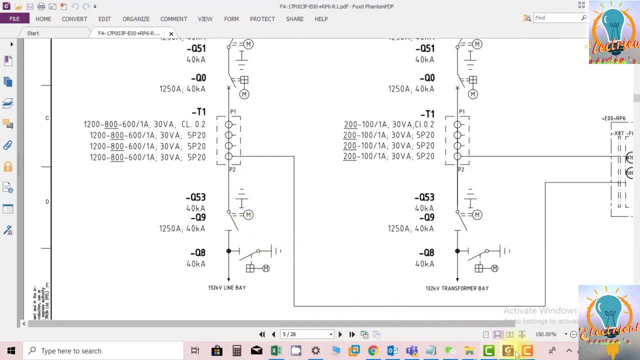 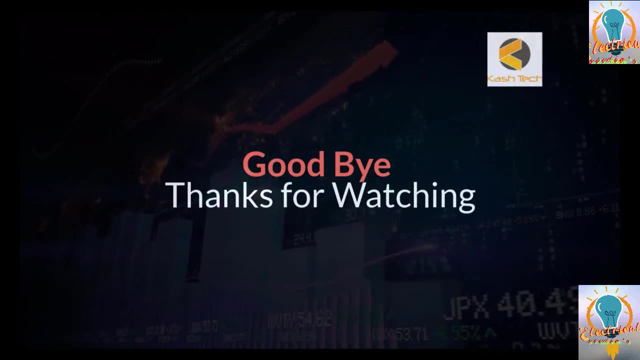 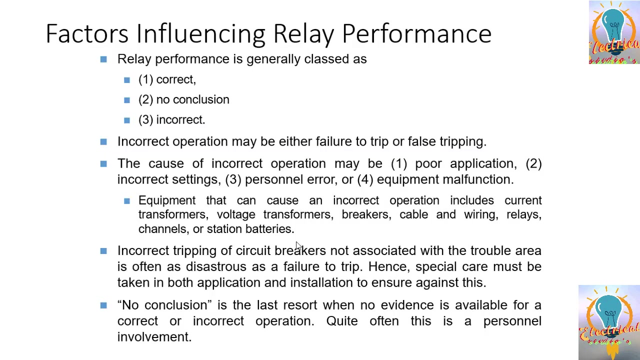 giving alarm at control panel and SCADA alarm is connected. so this was all about the single line diagram. thank you very much. hello and welcome. in this section we will see what factors that are influencing the relay performance. so we can classify the relay performance in three different categories. category 1 is the relay has performed. 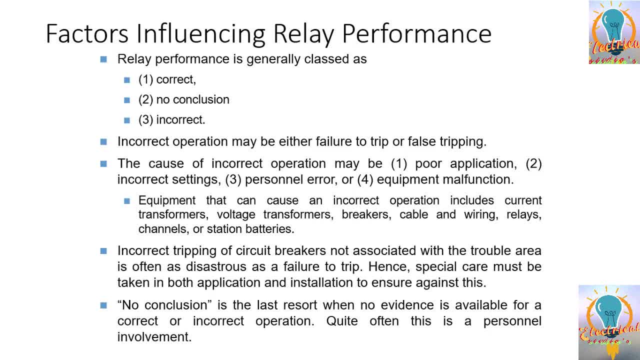 correctly. category 2 is: the relay has no conclusion. category 3 is: relay has not operated correctly or incorrectly, so the incorrect operation may be either failure to trip or failure to fail For false tripping. the cause of incorrect operation may be poor application, incorrect settings, personal error, equipment malfunctions. 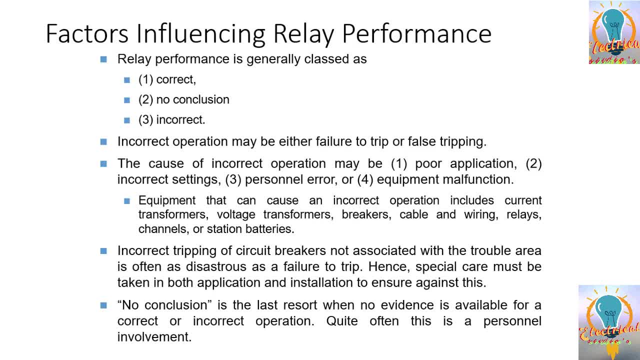 Equipment that can cause an incorrect operation includes current transformers, voltage transformers, breakers, cobbles, wiring relays, channels or station batteries. Incorrect tripping of circuit breaker not associated with the trouble area is often as a disaster as failure to trip. hence special care must be taken in both application and installation to ensure against this. 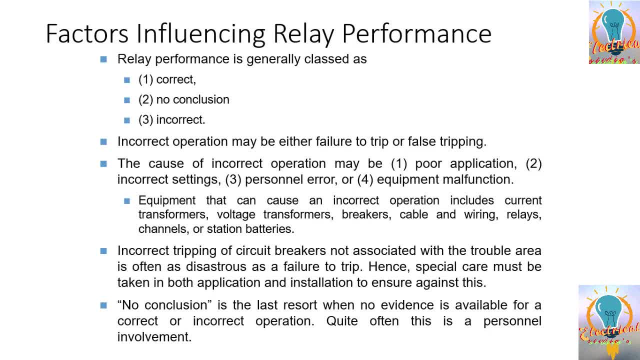 No conclusion is the last resort when no evidence is available for correct or incorrect operation. Quite often this is a personal involvement. So there are three different type of scenarios. One scenario is when the production is operated correctly. The other scenario is incorrect operations. 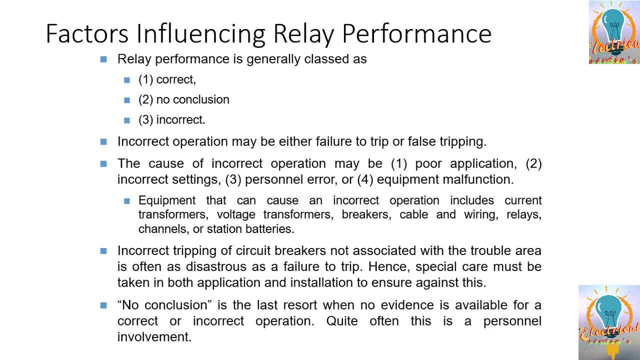 Incorrect operations can happen because there could be a wrong setting in the protection relays. Most of the trippings which are caused are basically mall tripping, unfortunately, and these are due to the wrong settings. Other option could be, for example, tripping may cause by CT saturation, or it may cause by VT itself. 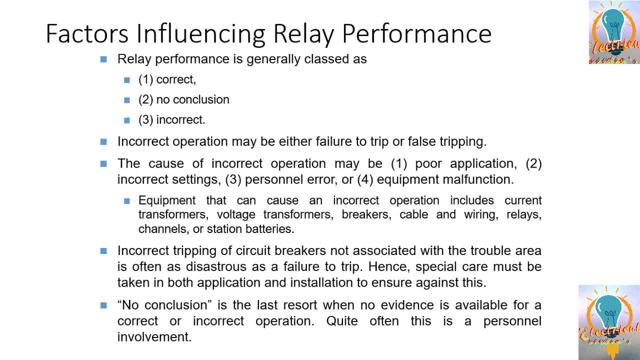 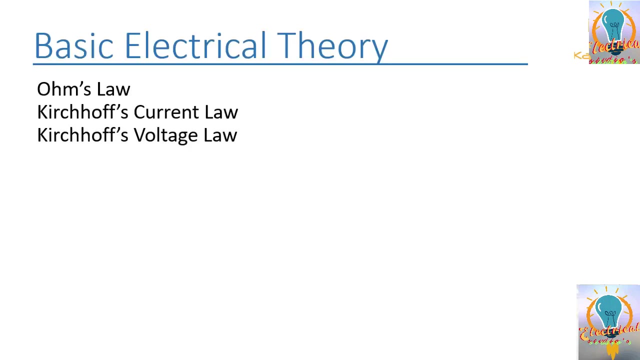 So sometimes the relay mall functions, Sometimes the relay has not done anything. so there is no conclusion, enough basically data available to decide the relay should have operated or not. So these are some factors which are influencing the relay performance. Welcome friends. in this section we will go through basic electrical theory. 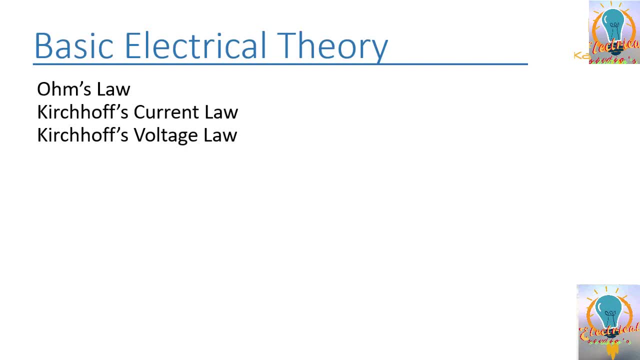 So we will see some equations like Ohm's law, Kirchhoff's current law and Kirchhoff's water law. So you can see, we will start with basic power equations: V is equal to I into Z, where Z is equal to R plus GX. 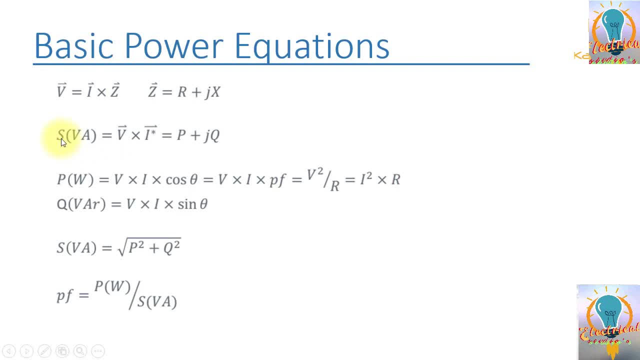 These are basically the vector quantities. S is apparent power, which we are saying. VA is equal to voltage into current And in the rectinal components it can be shown as P plus JQ. P is the current. P in watts can be written as voltage into current cos of phi. 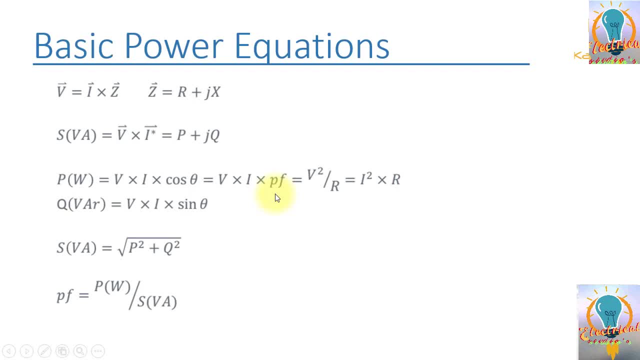 Voltage and current into the power factor. Cos of phi is basically same as the power factor, which is equal to V squared divided by R, which is equal to I square R. Q is measured in VAR, which is equal to V, into I, into sine of the angle. 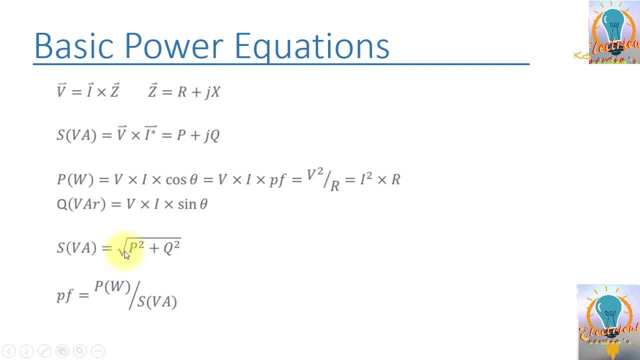 S is equal to under root P square plus Q square. power factor Can also be calculated by P divided by S. Basic power equation: Three-phase power is equal to 3 into single-phase power. Three-phase power also can be calculated into 3 into V line, to neutral, into I single-phase. 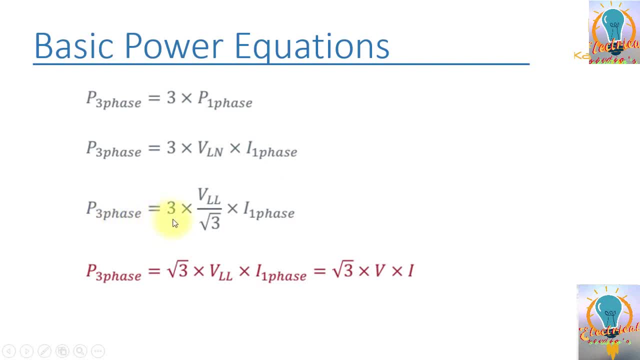 Or in the other way we can calculate three-phase power is equal to 3 divided by V line to line, divided by under root 3 into I1 single-phase, So P power or S three-phase. normally the equation we are using, mostly in case of transformers and generators and everywhere, is under root 3 V line to line into I single-phase, or is equal to under root 3 V into I. 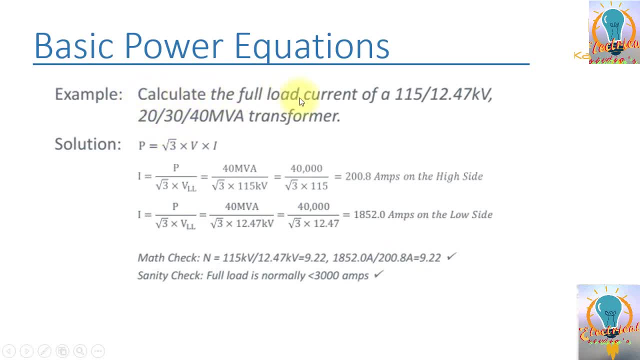 So we will go through an example where we will calculate full load current of 115 by 12.47 kV. So we have 20,, 30,, 40 MVA power transformers. So first of all, why a transformer has written with three different ratings? 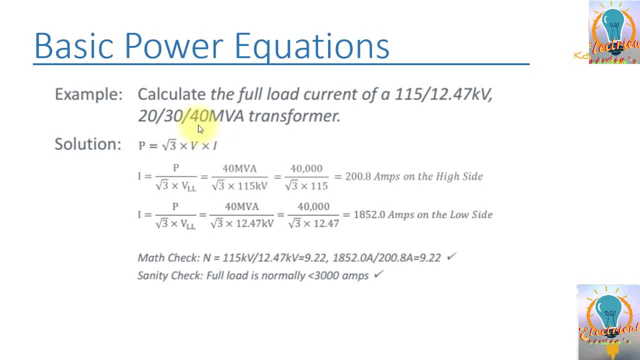 The reason behind is the transformer rating depends upon the cooling method. So if the transformer has three levels of cooling, two levels of cooling here, So like fan group 1 and 2, if both fan groups are off, so this transformer can. we can draw the power up to 20 MVA. 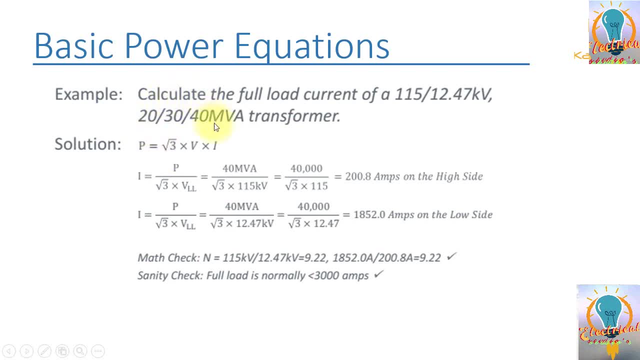 So if the fan group 1 is on, you can draw the power up to 30 MVA. So if fan group 2 is on, you can draw the power up to 40 MVA. So that's why the transformer rating is shown in different values. 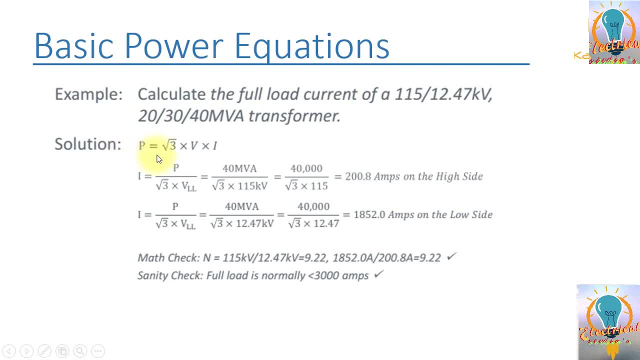 So let's calculate the full load current. So P is equal to under root 3 V into I. So I is equal to P divided by under root 3 V LL. So then it's equal to 40 MV divided by under root 3.. 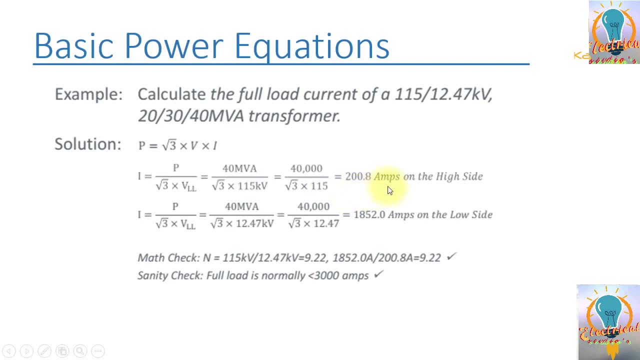 For HV side the voltage is 115 kV. So we have calculated The HV full load current as 200.8 amperes on the high side. So in the same way we will calculate the current. We have to just divide it by the low side voltage, which is coming as 1852 amps. 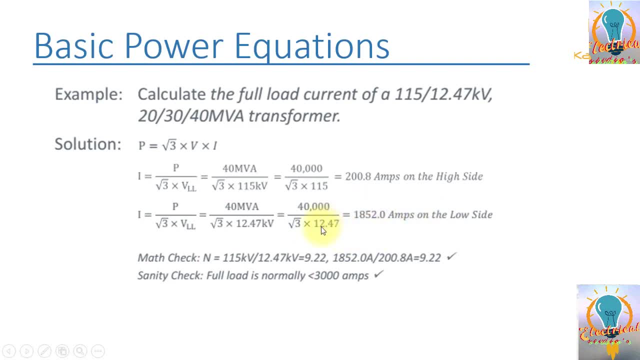 So at low voltage side the current is more but the voltage is less. But at the high voltage side the current is less but the voltage is more. But the power will remain same on the both sides. So no difference here. 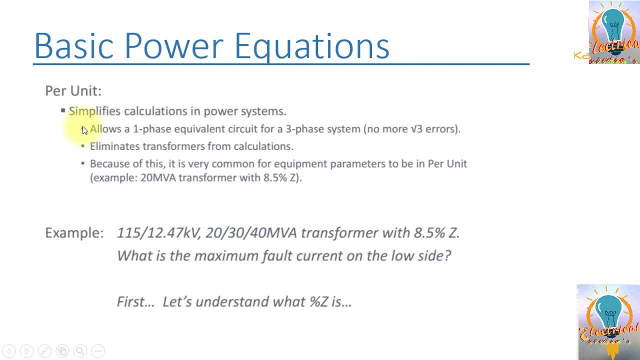 So next we will just go through per unit system briefly. Per unit system simplifies calculation. power system. Allow singe phase equivalent circuit of 3-phase system, No more under root 3 errors. Eliminates power transformers for calculations. Because of this it is most remaining correct for equipment parameters to be in per unit. Example: 20,000. yeah, ok精, hectanoude unit per unit To have. a very good point of recoupment parameters To have, and so double The circuit is just declared very good, we can sleep for it. no more under root 3 errors and it will have efficient restrictions in power. notorious force. 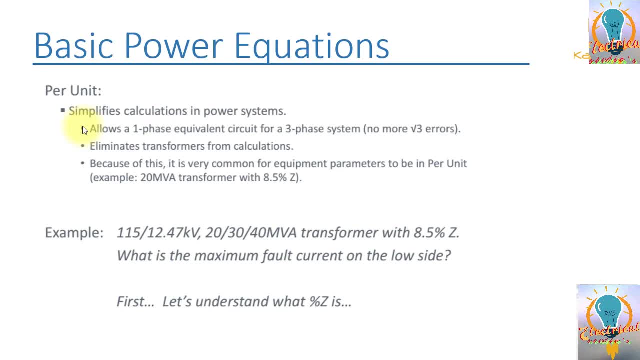 Power and the appeared time does not make sense much because of technology, an ultrasonic to demonstrate, because of fold design. Okay, so these are then it's actually painless. We are just explaining the power. and then is long in Lima MV transformer with eight point five percentage impedance. so whenever you you 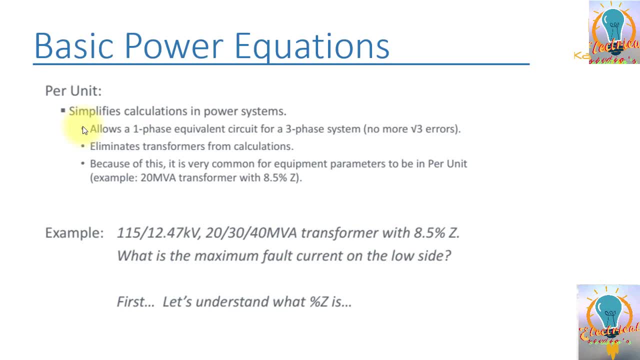 you will see the nameplate of an, a transformer. you will see the percentage impedance they are showing in, always in per unit or percentage. so we will take an example. we can see we have a transformer which the rating is 115 by 12.47 kV and the rating is 20, 30 to 40 MV, a transformer with eight point five. 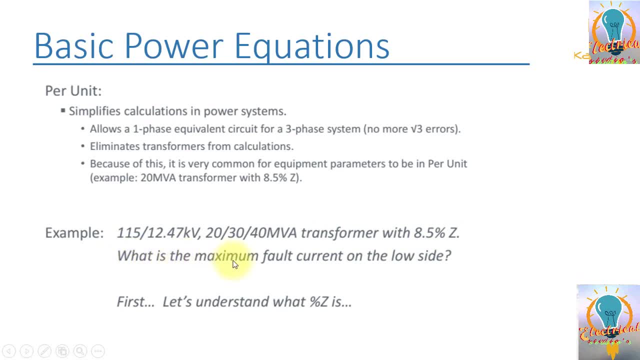 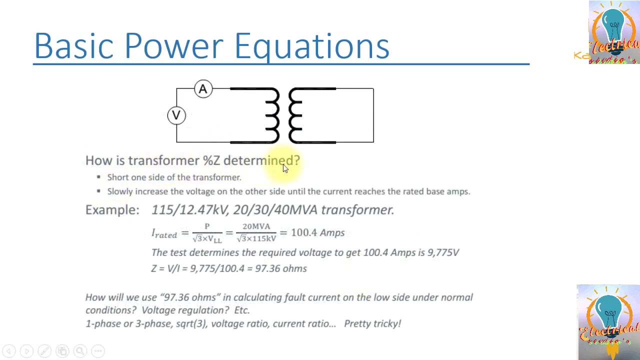 percent is the percentage impedance. what is the maximum fault current on the low side? so we can, we can calculate. first of all we should know the percentage impedance. so how is transformer percentage impedance is determined? so short one side of the transformer. slowly increase the voltage on the other side until the current reaches a rated base amps. so this is the 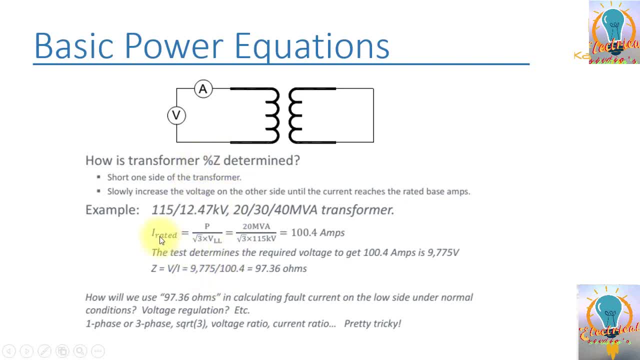 method of finding percentage impedance. so you will get this formula: I rated at: 20 MVA is hundred point four ampere. at HV side the test determine the required voltage to get hundred point four amps is nine point seven seven five volts. so it means that impedance that is equal to 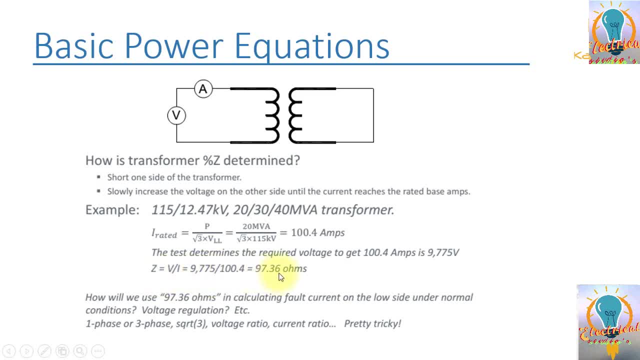 V divided by I, which is equal to ninety seven point three, six ohms. so how you will use ninety seven point three, six ohms in capability and we can then weight a transformers body. and now we can see that voltage is not load. so this is the ratio. so I know that voltage is sold and the 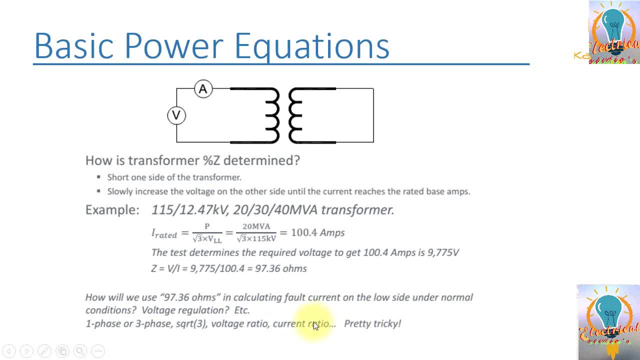 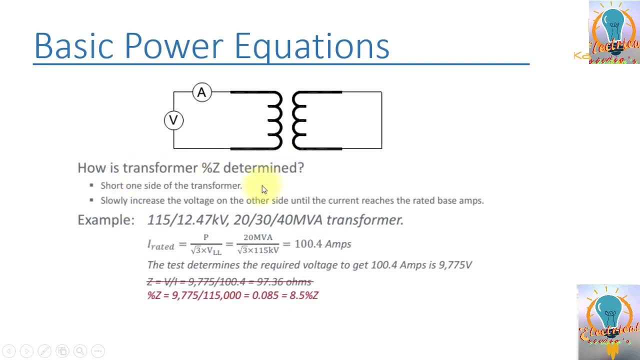 voltage value. this is its loadables. this is voltage we will give and this is the primary hurdle. forsized graph. you can see we have put the voltage value on the low side. we can say there is a loss of impedance between the back. physi gutes. 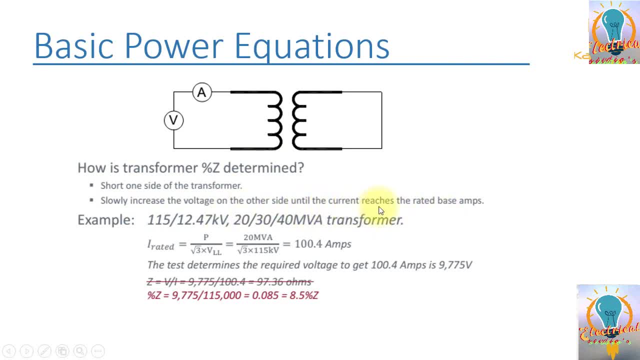 as well as surrendery of the beam radiation. so if I measure the voltage approximation, so the voltage calculation is잖아요. band Berry, proof: give relief of theegd voltage case S Line bar. and perhaps this was light. if you don't know the method of designs, I will give a chain out of a Correct. okay, one phase with fold. 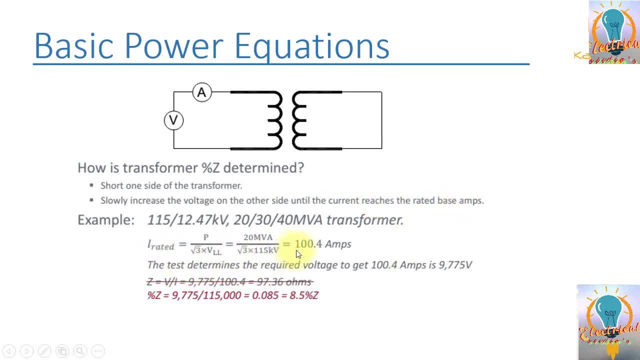 it base amps, so you can get this value again. this is 100.4 ampere. the test determine the rate required voltage to get 100 ms, 9.775 volts. so percentage impedance can be calculated by dividing v, divided by i, so 9.775. we are dividing it by 115 and we are getting is 0.085, which is equal to 8.5. 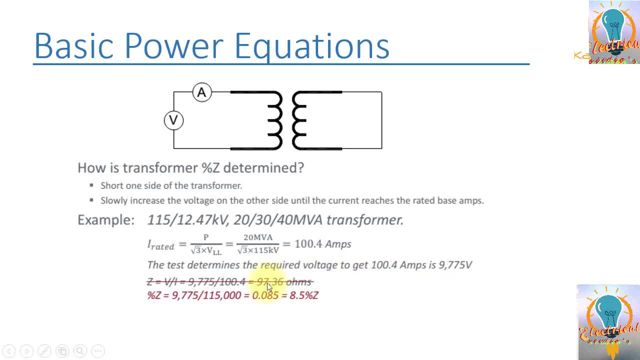 percentage impedance. so this is the formula. in this way we are doing the, we are calculating the percentage impedance using per unit value. we are not using this formula. so this formula is very easy to understand and very easy to do it. so you just have to divide the ohms by the voltages. 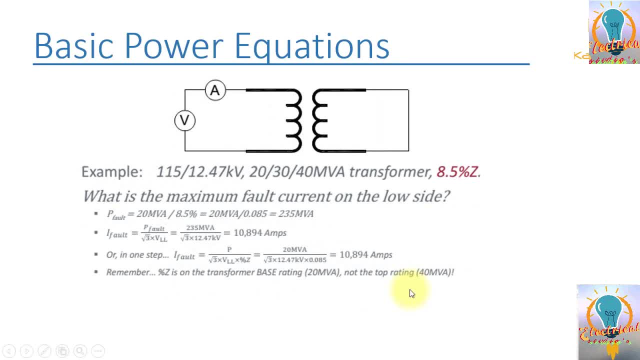 of the hv side, you will get the percentage impedance. so this is another example. uh, what is the maximum fault current on the low voltage side, if you know the percentage impedance- so we have done the calculation- you have to divide mva. divided by percentage impedance, you will get two, three, five mva. so this is the 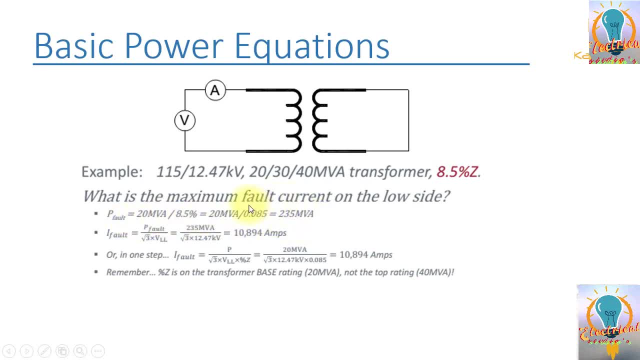 fault mva. so you can calculate the fault mva using this formula. this is very simple. so you have, and you know, the mva rating of the transformer divided by the percentage impedance, you will get the fault. if you want to collect the fault current, you just uh, in this way, simply using this formula, i fault. 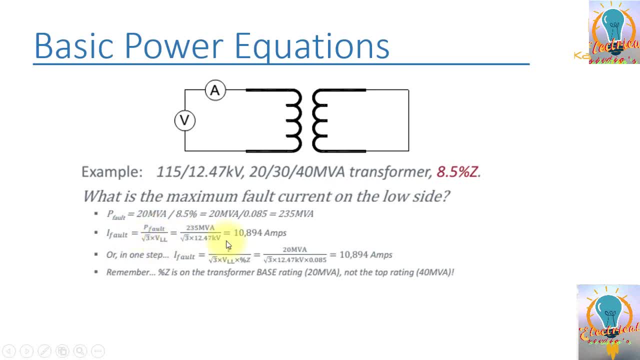 is equal to p fault or s fault divided by android 3 to v, line to line. so in this way you can calculate the fault on hv side and lv side. so remember percentage impedance is on the transformer, base rating 20 mva, not the top rating, 40 mva. so you need to know what is the base rating of the 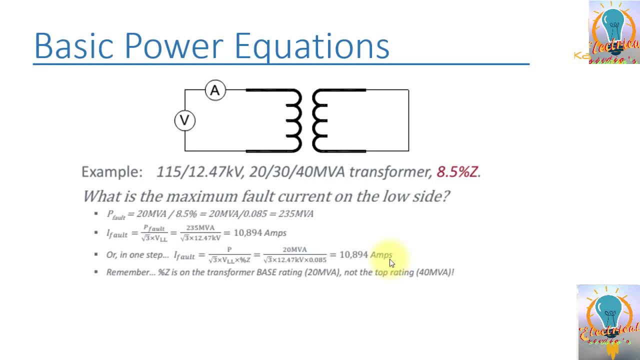 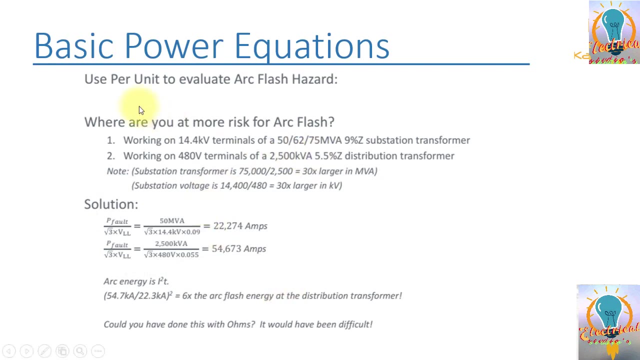 transformer. so normally the personal impedance is selected on the base rating, which is the least rating of the transformer. so you should the nameplate, you should be able to know that what is the base rating. so now we will use per unit system to evaluate the fast. okay. 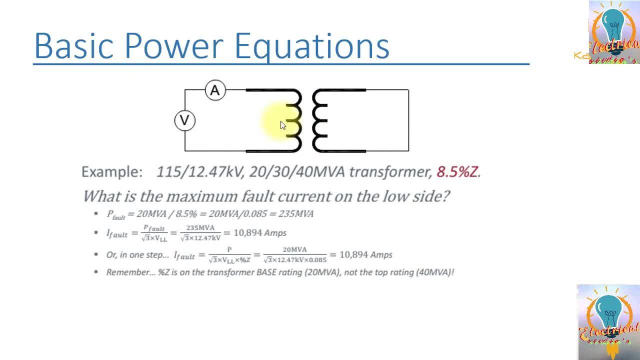 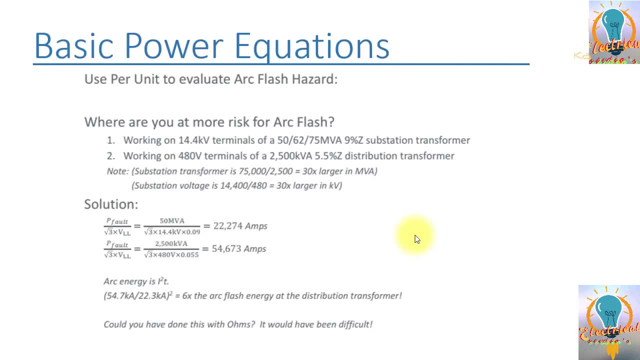 let it do it in the next section. so thank you very much. in this section we will use per unit values to calculate the and to evaluate the arc flash hazards. so where are you at more risk for the arc working on 14.5 kv terminal of 50, 62, 75 mva? 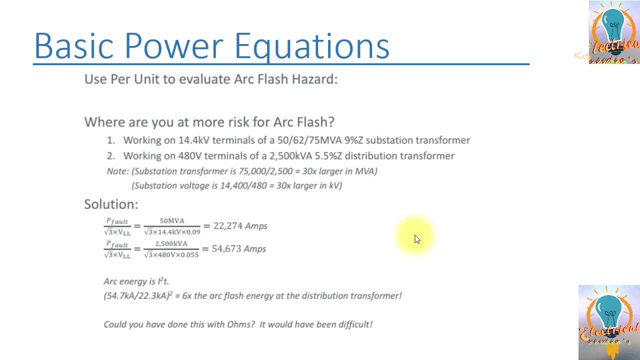 nine percent percentage impedance of civilization transformer, or working on 480 volt terminal of 2500 kva, 5.5 percentage impedance of distribution transformers. so this is an example, so we will see the different type of transformers, so which have more hazard of arc flash. so solution is: 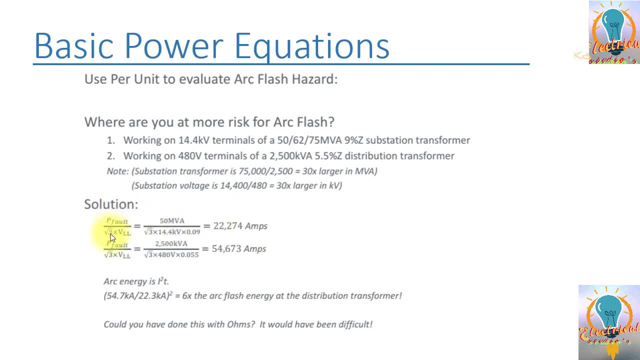 we will calculate basically the fault current in case of both transformers. so this is fault current calculated for the type 1, where you can say voltage is 14.4 kbs, the fault, the fault amps, is 222 kohms approximately and for the low voltage voltage are very less. this is 480 volts and here we have 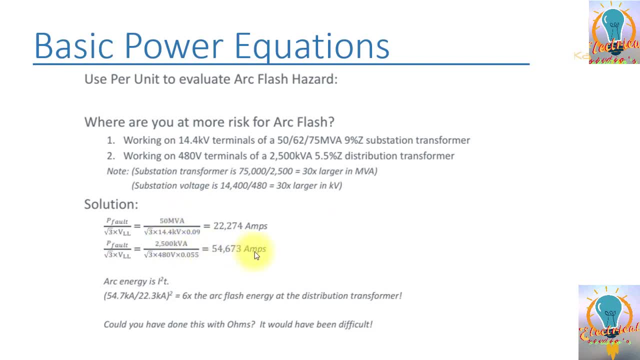 high volts. so the current is 54 kilo amperes. so by this example we can see the arc energy we can calculate is equal to: I square into T. so we, once you calculate the arc energy for fourteen point four kV, the arc energy, and then 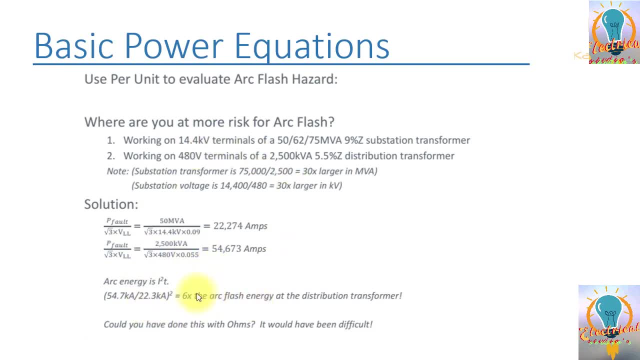 you have to divide it by this one. it is giving that. it is understood that the arc flash energy, a distribution transformer, is six times more than the arc energy at the fourteen point four, four kV transformers. could you have done this with ohms? it could have been difficult. so this is an example of art, fresh study. so we have. 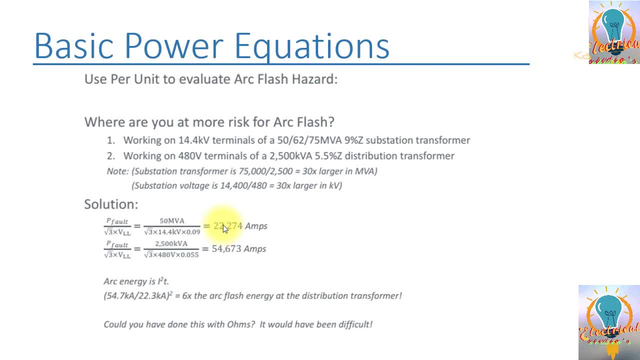 seen the impact of arc. basically, the concept is that ark is not depending upon the voltage, arc is depending upon the current. so more the current, the more will be the arc. and if the art current is, if the art will be more, then they will be a more energy in the arc, so energy in the外. 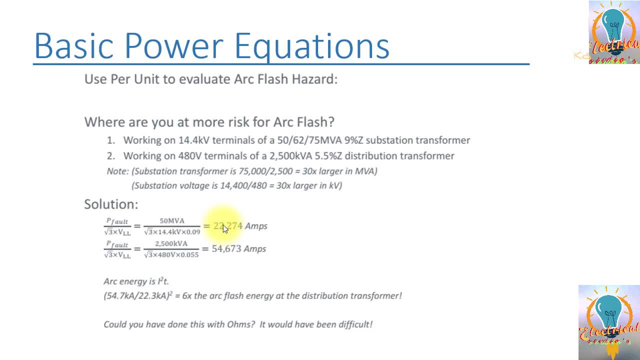 is the increase square of the time. so if even that at low voltage the impact of R is more, because the distribution transformers doesn't have that much percentage impedance, so we can see the distribution transformer here has percentage of five point five percent, whereas that main transformers, power transformers. 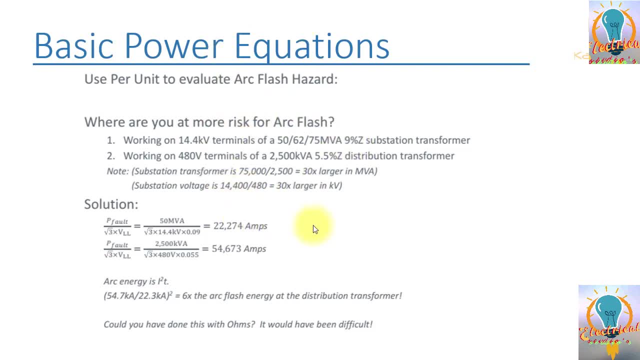 have the percentage impedance of nine percent. so this is a very good example to understand that how which equipment has more arc flash hazard. so a layman will will think that forty point four kV, that voltage level is more, the transformer, MVA, is more, have a more arc flash. but with this calculation you know. 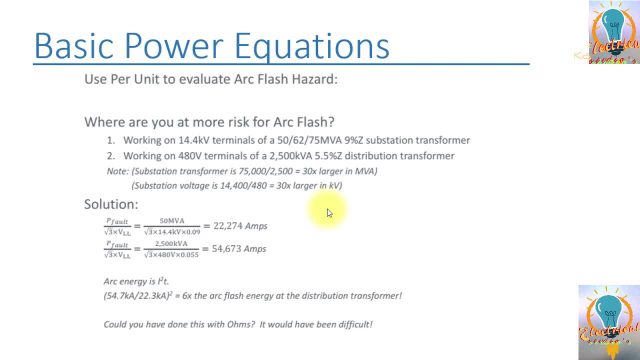 that a very small transformer of you can say 0.25 MVA and 480 volts, has a very, very six time more hazardous. and then a bigger transformer, 75 MVA, for the arc flash. so you need to be aware of the fault current before you are starting the work. so it's more important to wear 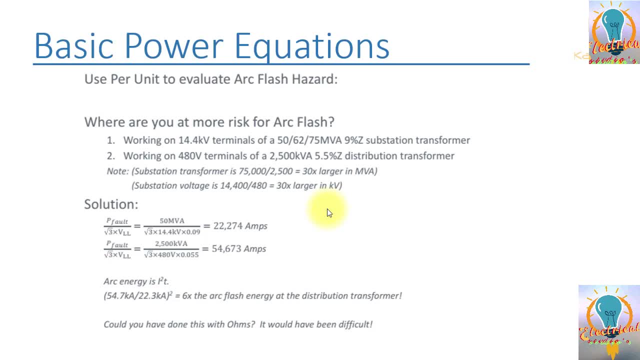 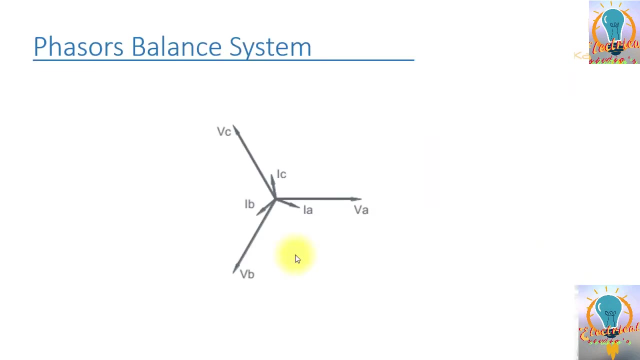 the arc flash equipment on the 480 volts in this case. so this is how this arc flash studies is important. I hope you enjoy this lecture. thank you, hi. friends, in this section we will go through the phasor system and different types of Ford. what will happen if there is a different type of fort in the? 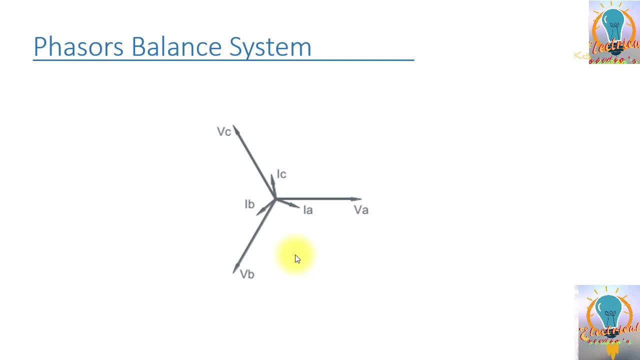 phasor system. so here you we can see if the system is balanced. so you can see, all three voltage are balanced and placed equally at 120 degrees and the current is also balanced and in the symmetry and it is at 120 degree place. here we can see. 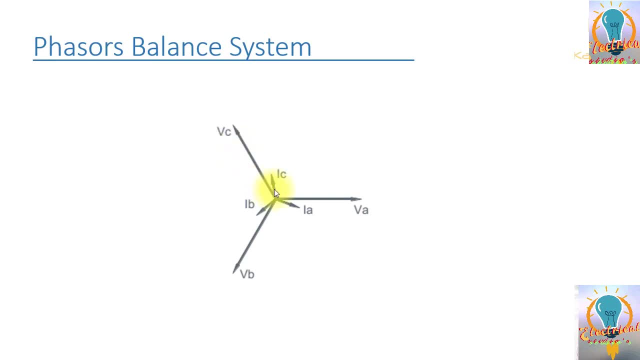 see the current is lagging the voltage. it means it is showing that load has a lagging power factor. so this is the waveform for a balance system. so now we consider a three-phase fault. if there is a three-phase fault in this three-phase fault, you will see that current three-phase current is increased too. 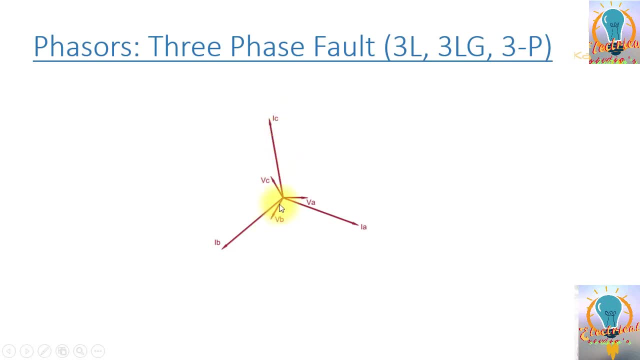 much and the three-phase voltage will be reduced. so you can see, the current has increased and voltage are decreased, so but the symmetry is not disturbed, so symmetry of voltage and current remain the same. so this is basically what happened when and there is a 3 phase fault again, we will start if we for. 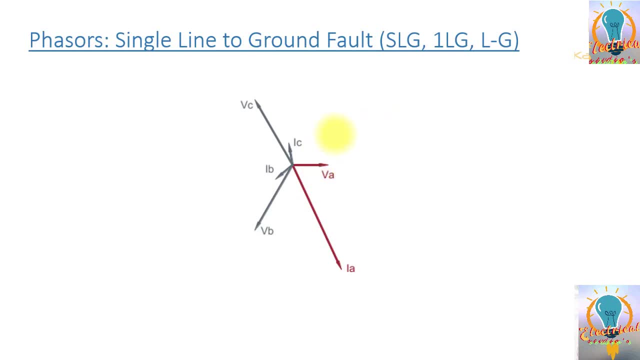 example, if you have a balance system and then if there is basically single line to ground fault. so you see, this is phase a, this is phase B and this is this is phase a and this is phase of now. see, to ground fault. du, I cannot Politik求. 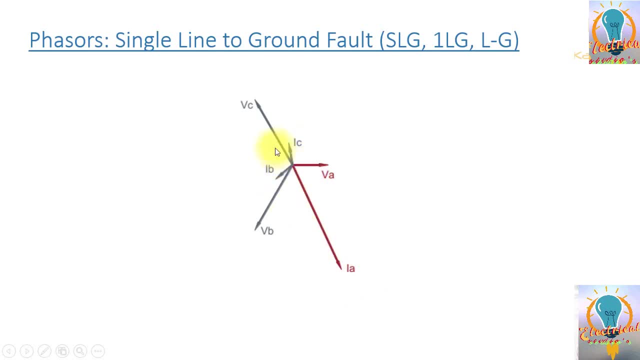 phase B and phase C. this is VA, VB and VC. so if there is a phase two ground fault- previously it was looking like this- everything was fine in balance. so when there is a fault on phase a, so phase a voltages are reduced because this loop is under fault and the phase a current is increased. so this is what happened. 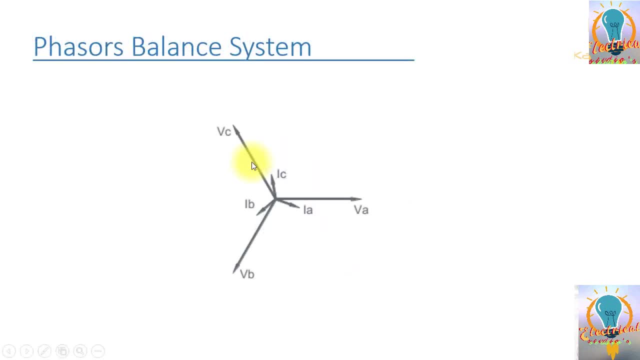 when there is a fault on VC. so again, we will consider a balance system first, and then you can see if there is a face to face fault. so in case it was, it was like this. so then we have fought on phase e and phase C, so phase a and C, both will. 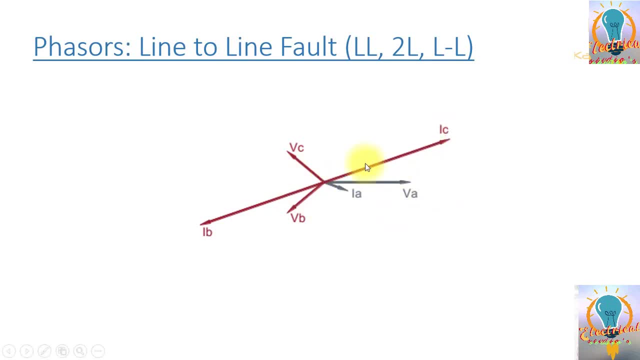 be equal and opposite because the current will be entering through phase a and a, phase B and leaving phase C. so now the angle is disturbed. so angle between these two phases will be out of phase by 180 degrees and you can see the phase B and C. the voltage will be collapsing, so this will be the waveform of the system. 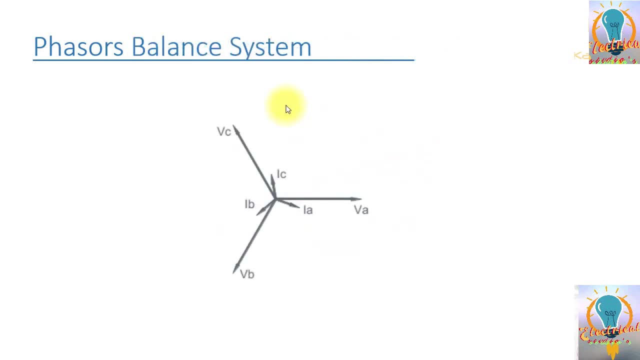 this will be look like this. so again, we will consider first the balance system and then we consider that we have line to line to ground fault. so in this way you can see we have fault on B and C and then you can see the voltage of B and C. 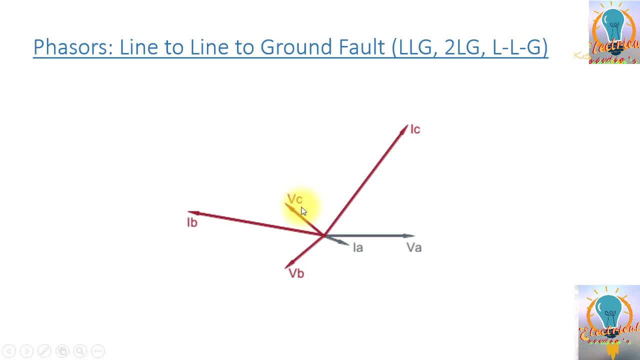 are reduced and the current in B and C is in in this direction. so it was B was here and C was here. so the voltages are just reduced and an angle of B and C slightly tilted towards each other and the current you can see also is in different direction: B and C. 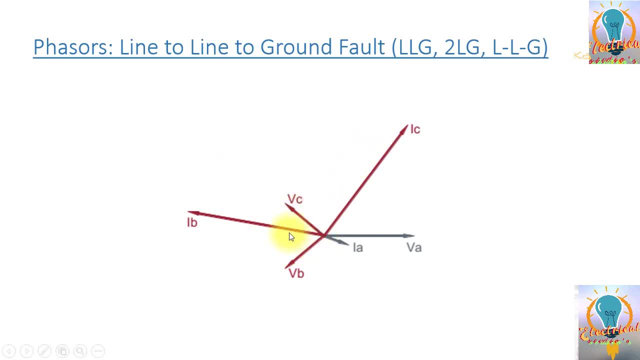 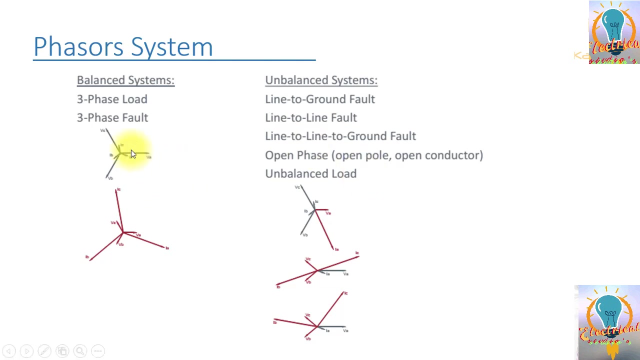 both are moved. so because now both conductors are grounded and now current is not out of phase between B and C but there is a huge current, we will consider a fault balance system again and then we will come to the phasor system. so we have a balanced system, we have unbalanced system, so we can divide. 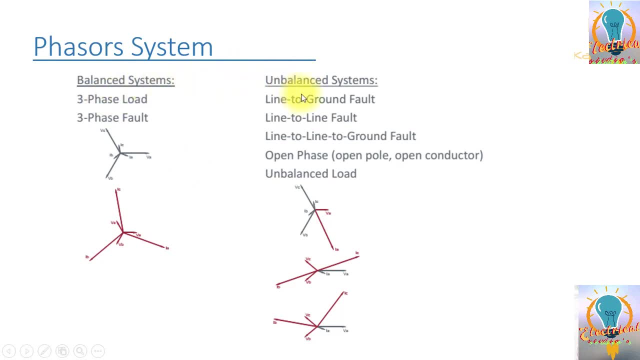 phasors in two groups. one is balanced and another one is unbalanced. in the balanced system, for example, it is a three phase load. we have balanced phasor, so voltage is a high, current is under limit and the three phase fault is also balanced, symmetrical. 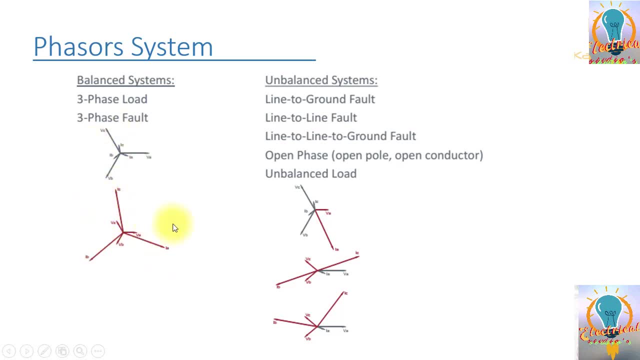 system, but in this one current is higher and voltage is less, but symmetry of the system is not disturbed, whereas in unbalanced systems- single phase to ground fault, double line to ground fault, phase to phase fault, unbalanced load- these are all example of unbalanced system. so this was a little introduction about the 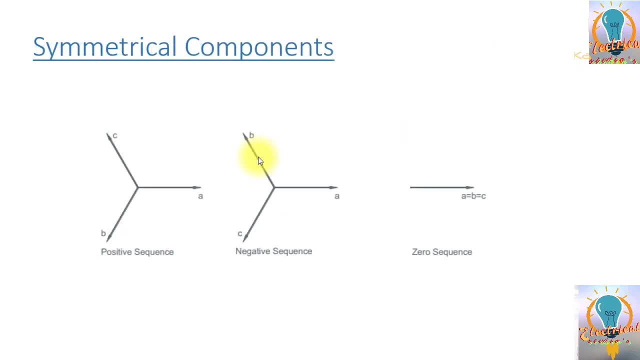 phasors. next topic will be about symmetrical components, so we will just have a little introduction about the symmetrical components. basically an unbalanced system. it can be divided into three different balance systems: one is positive sequence, one is negative sequence and one is zero sequence. so zero sequence. you can see all three. 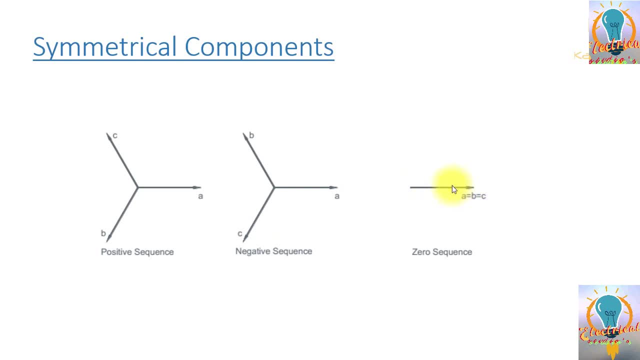 components phase A and B. all three are in phase. positive sequence is same as the normal healthy system. it has the same sequence: a, B and C. so negative sequence: it has a reverse sequence. so first a will come, then C will come, then we will come. so this is the little presentation of the medical components. so any 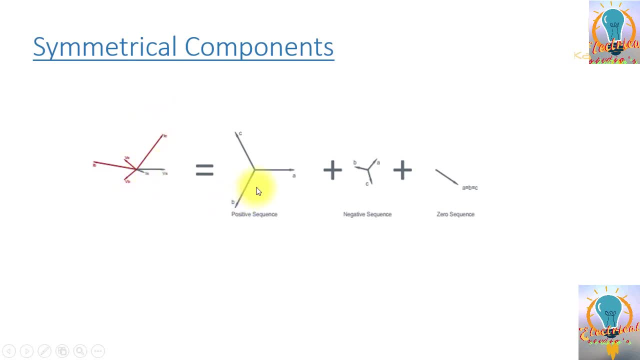 unbalanced system, as I have told you, can be equally presented, can be presented by a positive sequence and by a negative sequence and by zero sequence. so we we have to decompose an unbalanced system into three different sequences so that we can use it easily in your calculations. so this is just an. 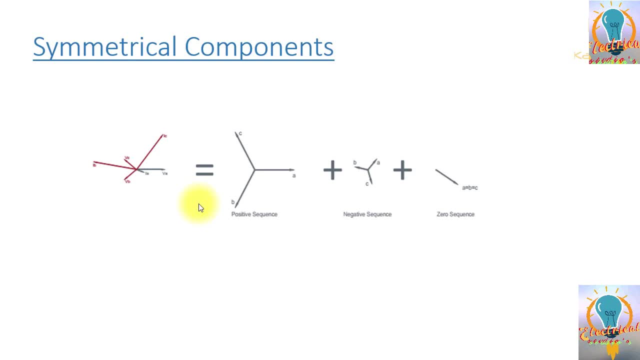 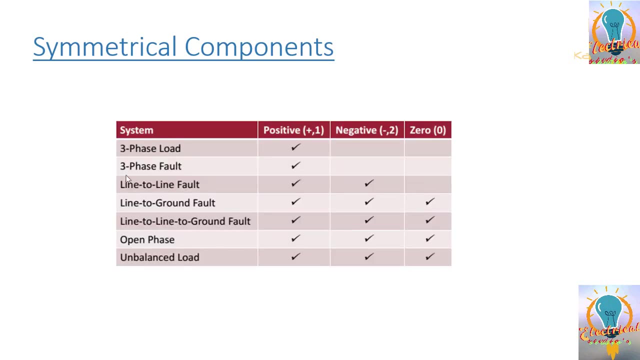 introduction idea of what synth symmetrical components. so here is a summary and definitely will see different types of fault and which type of components are available in it. for example, if for a three-phase load only positive sequence components are available, for three phase faults also the positive sequence available for line to line faults positive and 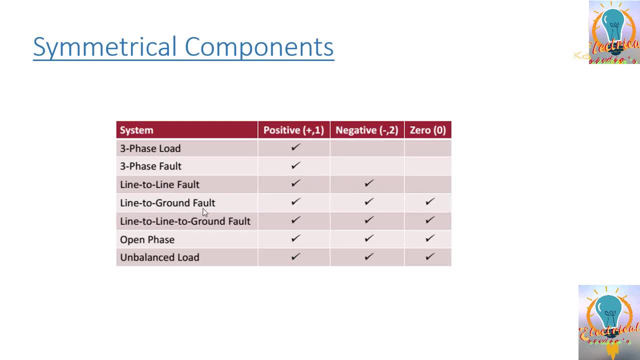 negative sequence is available. for line to ground: all three sequences are available. for line to ground to to fault line to line to ground fault: all three components are available. open phase- also positive, negative and zero sequence available if the phase is open. for unbalanced load: all three. 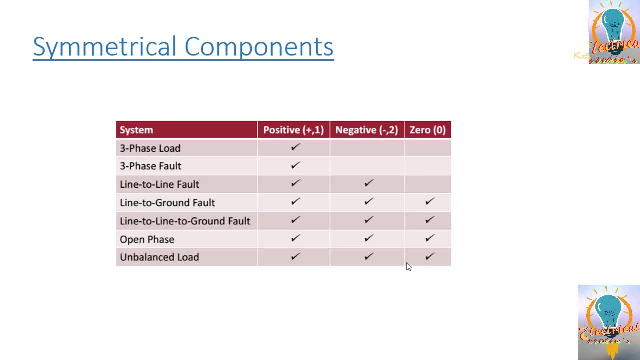 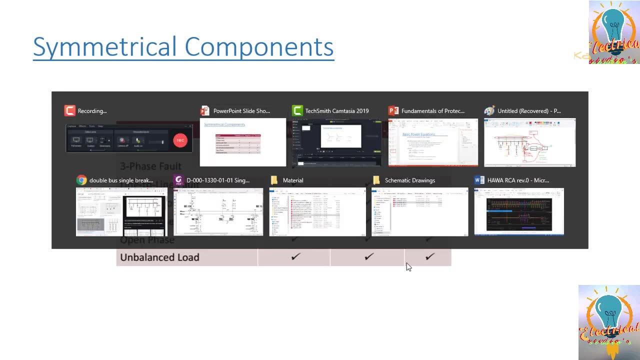 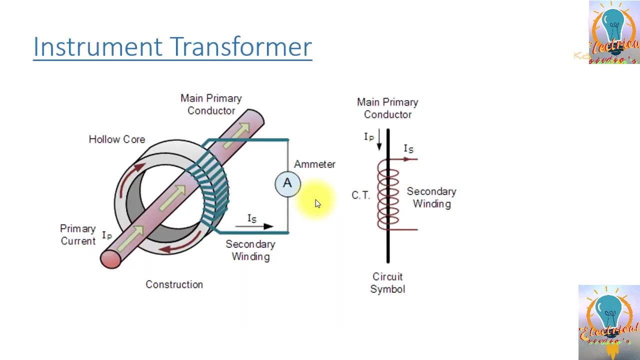 components are appealing. so this is just a summary and explaining their different types of forwards and conditions and availability of components. thank you. so in the substation there are two type of instrument transformers are available. one transfers terms of balances, adding zero sequence and so on, and its phase of change can very akan. 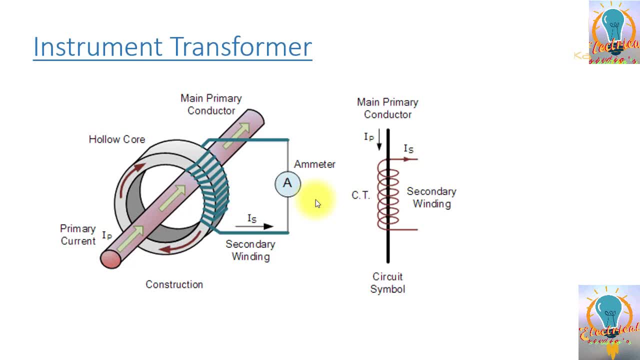 esa da huечение in semi output path. so let me put Netflix, and quite clearly this is a piece aдыman. so in the substation there are some secondary components which, clearer having to stay all four transformer is called as a current transformer, whereas the another instrument transformer is: 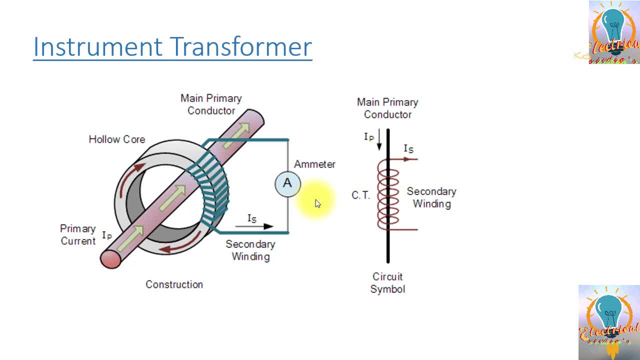 called as a voltage transformers. so we will start with the current transformer. so this is basically very simplified diagram of the current transformer. so there is a conductor and this is called. we are calling it as a primary IP. primary current is flowing through it and this is basically the 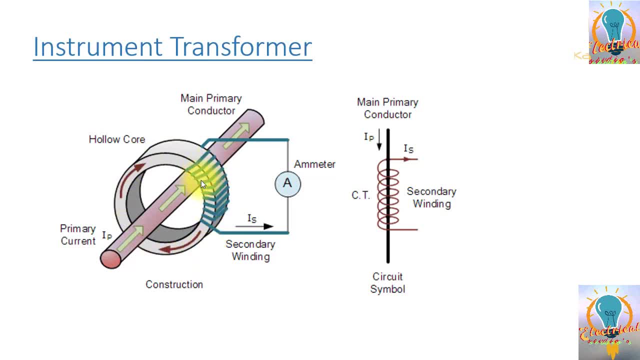 hollow, core type of city and this is basically guessed. and ratio- primary trend ratio- will be considered in this case 1 and secondly, you can see there are lot of trends and then you can see that there is a primary current and, depending upon the ratio, there will be a city secondary. 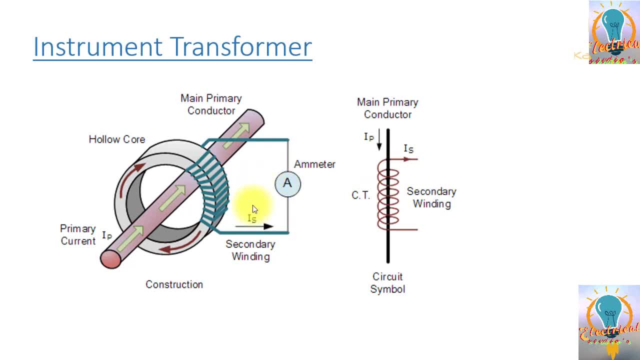 current and it is connected to ammeter. so, for example, why we are using here a current transformer, why we consider exactly a circuit? because, for example, in a circuit there would be aैon MCA. we are not measuring directly the current in the system. so the reason is, for example, if you are 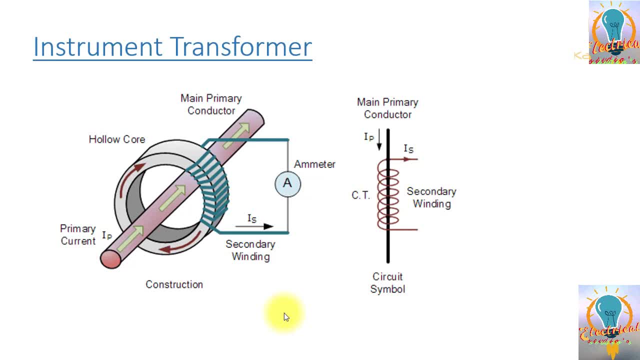 working on 132 kv level. first of all, if you, if you are trying to put the ammeter in the circuit at 132 kv level, you have to design a ammeter at the insulation level of 132 kv, which will be extremely costly, costly and and not feasible. the size will be very big and it will be extremely 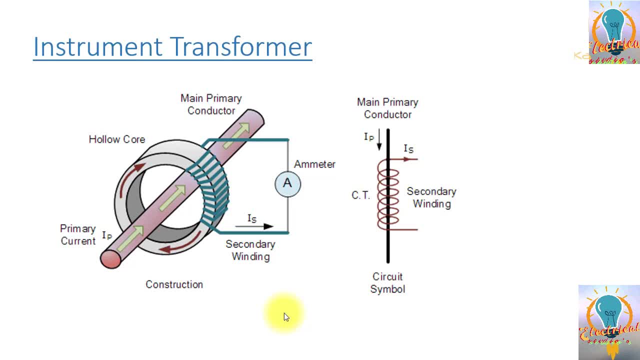 costly. secondly, uh, if you want to connect the equipment at the high voltage level, the current, for example, at the high voltage is flowing, is 1200 ampere. so then you, it means that you need to design a ammeter at 1200 ampere rating, and this size will be again huge. so the best idea is to 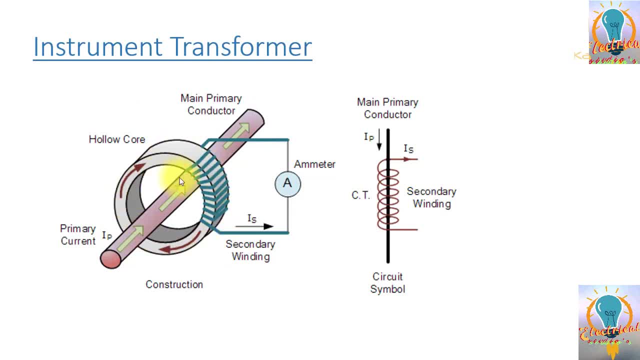 step down, to find a way to step down the current and also to isolate the voltage and connect it to some smaller device at the remote area, remote place, and you can do the measurements of current or voltages or you can do the protection features. for example, i have designed this, uh. for example, we have designed a 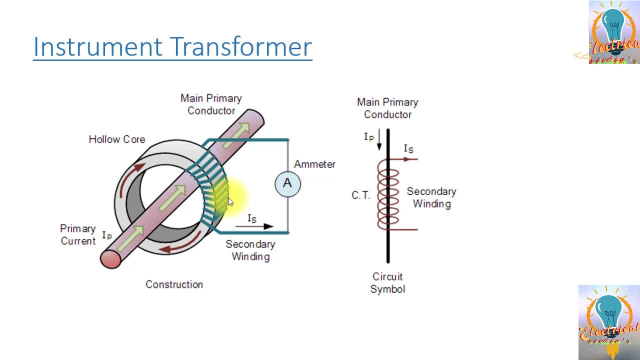 transformer. because, you know, the transformer has basically, uh, the transformation ratio, so it can down. when it step down the voltage, it is increasing the current. and what is stepping up the voltage? it is basically decreasing the current. so here you can see, we have put a ring core ct. 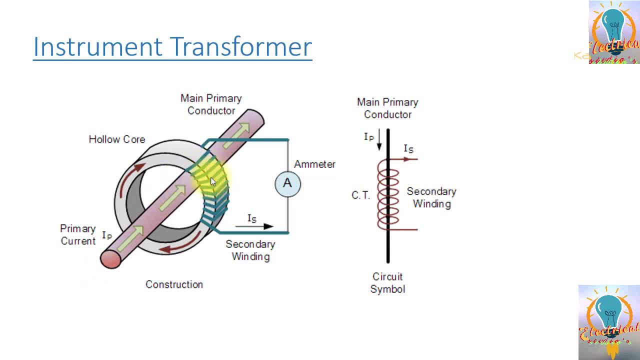 and we have put a is, a ct is kind of step up transformer, so voltage will be up but the current will be reduced, so it is put in a ring so voltage will be negligible. here and we are, we have shorted ct secondary and you can see in this way if, for example, 300 ampere is flowing through primary. 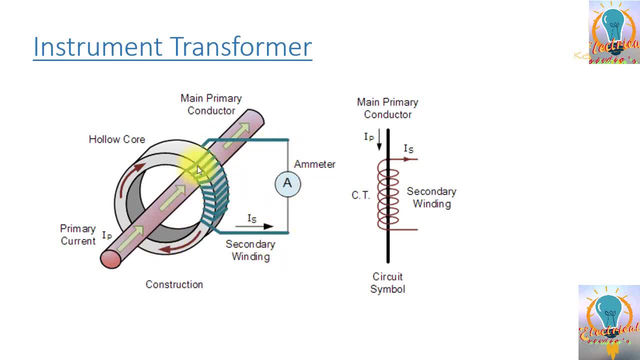 there will be less current at the secondary, depending upon the ratio. so we can define this ratio by: n. 1 divided by n 2 is equal to i2 divided by i1. so this is the we are calling it. this is as a primary, this is the bar is showing as a primary and this uh secondary current is shown by: 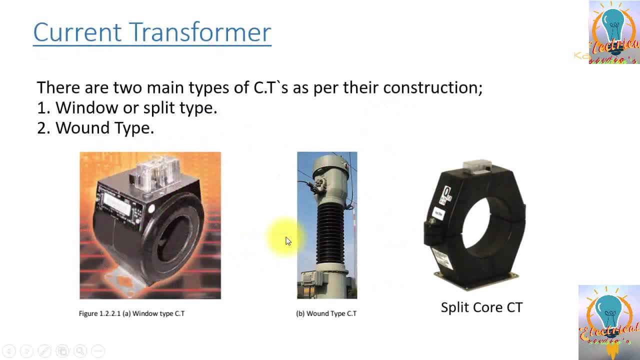 is and ip mediaIridge问 port of workBLE ACI ACI, ACI, ACI, ACA, ACI ACI ACI ACI. so this is a little concept of the CT, that why we are using CTs or even VTs in the substations. 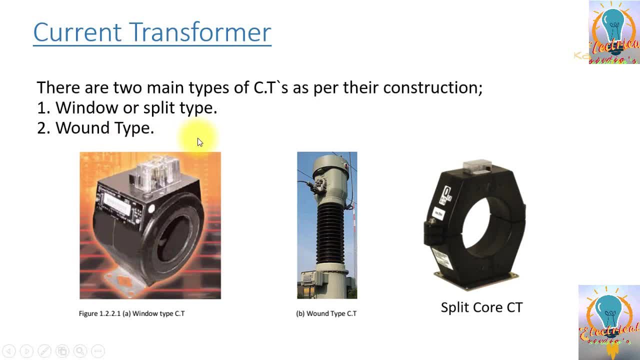 this is one of the reason and there are two different types of CTs basically available. one is wound type or window type or split type. another one is wound type. so this is example of wound type CT, so the conductor is connected at the one terminal and another. 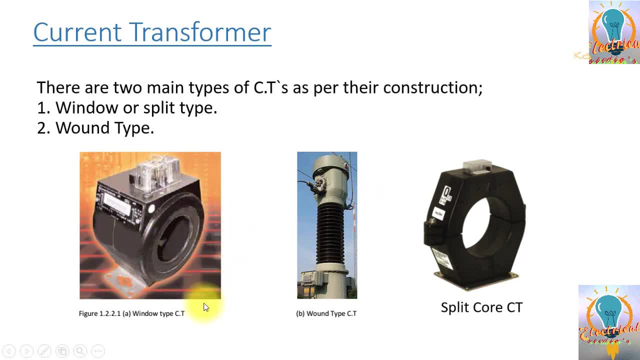 terminal is connected to the other side, so this is basically the window type. so conductor is passing through this. for example, you can pass a cable through this and this is split core type. so even if the cable is already installed, you can split it, open the core and 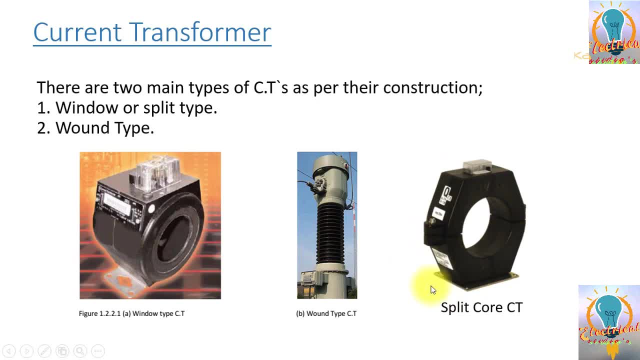 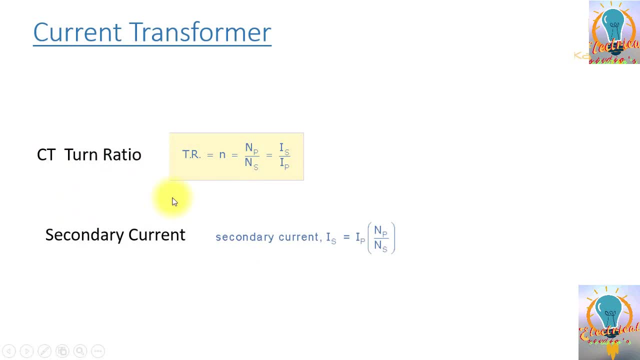 you can then again connect the core back and tight it. then you can connect the CT in series. so, as I told you, the CT ratio is measured by the simple formula Np. primary trans divided by secondarytrans is equal to secondary current divided by primary current. so secondary current can be calculated by using the formula. this is equal to primary. 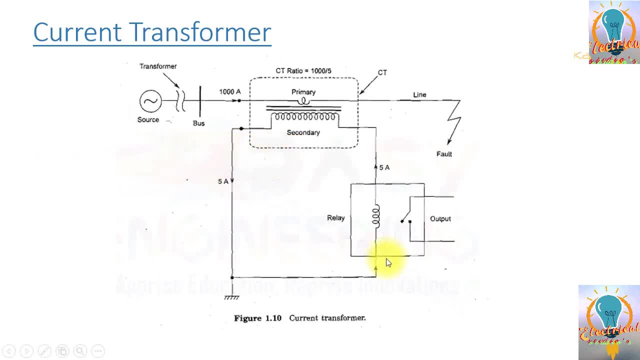 current into Np divided by Ns. this is basiclly a very easy, simple presentation of current transformer. so you can see this is the bus and this is the generator and you can see this is the generated signal which we are from know from the AC. whole Seems like there. 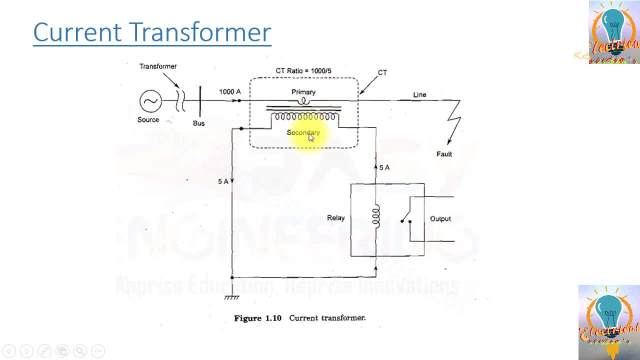 we have put our CT in series and this is basically a secondary winding and this is called as a primary winding of the current transformer and this is a relay which is sensing the current. so here ratio, a CT ratio is 1000 by 5 ampere. so 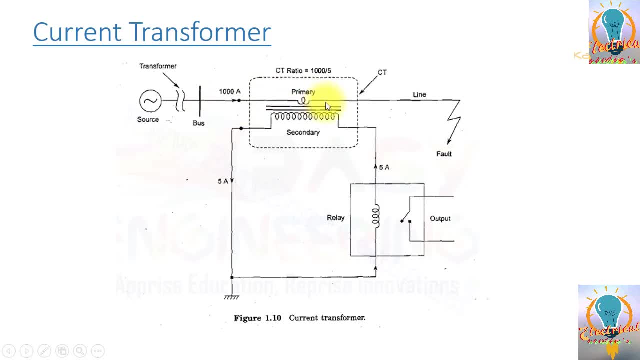 for example, if there is a fault, 1000 ampere is flowing through the primary, but the ratio is such that if 1000 flow on the primary, 5 ampere should flow on the secondary side. so the 5 ampere is flowing to the secondary side. so relay. 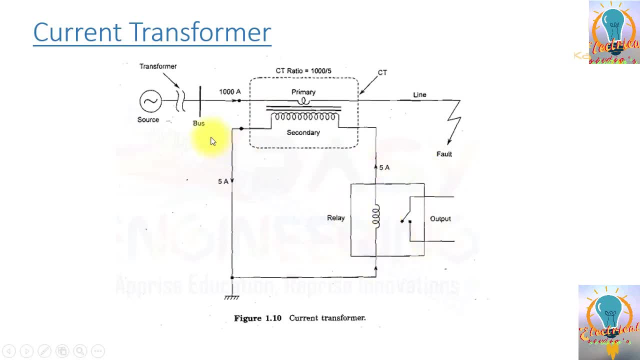 we have installed only 5 ampere relay. the fault current here is 1000 ampere but, just for your curiosity, the normally the fault level is in kilo amperes and we are using the relay because, thanks to the CTs, we are using relays of. 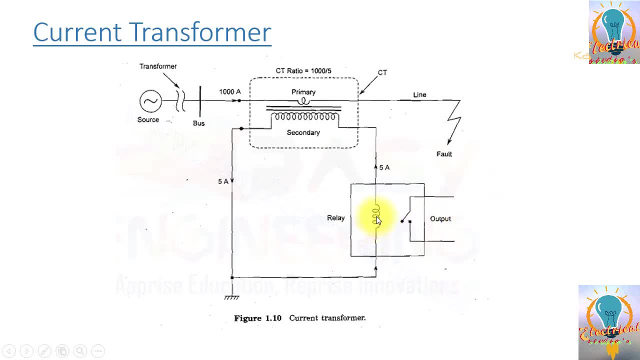 only 1 ampere in the field. so the relay, for example, setting is 4 amperes, the relay will pick up and it will operate and it will trip the breaker and to isolate the fault. so this is the function of current transformer: it is reducing the current to manageable level. 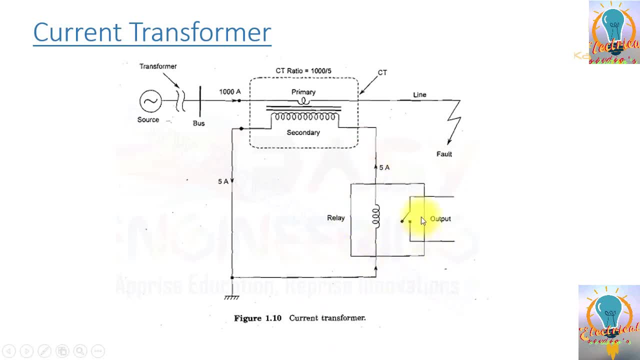 so and in the relay we are in the modern relays- there is option of putting CT ratio and even you can do the settings in primary or secondary. there is a switch you can select in numerical relays so you can do after putting the ratio. you can do the settings in primary as well as in secondary. 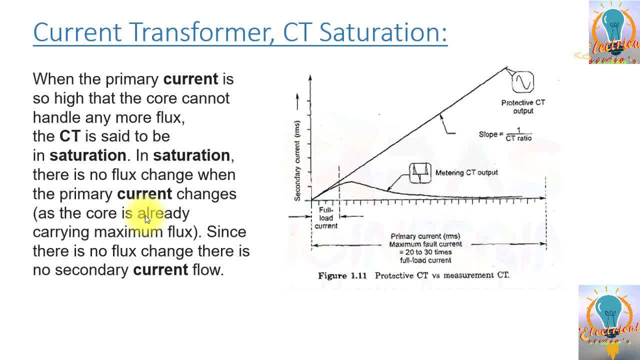 so then there is another concept of CT, which is called as CT saturation. so when the current passes through the CT core, basically CT core also has some capacity. so when the flux is full, when the flux capacity is full, there is no rate of change of flux in the core and you can say the core is saturated. so 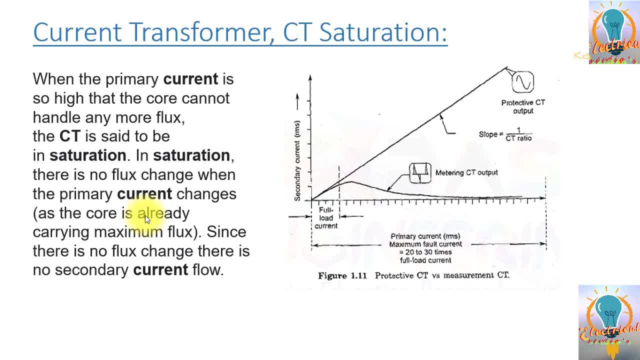 when the flux after some certain time is full and there is no rate of change. so it means that there is no rate of change, there will be no induced voltages. so we can say the core is saturated and the output of the CTs is reduces and it seizes and the waveform is. 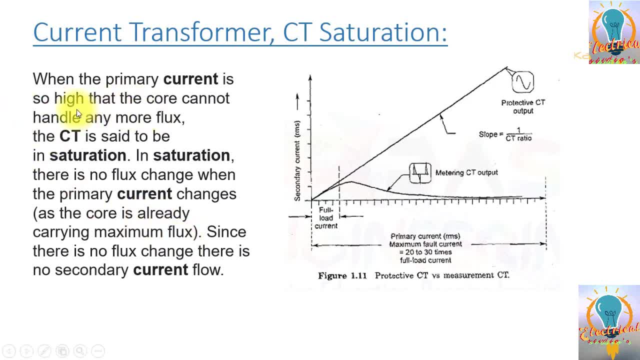 very bad shape when the primary current is so high that the core cannot handle any more flux. the CT is said to be saturation. in saturation there is no flux change when the primary current changes as the core is already carrying maximum flux. since there is no flux change, there is no secondary current flowing, so 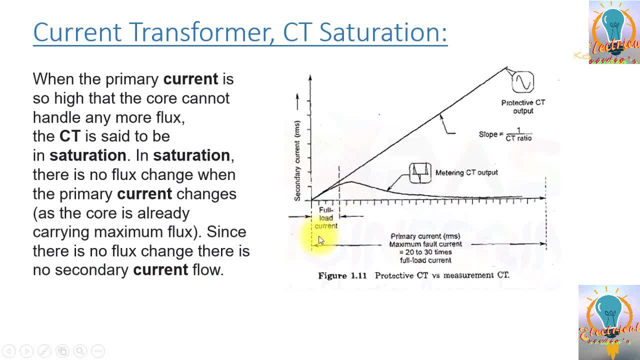 here I have shown you. this is the full load current. this is basically the meeting. we have shown the meeting CT core. so meeting CTs are designed to saturate after certain amps, for example, if 110 to 120 percent. after that they are designed to saturate because they are not there for protection. so if there is 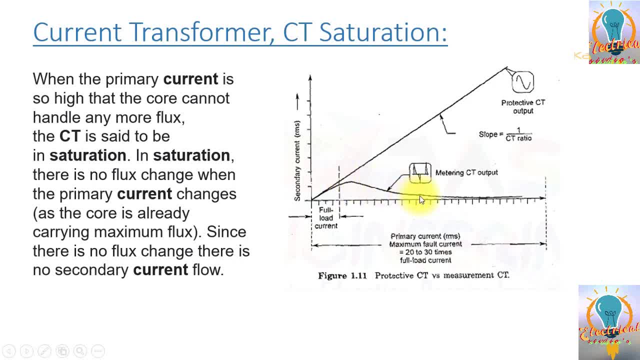 too much current they will saturate. no need to make a CT of bigger size for the metering because it will operate always within the maximum load current and you can see this is basically the waveform for the protection CT. so protection CT will not saturate because it it when the fault comes. the level is. 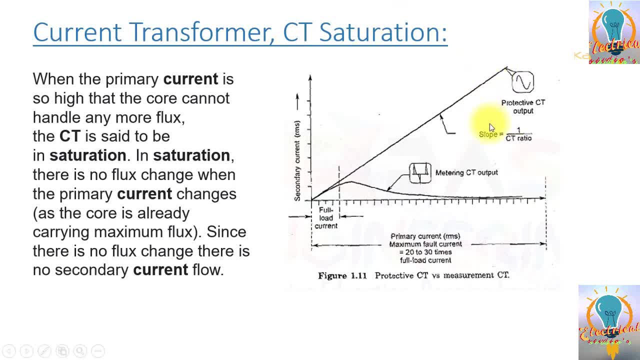 in flow amperes and the protection CT has to be connected to the protection relay and the protection relay has to decide during fault time that to trip and to make all decisions. so that's why the protection CT- you can see here the waveform of protection CT- is still sinusoidal at higher value of 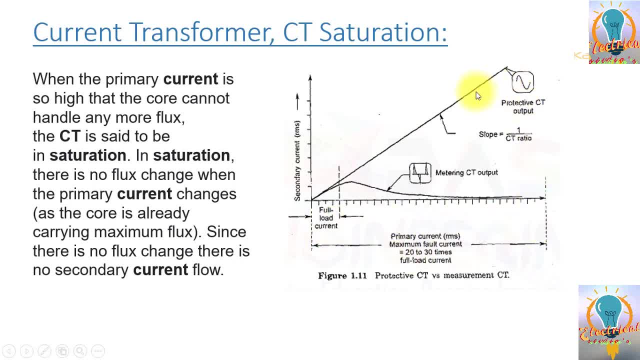 current, this is approximately 20 to 30 times. the waveform is still sinusoidal. so, whereas if you see the meeting core, the waveform city saturated at this point and you can see the waveform is no more sinusoidal, the waveform is a sawtooth. it is in the form of spikes. 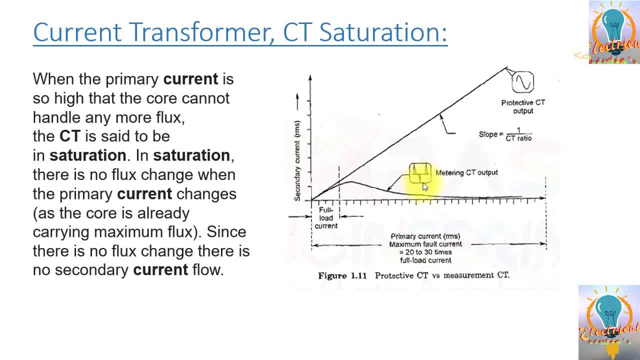 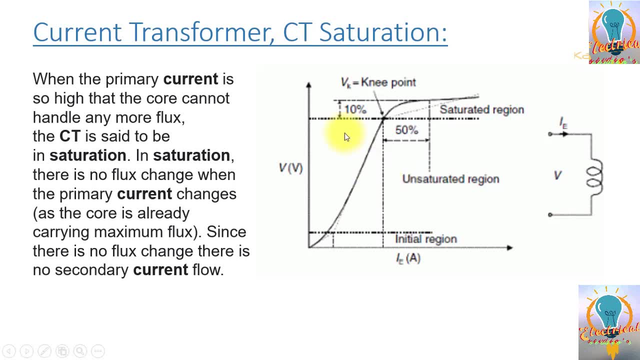 so the the protection city is not saturated, whereas the meeting city is saturated. so how you can define the saturation? so when the current is increased, secondary current is increased. the exciting: if you, if you increase the voltages, if you are injecting the voltages to the city, 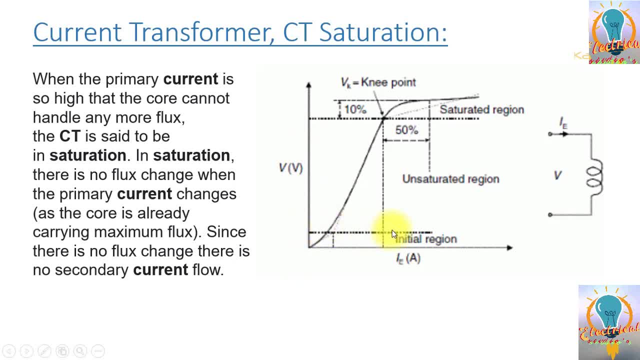 secondary. if you increase the voltages the current in the city secondary will also increase. so there is a real linear relationship. in the start 10% increase in the voltage will also resulted 10% increase in magnetizing current in the city secondary. but point will. 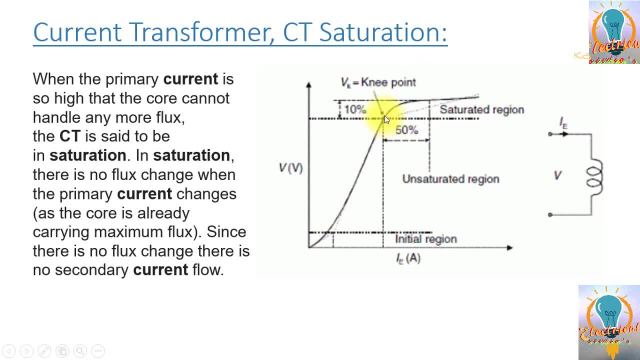 come where 10% increase in city secondary, this attrition will start happening, will increase 50% current in the exciting core. this point is called as a knee point and this knee point is defined on the normally city nameplate or in the manual. you can find out the knee point normally. we are testing the relay and 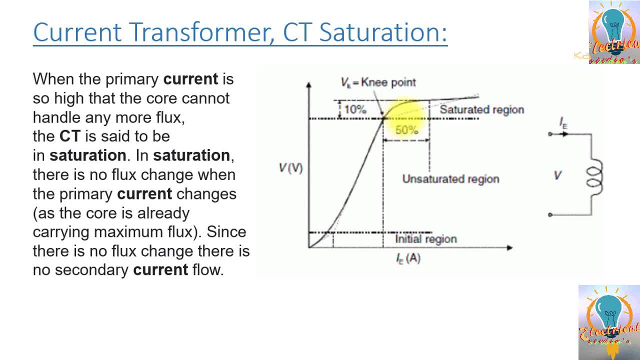 we are checking the knee point of the city and automatically also the knee point is calculated. when the primary current is so high that the core core cannot handle any more flux, it is said to be saturated. so this is an again the example of city saturation. you can see this. 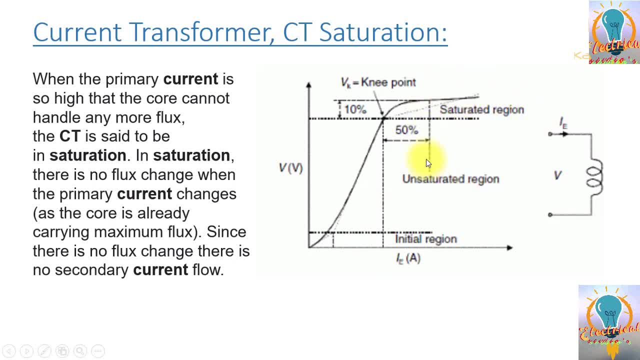 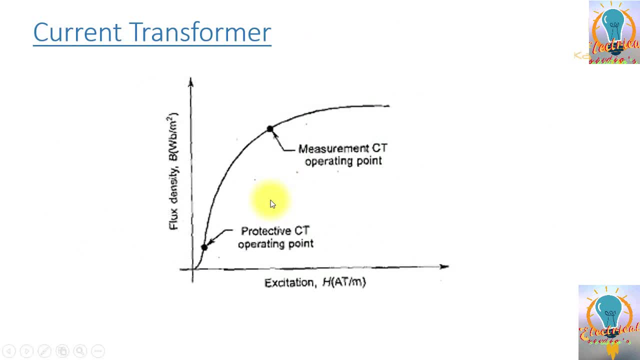 is the saturation, that's the ratio reader saturated region and this is the unsaturated region. so, and this is the knee point, as I explained you. so again, we are showing the operating. this is the basically flux and excitation diagram and you can see this protective city. 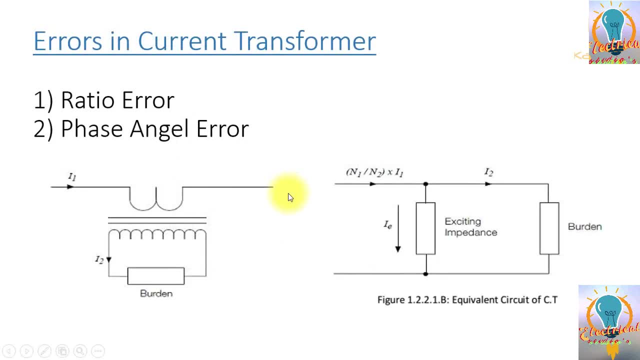 operating point, measuring city operating points. then we will discuss some errors in the current transformers. so there are two type of the errors in the current transformer. one is a ratio error and another one is a phase angle error. because a ratio error is because of excel. each transformer have also exciting in order to drive the magnetism it will draw. 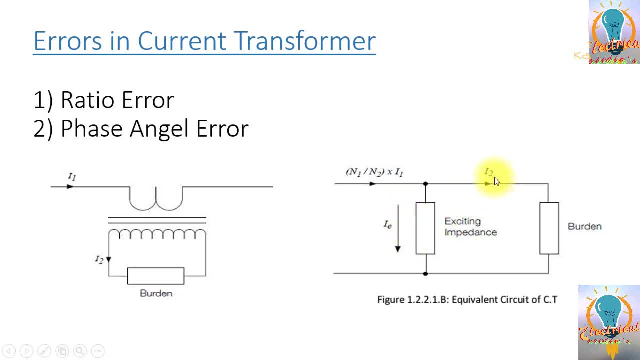 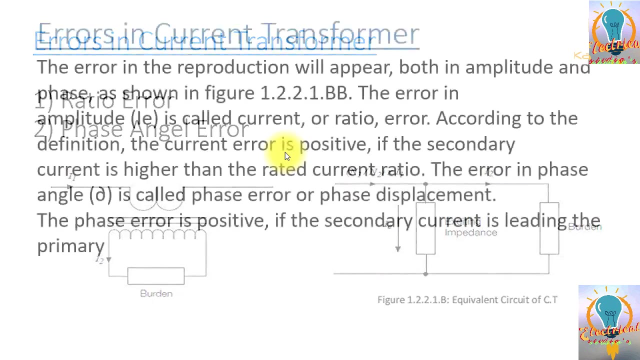 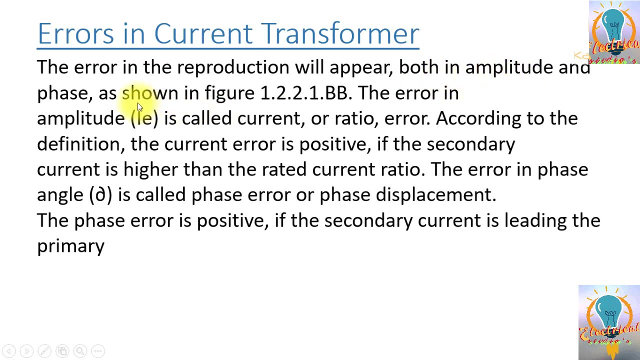 some exciting current. so this exciting current will be minus from secondary i2 current. so this exciting current is basically will create error in the city secondary. so design should be done so that error should be removed off of limits and the error in the reproduction will appear both in amplitude and phase as shown in figure, and really in the amplitude is called ratio error. 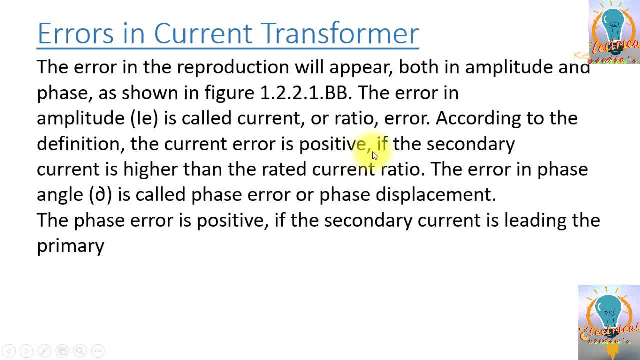 or into definition. the current error is positive if the second recurrent is higher than the rated current. the error in the phase angle is called phase error or phase displacement. the phase error straight from the orientation and surface strain. and finally extra phase tilt, which positive if the secondary current is leading the primary current. so nowadays, 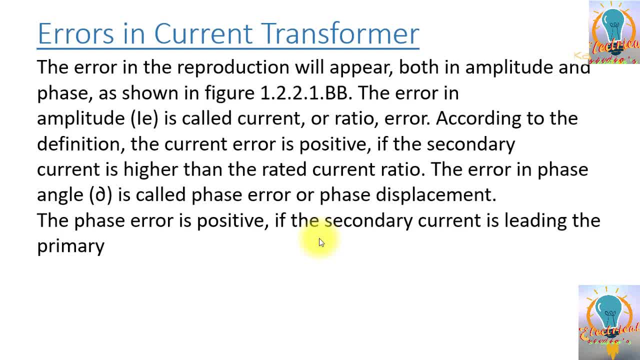 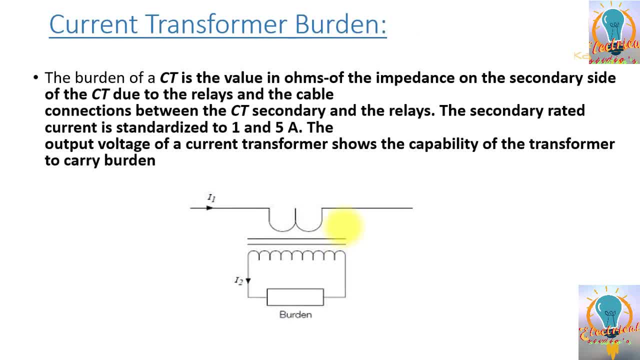 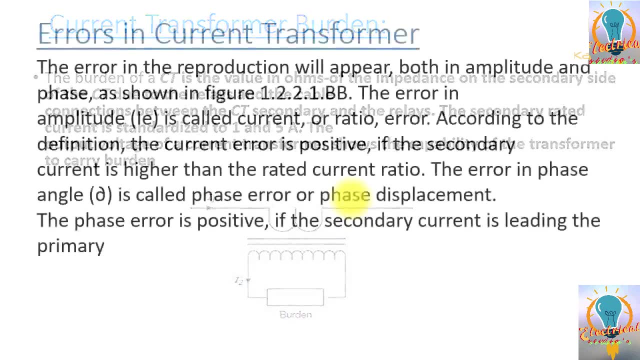 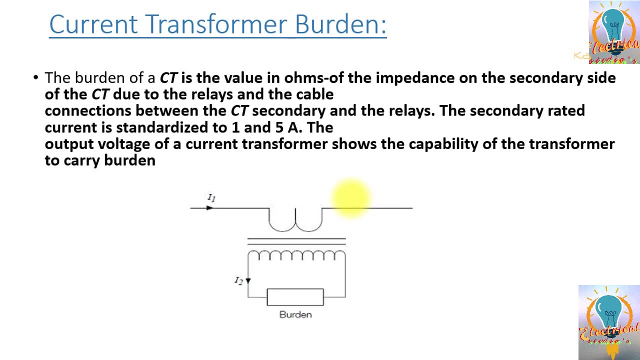 the equipments are automatically calculating phase angle errors and the ratio errors and then they are giving the results. so another topic is current burden. so we will discuss, okay, the current burden. the burden of the CT is a value in ohms of the impedance on the secondary side of the CT due to relay. 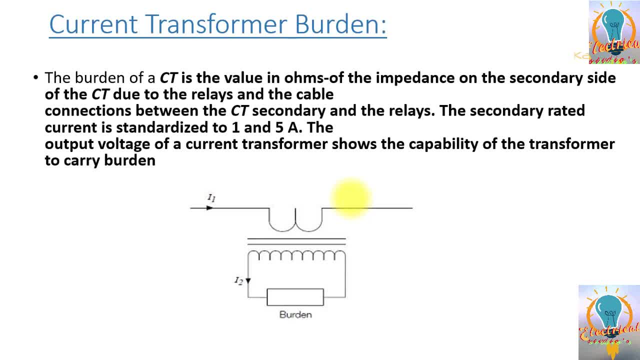 and the cable connections, CT, secondary and the release. the secondary rated current is standardized in 1 and 5 amps. the output voltage of the current shows the capability of transformer to carry burden. so whatever you connect to the secondary side in ohms is called basically a burden. so this burden is the 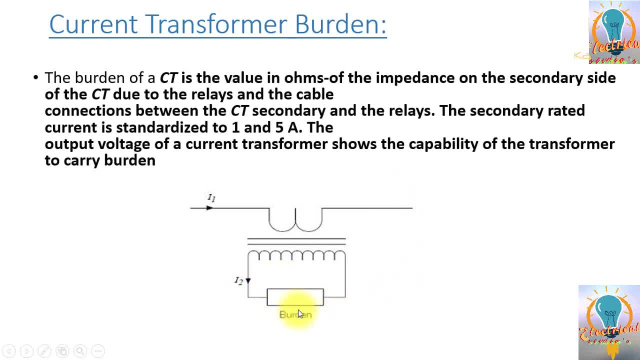 sum of lead resistance and the value of current and the VA burden of the relay, which is already defined in the in the manual. and also you can measure the VA burden: simply you need to inject rated current, 1 ampere, 5 ampere in the loop and then you can measure the voltage and then you 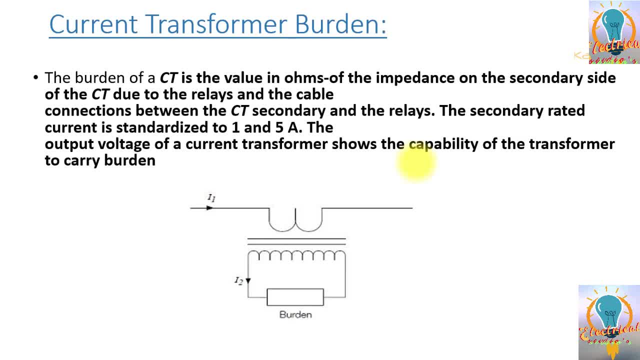 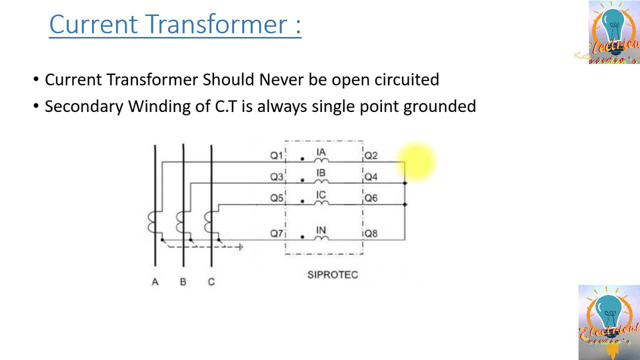 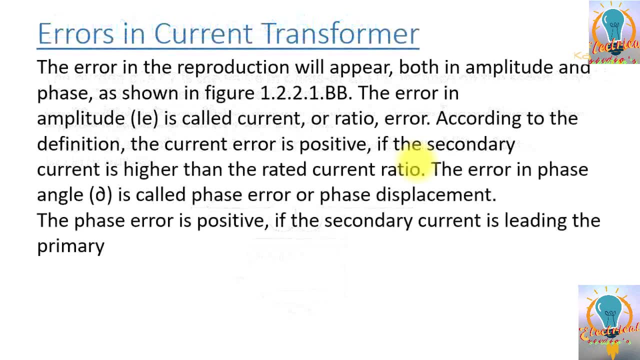 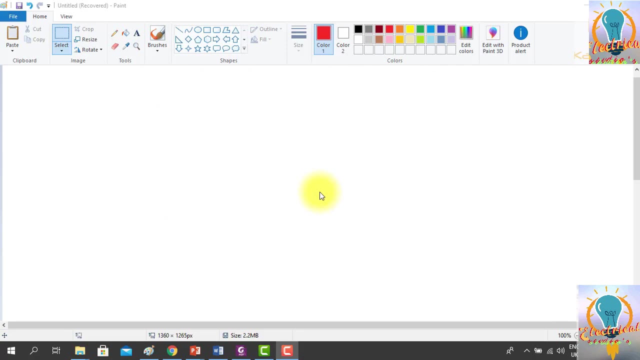 can multiply V into I to calculate the VA, actual VA burden in the field. then we will discuss here. the current transformer should have never been open-circuited. secondary winding of CD is always single grounded. hey friends, previously we have seen something regarding current transformer theory, so I will discuss with you now practical problem that we have faced. so 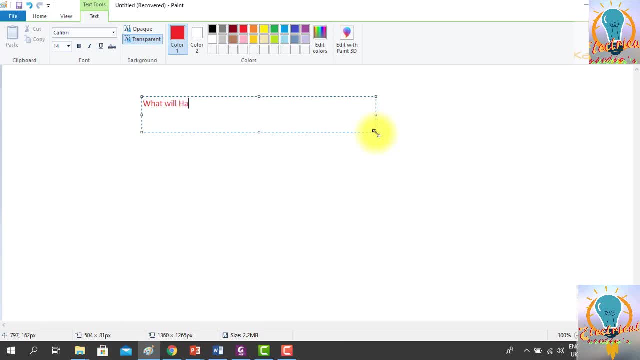 question is what will happen? in short, how it reacts to this coil if we swap, if we swap netring and protection core in our system. so what will happen if I connect, if I have a protection relief, for example? this is a protection relief and this is the major part of refining the coil. 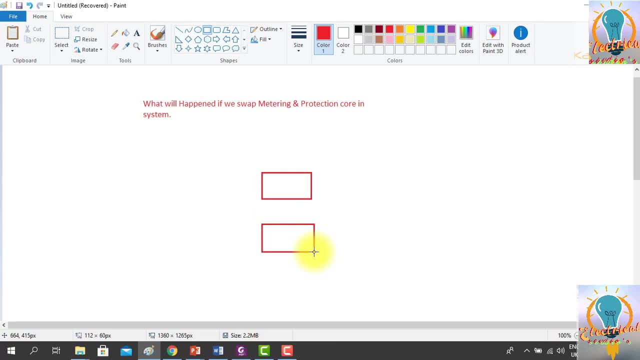 and this is the measuring device, and I have two cores, CT cores. okay, this is the conductor, for example, this is a core one, this is a core two and this is a protection core 5p20, for example, and this is measurement core plus 0.2. so both have same ratios, like 300 by 1, 300 by 1, okay, so 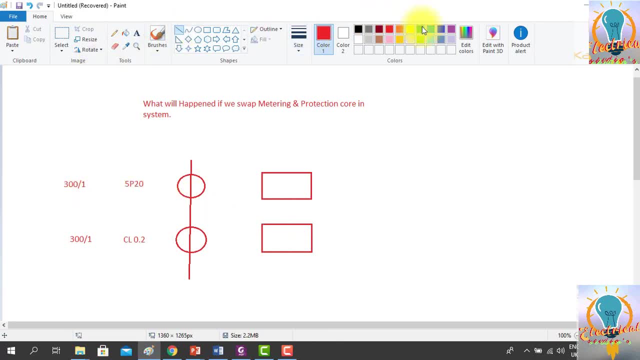 both have same configuration and if I connect this mark, this is basically the over current relay, for example, over current relay, and this is basically the meter. so if I connect this, what happened practically? and we find the issue, if I connect the metering core to this over current relay and the protection core I connect to the metering. so 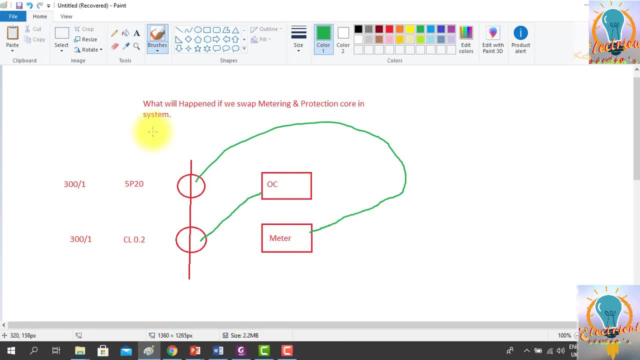 what will happen? so I have, we have just finished in a lecture. you know I have explained you everything. so what? what do you think? what will happen if we make different connections? both have the CT ratio, similar CT ratio and both have similar second DCT ratio. so what will happen? I? 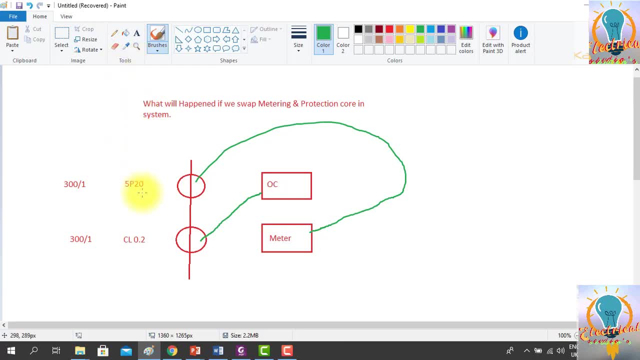 will explain you now. just now, for example, the fault current is coming 20 times. so if there is a fault phase to ground fault, there will be a current. so let's see the fault current here is flowing through. this is 20 times. it will be equal to 300. 300 into 20, which is equal to 6,000 or 6. 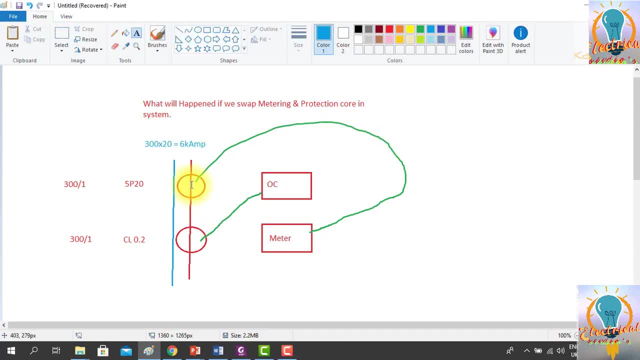 kilo amps, so 6 kilo amps is flowing through this. both of the CT and the current current is coming. so when six, when the current is reaching to instead of 300 to 350, for example, so there will be six kilo amperes flowing. so this CT metering city is designed to saturate at overload. 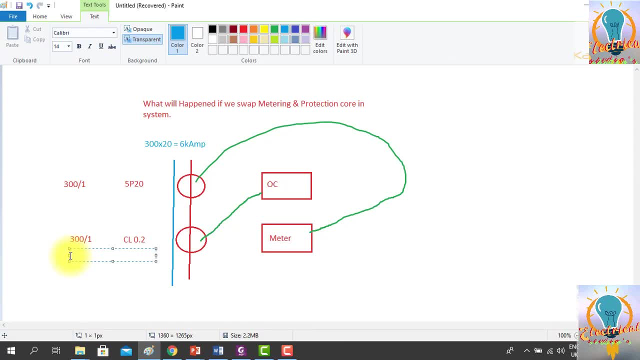 so this will be saturated at 120 percent. so it will be kind of 360 or maximum 400 amps. this CT will saturate. so the fault level is 6 kilo amps. if this CT is saturated there will be output of the CT. secondary will be zero and the over current relay will not sense a fault. whenever there is a fault, this relay 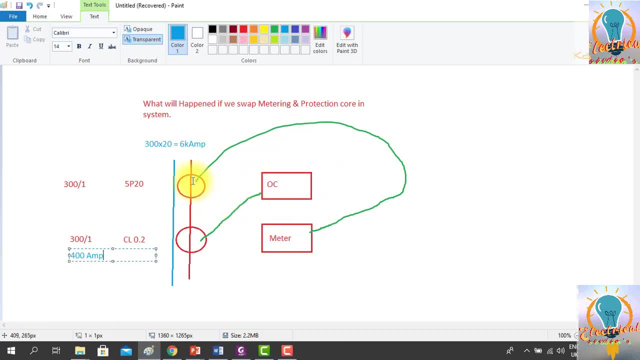 will not sense a fault and at the other end, when there is a fault, so this fault current will be fitted to the meter. so this current will be in the range of, for example, we have 6000 amps, so we will see how much will be the secondary current. 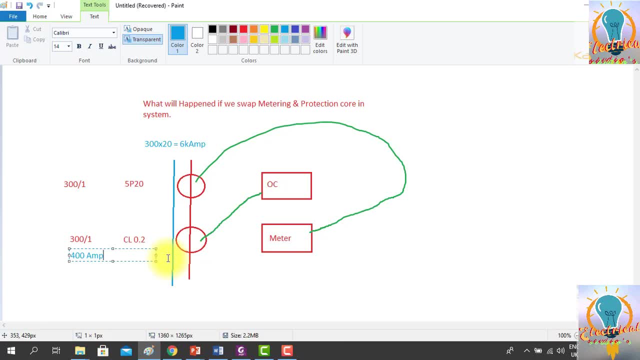 6,000 divided 300, so it will be approximately 20 kilo ampere will flow through the meter. 20 empires 20 amps, so this 20 amps. we can also damage the meter. but the more damaging is that the protection will never operate in case of fault. 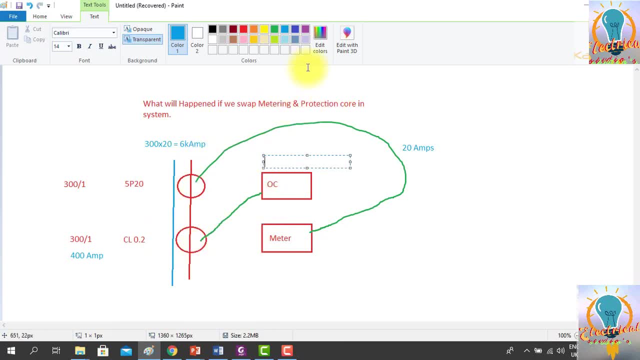 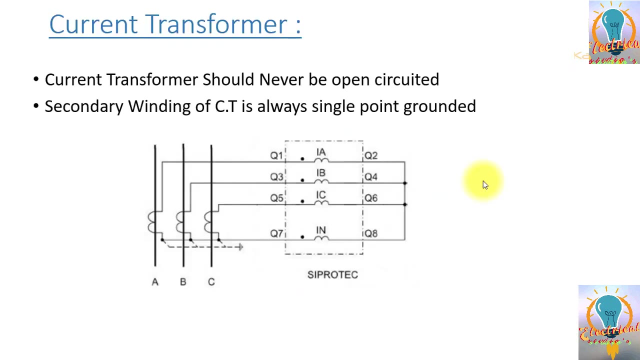 protection, specific protection, is not operating. another protection as a backup protection will operate. so this the problem: that we find out one of the substation and this is very practical example that how the metering and protection core works. thank you very much. hey, friends, it's important to note that for the CT, the city's current transformer, 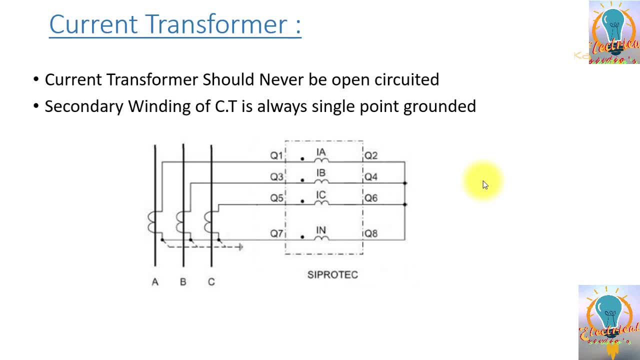 circuit should never be open circuited in any case. so this is because that current transformer generally work at low flux density. the core is made of high quality material. to give a small magnetizing current on the open circuit, the secondary impedance becomes infinite and the core saturates. this induces a 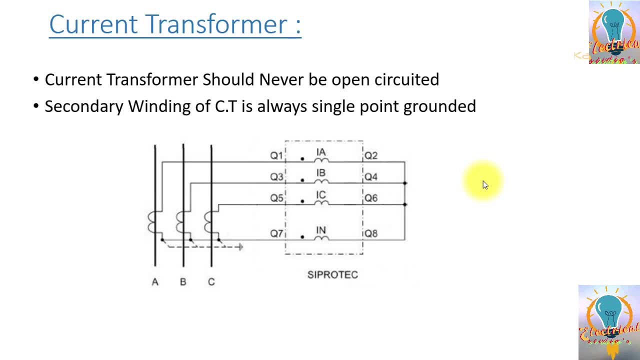 very high. voltage in the primary winding up to approximately system voltages, and the corresponding volts in the secondary will depend on the number of voltage in the primary winding up to approximately system voltages, and the corresponding volts in the secondary will depend on the number of turns multiplied by the ratio, since the city normally has much many turn raised. 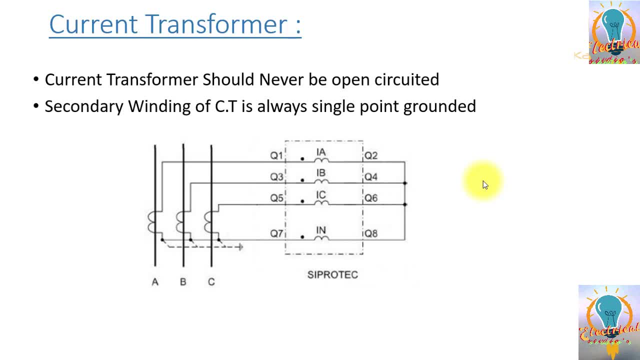 turns in secondary compared to the prime, the voltage generated on the open circuit CT will be much more than the system volts leading to flash over. so this is the concept and if the city is lightly or not loaded, the flashover will be not that much high. but if the city city is loaded and you are trying to 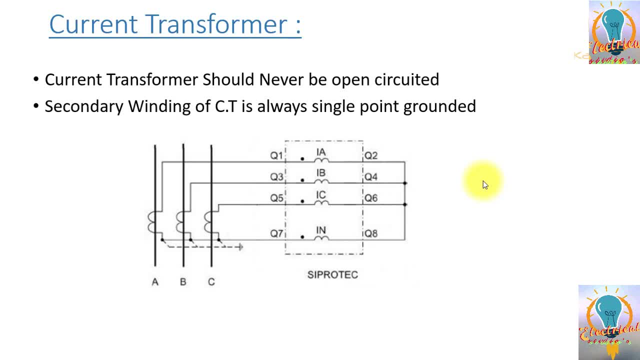 open the city, then the flashover: you can consider that it's. it's a very high flashover. so CT opening is always a very, very, you can say, dangerous phenomenon that has to be avoided. so need to take care. the city should know never be open in any case. secondly, we will discuss the topic as 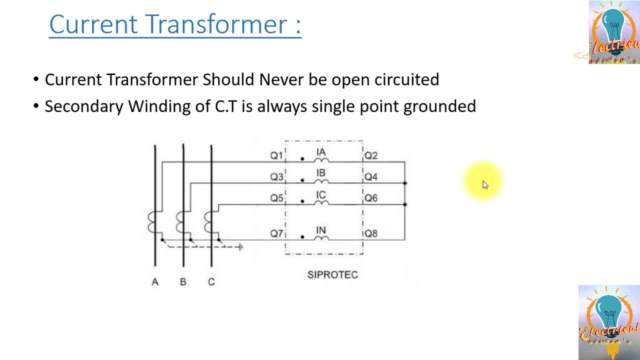 city secondary winding always is grounded at a single point, so it's always required. you can see in this figure this second you are always when the secondary winding is is grounded, the star point is made. so you can see then they have then the connections that they have from the yard they have taking. 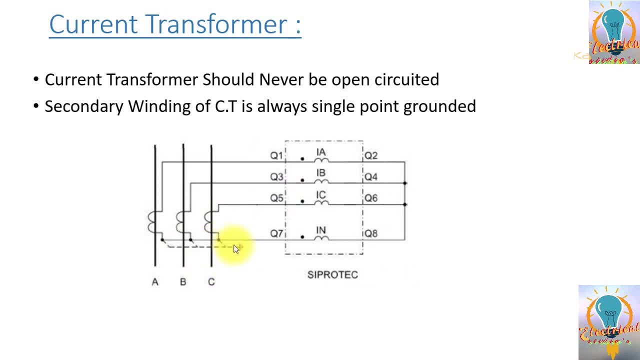 three wires to the relay and they make a star point, the such yard, and they make a ground connection and they take a single wire to the relay. so it's important to connect, basically star point at one point and avoid the multiple groundings. so grounding is important in order to make a reference. so if it is, 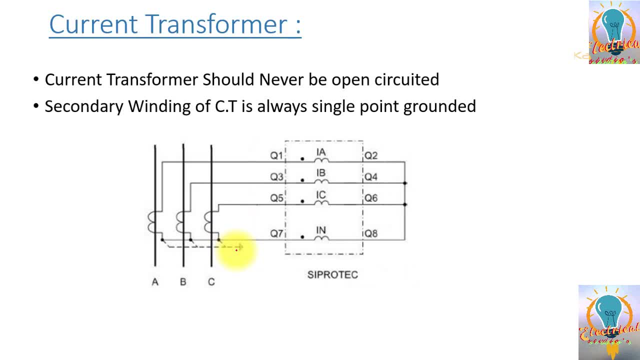 the system is ungrounded, there is no reference, solid reference, of phasors. and the second thing is: if there is an aesthetic charge or a voltage rise, it will be grounded through this earth. the third thing is: if you are grounding the city circuit for the multiple points, for example, if you ground from the suture, 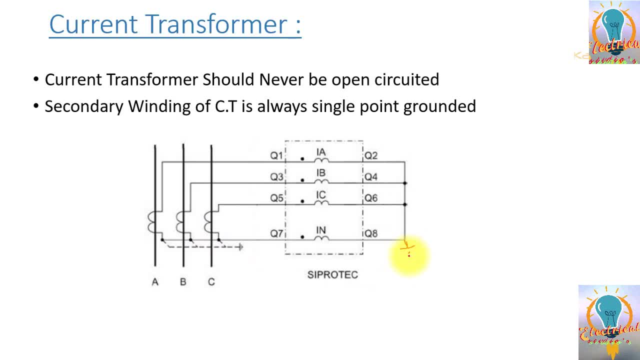 side and also if ground star point of the of the relay. so what could happen is. so now there are two paths or the earth fault current to flow. one is through this I am. another path is through the ground. so in some of the cases the current mostly flow through the ground and this earth element is bypassed. so if 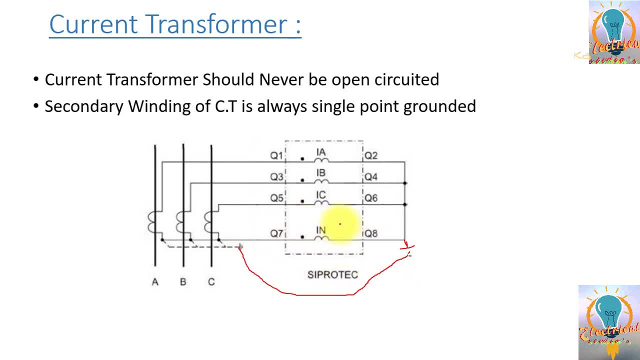 there is an earth fault, the relay will not be up. so this is an example that why it's important to make a thing at one point. so another thing that is important here is if you make a multiple down, you have ground here and here. so if there is a ground fault, so you know the in case of 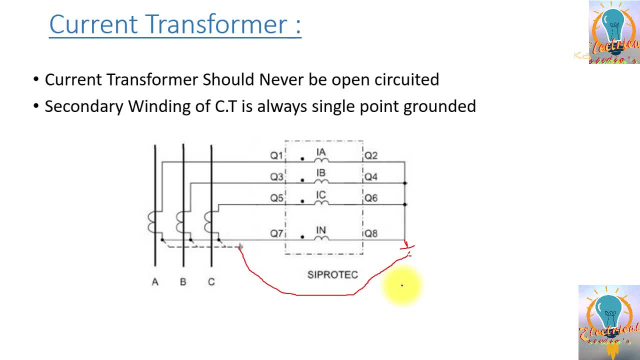 fault current. it will try to flow on all possible available paths. so this is also a low, low current path. so it will try to flow from the earth. it will go up and it will then try to flow through this element and then from the another earth fault element it will be coming down and back. so this is the another. 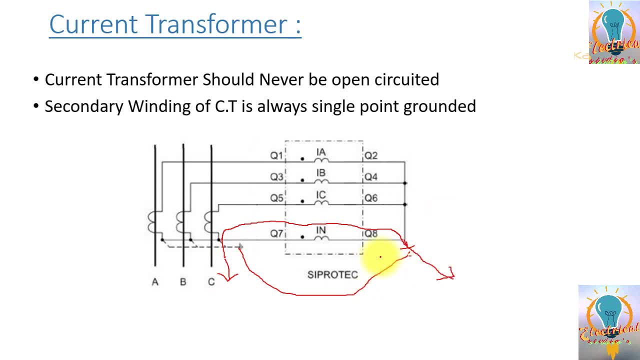 issue that could happen because of multiple points. so what happened? if there is a fault in system at another feeder, so you will find that the adjacent failure is tripped on the earth fault and you will keep on finding what's the reason, then reason is the reason. 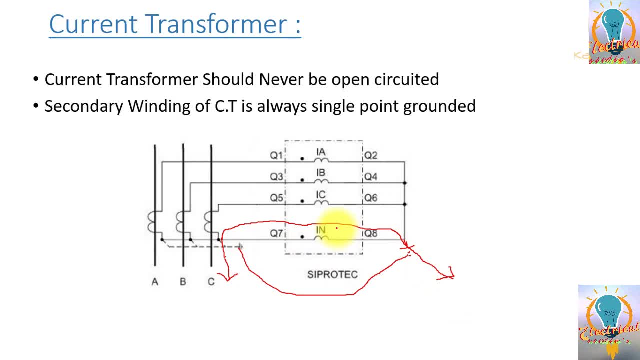 multiple point is grounded and the fault current has gone through this element. so when you will see the fault records you will able to know that there is a fault current at the same time when the fault appeared on the adjacent line. so that's why it is a practice to avoid the multiple grounding on the CT star points. 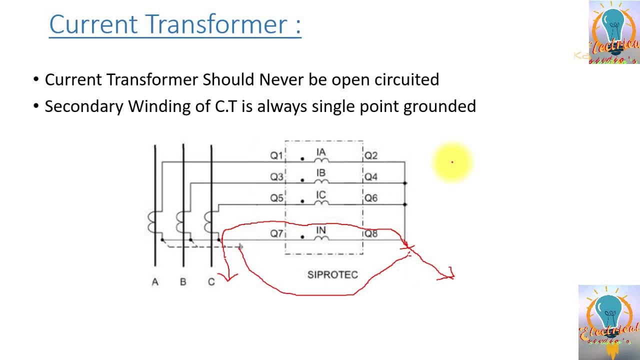 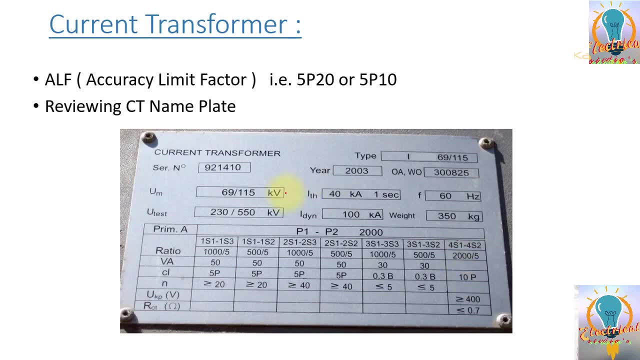 and there is a check. there's a very important check on each CT circuit to check the single point. I think, hi, friend, in this section we will just review a CT nameplate. you can see this is basically basically a CT. the rated voltage of CT is for 69 to 115 kV, the rated short circuit level for the see. 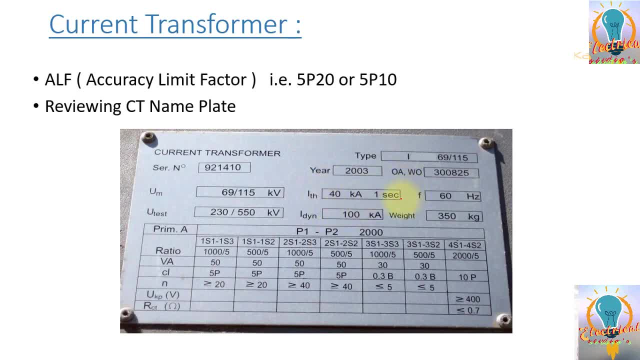 this specific CT is 42 ampere for one second. this is the short circuit rating of the CT. frequency is 50 Hertz and you test is 230 by 550 kV. so iDynamic is 100 kilo ampere, weight is 350 kg. so here you can see the. it has primary side has ratio of 3000 and 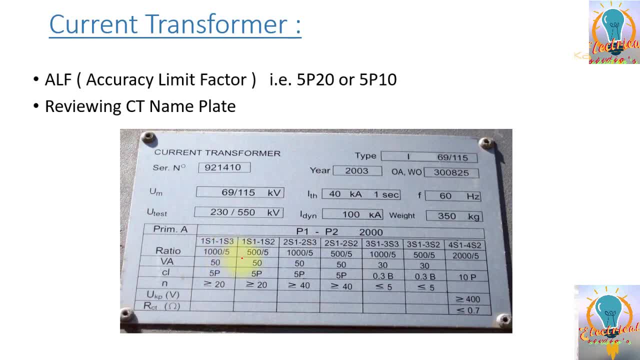 secondary side, there are different ratios. you can see 500 by 5, 500 by 5, 1000 by 5. so this is primary rating is 2000 ampere for the for the CT, whereas different CT ratios are available and selected. this is basically. 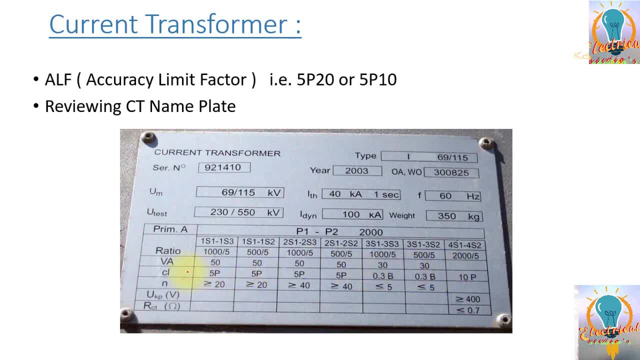 the VA rating of each CT is provided and this is basically the class. this is the protection class of the CT and this is basically the measuring class. and here you can see that this is the knee point voltage for one core. this is normally used for the bus power protection, so they are also provided. the 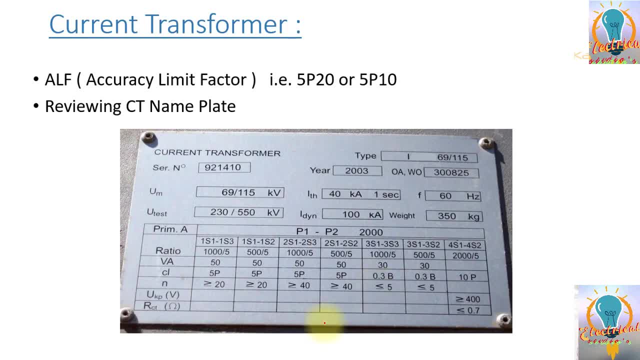 knee-point voltage for one core, which is for 10 P, and then they have provided also resistance of the city. this is used for calculation of basically CT sizing calculations and calculating the total burden. you can add this also in your calculation. so here you can see basically in this one they have not. 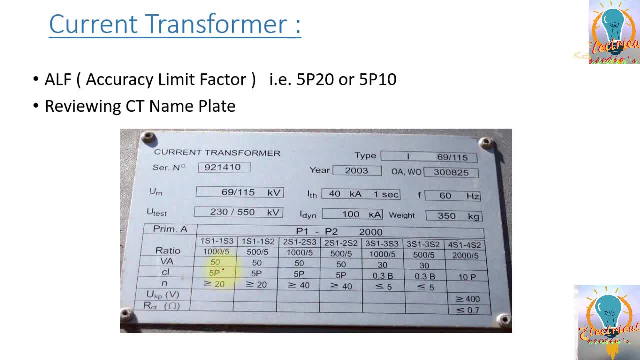 written. the accuracy limit factor in the name plate, like five percent, is present in the name plate number and this is used for the 5p10 or 5p20. they have not mentioned the times. what does it mean by 5p10 or 5p20? it is called. 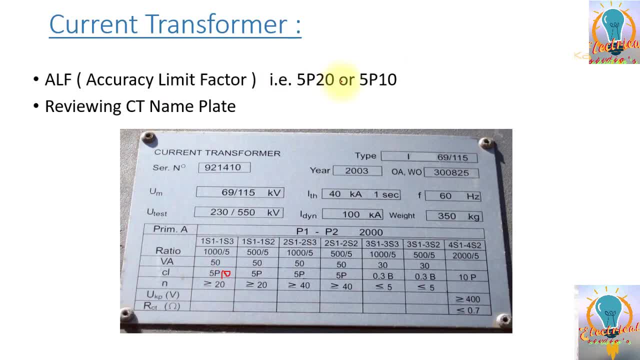 as accuracy limit factor, and meaning of this is that at 10, for example, 5p20 means at 20 times fault current, if the CT ratio is 1000 for this core, and this is if 5, if this core is 5p20. 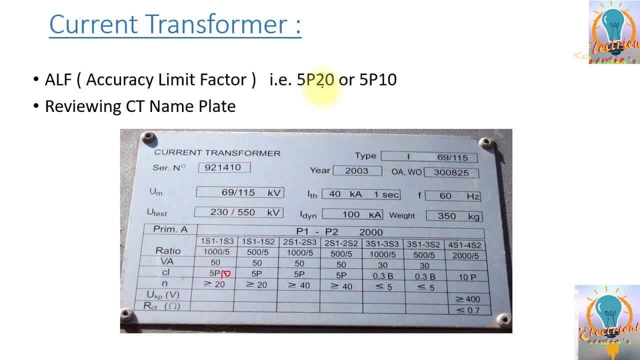 and 20 companies. 20 kilo ampere fault current is there, then there will be error in the reading will be 5%. so this is how the accuracy limit factor is taking care. so this is just it. little introduction about the CT name blade. hi, friend, in this section we will just review a CT name plate. you can see: 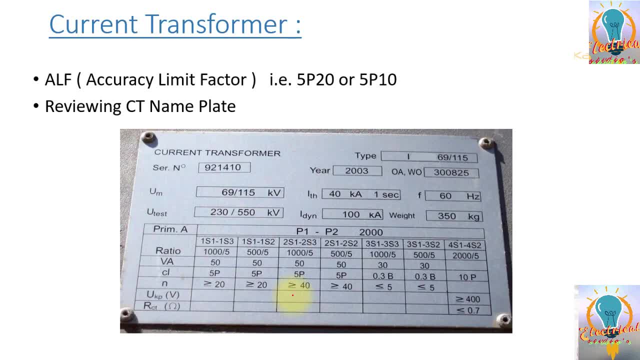 this business. basically, basically a CT. the rated voltage of CT is for 69 115 kV. the rated short circuit level for the see this specific CT is 42 ampere for one second. this is the short circuit rating of the CT. frequency is 50 Hertz and you test is. 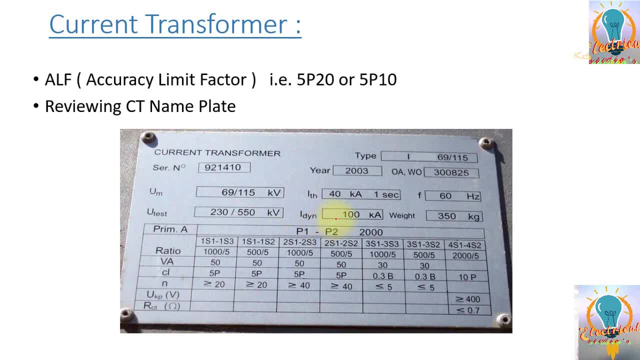 230 by 550 kV. so I dynamic is 100 kilo, ampere weight is 350 kg. so here you can see the. it has primary side has ratio of 3000 and secondly side there are different ratios. you can see 500 by 5, 500 by 5, 1000 by 5. so this is primary. 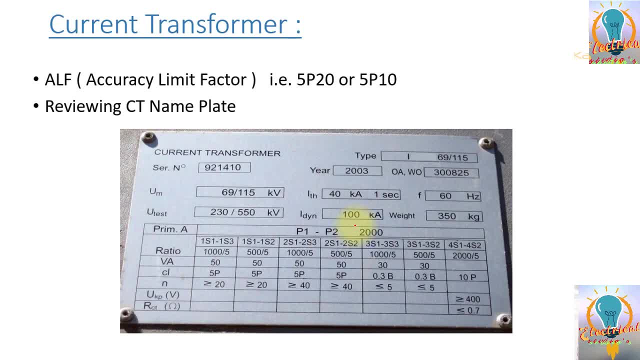 rating is 2000 ampere for the for the CT, whereas different CT ratios are available and selected. this is basically the V rating of each CT is provided and this is basically the class, is the protection class of the CT and this is basically the measuring class. and here you can see that this is the knee point voltage for one core. this 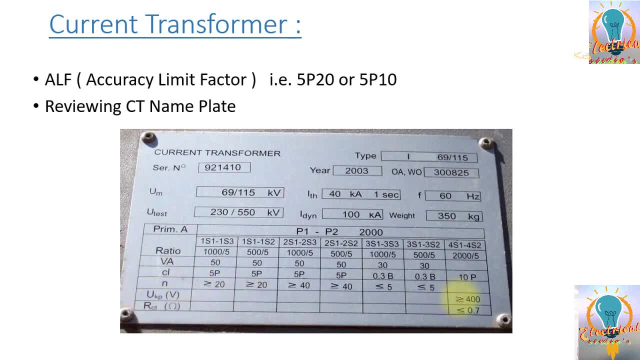 is normally used for the bus power protection, so they are also provided. knee point voltage for one core, which is for 10 P. it has a very highbrig rate which is usually promised to draw 50 perspective in this test, and this is basically the X-axis, the correct one. 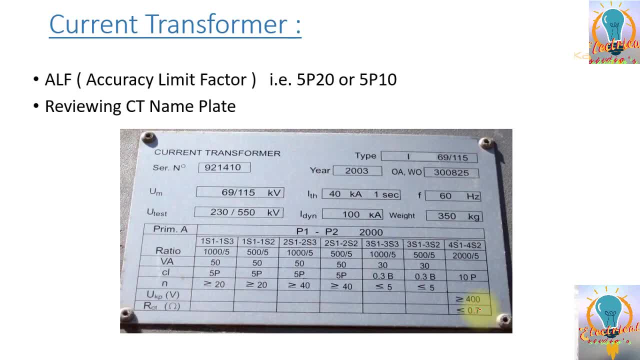 generally in this test you will be getting 100 ambient noise. then it is only 127. preโ�´ при. they have not mentioned the times. what does it mean by 5 p 10 or 5 p 20? it is called as accuracy limit factor and meaning of this is that at 10 for 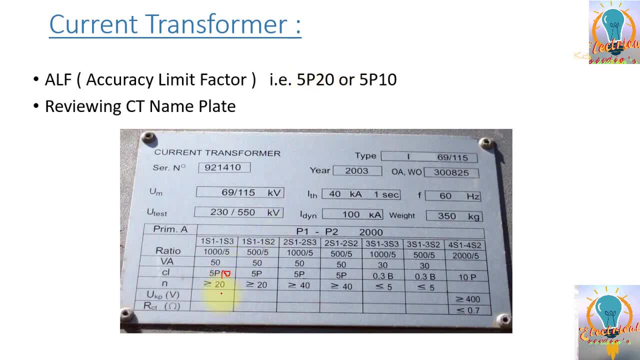 example, 5 to 20 means at 20 times fault current. if the CT ratio is 1000 for this core- and this is if I- if this core is 5 p 20 and 20 times 20 kilo ampere, fault current is there, then there will be a error in the reading will be 5%. so this: 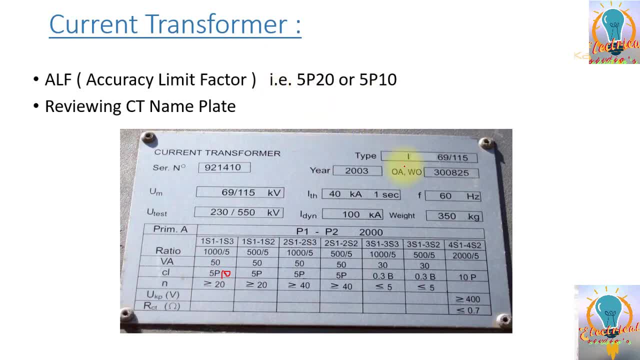 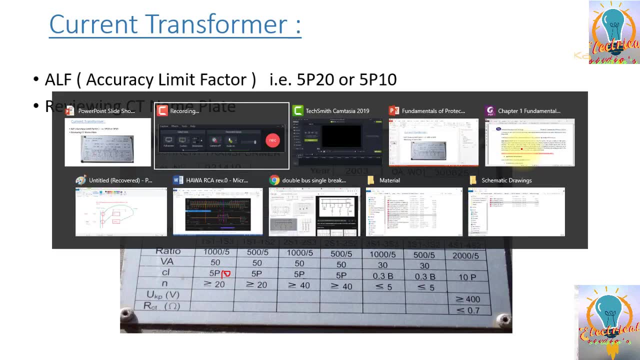 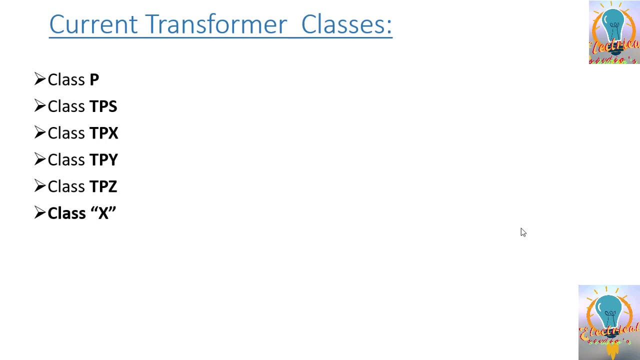 is how the accuracy limit factor is taking care. so this is just a little introduction about the CT nameplate. welcome friends. in this section we will go through the classes of different classes of CT, so the class of CT can be. you can see that in this section we will go through the classes of different classes of CT, so the class of CT can be. 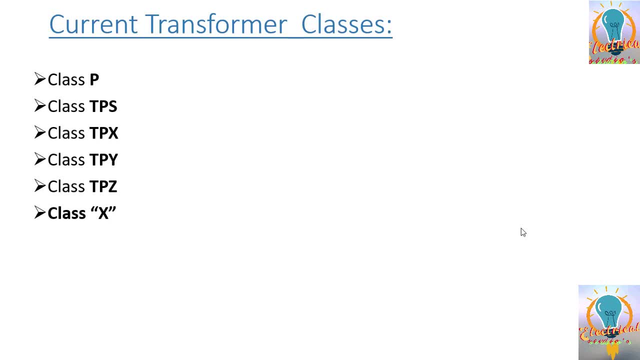 different classes of CT. so the class of CT can be of class P type, class TPS, class X, class T P X, class T P Y, class T P Z and class X. so for class P the current transformer accuracy limit is defined by composite error with steady-state symmetrical primary current. this specification is: 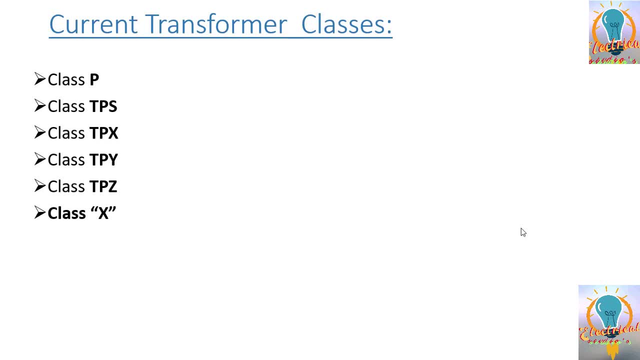 most useful when applying simple time delay protection. there is no limit is specified for the residual flux for class TPS. the IEC and RME cancel value values have oneirty of these type of specifications. the IEC specification for teachers are similar to class-c of class T. 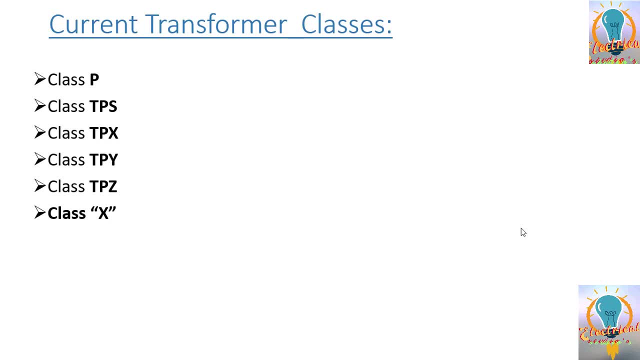 oh, and this very important enough also for OS Fußgänger at that time. it isn't the लेग and the ̄ğweitions that I do not want to commit issue as well as do process for classes of TPS. Class TPX accuracy is defined by peak instantaneous error during specified transient conditions. 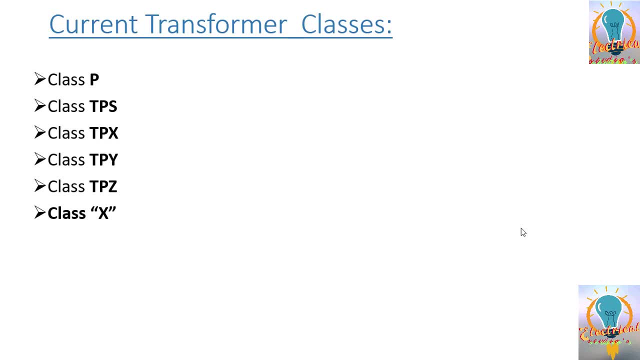 No limit is specified for remnant flux indicative of non-gapped CT cores. Class TPY has smaller air gap, hence its residual flux is very small. limit is 10%. Class TPZ has an air gap not necessarily suitable for high speed applications. 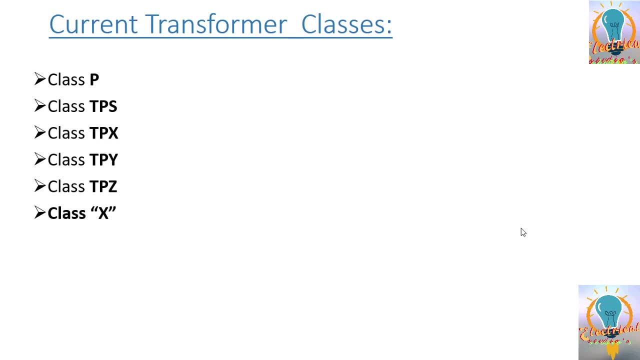 The larger air gap provides a very short secondary time constant with very short DC collapse time, making CT ideally suitable for breaker failure protections. Class X current transformers protection. current transformers specified in terms of complying with class X specification is generally applicable to unit systems like bus power protection. 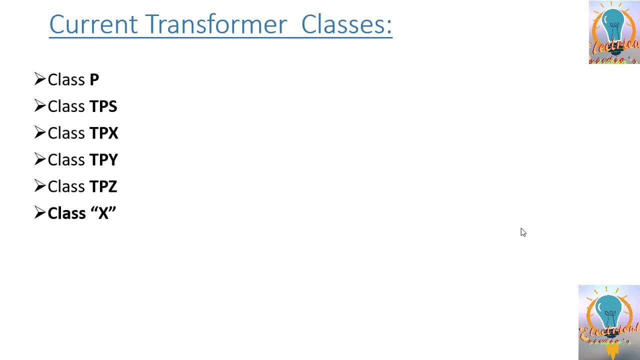 where balancing of output from each end of the protected plant is vital. So this is just some definitions of different classes. so this is just to give you an overview. there are different types of classes available and where we are using them. so just introduction. I hope you enjoy this lecture. thank you very much. 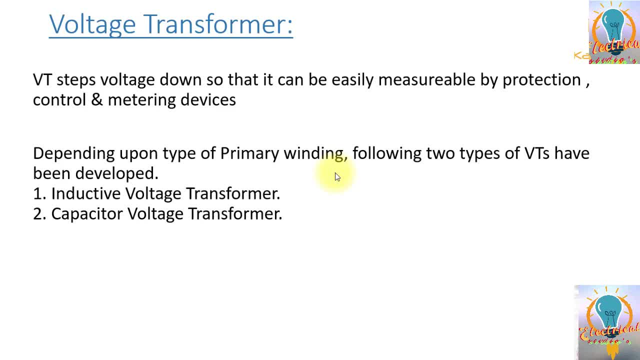 Hello and welcome friends. in this section we will study the voltage transformer first of all, why we need a voltage transformer. so you know that at the high voltage side the voltage are in kVs, like 132, 220 and 500 kVs. the voltage level is so high. so if you want 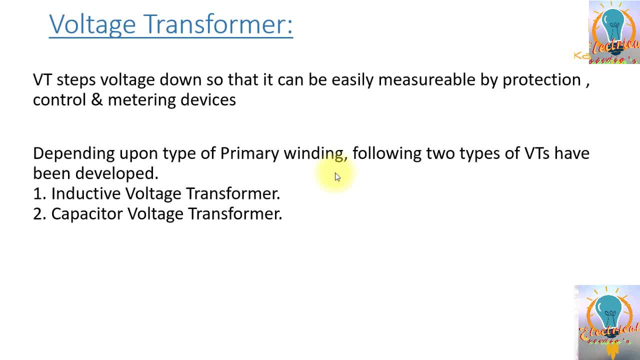 to make an instrument who can measure at the primary. you need to make the equipment size- voltmeter or whatever will be very big. you will need to have a very big insulation and difficult to carry and to move. So that's why the voltage transformer was designed. so the concept here is that voltage 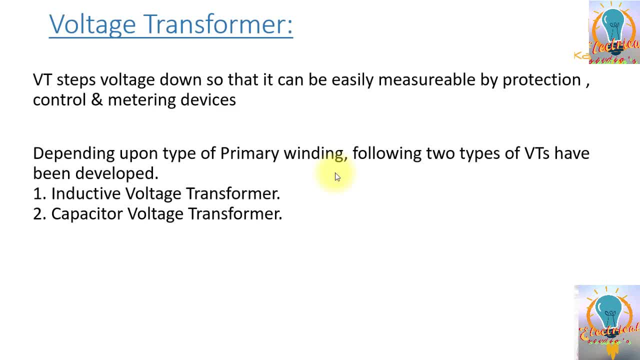 high voltage will be reduced to the low value and using a multiplying factor on the display or in the meter, which is called as a VT ratio, you can calculate back, calculate the primary currents. So there are two different types of VTs so far which are used in substation. one is inductive. 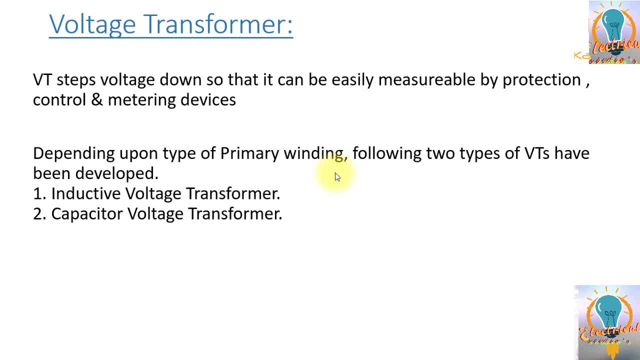 voltage. type: inductive voltage transformer. Other one is inductive voltage transformer. I will go through all the components and look at them one by one. Other one is a capacitive voltage transformer. So inductive voltage transformer is a normal transformer which is just stepping down the 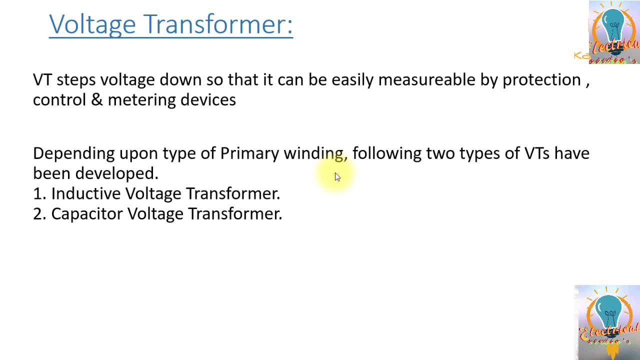 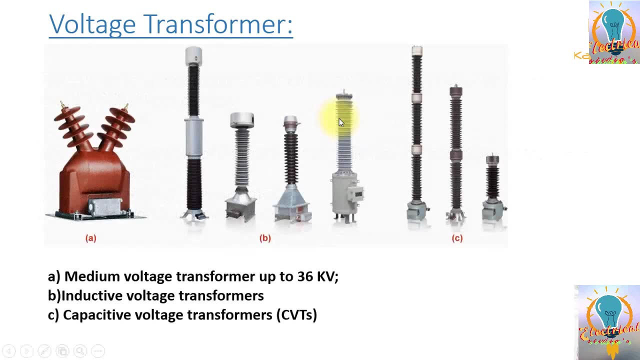 voltages. whereas capacitive voltage transformer is one capacitor, voltage divider is used and then at one capacitor at the end, the conventional transformer which is used so has to move one. so this is in this picture. you can see different, different types of transformer. this voltage transformer. 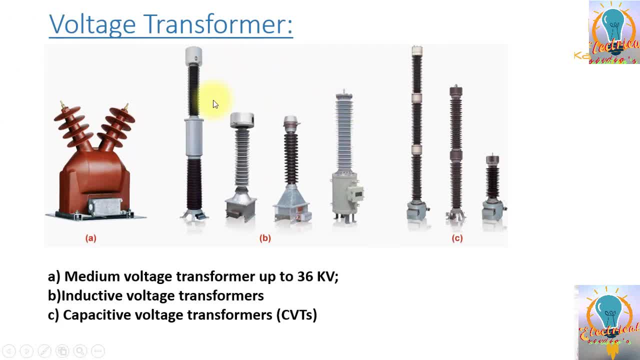 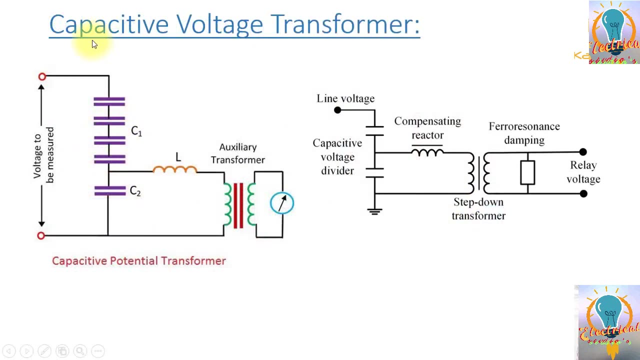 is normally used at low voltage level and this is inductive type of transformers are used up to 132 kV level normally and this is ccvt based capacitive voltage transformer. these are used at 220 and 500 kV voltage levels. so here you can see. this is example of capacitive voltage. 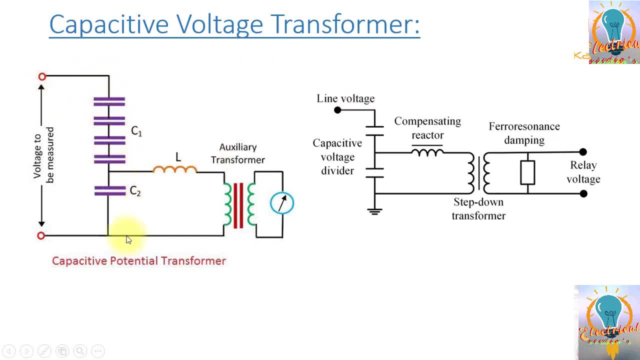 transformers. first of all, the voltage is divided across capacitors. at the end of the capacitor you can see the. basically a small transformer which is normally up to the rating of 1 to 5 kV, is used. because of capacitance. there will be change in angle, so this angle will be compensated. 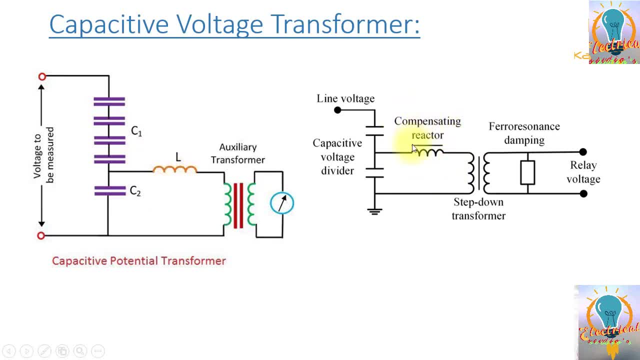 using this compensating reactors. so this is a tunable coil. so during when it is delivered from the factory, they are already tuning it. but with the passage of time, if some of the, for example, capacitors are fused, so you can also again adjust here the phase angle. 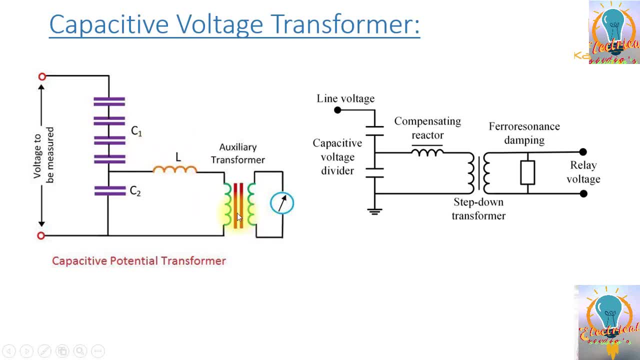 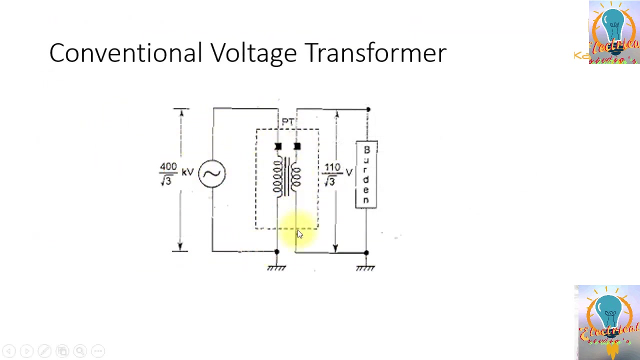 in the same way. here there is a transformer which is also called as emu electric magnetic unit. it is kind of commutational transformer and it has a rating of up to 5 kV. so at the secondary side you will get the ok normal secondary voltage of the transformer. this is we are showing a. 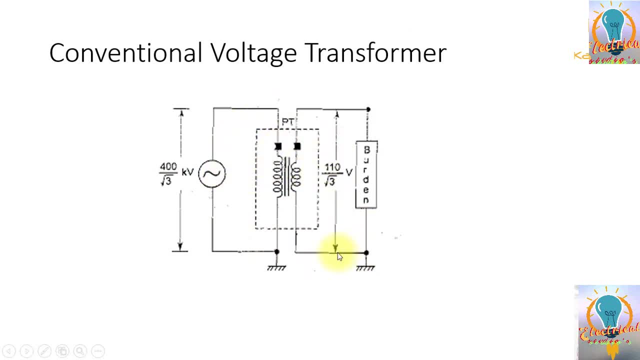 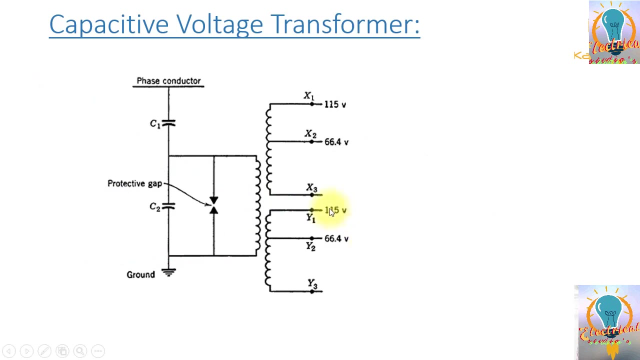 normal conventional transformer. this is normal PT and the relay is connected to the secondary of the PT. also we are calling it as a burden. so this is another presentation of the CVT. here they have installed a protective cap, so if the voltage increase beyond the limit, then this is just like a spark plug. 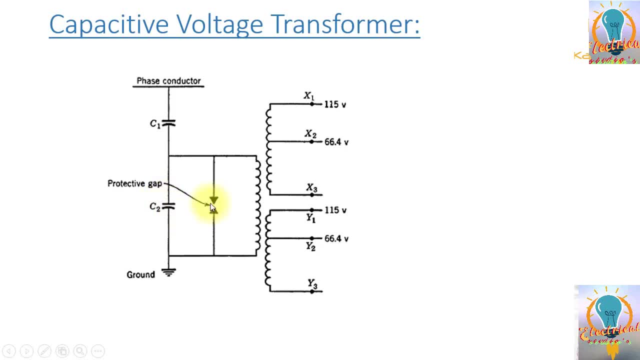 though. so this seat, this capacitor will be basically, and this capacitor and this EMU unit will be bypassed. you can see, this VT has one primary winding and it has a two primary secondary voltage and one primary winding and it has two primary secondary windings. this is multi core and multi ratio, so there are two taps at this step. 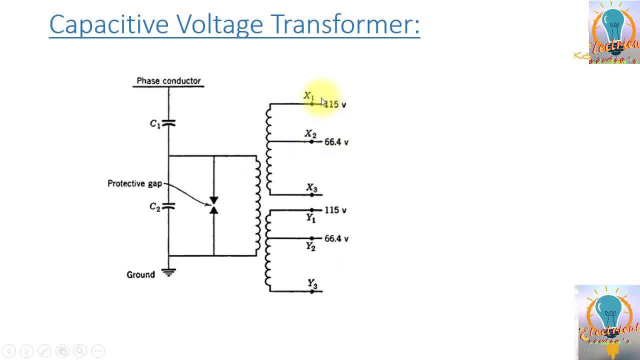 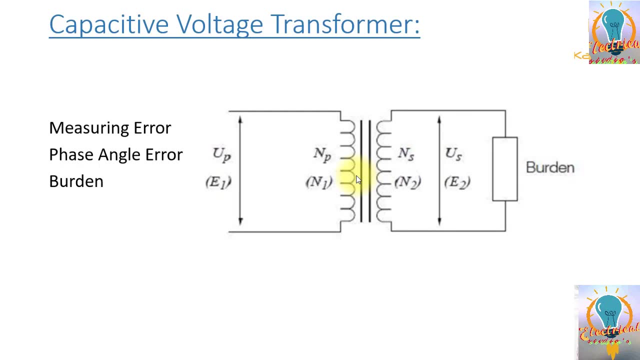 you will get the voltage 66.4 volts and at this step you will get 115 volts. so in the voltage transformer, just like current transformer, there are two type of errors: one is measurement error and another one is phase angle errors. and the load which is connected to the secondary side of the VT is called as a. 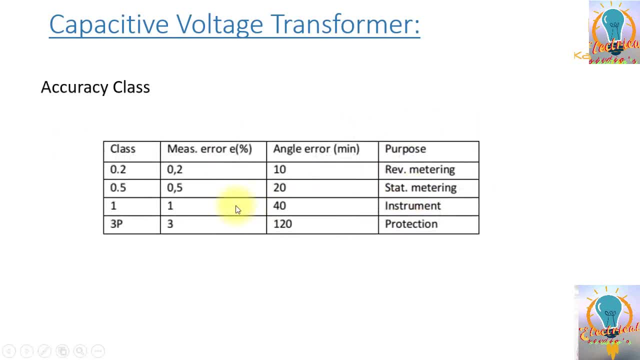 burden. so here you can see the accuracy class, different accuracy class and where they are used. for example, 0.2 accuracy class of the VT and basically is used on revenue metering and 0.5 accuracy class is used on on normal metering static. 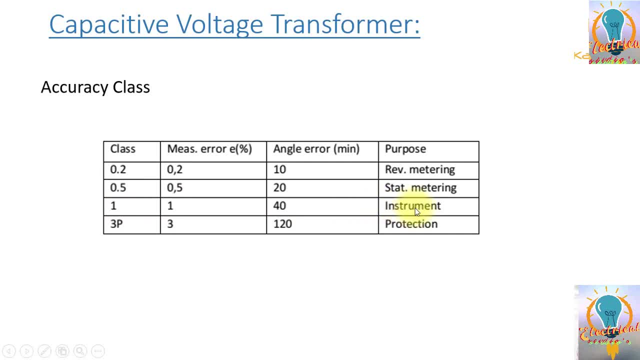 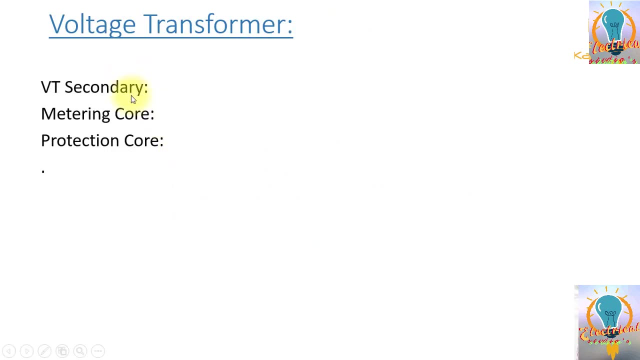 metering. class 1 is used on instrumentation and class 3p means 30% of error is used for protection release. so voltage transformers have in the secondary side. they have two different type of course. one is meeting core when one is protection core. meeting core is: 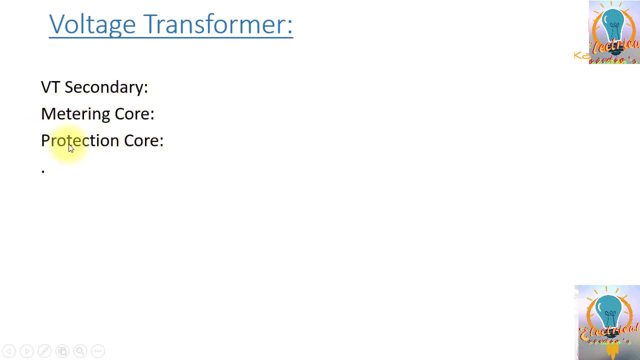 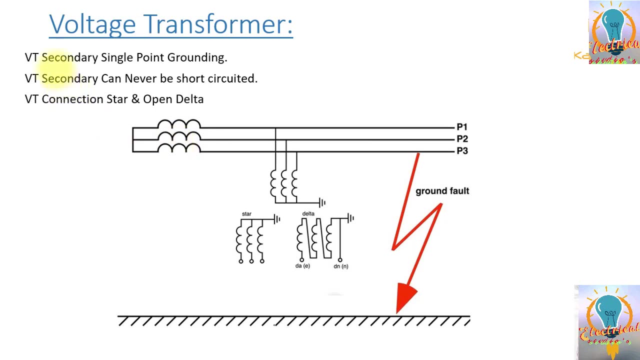 more accurate and error is less where the protection code it has more error. so here you can see the world VT. secondary single point grounding- we can never be short-circuited with this connection- star and open delta. so these three topics we will cover in this section. so, like CT, VT also has to be. 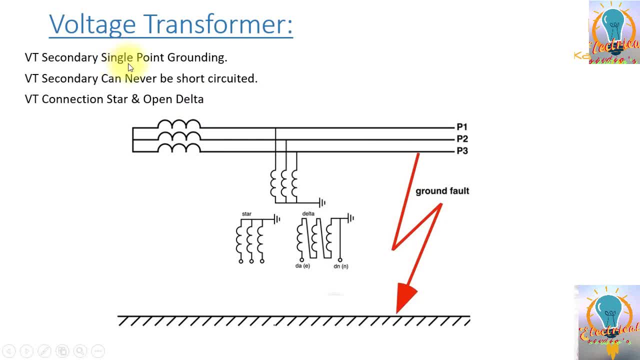 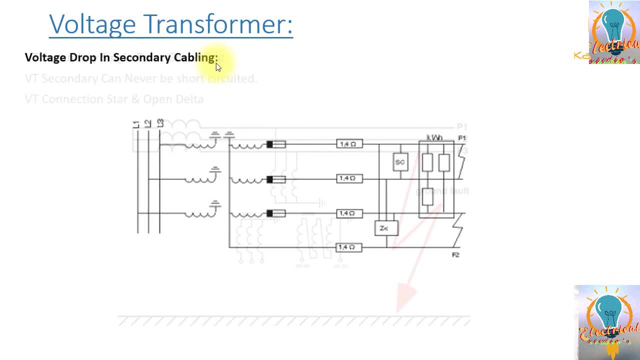 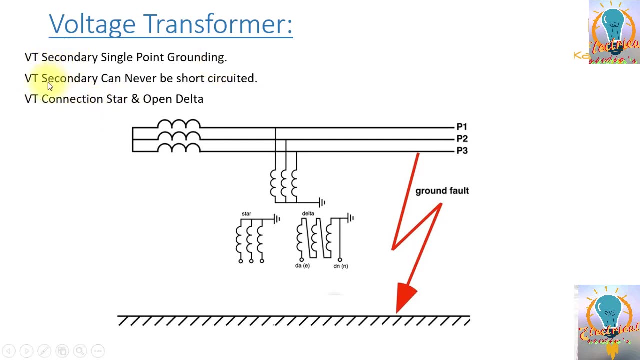 grounded at single point. multiple point grounding is not allowed in the VT. if the VT is not grounded then there is a no solid ground reference and the phasor will be in rotation. so you will not able to get all three phase two ground voltages correctly. 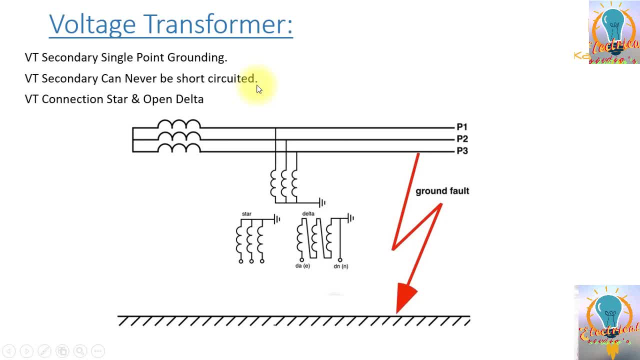 the VTE secondary can never be short circuited. we have in previous section. we have seen that CTE can never be open circuited. the voltage transformer is a reverse. it should never be short circuited. normally our MCB is installed to detect any short circuit. if there is a short circuit, MCB will trip. 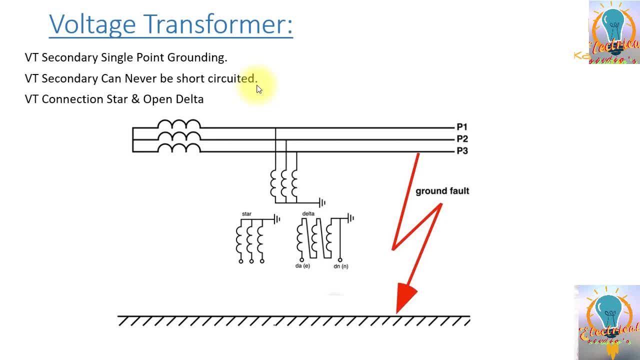 and interrupt the fault. current number three is now VTE. connection can be done in star and in the open Delta connection. so here you can see. this is basically the CAVG primary winding. this is the second of winding. this finding is connected with star in. this finding is connected in open Delta connection. so 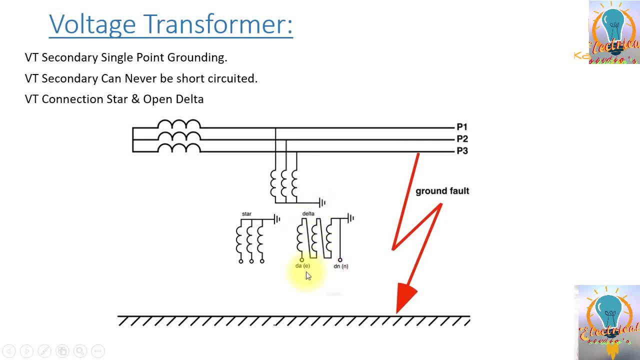 it's a Delta, but it's open. so what will happen? if there is a balanced condition, then all three phases will be same and then open Delta voltage, which is basically 3 V naught, will equal to zero. but if once expression is carried on the other side, if this stays there for 1 second, 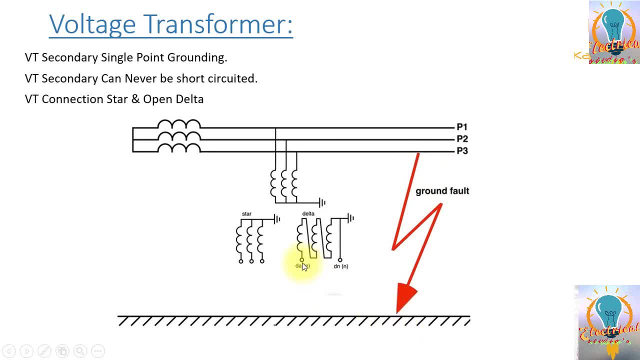 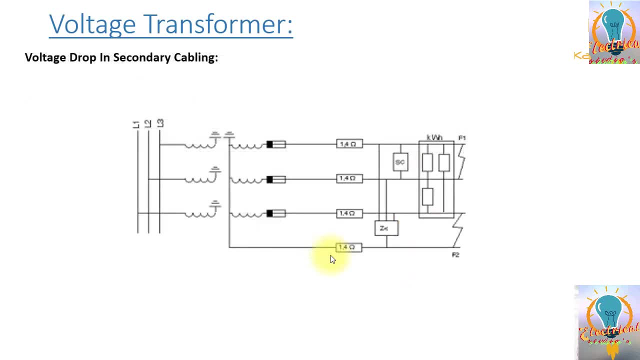 phase is grounded, it means there is unbalance. now the voltage will appear across this open Delta. so when we are designing the basically VT circuit in the substation we need to consider the voltage drop in the VT circuit. it should be within the permissible limit, otherwise it will use and a 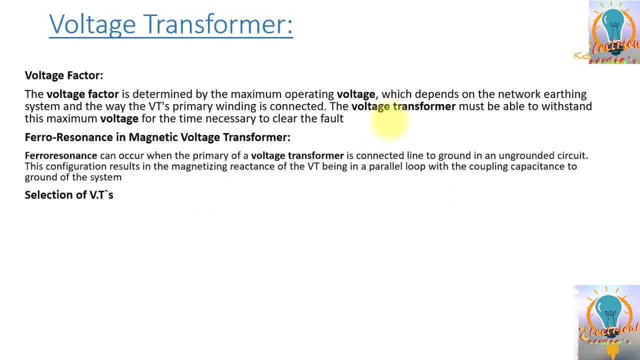 significant error in the relay calculations. so, voltage factor: what is the voltage factor? voltage factor is determined by the maximum operating voltage, which depend on the network earthing system and the way the VTS primary windings is connected. the voltage transformer must be able to withstand this maximum voltage for the time necessary to clear the fault. so 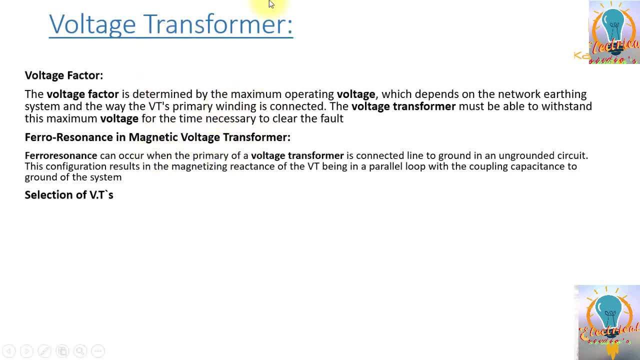 voltage transformer is maximum operating voltage. a transformer can bear voltage factor. so if the rating is, for example, of a VT rated for 100 kV and the voltage factor is 1.5, it means that it can bear the maximum voltage 150 kV for a given time. so another topic is: 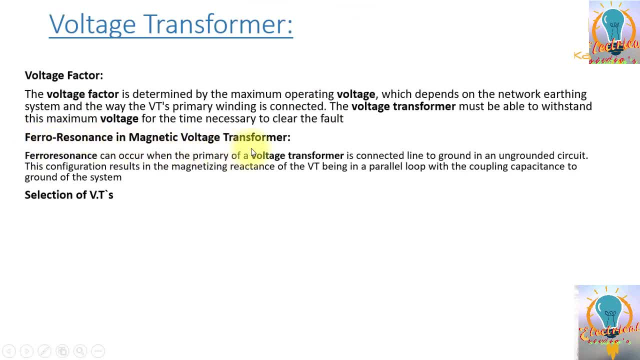 Faro resonance in magnetic voltage transformer. Faro resonance can occur when the primary of voltage transformer is connected line to ground and an ungrounded circuit. this configuration results in magnetizing reactance of the VT being in parallel loop with the coupling capacitor to ground and the system. so this is just an basic definition. you don't want to go. 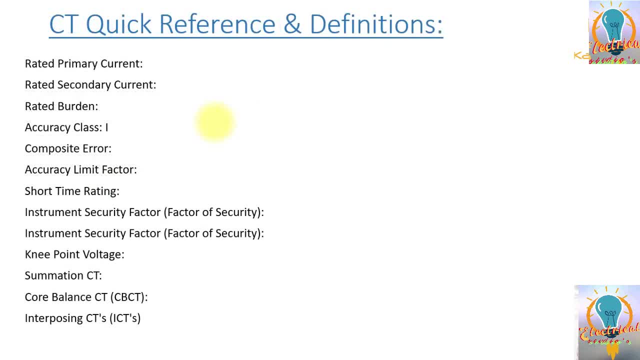 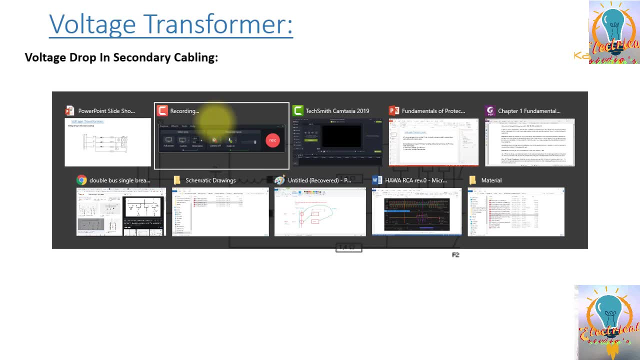 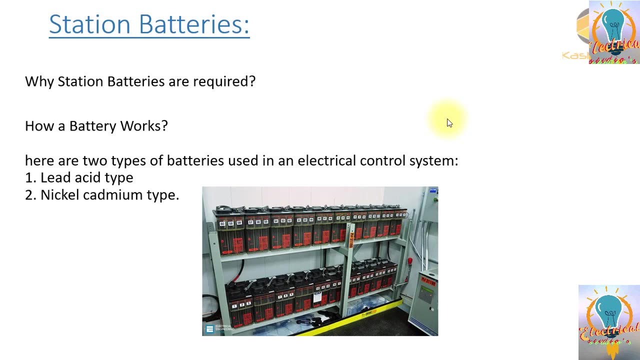 here in detail to explain this. so this is about the voltage transformer. so I hope you enjoy this lecture. uh hi, friends, we will start our new topic and that is related to some introduction about the station batteries. so why we need station batteries at the substation? uh, basically, the, you know the. 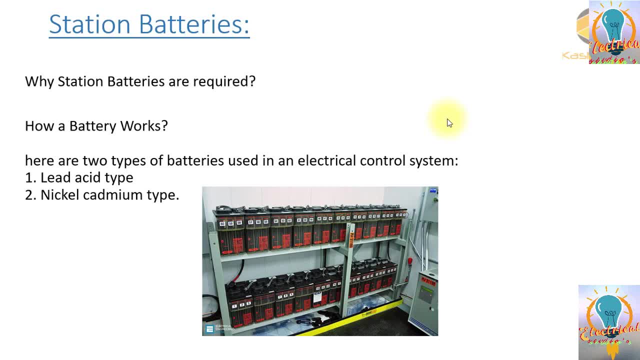 AC power is fluctuating and there are the cases when the AC power is lost, so and they also, there is no backup for the AC power. so, uh, or taking some of these things in account and considering these things, where battery banks are designed and how battery banks are basically working. first of all, AC supply is connected to a DC. 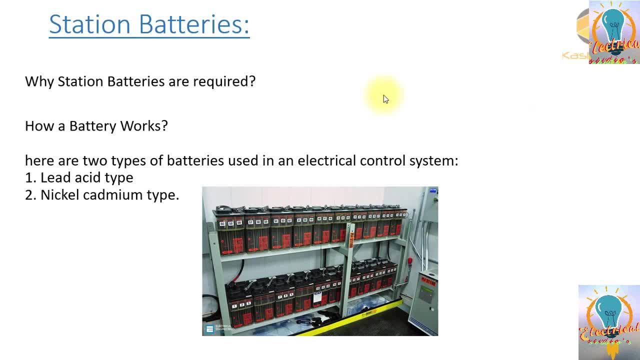 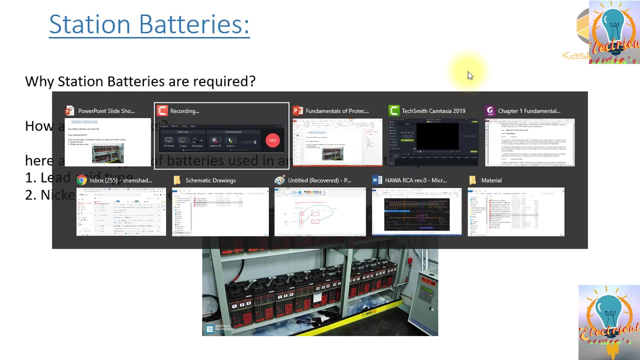 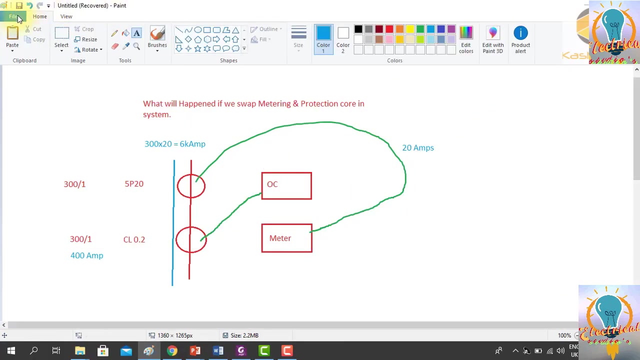 AC supply into the DC supply and one end of the charger is connected to the uh, basically the battery batteries and it's charging the batteries, and other end is connected to the, So it is supplying the dc, db and the batteries in parallel, so we can have 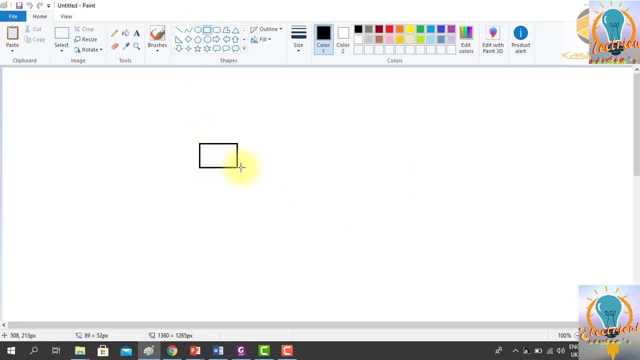 So we can imagine this: that, for example, this is the charger and this is the AC supply. three phase AC supply is connected here, okay, and output of the charger. one output is connected to the batteries. for example, these are the batteries and this one is the dc db. 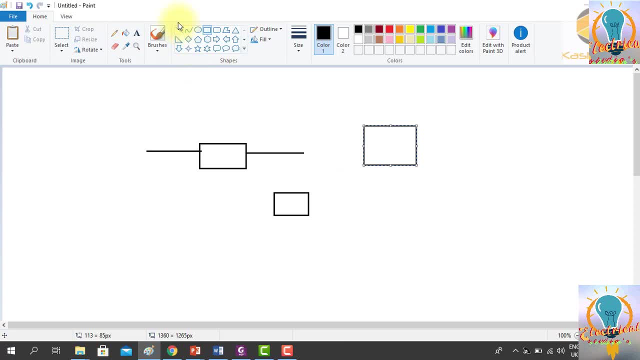 So this is, for example, the battery bank and this is the dc db and normally at any substation is provided by two battery banks. So let me first write: This is charger and it is converting AC supply. here we have three phase AC supply in the 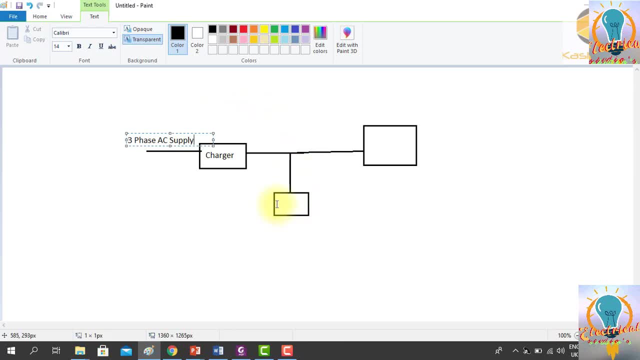 substation, So, or any power plant, and this one is basically the battery bank. This one, for example, is the dc distribution board. we can say one. So this is the normal configuration of substation, and here then this is taking supplies to. 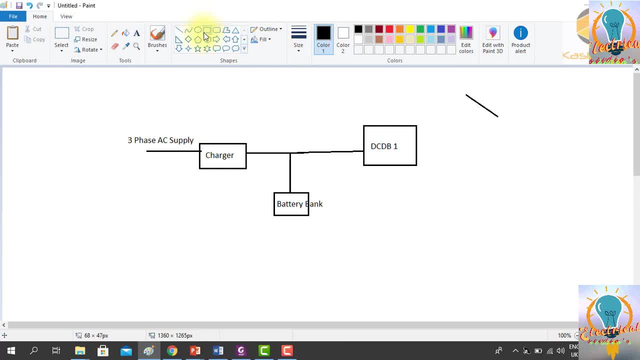 further protection panels, protection panels, control panels, Then switchyard all different places sticking giving the supply, so it is like a protection panel, relay panel, RP, control panel, CP, and then switch gear like cycle breaker, isolator etc. So then further supply is distributed to all of these. 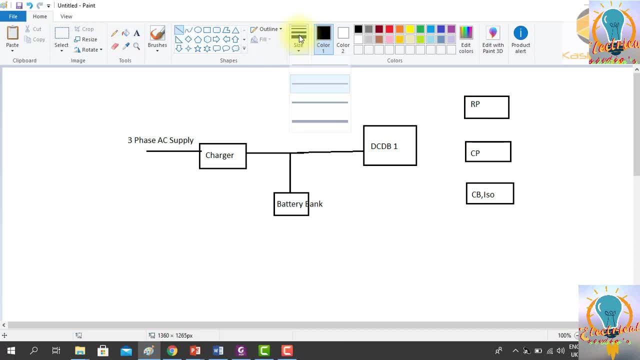 So this is the dc db Through dc db, Through dc db. So here it is getting supply and here, basically, they have the diodes, dropping diodes, So wire battery, for example, here the if the system voltage requirement is 220 volts. system voltage requirement is normally, for example, 220 volts. at the substations the battery will charge at, not at 220 volts. at float also it will charge at 242 volts, for example. charging will be at the higher voltages. so the generator. at the terminal output of the generator, these are called as: 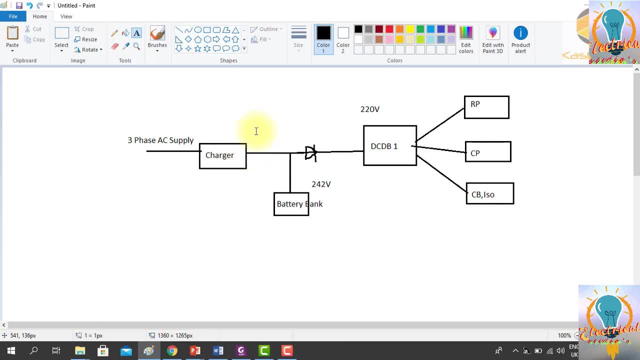 terminal voltage. terminal voltage will be round about in the float mode will be round about. you can say 242 volts. so this will be directly connected to the battery bank and after that there will be a number of dropping diodes. so these diodes will drop the voltage and will bring it to 220 volts. 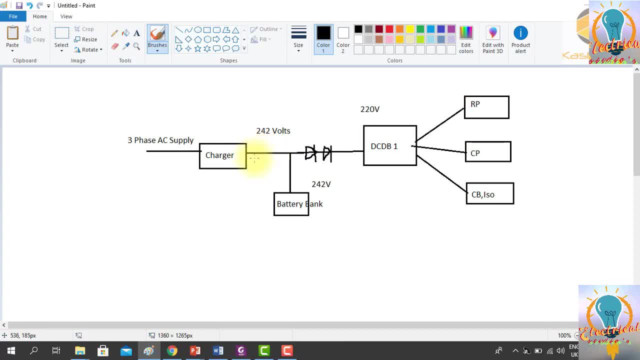 so there is a term of feminine voltage will be. it will be here and there is a voltage after this dropping diode which will be the distribution vote. the purpose of dropping diode here is to reduce the voltage so that it can be used at the distribution level. so normally in the substation there are two banks of. 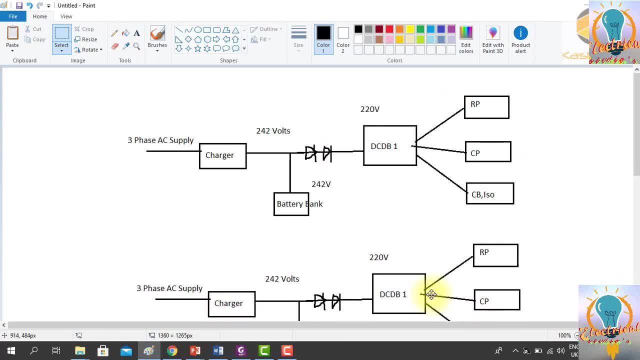 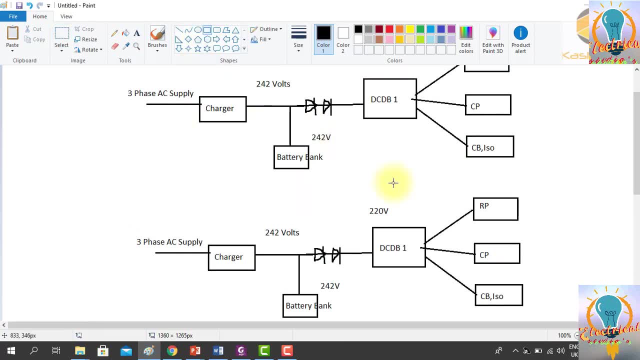 batteries. there is no one bank, there are two banks of batteries and these are connected through a coupler. so this is the Norman configuration, this is a bus coupler, for example. so now if, for example, the AC supply is fail, here, the AC supply, if this is Applies, fail. so what will? 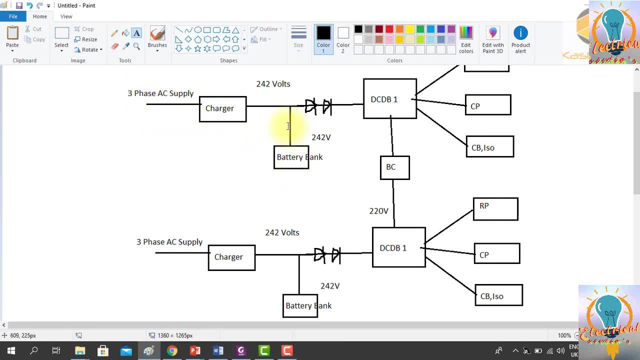 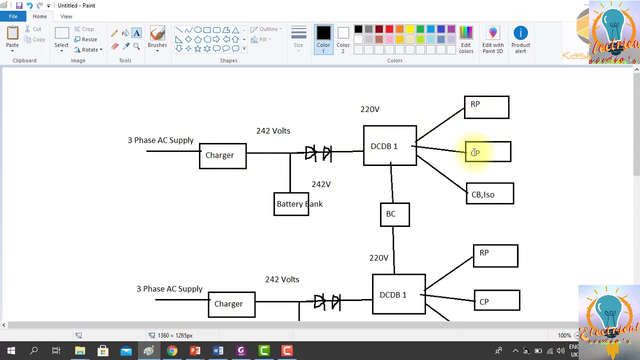 happen, Then this battery will be supplying the voltage to DC DB directly, So these dropping diodes will be bypassed and the battery will be supplying the voltage to the DC DB directly and the supply to the relay panel, control panel and the CV will. 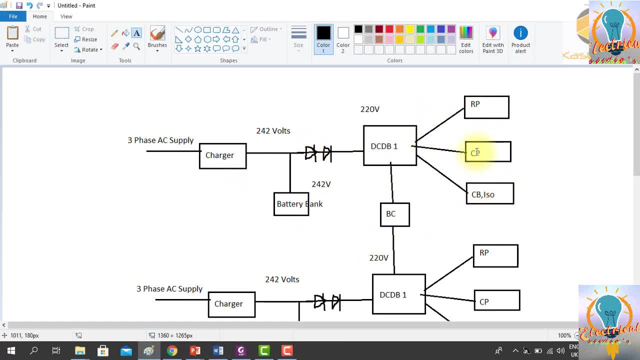 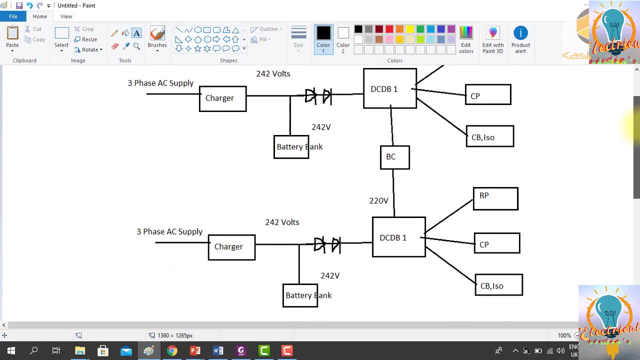 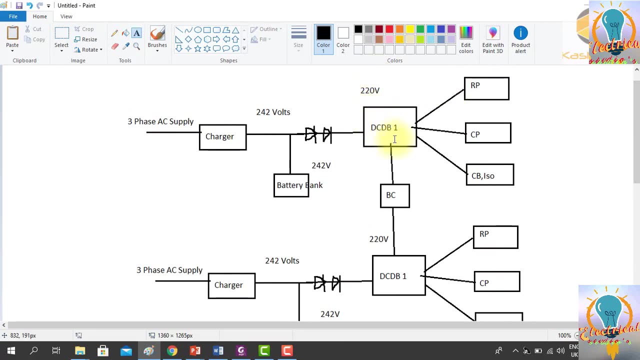 not be disturbed. So this is the advantage of DC, DB and the battery banks. So normally they are giving two chargers, set of two chargers and two battery banks, and this is the reason is behind. is that, for example, if the one complete set is failed, 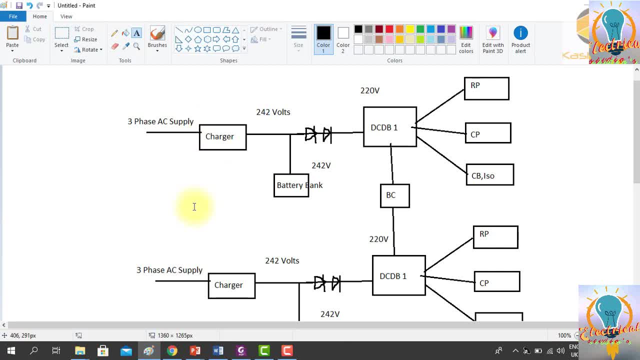 If, for example, this battery bank charger there is a fault and this complete set is shut down, So there will be no power available at DC DB 1. So the bus coupler: It can automatically close in that case if it experience that there is no supply at DC. 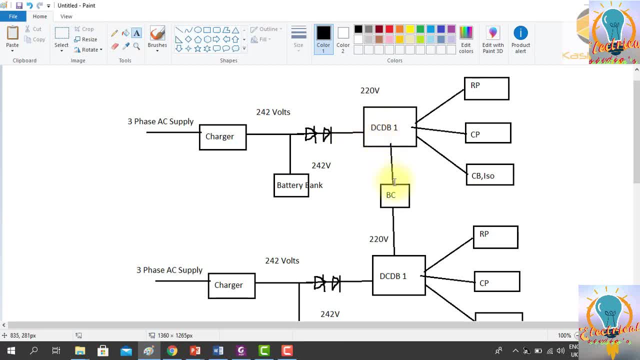 DB incomer side, Then this coupler will close and it will give supply from this charger to DC DB 1.. So charger 2, this is the charger 1, for example, and this is the charger 2.. Charger 1 will give if the charger 1 is shut off. 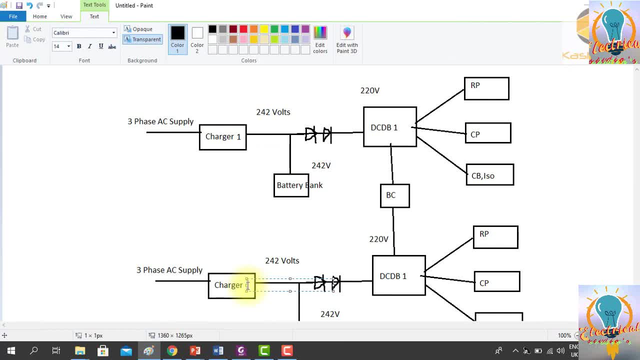 And also the battery bank. So this is the charger 1.. This is the charger 2.. So this is the charger 1.. So this is the charger 1.. If the battery bank is shut off, then charger 1 will be switch off and the charger 2 will. 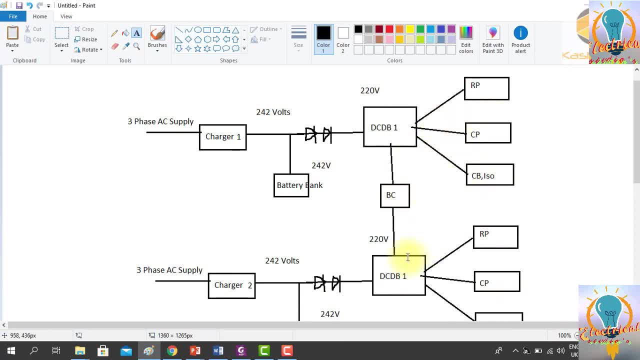 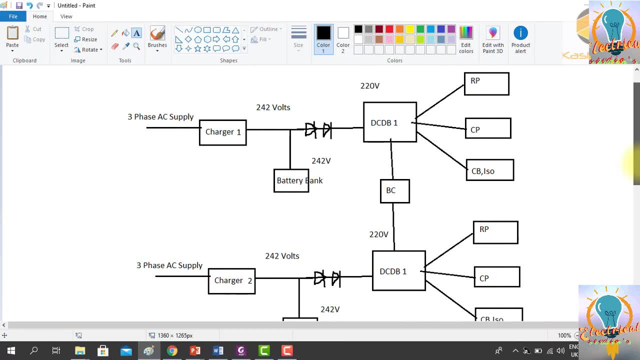 give supply to the all protection systems. So this is the purpose of the protection batteries in the substation: to provide backup power, to provide stable power. Charger is doing converting AC to DC and it's providing smooth DC supply, regulated DC supply to all our control and protection panels. 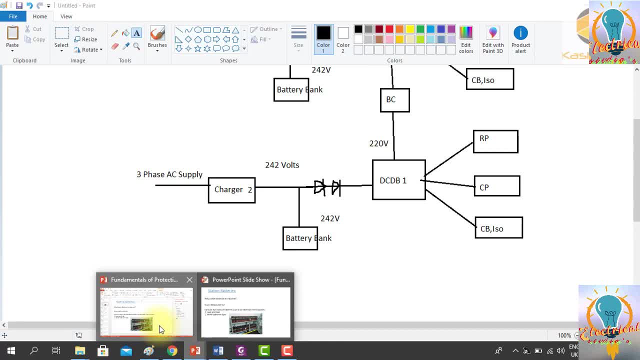 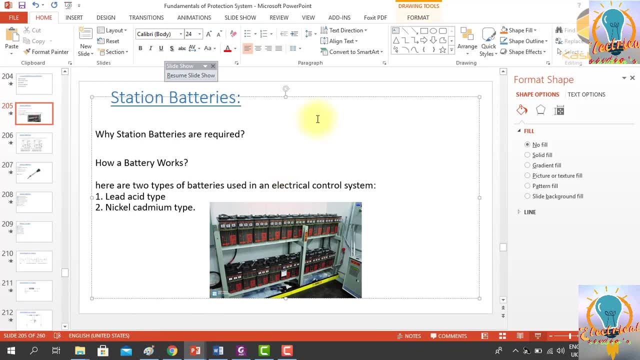 So this was little brief about the protection systems that we, about the, about the battery system that we are using in for the protecting our equipments and operation and control. So how battery works. This is very simple: Battery is basically converting electrical, first of all electrical energy into chemical. 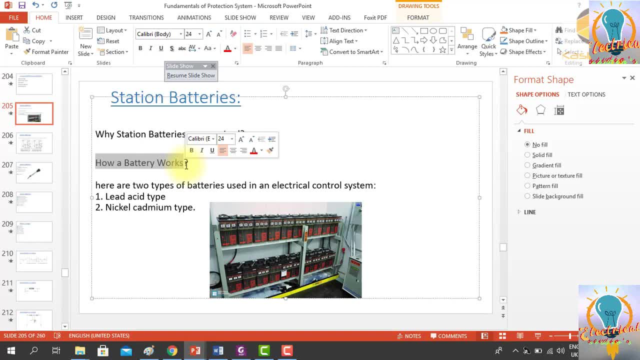 energy during the charging process and when load is connected to AC, To it, it is start discharging and then the chemical energy is converting back into the electrical energy. So the process is used here is electrolysis. There are two different types of batteries which are used in the substation. 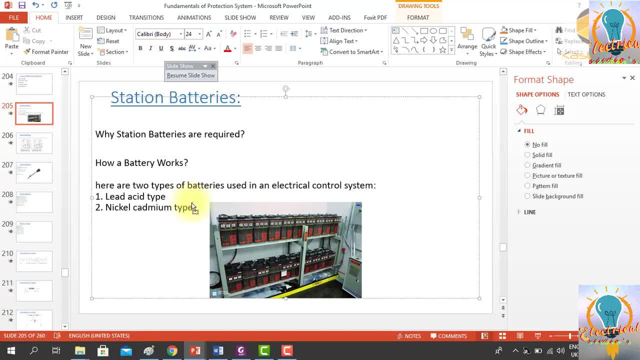 One is lead acid battery and another one is basically the nickel cadmium battery. So these are the two different batteries that are used. So we are using lead acid battery less than the nickel cadmium battery, And when we plug the dead battery in here, the Look authority works like well this. 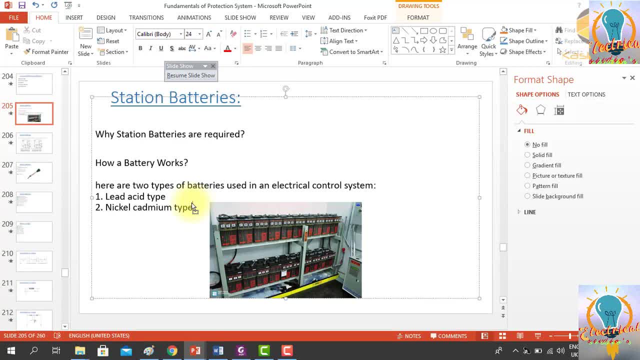 is a arrangement of an acid battery and a lead acid battery to be provided directly to the electrical board, So the current voltage fromNow coming out Right water as the electrolyte gets diluted due to charging and discharging. the batteries also discharge hydrogen during the cycle and it is very necessary to restrict this discharge to 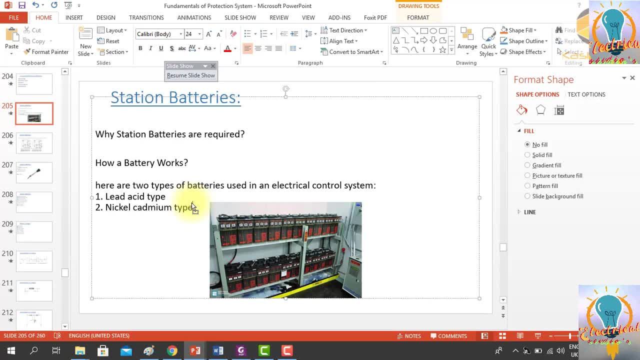 less than four percent by volume to air to avoid surrounding becoming hazardous. the higher discharge of s2 is in lead acid cell has resulted in the manufacture of sealed, maintenance free or wall regulated acid. we are la batteries here. the s2 discharge is restricted to below the hazardous. 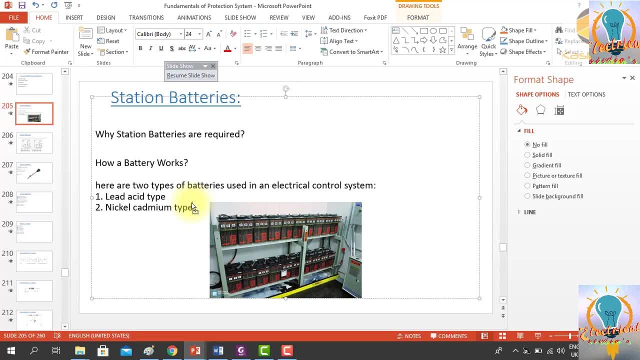 limit. hence, for conventional switchgear protection application, sealed nickel cadmium batteries are not required as such. the sealed nickel cadmium cells are only used for small battery cells using more modern electronic gadgets. the rechargeable lead acid cells normally used in such gear relay applications are generally of the plant type and have an 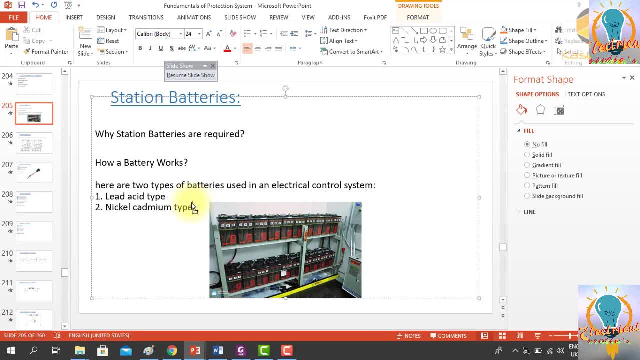 electrical voltage of two volts. the cell contains pure lead positive plate and lead oxide negative plate and electrolyte of dilute sulfuric acid. the nickel cadmium cell has electrical voltage of 1.2 volts, containing nickel compound as a positive and cadmium compound as negative. it's with potassium hydrogen solution as electrolyte. so there are some. 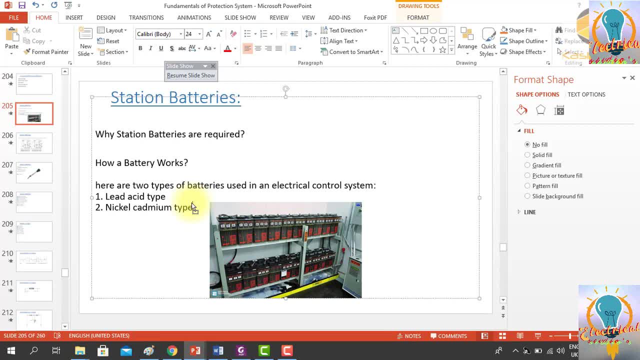 advantages and disadvantages of this, this type of batteries that we can discuss. the following are the advantages and disadvantages of nickel cadmium batteries or lead acid batteries. and the nickel cadmium batteries have better mechanical strength, they are easier to maintain, they have a long life space and weight is. 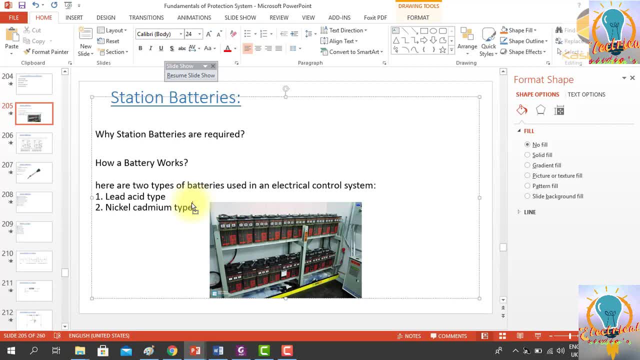 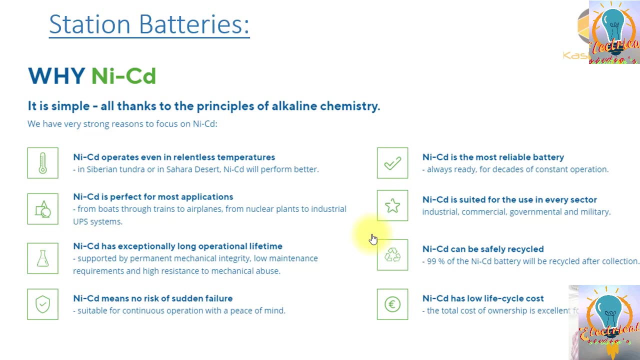 low. they have low as to discharge and no spillover issues. the disadvantage of nickel cadmium is lower cell voltages. they are more expensive and higher current consumption for charging not recommended at higher ambient temperatures. so these are some advantages and disadvantages of the battery. welcome friends. now we will discuss some advantages of nickel cadmium batteries. so 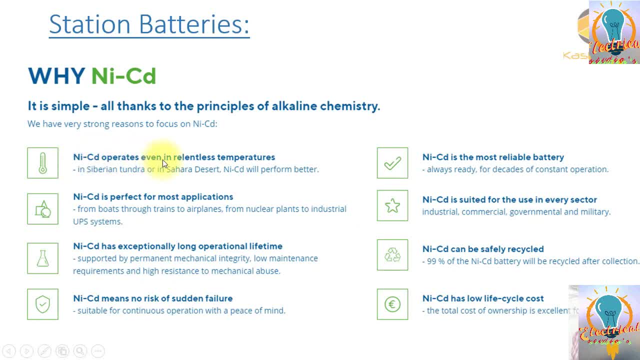 advantage of nickel cadmium battery that it is operates. it can operate on higher temperature. so whereas lead-acid batteries, when the temperature increases, their life expectancy is also decreased, but nickel cadmium batteries are more tough and more strong to face the temperature. so if if you are installing a battery in an area where temperature is at 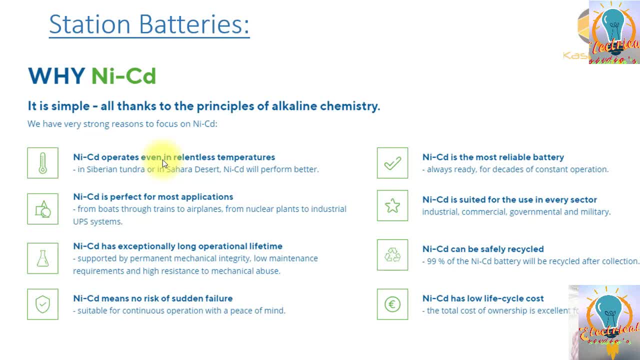 extreme so you have to come. it's better option to use nickel cadmium. so nickel cadmium is perfect for most applications. so, for example, you can install it in boats, aeroplanes, nuclear power plants, ups, so it's always suitable. nickel cadmium has exceptionally long. 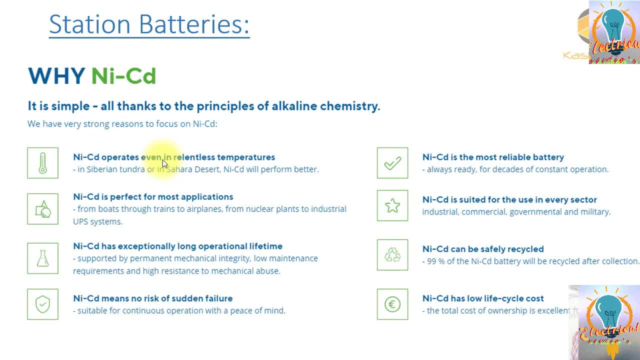 operational lifetime, so the lifetime of the nickel cadmium battery is very long. it's basically a low maintenance and it's mechanically strong battery. nickel cadmium batteries are very good in terms of battery life, so nickel cadmium means no risk of sudden failure, so suitable for continuous operation. 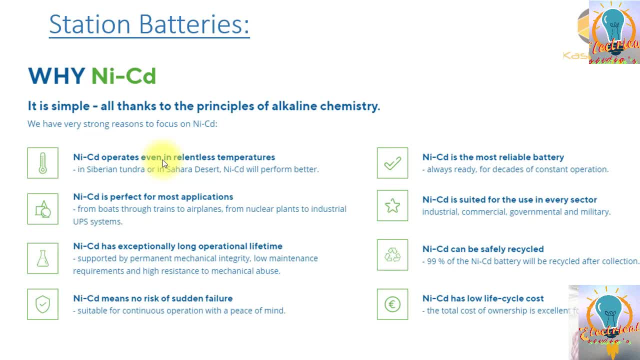 with peace of mind. so as compared to lead-acid, nickel cadmium is. there is no risk of suddenly some cells are failed. so this is nickel cadmium is better in this case. nickel cadmium is most reliable battery, so nickel cadmium is considered as most reliable battery in in the in the field of: 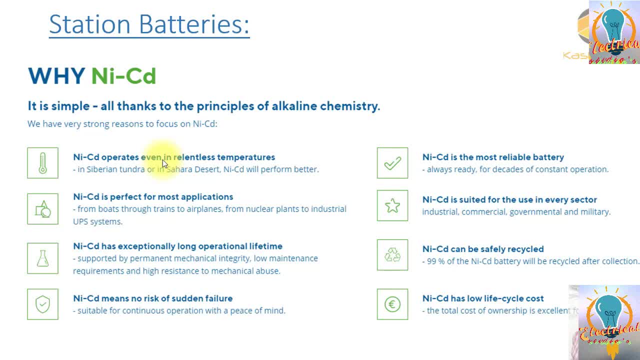 power plants and substations use in every sector. nickel cadmium can safely be recycled, so recycling is also possible. 99% of nickel cadmium batteries will be recycled after collection. nickel cadmium has low life cycle cost, so initial cost of nickel cadmium is high. but if you divide the cost of nickel cadmium with the 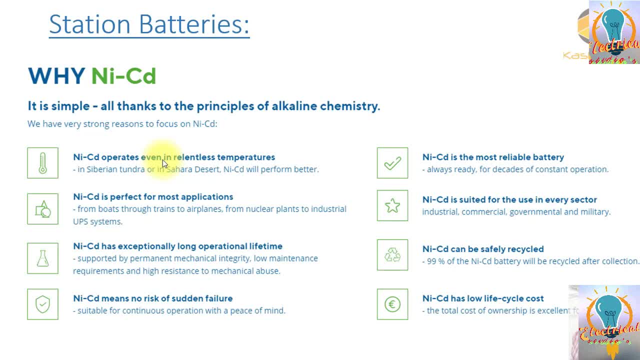 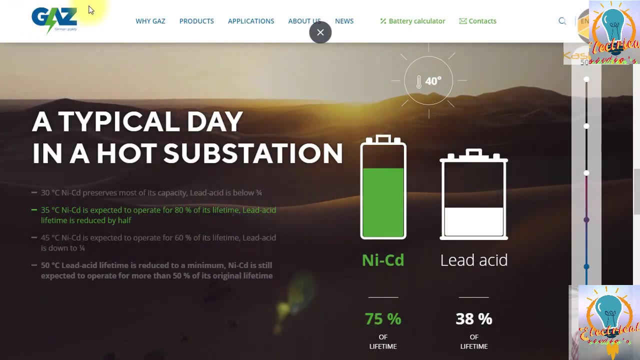 total number of year plus less maintenance cost. the total cost is called as life cycle cost at the end of the year and the total cost is called as life cycle cost. and the total cost is called as life cycle cost. so this is basically a gas company and the gas. the gas is basically the German company, which. 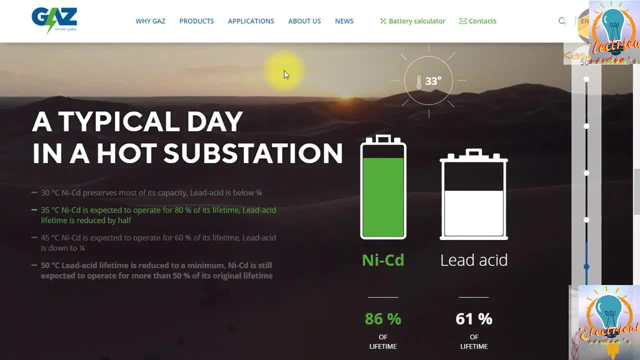 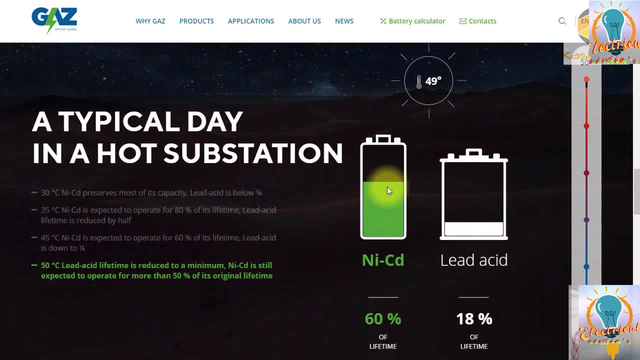 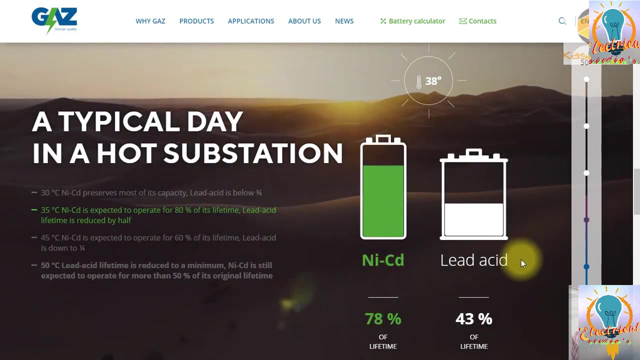 manufacturing the nickel cadmium batteries. so here they have shown on their website that how nickel cadmium life time is reduced with increasing temperature. so here is on the left side is basically the nickel cadmium battery. on the right side you will see the lead acid battery. so as the 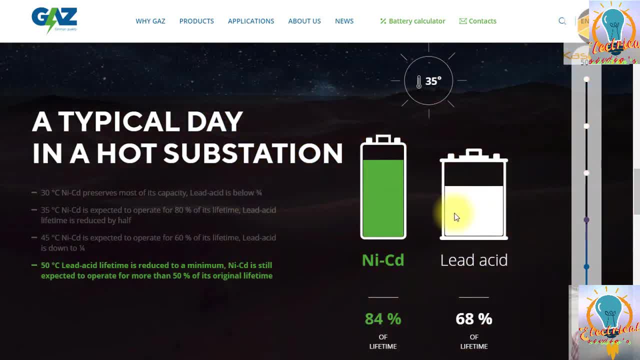 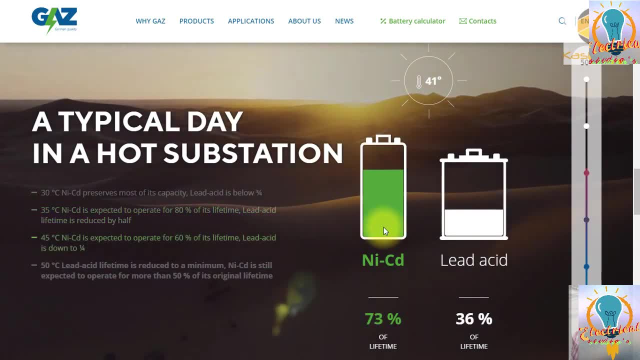 temperature is increasing the life of nickel, cadmium and lead acid both are decreasing, but the lead acid life is decreasing very fast as the temperature increased. so this is very nice presentation and it's giving a good comparison. so I hope now this- this is this presentation- is really helpful for you to 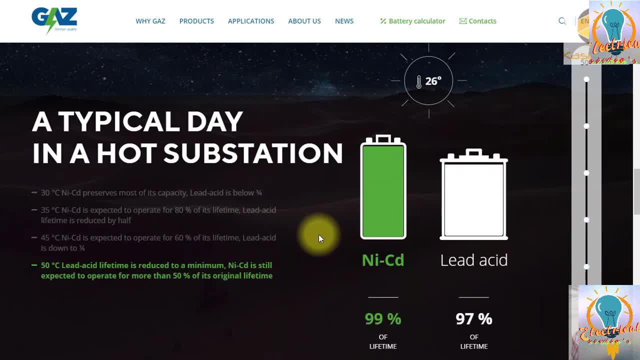 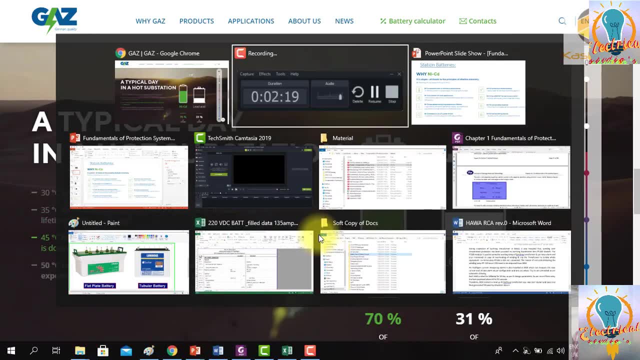 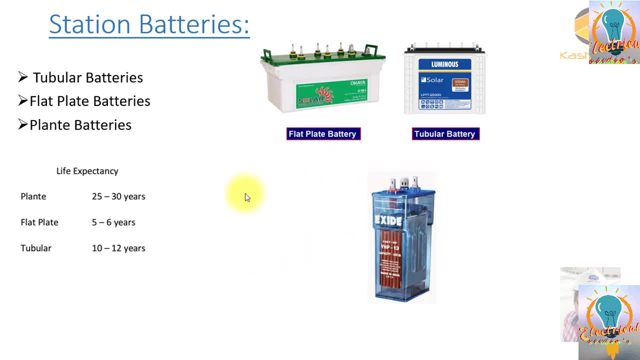 understand the benefits of nickel cadmium in the substation. so now more and more nickel cadmium batteries you will see in the substation in future. thank you very much. hey, friends, the batteries can be classified into three different types, based on the plates which are used in the batteries, though. 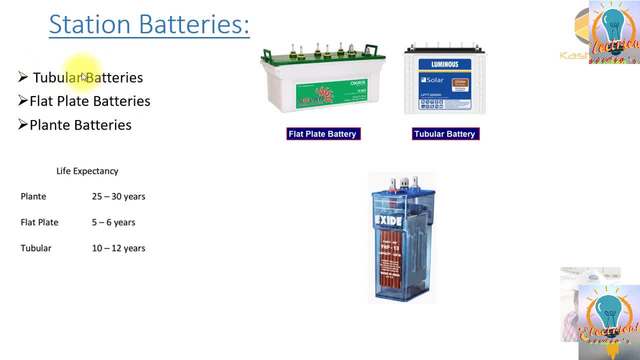 three types could be: tabular batteries: the. in this one, the type, the battery plates are in the form of cubes. then it comes to flat plate batteries. the flat plate batteries are where the basically anode and collect cathodes are in the form of basically plates and in which you 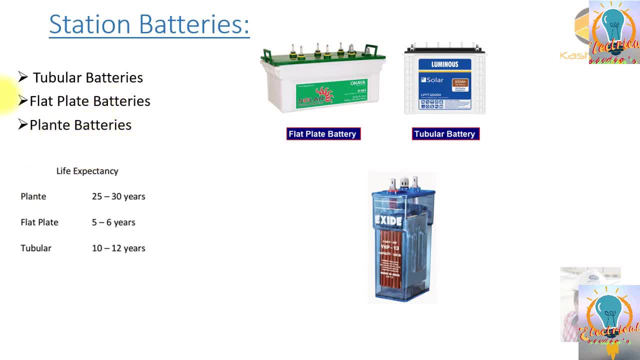 will see the square boxes. so and then plant a batteries and these are planted. batteries are basically the initial, very initial form of batteries, in which cathode and electrodes are basically rods, electrical rods, and in between the insulation was used to be placed. so the life expectancy of these batteries planted. 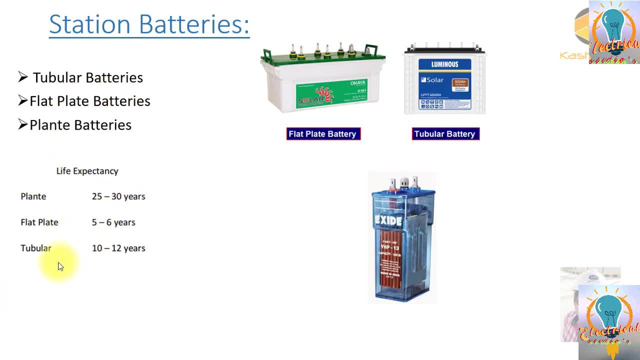 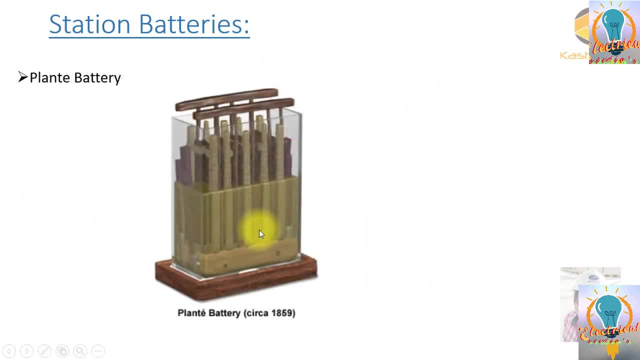 batteries 25 to 30 years, flat plate is 5 to 6 years and tubular is 10 to 12 years. so this is basically the example of plant a battery and this is one of the very old batteries that were invented. and this is the picture of battery that was invented in 1859. this battery was invented by a 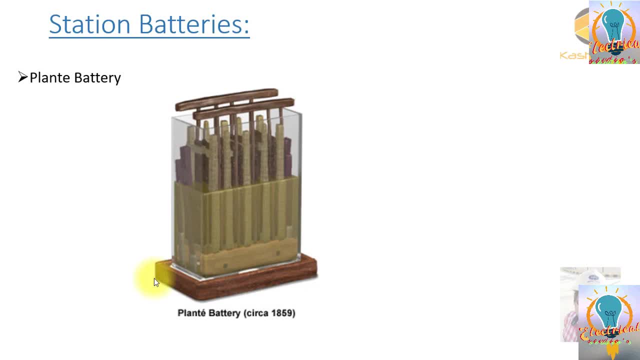 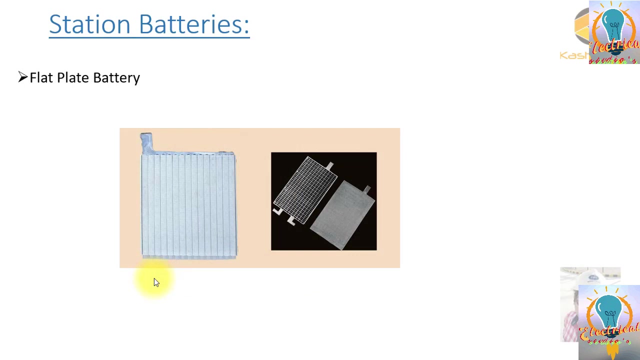 scientist named gaston planted, and this is one of first battery, one of its kind, and then mention here was 1959, so this is one of the very initial batteries. then it comes to flat plate batteries. you can see the battery cathode and cannot disa. 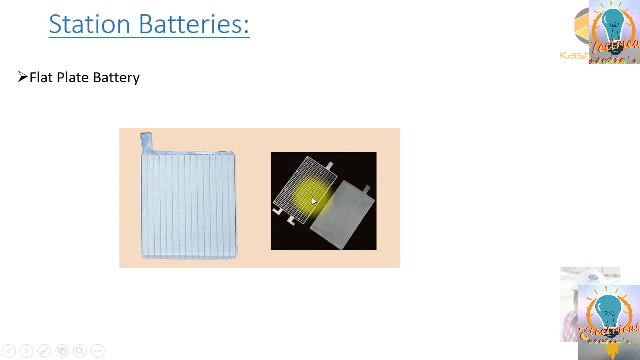 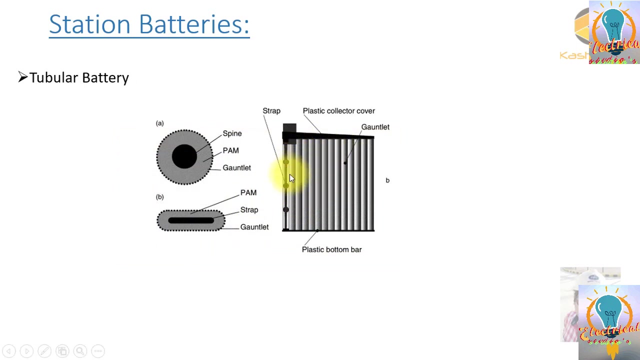 anode and cathode structure. it is fine in the point, in the form of flat plates, and you will find these batteries mostly now in the cars- electric cars- and this is basically tubular bit battery system in which the anode cathodes are in the form of tubes and these are very, very reliable and these are deep cycle. 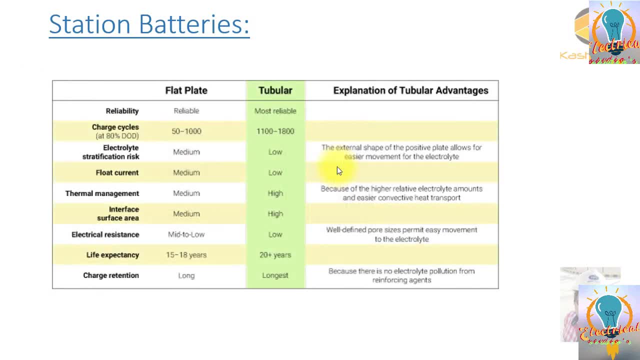 batteries. here is some comparison of the flat plate and tubular batteries. you can see reliability: tubular are more reliable and also tubular battery is more expensive. you can see charge cycles, so clearly the tubular batteries have bigger and more reliable charge cycle. and then electrolytes stratification risk is medium. here it's low because 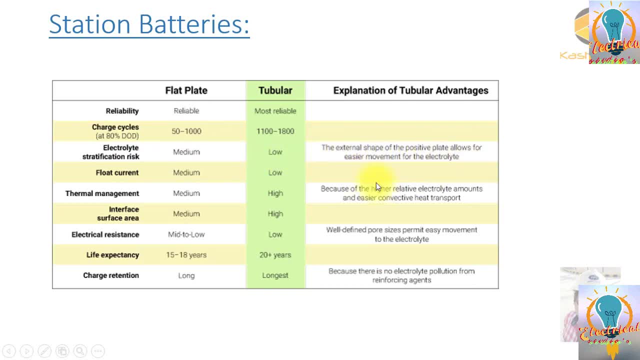 external shape of positive plate allows for easy moment for electrolyte. float current here is medium and the float current here is low, so it's less burden on the charger. thermal management is medium and the tubular thermal mat management is high because of construction. is this tubular battery? 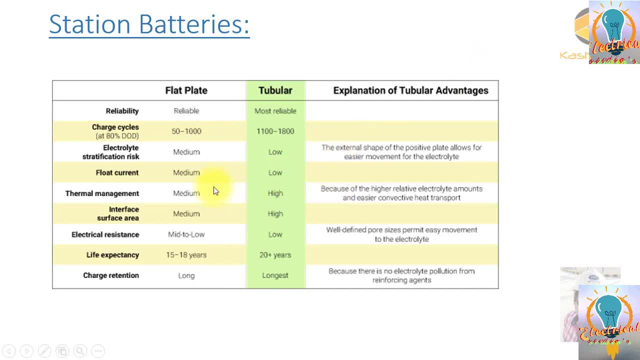 will not heat up as 글 quickly as the flat plate battery. surface area is medium and surface area is high. electrical resistance is mid to low. and here the electrical resistance is low why? because well-defined pore size permit easy movement to act to the electrolytes. life expectancy of tubular is more than the flat plate charged. 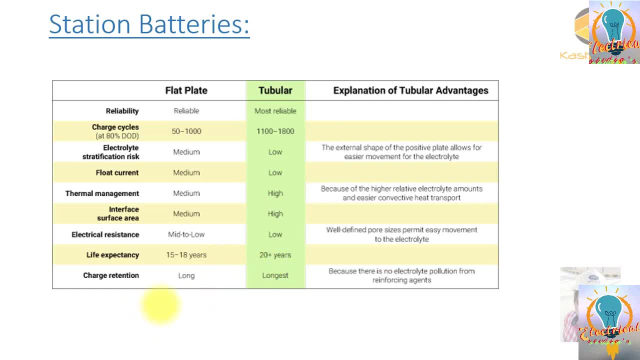 engine in the flat plate is long but in the tubular is its longest because there is no electrolyte pollution from reinforcing agent. so this is little comparison of these two batteries. so I hope this has given you an idea and on the station's mostly you will see the tubular batteries which are deep cycle. 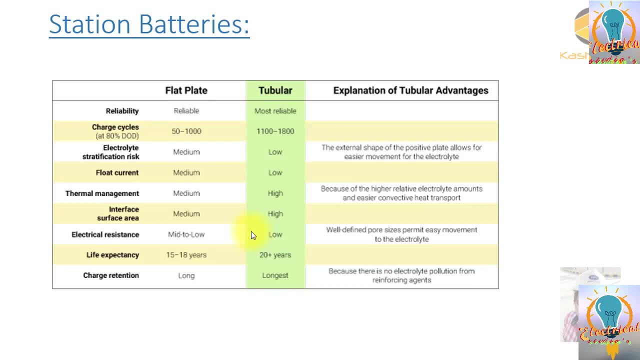 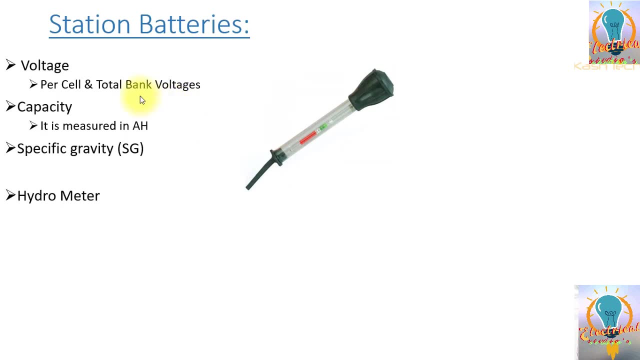 and which are more reliable. thank you very much. I have friends. we will start our new topic and that's in this topic we'll study the voltage capacity, specificity and energy resistance of this Lorin battery. some information about the hydrometer. so the per cell voltage of there are two. 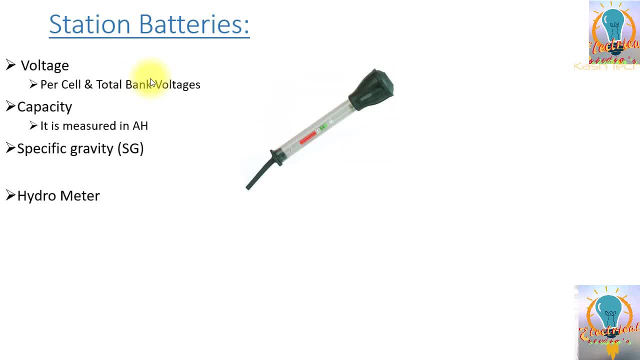 different type of batteries. one is basically the nickel cadmium battery and another one is a lead acid battery. for the nickel cadmium battery, the voltage per cell is normally less, and it's 1.2 volts per cell, whereas for the lead acid battery, then, number one voltage is almost 2 volts per cell. so 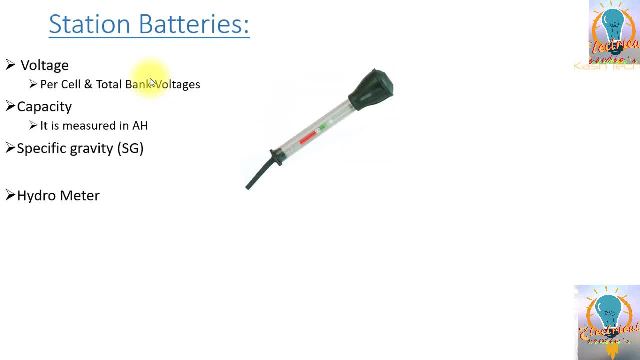 you know that in in in the substation we have to form a bank of 220 volt and 110 volt, for example. so you need to connect the batteries in series. so, for example, if you want to care, if you want to use nickel cadmium battery to form a 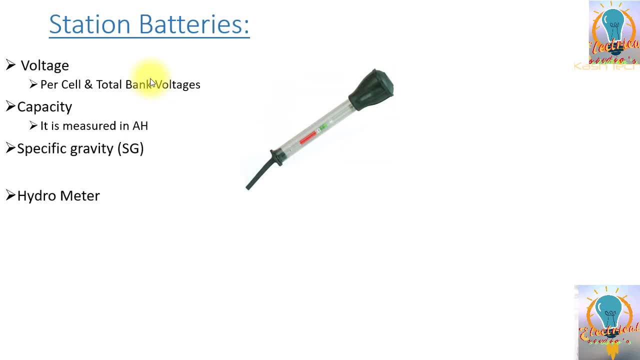 110 volt bank, then you need 92 nickel cadmium batteries. 92 into 1.2 will be 110. and if you want to prepare a 110 volt DC bank battery bank by using a lead acid, then you need a 55 total number of cells. so this is. 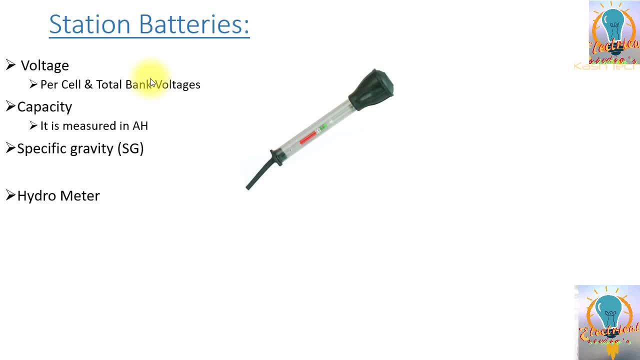 little introduction about the voltage rating of the battery in the banks. then next come is basically the capacity of the battery. so capacity of the battery is measured in ampere hour. it mean that if a band battery is battery, single battery rating is or the bank battery rating is. 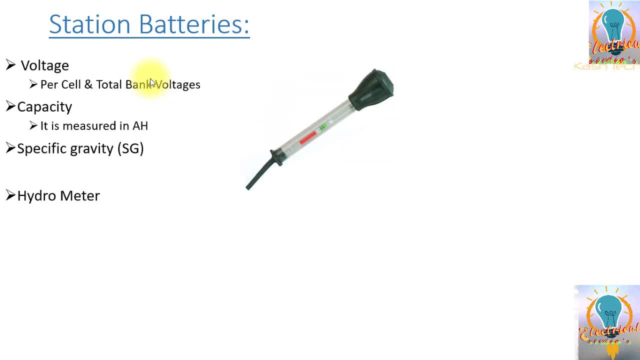 hundred ampere hour, so it mean that it can supply 10 ampere for 10 hours, or- it makes things somewhat complicated since we want to build the ampere in 2 hours- can supply 1 ampere for 100 hours, so it means that you need to multiply Ampere. 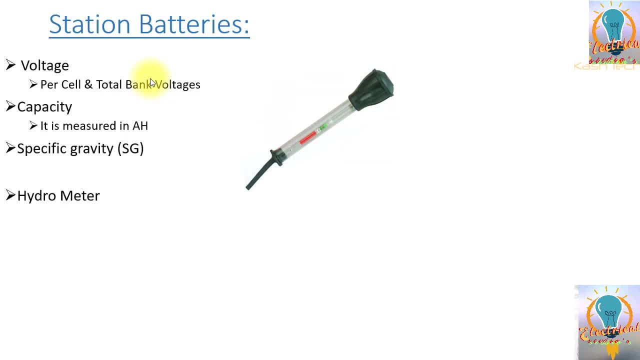 into hours, but the range should be within that specified rating. so the girth should be reduced to 5 k. Results: battery should be able to supply the rated or minimum allowable voltage to the network within 10 Amts time. Let's talk about equivalent battery. 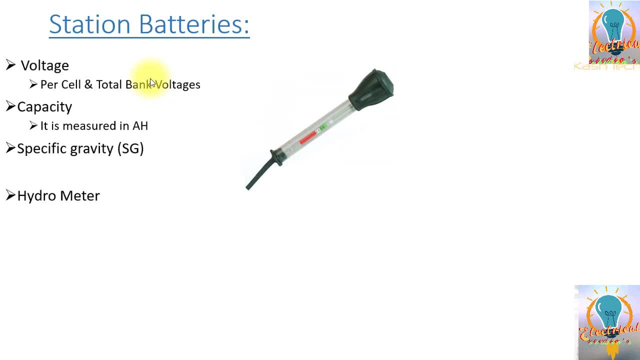 its capacity defined. So this is basically the concept. Now, regarding specific gravity, a simple hydrometer reading indicates the state of charge in the cell. Specific gravity is basically when the lead-acid batteries and the electrolyte is charged, the specific gravity is high. When the electrolyte is discharged, the specific 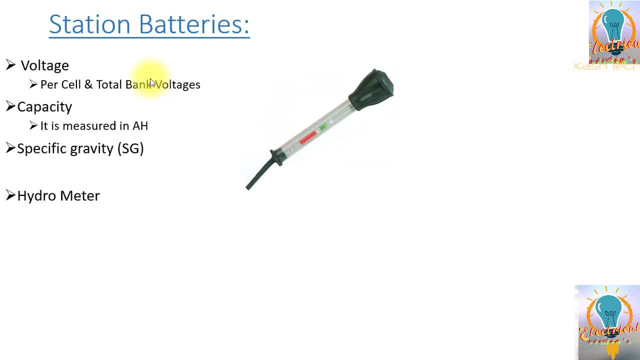 gravity becomes low. So it's basically how much the specific liquid is heavier than the water. It's measuring this thing And for lead-acid batteries, the hydrometer operator needs to come and check regularly the specific gravity of the battery. 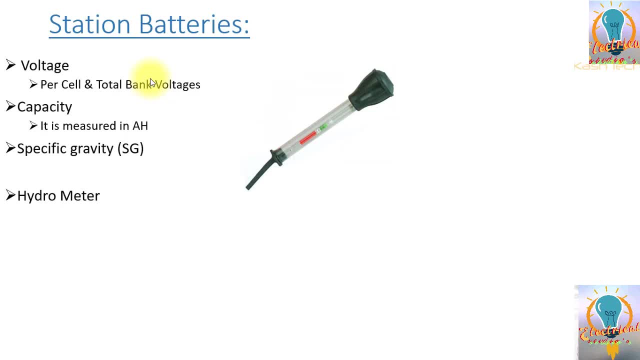 In order to confirm that batteries are charged and everything is fine. But for the lead-acid batteries, the gas manufacturer is not relating the specific gravity with the charge, charging and discharging of the batteries, because this is a different type of batteries, like nickel, cadmium. 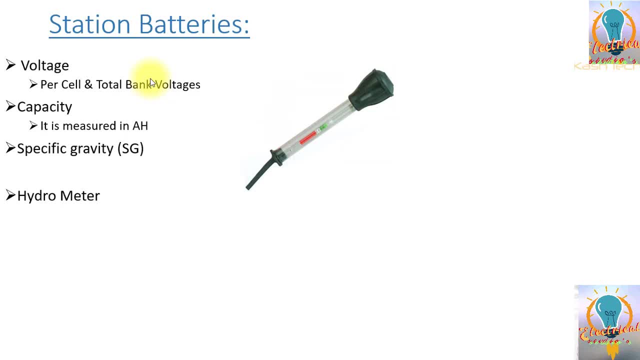 So a simple hydrometer indicates the state of charge in a cell. A fully charged cell will have a specific gravity reading of between 1.025 and 1.215. as a thumb rule in lead-acid battery, Open circuit volts is equal to specific gravity plus 0.84.. Thus the open circuit volt at 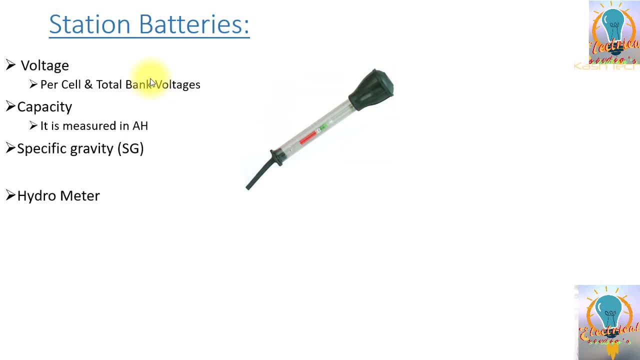 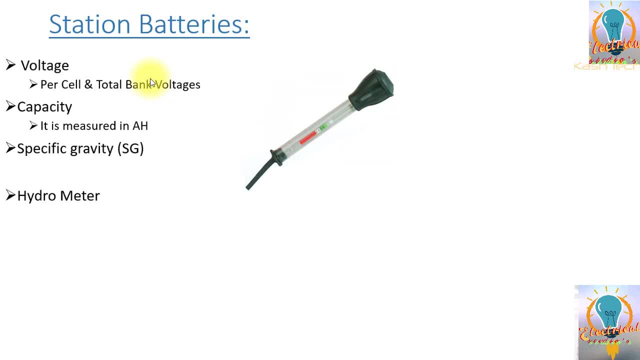 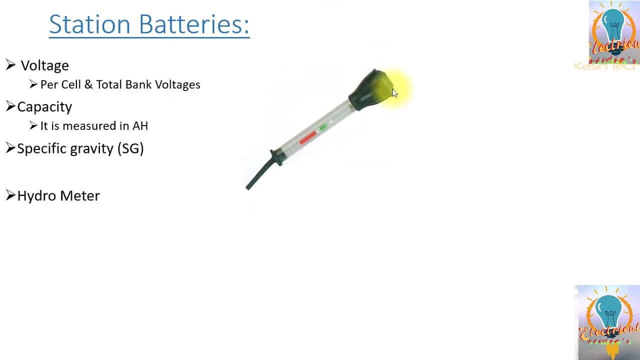 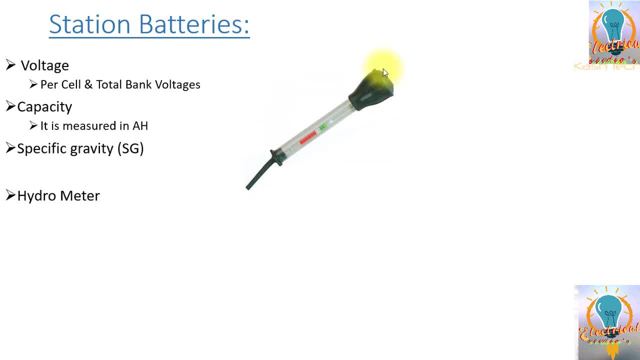 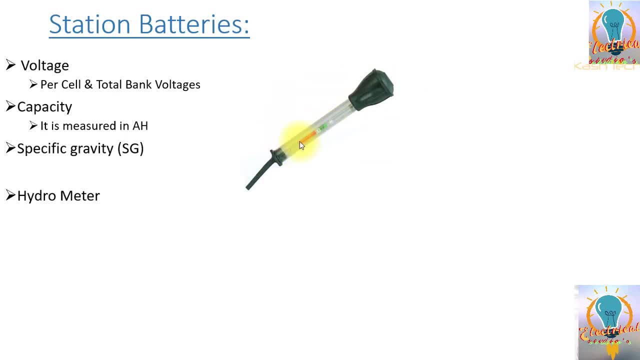 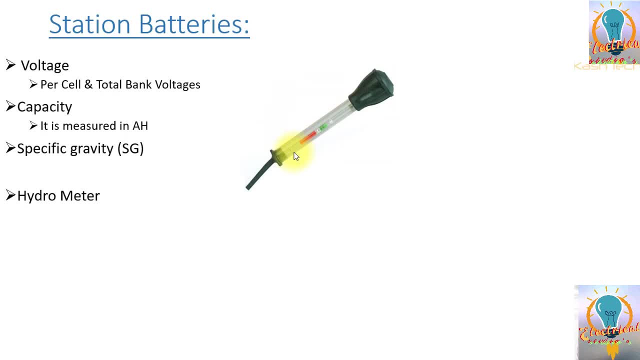 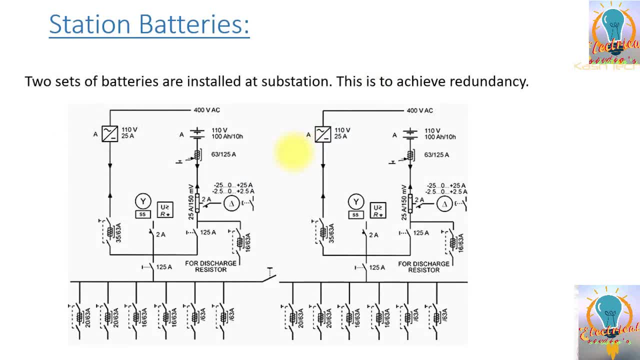 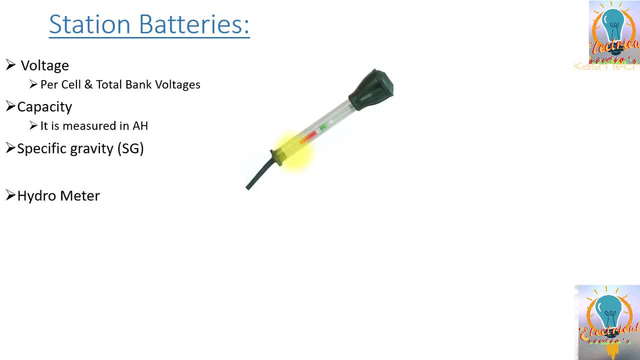 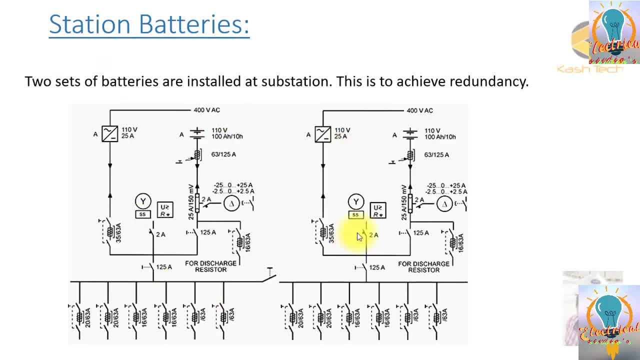 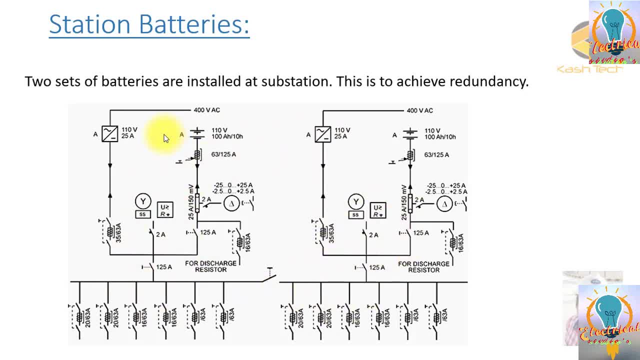 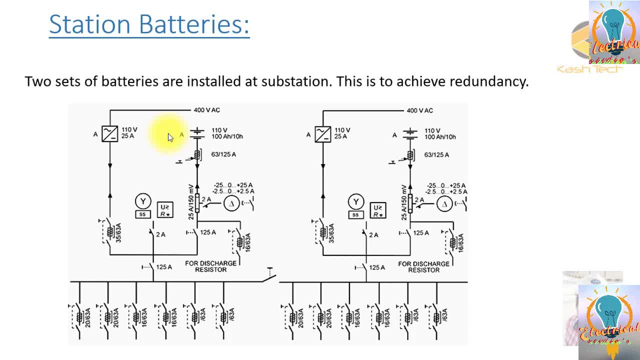 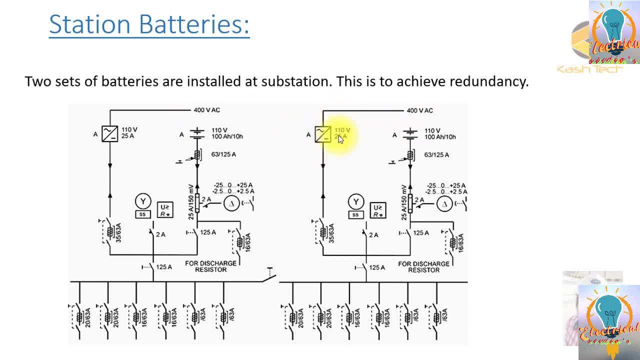 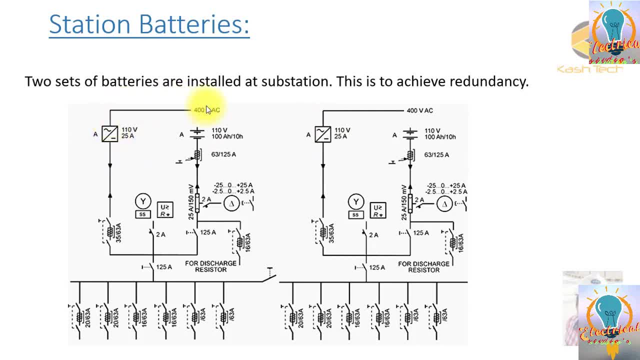 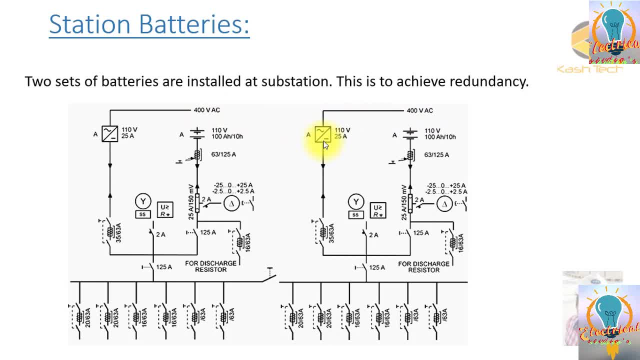 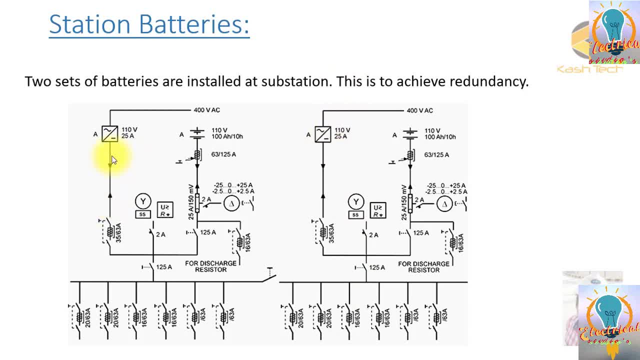 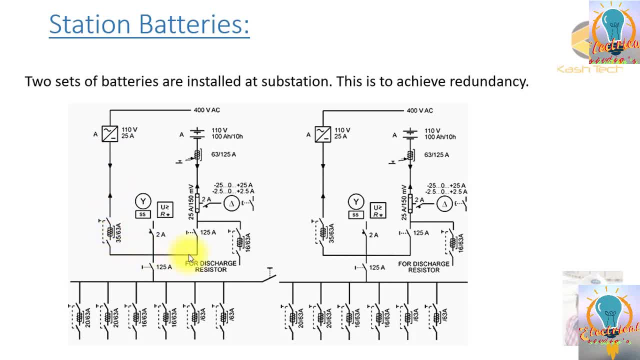 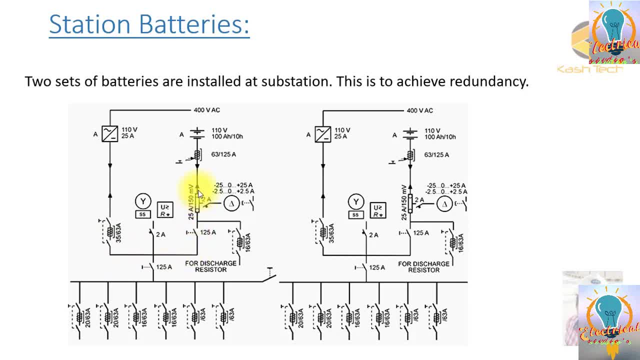 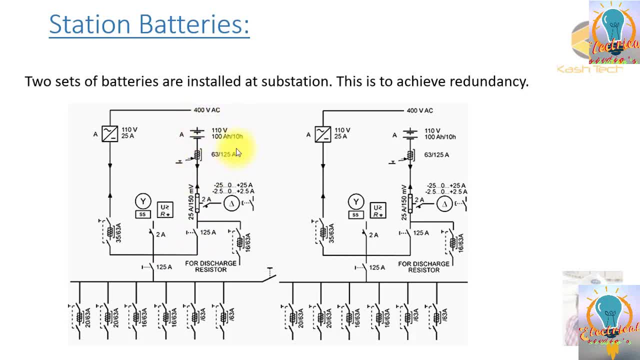 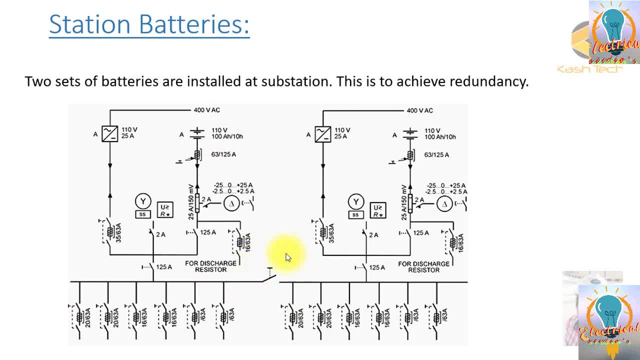 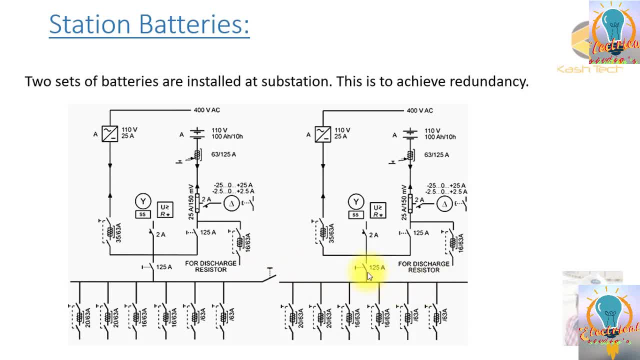 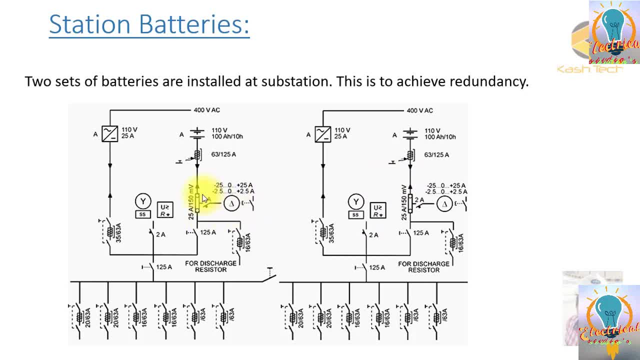 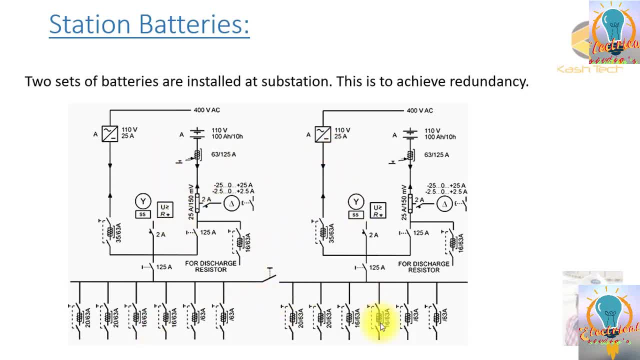 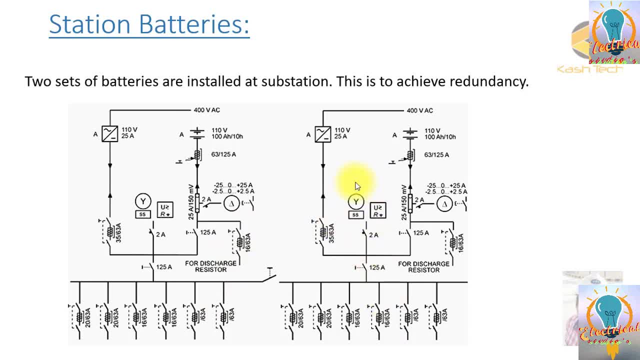 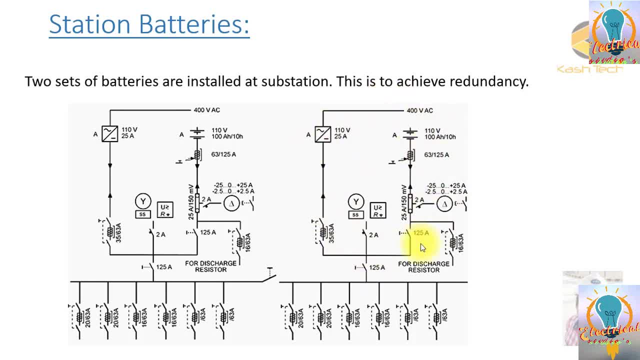 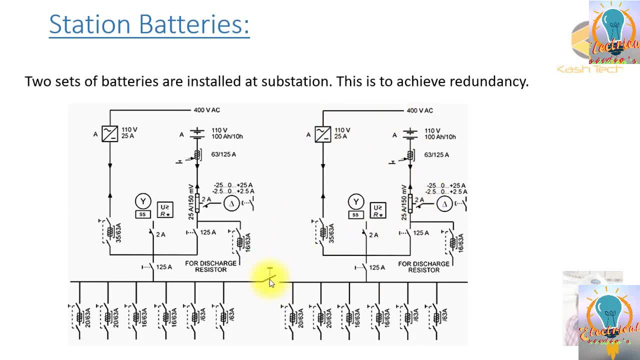 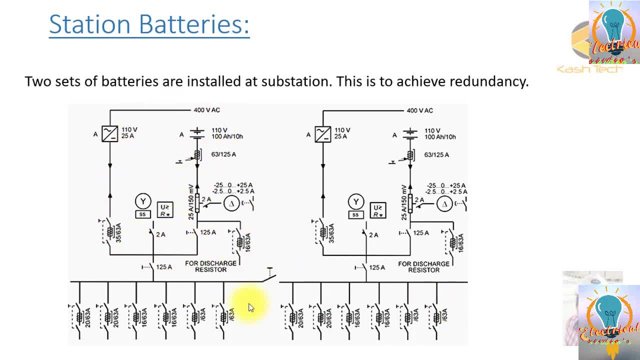 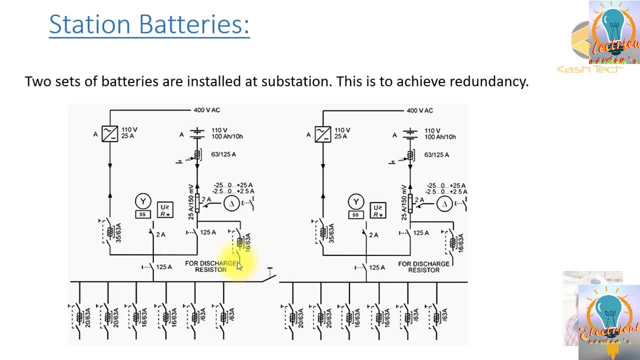 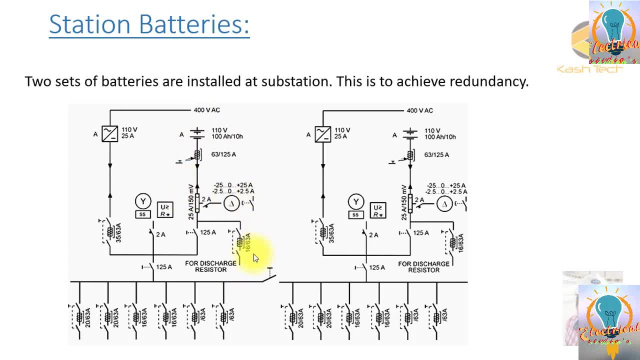 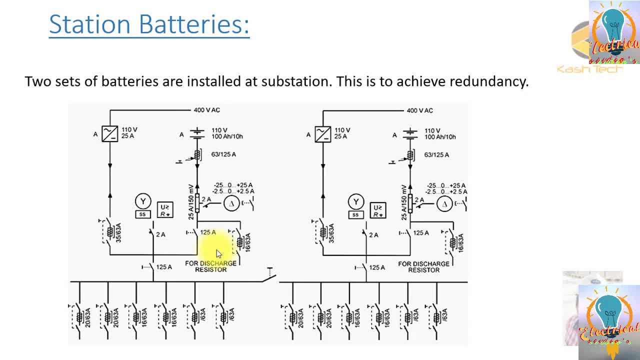 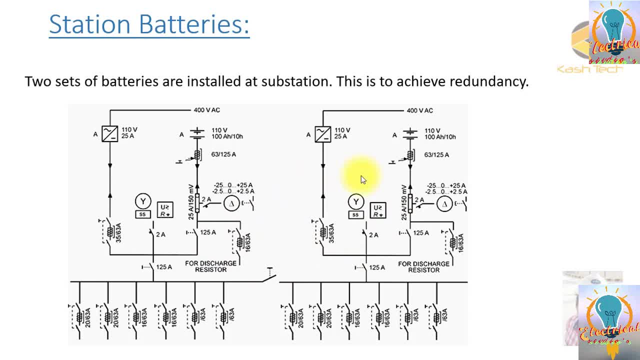 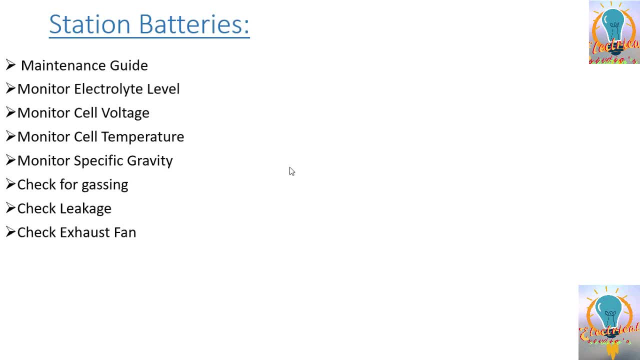 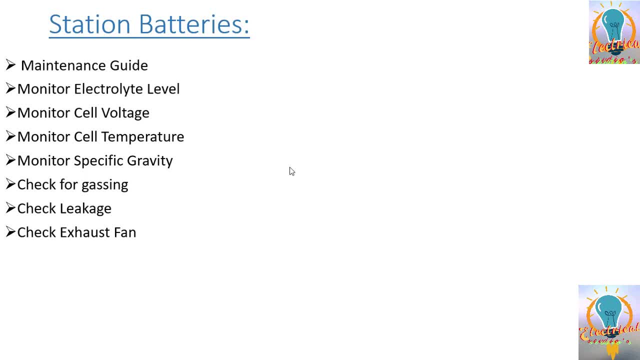 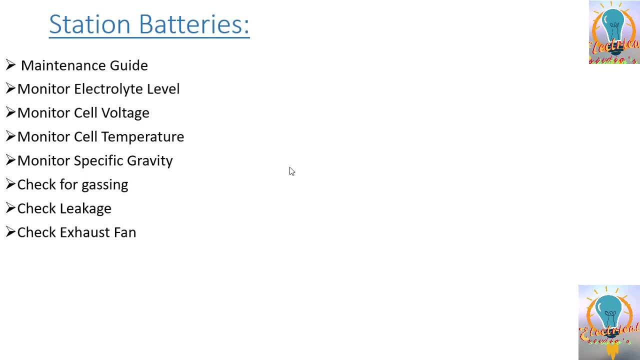 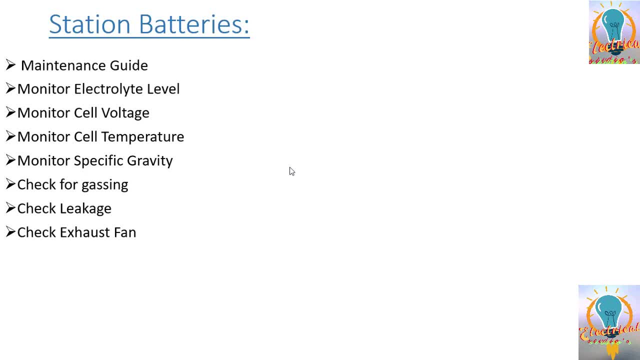 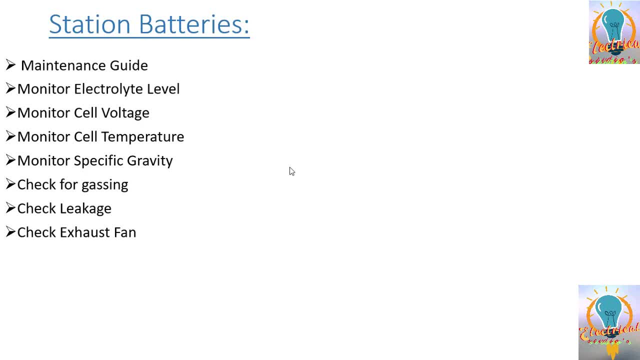 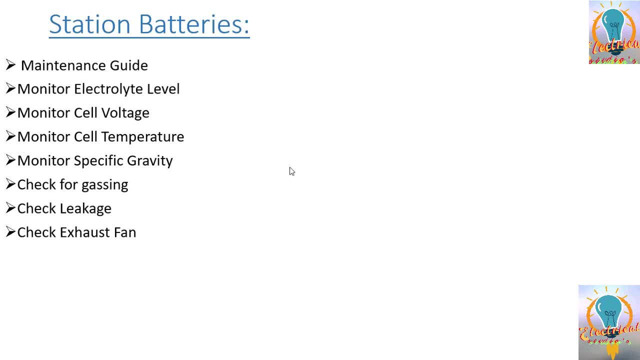 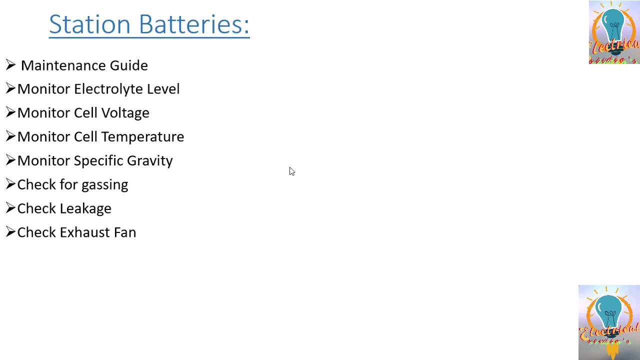 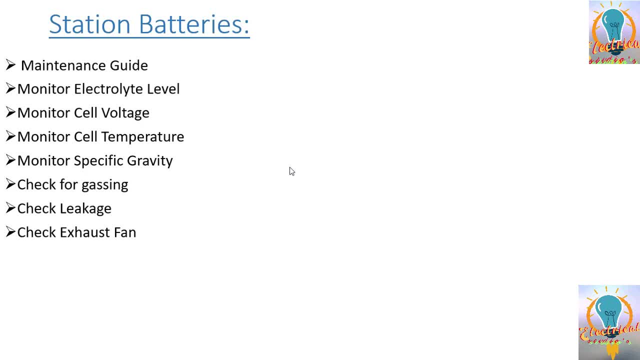 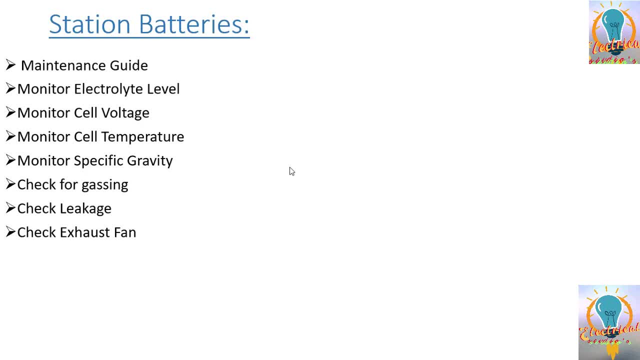 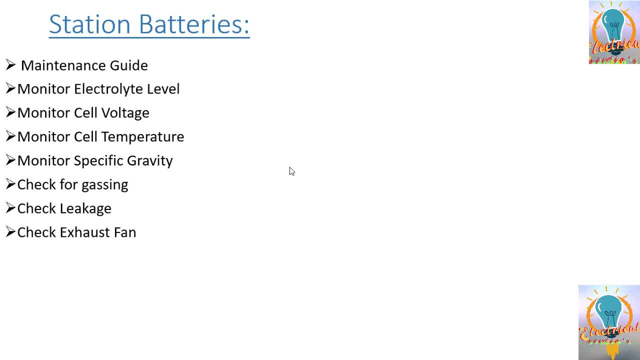 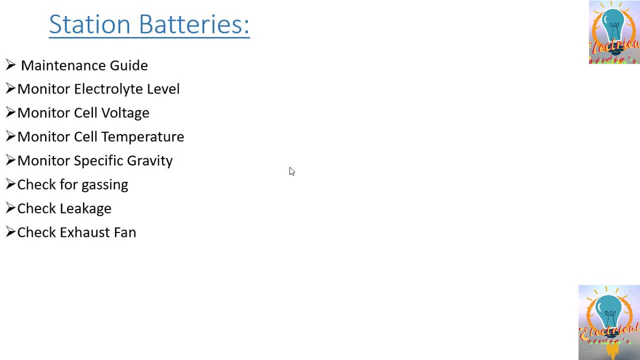 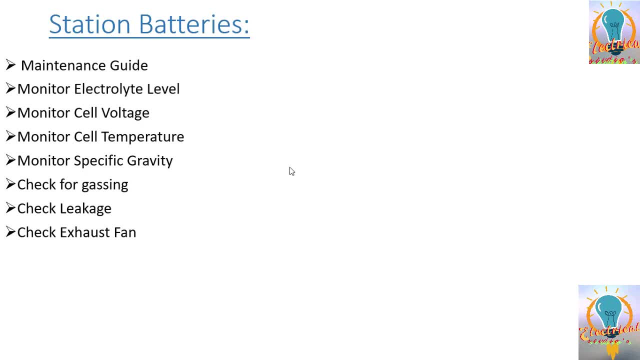 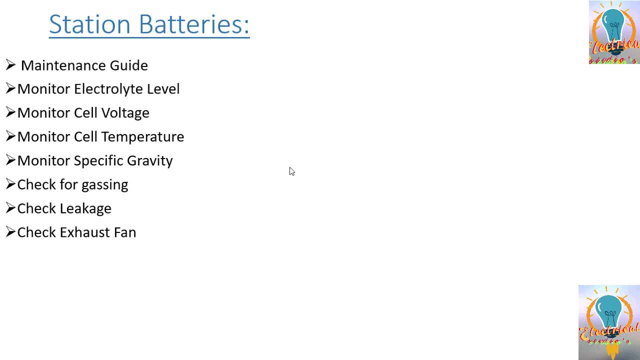 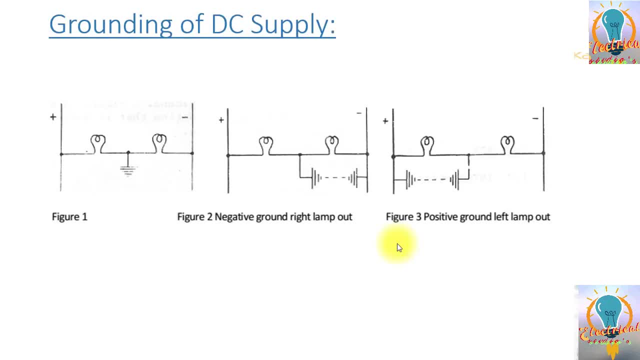 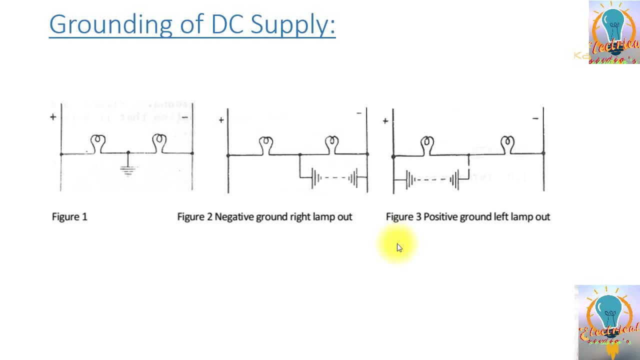 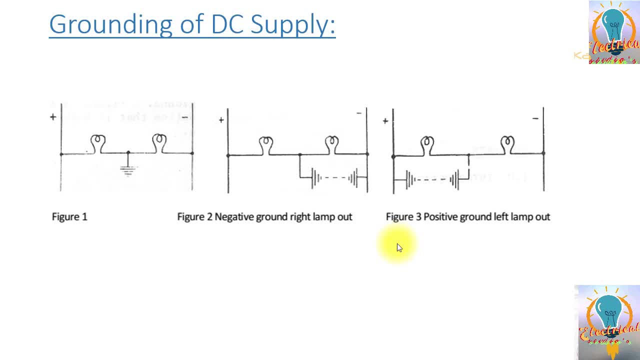 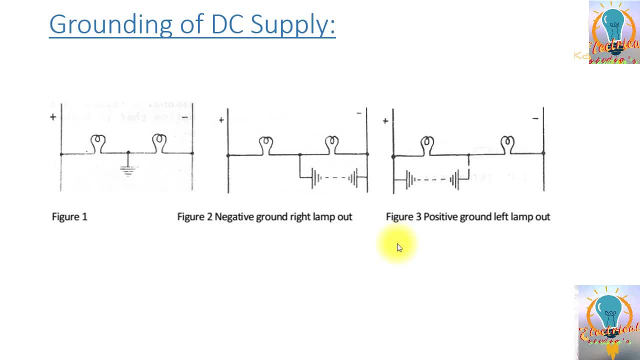 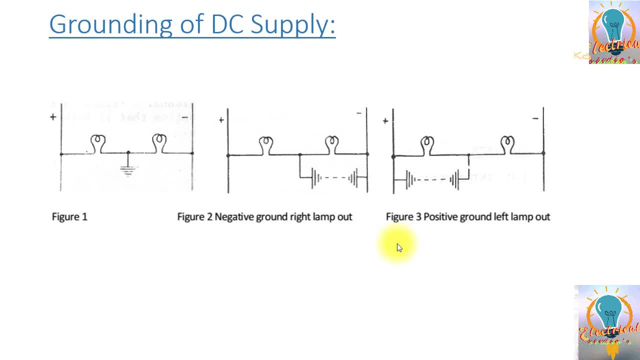 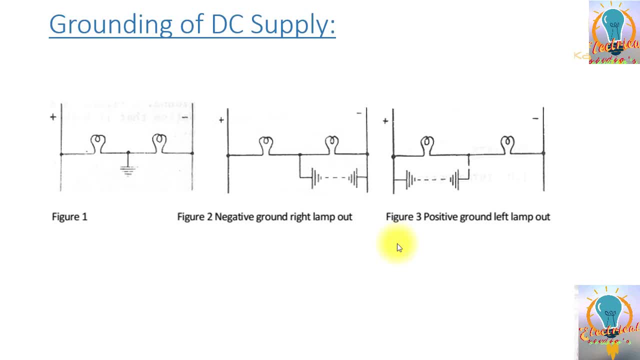 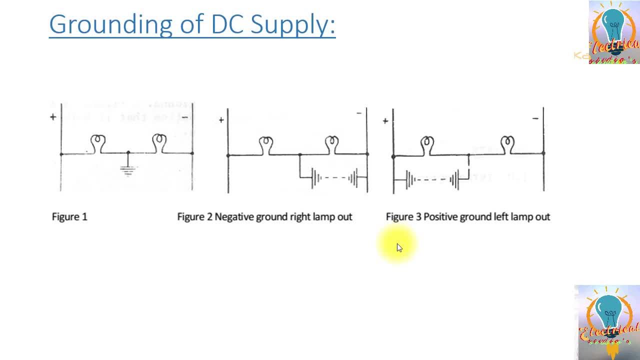 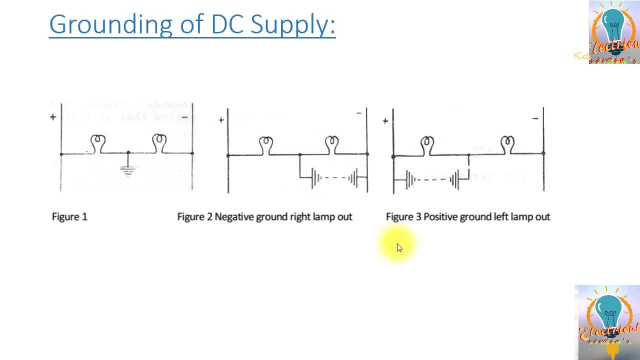 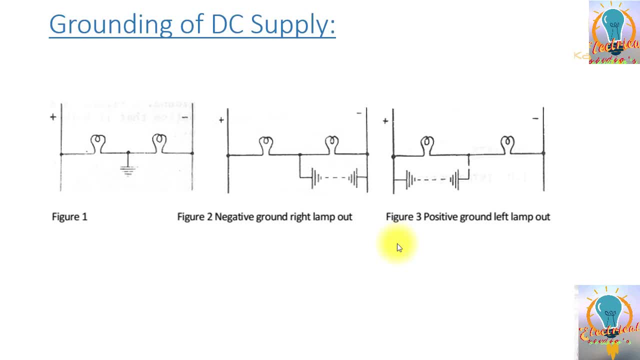 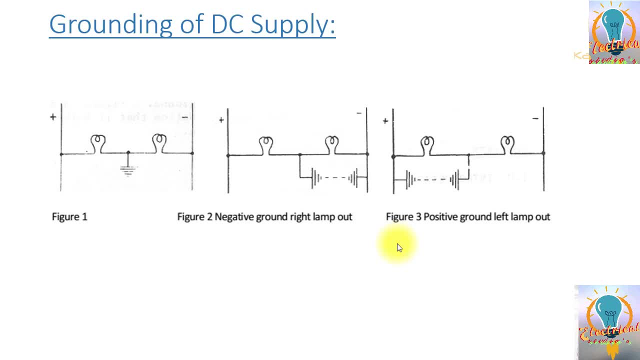 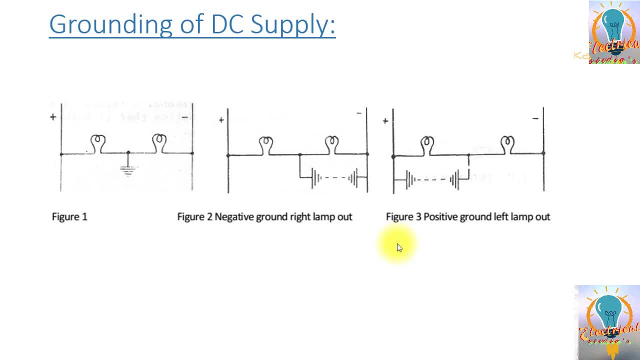 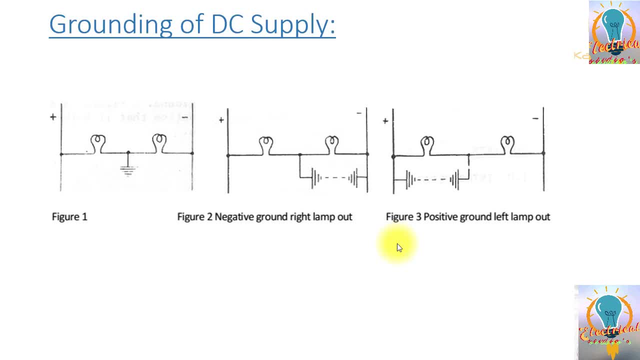 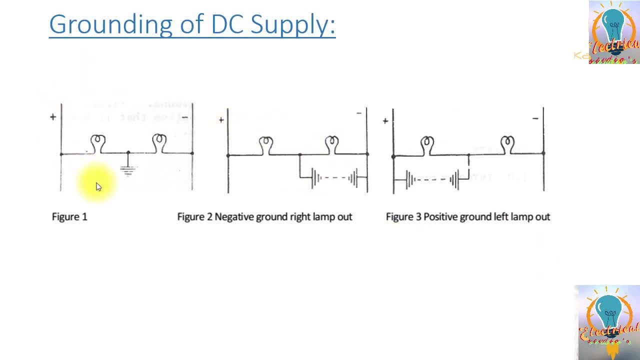 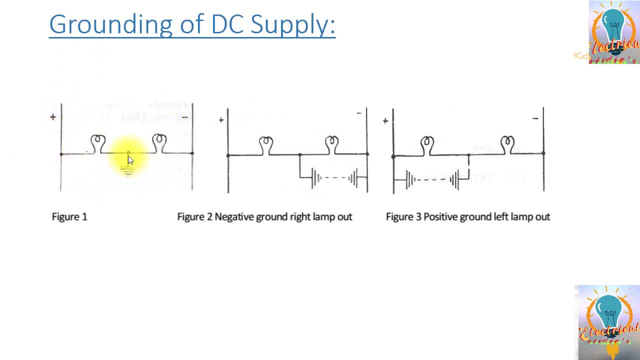 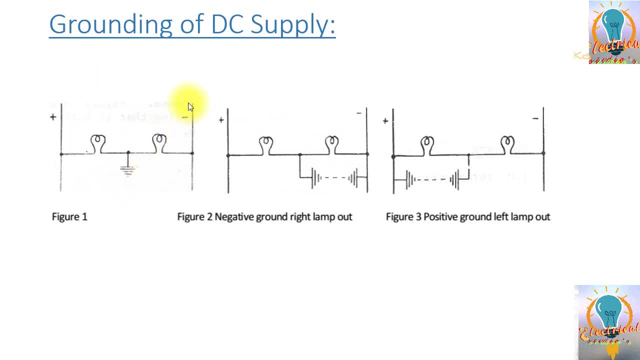 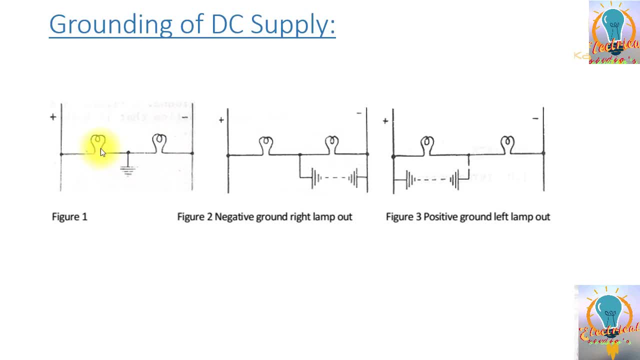 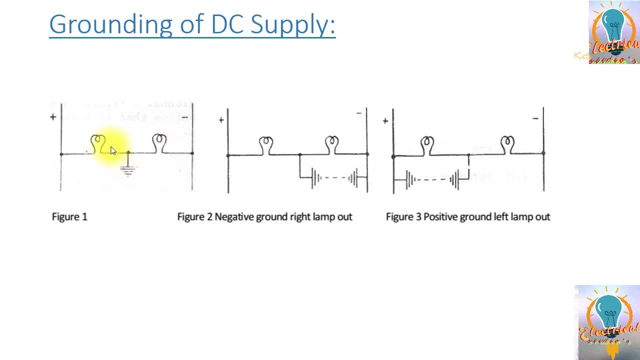 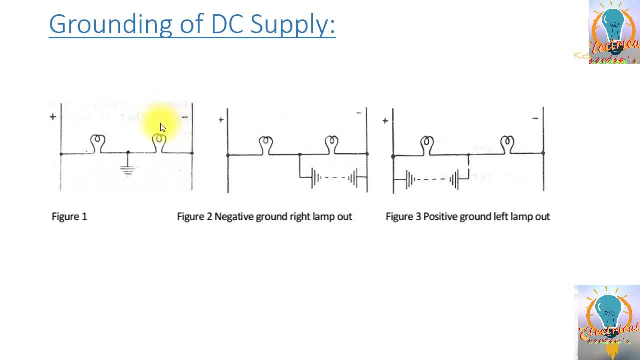 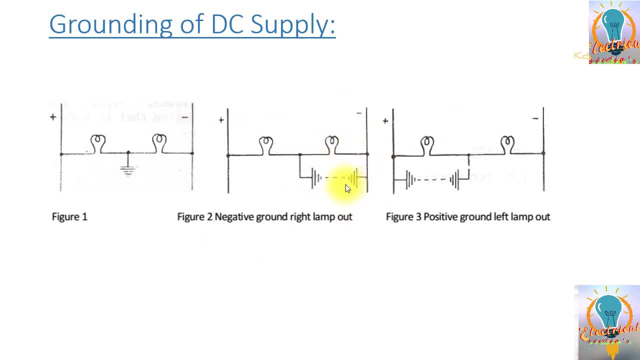 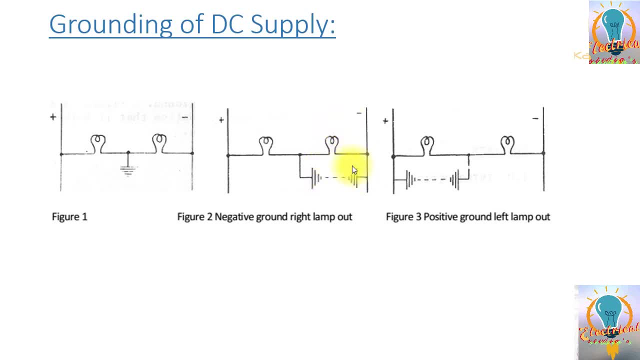 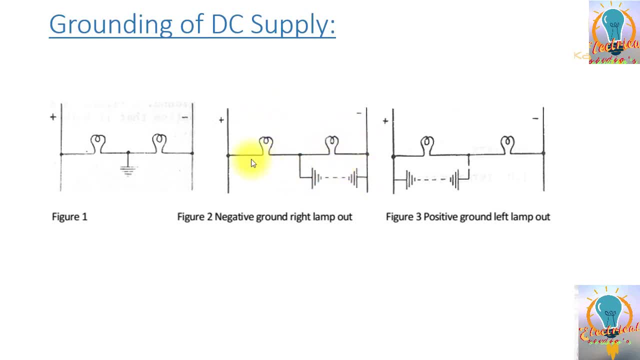 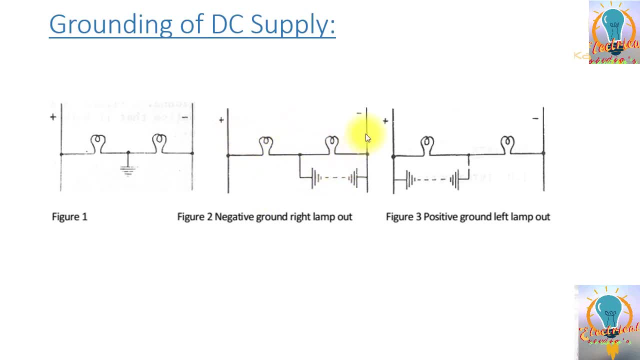 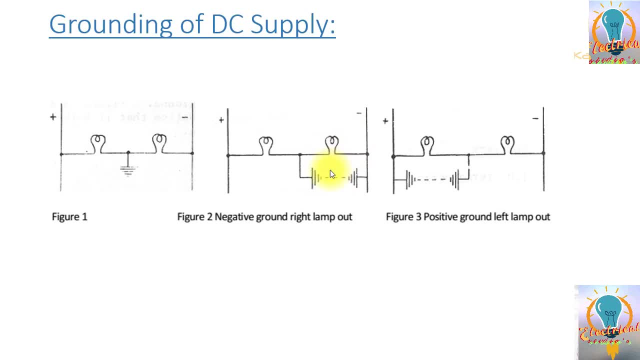 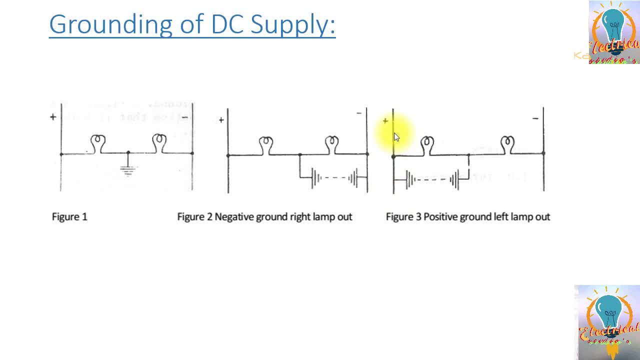 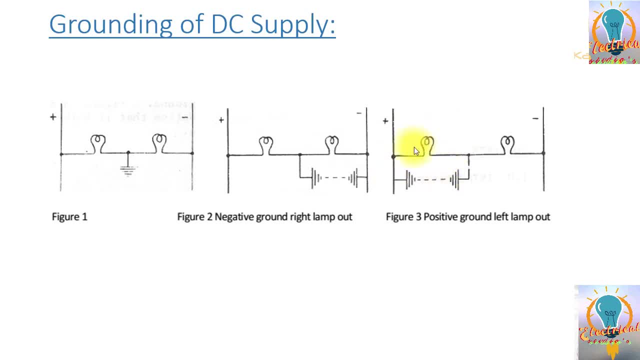 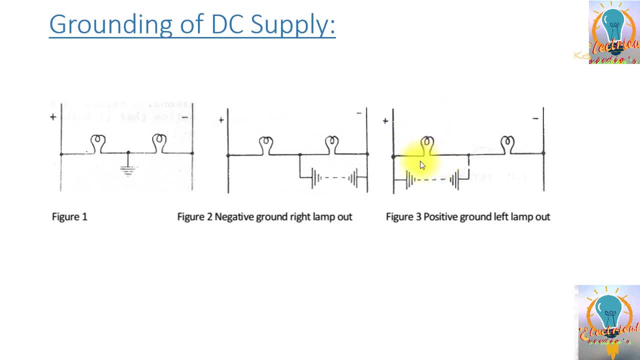 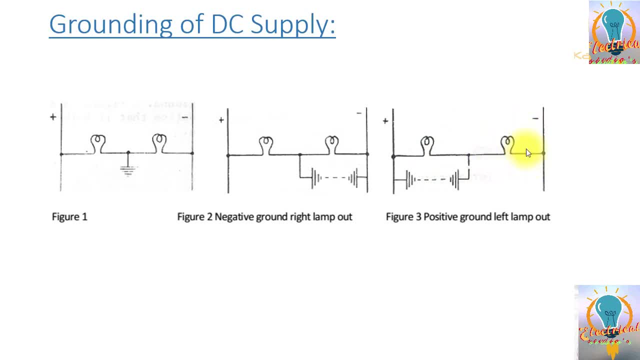 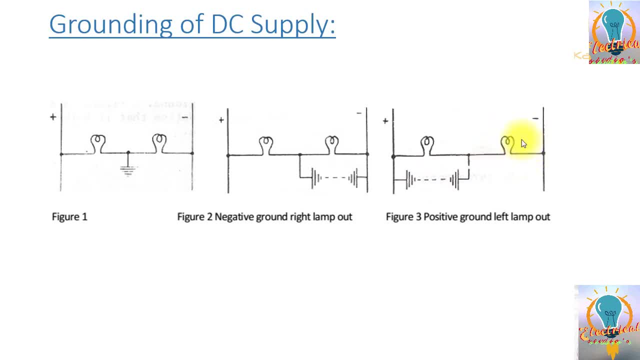 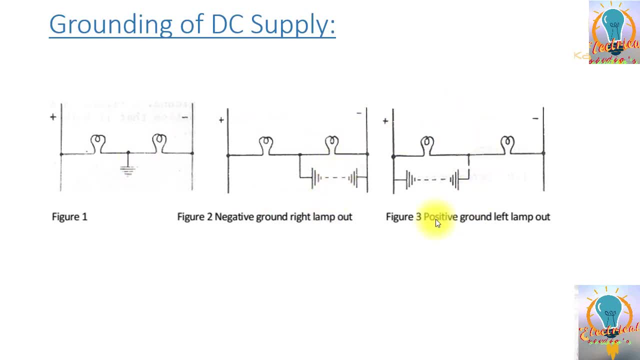 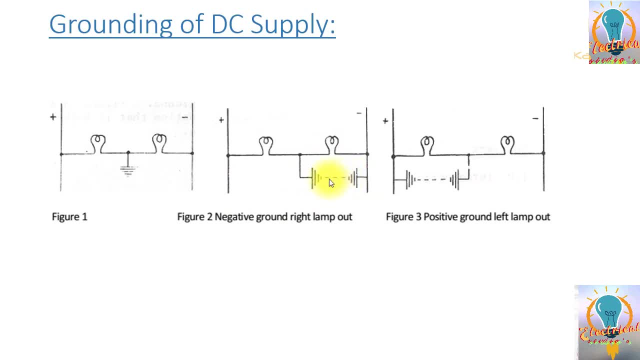 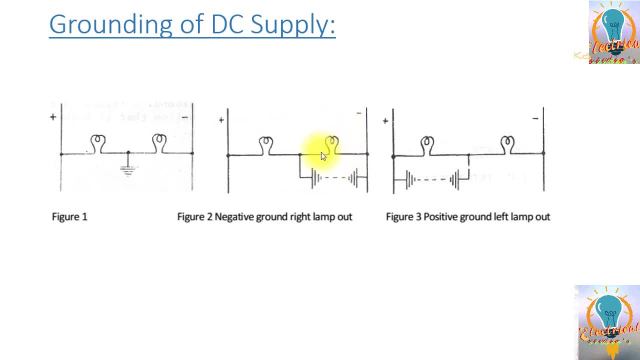 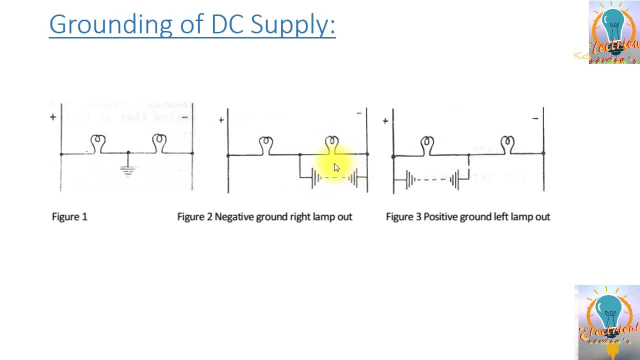 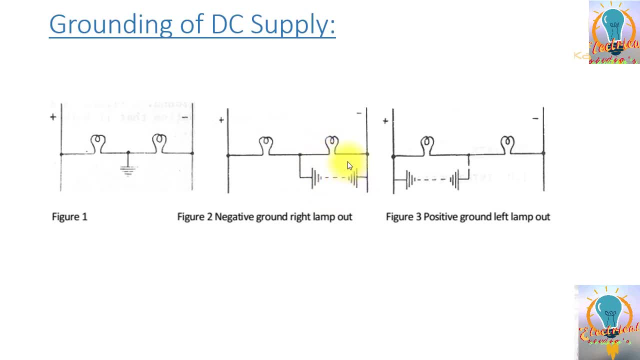 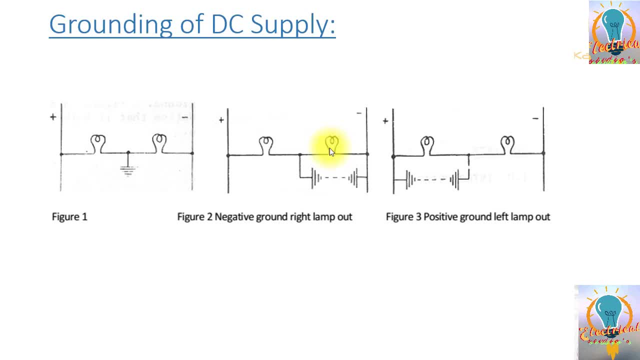 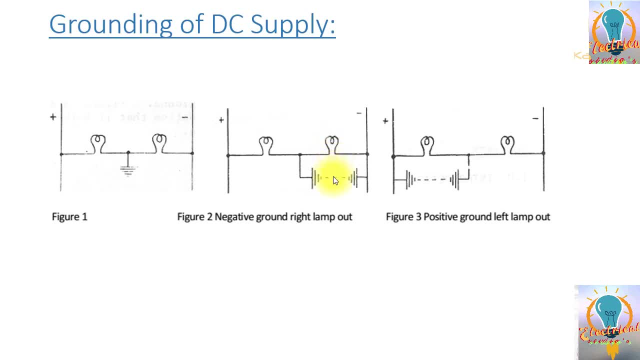 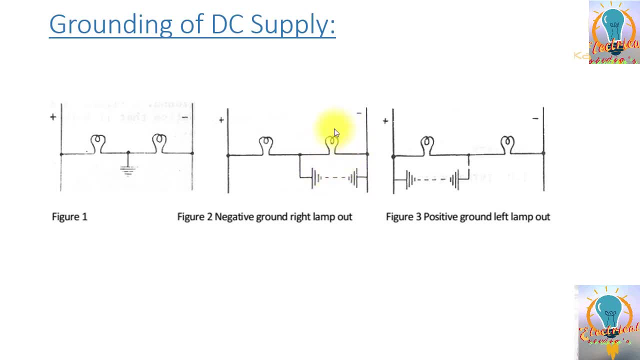 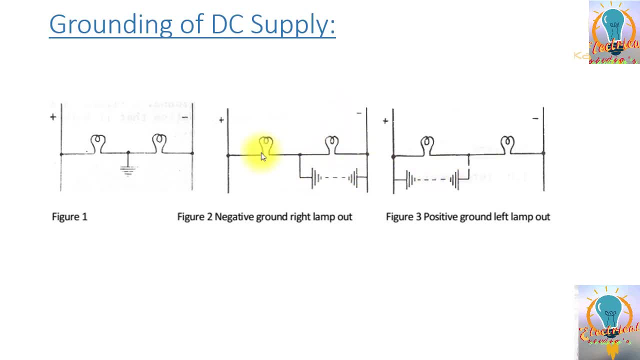 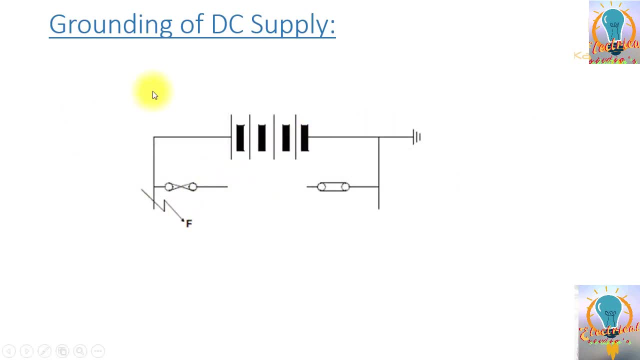 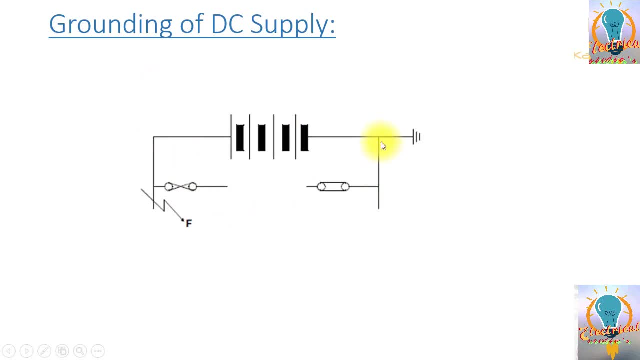 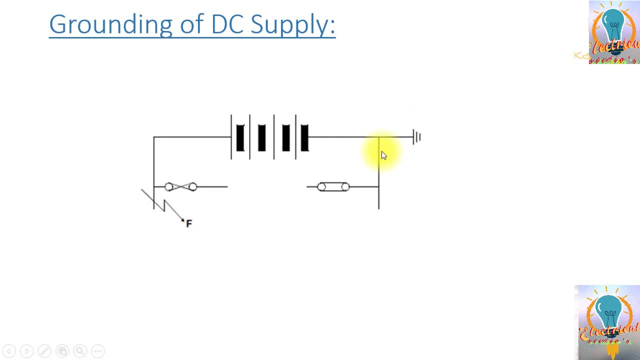 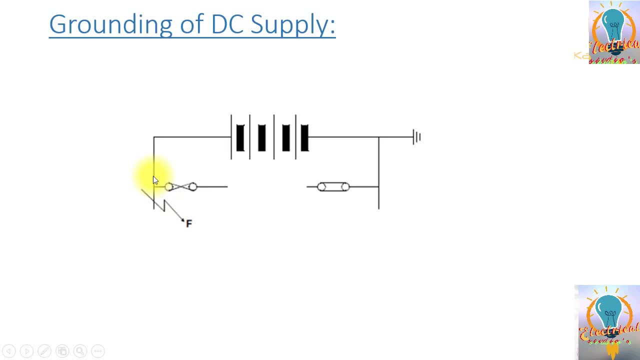 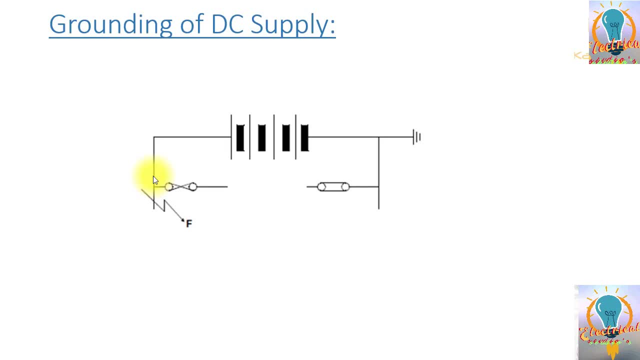 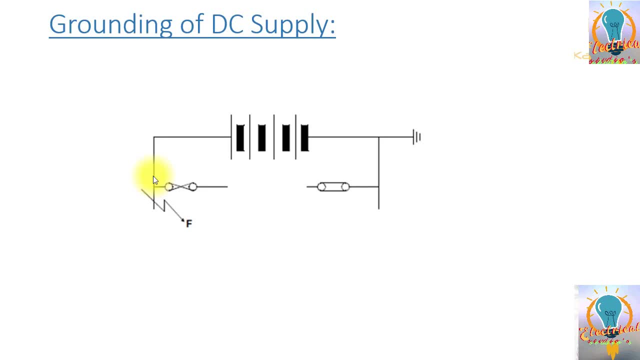 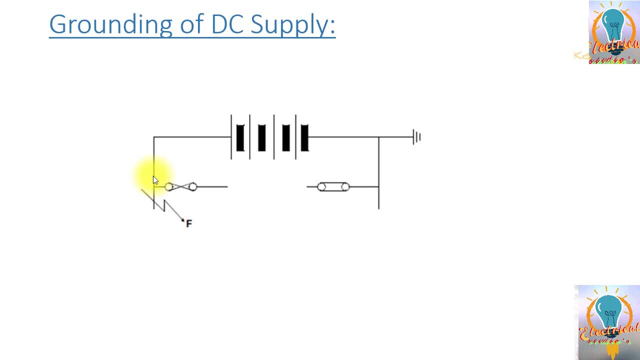 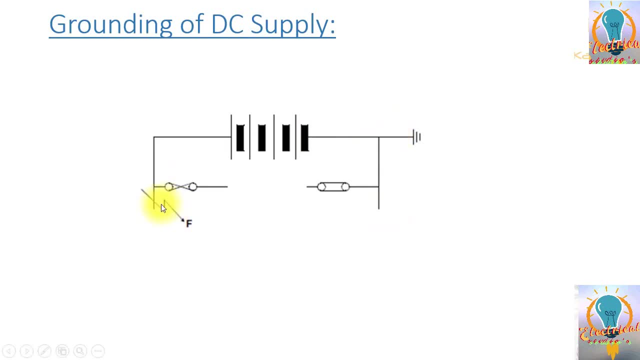 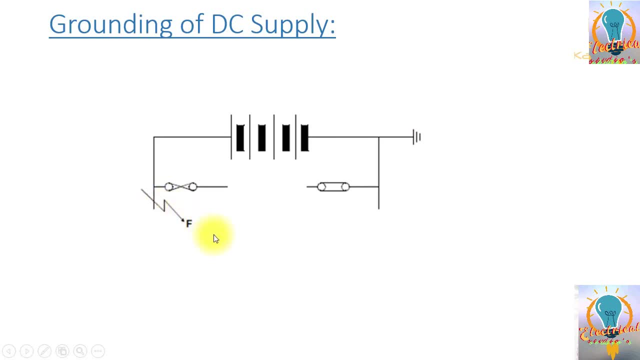 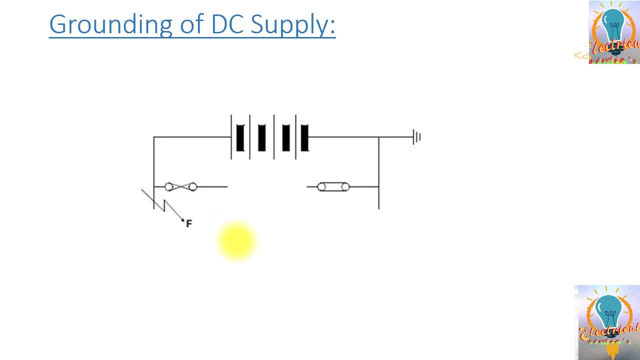 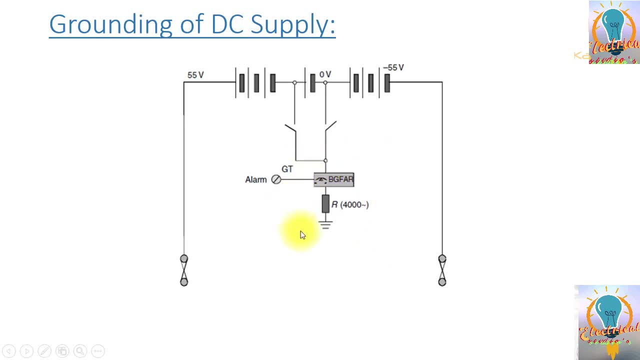 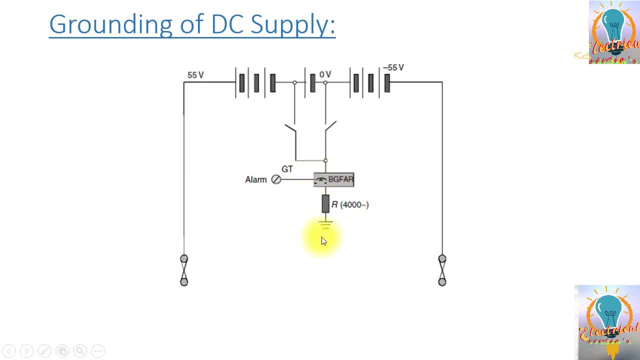 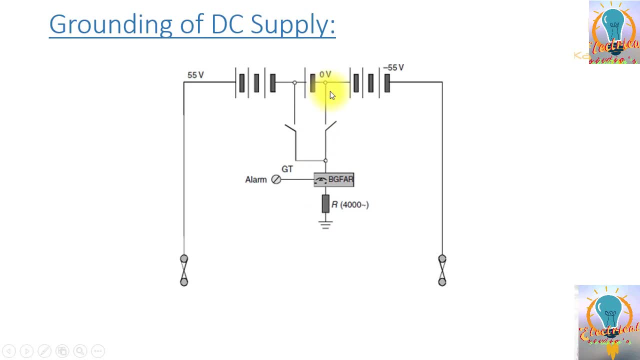 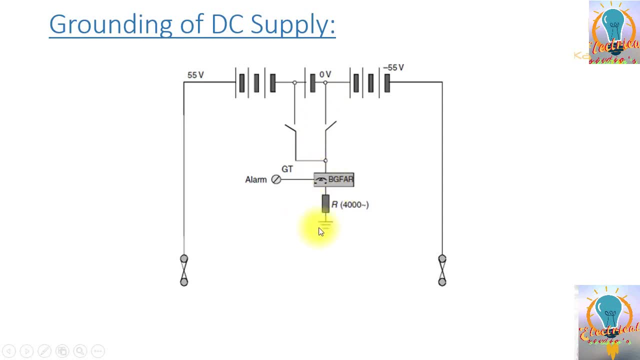 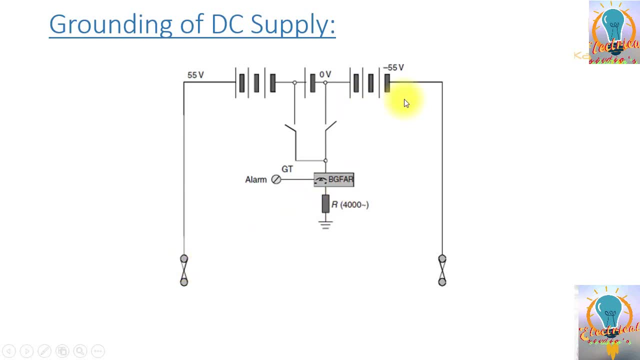 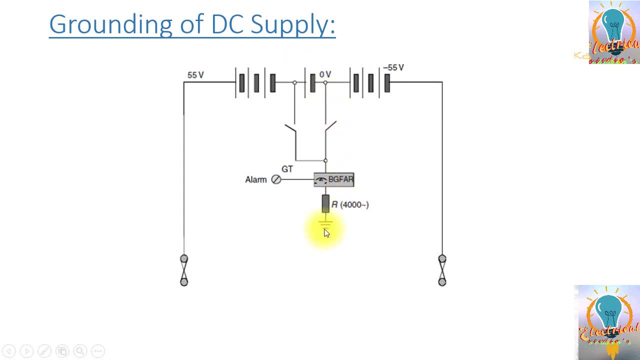 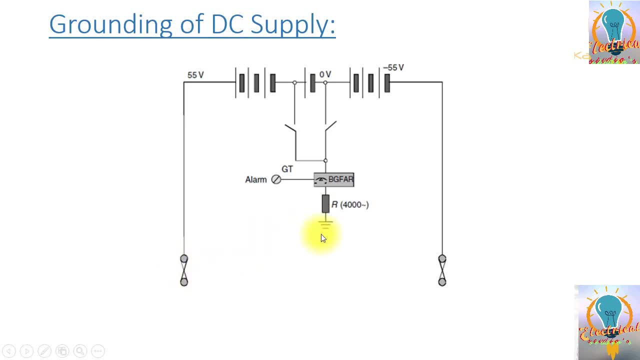 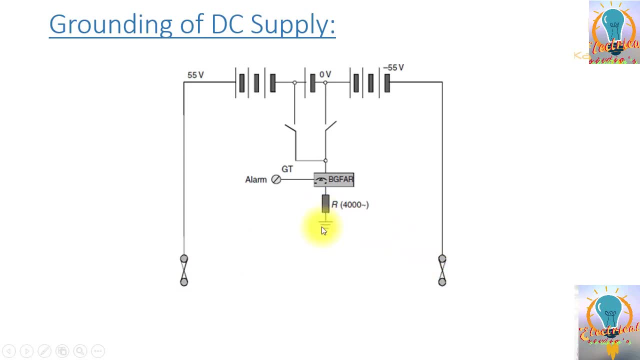 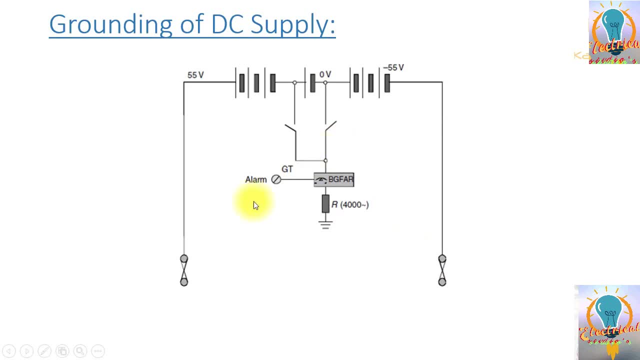 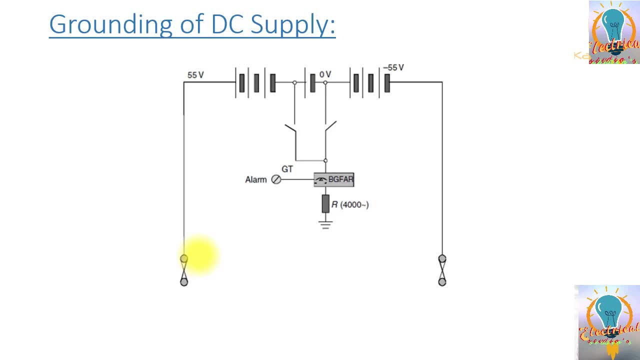 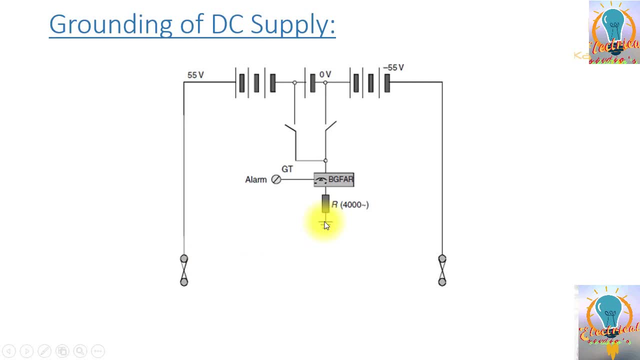 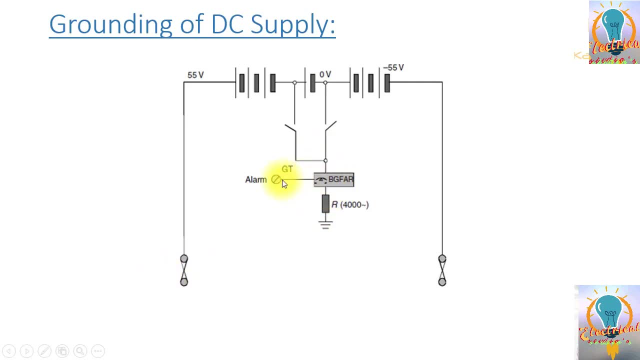 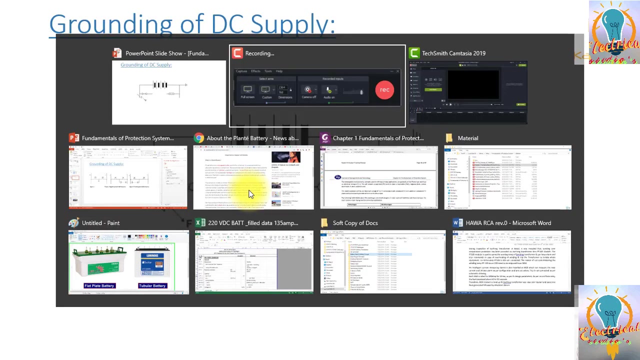 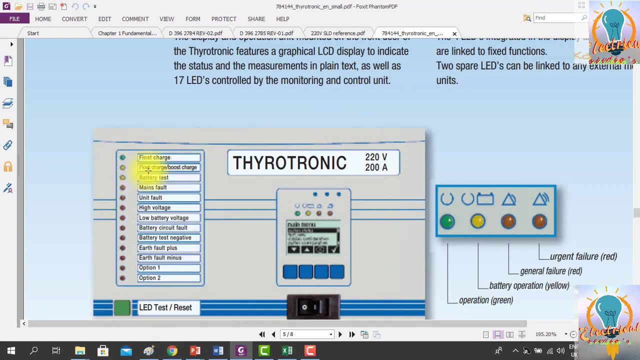 some current will flow through this relay and it will create alarm that system is grounded. So these are some methods that are used in the DC system to create a ground and to detect the ground fault. So here this is basically the DC charger. this is the display and you can see lot of different. 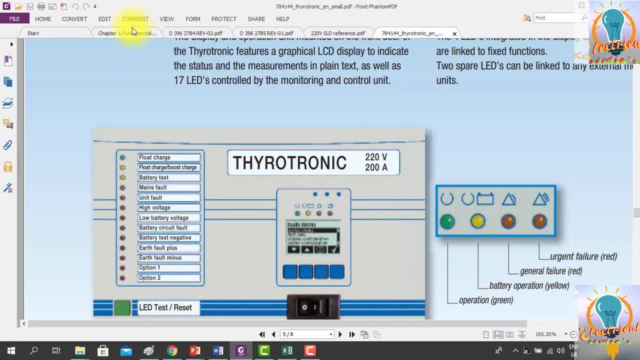 LEDs here. So here you can see this is the basically earth fault plus. it mean the plus has grounded, earth fault minus and between the minus has been grounded. So this system is detecting the fault and this system is using the same technique that we have just discussed. 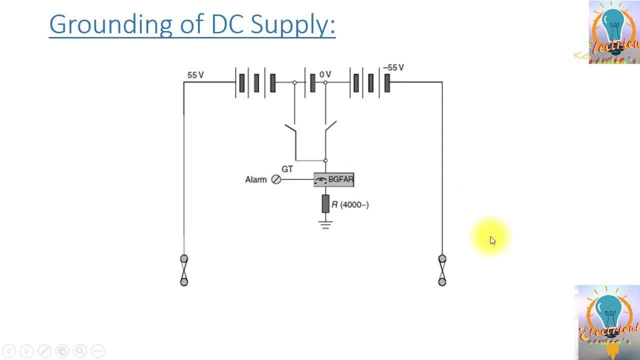 that is, this type of connections. So this is basically a very good idea to understand and how it is detecting that this plus is grounded and minus is grounded. It is simple: if the plus is grounded, the direction of current is in one direction. if the minus is grounding, the direction of current is in another. 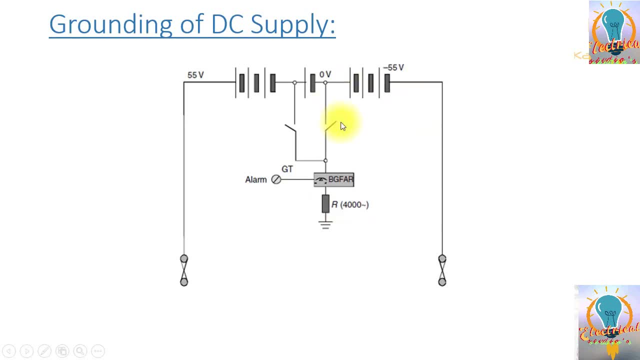 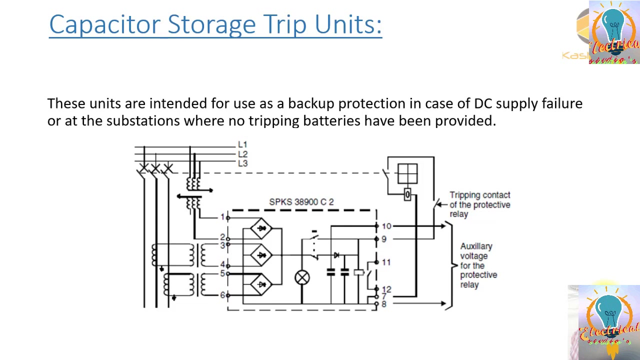 direction. So these are some techniques by which we are grounding the DC system, and this is just to protect the system and monitor the system. Thank you very much. So we will start our also new topic and that's related to capacitor storage strip units. So these are the units which are intended for. 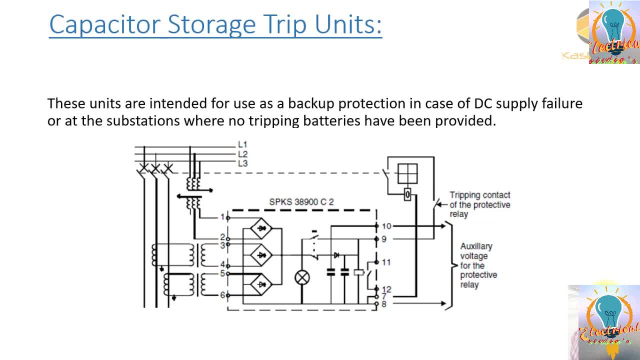 use as backup protection in case of DC supply failure or at a substation where no tripping batteries have been provided. So in Pakistan there is a utility which is called a K-electric and what happened here is basically- there are some incidents- more than once that whole the substation is burned out, and when the 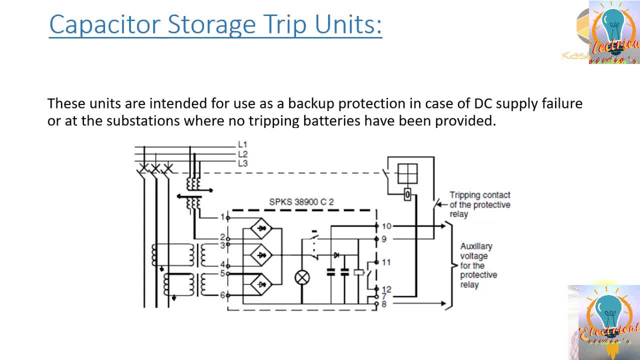 investigation was took place. then they find out that the DC system has been failed, so no protection operated on the local grid, and that resulted in total fire and failure of all the substations. So later on they decided to use capacitor storage strip units, So in case, even if the DC supply is failed or even AC supply is failed, whatever, 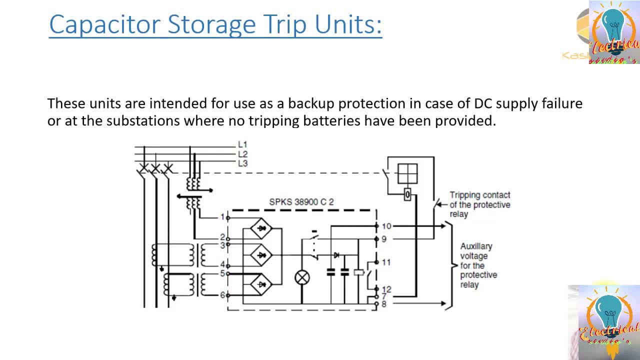 is the case, these units are powerful enough to trip the circuit breaker. So the concept is is that as soon as the DC supply is failing, the breaker will trip through this device. So this device is monitoring the DC supply continuously and as soon as these supplies fail, regardless of anything, it will trip the breaker. So 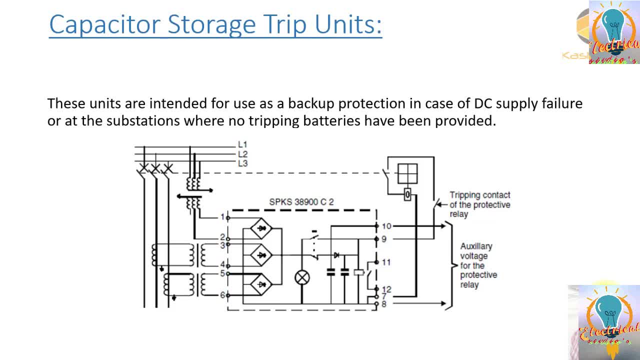 this is kind of protection to the priority has given to the protection then on the reliability or continuity. So as soon as there is a DC is failed, this, the energy is stored in the capacitor and the breaker will trip through this energy. So another example of using this storage capacitor storage unit is 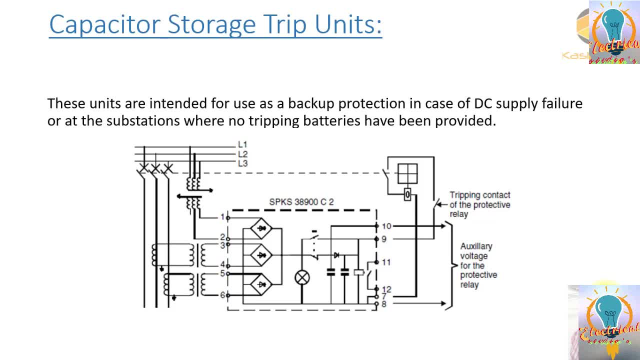 in Ringman units, for example, where there is no DC bank is available. So existing AC supply is used to charge this capacitor storage units and to make the trappings through it. Now here I have shown a very basic diagram for the capacitor storage unit, How the capacitor 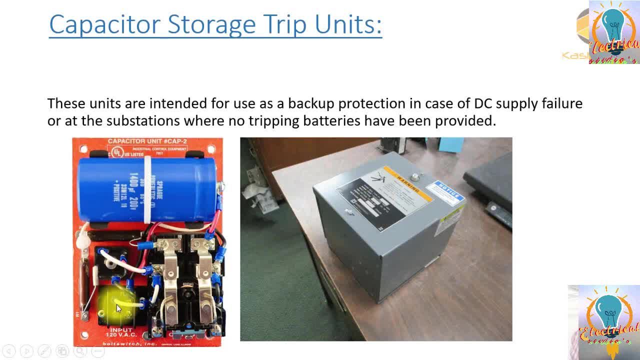 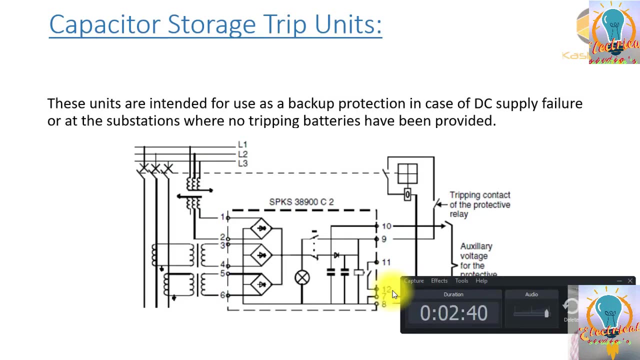 storage unit look like you can see. this is the inside from the capacitor unit And this is basically. if you see in the panel, you will see this type of capacitor storage unit in the panel. So this was introduction of capacitor storage unit. I hope you like this lecture. 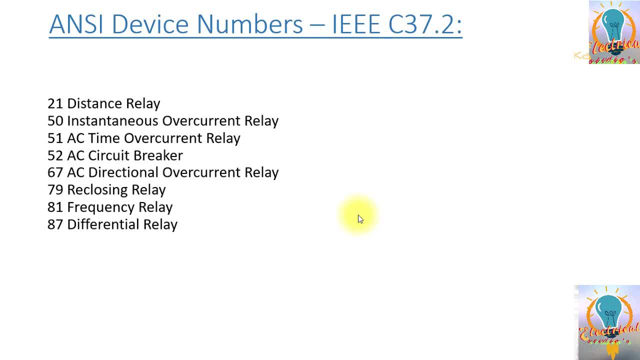 And see device codes as per IEEE CH378.. The protection devices and control devices in the substations are shown by the NC codes in the drawings, in the single line diagrams, in the three line diagrams. So it's always important and to learn these codes if you want to study. 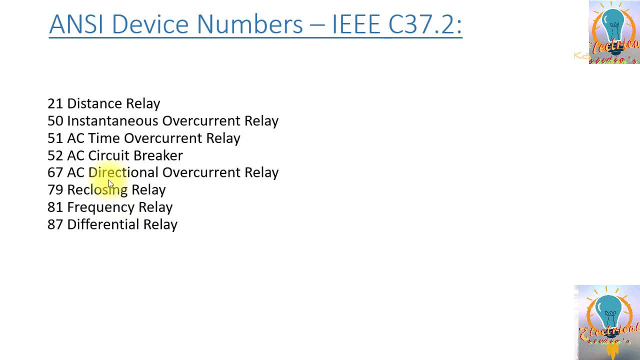 and read the drawings. So, for example, 21 is a code that is used to represent the distance relay. So 21 is a code that is used to represent the distance relay. So, for example, 21 is a code that is used to represent the distance relay. 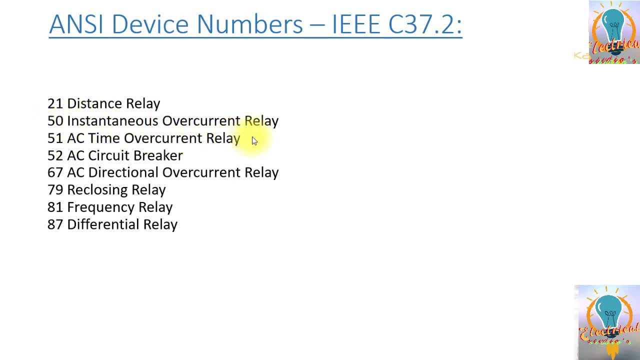 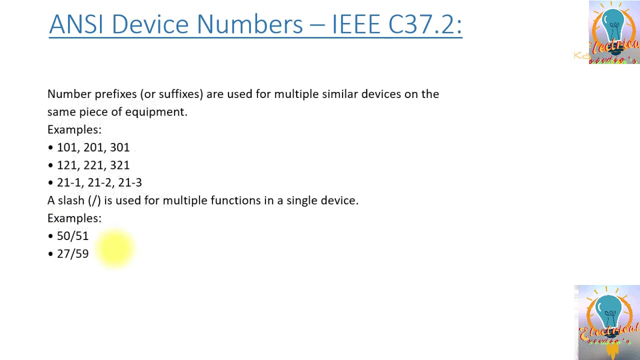 50 is the device code to represent instantaneous over current relay. 51 is AC time over current relay. 52 is AC circuit breakers. 67 is AC direction over current relay. 79 is used for auto recloser, 81 is used for frequency relays And 87 is used for differential relays. 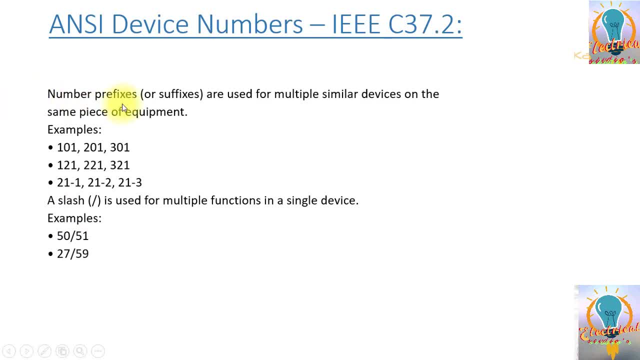 So there are some prefix or suffix which are used for multiple similar devices on the same piece of equipment. For example, you can use 101, 201, 301 and you can use, for example, 21-1, 21-2, 21-3.. It is showing. 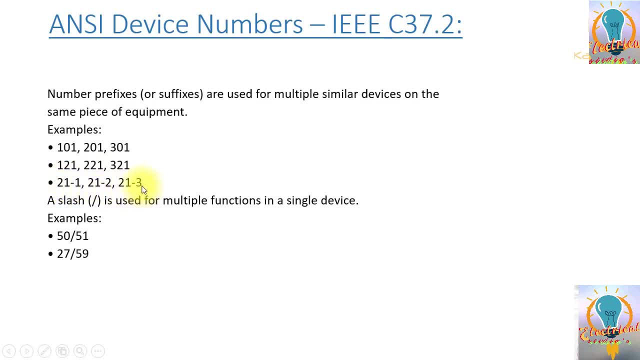 that there are three different distance relays which are installed here. So a slab is used for multiple functions in single device. For example, if a device is have the function of over voltage and under voltage, so you can use 27 slash 59. And if the device is 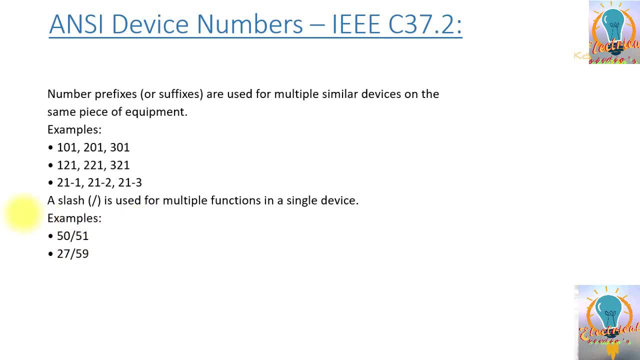 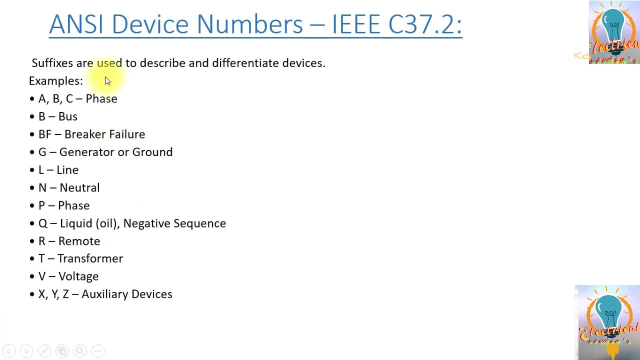 instantaneous and time delay over current. you can use 50 slash 51.. So there are some prefix suffix which are used to describe and differentiate devices. examples: ABC is used for phases, V is used for bus, BF is used for breaker failure, G is used for generator or ground, L is used for line. 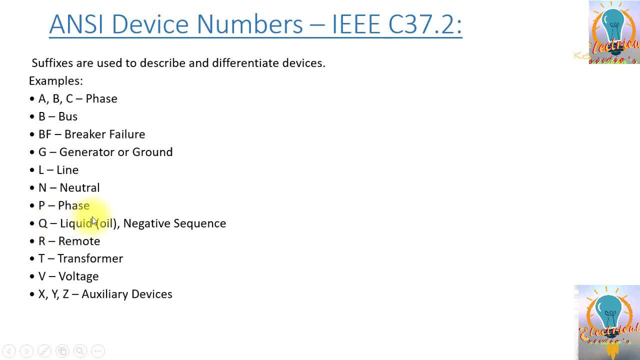 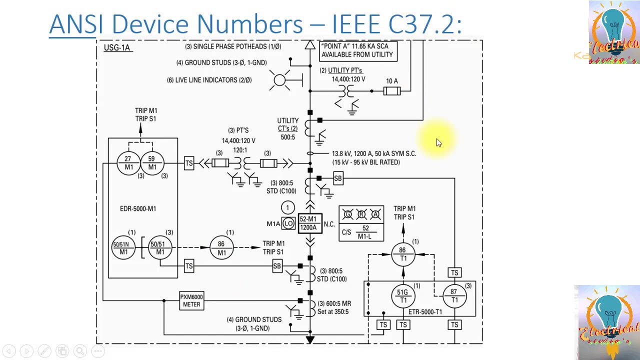 N is used for neutral, P is used for phase, Q is used for liquid or negative sequence, R is used for remote, T is used for transformer, V is used for voltage And XYZ are used for auxiliaries. This is a single line diagram, So if you 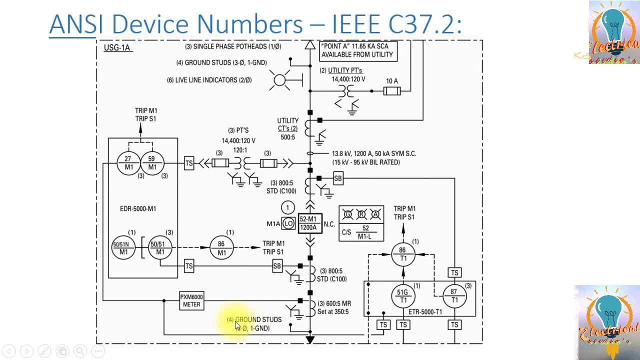 know the codes that we have recently learned. you can find out different devices in it. For example, this is basically over voltage device 59. This is basically under voltage device. Here you can find out more devices. This is the breaker 52. This symbol is showing the breaker. The rating of breaker is 1200. 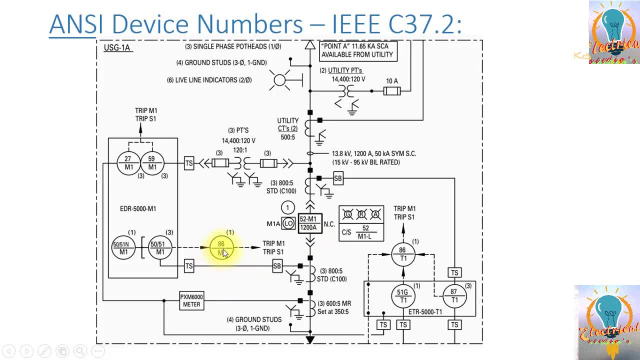 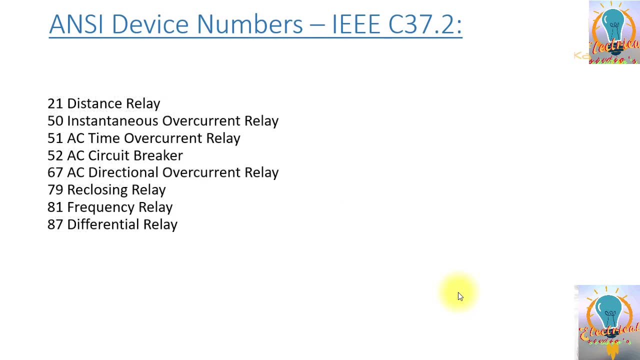 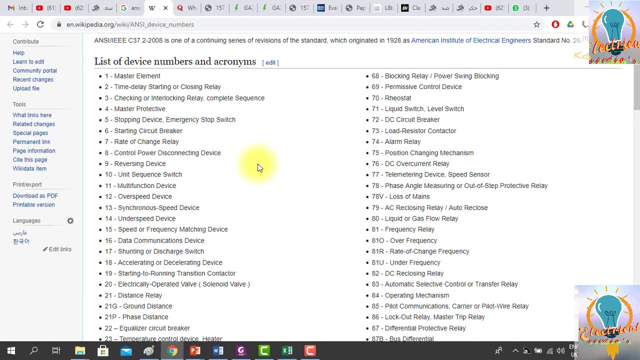 ampere. 86 is basically the lockout relay. So in the same way you can find different devices. 87 is a differential conduction And there are lot of more NC codes that you can find. You can find a complete list of NC device codes on also on Wikipedia, So you can see. 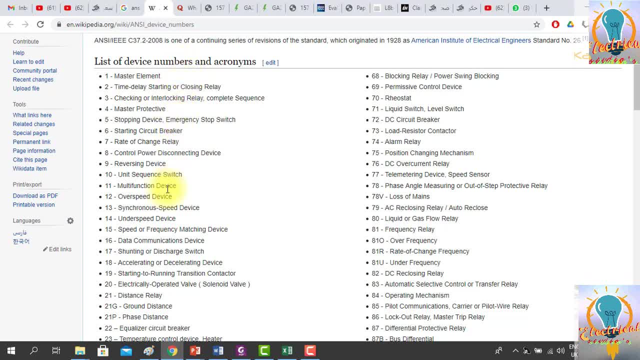 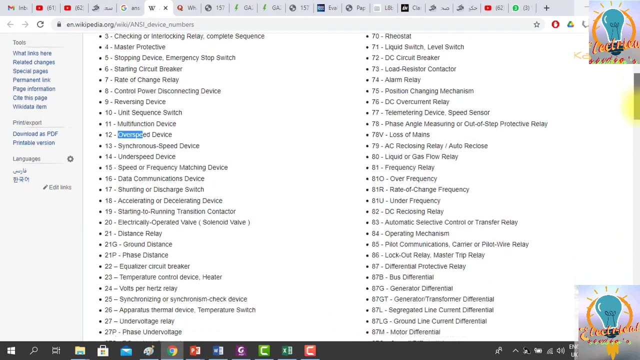 the list of different devices codes I have in my slides showing the very highly used device codes. You can find distance is 21 here, Over speed device is 12 here. So these are all kind of devices. Ground distance is 21.. 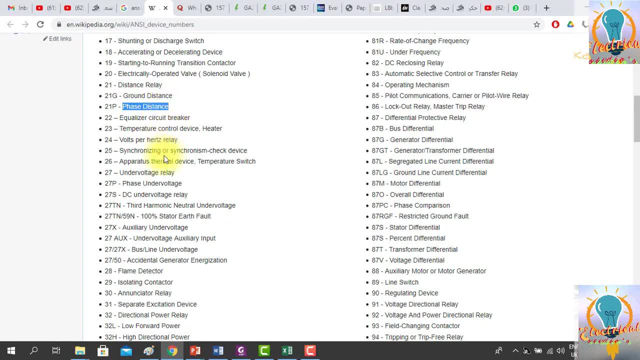 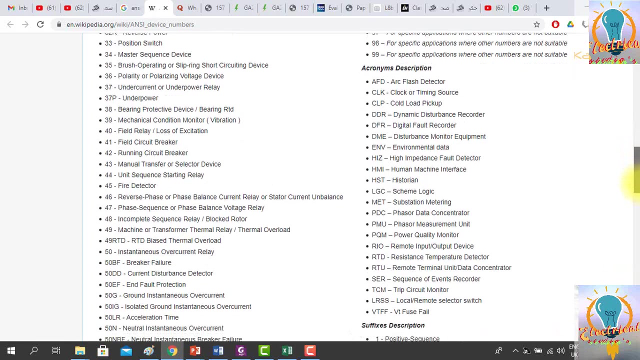 G phase distance is 21 P. for example. you can see under voltage, voltage, 27 phase. under voltage is 27 P DC. under voltage is 27 S. so try to learn this device course. this will be help you to understand the production things quickly. and here you can find some acronyms, descriptions, also like RF flash. 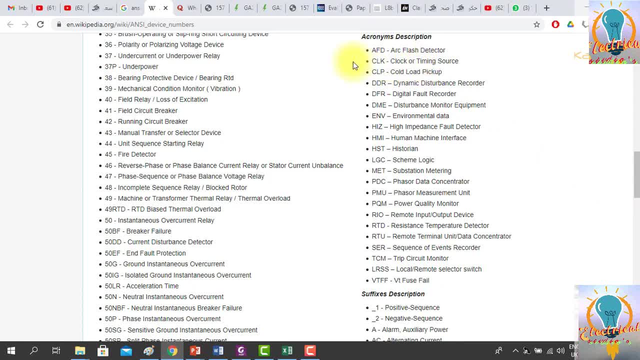 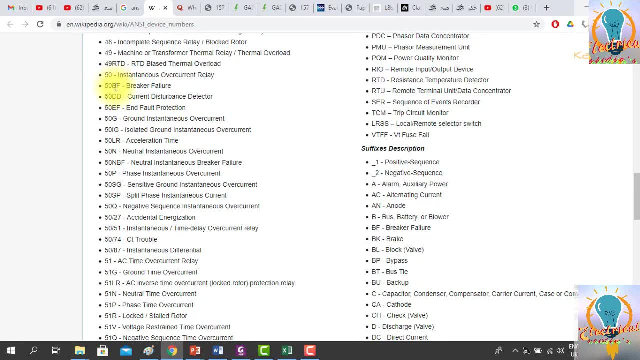 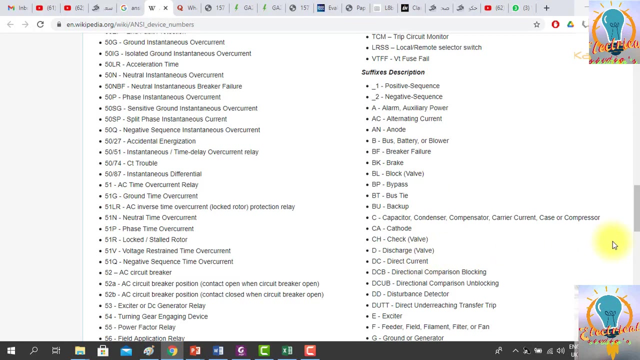 deduction: AFD, clock or timing source: CLK. so there are a lot of things that you can go and study yourself. 50 is basically instantaneous over current relay. 50 BF is breaker failure. 50 G is ground and here you can find more list of suffixes. 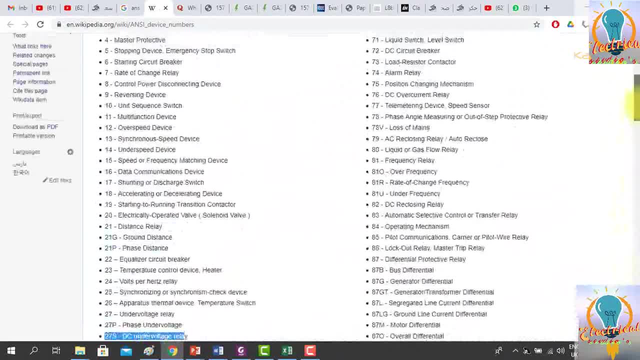 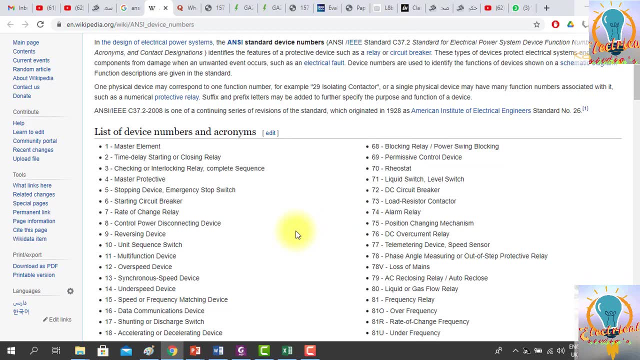 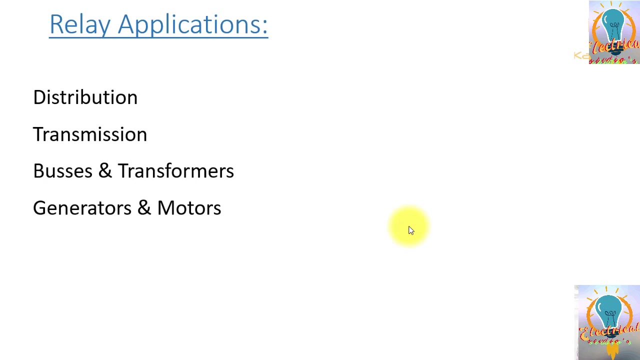 and prefixes. so this is a good example this Wikipedia is giving you all. the MC code is, as per Ikc standard, C7.2. so I hope that you enjoy this lecture and welcome to the next lecture. hey, friends, in this section we will study the relay application. we will see which type of regressionuchen. 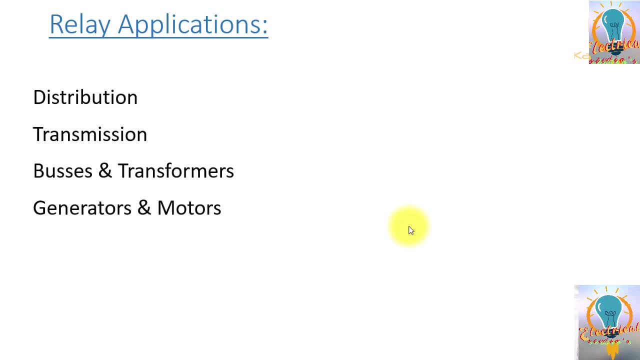 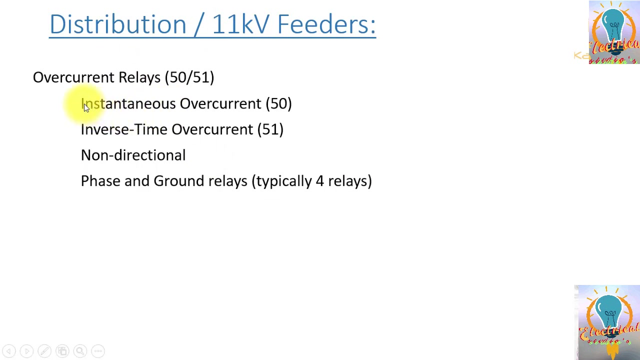 reads installed on what type of vision equipment? so you'll see what set of production screen. because shouldn't be installer distribution networks, transmission network, buses, transformers, motors and generators? so here you can see. on the 11 kV distribution feeders you will find mostly over current. 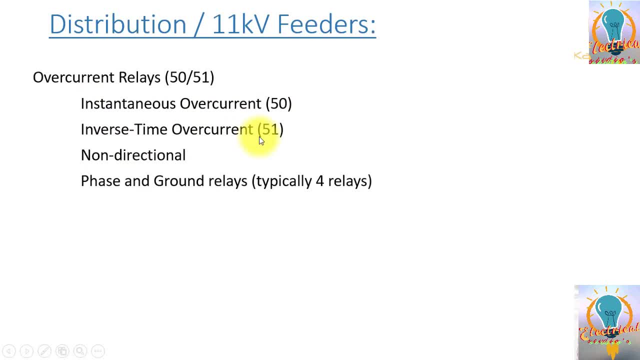 relays, instantaneous over current relay, inverse time over current relay, non-directional relays and phase and ground relays, typically four relays. and if this 11 kV feeder is connected to a source like a power plant or generation source, there you can also find the directional earth fault relay. 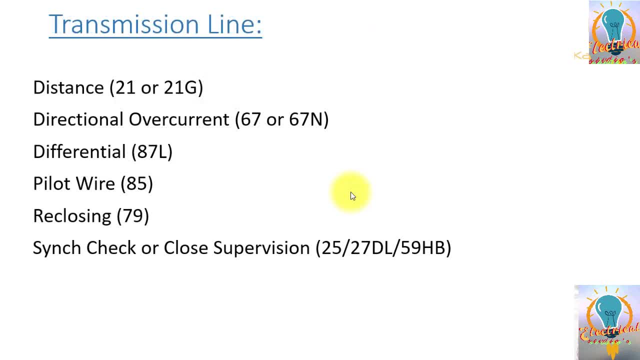 also there on the transmission line you can find a distance relay 2121p or 21g directional over current is also installed on the line. differential production relay 87l, pilot 5.0 design scheme auto recloser, sync check relays are also installed on transmission line level. 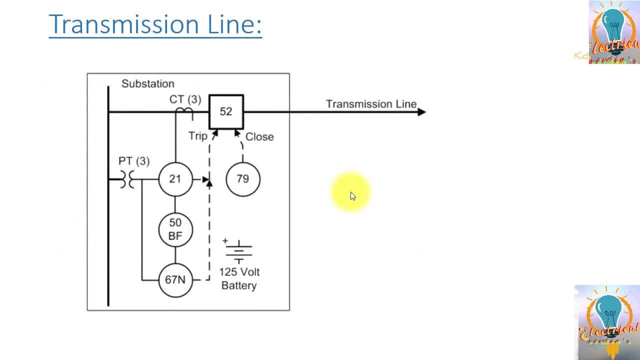 and closed supervision relays. so this is basically a single line diagram. so you can see there is a CT and there is a PT. a CT is connected to distance relay, first 21, and then it is connected to over current, instantaneous over current. there is a failure relay and then it is connected to a directional over current relay. 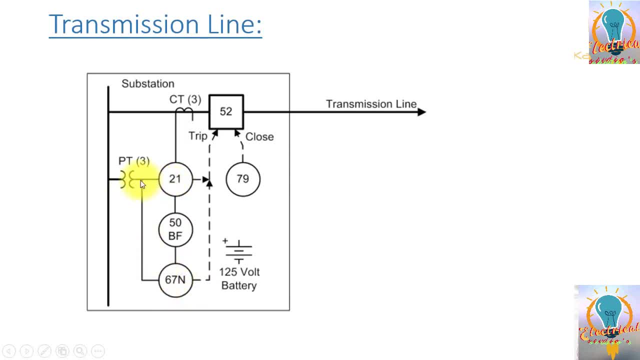 so VTE is connected to distance relay and also to the directional over control, because directional over current relay need a polarizing quantity to decide the direction of current: is it in forward direction or in reverse direction. here you can see an auto recloser and this is basically. we have shown very simple scheme. 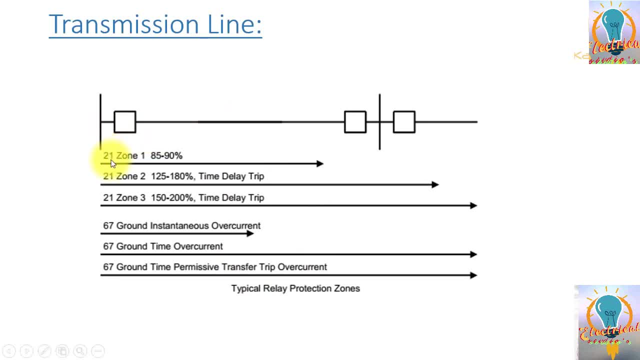 for the transmission line. zone one is taking normally 85 percent to 90 percent of the line. zone two is taking as 125 to 81- 80 percent of the next substations. zone three is 150 to 200 percent of time delay trip of the third substation. so this is basically. 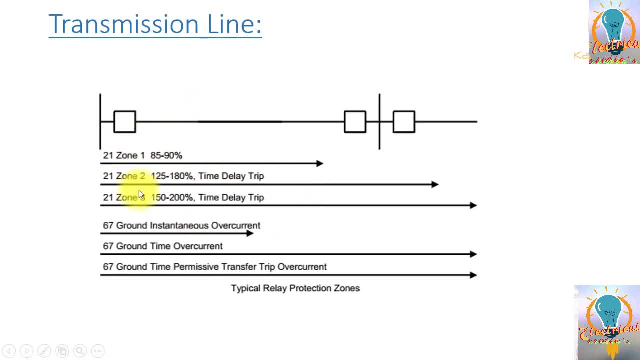 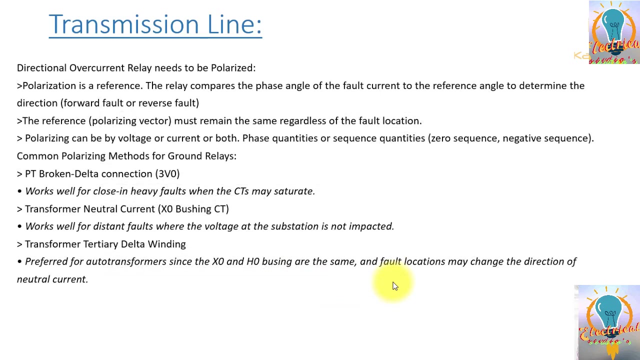 zone one, zone two, zone three. so this is basically the coverage and then for the directional over current, the ground rational over current is instantaneous and there is ground time over control also installed in it and the ground time permissive transitive is also installed here. so directional over current relay needs to polarize. polarized session is a reference. 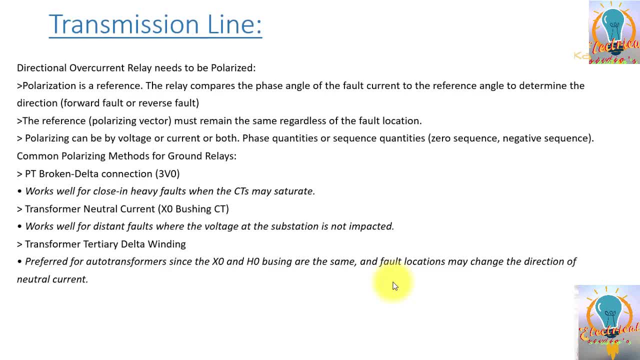 the relay compares the phase angle of the forward current to the reference angle to determine the direction, whether it's forward direction or it's a reverse direction. the reference polarizing vector must remain the same regardless of the fault location. polarizing can be by voltage, the water 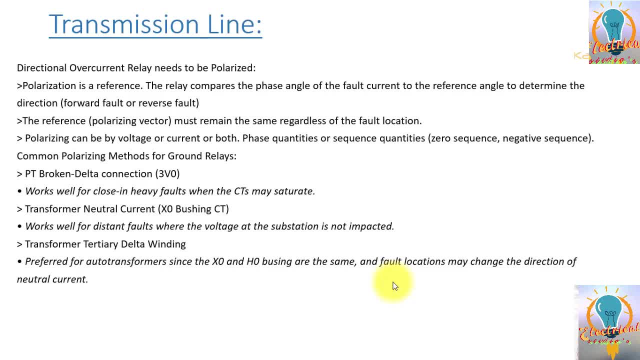 or current or both phase quantities or sequence quantities. there are some common polarizing method. one method is to take open Delta voltages- 3 V naught- and then you can work well for close in heavy faults when the CDs may saturate. transformer: neutral current X naught watching CT transformer tertiary Delta. 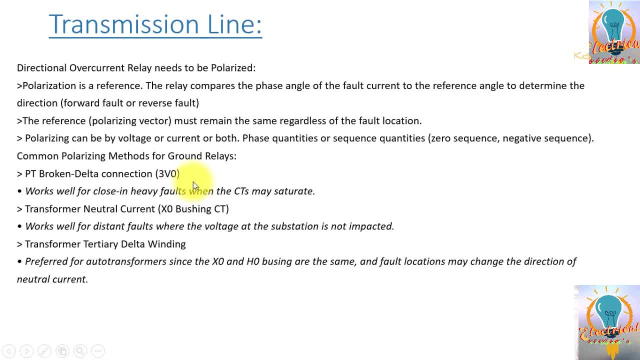 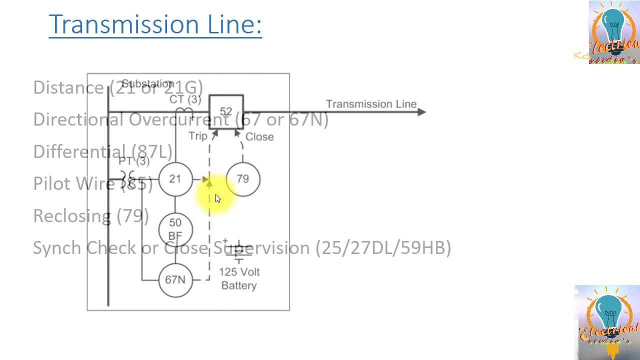 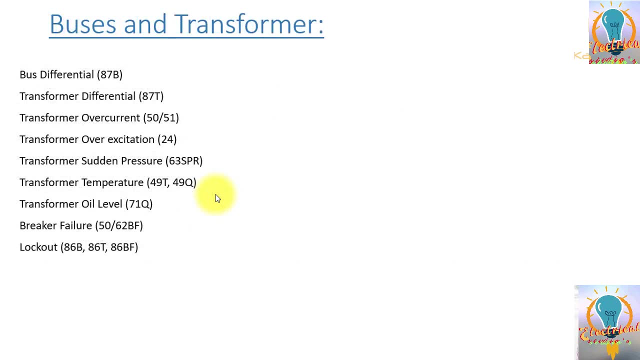 winding. so these are different polarizing quantities that you can connect to it and you can connect with the direction or spot really. then there is a bus and the transformer. so on the bus bar you will see a bus bar differential protection and bus bar differential protection is normally can. 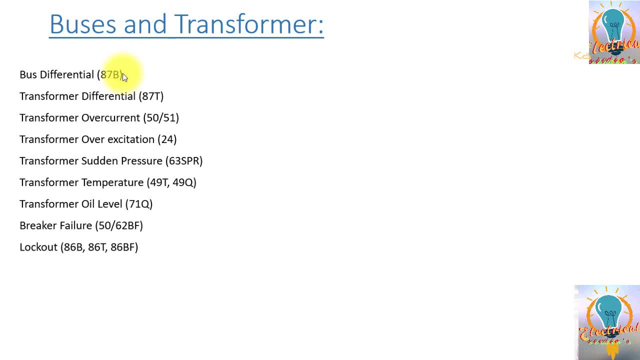 be of two types. one is low impedance bus bar differential protection. another one is a high impedance bus bar differential protection. then you can find a partial protection on the transformers. on the transformer, you all, you all, you will also find an HV overcurrent and we over current protection, as we earth fault and LV affect protection, you will. 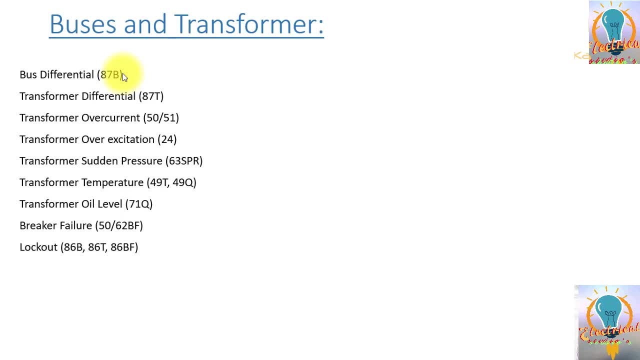 find HiSat protection or current production stage 1 and 2 on HV. and also you will find high set or competition stage 1 in 2 on lv side. you will find oil exhalation on the transformers. you can find sudden pressure protection. you can find temperature protection. 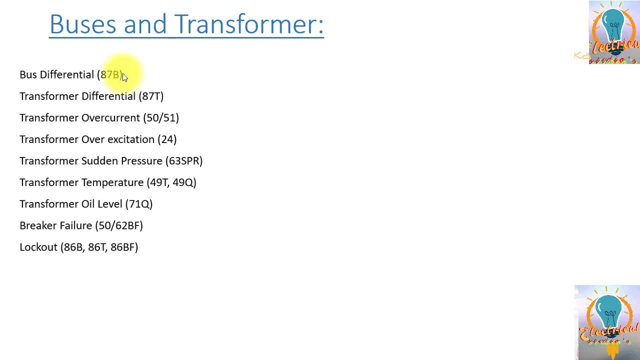 basically in the transformer winding temperature and oil temperature gauges are installed in the stage one it will run the fan group one, for example. stage two, they will run the fan group two. if also they have a forced oil cooling, then they will also start the pump. after that they will. 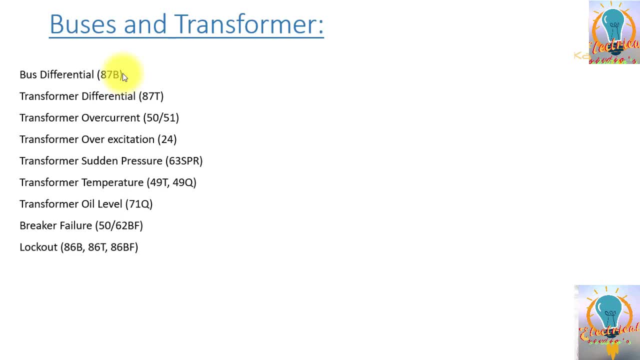 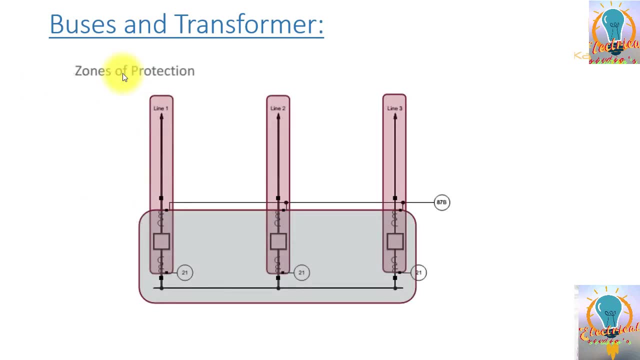 give the alarm and then in the last, they will initiate the trip. then there is a breaker failure protection, there is a lockouts. here we have shown the different zones of protection. this is basically the bus bar protection. so bus bar is covering the breaker, we and also the bus, whereas the line protection is covering 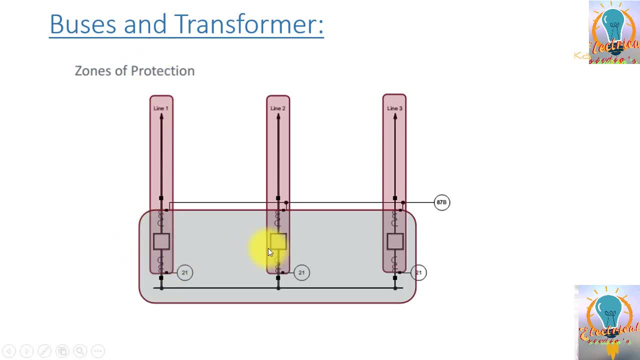 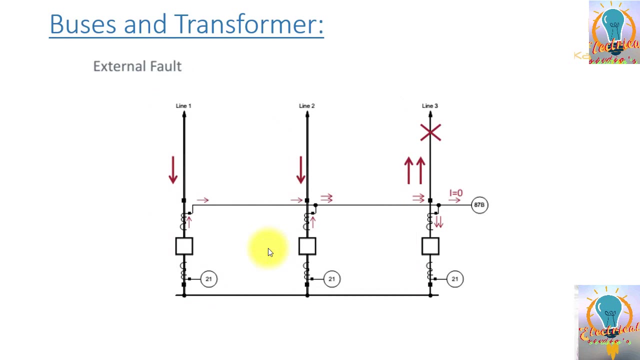 the breaker and the line. so this is always a good idea to give a to make the loop bus bar zones overlap. so all the areas in the protection system should be covered by some zone. so here, this is just an example. if there is external fault, okay, then the differential current inside the bus bar will be zero, only the line will trip. 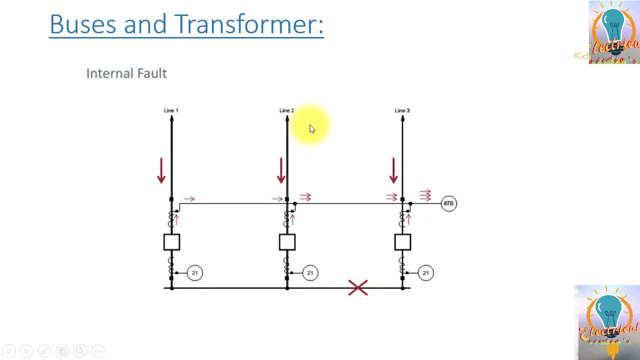 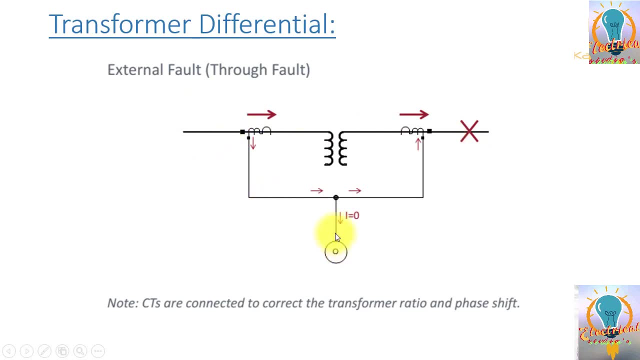 and if there is internal fault then bus protection will operate in the same way you can see. if there is external fault on the transformer, differential protection, current in and out will be same. so there will be zero differential protection, there will be zero differential current and the transformer differential will not operate. so if there is an in zone fault, 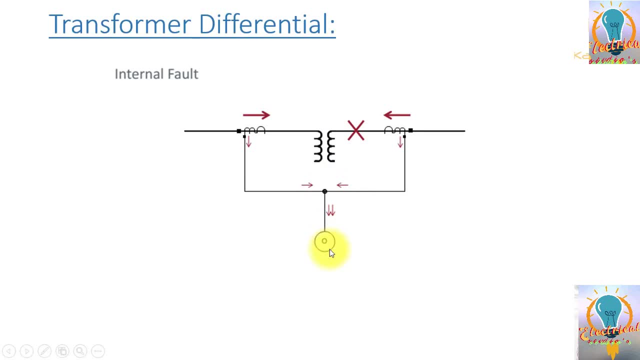 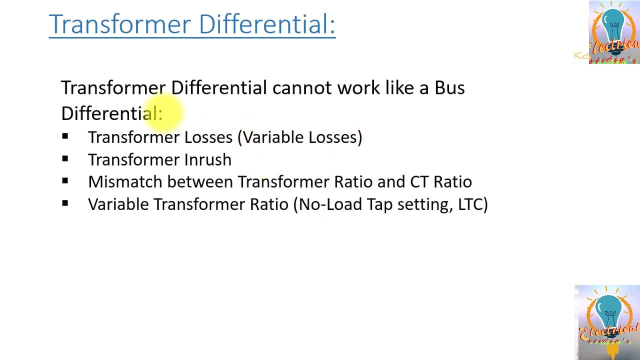 so you can see the both current will add up, differential current will be high and then the bus and the differential protection will operate. so transfer differential protection cannot work. like you can see in this picture, the skimmer, the bus bar, needs a little bit more adjustment because essentially it should not disturb due to absence of the bus bar change. 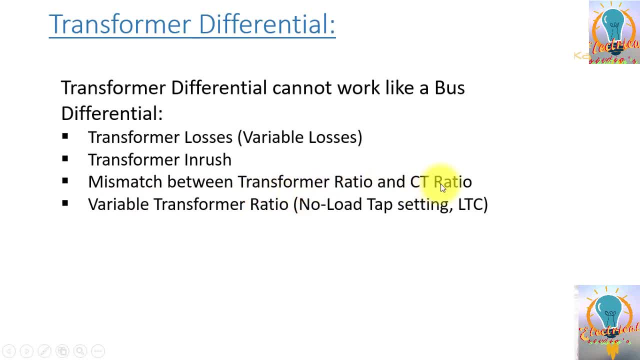 and it is actually font production from wireless to wireless, but in this case you can see that, however, this one is based on the weight and power clarity factor. so, for the different production of the bus bar, because there are some losses in the transformer, there is a transform and ind garage, there is mismatch between transformer ratio and cts on hp and rv side, and there is also tape changer winding, which is normally 10, which is also including error. so all of these things are contributing to design special differential transformer protection so that так怎么. 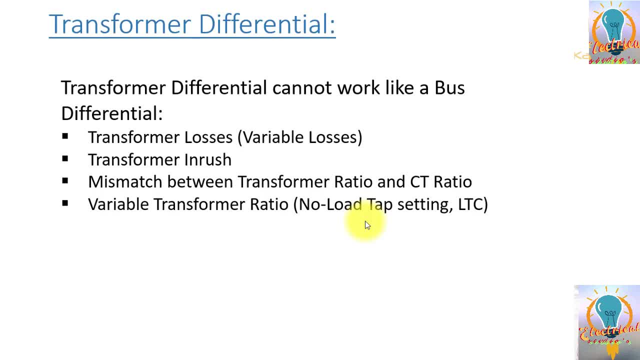 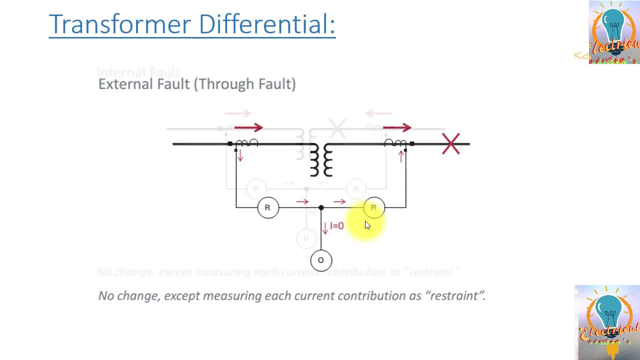 in this one we have to keep a slope at a higher value. We also have to take care of inrush. There is blocking due to inrush in this transformer differential. So on the generators and motors: in the generators and motors you can see: 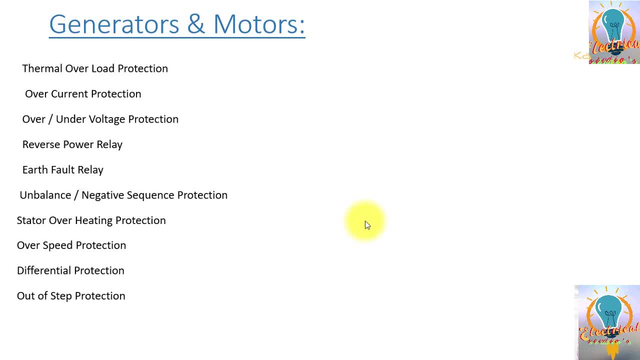 thermal protection is installed over. current protection is installed over and under. voltage protection is installed. reverse power relay is installed. earth fault relay is installed. unbalanced and negative sequence protection is installed. stator overheating protection is installed over speed protection differential. 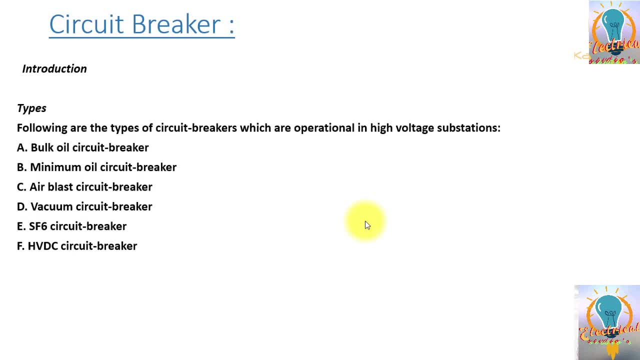 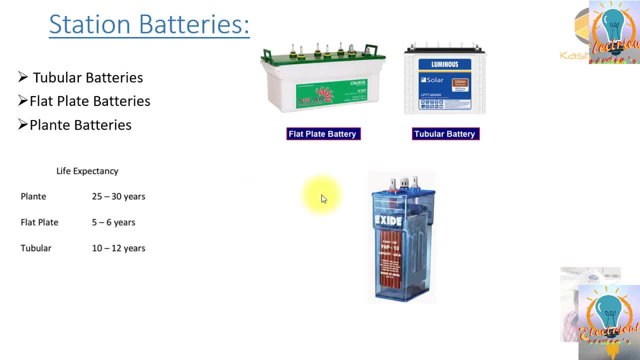 protection out of step protection. So these are all the examples of the protections which are installed in different type of equipments. Thank you very much. Hey friends, the batteries can be classified into three different types, based on the plate which are used in the batteries. 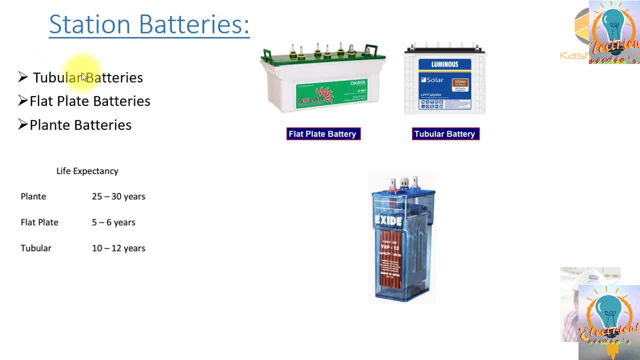 Three types could be tabular batteries. In this one, the type, the battery plates are in the form of tubes. Then it comes to flat plate batteries. The flat plate batteries are where the basically anode and cathodes are in the form of basically. 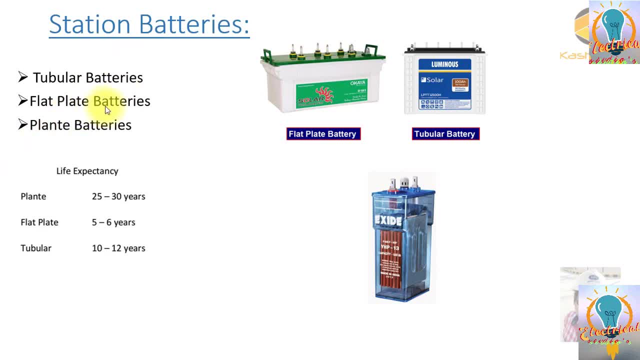 plates and in which you will see the square boxes And then planted batteries. So these are plant batteries And these are planting batteries are basically the initial, very initial form of batteries in which cathode and electrodes are basically rods, selectable rods. 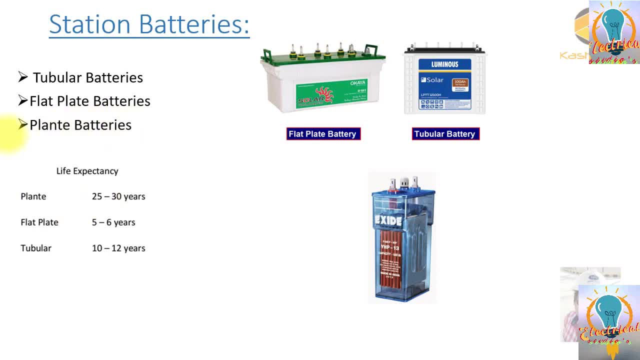 And in between the insulation was used to be placed. So the life expectancy of these batteries- planted batteries- is 25 to 30 years, Flat plate is 5 to 6 years and tubular is 10 to 12 years. So this is basically. 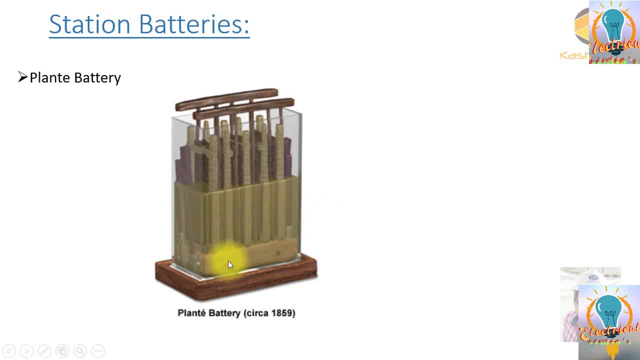 OK, Thank you, Mr. This is basically the example of Plantet battery and this is one of the very old batteries that were invented, and this is the picture of battery that was invented in 1859.. This battery was invented by a scientist named Gaston Plantet and this is one of the first. 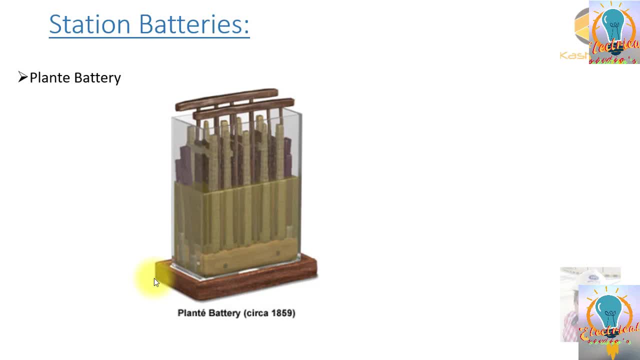 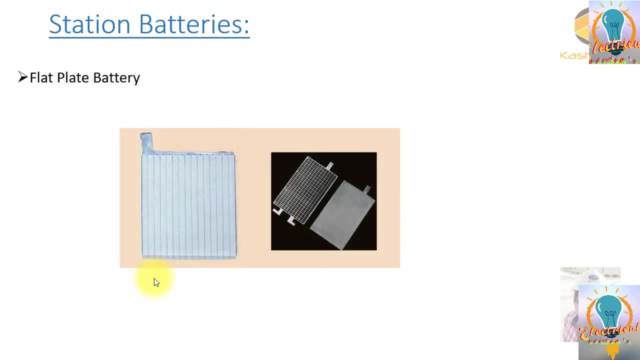 battery, even of its kind, and the invention year was 1959. So this is one of the very initial batteries. Then it comes to flat plate batteries. You can see the battery anode and cathode structure. It is in the form of flat plates and you will find these batteries mostly now in the cars. 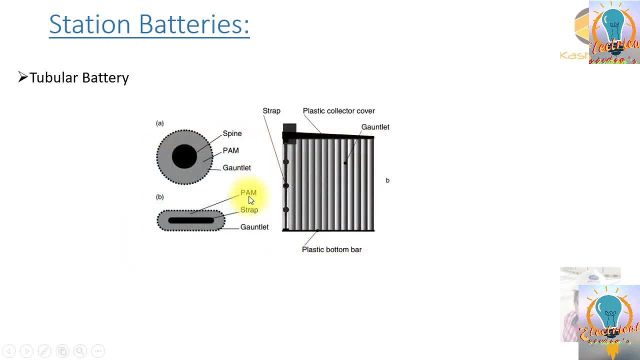 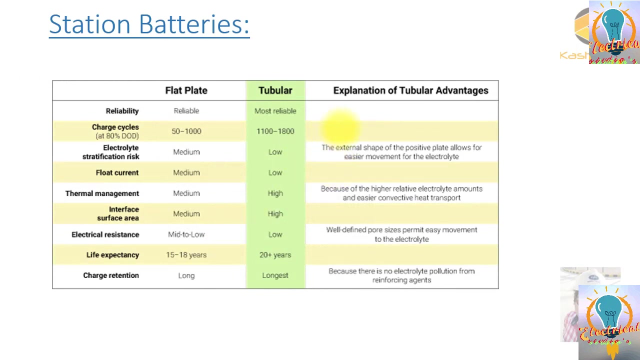 electric cars. Okay, And this is basically tubular battery system in which the anode cathodes are in the form of tubes, and these are very, very reliable and these are deep cycle batteries. Here is some comparison of the flat plate and tubular batteries. 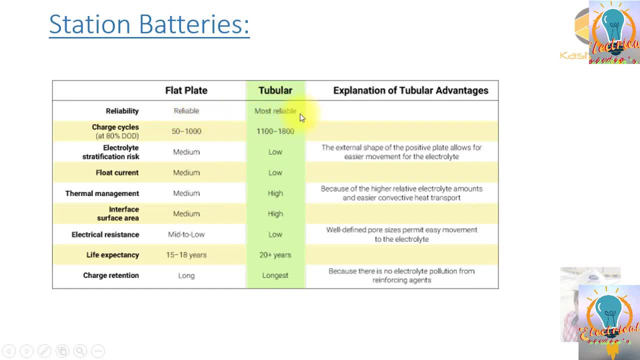 You can see reliability: Tubular are more reliable and also tubular battery is more expensive. Okay, You can see charge cycles. So clearly the tubular batteries have bigger and more reliable charge cycle. And then electrolytes stratification risk is medium. 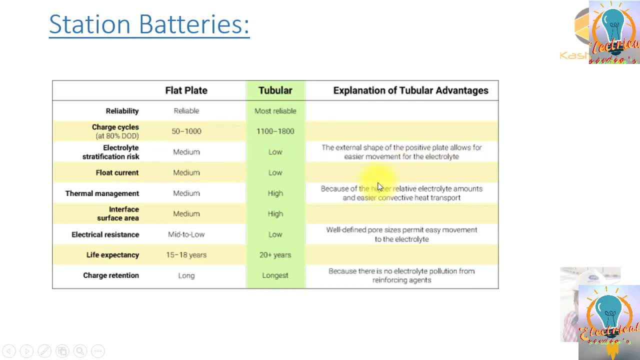 Here it's low because external shape of positive plate allows for easier movement for electrolyte Float current here is medium and the float current here is low, so it's less burden on the charger. Thermal management is medium And the tubular batteries are more reliable. 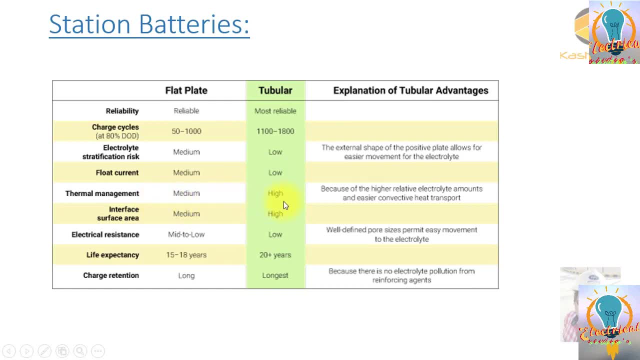 You can see charge cycles Here it's medium and the tubular thermal management is high. Because of construction, this tubular battery will not heat up as quickly as the flat plate battery. Surface area is medium and surface area is high. Electrical resistance is mid to low and here the electrical resistance is low. 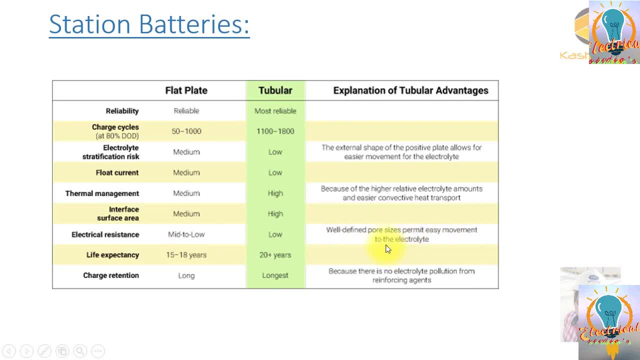 Why? Because well-defined pore size permit easy movement to the electrolytes. Life expectancy of tubular is more than the flat plate. Okay, Charge range in the flat plate is long, but in the tubular is its longest because there is no electrolyte pollution from reinforcing agent. 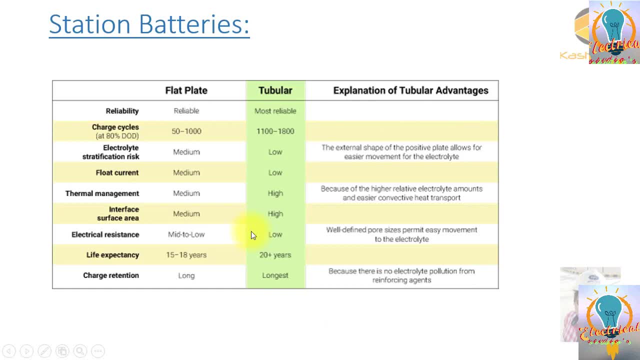 So this is a little comparison of these two batteries. So I hope this has given you an idea And on the stations mostly you will see the tubular batteries which are deep cycle and which are more reliable. Thank you very much, Thank you. 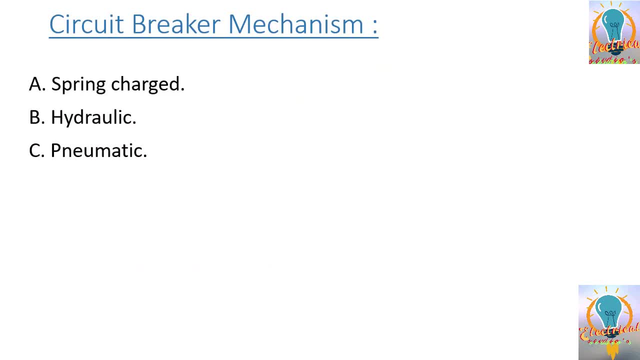 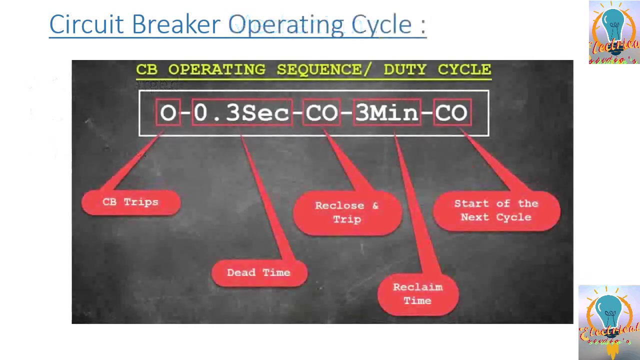 Bye. Thank you very much. Hey guys. now we will discuss here this different type of circuit breaker mechanism. So there could be three different type of mechanism. One is spring charge, one is hydraulic and one is pneumatic. So these are three different type of mechanisms which are used. 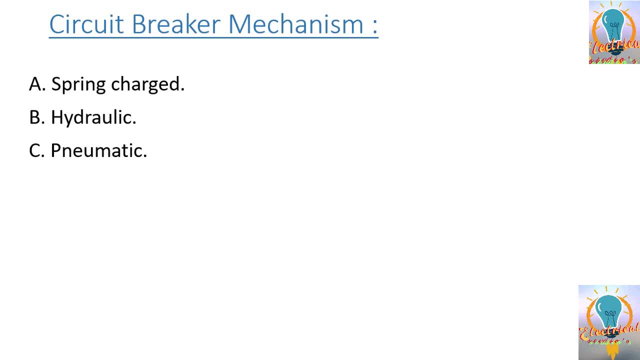 Initially the spring charge was created for up to 132 kV now, but you can see the spring charge is also used, So you can see that up to 500 kV they have created. spring charge is basically mechanism, is very maintenance free or most maintenance free, and it is really cost effective solution. 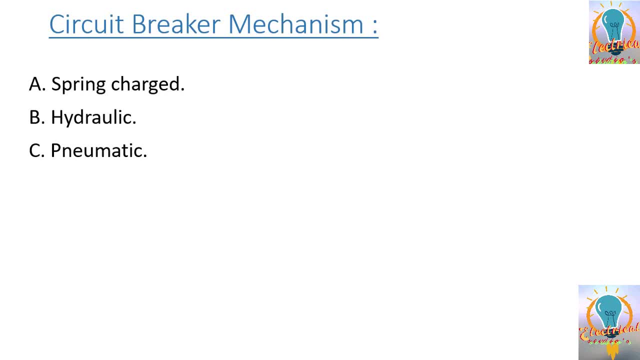 Hydraulic mechanisms. initially, when the spring charge was not established, hydraulic mechanism was used. but hydraulic mechanisms have the disadvantage that you need to create constantly a high pressure to be ready for to break out the trillium. Okay, Okay, Okay, Okay. Yes, this is the second one. 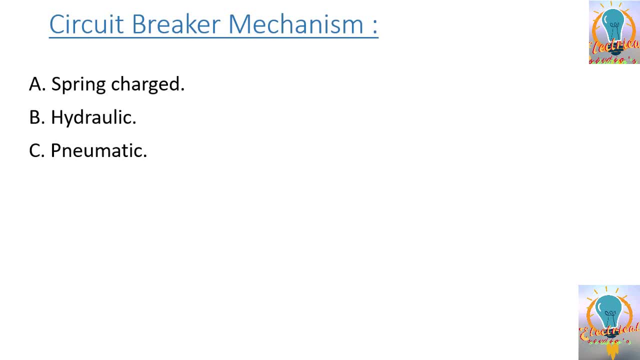 First one is the pneumatic mechanism. So this is also a pneumatic mechanism. You will see the pneumatic mechanism in the circuit breaker name plate. So you can see in the circuit breaker name plate there is a lot of leaky issue of leakages. 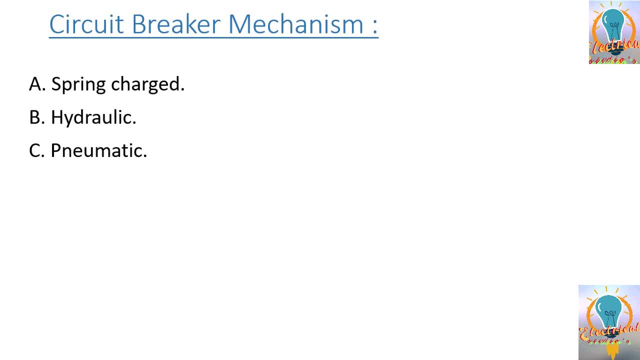 in this mechanism. So that is not preferred now. The third is pneumatic mechanism. So this pneumatic mechanism also with the high pressure of air this breakers mechanism used to operate, but also this is now less likely to use because of high maintenance. 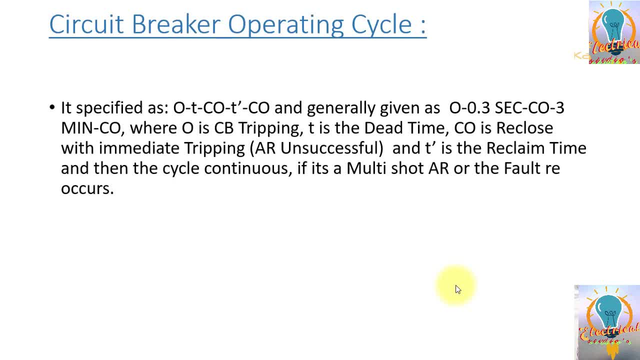 costs. Hey friends, When you see the circuit breaker name plate you will see circuit breaker operating cycle details like open, close, open and close, open, and in between you will see the time. so I will try to explain here what's the meaning of this basically. 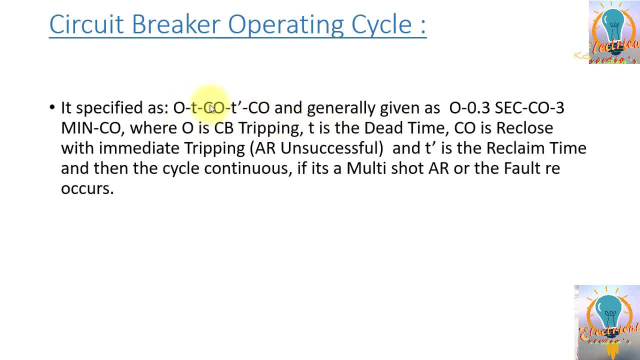 this type and we will see that. you can see it is specified as open time, close open time and close open and generally you will find this data on the nameplate of the circuit breaker: 0 open, then there is a time delay of 300 milliseconds, then close open and then 3 minutes so, and then you can again close open. so 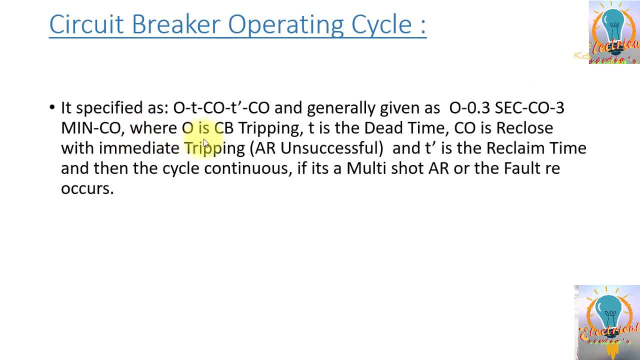 this is basically in the opting cycles where O is circuit breaker tripping, T is a dead time and C is a reclosed time. C is a reclosed with immediate tripping here successful and T is a dead time, T is a reclaim time and then the cycle continues. if it is a multi-shot error or 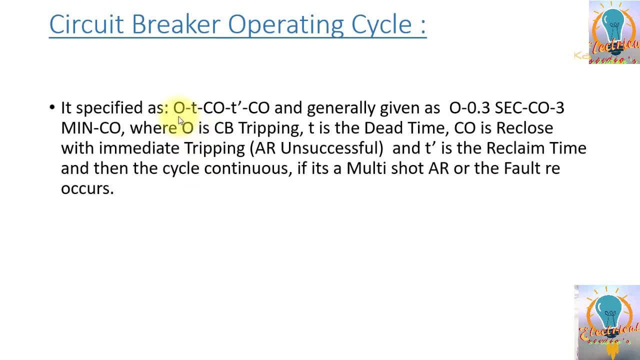 fault reoccur. so when you are doing commissioning, sometime manufacturers- or sometimes client, is also asking to measure this opening cycle of the breaker. so first of all breaker is tripped, then it is given a delay of 300 milliseconds, then it grows again and then trip again. then it's given three. 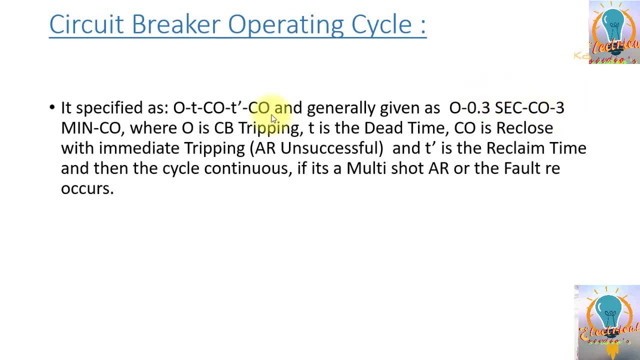 minute second, which is for reclaim time, and then it is closed, open again. so 300 millisecond here delay is considered for the dead time and the three minute is considered is for the reclaim time. and now, what is a dead time and what is a reclaim time? dead time: when there is a fault, arc will form and breakers will. 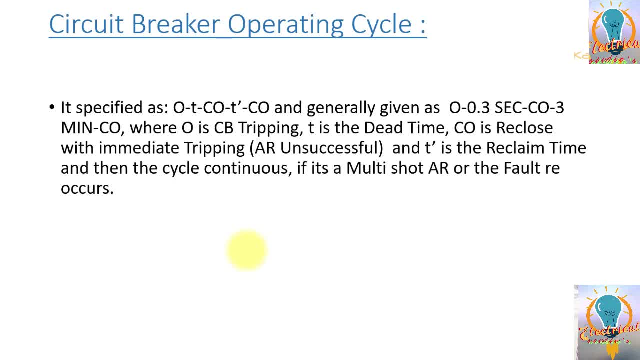 take some time to quench the arc and isolate the line. so this time they have given 300 milliseconds so protection system to operate and quench the arc if we want to close it again before the arc is extinguished. it mean that if arc is extinguished we want to reclose the. it mean the fault is persist. 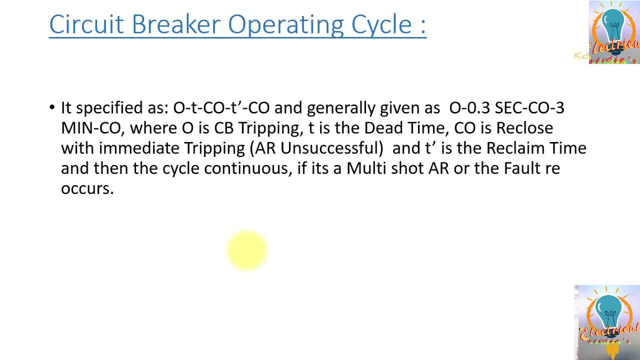 persisted because arc has a low impedance and it has a low resistance. if you are trying to close in the breaker again, reclosing if the arc is not extingbish, it mean that you're closing it again or do a fault so, and then it's closed again after dead time. arc is. 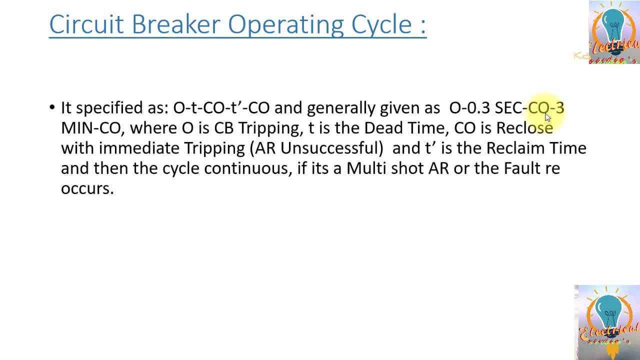 extinguished, it's closed again and then, for example, strip again because of the fault said. then it's given a reclaim time of three means like three minutes. so in three minutes it will check that fault is not come back and then again that fall is not come back, and then again, after reclaim time, will check the. 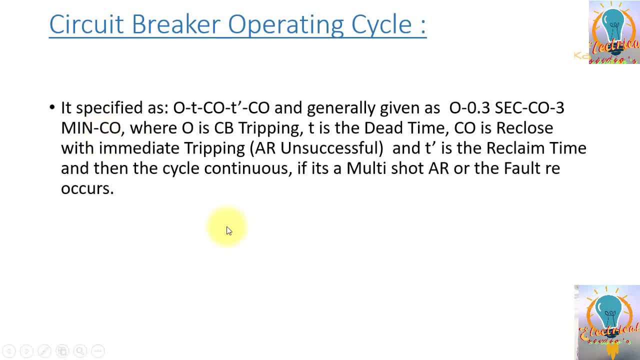 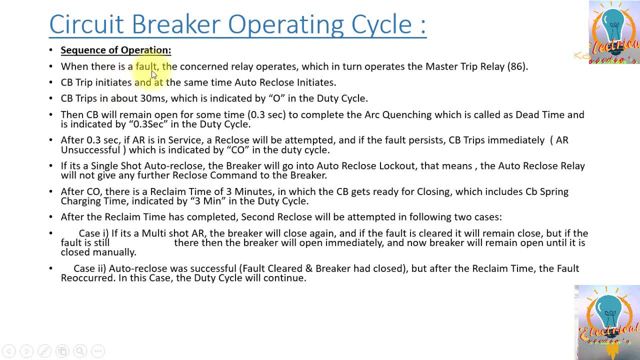 time we have make a closed open cycle. so let's go to this sequence one by one. when there is a fault, the connect concern relay operates, which is in turn operate the master trip relay, 86 circuit breaker trips initiate and the same time artery closure initiate. so there is a fault on the line relay operate the 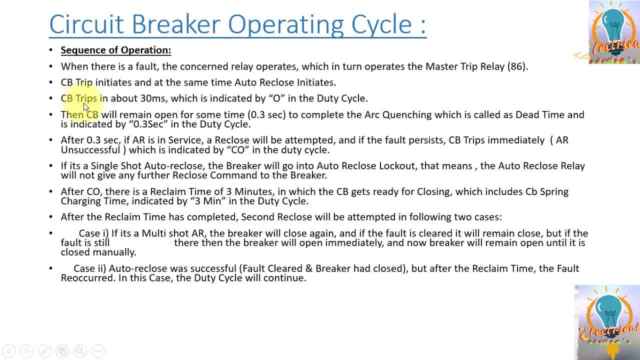 tripping and it is also initiate the artery closure. CD trip in about 30 milliseconds, initiated by open in the duty cycle. so circuit breaker will trip approximately 30 to 50 milliseconds between that open cycle has started. then circuit breaker will remain open for some time, that is 300 millisecond to 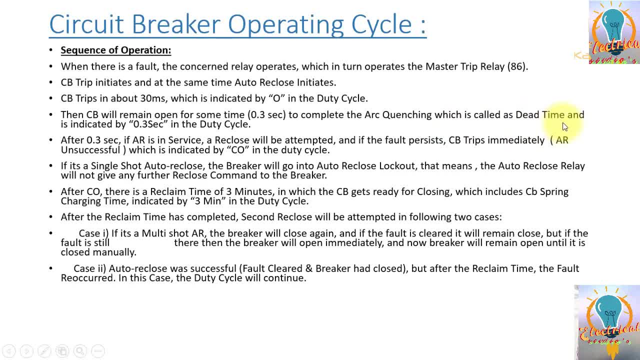 complete the arc quenching which is called as dead time and is indicated by 0.3 seconds in the duty cycles. so 300 millisecond will be given for arc to quench and it will be shown as a duty cycle of the breaker. after 0.3 seconds, if the air is in service, our recloser will be. 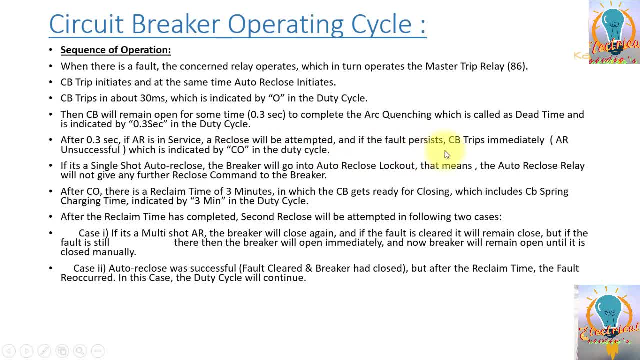 attempted and if the fault persist, circuit breaker immediately. circuit breaker immediately which is in operate and circuit breaker trips immediately which is indicated by CO in the duty cycle. so we have that after dead time AR was in service and the AR has initiated the reclose which is shown by C here, but the fault were persisted so it is open again. if 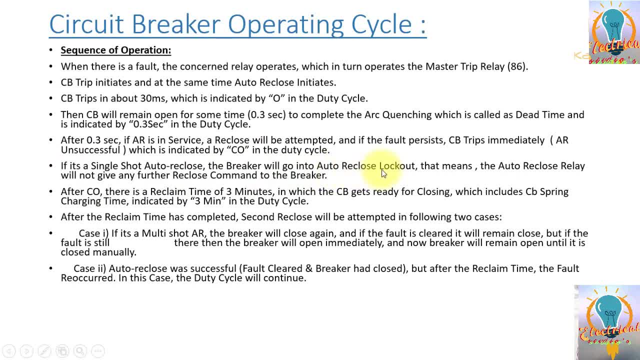 it's a single shot. auto-closure breaker will go into auto-closure lockout. that means auto-closure relay will not give any further reclose command to the breaker after close open. there is a reclaimed time of three minutes in which the circuit breaker gets ready for reclosing, which includes CB spring. 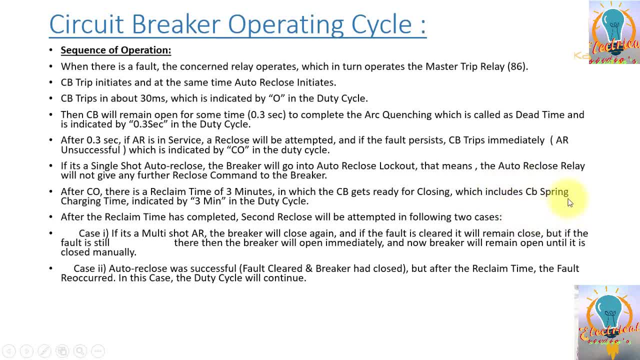 charging. so it has to recharge the spring within this time indicated by three minute in the duty cycle after the reclaimed time has completed. second reclose will be attempted in following two cases. case one: if it's a multi-shot AR, the breaker will close again. if the fault is clear, it will remain closed. but 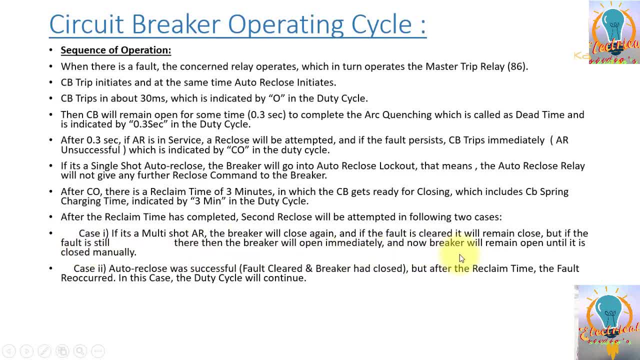 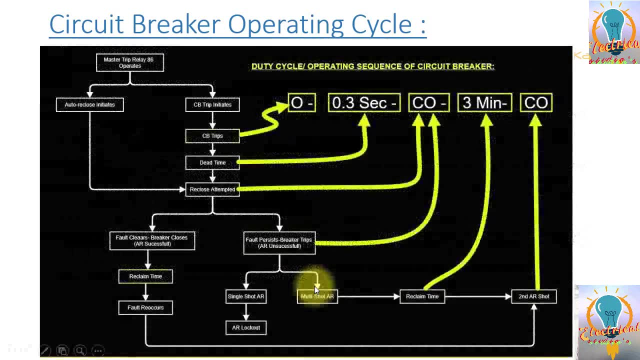 if the fault is still there, then the breaker will open immediately and breaker will remain open until it closed manually. auto-closer was successful fault clear. breaker had closed, but after the reclaimed time the fault recurred. in this case, duty cycle will continue. so this is basically the duty cycle again. so this is I have shown you. 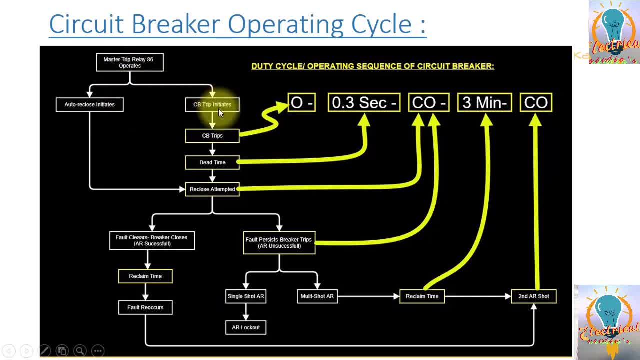 by a graph, for example, the protection relay operate and the protection relay will trip the circuit breaker. so you can see it operates and trip the circuit breaker at the same time it initiate the auto-close. after the dead time of 300 milliseconds, auto-closer will attempt breaker reclose. so this is that. time of 3 minute second has passed. 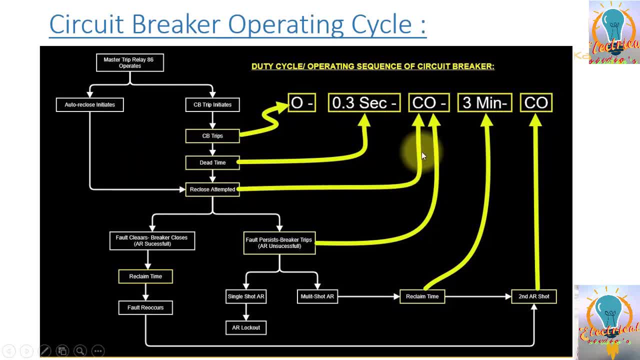 after that are: people will attempt to reclose. the breaker give the closing command. so now, if the fault is persisted, then the breaker will trip immediately. ok, and the breaker will trip immediately, and that is normal. the breaker is stripped, now the breaker will. the reclaim time will start, which 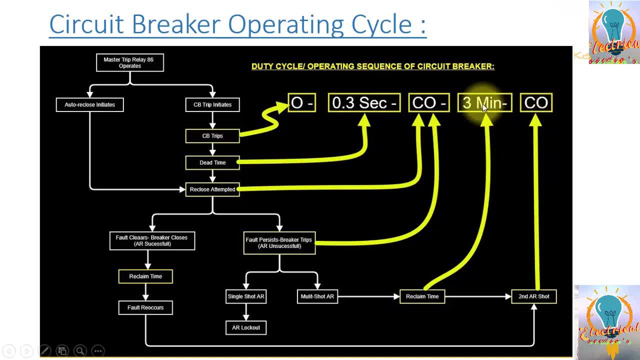 is three, three minutes. in this reclaim time, breaker will be ready to and to go for for another reclose cycle. this reclaim time defined by manufacturer- normally it is three minutes. in this three minutes recalls breaker spring will be charged. so after these three minutes, after recloser again will give. 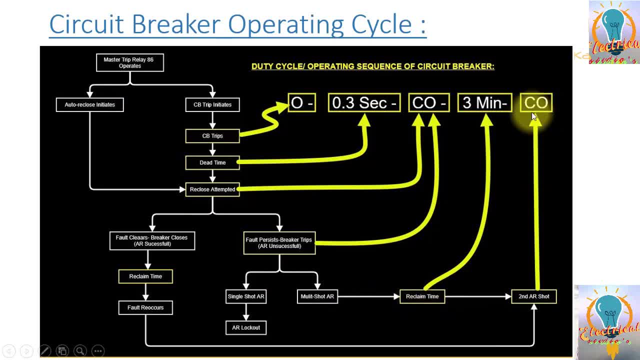 another close command and if the air is successful, recovery remote remain close and if air is not successful, the breaker will open and again the another reclaim time will start, depending upon how many shorts are designed for the system. so in the order of blizzard, really, you can set this dead time in reclaim times, but you 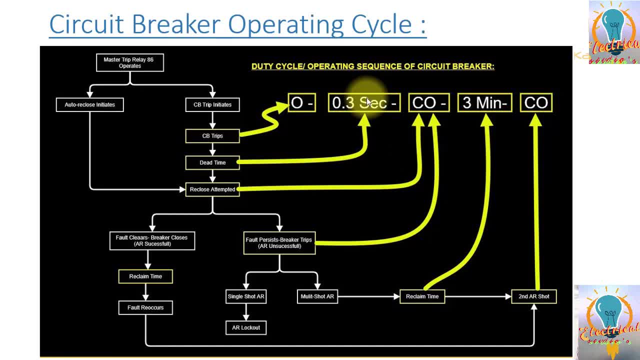 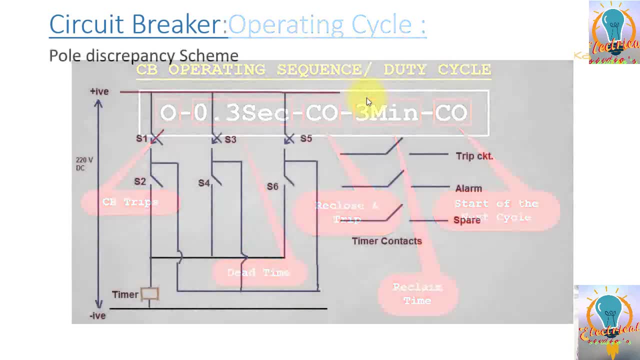 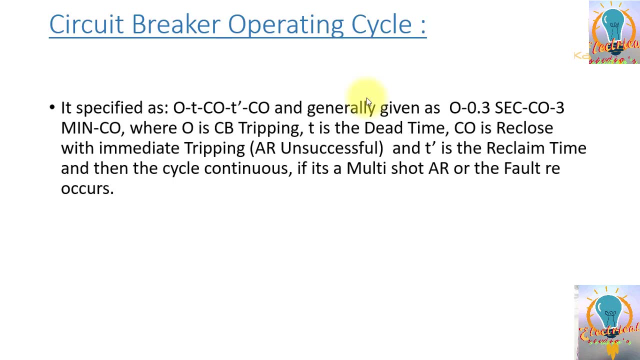 need to check the circuit breaker name plates. what are the recommended dead and reclaim times of that specific circuit breakers? we should be in line with that. so again here, I have shown you this circuit breaker duty cycle. so this was some brief discussion about the circuit breaker duty cycle. I hope you enjoy this. 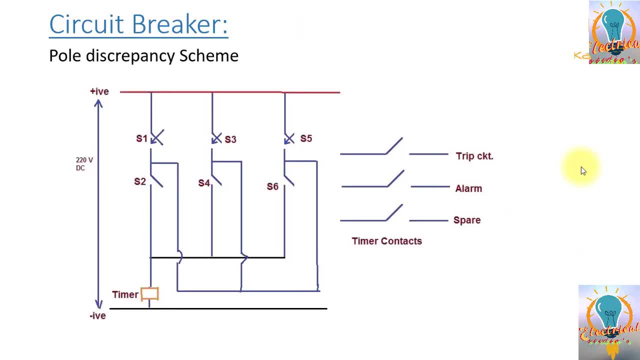 lecture. hey friends, we'll start just a brief new topic about the pole discrepancy. what is a pole discrepancy in the production systems? a pole discrepancy is basically is is a timer relay which is installed in the circuit breaker where each pole has a separate mechanism, operating mechanism. this is normally at 220 and 500 kV voltage levels. mostly what happened just 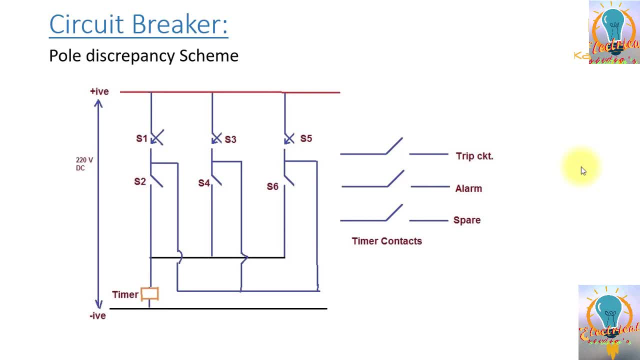 consider the case that there are three phases: a, B and C. if one of the phase for will phase a fail to close and two phases, two poles, are closed, this, this is basically abnormal condition and this has to be monitored. so, basically, this monitoring of this is done by a timer. 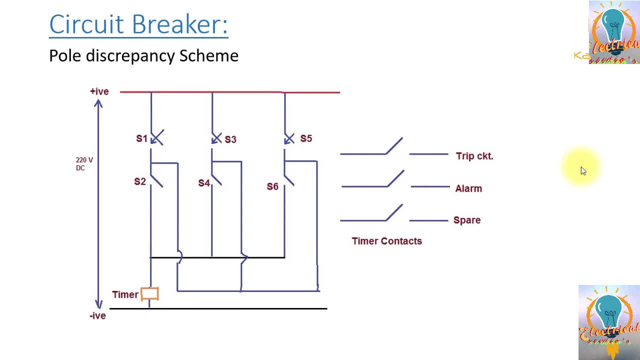 timer checks. basically all the contacts of the breaker should be open or closed. if one of the contact is stuck up, a scheme is fired up in such a way that the timer will start and timer will in stage one is called as hold discrepancy timer, so timer in stage one will try to re-trip the breaker. 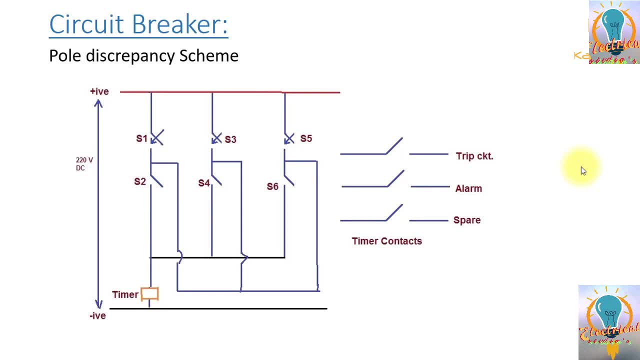 tip coil one and two and still, if it's not clear, then in stage two it will operate the breaker, failure protection of this specific breaker so that it should isolate this breaker from the system. so you can see this. basically, i have shown a basic scheme. this is a timer and they can put. 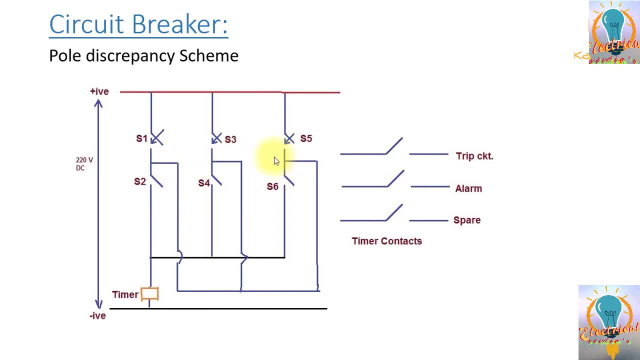 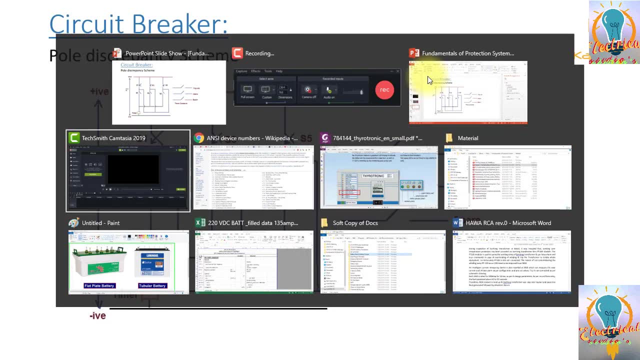 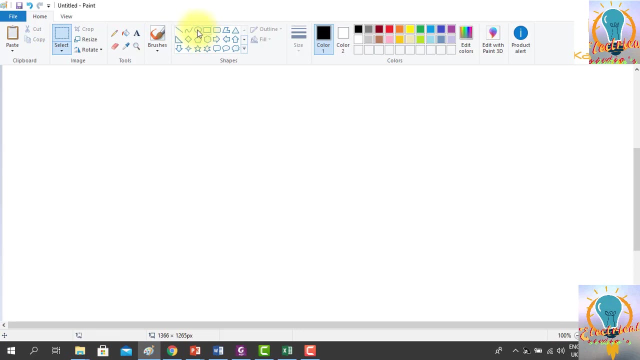 this contacts in series like this. so let's draw this scheme. let's draw this scheme here. so, in order to draw this scheme, we have two sets of contacts. let's make two sets of contacts so. so We will install a timer relay here and we will supply this relay with negative. 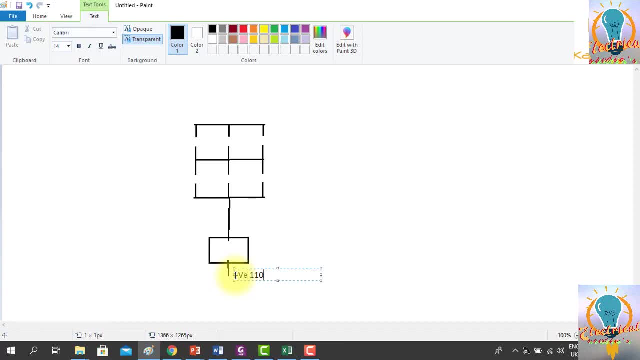 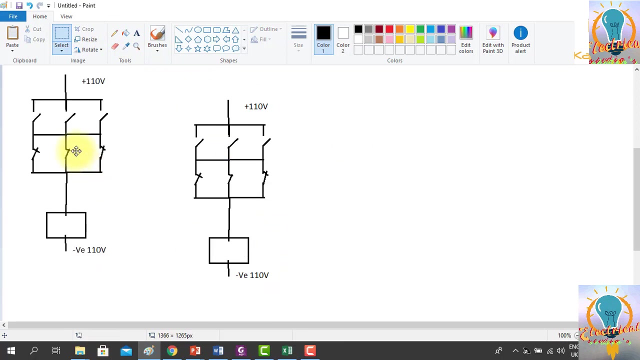 And on the top we will supply here this circuit as plus 110 volts. Okay, now we will make one contact as normally open and one contact as normally closed. This is normally open contact. These are normally closed contact. Okay, So this is the condition of contact when breaker is, for example, open. 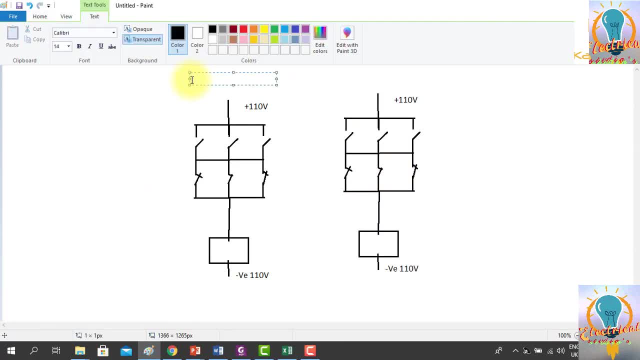 Here the breaker is open, CB is open. Here we want to, we will give command the breaker to close. So this is basically phase A, This is phase B, So here, and this is phase C, So similarly we have phase A and B and C here. 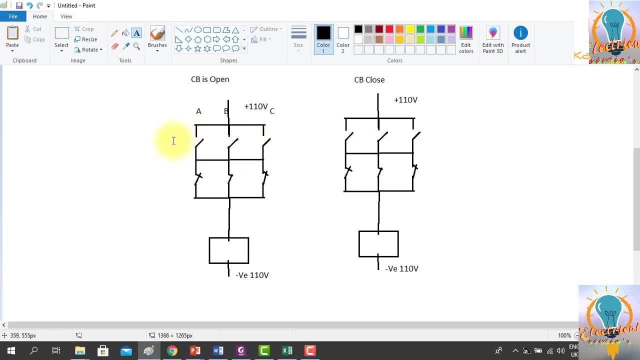 So if breaker is open, all the phase normally open contacts are open and all the normally closed contacts are closed In the same way if the breaker you want to close it. for example, two poles are healthy: A and B, B and C are healthy and A pole is stuck up. 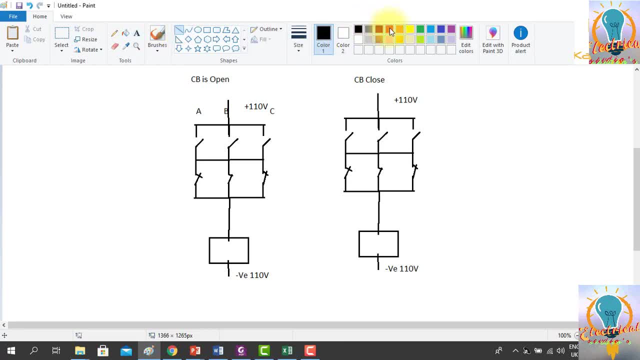 So what will happen here If this contact is closed? normally open contact will close like this. This will be closed also. So this will be closed, Also because these contacts are operated and this contacts will be open. So I will mark it here. 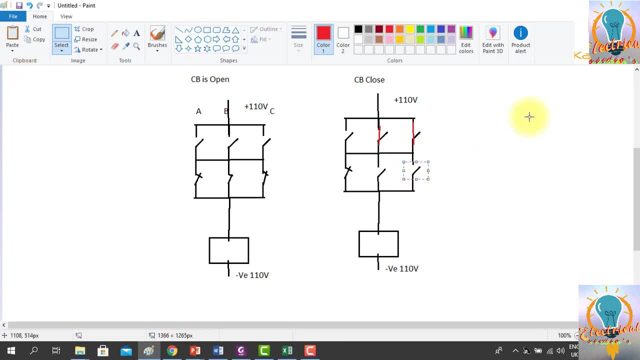 So this contact is open here. So now two poles are closed. Pole number B and C. This is B, This is C. Okay, Okay, Okay, Okay, this is A. so two poles are closed and this pole is stuck up. so you can see now that the DC supply. 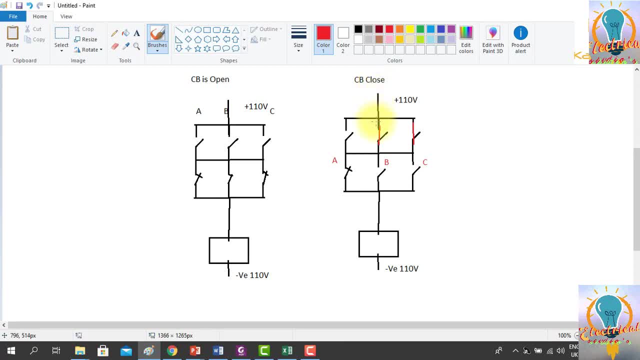 will be through. in this case, positive will come from the top and from here it will come to the common point. and because this pole is stuck up through its normally close contact, this timer pole discrepancy rate timer will start. so this is P D relay and stage one is hundred milliseconds. 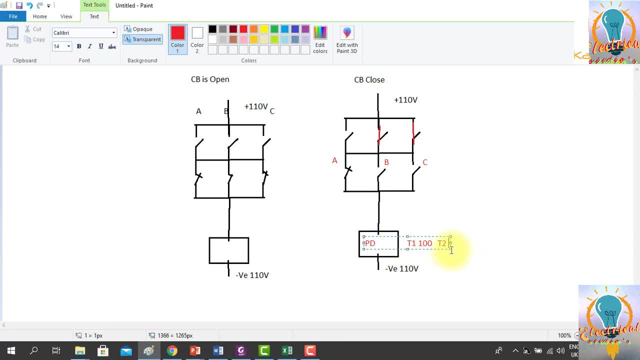 stage two is, for example, 200 milliseconds. so in stage one that time will start at hundred milliseconds- will try to re-trip the breaker. it will give tripping command to TC1 and TC2 to operate if it trips, okay. if it isn't trips, it will give tripping commands to breaker failure. 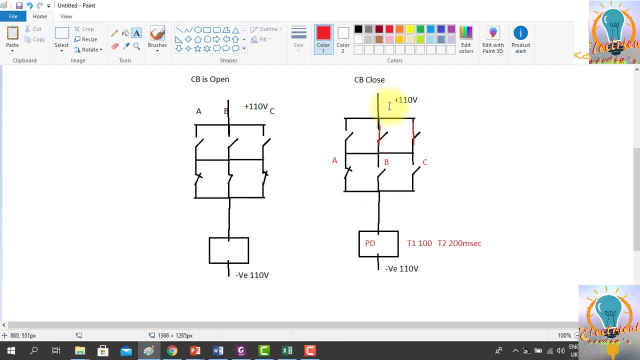 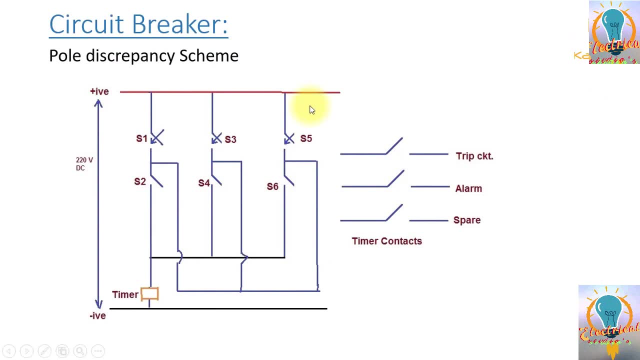 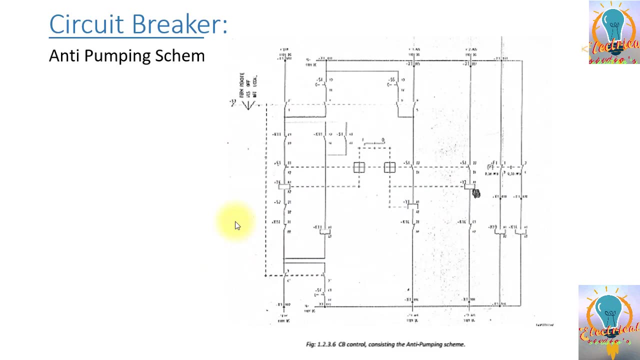 protection of it will initiate the breaker failure. protection of this specific breaker. so this is the example of how pole discrepancy relay operates. I hope you enjoy this section also. hi, friends, now I will give you some introduction about the anti-pumping relay and so basically what anti-pumping relay is doing. first of all, we will understand the pumping phenomena. 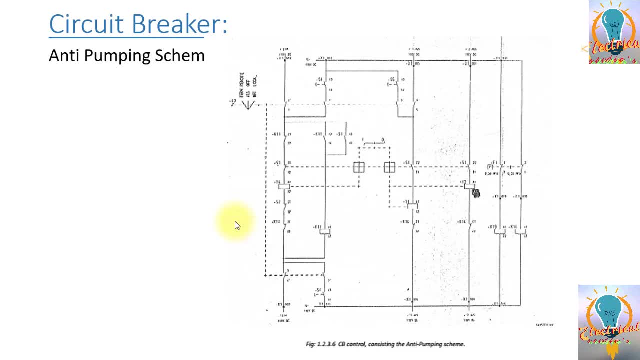 that could take place in the production system. the pumping phenomena is that. just consider operator. and if he, when he is trying to close the breaker, he will push the pole discrepancy switch and it will, for example, hold the switch on its position for one second or two seconds. 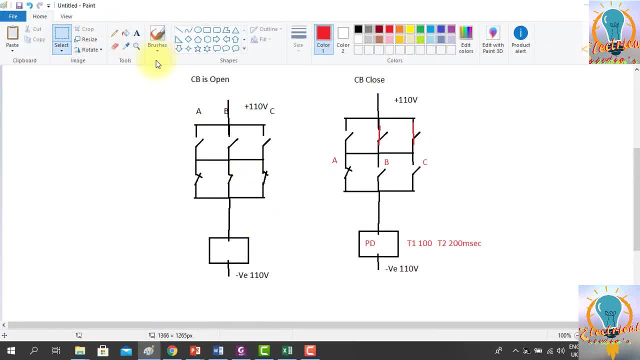 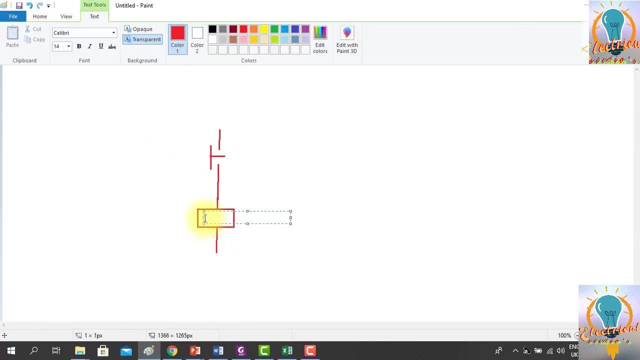 so let's draw this on this board. so let's draw this on this board. so let's draw this on this board so it will try to hold this switch. let's draw the circuit breaker closing coil, okay, and then we will draw basically a command. we will draw push button, we will try to make a pole discrepancy switch, okay, and this is the closing. 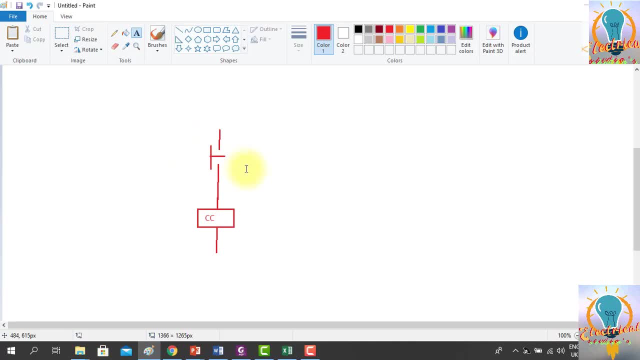 coil. so if operator is pushing this it will pass the supply to the closing coil and the closing coil the break will close. just suppose the operator is hand is still on the switch, because it will be at least one second or two seconds on the switch. it takes time and 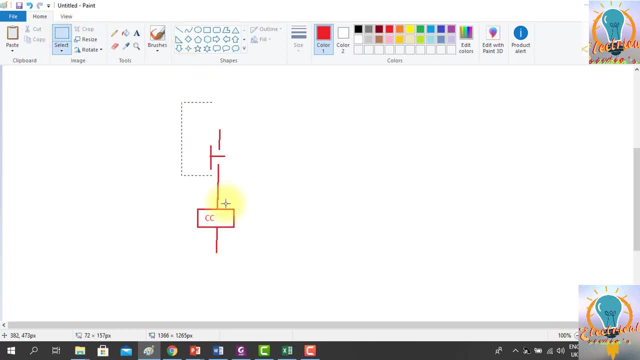 at the same time, fault is appearing on the system. so if fault is appeared on the system, then you can see the breaker will trip, but his hand is still on the switch. so what will happen? breaker will trip, for example, in 40 milliseconds, 45 milliseconds or you can. 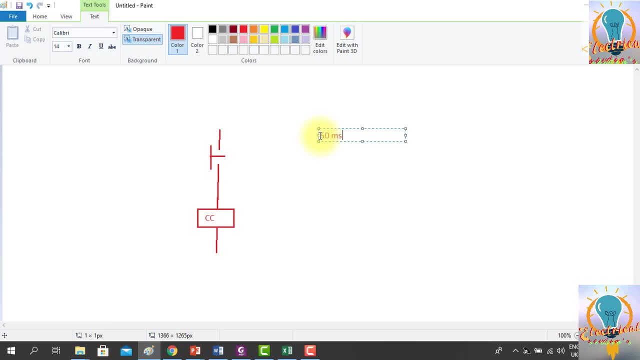 see 50 milliseconds so breaker will trip. but because the hand is still on the switch, switch is still pressed so the breaker will again close. so but fault is not clear, then again it will trip. so in in a second of time you can see if you divide certain by 50 milliseconds or if you divide even by 100 milliseconds. the 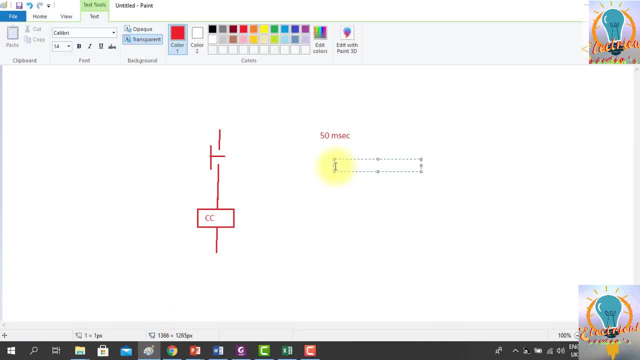 breaker will close 10 to 15 times in a second. if this situation happen, if you are closing to close the breaker, at the same time fault occurs. so this is called pumping action. so we need to avoid this action. so we need to avoid this pumping action. so we need to install a relay which should protect. 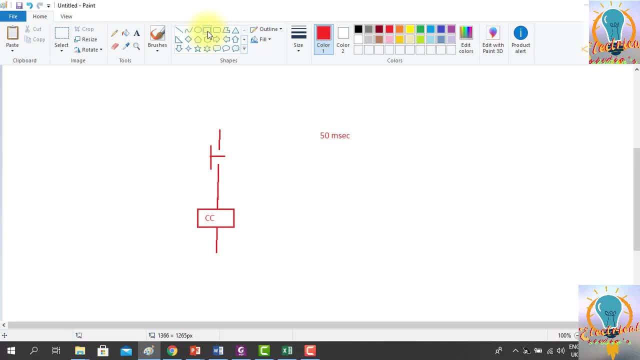 our system and it's called as an anti pumping relay. so how it works. basically, let's install another relay. this is the relay. okay, we can connect this relay with this switch, and one of these relays, or the relay here, are normally open contact, normally closed contact. 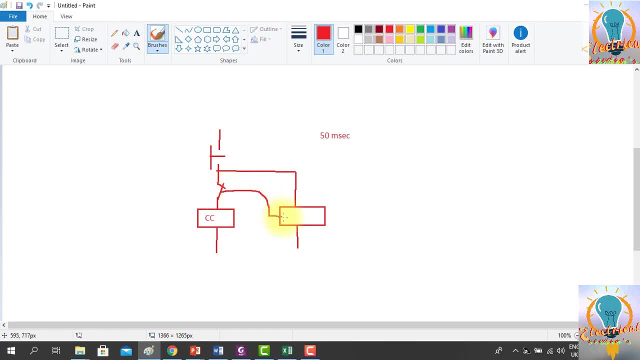 normally close contact of the relay is kept. this is the contact of. have put another relay which is called as an anti pumping relay. so when operator switch press the switch here, this contact will close. this anti pumping relay will energize and also closing command will be given to the 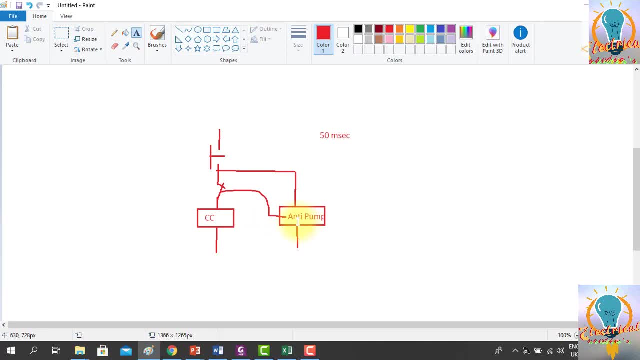 closing coil when this relay picked up. okay, so let's draw the seal in contact of the. really also we have to make the ceiling contact here if you take a solid positive supply. so here we have solid positive available. here we have diodes of electricity in relation to the diodes of liquid molto gas, and here here 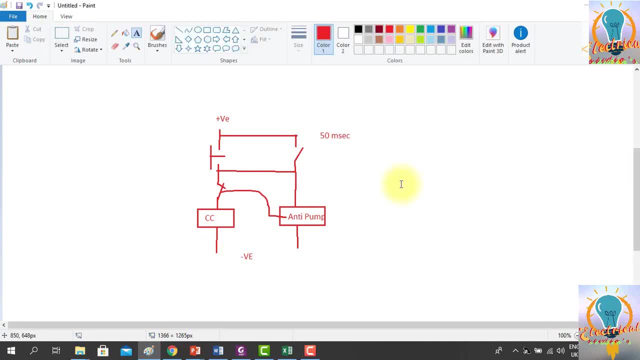 we have second phi, agriculture, high demand. so for these properties the negative available. so when operators push the switch, in this case anti pumping relay will energize and also close. command will be issued to the breaker. breaker will close, for example, as soon as the anti pumping relay. 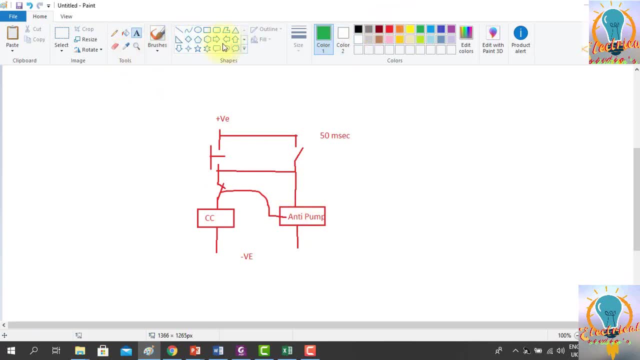 picked up. this contact will now move to close. so this contact will close. so this contact is closed. it means that this, the new position, will be like this: this contact will move on and this will be closed. now this contact is closed. so positive is available through this anti pumping relay. okay, so the hand is. 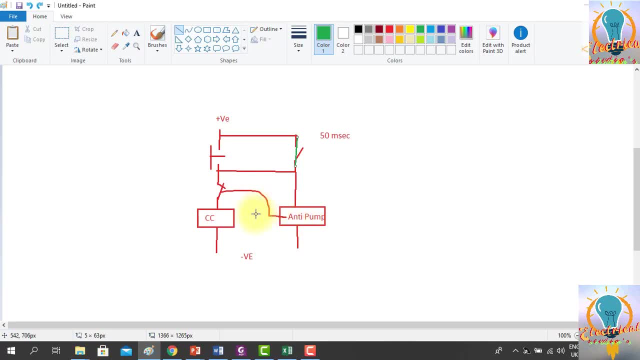 pressed and you can see when this relay is picked up, it will cut down the supply of the closing coil. this contact will now open because the relay is picked up. this is now closed contact and it will cut down the supply. so it's the operator hand is still is on. 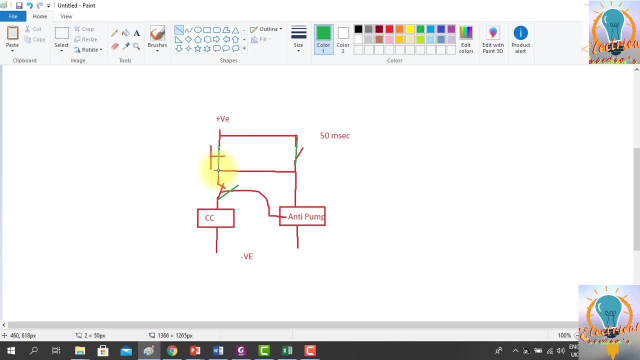 the switch here, for example. so only one pulse will go to closing coil and the anti pumping will cut this pulse and it will seal in through this contact and then, if the fault comes, breaker will open. if his hand is still on the contact, the next pulse will cannot be given and this anti-pumping relay will be reset. we 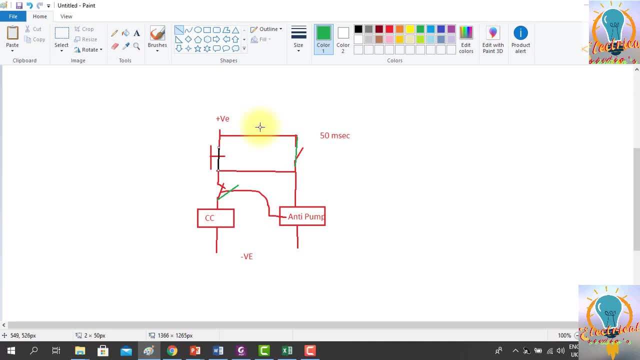 have to put another contact here by normally open contact of this switch. so when this switch and this switch is closed, this point is closed. when this person take off this switch, this is the auxiliary contact of this switch. so when the operator remove this switch, at that time is anti-pumping relay also reset and this contact is also closed. so this is some. 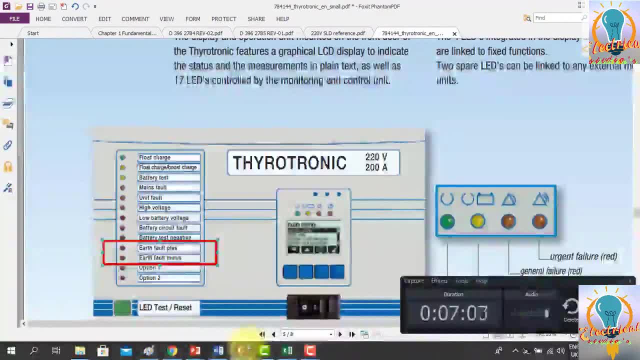 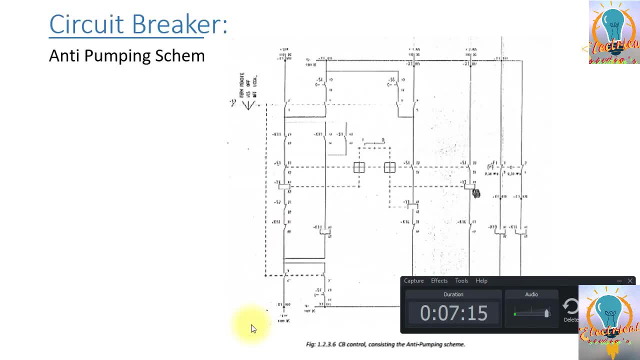 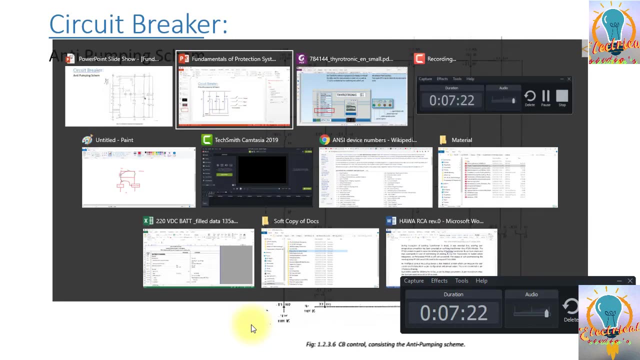 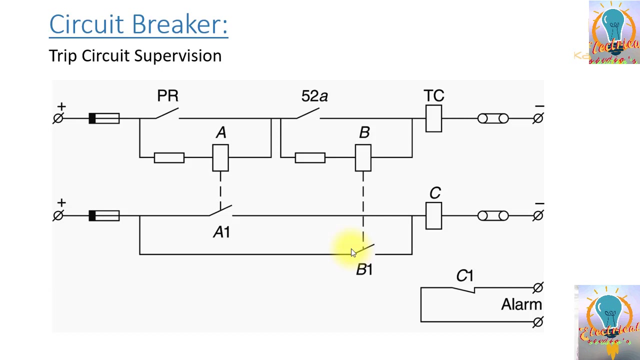 example of anti-pumping relay- how it's working. I have separate training on this, one introduction to protection design one and two that you can go through and understand more in detail. so I hope you enjoy this lecture. hi friends, now the new topic here is a trip circuit. 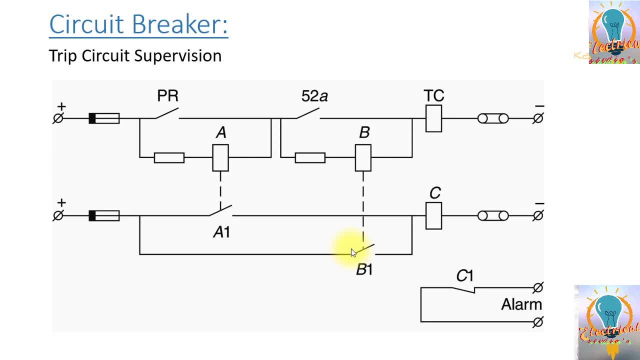 supervision relay and this basically tripping coil in of the circuit breaker is more fun of the most important device to monitor, because if the tripping coil of breakers is failed it means that Whenever the fault comes, everything is okay. but but a breaker cannot be tripped. 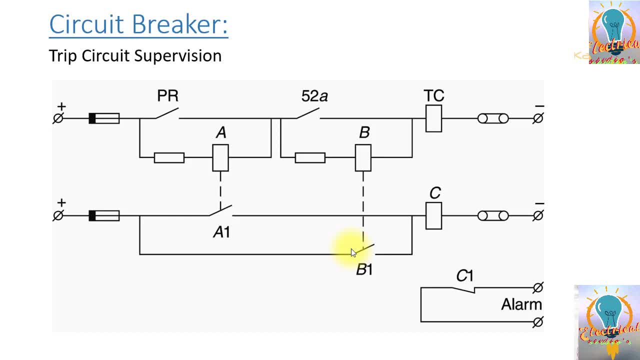 So that's why the need arise to monitor the healthiness of tripping coil all the time. So the healthiness tripping coil is monitored by a trip circuit supervision relay. Here you can see this is a tripping coil and this is a trip circuit supervision relay circuit. 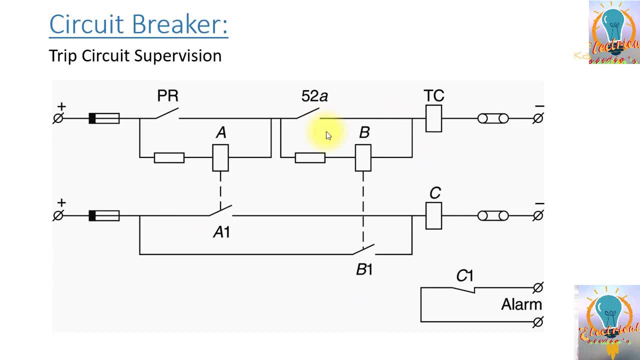 So how it operates basically is, for example, if the circuit breaker is in open position- So 52a is normally open contact- It will also will be open position So you can see the. the tripping coil will monitor. negative will pass through the tripping coil. 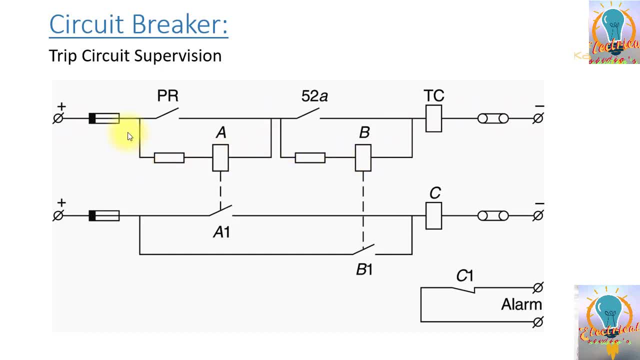 through B and through A and to the positive. so in this way, you can see, the both coil will be picked up and it will show that the system is healthy. So, But in case, for example- and this is basically the You can see here- is this is the contactor, So when both are, 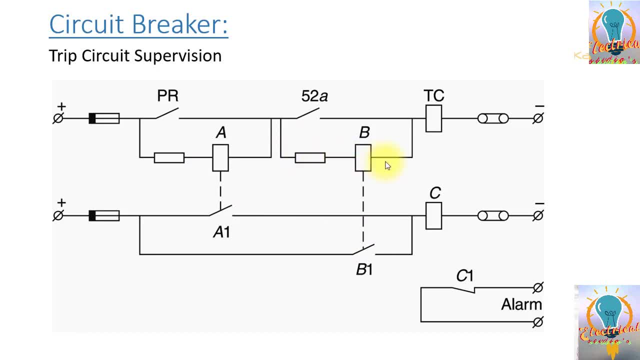 in the, in the case when the breaker is open so we can monitor the tripping coil, both coils will pick up, even close, and even will be closed and C will picked up. and this is the normal close contact of the Basically this contactor. so Then C is picked up, This will be open and there will be no alarm. 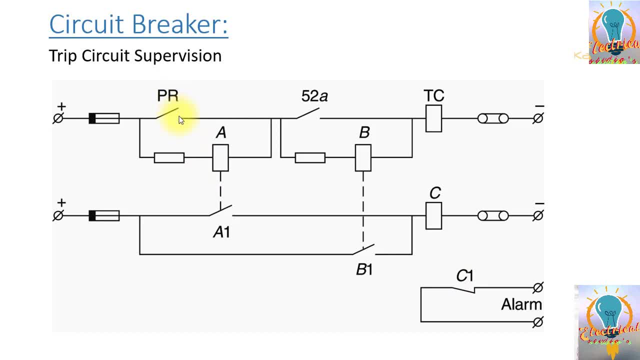 so here you can see if somebody is issuing the. You can see protection delay is operating and it is issuing the trip command. Is it, for example, now the breaker is closed? So if the breaker is closed, you can see, 52a will be closed. So the tripping will be monitored by a tripping coil. this coil B will be bypassed. 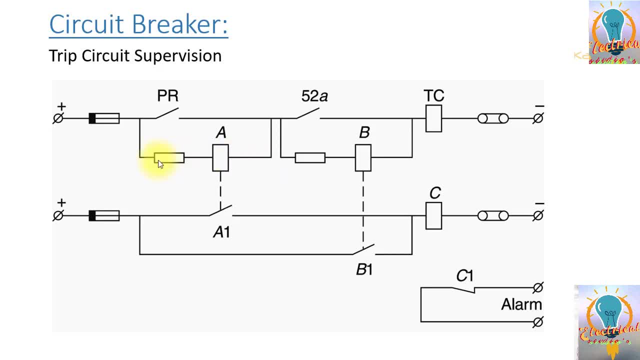 so through 52a it will come to A and then It will be monitored by coil a. so coil a will pick up and it will energize C and alarm will not be initiated. so in case, if there is a Failure of the wire or failure of the coil, coil becomes open. There is no written negative and 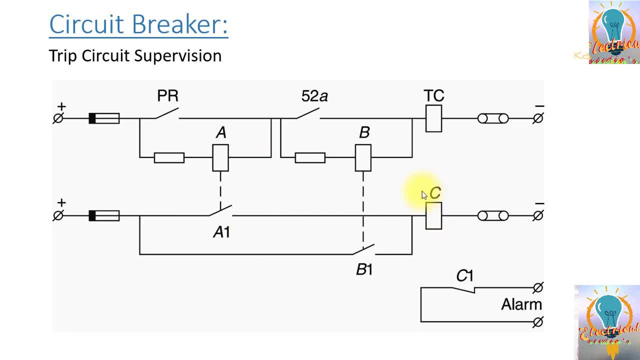 The A and B will be reset, So the C will be de-energized and then you can see the alarm will be initiated, because it's normally close contact. so there is another case for just just a Information, that if, for example, if the breaker is closed, then you can see 52a. 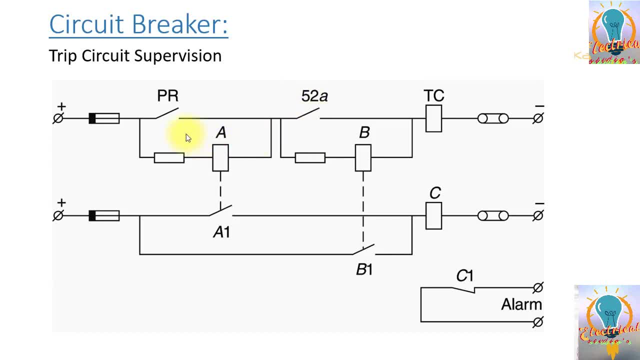 contact will be closed and At the same time, if somebody, protection really operates. so you can see at that stage B and E, both are getting bypassed. So in order to cover this time, because stripping pulse is approximately 100 to 120 millisecond at max, breaker is opening in within. 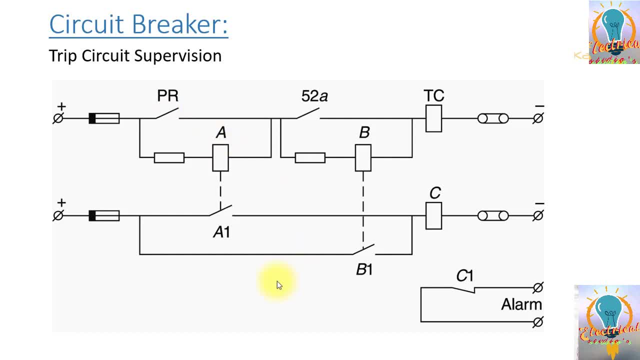 a time of 50 to 60 milliseconds at max. So basically, a timer is installed and if this timer will Hold and keep on energizing the conductor for the given period of time, so that during this time protection should not Operate and give alarm unnecessarily. So this was some introduction about the tape circuit supervision. 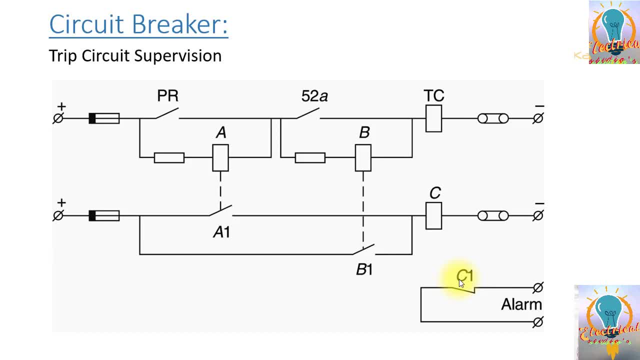 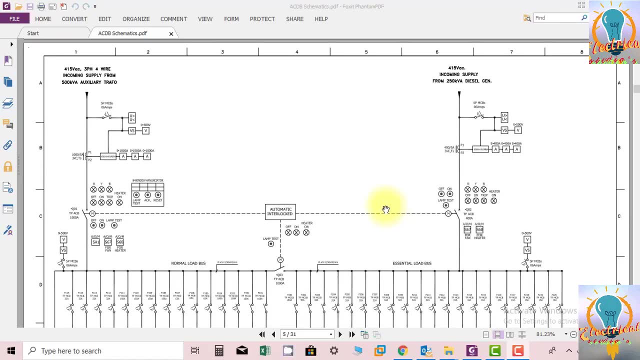 if you are more interested to Join about the drawings, You can check my other available trainings and you can start your learning. You guys, welcome in this section. we will study With single line diagram for the ac distribution board. So this will give you the idea How the ACDB works and then later- not- we will start. 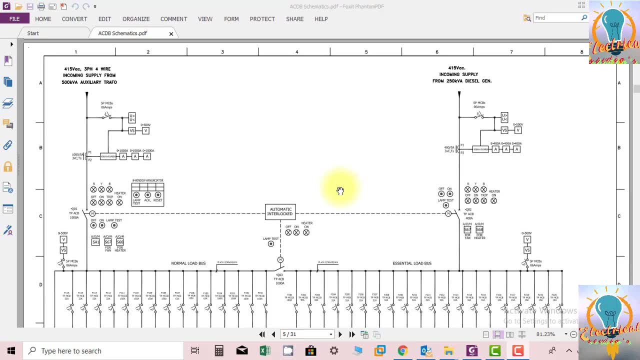 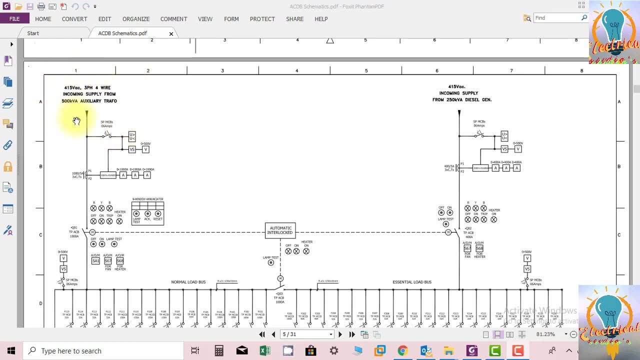 Detail drawing for is distribution road. So just for your knowledge, you can see here that at any substation there are two sources are provided for AC power. one source is filled through auxiliary transformer in the substation, which could be 11 TV by 415 volts, and another source is, for example, if the supply is the supply of substitution is failed. 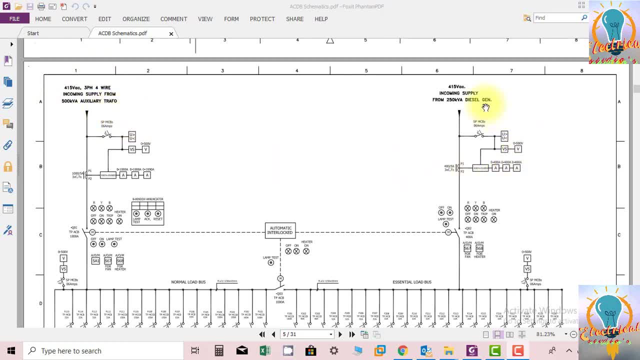 that in that case the backup could be provided through generator. in our case- you can see, here it is- these are generator 250 TV, so these are called as incoming supplies or incoming supplies. as incoming supply, that means that we are providing backup from generator to hin Pasteur. 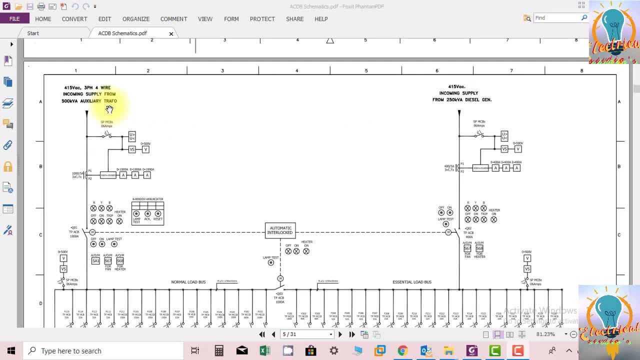 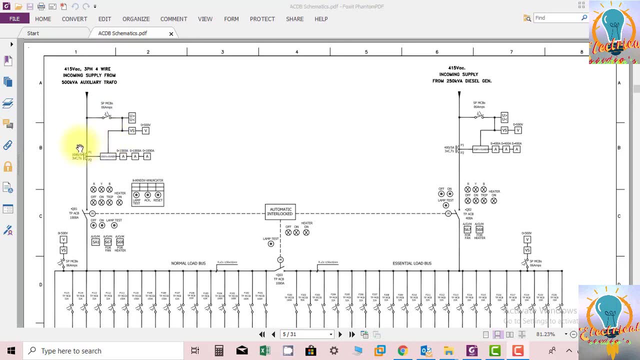 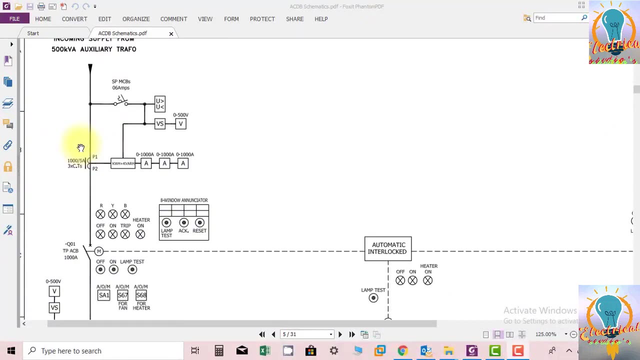 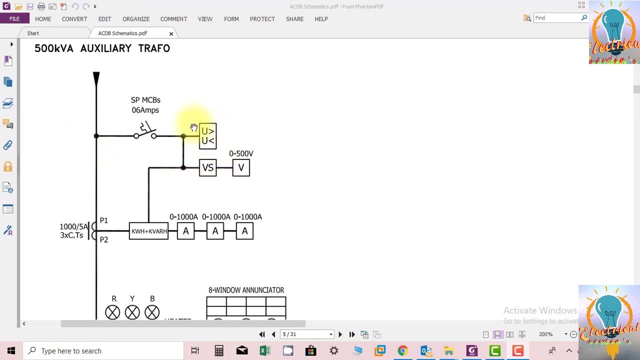 feeder for the AC distribution systems. so here you can see. if you go further, I will start with first incoming from the auxiliary transformer. so first we will familiarize with the symbols. so here you can see. they have installed here a relay that is over voltage, and under voltage it means the relay will monitor that is. 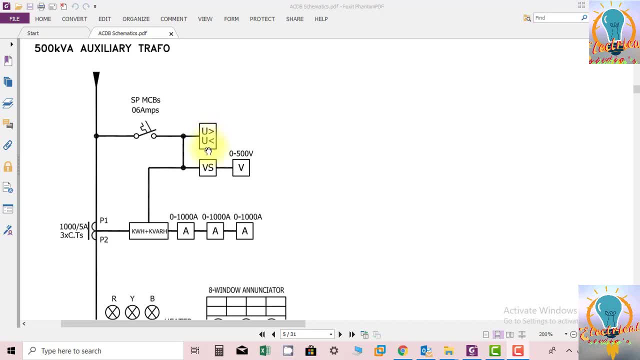 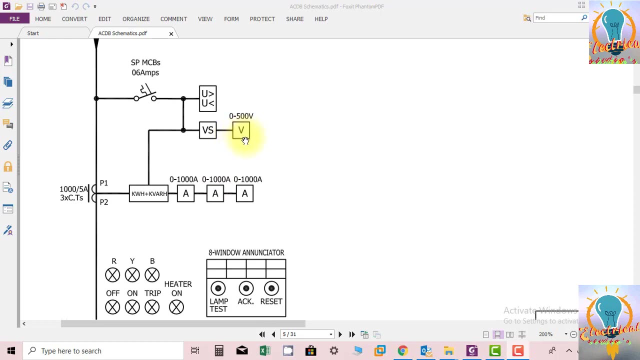 there any over voltage or under voltage and that accordingly, it can trip the breaker as per the required settings. this is the MCV, which is protecting any short circuit happen here. okay, and these are the basically voltmeter which is connected and this voltmeter is showing supply. 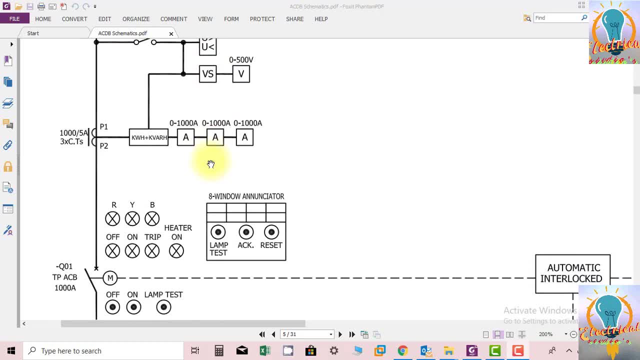 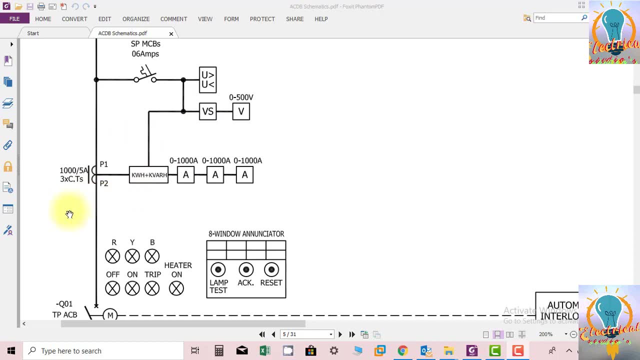 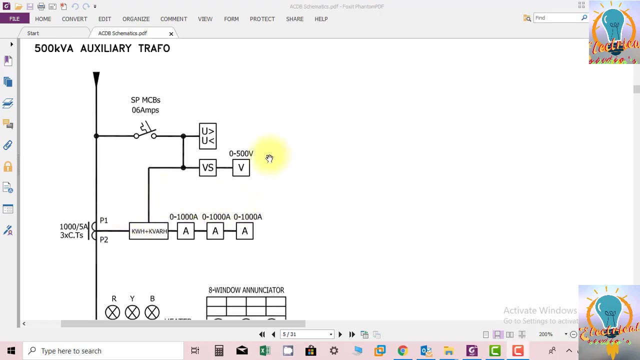 of the AC distribution system. so this is the supply of the AC distribution system which is coming from in from the auxiliary transformer. it means this supply will be available in the cable box at the cable side or yard side. so once the auxiliary is energized you can see the voltages on the voltmeter here. 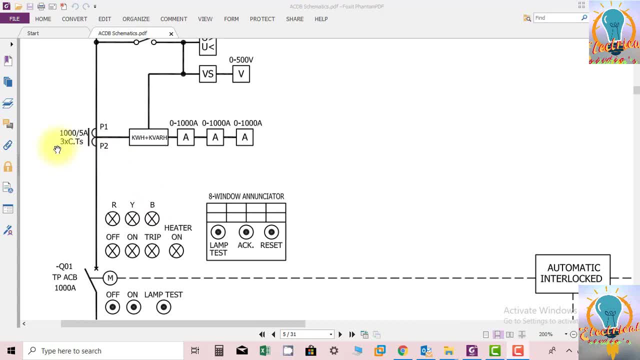 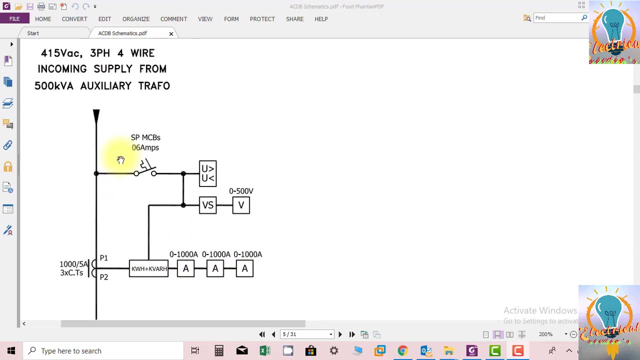 okay, then they have shown here a CT which ratio is 1000 by 500 amperes. so the CT is feeding meter, energy meter which is measuring twh and karh, and then three ammeters are connected. so this is the symbols of single-another. 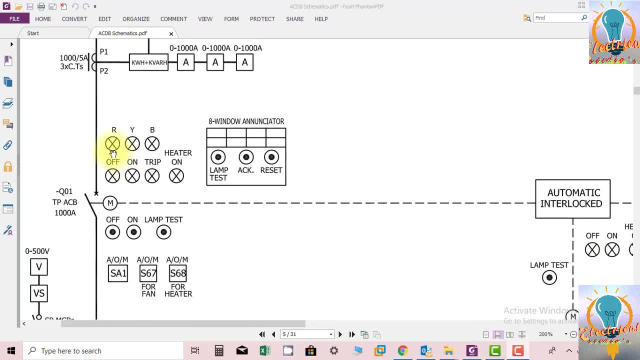 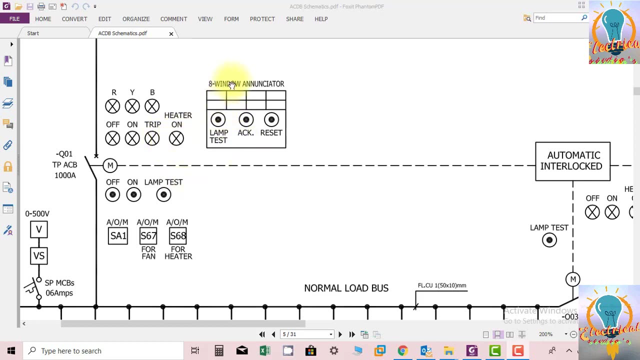 diagrams. then they have connected 3 LEDs each for one phase- red, yellow and blue- and and then they have heater on indication. they have shown here also on unseater where you have option of lamp test. when you press, all lamp will glow. that will make sure that lamps are healthy and 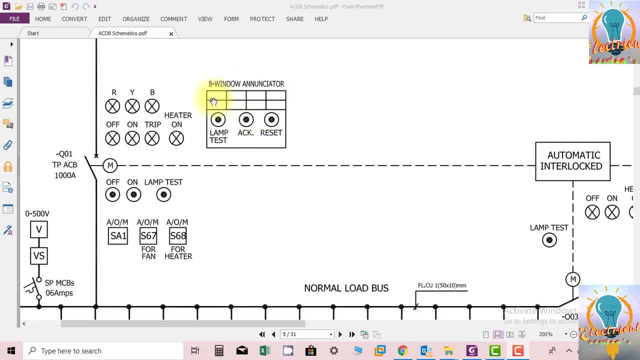 when some indication appear, the lamp will glow and it will blink, flicker and there is a hooter in the substation and this hooter will will be on, so there will. it will be a loud noise so you can when press acknowledge this hooter will be off and blinking will be still, so you can see. 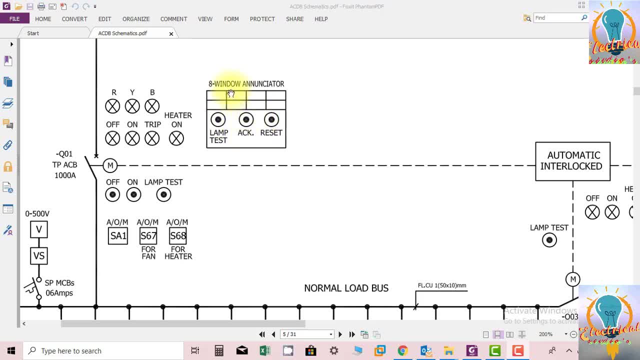 the indications here. so if indication is attended when you press the reset button it will go automatically off, but if indication still persist after pressing the reset button, it will not reset. this is the main incomer breaker of incoming one which is not named as q01, rated at 1000 ampere, and this is motor operated and this line is showing that it is interlocked. 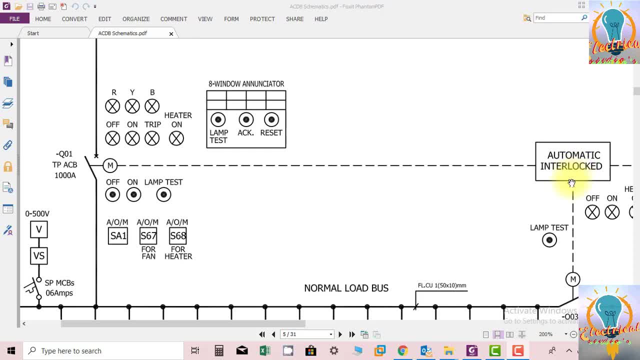 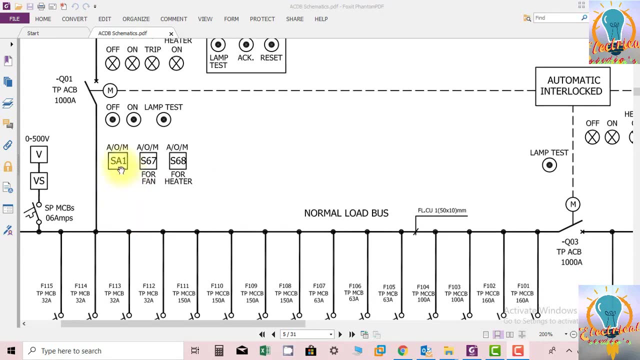 so later we will see the interlocking diagram and also we will see the interlocking circuitry, how it is made possible. here you can see the switches are provided. these are selected switches. you can put this uh encumber in automatic off or manual position means if you keep it automatic. 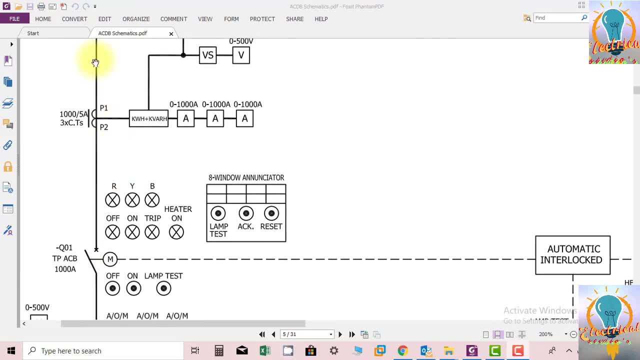 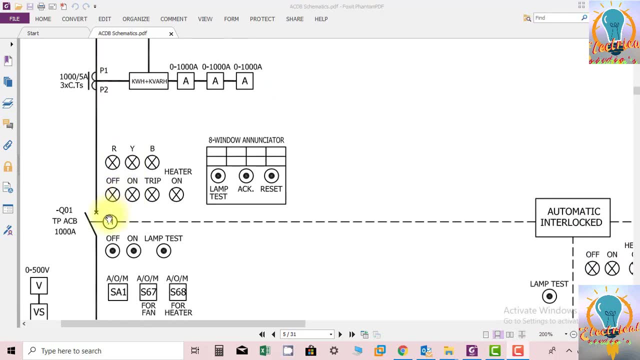 what will happen. as soon as there is a supply at the income site, at the yard side, at the cable side, this relay will sense and automatically this will switch on the breaker. so this is automatic option. when you keep it off, the breaker will become tripped, and when you make it. 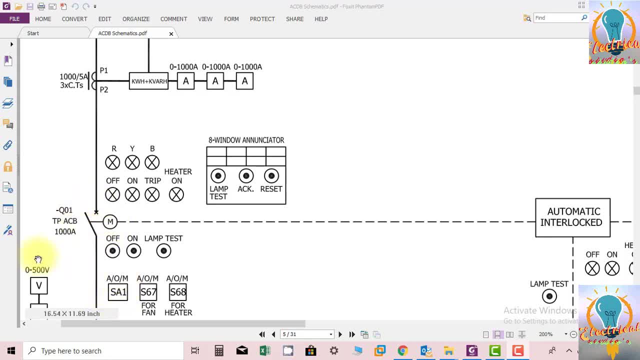 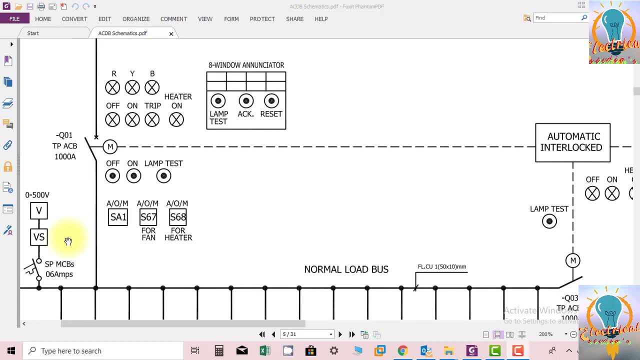 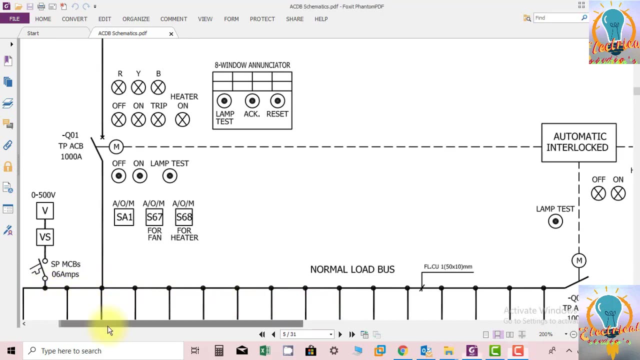 your house will become fit, and when you make it manual, then you can manually switch on and off this breaker. this will not update through interlocking or any automatic operations. so then when you close this breaker, the power is feeded to this bus and you can see, at this bus they have connected a voltmeter and this is voltage selection vs. 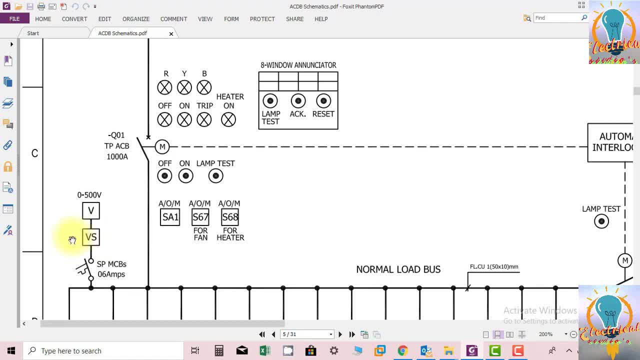 for each phase can select. for example, in the practically: if you want to see red phase voltages, you can put the selector on red, and if you want to see yellow phase voltages, you can put the selector on yellow. similarly, you can also see blue phase. this is the mcb, which is protecting any short circuit. 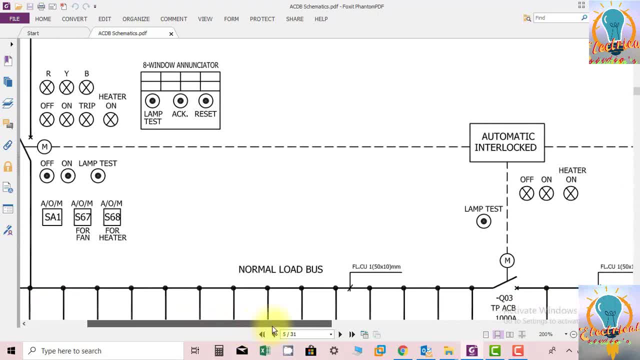 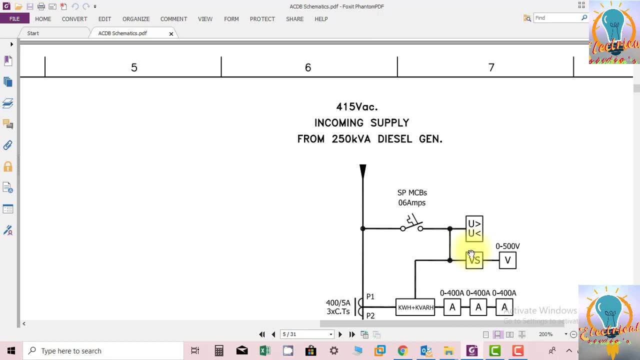 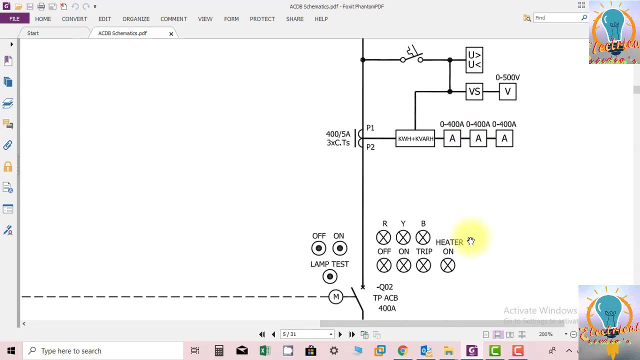 in this circuit. so this is basically the incomer side. now we will see the signal and diagram for the diesel generator side. diesel generator side. the signal and diagram is same as i explained. you can do self study here. it is the same as the incomer one. 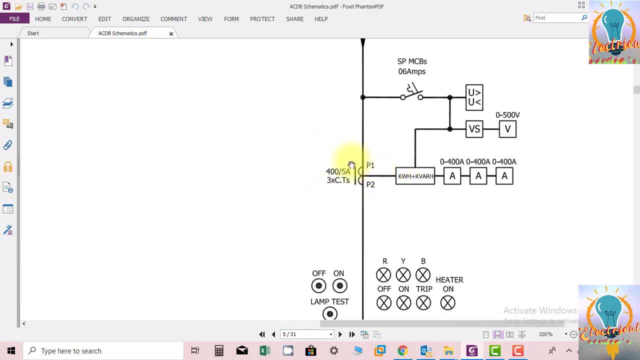 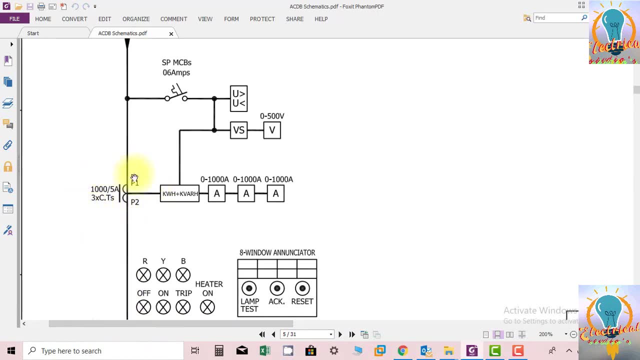 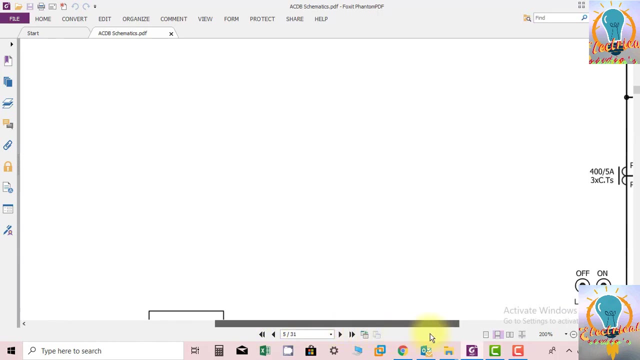 the difference here is they have utilized a small ct ratio is five, four hundred by five, whereas the main incoming one through all the transformer, digitalizing thousand by five ampere ct. the reason is that the generator, which is called as an emergency generator, don't have the capacity to supply a full substation, so that's why its rating is. 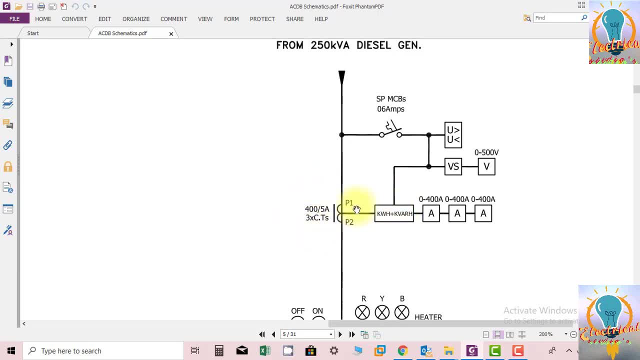 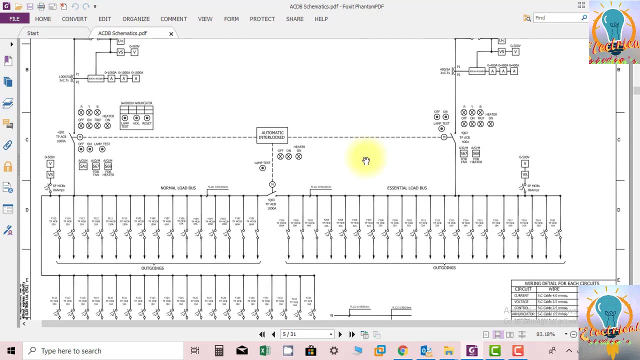 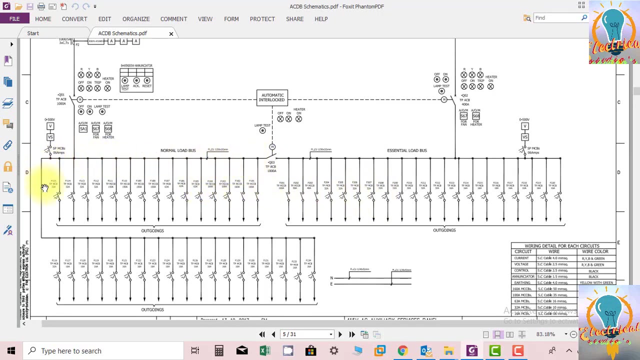 less, and this ratio is also is less ct ratio. the ct ratio is selected as per the load current. so now we will see the bus bar arrangements. so here you can see the bus bar is divided in two parts. the path one is normal load bus, you can see. 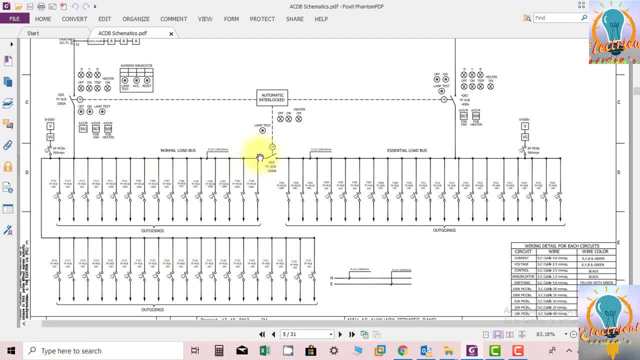 from here up to this point is a normal load bus, and then there is a tie breaker which is qgo3, and then there is an ssd s. in this case this is a direct transition load bus. so in a normal, when the station is normal and 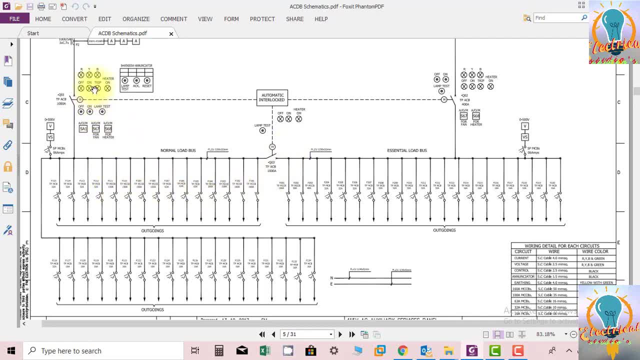 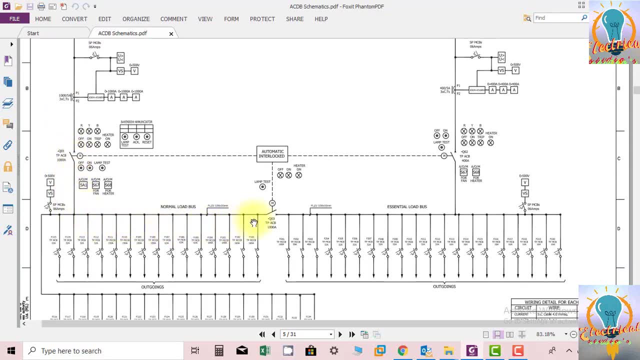 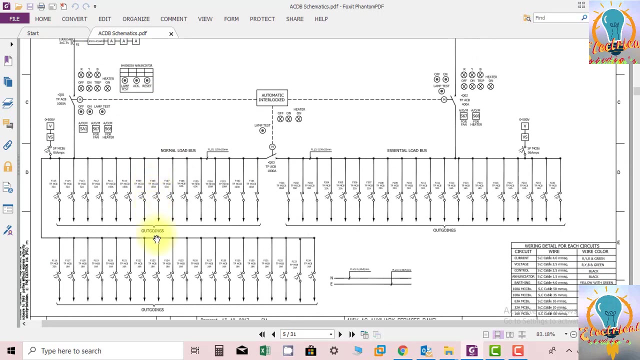 supply is fit through auxiliary transformer. in that case, if you keep the system automatic, the power will be feed by auxiliary transformer from here and then it will be feed to normal bus and this tie breaker will be remain closed automatically. it will be closed. it means normal condition. the auxiliary transformer will supply voltages or load. 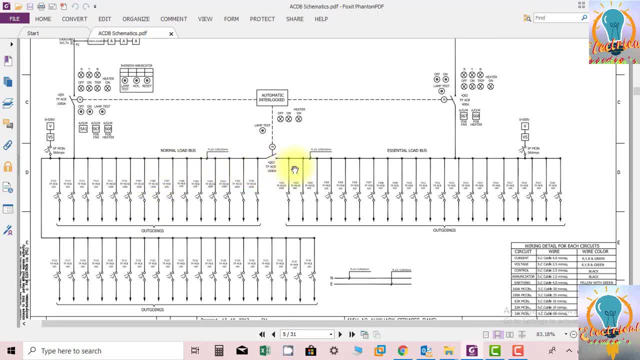 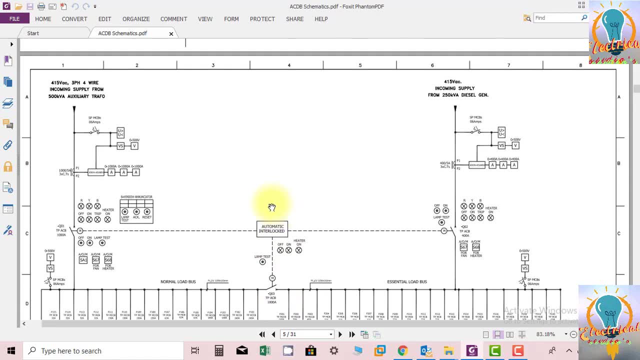 current to normal bus and as well as on essential bus. but in in in case, if incoming transformer, incoming feeder trips or this substation blackout or the feeder of the transformer trips, in that case there will be no supply here. the under voltage relay will trip this breaker and the coupler also will trip. 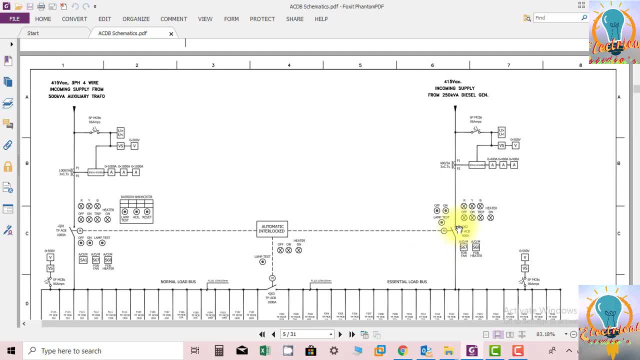 and after a few seconds to after few seconds it be one minute or two minutes, depending on the set, our setting. we have one minute settings. after one minute the generator will. this breaker will close and the supply will be fed through the generator. but it will not feed all both buses- normal bus or essential bus- but it will feed. 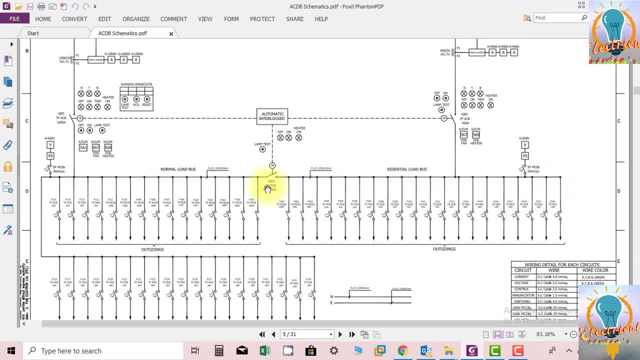 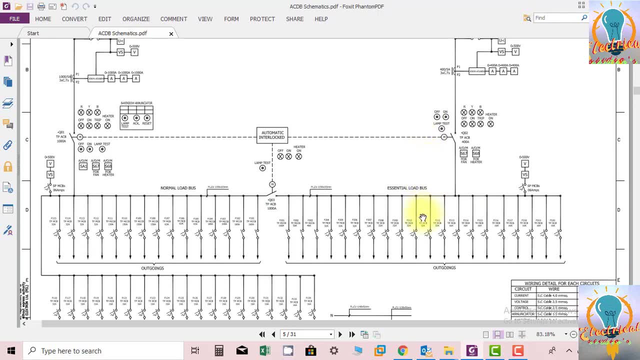 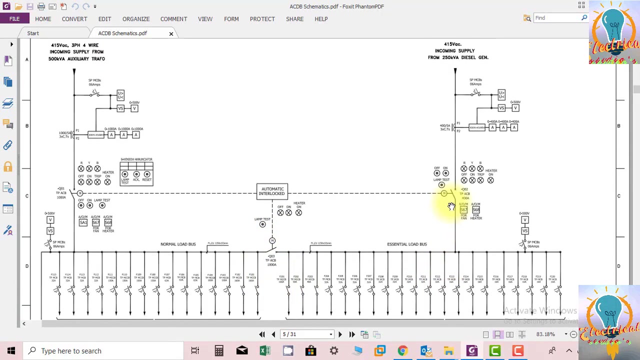 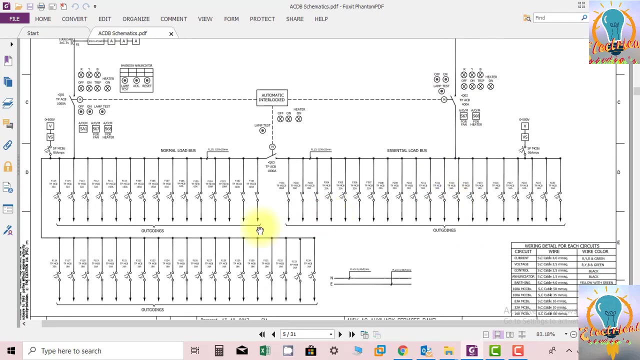 only the essential loads connected to essential bus because the generator cannot take the load of full substation. but if this generator have enough capacity to take the full load, so scheme could be modified to connect this breaker. even when the supply is fed through social line, this are generated so we- this is all about the single and diagram. 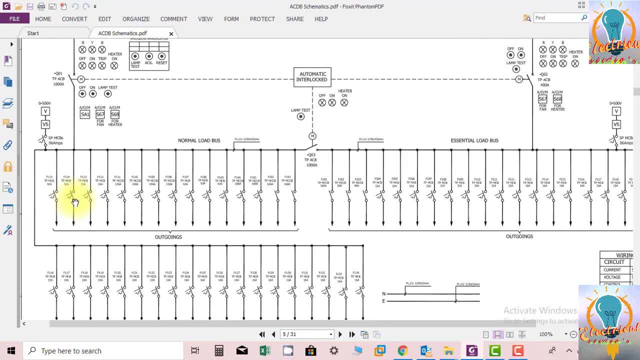 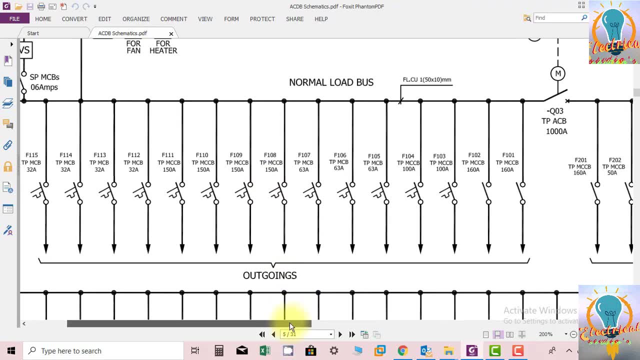 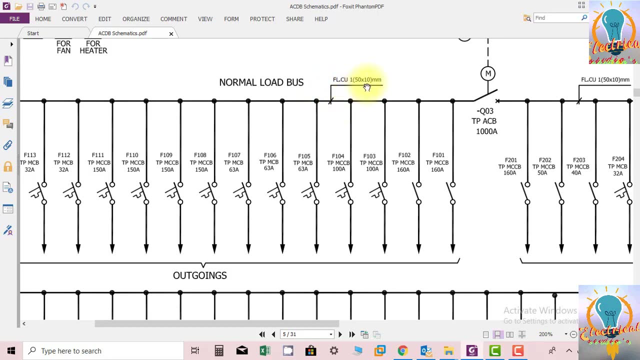 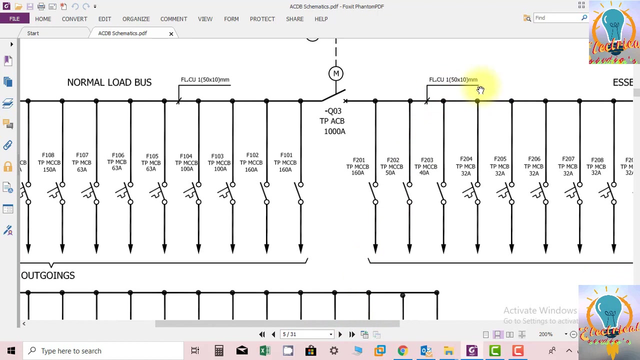 these are. you can see the outgoing mcb's. each is rated at 150 ampere. you can see the rating. the size of copper of the main bus is fifty by ten mm the current width into length. so again, this is the size of the main bus and you can see the outgoing.